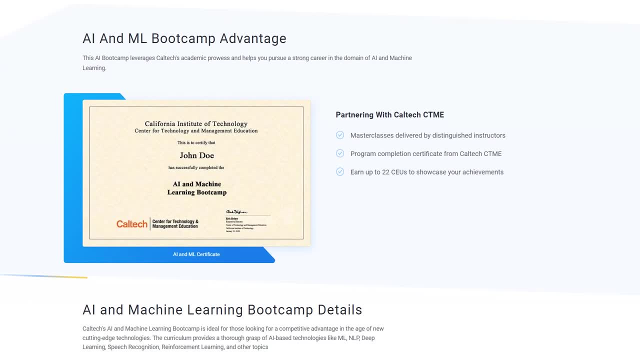 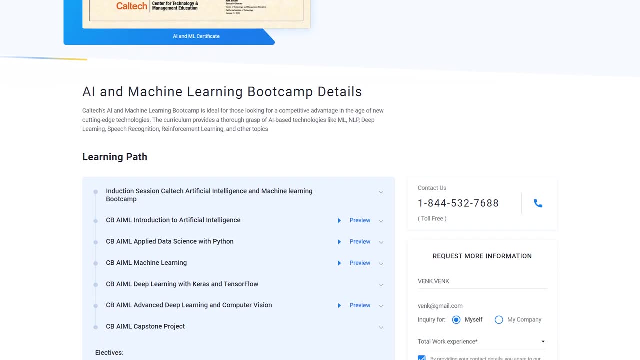 What sets our bootcamp apart is our partnership with Caltech CDME, ensuring academic excellence and industry recognition. We hope you will find this video helpful and we hope you will learn a lot from it. By successfully completing the bootcamp, you will earn a prestigious certificate and up. 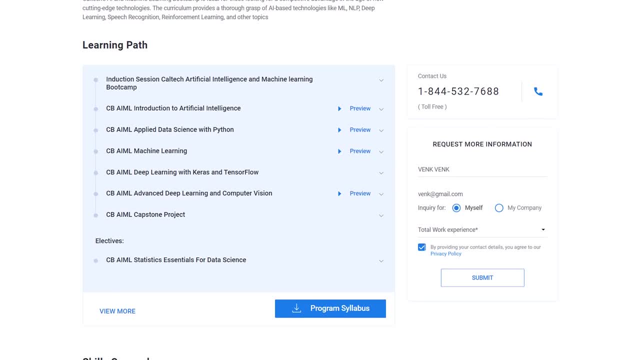 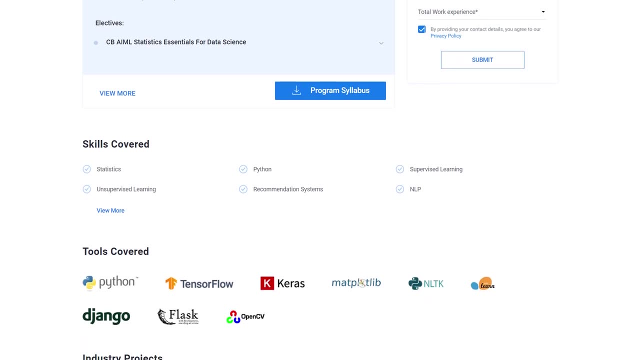 to 22 CEU credits from Caltech CDME, validating your expertise in the field. So are you ready to embark on this transformative journey? Are you ready to unlock the power of AI and take your career to new heights? If so, enroll in our AI Bootcamp today and 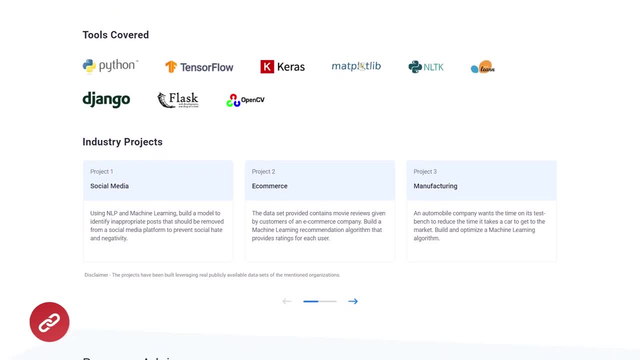 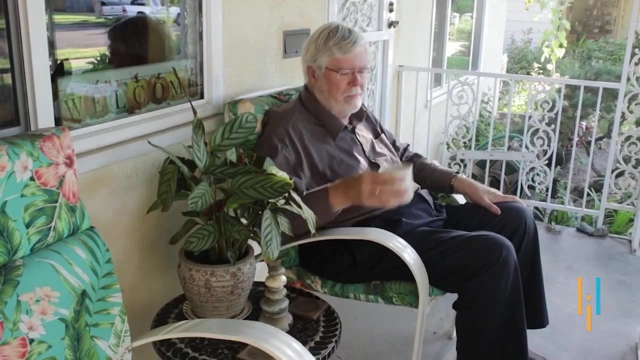 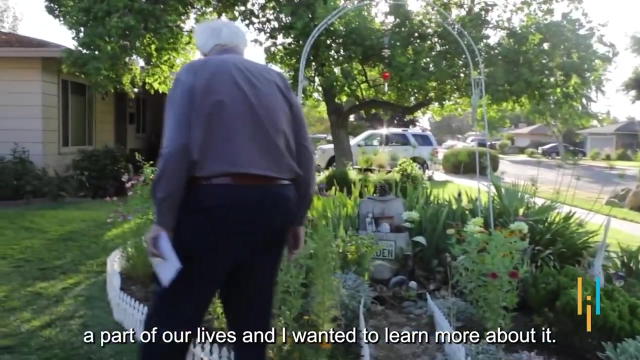 become part of the AI revolution. The course link is mentioned in the description box below, But before we begin, let's check out what one of our learners has to say about our courses. Artificial Intelligence has already become a part of our lives and I wanted to learn. 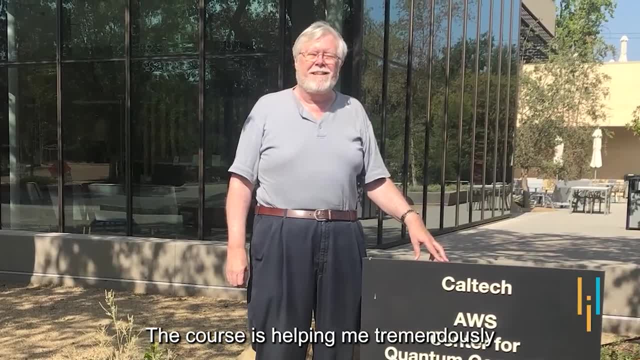 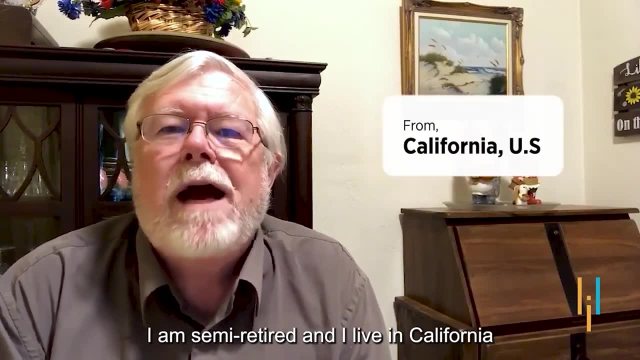 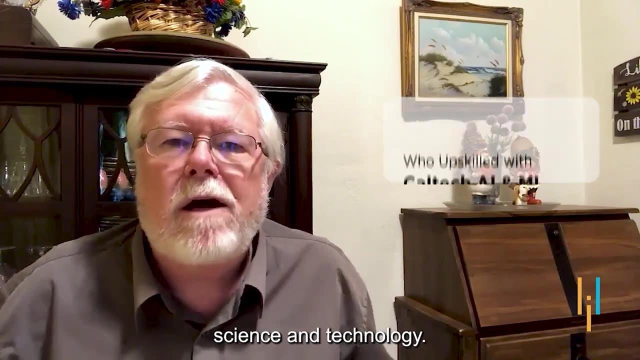 more about it. The course is helping me tremendously in my upskilling journey. Hi, I'm Daniel Dick. I'm 66 years old and I'm semi-retired and live in California with my wife and son. Since childhood, I've had a strong interest in science and technology. I was fascinated by the way systems worked internally and I've been interested in the way systems work internally. Since childhood I've had a strong interest in science and technology. I was fascinated by the way systems worked internally. I was fascinated by the way systems 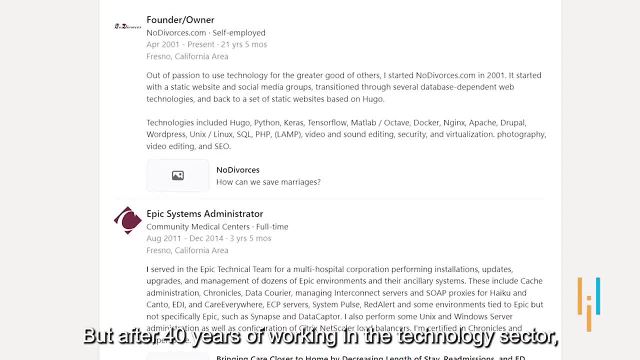 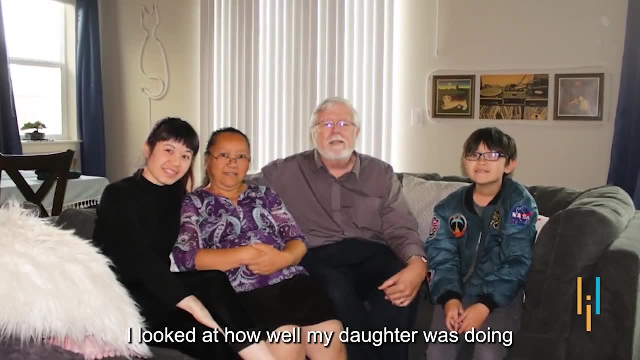 work internally and how algorithms performed. But after 40 years of working in the technology sector I could no longer work. It hit me hard. I looked at how well my daughter was doing as a software engineer. My daughter became my inspiration to upskill And over 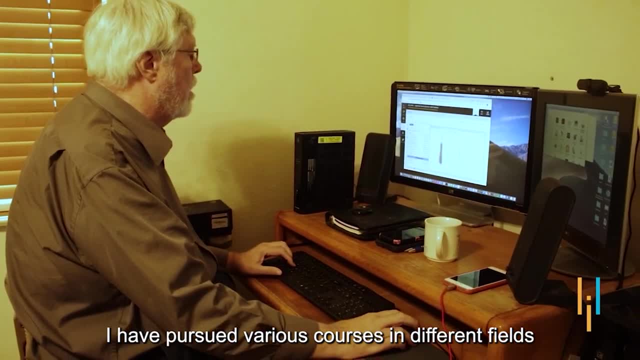 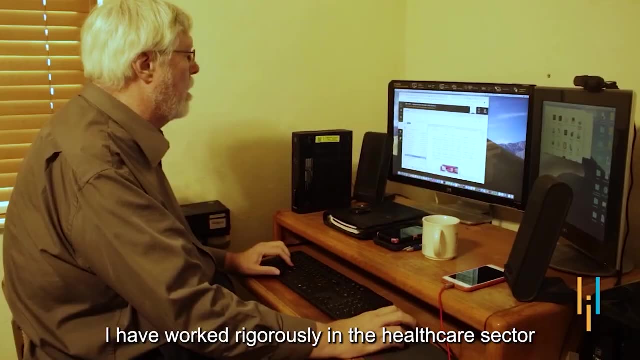 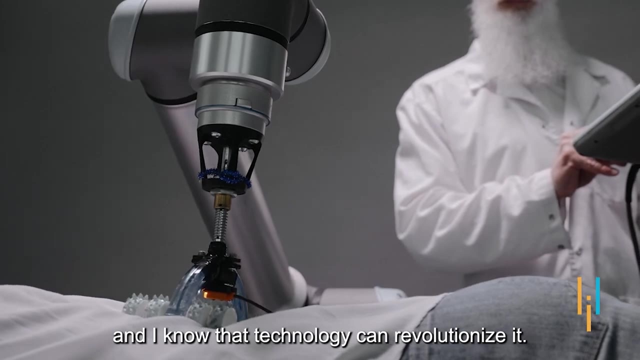 the years I pursued various courses in different fields of computer science. I realized that technology has the power to change the world. I worked rigorously in the healthcare sector. I worked rigorously in the healthcare sector as a technocrat And I know technology can. 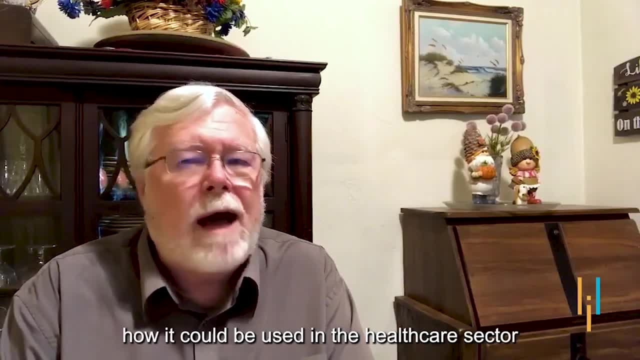 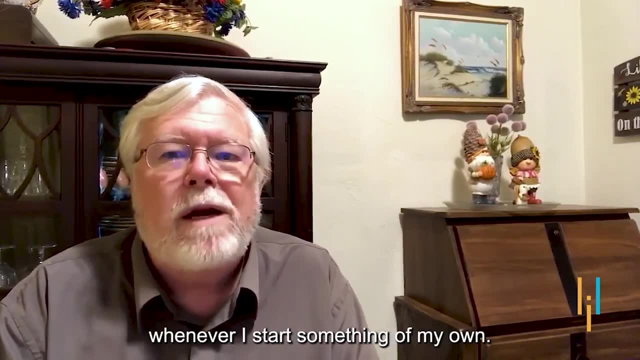 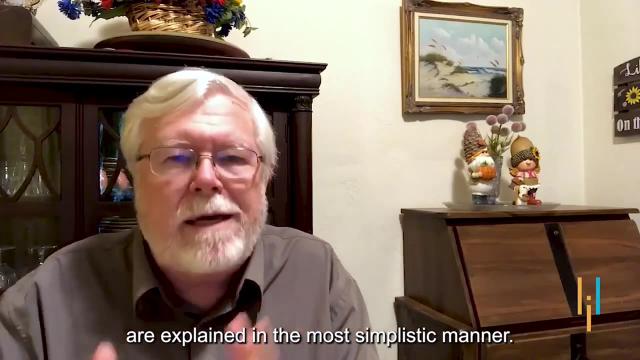 revolutionize it. I wanted to know how it could be used in the healthcare sector and other sectors so I could contribute to those domains whenever I start something of my own. The course is practical. All the minute details and concepts are explained in the most simplistic. 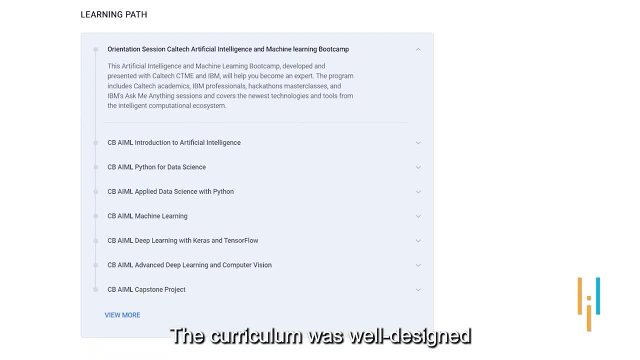 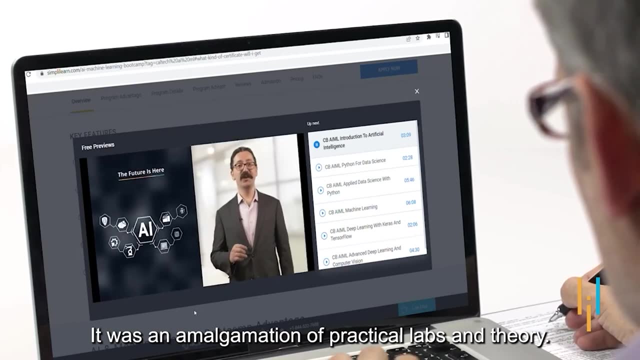 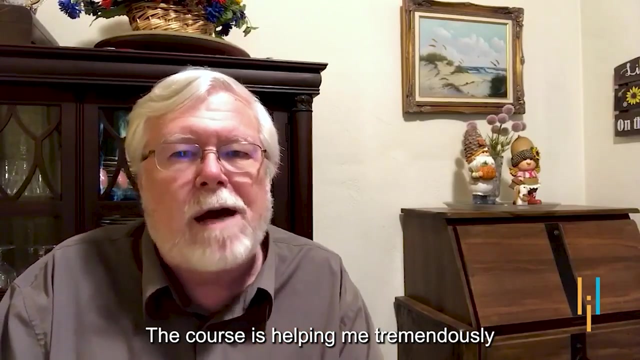 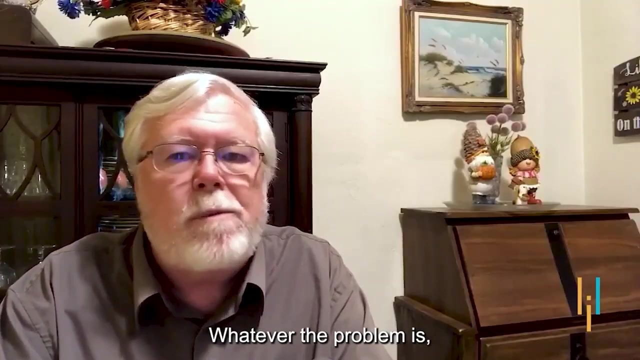 manner. The curriculum was well-designed, considering learners from different backgrounds. It was an amalgamation of practical labs and theory. The program focuses on building a problem-solving attitude in learners. The course is helping me tremendously in my upskilling journey in solving real-life problems. Whatever the problem is, you can either solve it or 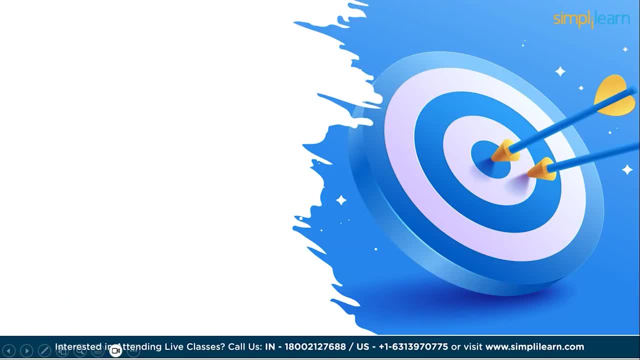 learn to solve it by upskilling yourself. And now we will have a look on the agenda for our AI basics tutorial, starting with what is Artificial Intelligence. Then we will have an overview of the AI roadmap for 2023.. Then we will have an explanation of different types of artificial intelligence. 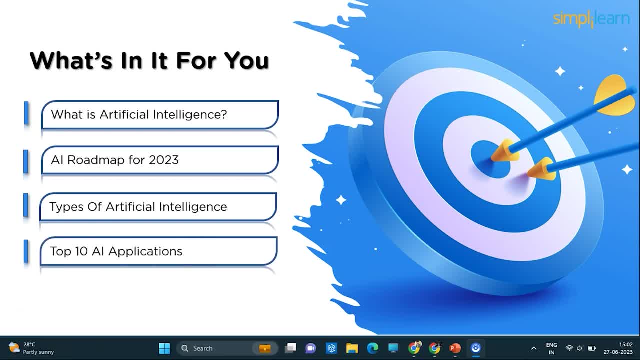 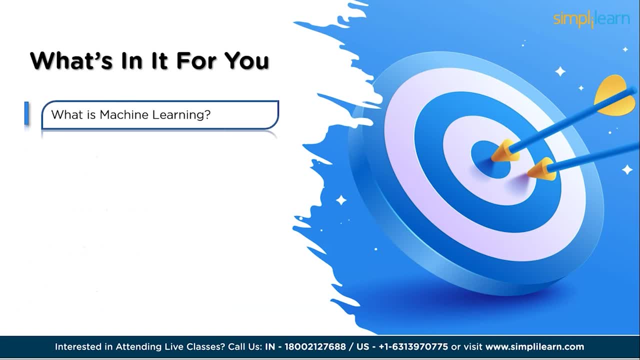 Then we will showcase the top ten AI applications, And after this we will see the future of Artificial Intelligence, And after that we will have exploration of Machine Learning, starting with Introduction to Machine Learning, Then overview of different types of Machine Learning. 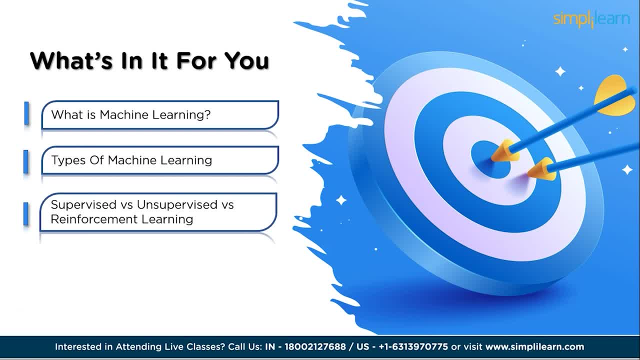 Then we will have comparison of supervised, unsupervised and reinforcement learning, And after that we will deep dive into Linear Regression analysis and its application in R. and then we'll have introduction to logistic regression and its implementation in Python, and then we have comparison of 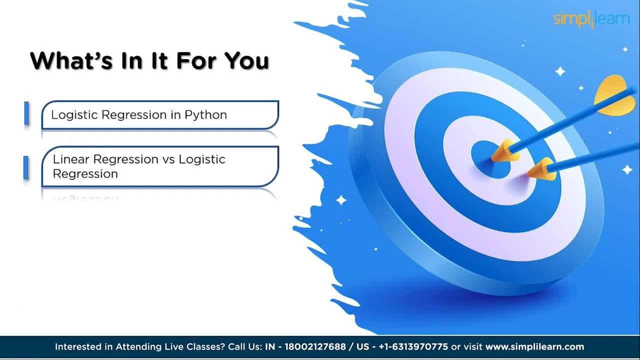 linear regression and logistic regression, and then we'll see machine learning techniques and tools, starting with classification in machine learning. then we'll explore decision tree in machine learning and then we'll showcase the top 10 AI tools for 2023 and after that we'll highlight the top 10 AI. 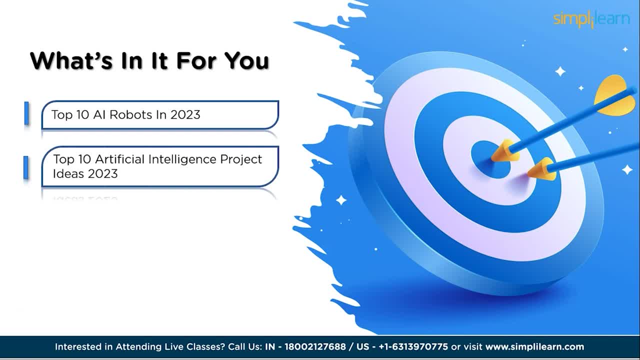 robots in 2023, and after that we'll present exciting artificial intelligence project ideas for 2023, and after this we'll have an introduction to the top 10 AI companies for 2023 and the discussion on the career opportunities in artificial intelligence for 2023. it's a weekend and John decided to watch the 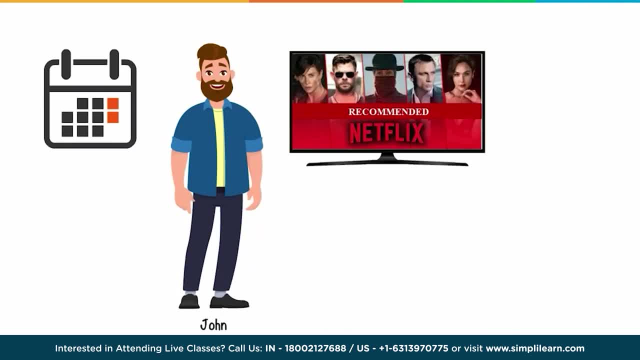 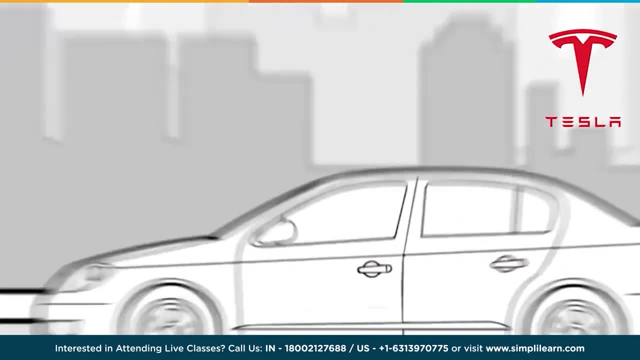 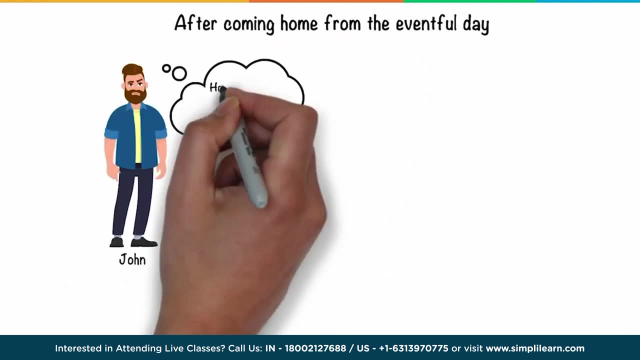 latest movie recommended by Netflix at his friend's place. before heading out, he asked Siri about the weather and realized it would rain. so he decided to take his Tesla for the long journey and switched to autopilot on the highway. after coming home from the eventful day, he started wondering how technology has. 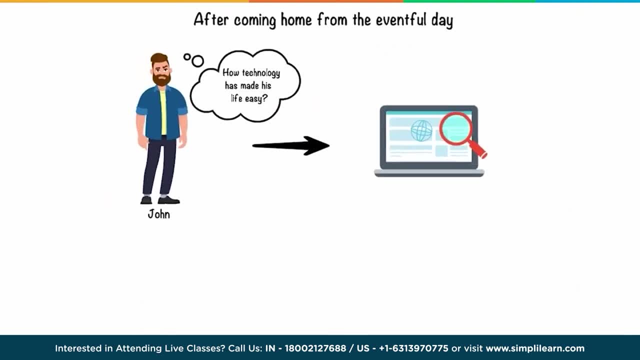 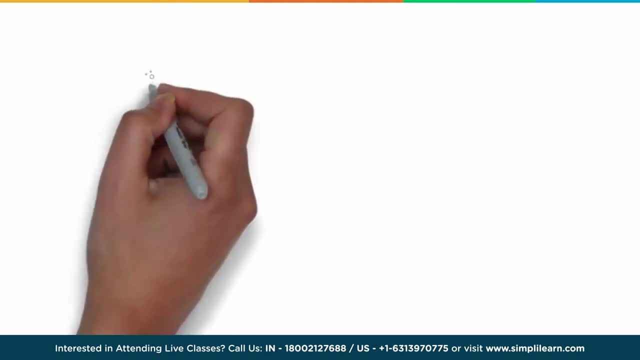 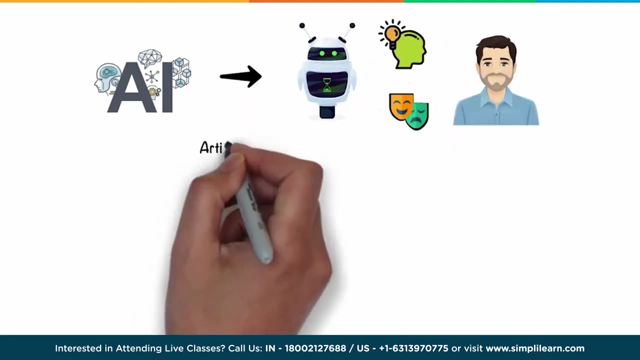 made his life easy. he did some research on the internet and found out that Netflix, Siri and Tesla are all using AI. so what is AI? AI or artificial intelligence is nothing but making computers based machines think and act like humans. artificial intelligence is not a new term. John McCarthy is the founder of artificial intelligence and he is the 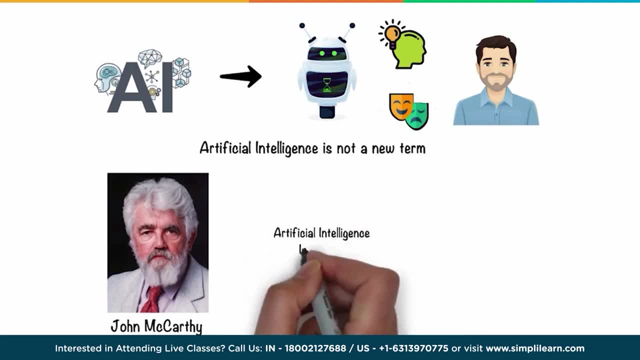 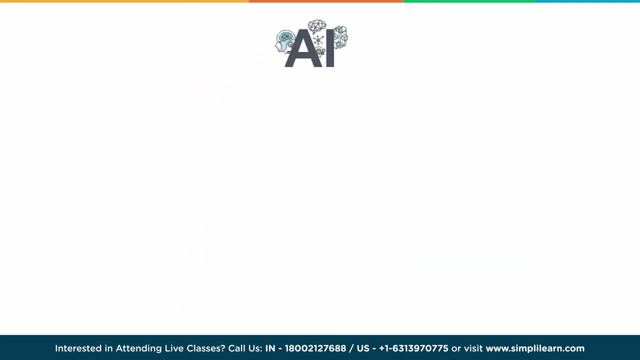 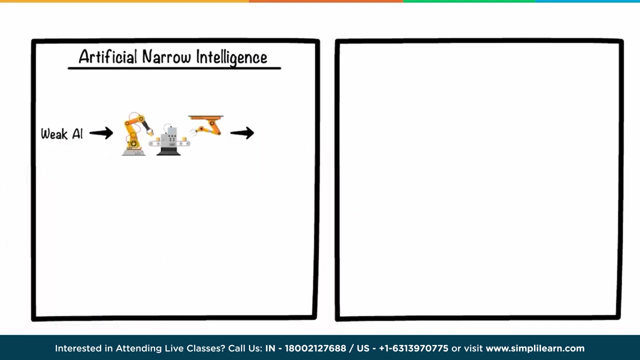 computer scientist coined the term artificial intelligence back in 1956, but it took time to evolve, as it demanded heavy computing power. artificial intelligence is not confined to just movie recommendations and virtual assistants. broadly classifying, there are three types of AI: artificial narrow intelligence, also called weak AI, is the stage where machines can perform. 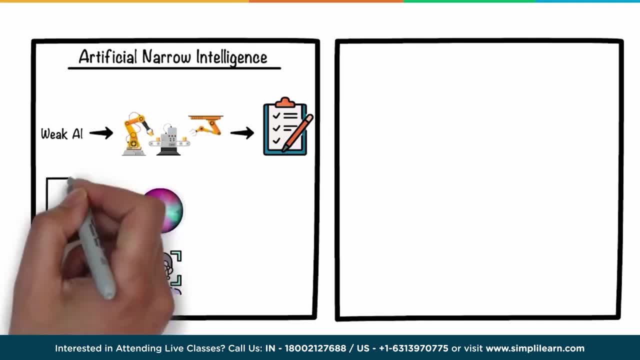 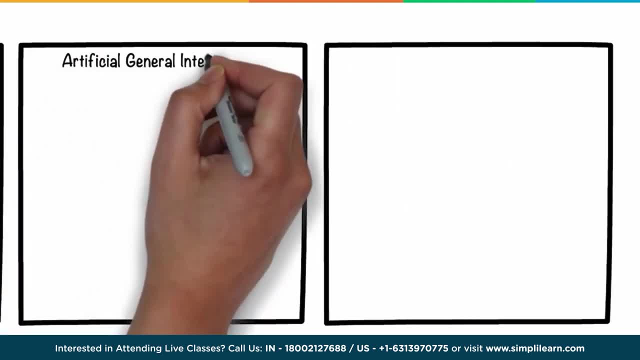 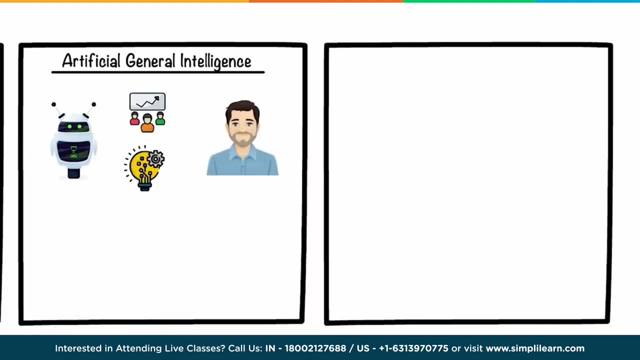 a specific task. Netflix, Siri, chatbots, spatial recommendation systems are all examples of artificial narrow intelligence. next up, we have artificial general intelligence, referred to as an intelligent agents capacity to comprehend or pick up any intellectual skill that a human can. we are halfway into successfully implementing this space: IBM's Watson, supercomputer and GPT. 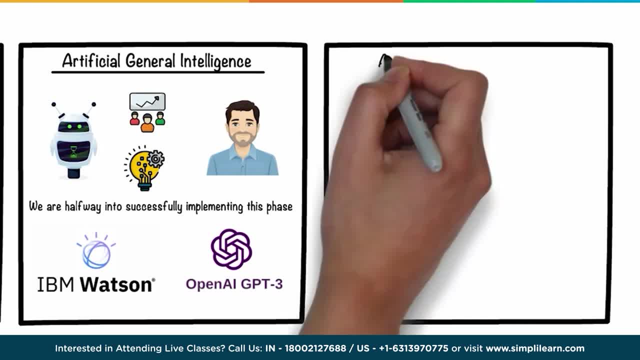 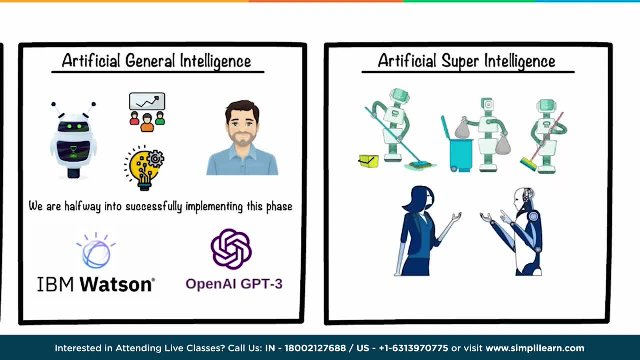 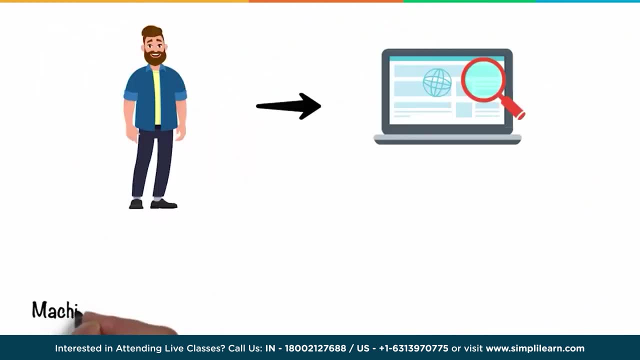 3 fall under this category. and lastly, artificial super intelligence. it is the stage where machines surpass human intelligence. you might have seen this in movies and imagined how the world would be if machines occupy. fascinated by this, John did more research and found out that machine learning, deep learning and 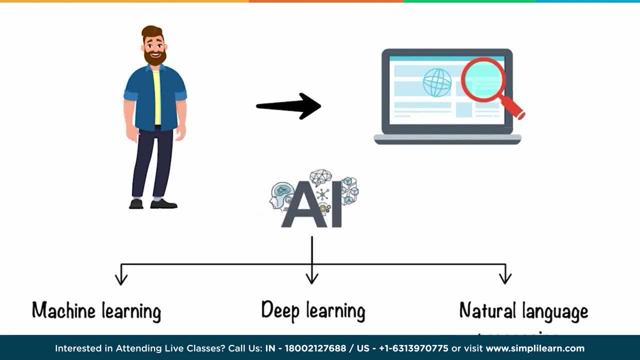 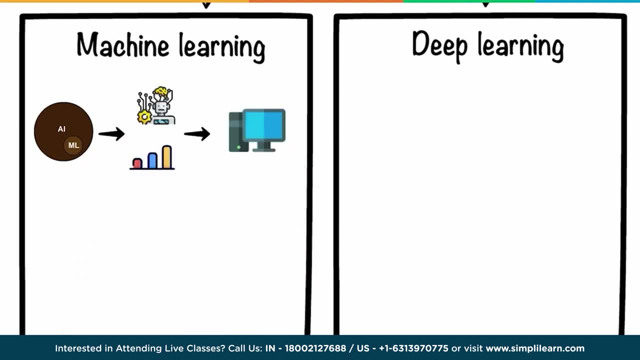 natural language processing are all connected with artificial intelligence. machine learning, a subset of AI, is the process of automating and enhancing how computers learn from their experiences. without human health, machine learning can be used in email, spam detection, medical diagnosis, etc. deep learning can be considered a set of machine learning. it is a field that is based on learning and improving on its own by 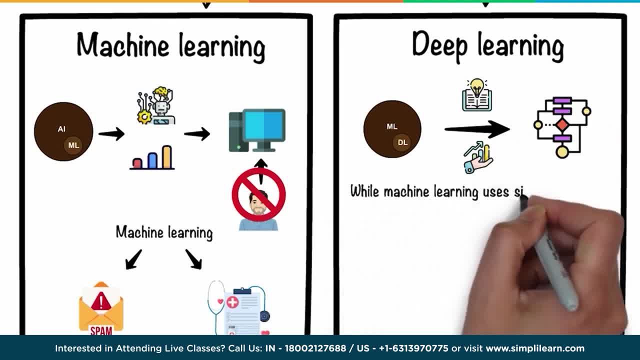 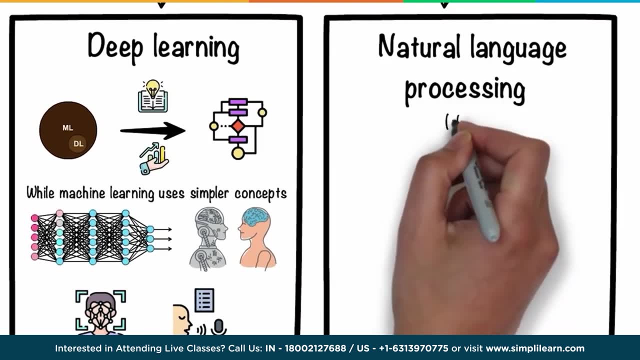 examining computer algorithms. while machine learning uses simpler concepts, deep learning works with artificial neural networks which are designed to imitate the human brain. this technology can be applied in face recognition, speech recognition and many more applications. natural language processing, popularly known as nlp, can be defined as the ability of machines. 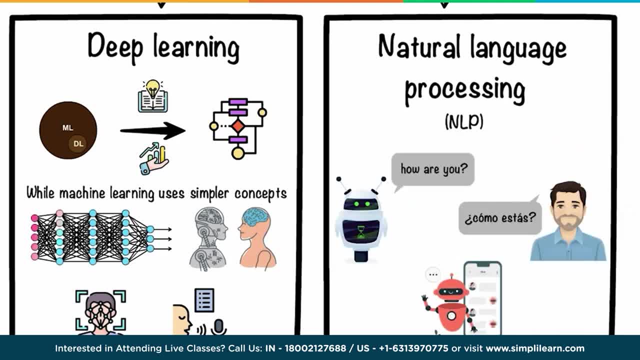 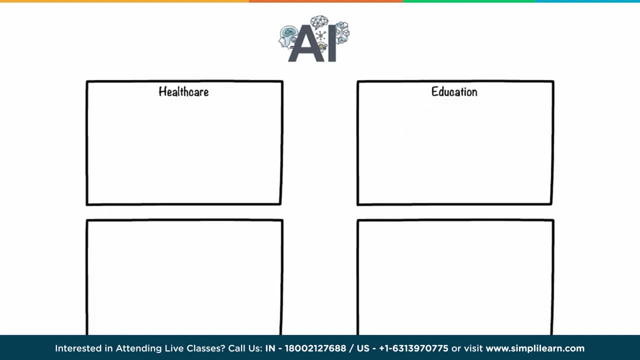 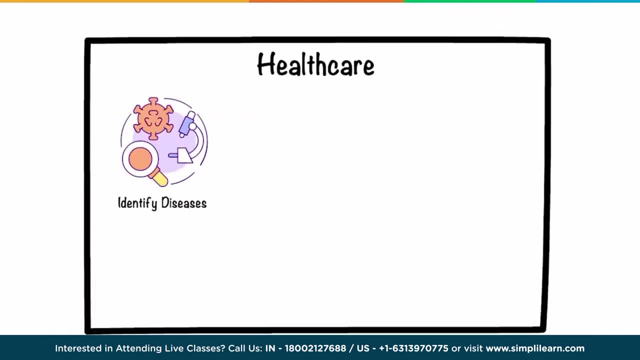 to learn human language and translate it. chat bots fall under this category. artificial intelligence is advancing in every crucial field, like healthcare, education, robotics, banking, e-commerce, and the list goes on. like in healthcare, ai is used to identify diseases, helping healthcare service providers and their patients make better treatment and lifestyle decisions. 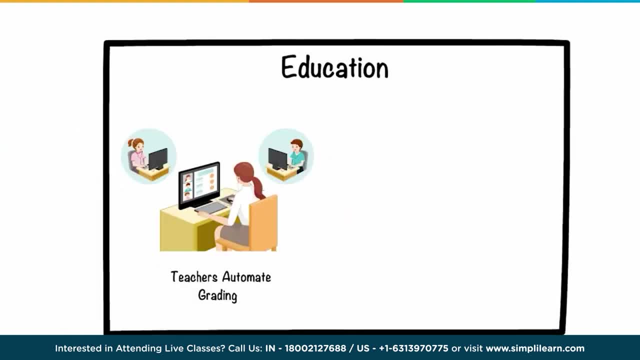 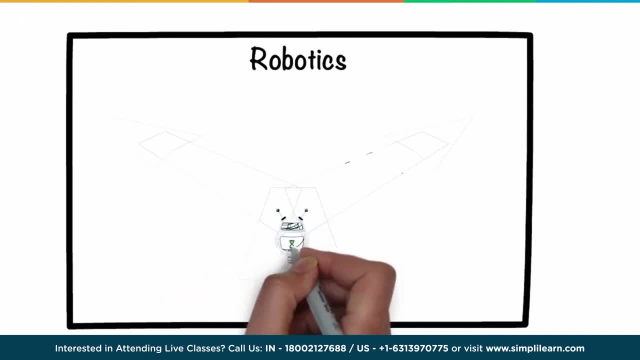 coming to the education sector. ai is helping teachers automate grading, organizing and facilitating their learning to improve their learning and their learning to improve their learning. to improve their learning. and facilitating parent guardian conversations in robotics. ai powered robots employ real-time updates to detect obstructions in their path. 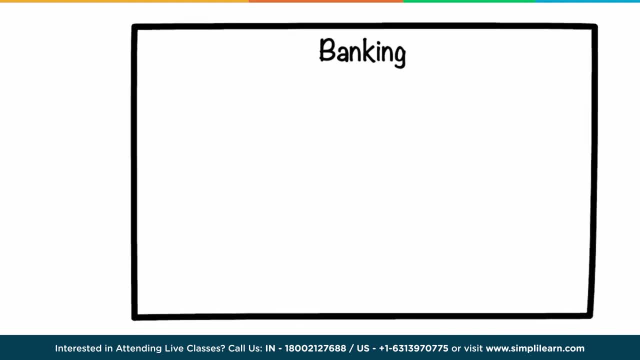 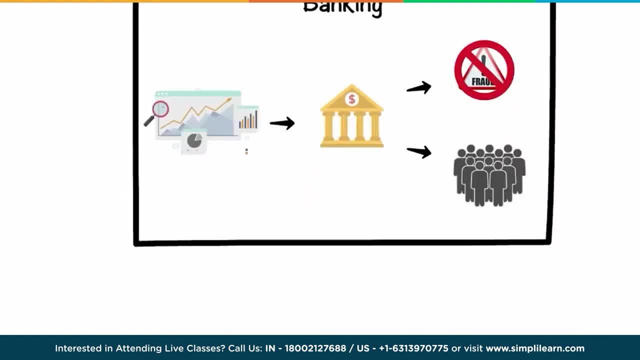 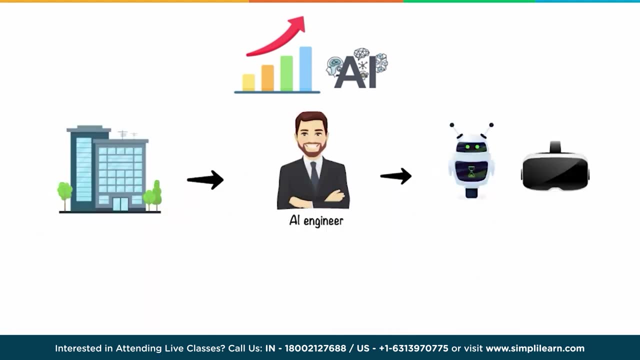 and instantaneously design their routes. artificial intelligence provides advanced data analytics. that is transforming banking by reducing fraud and enhancing compliance. with this growing demand for ai, more and more industries are looking for ai engineers who can help them develop intelligent systems and offer them lucrative salaries going north of 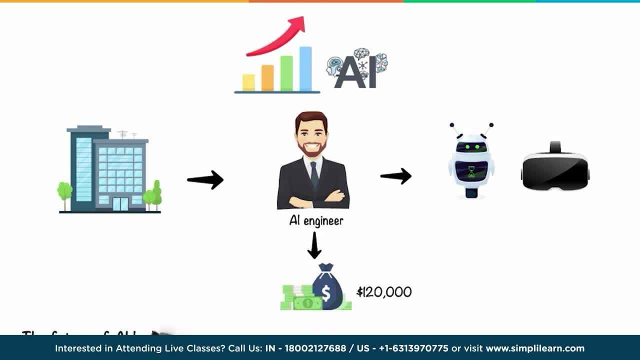 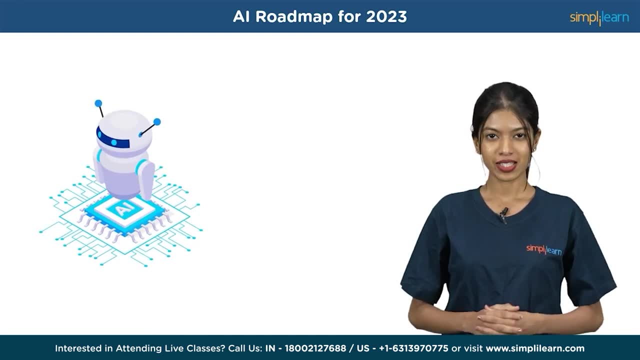 120 000. the future of ai looks promising, with the ai market expected to reach 190 billion dollars by 2025.. artificial intelligence is reshaping industries and transforming the way we live and work. it encompasses a wide range of technologies, including machine learning, deep learning, natural language processing, computer vision and many more. with its ability, 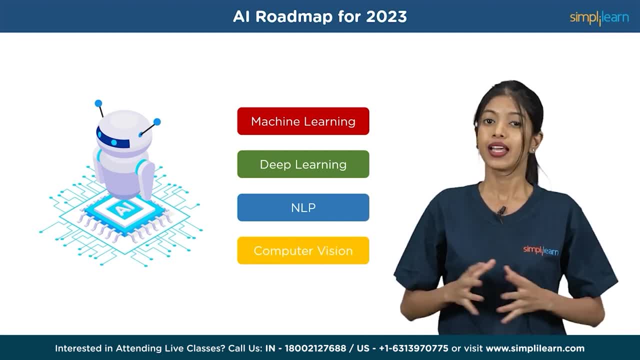 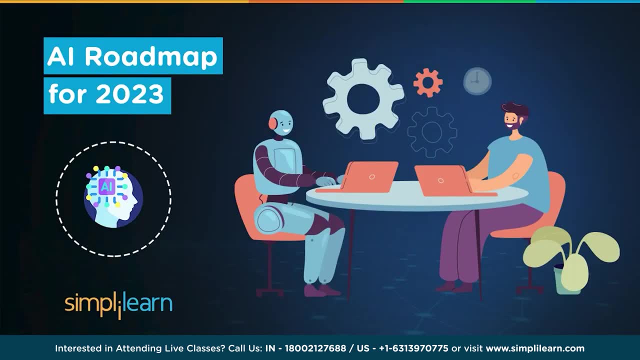 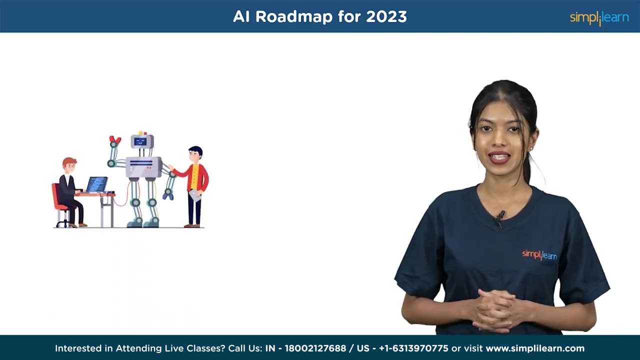 to analyze vast amount of data and make intelligent decisions. ai has become a game changer across various domains. hi everyone. welcome to simply learn's youtube channel. this ai roadmap guides you in navigating the path towards building a successful career in artificial intelligence. the ultimate goal of artificial intelligence is to create intelligent missions that can perform. 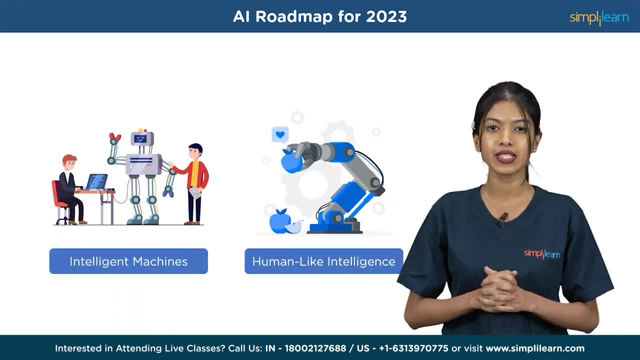 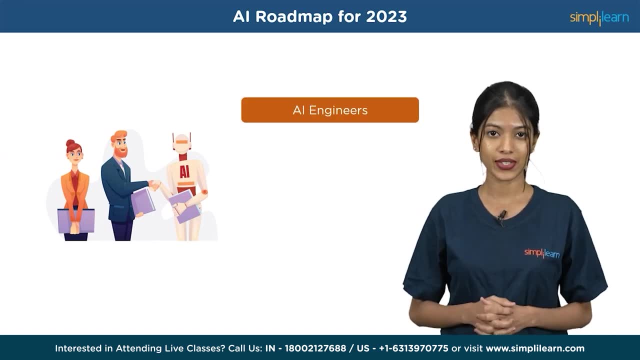 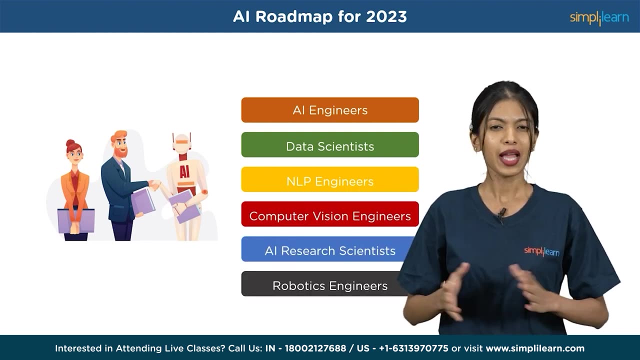 complex tasks, exhibit human-like intelligence and contribute positivity to society. ai presents exciting career opportunity in various industries and sectors. roles like ai engineer, data scientist, nlp engineers, computer vision engineers, ai research engineers and AI engineers are all ai research scientists, robotic engineers and many more offer exciting prospects for working with. 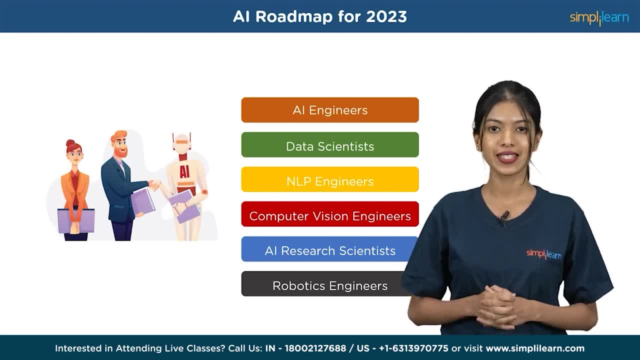 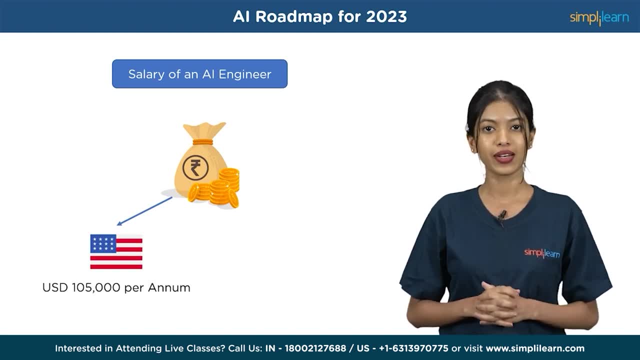 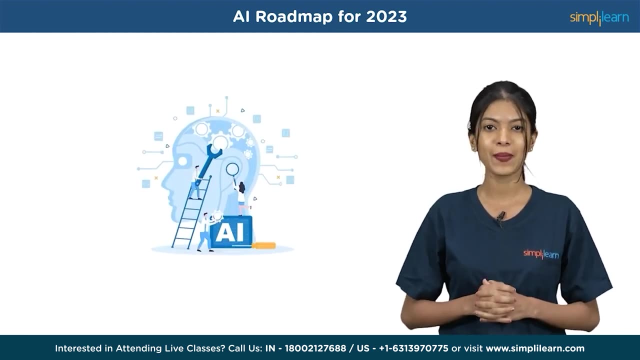 cutting-edge technologies and making an impact through artificial intelligence innovation. according to glassdoor, the average reported salary of an ai engineer in the united states is around 105 000 per year. however, in india it is 10 lakh per annum. leading companies worldwide are fully aware of the immense value of ai and are actively pursuing skilled ai engineers to contribute to. 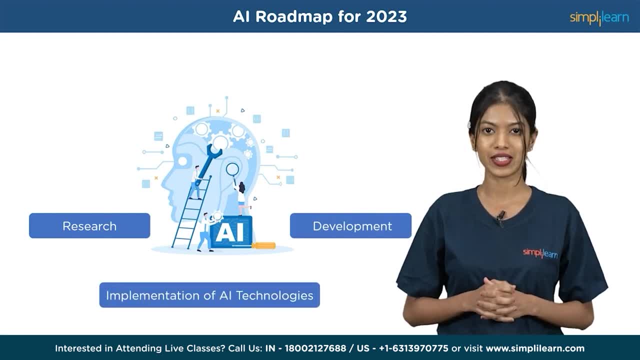 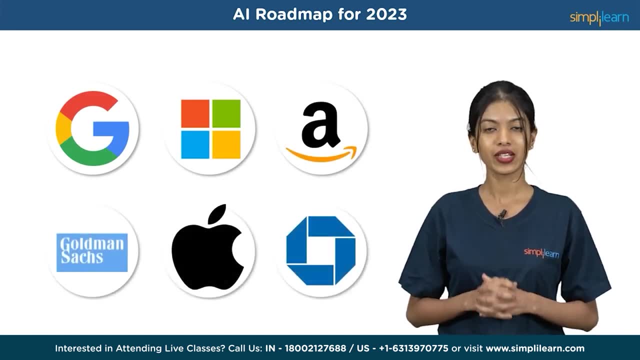 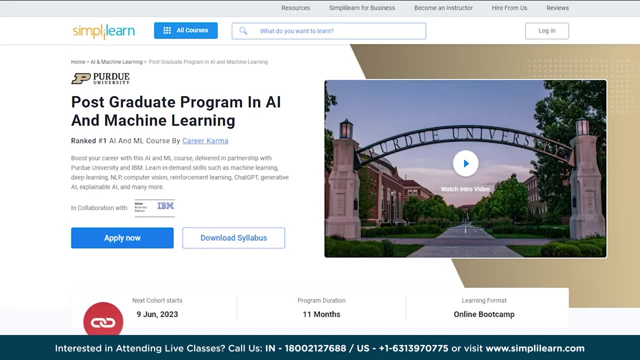 their research, development and implementation of artificial intelligence. innovation and development of artificial intelligence technology. among this top companies are google, microsoft, amazon, goldman sachs, apple and jp morgan chase. therefore, top companies hiring ai engineer provide excellent opportunity for aspiring professionals. on that note, eliminate your career with our ai and ml. 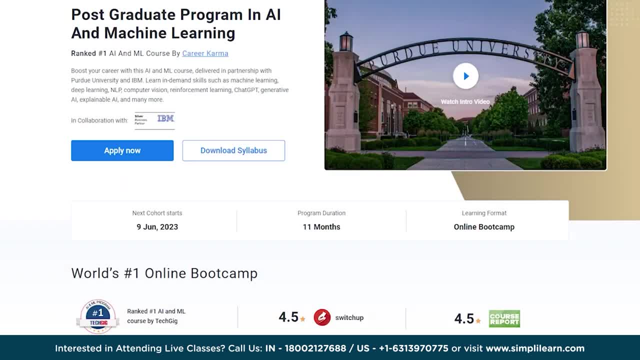 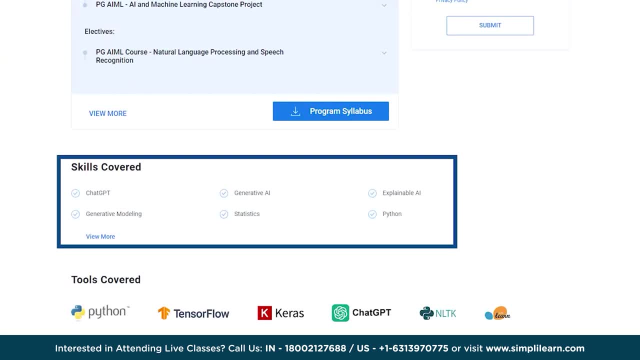 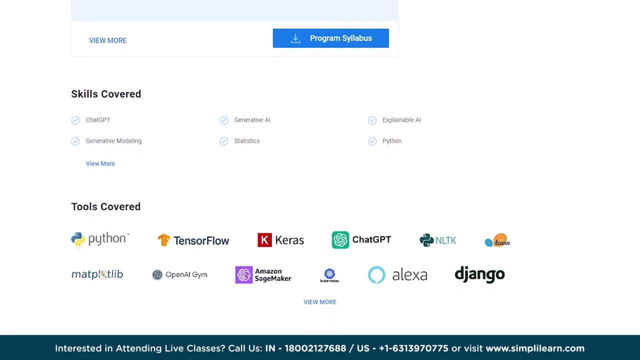 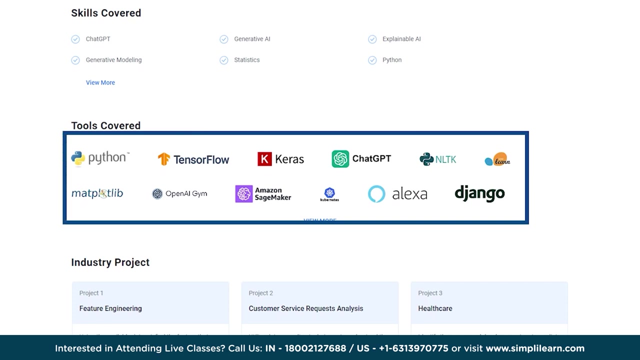 course developed in partnership with purdue university and ibm. gain expertise in high demand skills such as machine learning, deep learning, nlp, computer vision, reinforcement learning, chat, gpt, jpd, generative ai, explainable ai and more. unleash your potential and unlock exciting opportunity in the world of ai and ml. this course cover tools like python, tensorflow, keras, chat, gpt, open ai, gem. 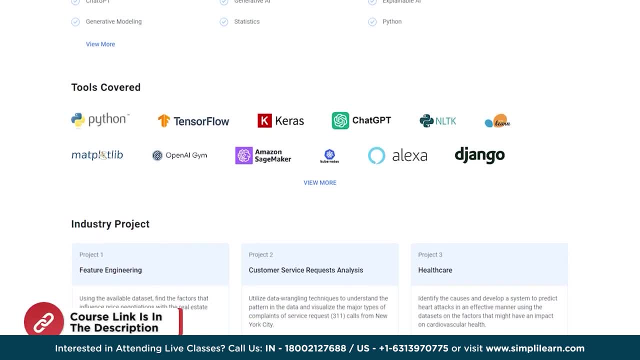 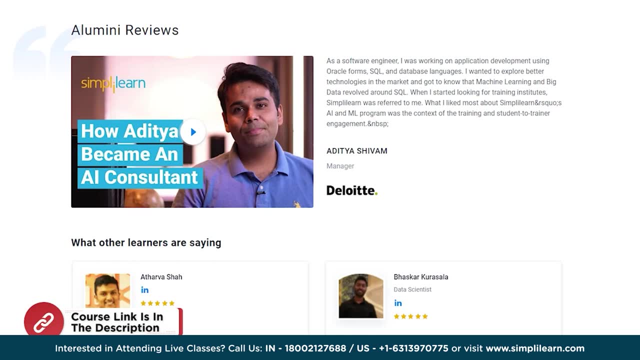 matplotlib and many more. so hurry up and find the course link in the description box for more details. our learners have experienced huge success in their careers. listen to their experience. find the simply learn course review link in the description box without any further delay. let's dive into the topic now. if you decide to become an 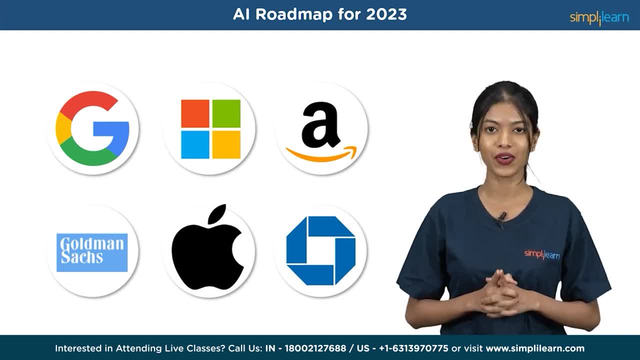 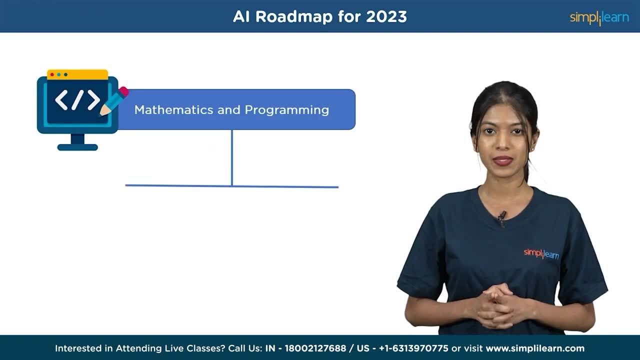 ai engineer. here are the steps you can follow to achieve your goal. firstly, obtain a strong foundation in mathematics and programming. gain a strong foundation in creating mathematic concepts like linear algebra, calculus and probability theory. in addition to that, it is crucial to acquire mastery of programming languages like python, commonly used in ai, and become proficient. 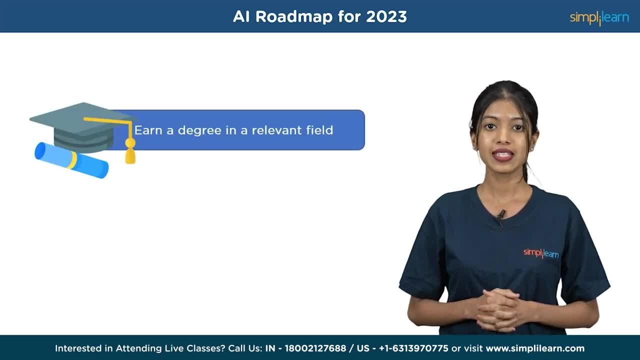 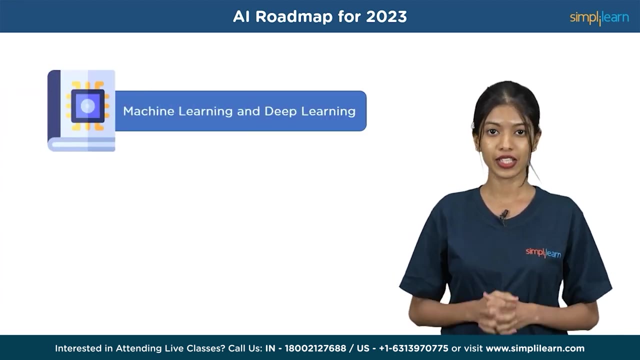 in coding, then earn a degree in a relevant field. that means earn a bachelor's or master degree in computer science, data science, ai or computer science and computer science and computer science or a related field to gain a comprehensive understanding of ai principles and techniques. next, gain knowledge in machine learning and deep learning to become a ai engineer develop. 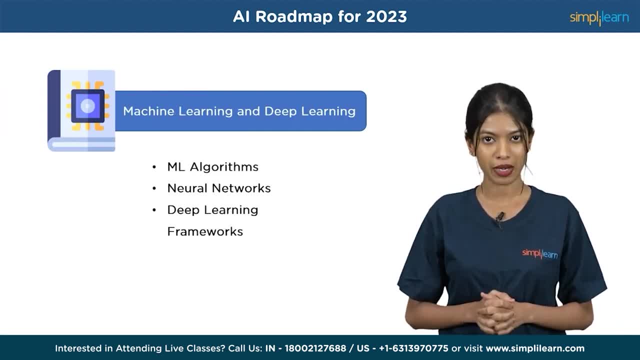 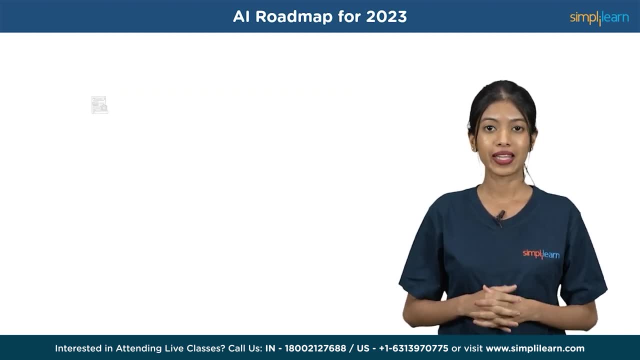 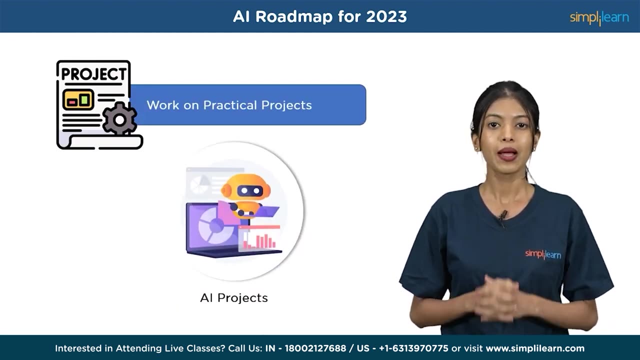 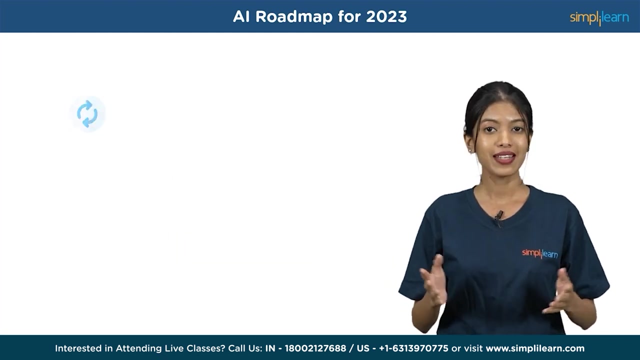 familiarity with ml algorithms, neural networks and deep learning frameworks- example, tensorflow, pytorch- to train and optimize models using real world data set, followed by that work on practical projects. gain hands-on experience and showcase your skills while working on ai projects. moreover, demonstrate your ability to solve ai problems, impressing potential employers. then stay updated. 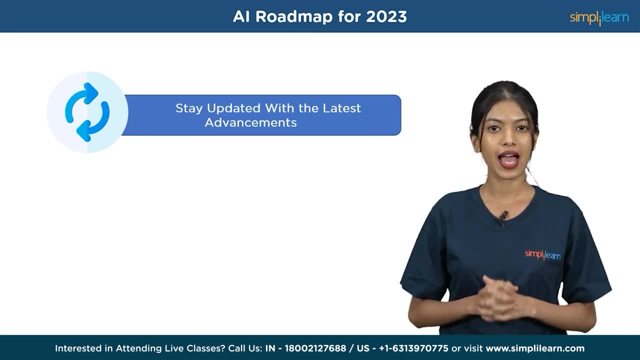 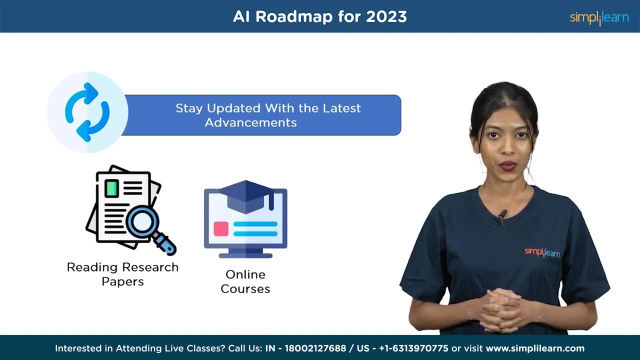 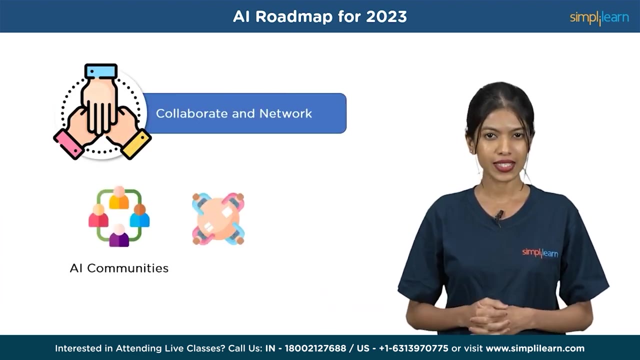 with the latest advancements. stay updated with the latest trends and research in ai, a rapidly evolving field, and expanding your knowledge by reading research papers, participating in online courses and workshops and joining ai communities. next, collaborate and network. engage with ai communities. attend conference, participate in online forums to connect with professionals in 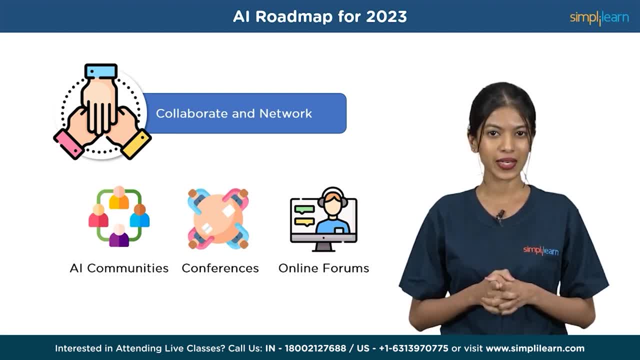 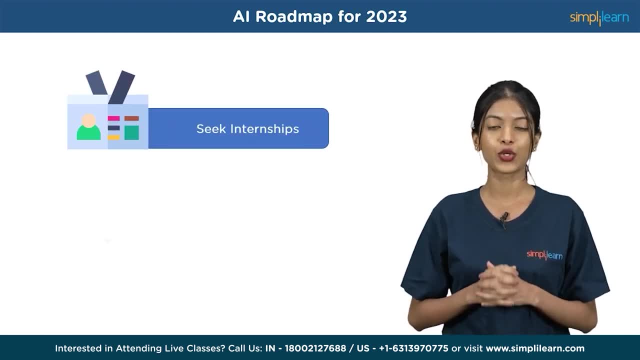 this field. collaborating with other AI engineers can be a great way to improve your skills, and with others can enhance your learning experience and open new opportunities later seek internships or entry-level positions. gain practical experience through ai internships or entry-level roles in industry or research institutions. this provides valuable exposures and help develop your skills. 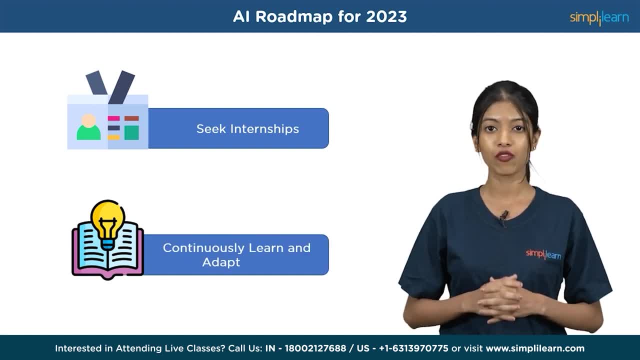 finally, continuously learn and adapt in the rapidly evolving field of ai, stay updated on new developments, explore specialized areas and embrace emerging technologies and tools to pursue a career as an ai engineer. now that we have covered the essential steps to become an ai engineer, let's explore the 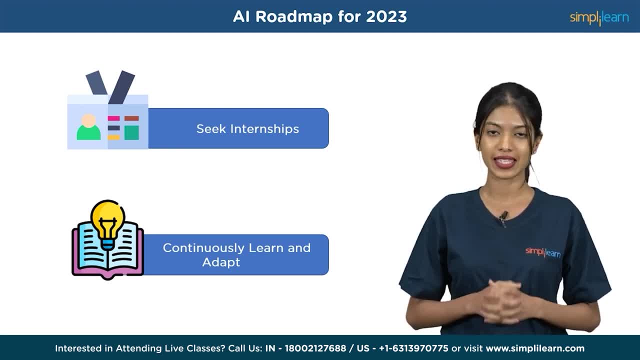 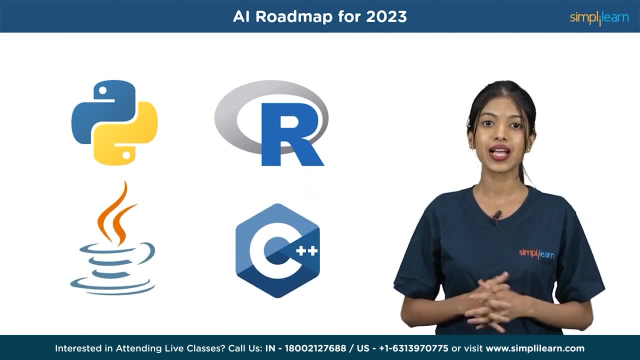 necessary programming languages and algorithms for aspiring ai engineers. so mastering programming languages like python, r, java and c plus plus is vital for acquiring proficiency in ai. this language enables you to construct and deploy models effectively. additionally, it will help if you gain a thorough understanding of machine learning algorithms, such as linear regressions. 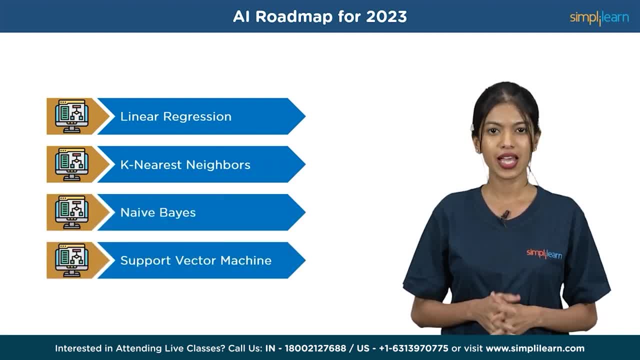 k. nearest neighbors, associations and support vector coupons. indigenous human intelligence. these languages and algorithms are fundamental tools in the field of ai. they will enable you to develop and implement effective artificial intelligence models. now let's give a minute to hear from our learners who have experienced juice success in their career. 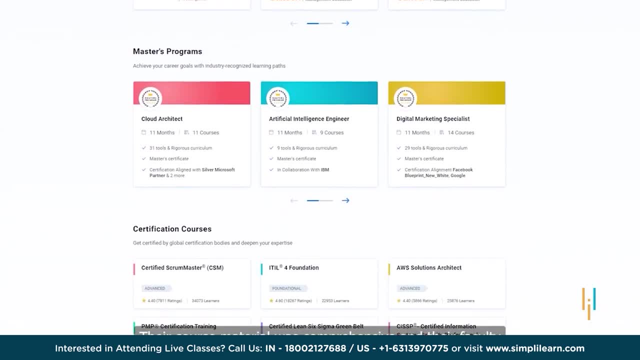 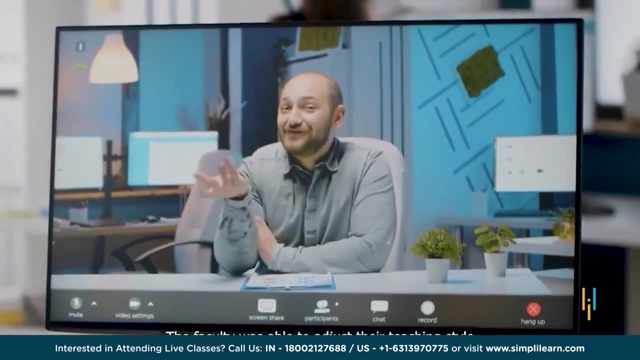 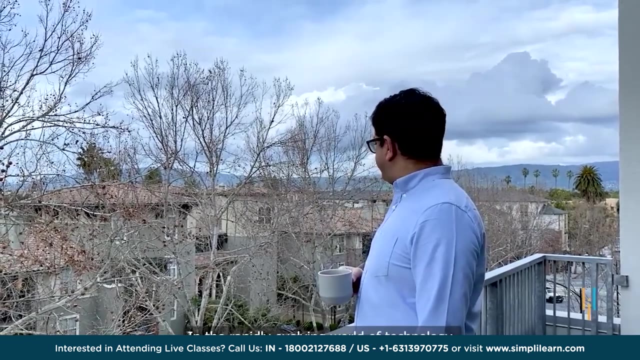 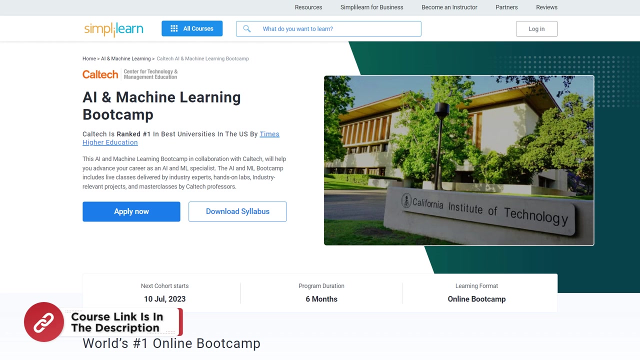 przypadku: knowledge uik� ah. six questions: the overall skill set of the class. in the rapidly evolving world of technology, it's important to keep upskilling for every working professional, and now we are thrilled to present our ai bootcamp that is designed to equip you with the knowledge and skills you need to thrive in this fast-paced 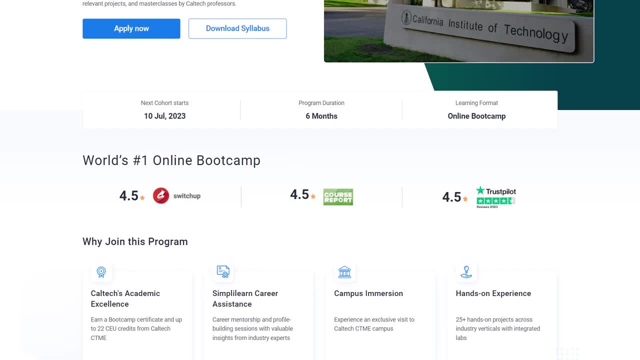 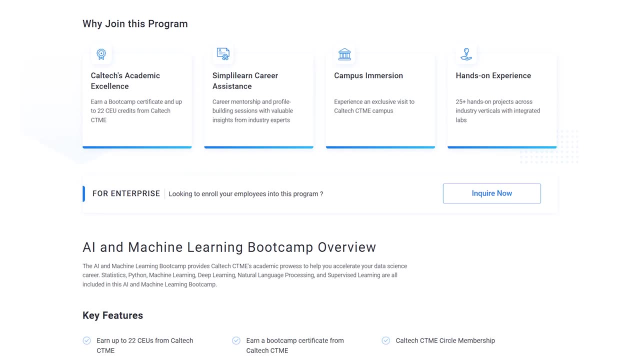 and ever-evolving field. in this six months intensive and immersive learning experience, you will have the opportunity to dive headfirst into the subject matter, gaining hands-on experience and building a strong foundation in ai. we believe in a practical approach where you will work on 25. 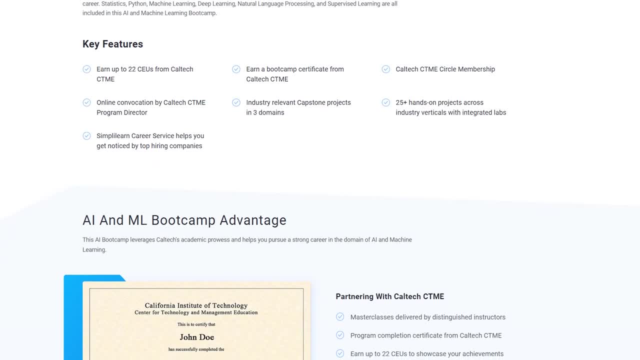 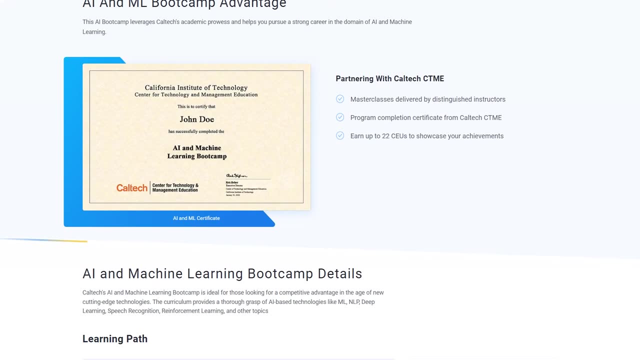 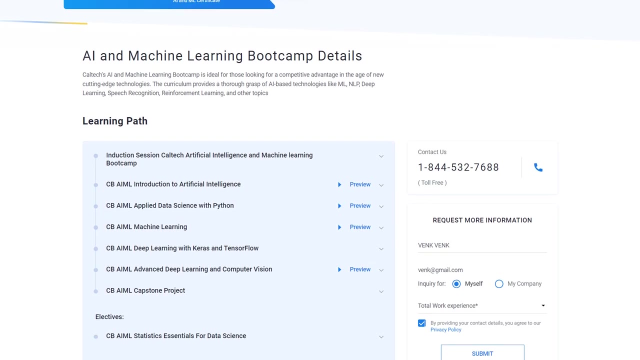 plus hands-on projects across various industry verticals, providing you with real world experience. what sets our bootcamp apart is our partnership with caltech cdme, ensuring academic excellence and industry recognition. by successfully completing the bootcamp, you will earn a prestigious certificate and up to 22 cu credits from caltech cdme, validating your expertise in 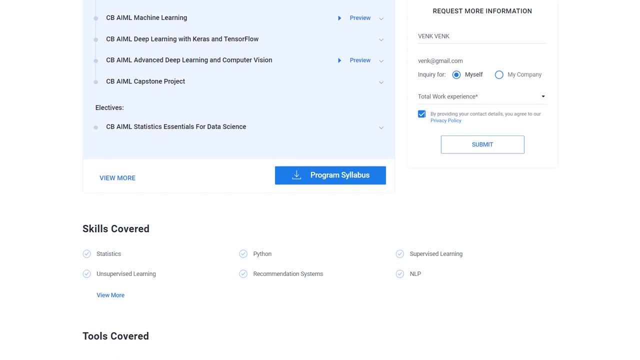 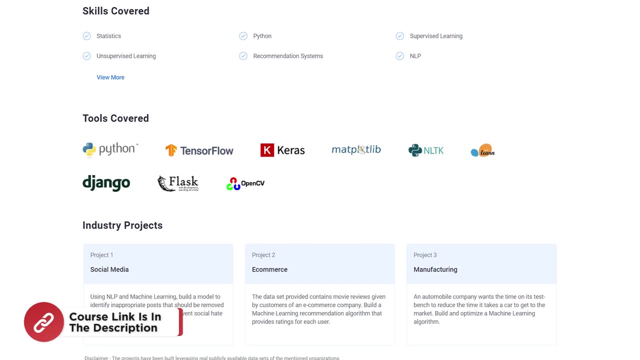 the field. so are you ready to embark on this transformative journey? you are you ready to unlock the power of ai and take your career to new heights? if so, enroll in our ai bootcamp today and become part of the ai revolution. the course link is mentioned in the description. 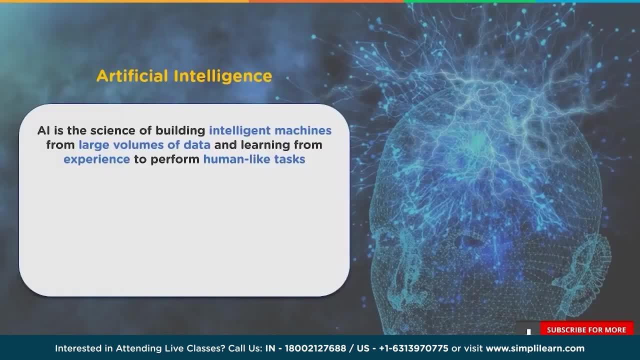 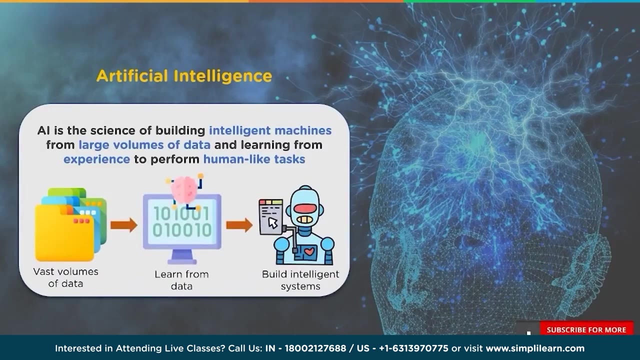 box below. first let's understand what really is artificial intelligence. artificial intelligence is the science of building intelligent machines from vast volumes of data. this data can be structured, semi-structured or unstructured in nature. ai systems learn from past experiences and perform human-like tasks. artificial intelligence enhances the speed, decision and effectiveness of 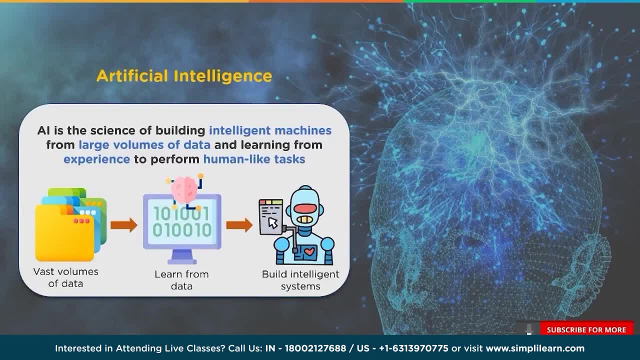 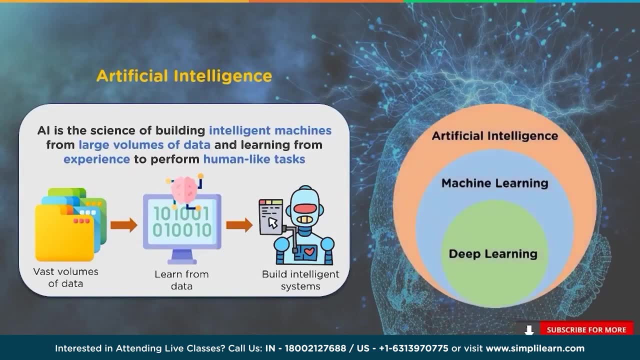 human efforts. ai uses sophisticated algorithms and methods to build machines that can make decisions on their own. deep learning and machine learning are the two subsets of artificial intelligence, so you need both machine learning algorithms and deep learning networks to build intelligent systems. ai is now being widely used in almost every sector of business, such as: 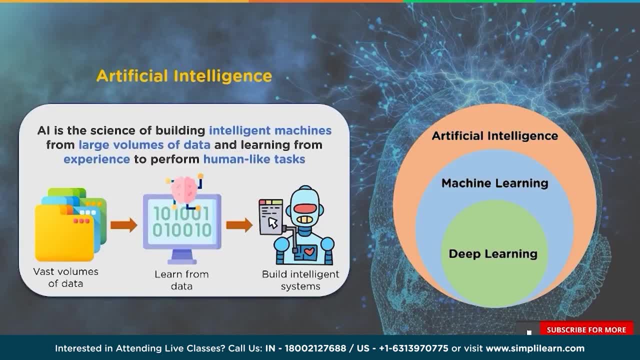 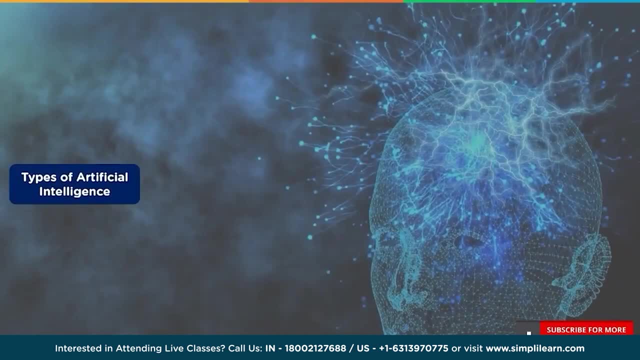 transportation, healthcare, banking, retail, entertainment and e-commerce. now let's look at the different types of artificial intelligence. so AI can be classified based on capabilities and functionalities. under capabilities, there are three types of artificial intelligence. they are narrow AI, general AI and super AI. under functionalities, we have four types of artificial 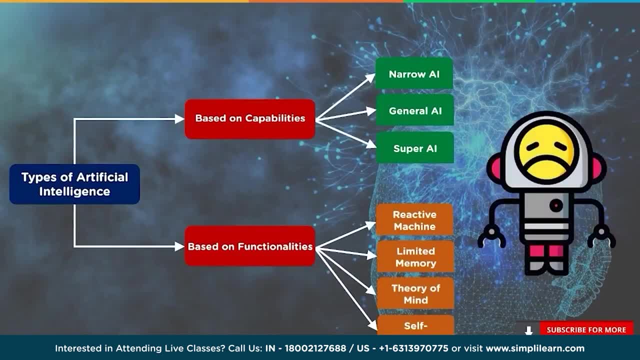 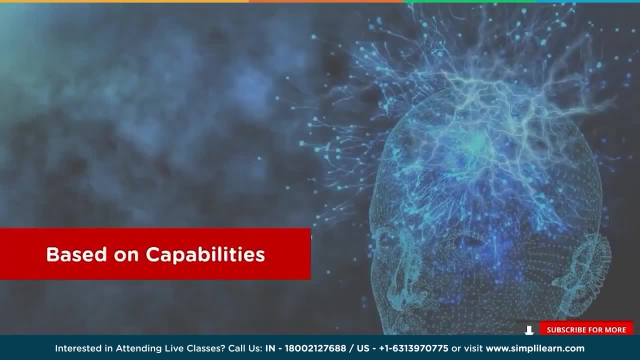 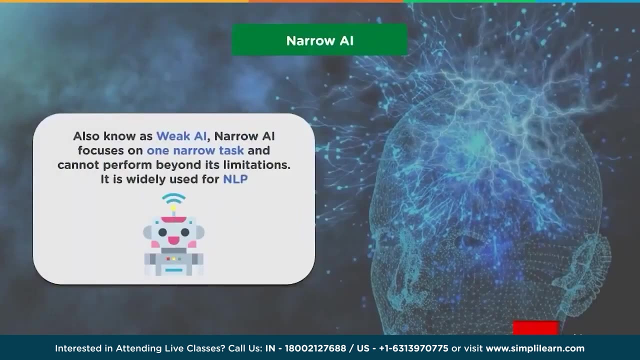 intelligence, reactive machine, limited memory, theory of mind and self-awareness. let's look at them one by one. first, we will look at the different types of artificial intelligence based on capabilities. so what is narrow AI? narrow AI, also known as weak AI, focuses on one narrow task and cannot perform beyond its limitations. it aims at a single subset. 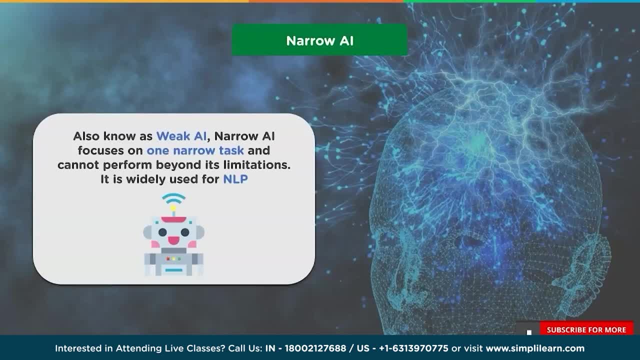 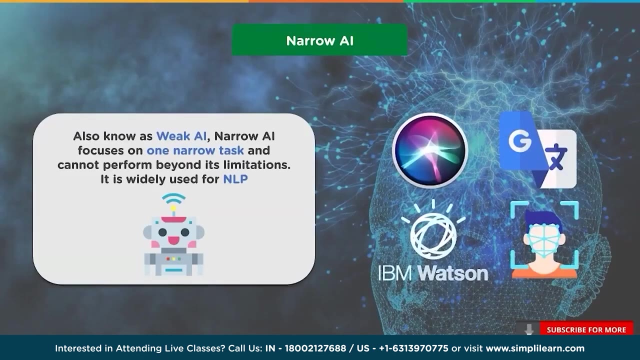 of cognitive abilities and advances in the development of new technologies in that spectrum. applications of narrow AI are becoming increasingly common in our day-to-day lives as machine learning and deep learning methods continue to evolve. Apple's Siri is a simple example of a narrow AI that operates with a limited, predefined range of functions. Siri often 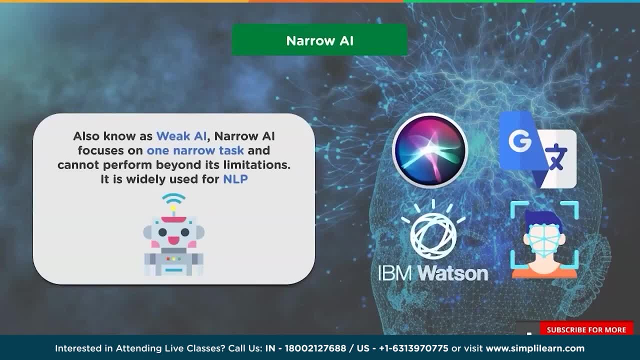 has challenges with tasks outside its range of abilities. IBM Watson supercomputer is another example of narrow AI, which applies cognitive computing, machine learning and natural language processing to process information and to develop new technologies and technologies in the future. IBM Watson once outperformed human contestant, Ken Jenkins to become the 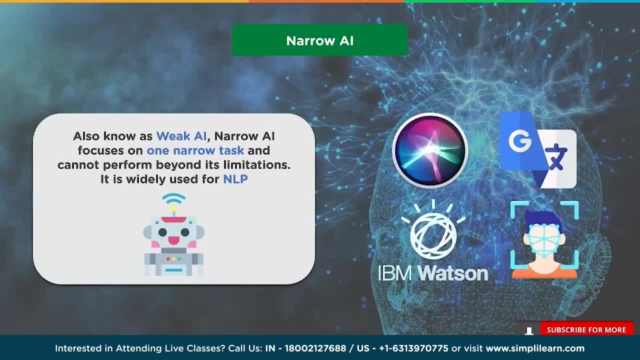 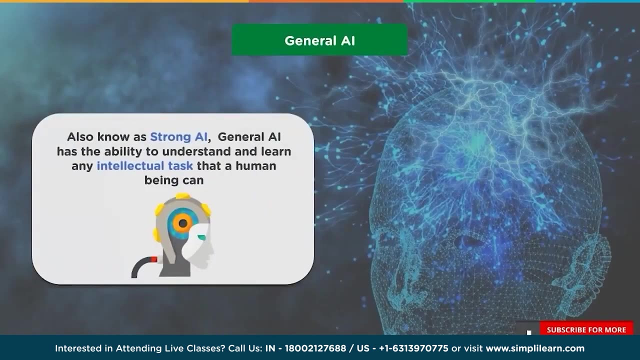 champion on the popular game show Jeopardy. other examples of narrow AI include Google Translate, image recognition software, recommendation systems, spam filtering and Google's page ranking algorithm. next we have general artificial intelligence, or general AI. general AI, also known as strong AI, has the ability to understand and process information. 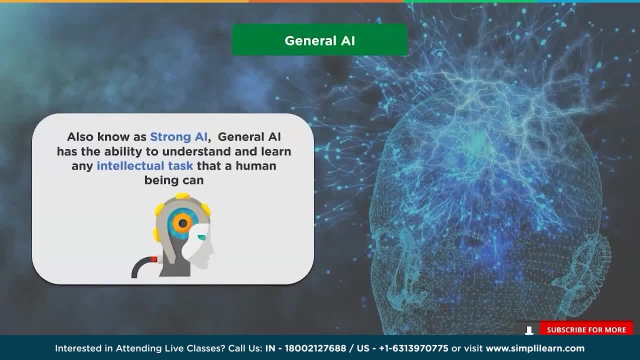 and learn any intellectual task that a human can. general artificial intelligence has received a 1 billion dollar investment from Microsoft. through open AI, it allows a machine to apply knowledge and skills in different contexts. AI researchers and scientists have not achieved strong AI so far. to succeed, they would need to find a way to make machines conscious programming a. 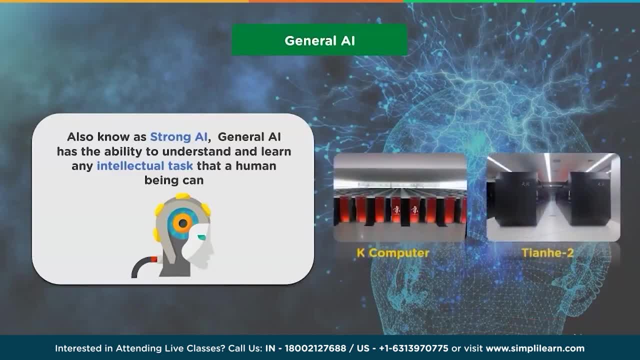 full set of cognitive abilities. Fujitsu built the K computer, which is one of the fastest computers in the world. it is one of the most notable attempts at achieving strong II. it took 40 minutes to simulate a single second of neural activity, so it is difficult to determine whether or not strong AI will be. 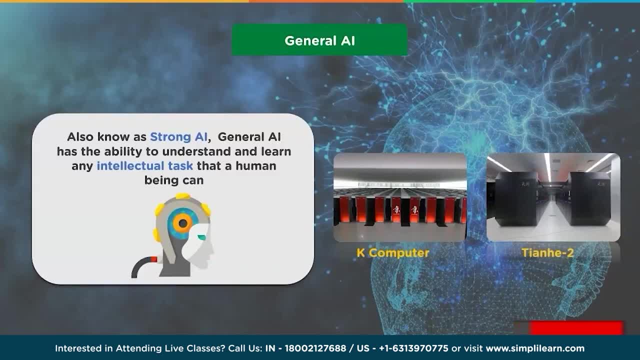 achieved in the near future. Tianhe2 is a supercomputer created by China's National University of Defense Technology. it currently holds the record for CPS at 30 3.8. 6 better flops. although it sounds exciting, the human brain is estimated to be capable of one exaflop. Now, CPS means characters per. 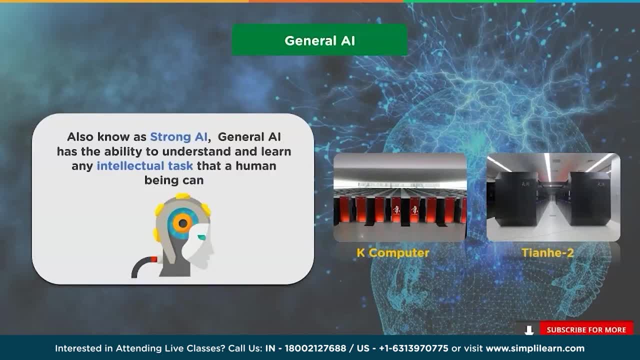 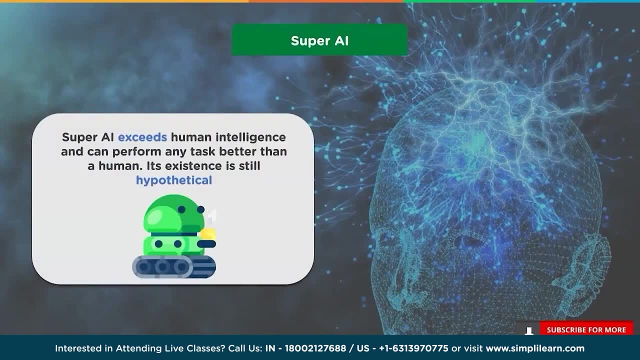 second, that a system can process. Third, in the list of AI that is based on capabilities, we have Super AI. Super AI exceeds human intelligence and can perform any task better than a human. The concept of artificial superintelligence sees AI evolved to be so akin to human. 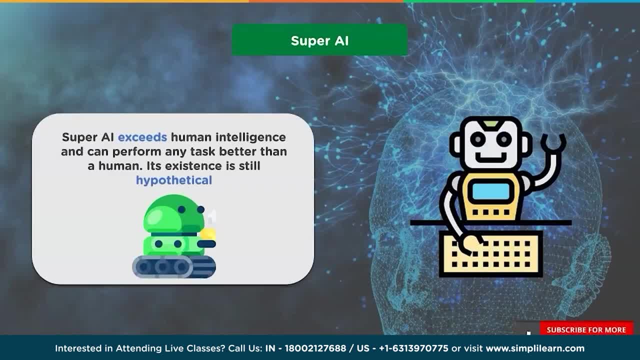 emotions and experiences, that it doesn't just understand them. It evokes emotions, needs, beliefs and desires of its own. Its existence is still hypothetical. Some of the key characteristics of Super AI include the ability to think, solve puzzles, make judgments and decisions on its own. 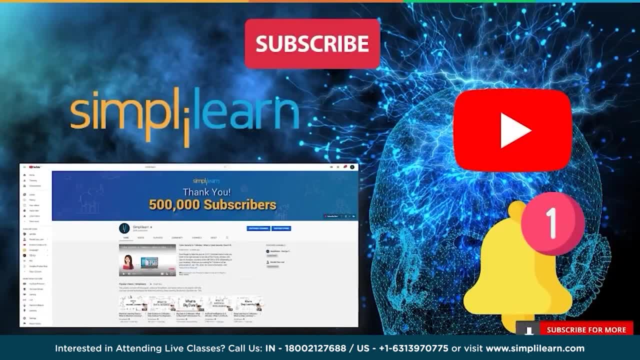 Now, if you have enjoyed watching this video so far, please make sure to subscribe to our YouTube channel and hit the bell icon to stay updated with all the latest technologies. Also, if you have any questions related to this video, please put it in the chat section. Our team of experts. 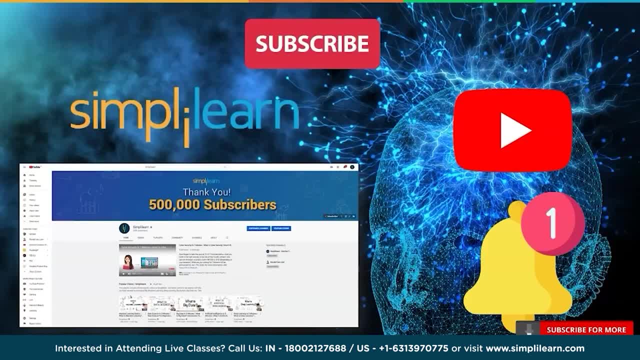 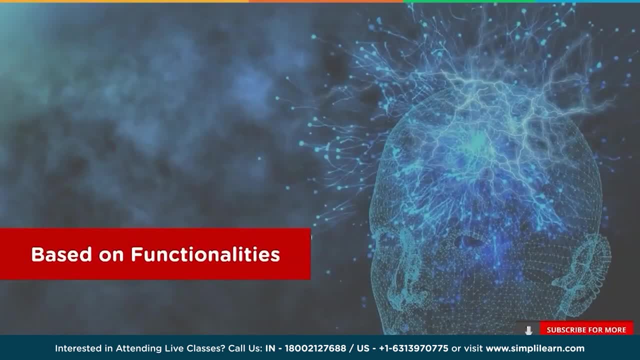 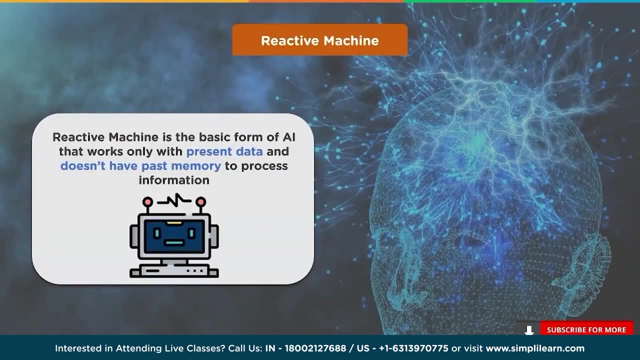 will help you address your questions. Moving ahead now, we will see the different types of artificial intelligence based on functionalities In this category. first we have reactive machine. A reactive machine is the basic form of AI that does not store memories or use past experiences to determine future actions. It works only with 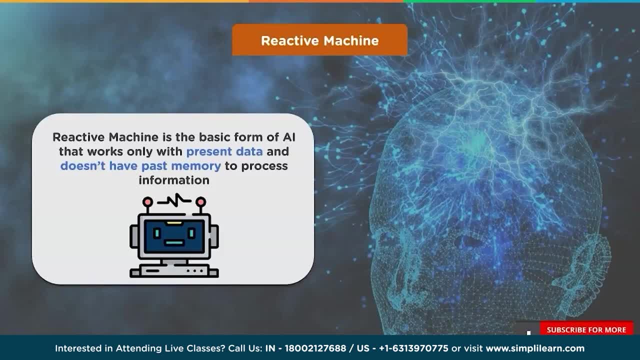 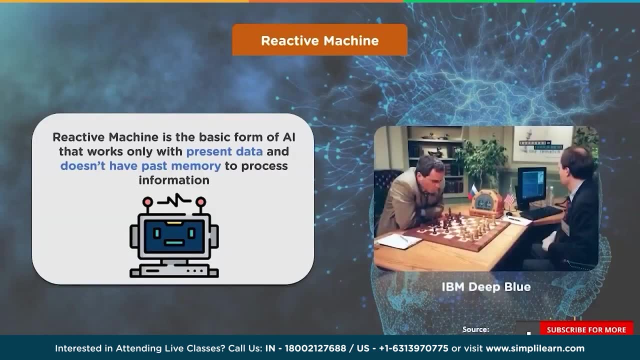 present data. They simply perceive the world and react to it. Reactive machines are given certain tasks and don't have capabilities beyond those duties. IBM's Deep Blue, which defeated chess grandmaster Gary Kasparov, is a reactive machine that sees the pieces on a chessboard and reacts to them. It cannot. 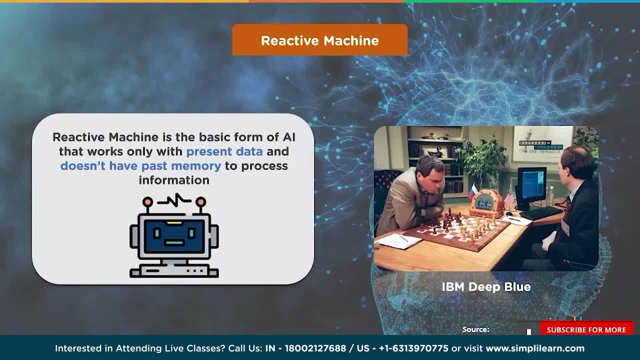 refer to any of its prior experiences and cannot improve with practice. Deep Blue can identify the pieces on a chessboard and know how each moves. It can make predictions about what moves might be next for it and its opponent. It can choose the most optimal moves from among the possibilities. Deep Blue it. 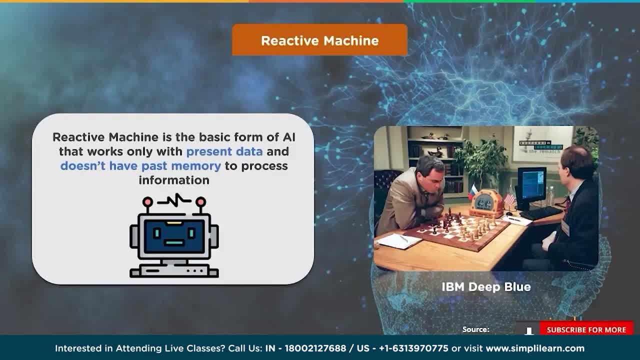 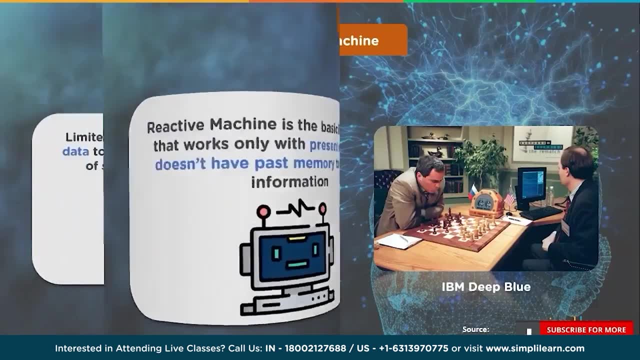 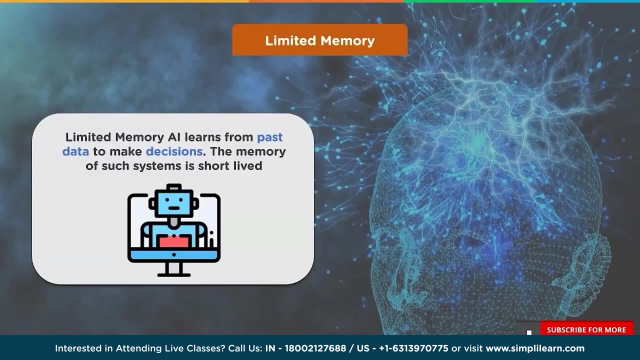 knows everything before the present moment. All it does is look at the pieces on the chessboard as it stands right now and choose from possible next moves Up. next we have limited memory. Limited memory: AI learns from past data to make decisions. The memory of such 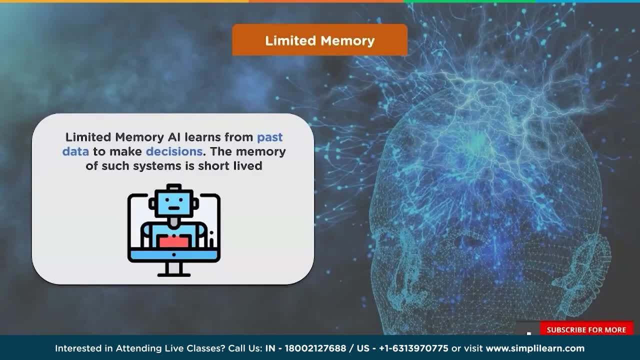 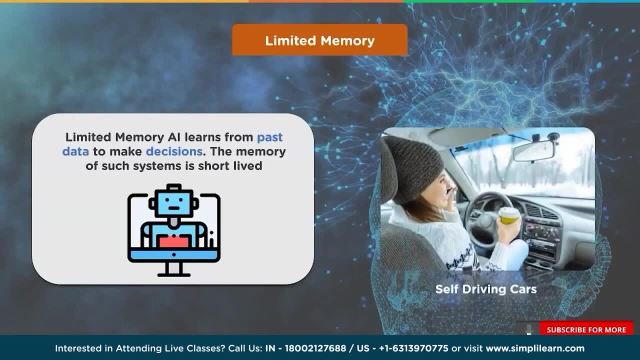 systems is short-lived. while they can use this data for a specific period of time, they cannot add it to a library of their experiences. this kind of technology is used for self-driving vehicles. they observe how other vehicles are moving around them in the present and as time passes, that ongoing. 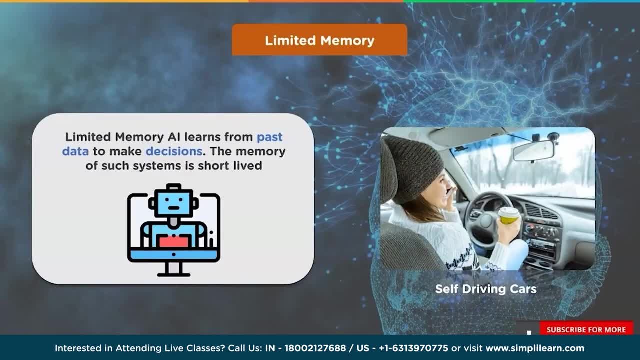 collected data gets added to the static data within the AI machine, such as lean markers and traffic lights. they're included when the vehicle decides to change lanes to avoid cutting of another driver or being hit by a nearby vehicle. Mitsubishi Electric is a company that has been figuring out how to improve. 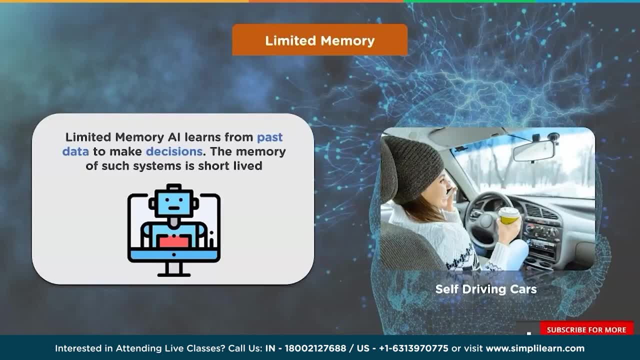 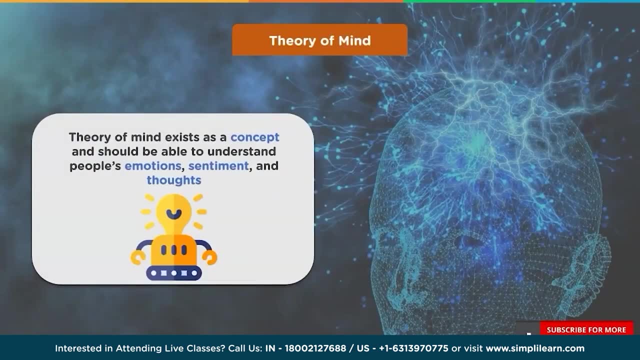 such technology for applications like self-driving cars. then we have theory of mind. theory of mind represents a very advanced class of technology and exists as a concept. this kind of AI requires a thorough understanding that the people and the things within an environment can alter feelings and behaviors. it should be able to. 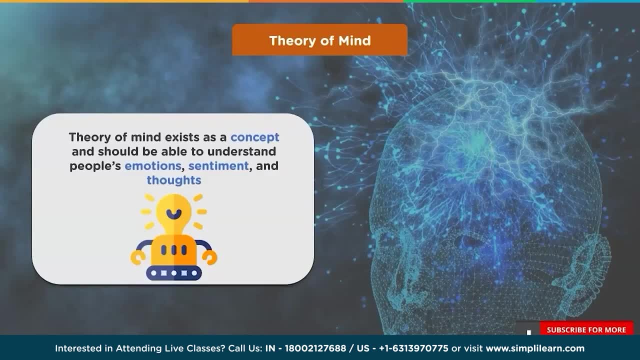 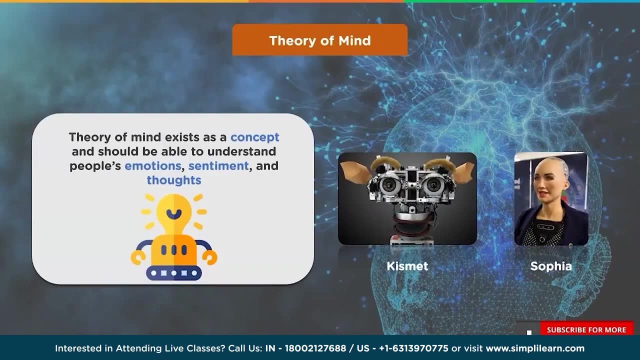 understand people's emotions, sentiment and thoughts. even though a lot of improvements are there in this field, this kind of AI is not complete yet. one real-world example of theory of mind AI is Kismet, a robot head made in the late 90s by a Massachusetts Institute of Technology researcher. Kismet can mimic. 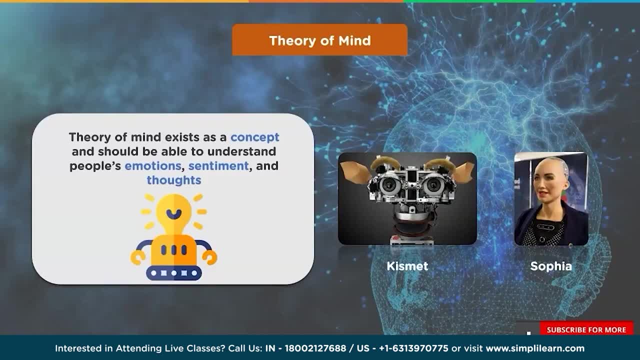 human emotions and recognize them. both abilities are key, advantageous in theory of mind AI, but Kismet can't follow gazes or convey attention to humans. Sophia from Hanson robotics is another example where the theory of mind AI was implemented: cameras within Sophia's eyes combined with computer. 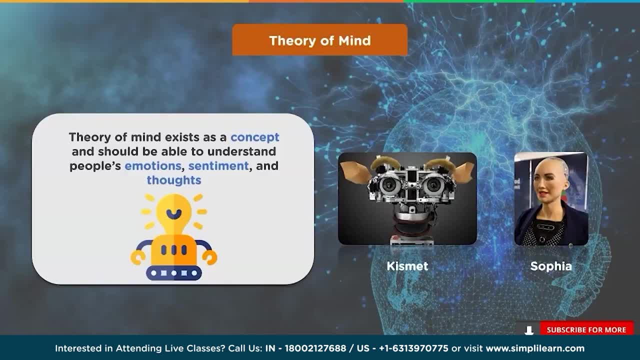 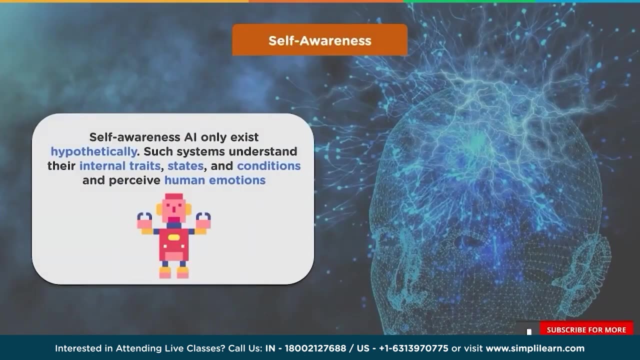 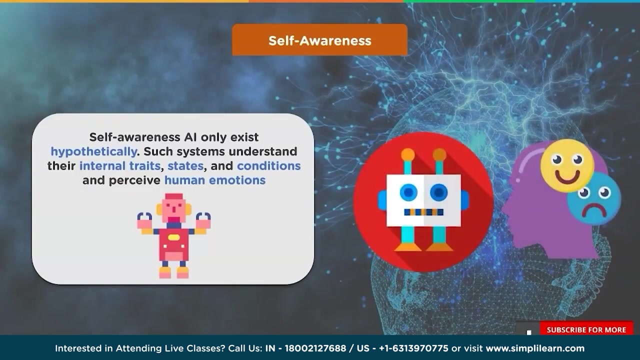 algorithms allow her to see. she can follow faces, sustain eye contact and recognize individuals. she is able to process speech and have conversations using natural language subsystem. finally, we have self-awareness. self-awareness AI only exists hypothetically. such systems understand that internal traits, states and conditions and perceive human emotions. these machines will be smarter than the. 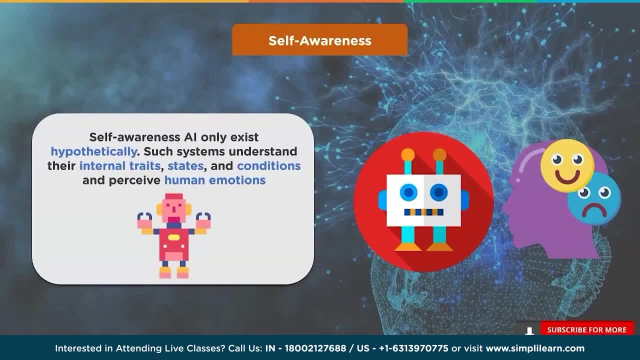 human mind. this type of AI will not only be able to understand and evoke emotions in those it interacts with, but also have emotions, needs and beliefs of its own. while we are probably far away from creating machines that are self aware, we should focus our efforts towards understanding. 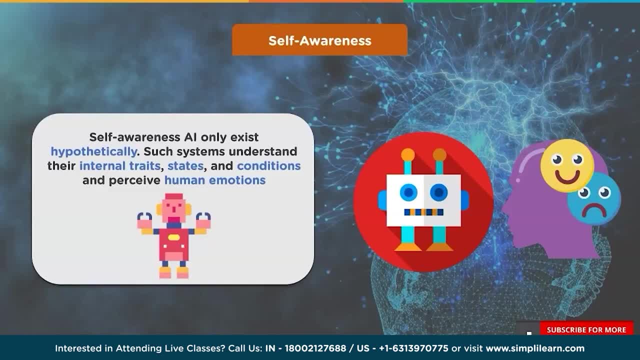 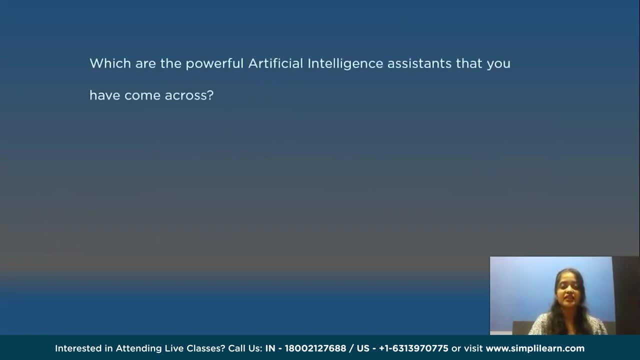 memory learning and the ability to base decisions on past experiences. so what? let me ask you a question: which are the powerful AI assistance that you have come across? please leave your answer in the comment section below and stay tuned to get the answer so that the top 10 applications of 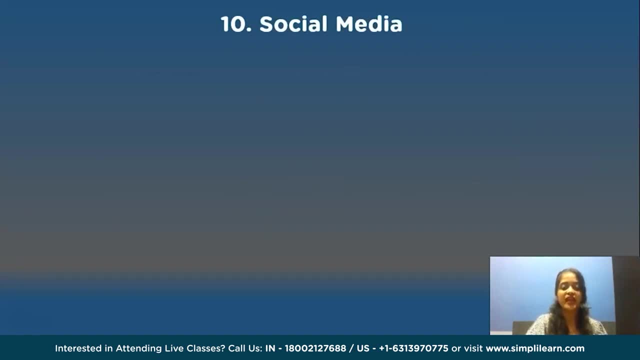 artificial intelligence social media. today, AI can create social media posts for you. It can draft and target social ads. It can also automate monitoring and it has powers that most of what you see in any given social network. Facebook's picture recognition tools have been popular among users for a while, but the company is constantly working. 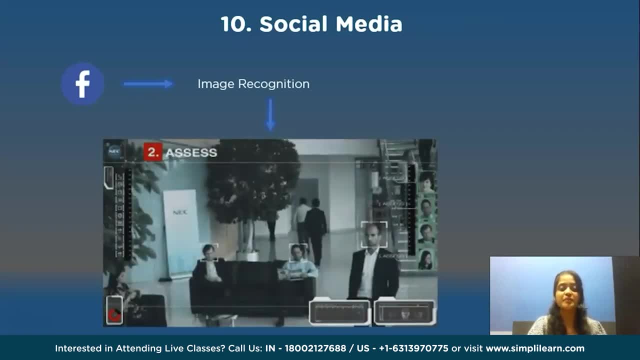 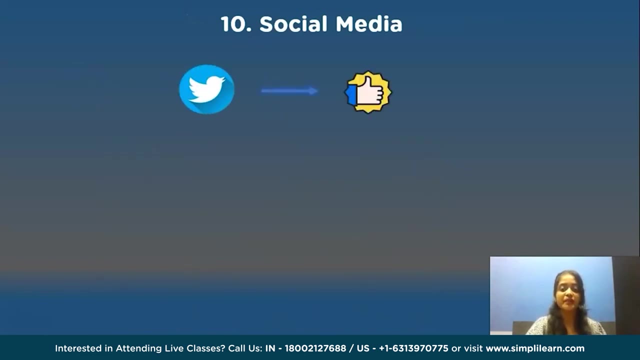 to make the algorithms better so that users can browse photos without relying on tags or other nearby information. It will help to tag people in photos. Twitter Understanding what tweets to recommend to users on their timelines is one of the numerous ways Twitter employs AI on its platform. It seeks to provide users with the most relevant. 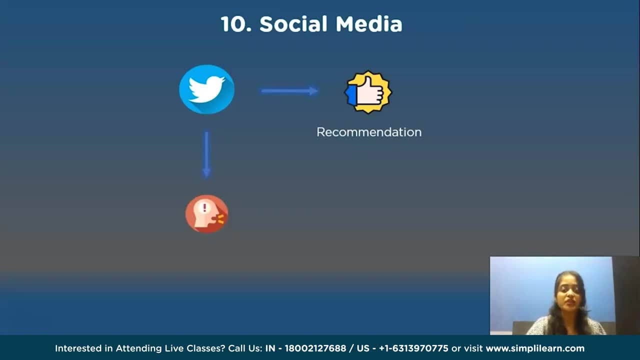 tweets possible for an individual user. The user has access to the Twitter account. Twitter has access to the Twitter account. experience Twitter also uses AI to combat offensive statements. Instagram. artificial intelligence is used by the platform to improve user experience, filters spam and increase the effectiveness of targeted advertising. 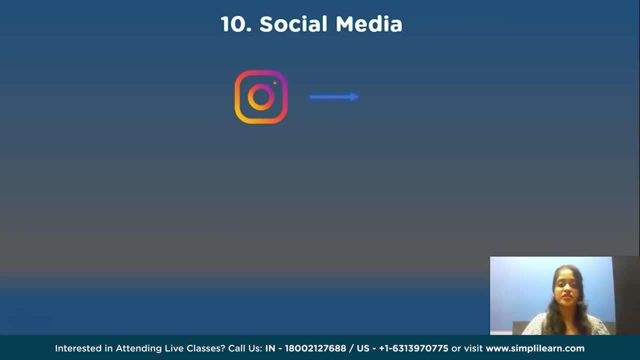 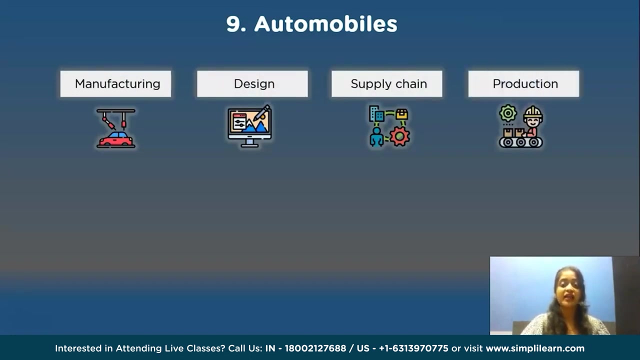 users in the platform can search images of a specific activity, venue, event, restaurant, food and discovery experiences with the aid of tags and trending information. automobiles: the automotive value chain, which includes manufacturing, design, supply, production, post-production, driving assistance and driver risk assessment systems, is successfully implementing artificial intelligence. 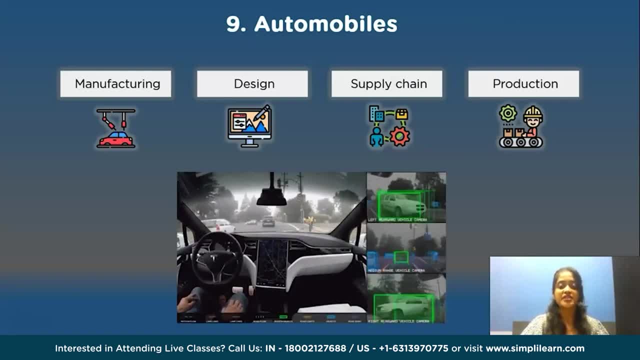 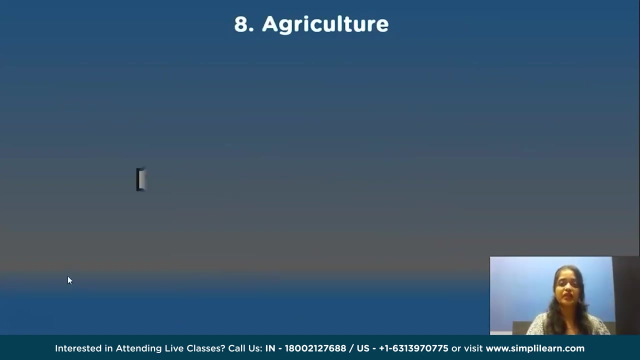 you it. Tesla keeps an eye on the driver's eyes to detect signs of drowsiness and keep them from dozing off while operating a vehicle. it is primarily used by the autopilot system to stop drivers from taking quick power naps while driving agriculture. Forbes reports that global spending on smart agriculture 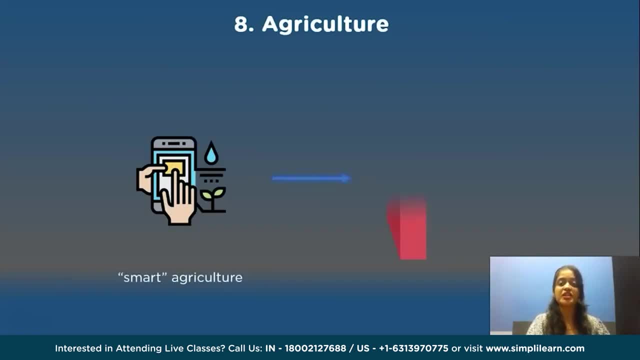 including artificial intelligence and machine learning. you is projected to triple to 15.3 million dollars by 2025. precision agriculture, often known as artificial intelligence systems, is assisting in enhancing the overall quality and accuracy of harvest. artificial intelligence technology aids in the detection of pest plant diseases and under nutrition. informs artificial 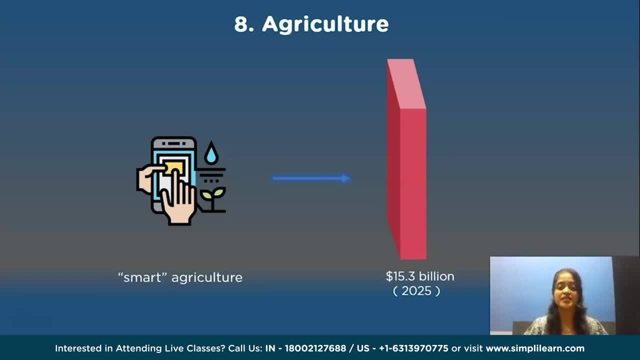 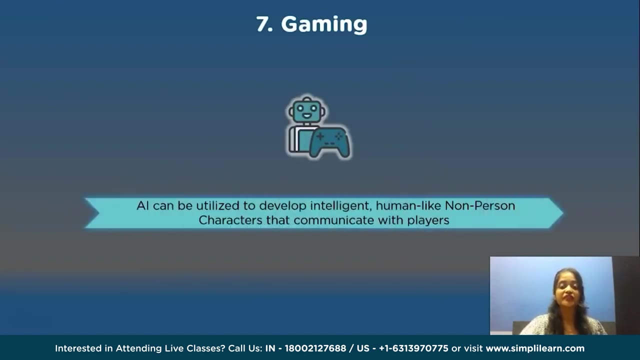 intelligence sensors can identify and target plants for resistant diseases, such as before deciding which herbicide to use. in the area Artificial intelligence in gaming: The gaming industry is another area where artificial intelligence technologies have gained popularity. Artificial intelligence can be utilized to develop intelligent, human-like, non-person characters that can communicate with the players In order to 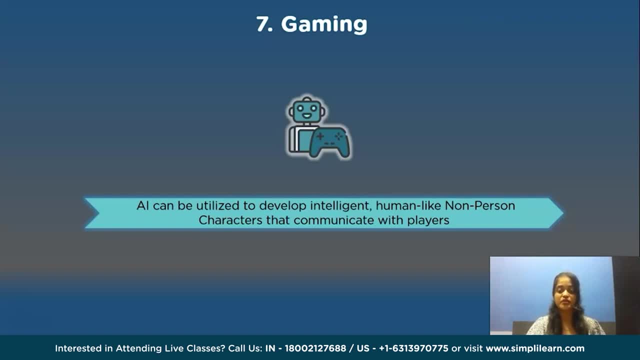 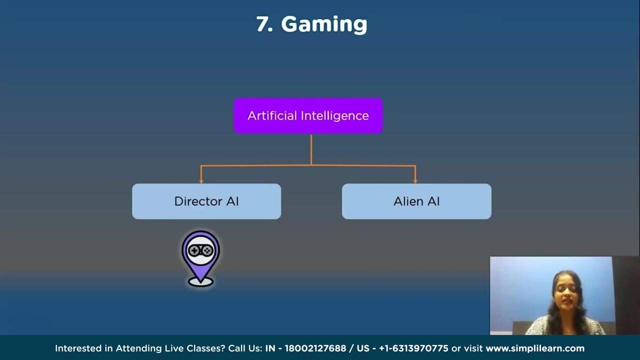 improve game design and testing. it can also be used to forecast human behavior. The 2014 alien isolation video game employ artificial intelligence to follow the player around all the time. Two artificial intelligence systems are used in the game. One is the director, artificial intelligence, who frequently knows where you are, and the 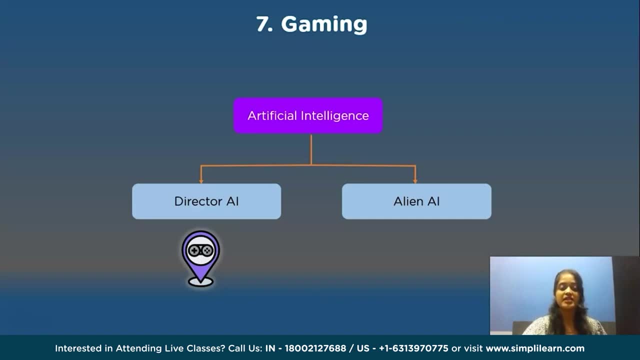 alien artificial intelligence which is controlled by sensors, behaviors and constantly changes the player. next comes artificial intelligence in healthcare. delays can be the difference between life and death in the healthcare industry. artificial intelligence in healthcare has the potential to help providers in many areas of patient care and operational procedures, enabling them to build on current solutions and solve problems quickly. 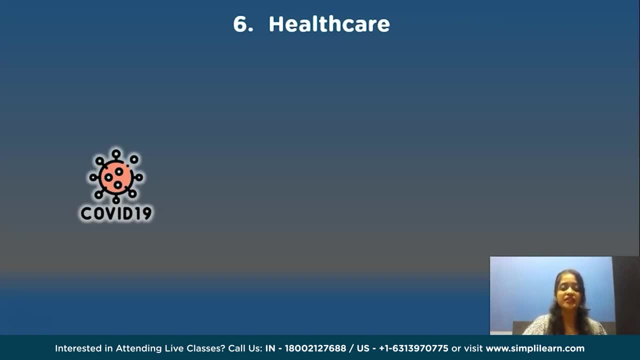 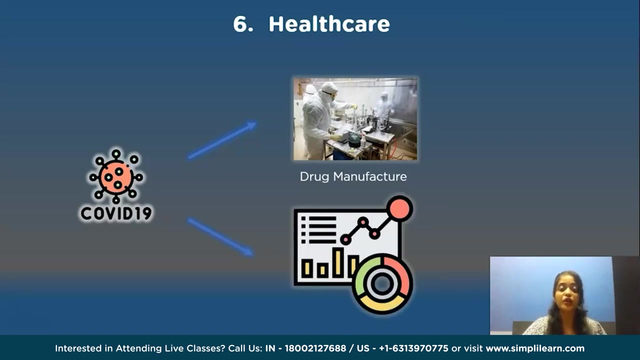 covid 19 has illuminated the process of developing vaccine. in order to create and test new medicines, drug manufacturers are increasingly turning to artificial intelligence solutions like deep learning. because there are so many potential chemical combinations, creating new medications requires processing a lot of data. artificial intelligence overcomes this difficulty. 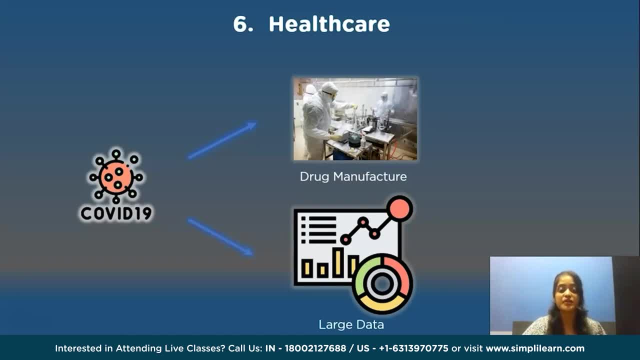 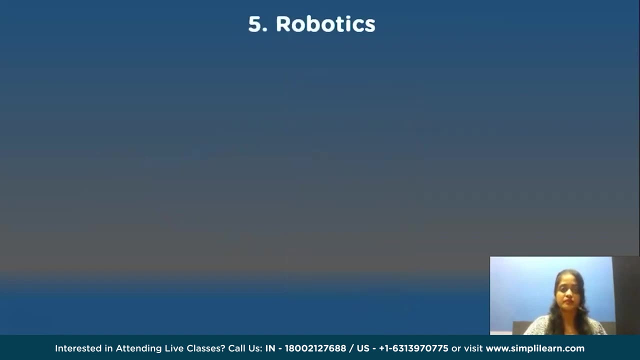 by utilizing artificial intelligence to develop new medicines. its exceptional performance with massive amounts of data. This capability results in a higher production of approved pharmaceuticals in a more rapid, less expensive and more effective research and development procedure. Robotics: Another area where artificial intelligence is frequently. 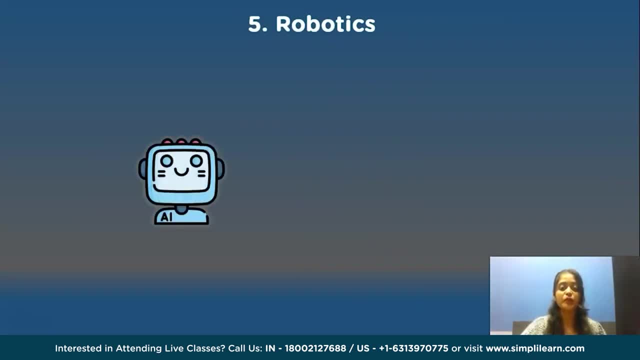 applied is robotics. AI-powered robots employ real-time updates to detect obstructions in their path and instantaneously design their routes. Robotics uses artificial intelligence to make machines more intelligent and capable of acting in variety of situations. Robots can also sense their environment or take in its views with the use of sensor Similar to. 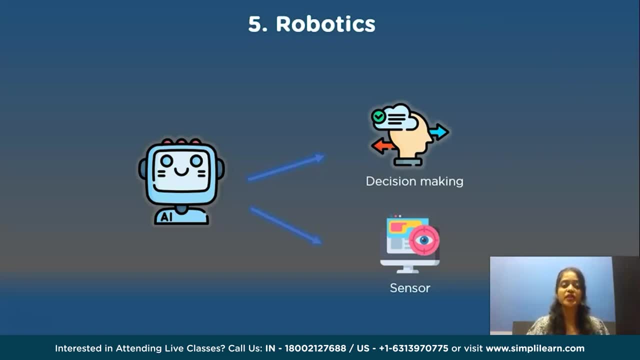 how humans can sense their environment, robots can also sense their environment. Similar to how humans have primary sensors, robotics uses a variety of sensing technology combined. There is a definite trend toward mobile autonomous robots that can intelligently gather, process and manage data in order to make the best decisions for manufacturing or production. 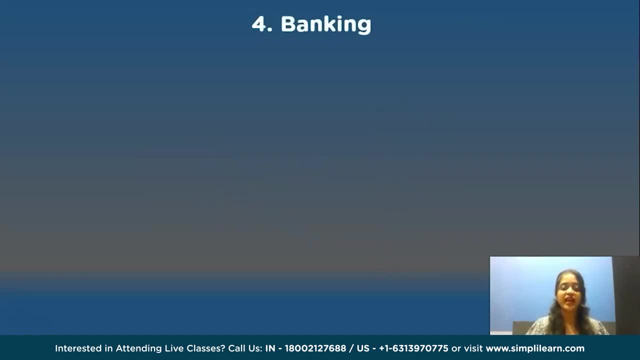 AI in banking. The use of advanced data analytics by artificial intelligence will transform banking in the future by reducing fraud-enhancing compilings. Anti-money laundering tasks that would typically take hours or days can now be completed in a matter of seconds thanks to artificial intelligence algorithms. Erika, a virtual assistant created by Bank of America. 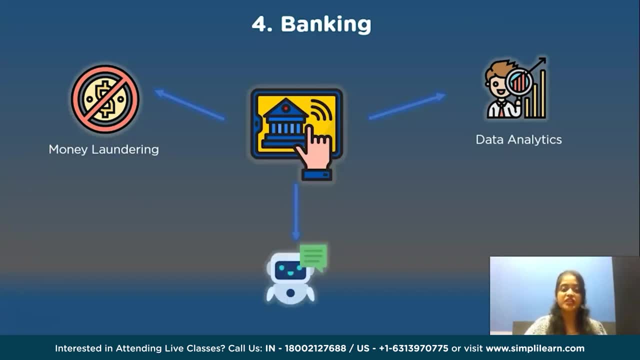 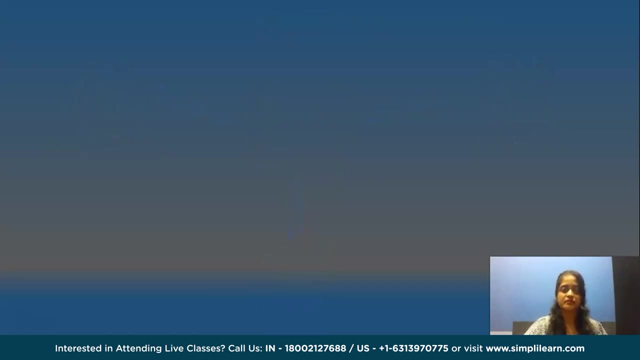 is among the best instances of artificial intelligence chatbots in banking applications. This artificial intelligence chatbot can take care of tasks like updating card security and creating credit card depth. Daily life use of artificial intelligence- Autonomous vehicles To teach computers to think and evolve like humans when it comes to driving in any environment and object recognition. to prevent accidents. companies like Toyota, Porsche, dior, Chargardt, all enableたtoimar driving in their environment and object recognition to prevent accidents. Using autonomous vehicles to produce electronic information about traffic on the roads and street can be used without enjoying the electric vehicle transportation & wet cars, Our eco-pilot mode. segundo, en ser nooni Kemacie. 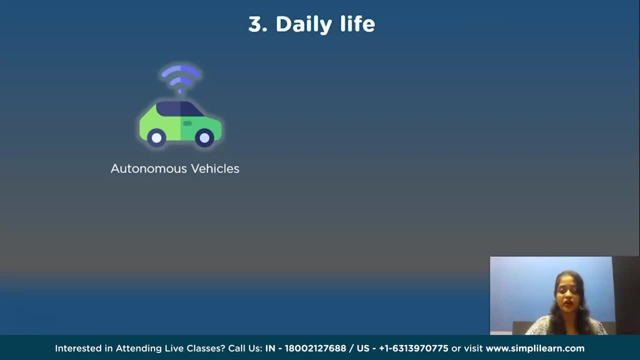 Toyota, Audi, Tesla use machine learning algorithms Spam filters –. The email that we regularly use features artificial intelligence that separates out junk emails and sends it to spam or trash folders, allowing us to see only the filtered material. Gmail, a well-known email service, has achieved a filtration capacity of roughly 99.9%. 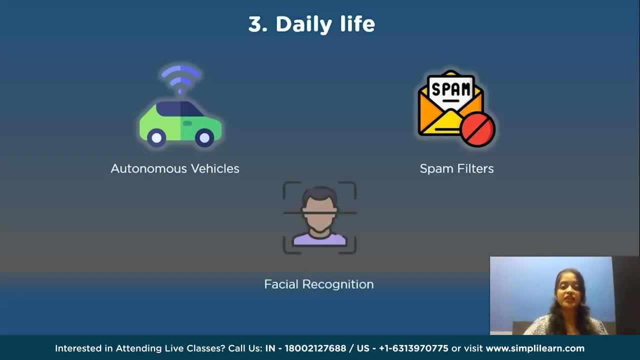 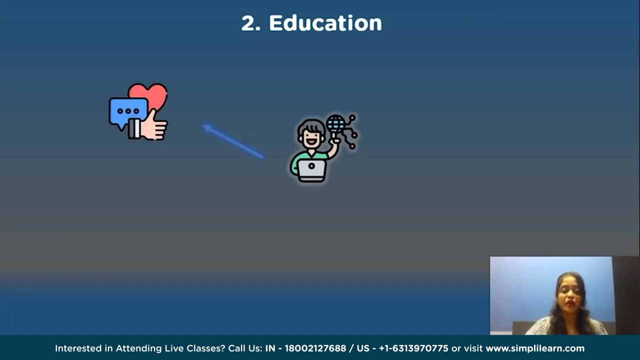 Next comes facial recognition – Facial recognition algorithms are used by our favorite devices, including phones, laptops and personal computers, to detect and identify users in order to grant safe access. Education sector – Artificial intelligence can assist educators with non-educational tasks, such as facilitating and automating personalized messages to students. back-office. 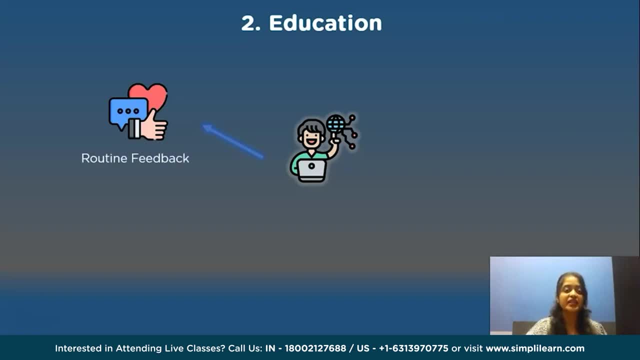 duties such as grading paperwork, organizing and facilitating routine feedback, managing enrollment courses, etc. A student can receive additional learning resources or assistance with voice assistance. even without the need for voice, A teacher can directly engage with the lecturer or teacher. This lowers the expense of producing temporary handbooks and makes it simple to provide answers. 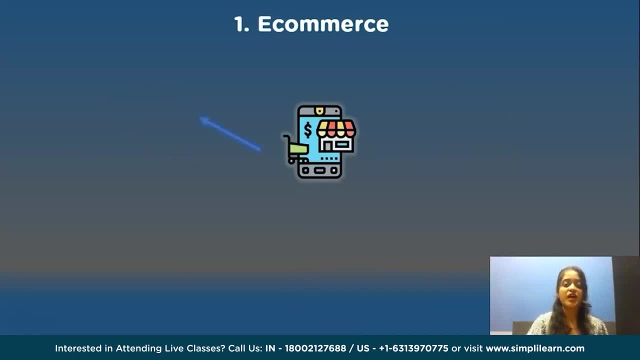 to frequently asked questions. Artificial intelligence is most commonly used in the field of e-commerce. During personalized shopping, recommendation engines are made possible by artificial intelligence technologies, allowing you to interact with your customers more efficiently and easily. The latest technology in email is a search engine. 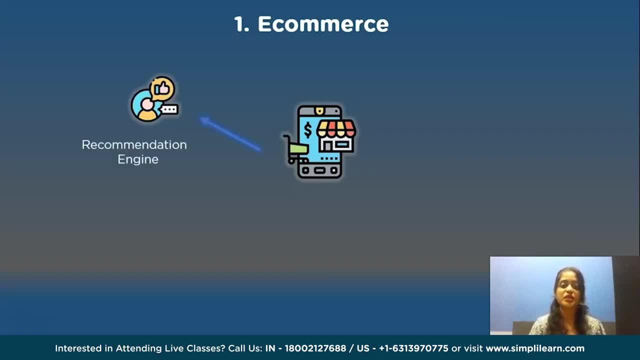 It is designed for accounts to search through emails and emails On the Internet. the search engine uses a search engine to search and find out direct information about users and customers who use it on a regular basis. The search engine is also designed to search lurid pages on e-commerce websites such as Facebook. 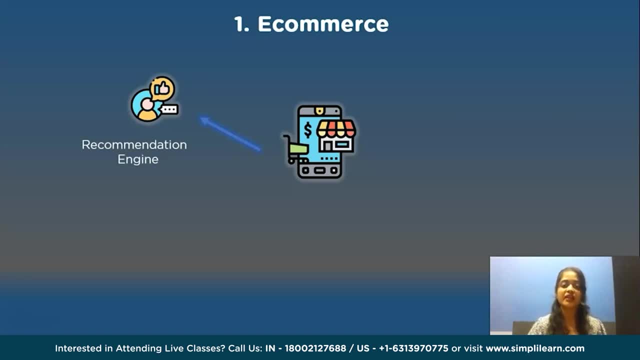 and Tweet Google and Facebook effectively. Their browsing history, preferences and interests are taken into consideration while making these recommendations. It helps you build stronger bonds with your clients and increases brand loyalty. For instance, almost every page of Amazon's website offers personalized product. 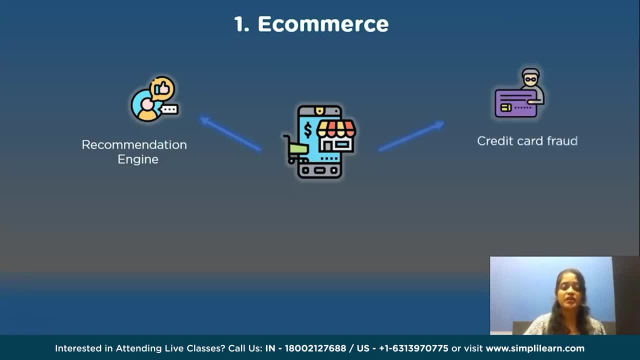 recommendations. Credit card frauds- fake reviews are two most of the significant issues that e-commerce companies deal with. By considering the usage patterns, artificial intelligence can help reduce the possibility of credit card frauds taking place. Many customers prefer to buy a product or service based on customer reviews. Artificial intelligence can identify and handle. 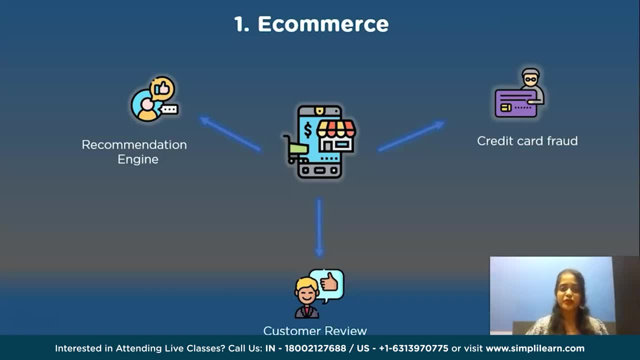 fake reviews. What is the answer to the question that I have asked about artificial intelligence assistance? They can be Google Assistant, Siri, Alexa, etc. In the area of artificial intelligence, significant advancements have been made and the results are clear. AI is a flexible tool that is applied across sectors to improve. 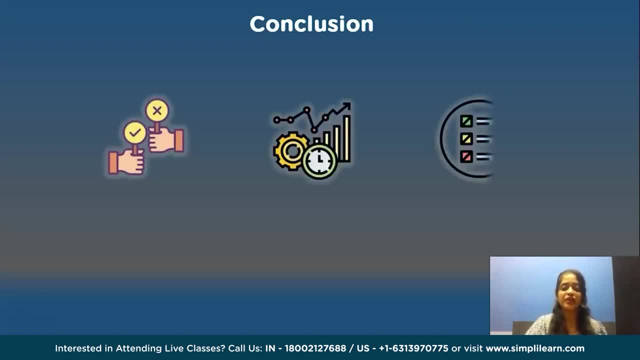 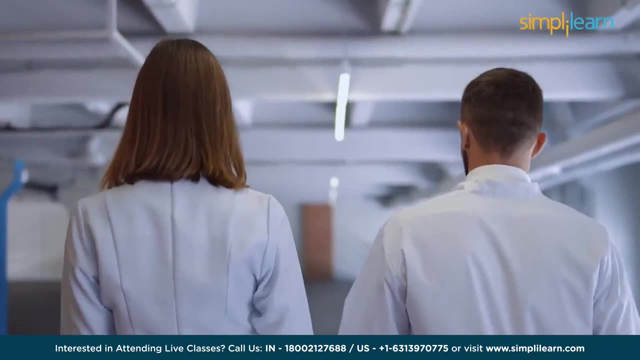 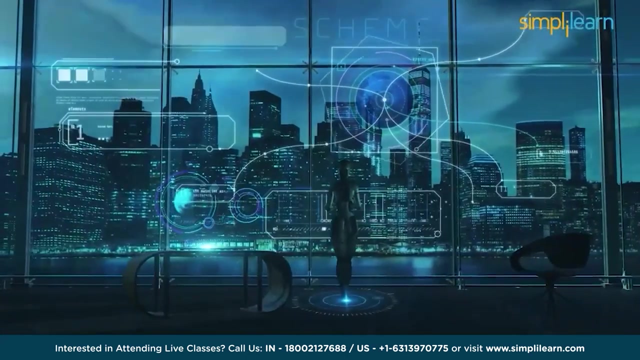 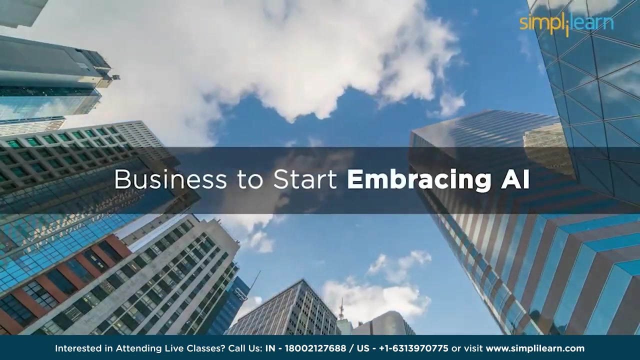 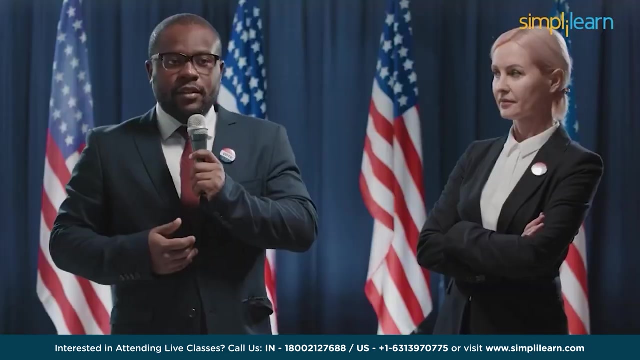 decision-making, boost efficiency and get rid of repeated tasks. AI can work바 лар AI. AI is a flexible tool that is applied across sectors to improve decision-making, boost efficiency and improve decision-making. AI can farm мог 賀. 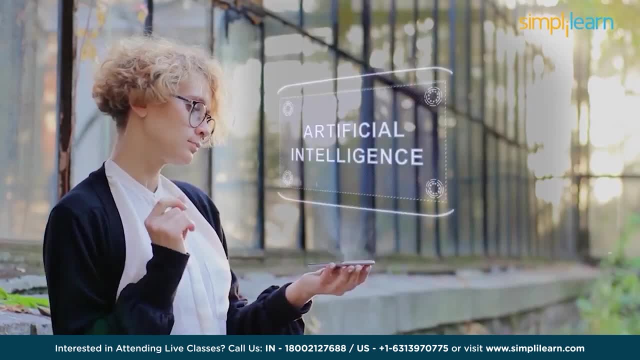 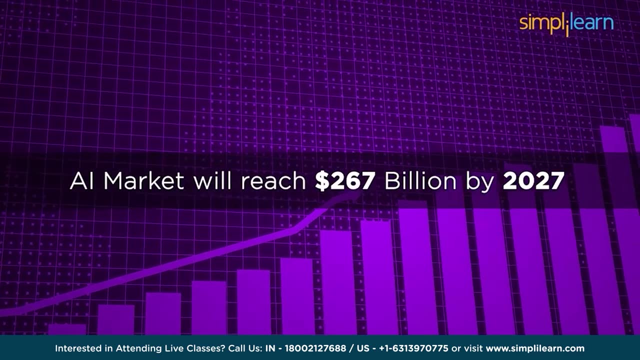 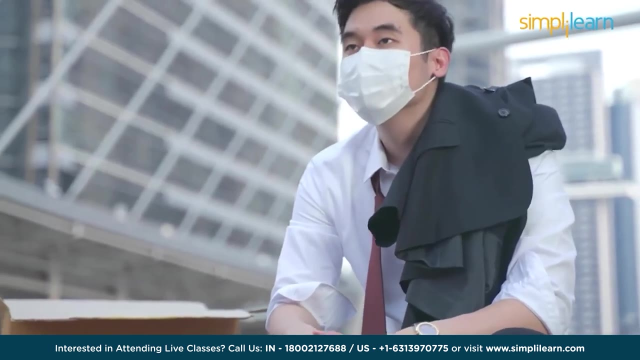 Although it could be risky, it's also a fantastic opportunity. It is estimated that the global artificial intelligence market will reach $267 billion by 2027.. People are worrying about losing their jobs as AI continues to advance, because it has revolutionized industries across all sectors. 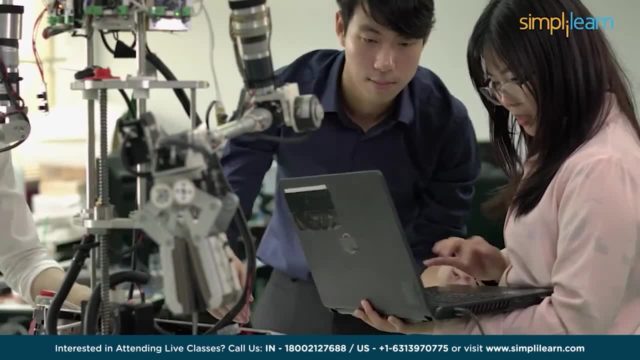 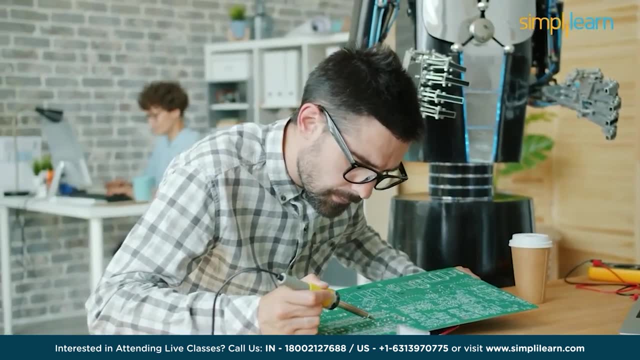 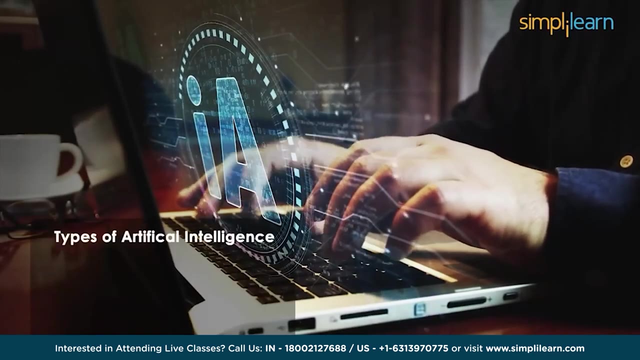 But AI has increased the number of jobs and possibilities available to individuals across all industries. Every machine needs a person to run it. Although AI has replaced certain occupations, it still creates more jobs for humans. AI can be categorized into three types. Firstly, weak AI performs specific tasks, like Apple's Siri. 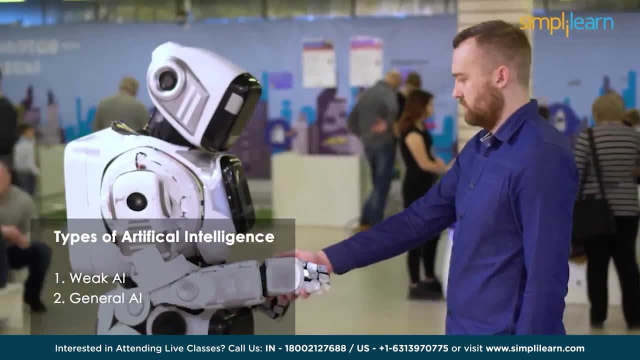 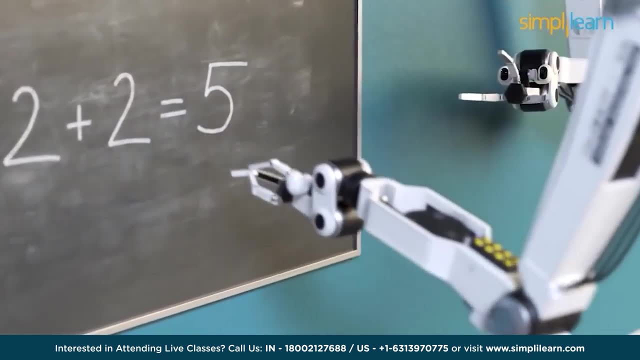 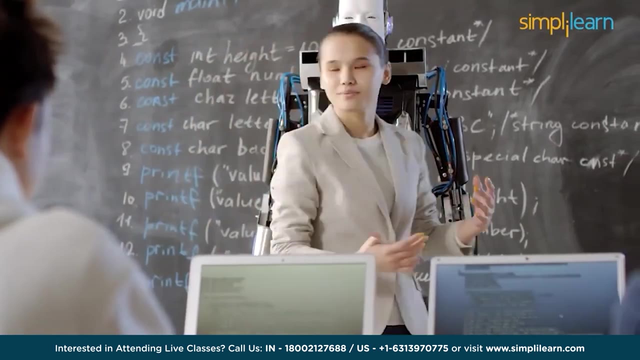 General AI performs tasks like a human. Super AI is more capable than a human, But both general AI and super AI are hypothetical and they are not yet developed, and research is going on. However, the development of such AI will take a lot of time. 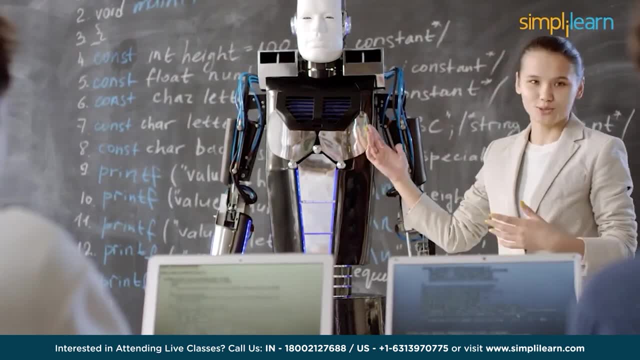 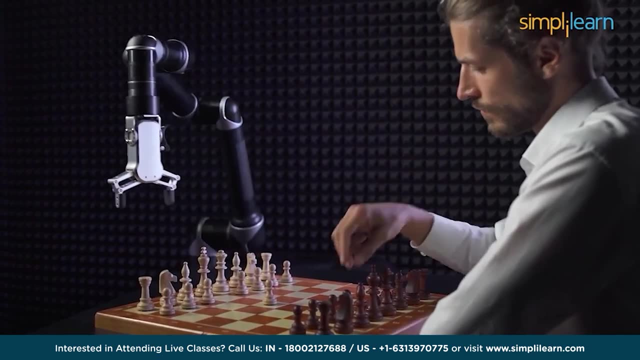 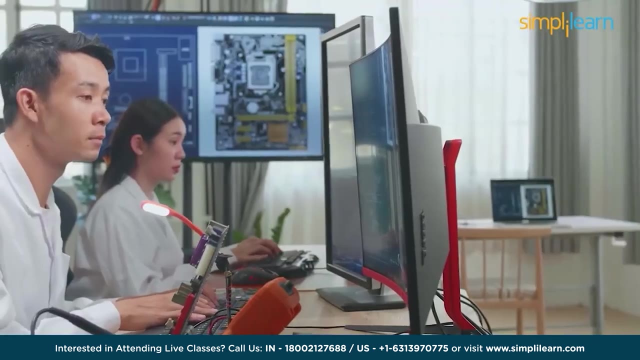 The development of AGI will accelerate within the following 10 years. In fact, according to researchers, there is a 25% probability that by 2023, AI will resemble humans when it comes to thinking capacity. Additionally, the current data boom, computer developments, 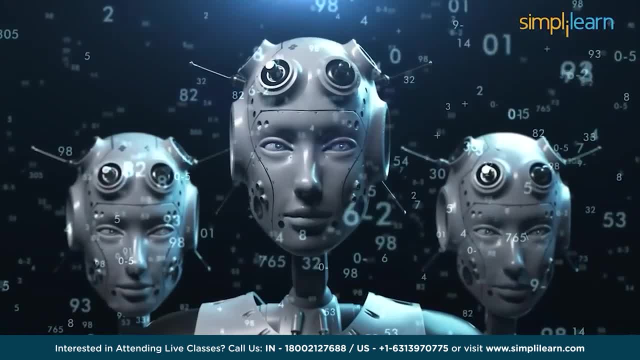 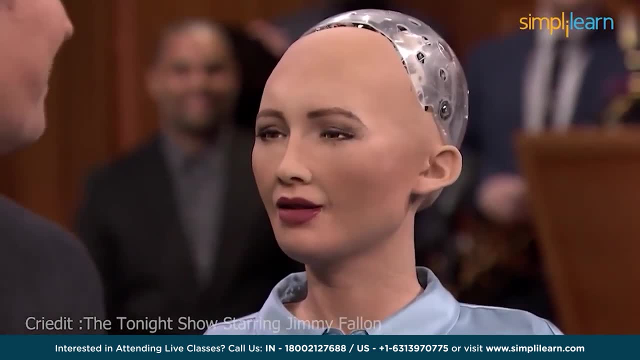 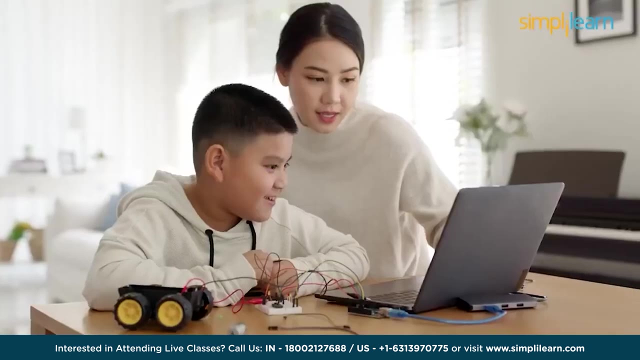 and improvements in automated methods and machine algorithms will provide a lot of room for AI to develop. AI will provide a solid foundation for platforms with human-level AI. AI has occupied crucial sectors like healthcare, cybersecurity, e-commerce, agriculture, robotics, education. 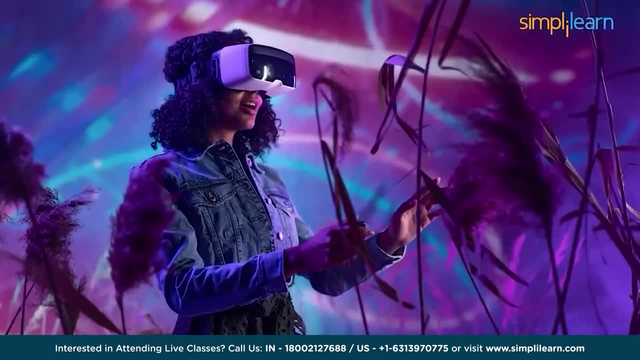 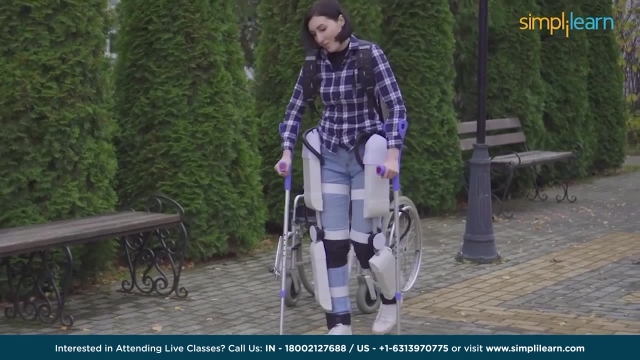 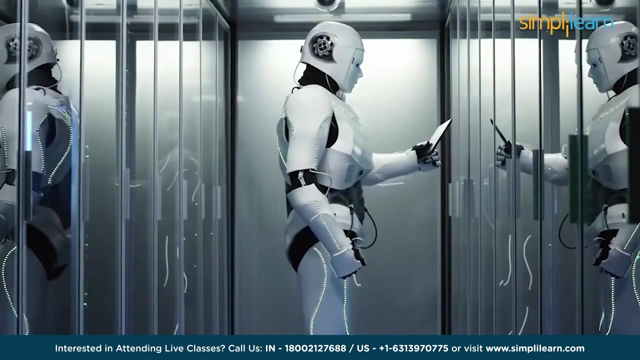 the military system, finance gaming and many more. AI is used in healthcare to identify diseases, helping healthcare service providers and their patients make better treatment and lifestyle decisions. We can say that without AI we couldn't have made the incredible recent advancements in fields like robotics. 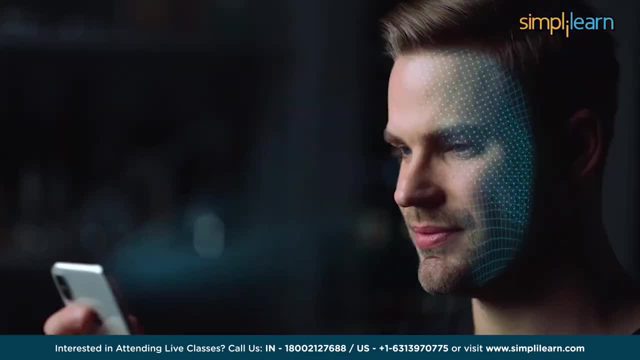 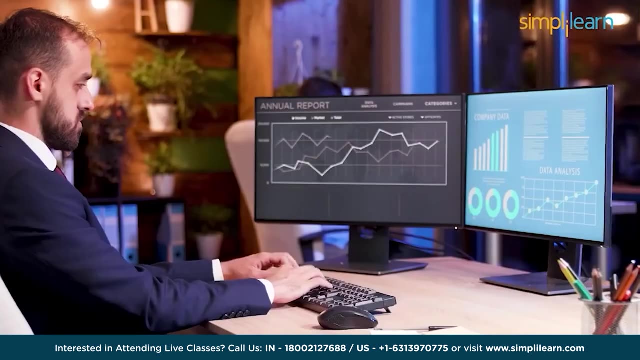 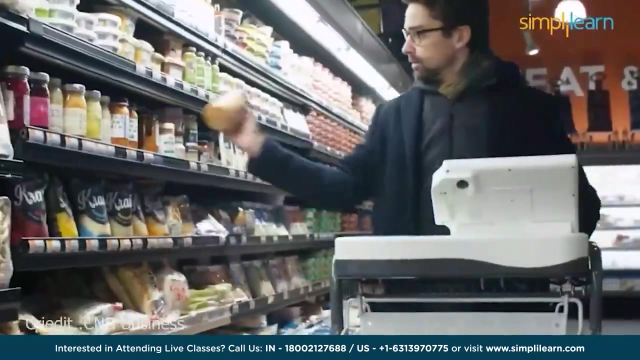 virtual reality chatbots, face recognition and autonomous vehicles, Smart robot advisors in finance, insurance, legal media and journalism will deliver instantaneous research or discoveries. In the upcoming years, it is anticipated that artificial intelligence and machine learning will become more prominent in the consumer market. 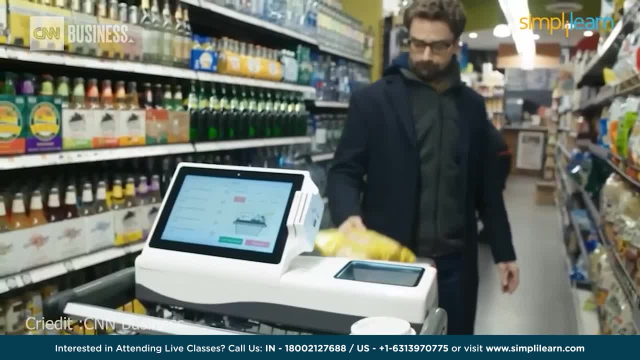 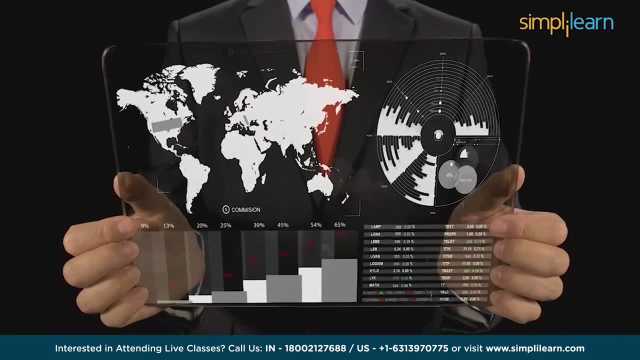 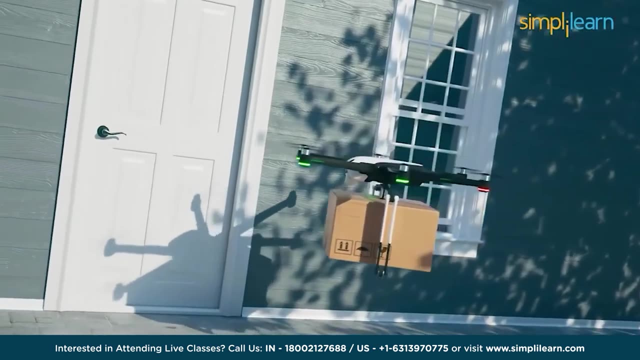 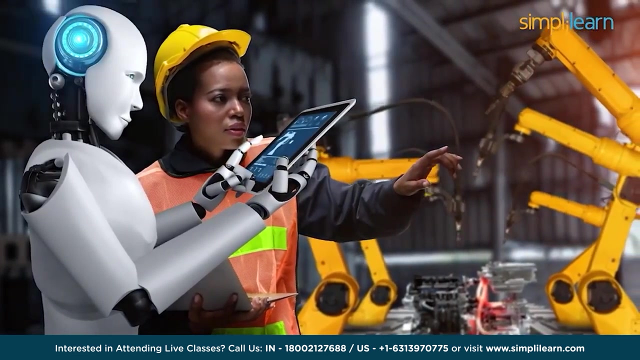 which will immediately affect how well web development functions. Virtual assistants, or chatbots, will provide professional advice. Other advantages include strengthening governance through better decision-making processes, shortening time to market for R&D initiatives, and streamlining transportation and supply chain networks. Given all these scenarios, AI is all set to revolutionize every sector in the near future. 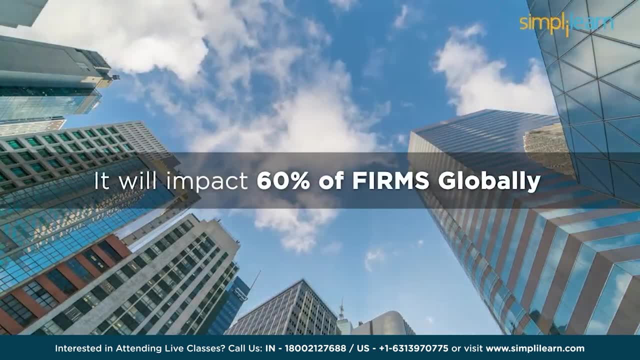 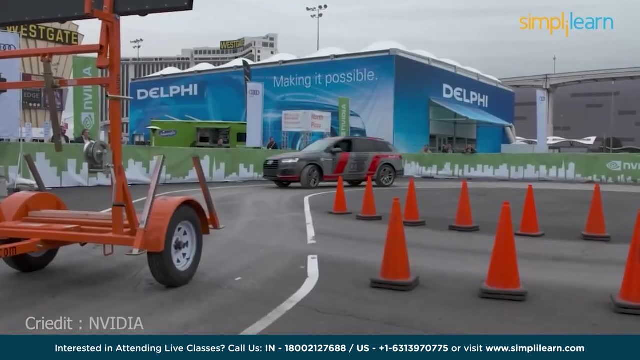 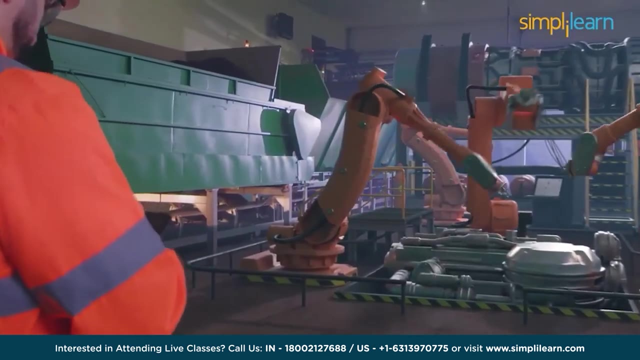 Given that it is expected to impact 60% of firms. artificial intelligence will continue to spread deeper into a wide range of industries in the upcoming years. It is currently driving development in our smart devices, cars and favorite apps. In the coming years, AI will invade every aspect of our life and eventually surpass human. 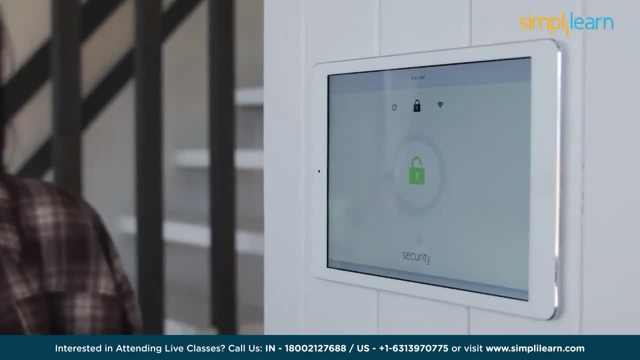 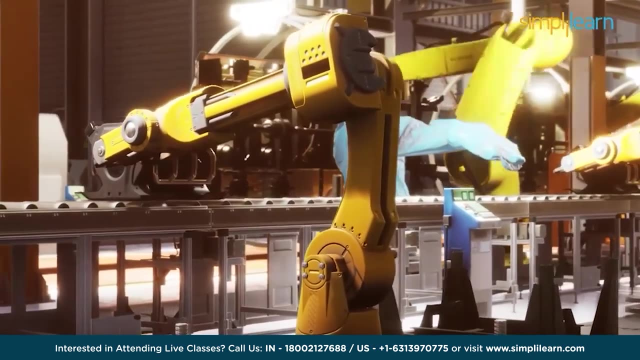 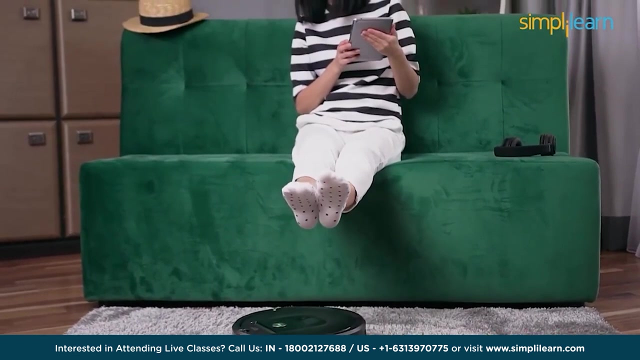 intellectual capacity. It won't be long before artificial intelligence becomes a common part of our everyday lives. As it becomes more prevalent, it will allow us to live more efficiently and improve our lives By increasing their effectiveness, efficiency and concentration on the primary tasks that require. 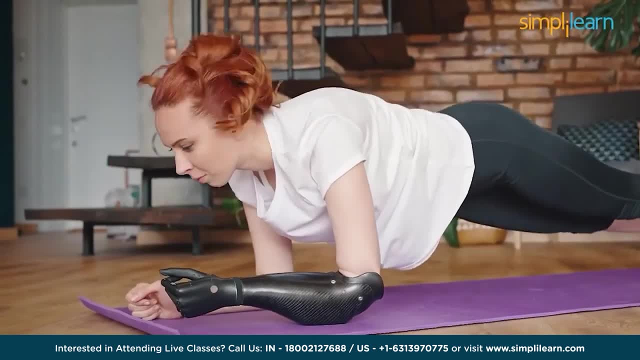 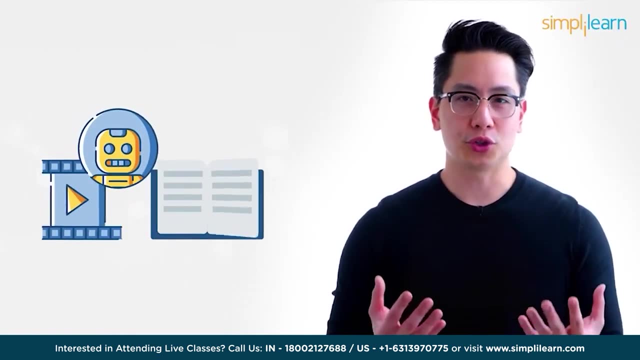 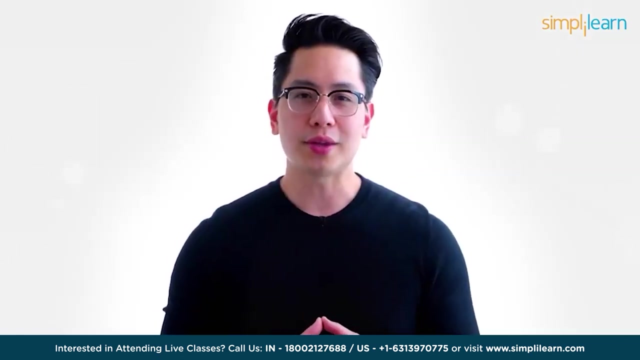 people's attention. AI technologies are transforming many industry sectors. Artificial intelligence will change the world for the better. Sci-fi movies and books depict a future with sentient machines capable of interacting with humans and performing tasks just like people would. What if we told you that this future? 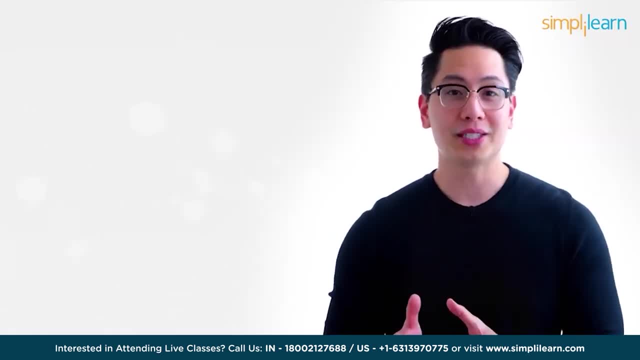 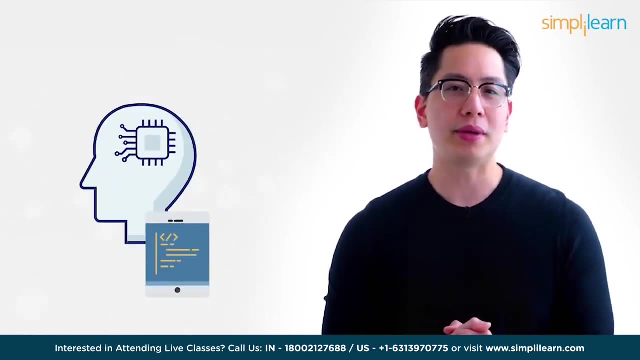 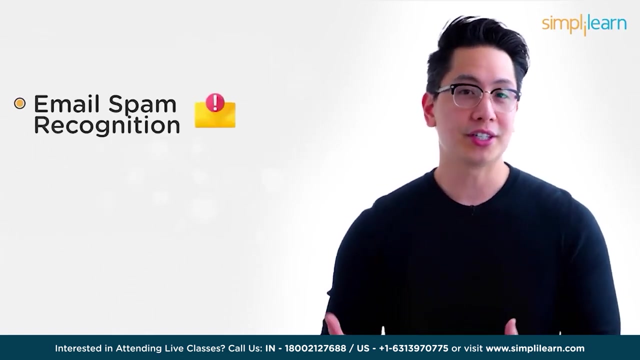 is already a reality. All of this is already made possible by machine learning. Machine learning is the science of programming machines to think and act like humans without being specifically programmed to. We already use machine learning in our daily life without knowing it. E-mail, spam, recognition. 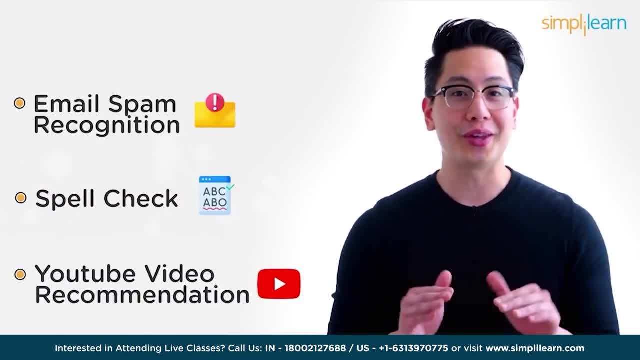 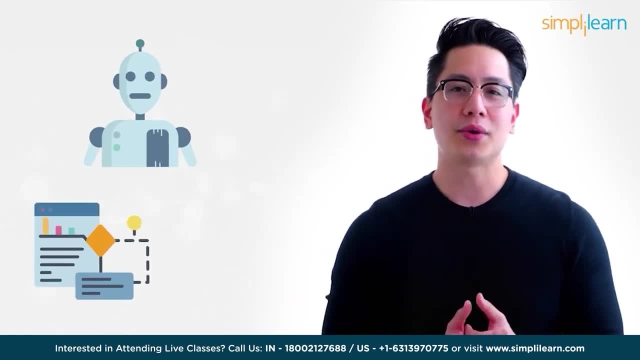 spell check and even the YouTube video recommendation which brought you here are implemented using machine learning. Machine learning uses algorithms to learn tasks. These algorithms are fed with data from which they learn to perform tasks. This means that over time, as changes in data occur, we don't need to use machine learning to operate our digital drawing, but to do so, we need to learn how to use the machine learning technology. Machine learning is a technology that we need to use in the real world. We only need to know how to use the software we are using. If you are a computer, you won't be able to master all the tasks that we are using. 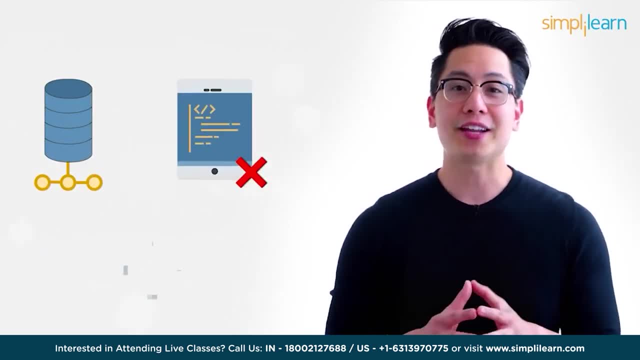 but you can use machine learning to learn how to use the software that you are using, which means that we don't need to reprogram our application. Just let it find patterns and learn from the new data. Machine learning is a subset of artificial intelligence. 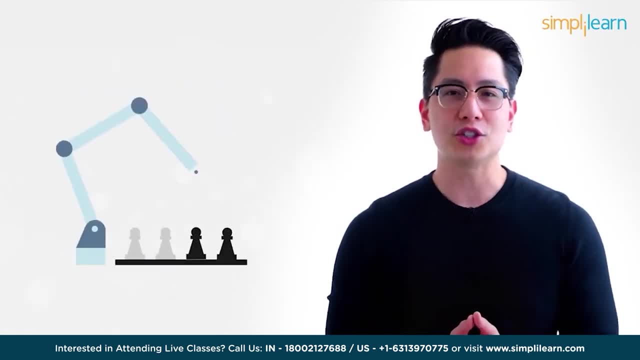 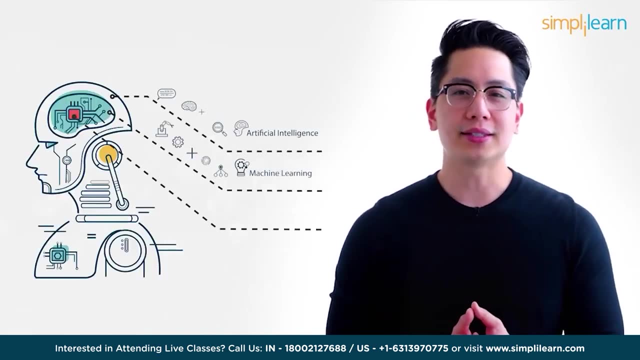 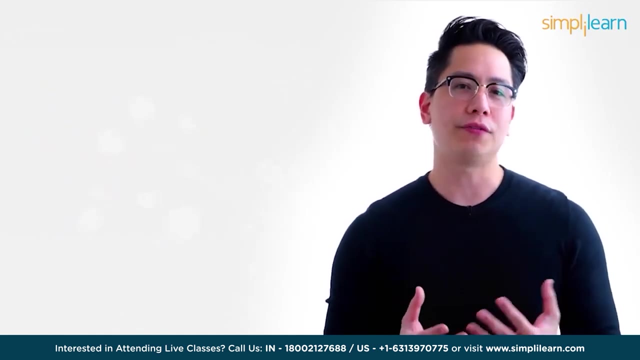 which is a science concerned with imparting human-like intelligence onto machines and creating machines which can sense, reason, act and adapt. Deep learning is a sub-branch of machine learning which is inspired by the working of the human brain. Machine learning is leading us to a future. 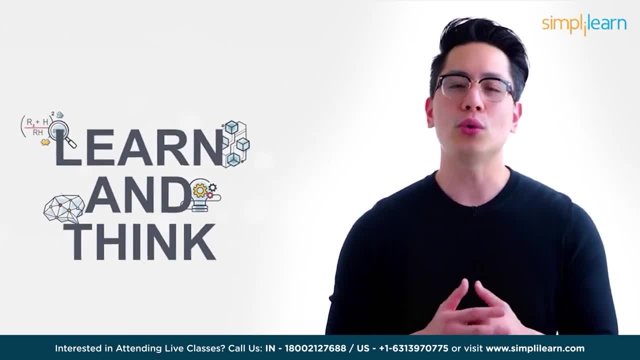 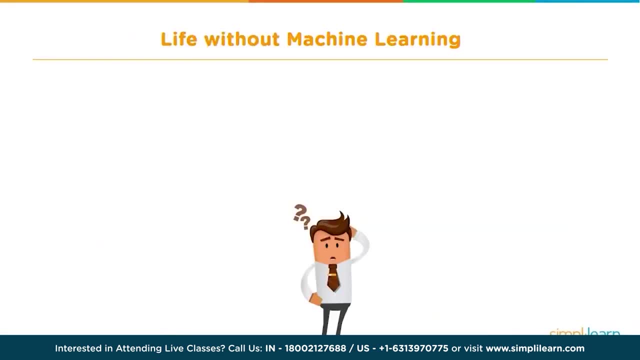 where machines can learn and think, and has opened us a whole new plethora of job opportunities. This was a brief intro to machine learning. Let's talk about a life without machine learning For someone who doesn't know anything about machine learning or artificial intelligence. 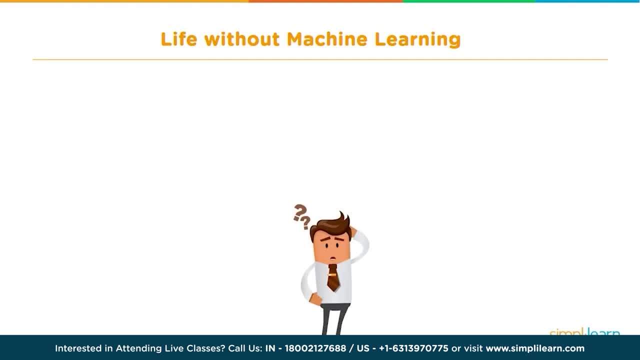 he or she might think that it is only being used in robots or machines and stuff, which is actually true, as portrayed by most of the sci-fi movies nowadays. But you wouldn't believe how much more machine learning is giving us, how much of it we are using in our daily lives. 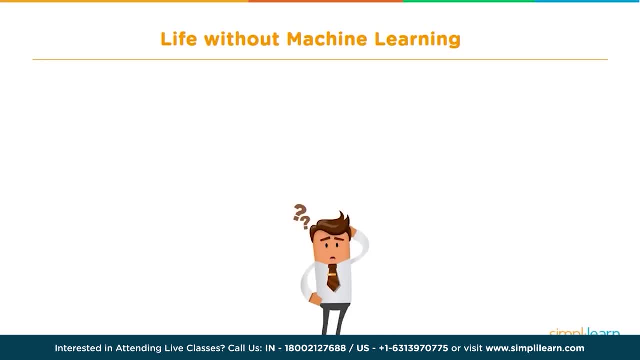 Let's say you need information on any random topic, say a computer, The first place you would check would definitely be Google, right? It would collect all the information on the word you search for and present it to you according to relevance. If there was no Google, 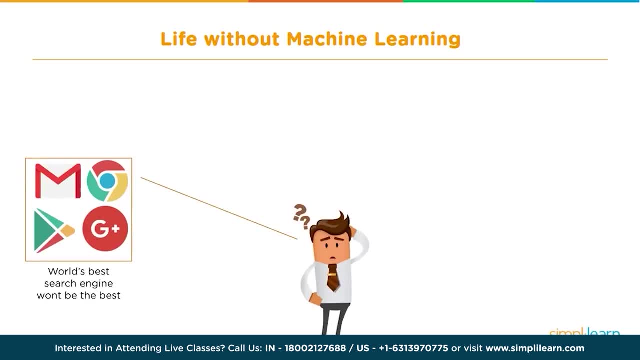 you would have to do it in a very hard way, that is, by going through tens or hundreds of books and articles, even after which you won't find the answer. If we go back four to five years, facial recognition would be a thing only shown in movies. 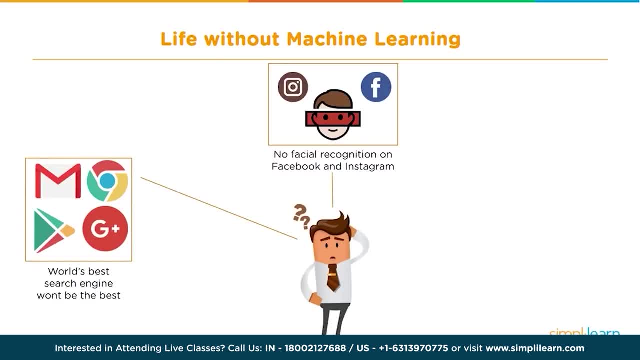 like Mission Impossible or Terminator or any of the sci-fi movies you pick, But machine learning has made it possible for Facebook and Instagram to use this feature for your benefits. You don't have to go through the trouble of tagging every single person present in a picture that you have posted. 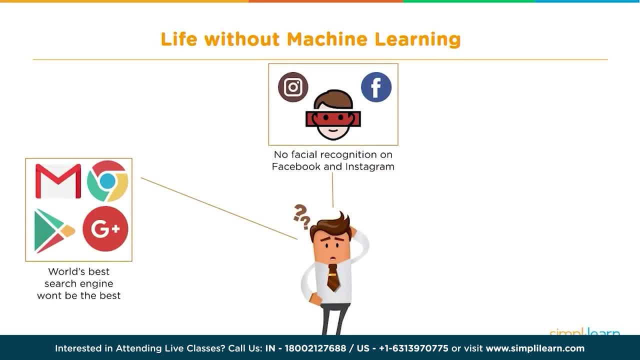 Facebook will automatically recognize the people in the photo and tag them for you. That saves a lot of time for you, doesn't it? Also, Siri, Cortana, Iris, all of them would not be there to help you if there was no machine learning. 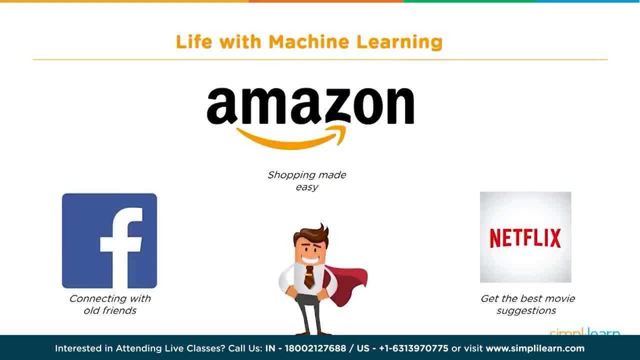 Now that we know life would be a lot more difficult without machine learning, let's look into the things that are run by machine learning and we are using them on our daily basis. Let's enter the world of gaming. PS4s and Xboxes have introduced virtual reality glasses. 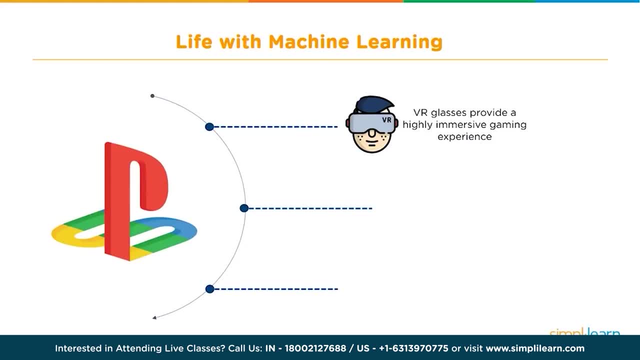 which brings a whole new level of detail into gaming. Every time your head moves in real world, it replicates the movement in the virtual world, providing an excellent gaming experience. Then there is gesture control gaming, wherein machine learning tracks your body movement and makes a corresponding movement in the game. 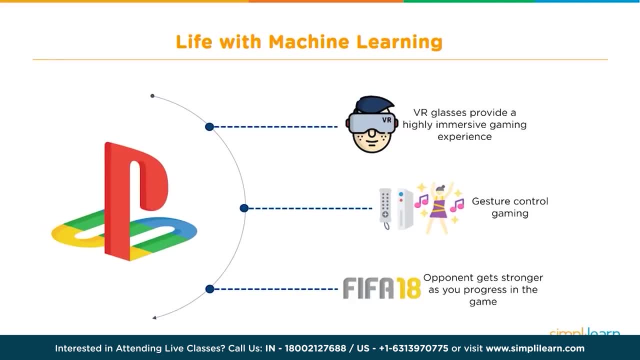 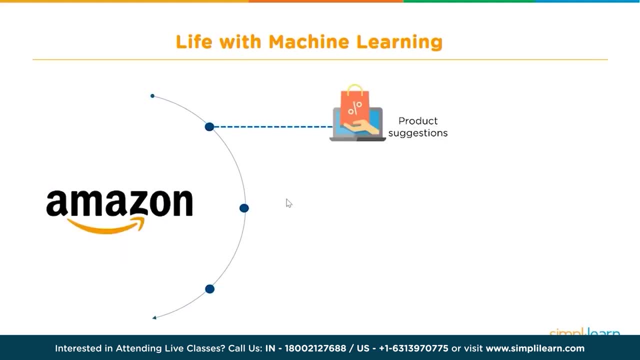 Finally, in the game FIFA, your opponent tends to adapt based on the kind of strategy or gameplay you follow. That is again done by machine learning. I'm sure you must have shopped a lot from Amazon, So let's look into some of the places Amazon makes use of machine learning. 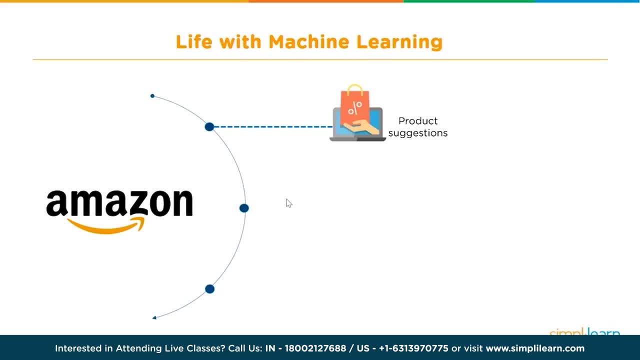 Let's say you buy a formal t-shirt on Amazon. As you buy it, it suggests you formal shoes, ties, blazers and apparels that go with what you have bought. That's the recommendation system powered by machine learning. again, The price on every product that you see on Amazon is varying every moment based on demand. 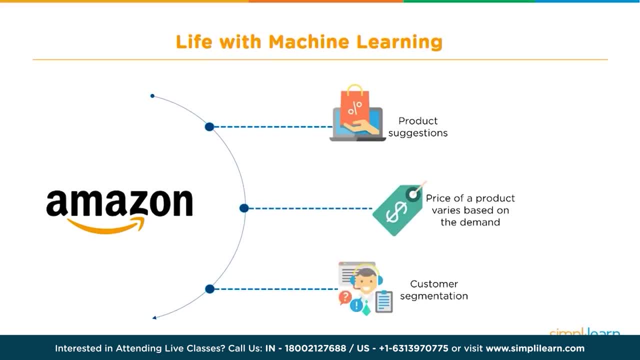 That's being done by machine learning algorithms. Then comes customer segmentation. Customer segmentation is one of the most crucial thing for all the e-commerce platforms. Machine learning helps them differentiate between customers based on what they buy, how frequent are they, and their reviews. 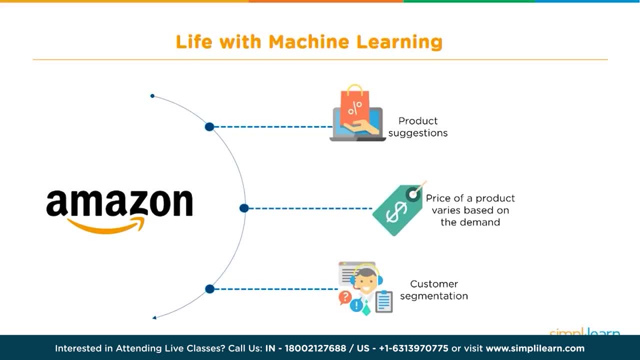 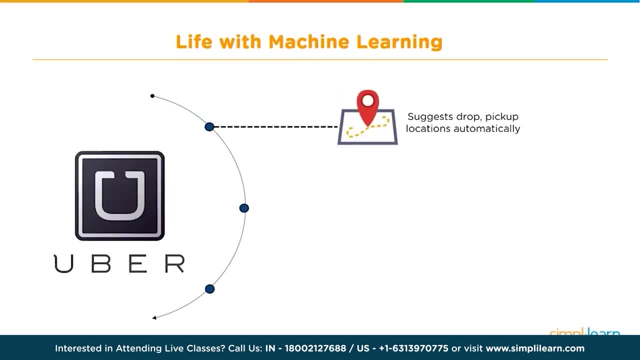 This helps the companies to make sure that their customers are taken care of and their needs are being fulfilled. Now let's talk about an app that you use on a daily basis to reach office on time. Yes, it's Uber cabs. Once you have traveled with Uber, 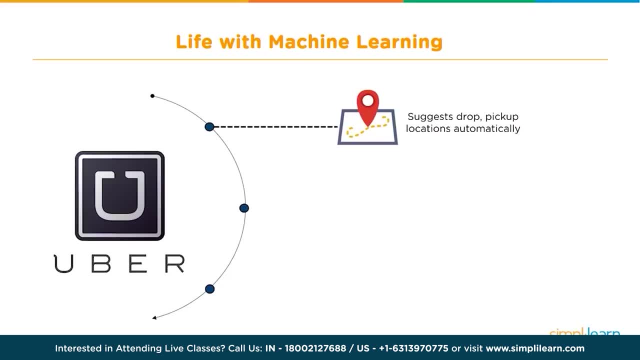 you must have noticed that it suggests you the places you might want to go, based on your previous journeys. When you're taking a share, how does the app make sure that the cab you get is traveled by the same route you want to travel in? 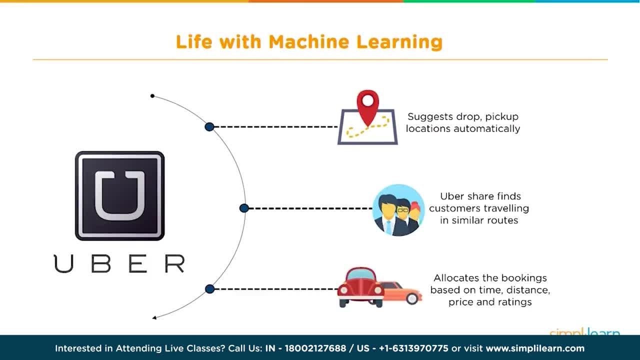 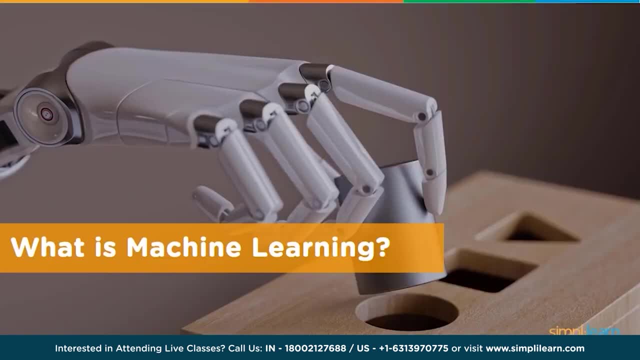 There are so many factors, like the distance, the traffic, the ratings- All of it is taken care of by machine learning. For the past five minutes, we have been talking about how machine learning is improving our lives, where all it is being used. 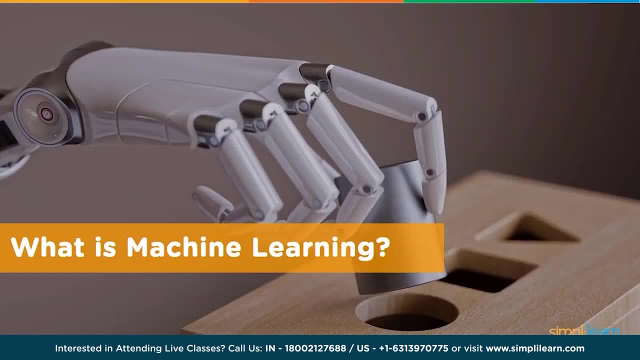 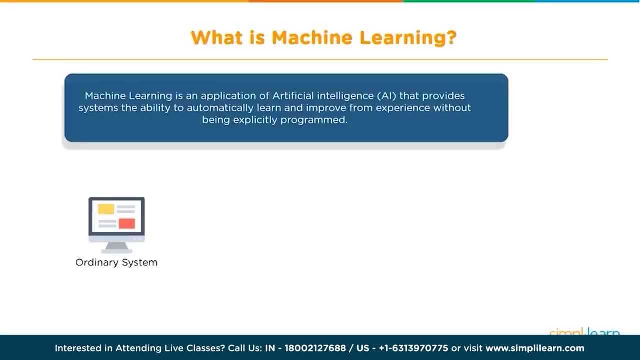 I have probably said machine learning a hundred times already. I think it's about time that I tell you what machine learning actually is. Let's take an ordinary system that you currently are using. It can't do much except from the basic operations that you already know about. 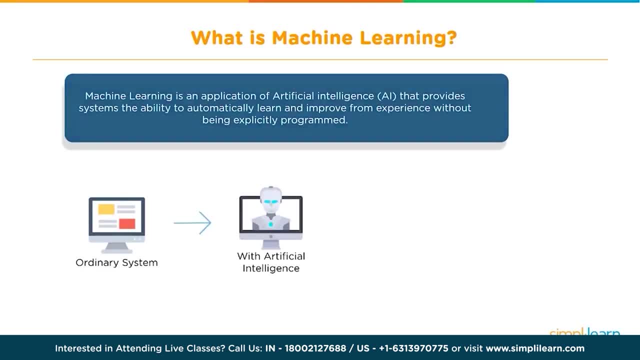 Now let's add artificial intelligence or, for a layman's point of view, let's give the same machine the power to think on its own. That is what machine learning basically is. It's an application of artificial intelligence that provides systems the ability to learn on their own and improve from experience, without being programmed externally. 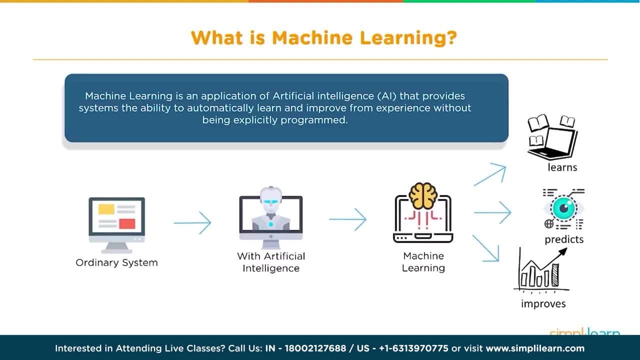 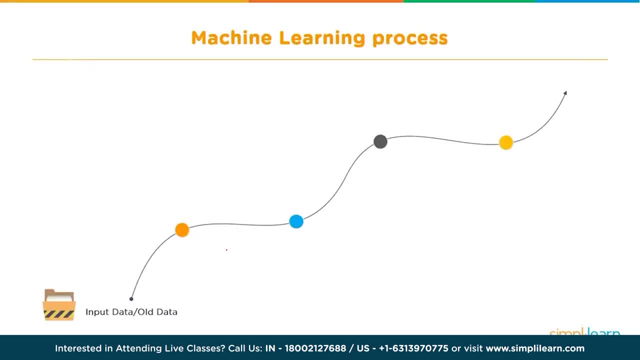 So if your computer had machine learning, it may be able to play the difficult parts of a game for you or probably solve a complicated mathematical equation for you. That could be really helpful. Let's dive in a little deeper and see how machine learning works. 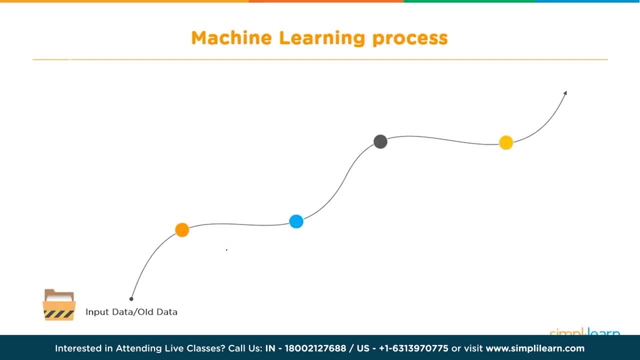 Let's say you provide a system with the input data that carries the photos of various kinds of fruits. Now you want the system to figure out what are the different fruits and group them accordingly. So what the system does? it analyzes the input data. 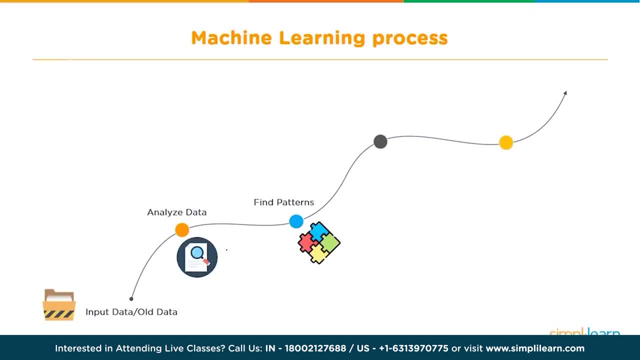 Then it tries to find patterns, Patterns like shapes, size and color. Based on these patterns, the system will try to predict the different types of fruit and segregate them. Finally, it keeps track of all such decisions it took in the process to make sure it's learning. 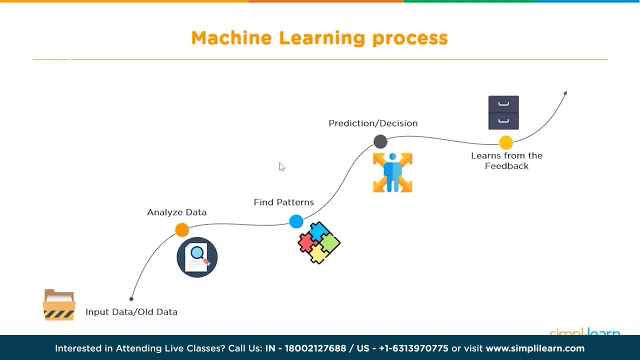 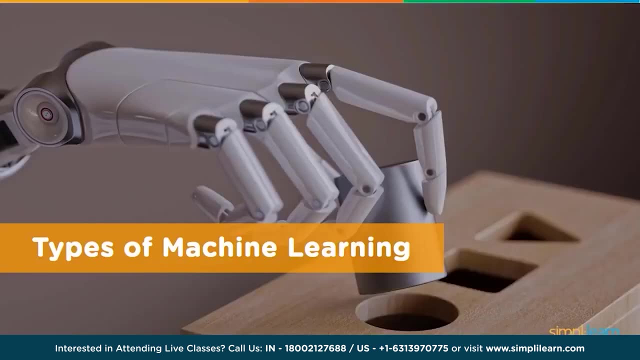 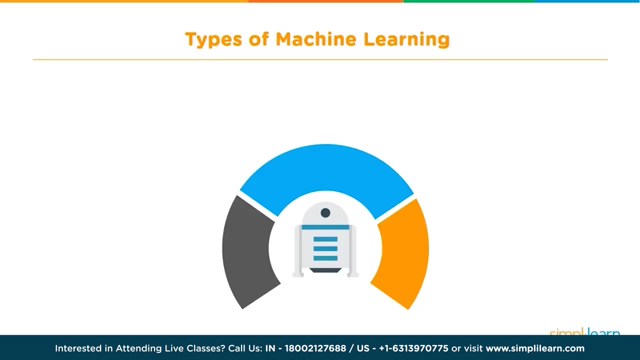 The next time you ask the same system to predict and segregate the different types of fruits, it won't have to go through the entire process again. That's how machine learning works. Now let's look into the types of machine learning. Machine learning is primarily of three types. 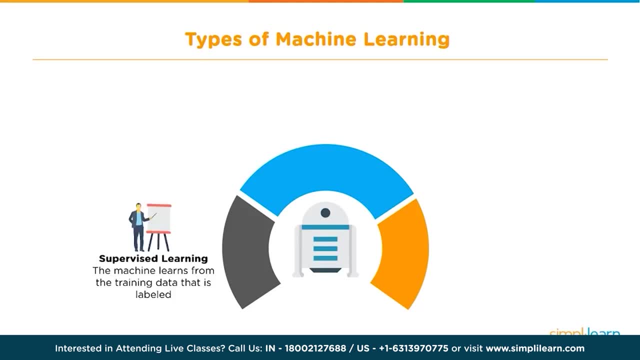 First one is supervised machine learning. As the name suggests, you have to supervise your machine learning while you train it to work on it. It requires labelled training data. Next up is unsupervised learning, wherein there will be training data but it won't be labelled. 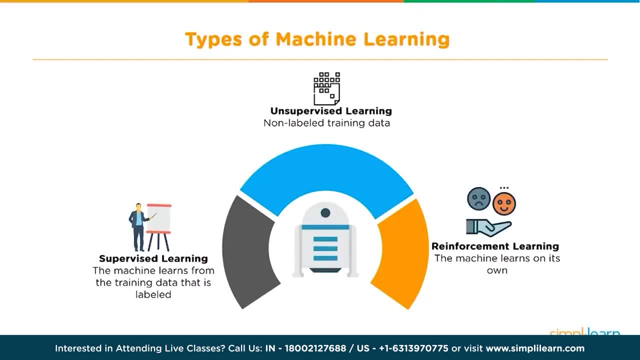 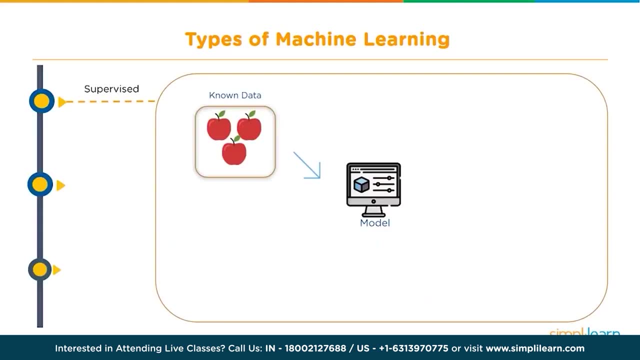 Finally, there is reinforcement learning, wherein the system learns on its own. Let's talk about all these types in detail. Let's try to understand how supervised learning works. Look at the pictures very, very carefully. The monitor depicts the model or the system that we are going to train. 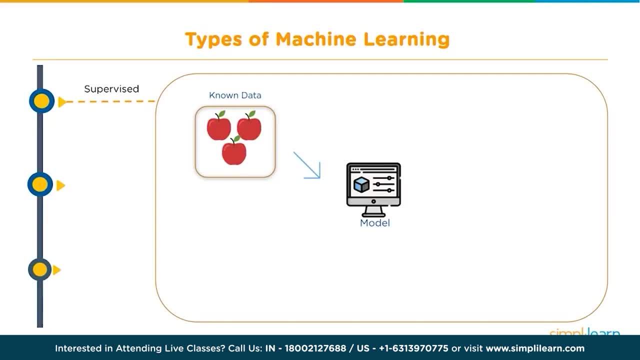 This is how the training is done. We provide a data set. This is a model that has pictures of a fruit like an apple. Then we provide another data set which lets the model know that these pictures were that of fruit called apple. This ends the training phase. 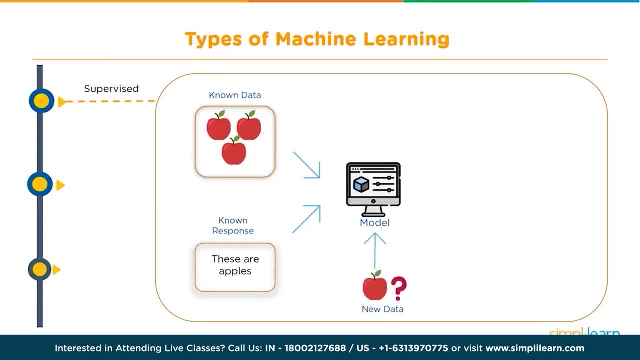 Now what we will do is we provide a new set of data which only contains pictures of apple. Now here comes the fun part: The system can actually tell you what fruit it is, And it will remember this and apply this knowledge in the future as well. 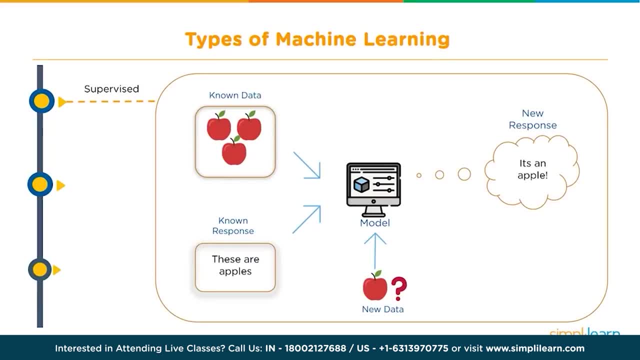 That's how supervised learning works. supervised learning works. You are training the model to do a certain kind of an operation on its own. This kind of a model is generally used into filtering spam mails from your email accounts as well. Yes, surprise, aren't you? So let's move on to unsupervised learning. 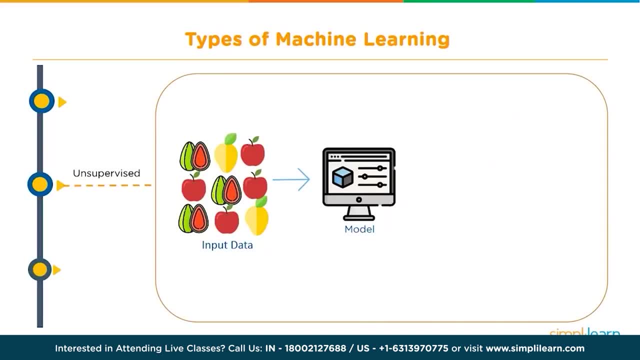 now, Let's say we have a dataset which is cluttered, In this case we have a collection of pictures of different fruits. We feed this data to the model and the model analyzes the data to figure out patterns in it. In the end, it categorizes the photos into three. 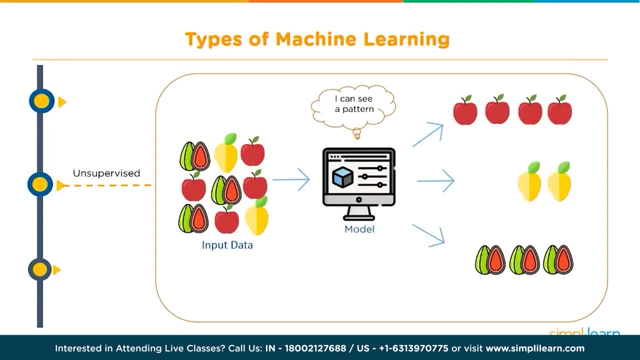 types, as you can see in the image, based on their similarities. So you provide the data to the system and let the system do the rest of the work. Simple, isn't it? This kind of a model is used by Flipkart to figure out the products that are well-suited for you. 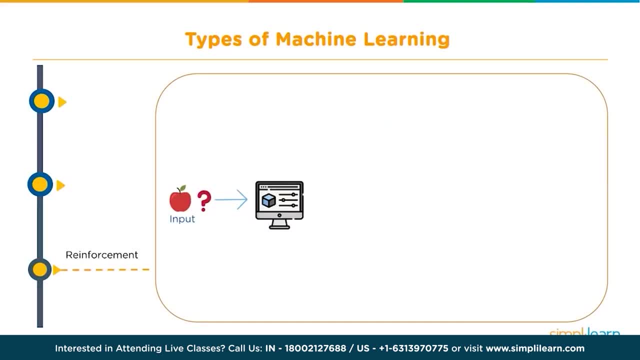 Honestly speaking, this is my favorite type of machine learning out of all the three. This type has been widely shown in most of the sci-fi movies lately. Let's find out how it works. Imagine a newborn baby. You put a burning candle in front of the baby. The baby does. 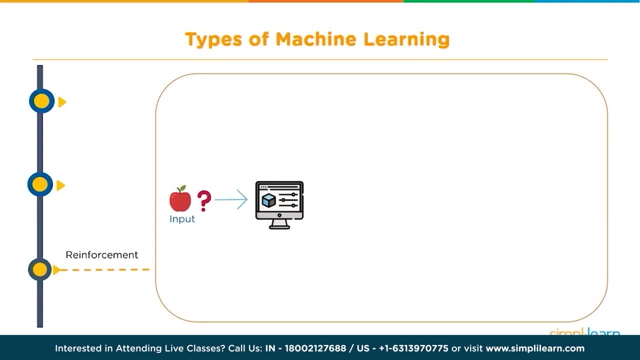 not know that if it touches the flame its fingers might get burnt, So it does that anyway and gets hurt. The next time you put that candle in front of the baby it will remember what happened the last time and would not repeat what it did. That's exactly how reinforcement. 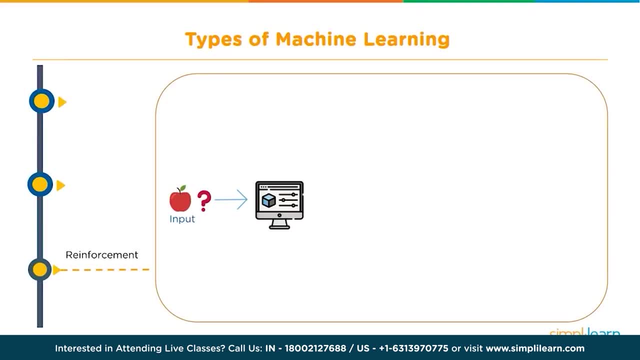 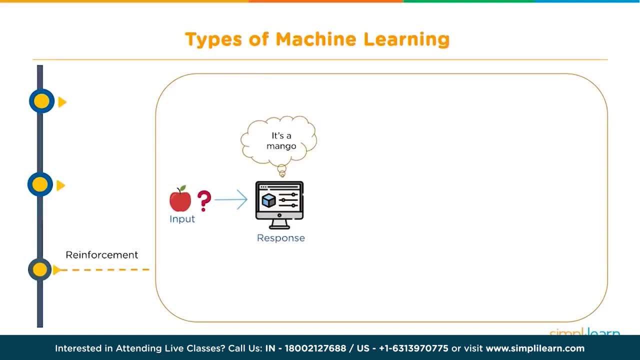 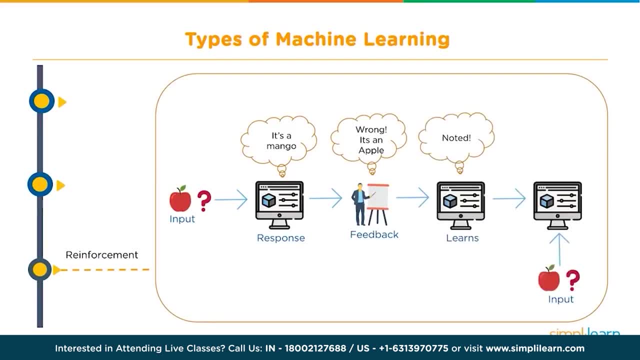 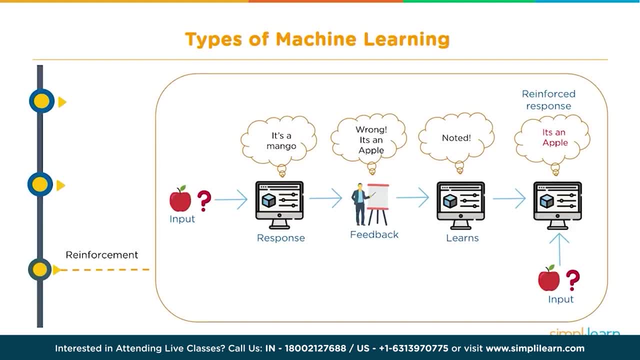 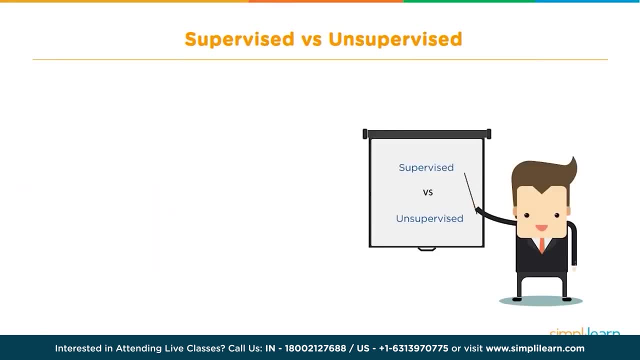 Creed or FIFA, wherein the level of difficulty increases as you get better with the games. Just to make it more clear for you, let's look at a comparison between supervised and unsupervised learning. Firstly, the data involved in case of supervised learning is labelled. 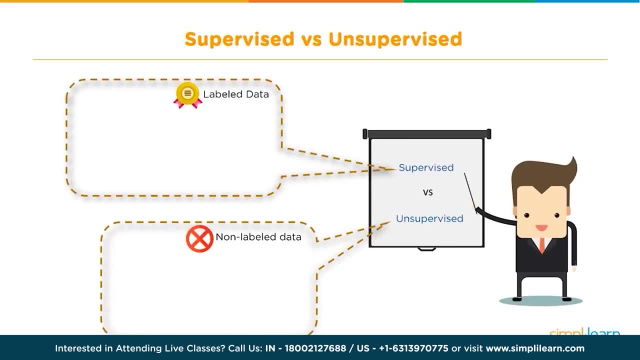 As we mentioned in the examples previously, we provide the system with a photo of an apple and let the system know that this is actually an apple. That is called labelled data. So the system learns from the labelled data and makes future predictions- Now unsupervised. 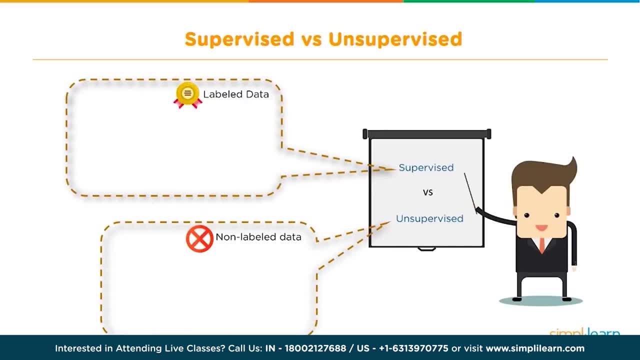 learning does not require any kind of labelled data, because its work is to look for patterns in the input data and organise it. The next point is that you get a feedback. in case of supervised learning, That is, once you get the output. the system tends to remember that. 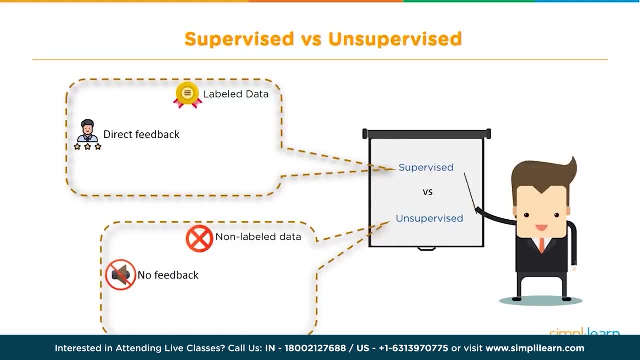 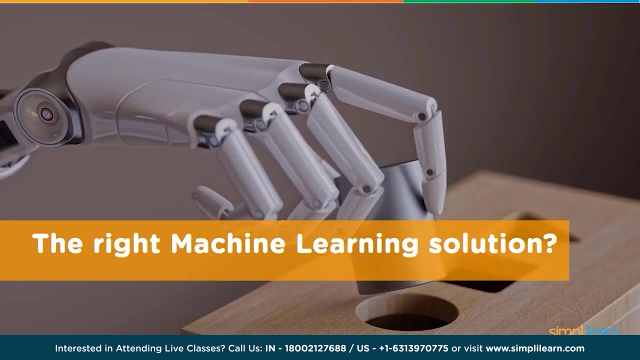 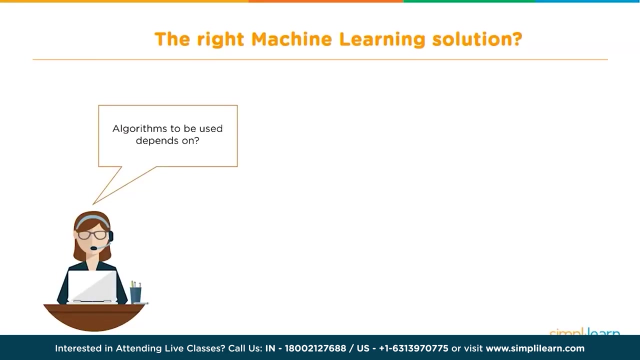 and uses it for the next operation. Subtitles by the Amaraorg community. Now let's talk about a question that everyone needs to answer before building a machine learning model: What kind of a machine learning solution should we use? Yes, you should be very careful. 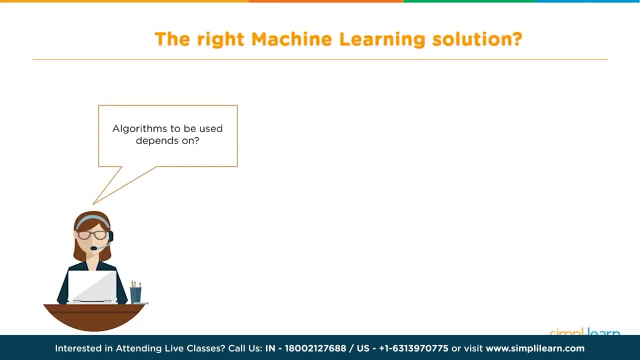 to choose the right kind of solution for your model, Because if you don't, you might end up losing a lot of time, energy and processing cost. I won't be naming the actual solutions because you guys aren't familiar with them yet, So we will be looking at it based on. 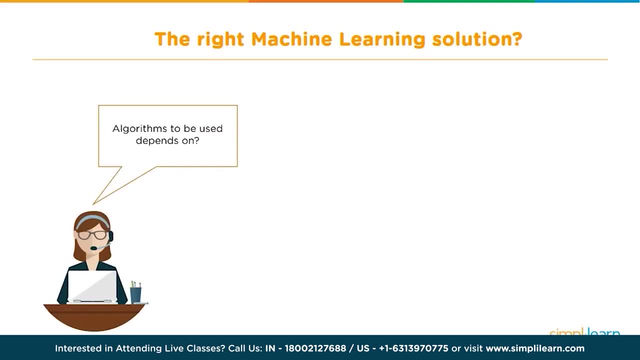 supervised, unsupervised and reinforcement learning. So let's look into the factors that might help us select the right kind of machine learning solution. First factor is the problem statement describes the kind of model you will be building or, as the name suggests, it tells you what. 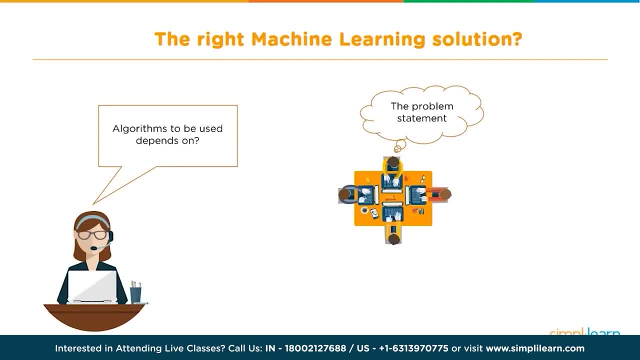 the problem is, For example, let's say the problem is to predict the future stock market prices. So for anyone who is new to machine learning would have trouble figuring out the right solution. But with time and practice you will understand that for a problem statement. 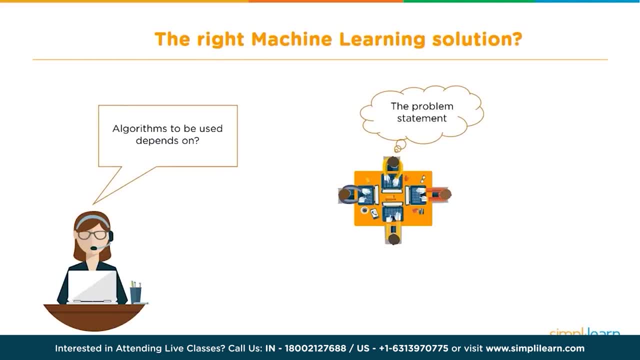 like this. solution based on supervised learning would work the best, for obvious reasons. Then comes the size, quality and nature of the data. If the data is cluttered, you go for unsupervised. large and categorical: we normally go for supervised learning solutions. Finally, we 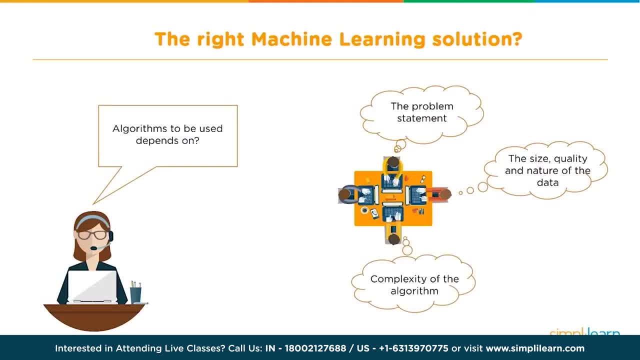 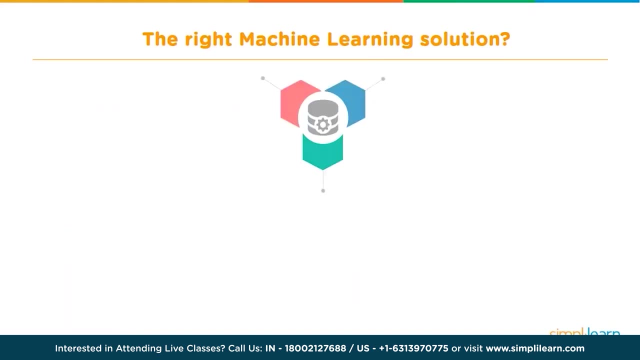 choose the solution based on their complexity. As for the problem statement wherein we predict the stock market prices, it can also be solved by using reinforcement learning, But that would be very, very difficult and time consuming. unlike supervised learning, Algorithms are not types of machine learning. In the most simplest language, they are methods. 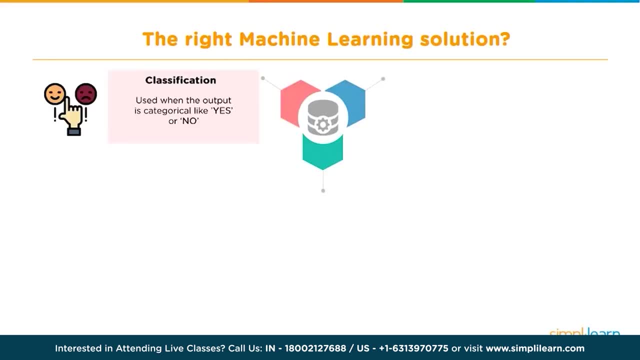 of solving a particular problem. So the first kind of method is classification, which falls under supervised learning. Classification is used when the output we are looking for is a Yes or No, or in the form A or B or True or False, Like if a shopkeeper wants. 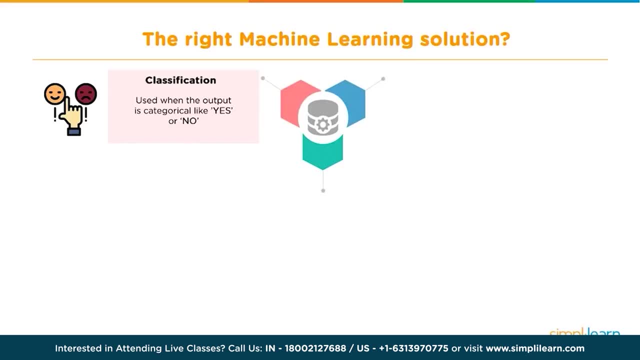 to predict if a particular customer will come back to his shop or not, he will use a classification algorithm. The algorithms that fall under Classification are: Decision Tree, Knife, Base, Random Finding and Basement, Model forest, logistic regression and KNN. The next kind is Regression. 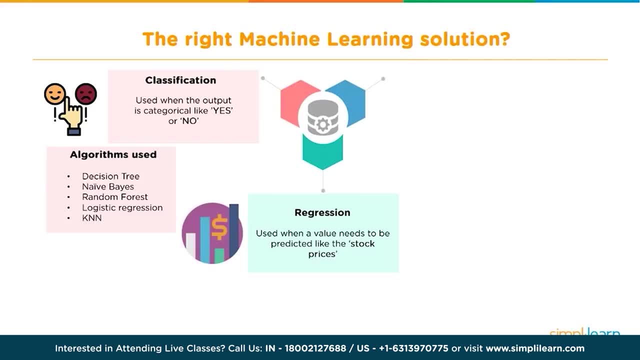 This kind of a method is used when the predicted data is numerical in nature, Like if the shopkeeper wants to predict the price of a product based on its demand. it would go for regression. The last method is Clustering. Clustering is a kind of unsupervised learning again. 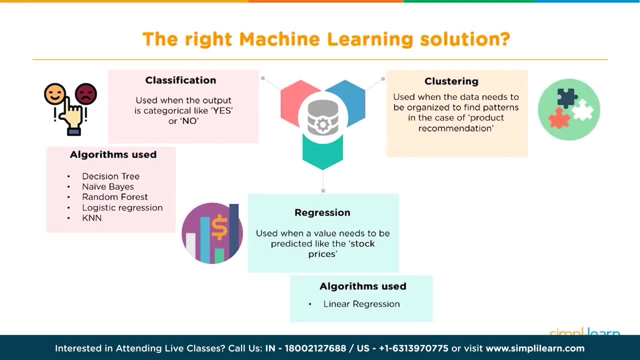 It is used when the data needs to be organized. Most of the recommendation systems used by Flipkart, Amazon, etc. make use of clustering. Another major application of it is in search engines. The search engines study your old search history to figure out your preferences and provide. 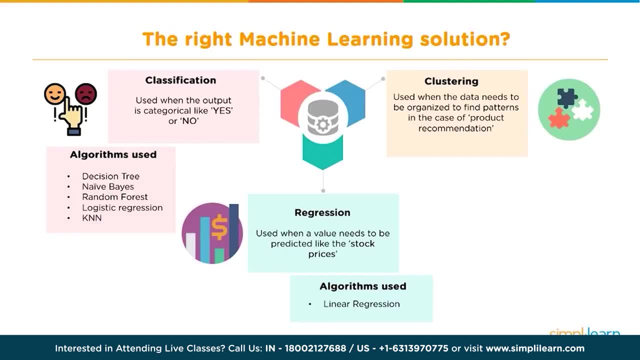 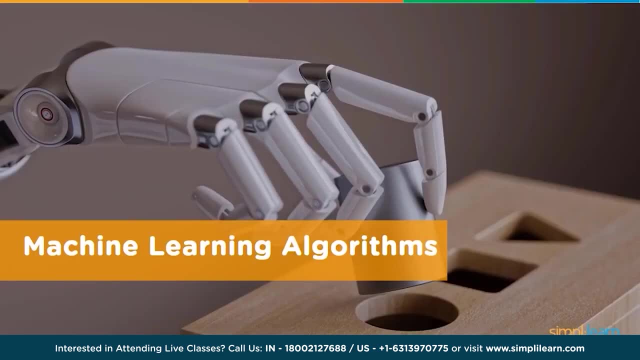 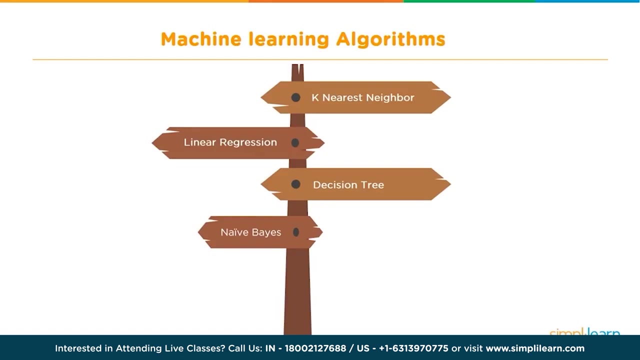 you the best search results. One of the algorithms that fall under clustering is K-Means. Now that we know the various algorithms, let's look into four key algorithms that are used widely. We will understand them with very simple examples. The four algorithms that we will try to understand are: K-Nearest Neighbor Linear Regression. 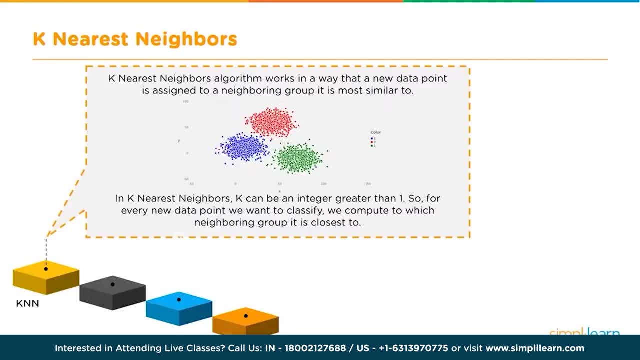 Decision Tree and Knife Pace. Let's start with our first machine learning solution: K-Nearest Neighbor. K-Nearest Neighbor is again a kind of a classification algorithm. As you can see on the screen, the similar data points form clusters. the blue one the 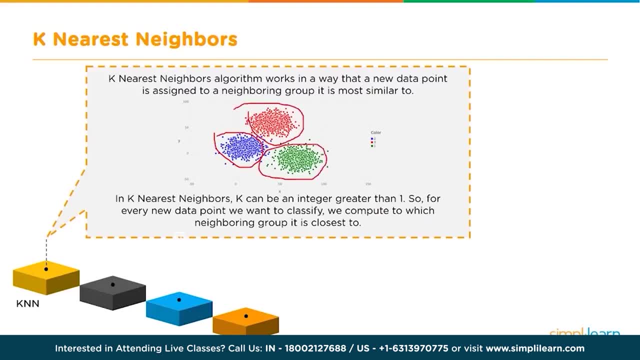 red one and the green one. There are three different clusters. Now if we get a new and unknown data point, it is classified based on the cluster closest to it or the most similar to it. K in KNN is the number of nearest neighboring data points. we wish to compare the unknown 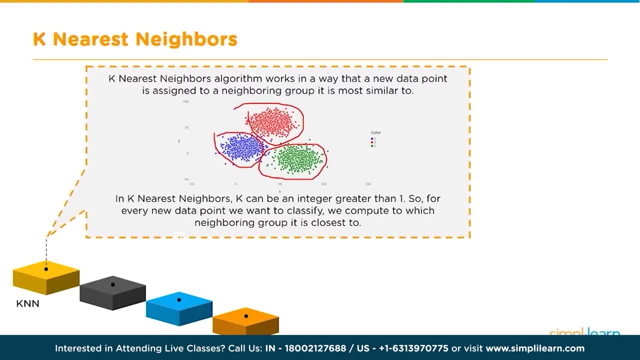 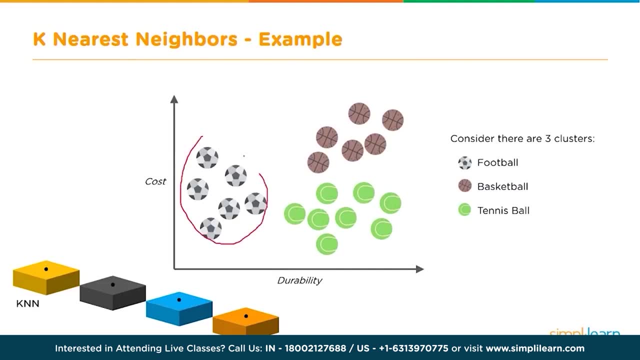 data with. Let's make it clear with an example. Let's say we have three clusters in a cost to durability graph. First cluster is of footballs. The second one is of tennis. The third one is of footballs. The fourth one is of tennis. 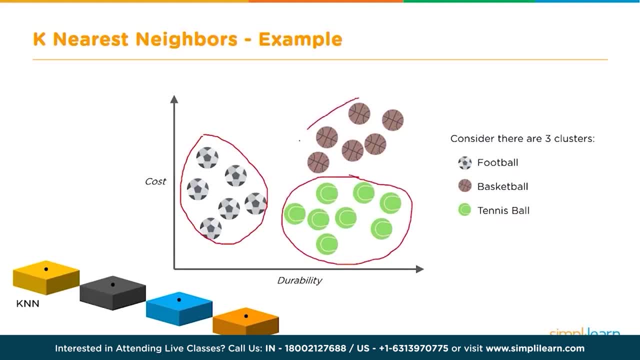 The fifth one is of tennis balls And the third one is of basketballs. From the graph we can say that the cost of footballs is high and the durability is less. The cost of tennis balls is very less, but the durability is high. 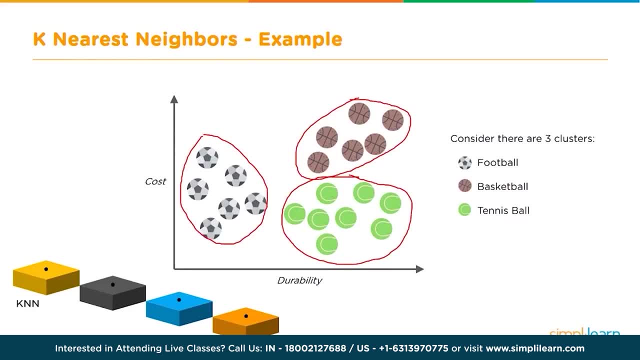 And the cost of basketballs is as high as the durability. Now let's say we have an unknown data point. We have a black spot which can be one kind of the balls, but we don't know what kind it is. So what we'll do? we'll try to classify this using KNN. 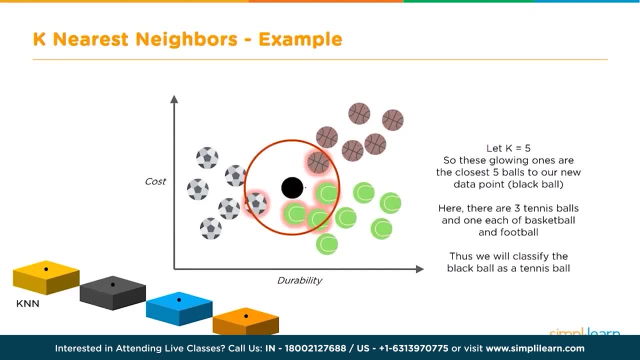 If we take, K is equal to five. we draw a circle keeping the unknown data point in the center and we make sure that we have five balls inside that circle. In this case, we have a football, a basketball and three tennis balls. 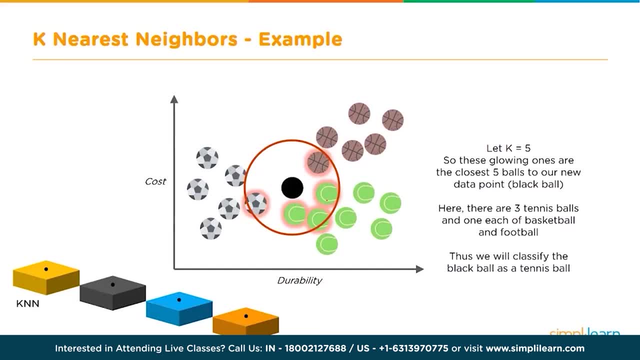 Now, since we have the highest number of tennis balls inside the circle, the classified ball would be a tennis ball. So that's how K-nearest neighbors are classified. K-nearest neighbor classification is done. Linear regression is again a type of supervised learning algorithm. 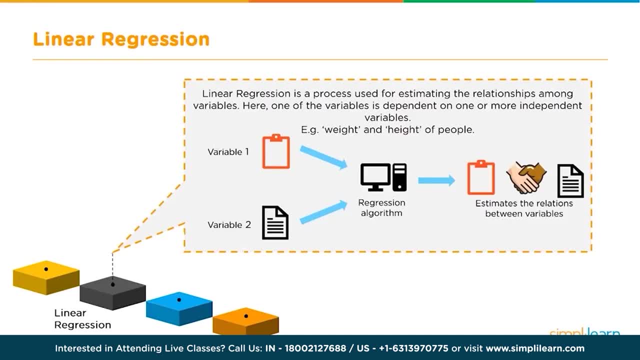 This algorithm is used to establish linear relationship between variables, one of which would be dependent and the other one would be independent, Like if we want to predict the weight of a person based on his height. weight would be the dependent variable and height would be independent. 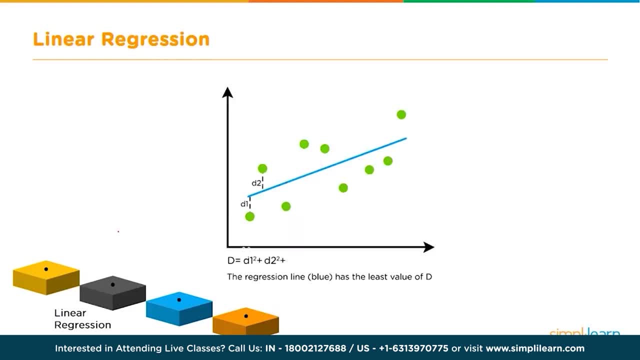 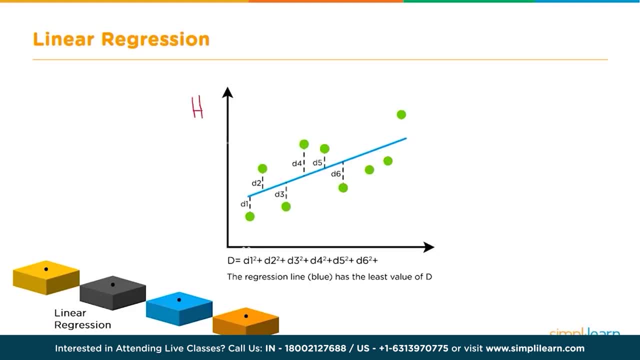 Let's say we have a graph here showing a relationship between height and distance. Let's put the height and weight of a person. Let's put the y-axis as h and the x-axis as h, So the green dots are the various data points. 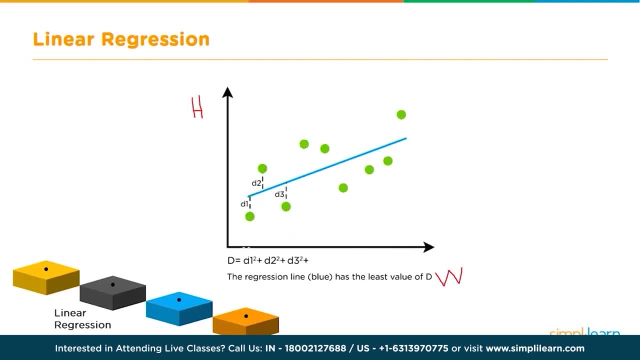 These green dots are the data points And d is the mean squared error. that is, the perpendicular distances for the line to the data points are the error values. This error tells us how much the predicted values vary from the original value. Let's ignore this blue line for a while. 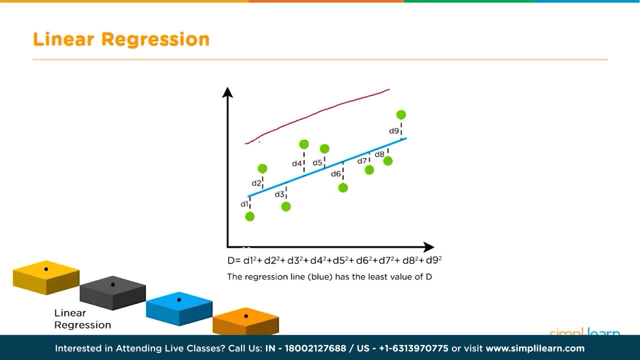 So let's say, if this is our regression line, you can see the distance from all the data points from this line is very high. So if we take this line as a regression line, the error in the prediction will be too high. So in this case the model will not be able to give us a good prediction. 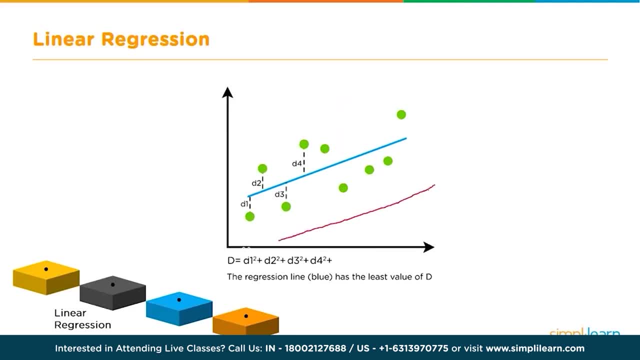 Let's say we draw another regression line like this: Even in this case you can see that the perpendicular distance of the data points from the line is very high, So the error value will still come as high as the last one. So this model will also not be able to give us a good prediction. 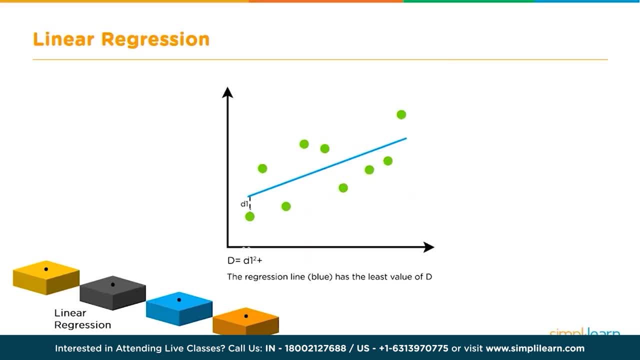 So what to do? So finally, we draw a line, Which is this blue line. So here we can see that the distance of the data points from the line is very less relative to the other two lines we drew, So the value of d for this line will be very less. 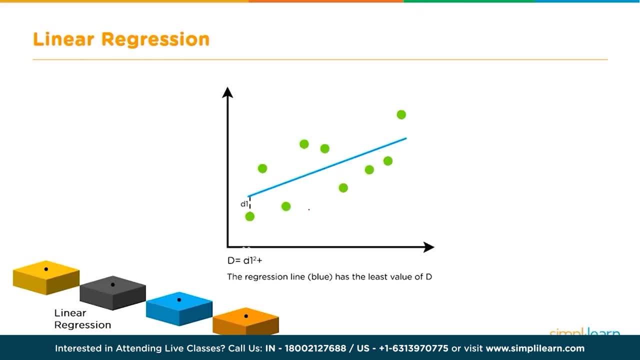 So in this case, if we take any value on the x-axis, the corresponding value on the y-axis will be our prediction And, given the fact that the d is very low, our prediction should be good. also, This is how regression works. 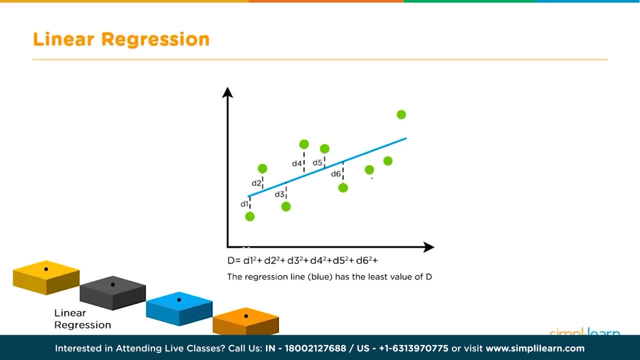 We draw a line, a regression line, that is in such a way that the value of d is the least, eventually giving us good predictions. This algorithm, that is, decision tree, is a kind of an algorithm you can very strongly relate to. 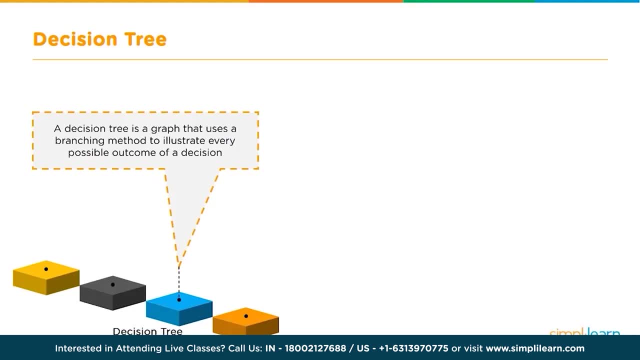 It uses a kind of a branching method to realize the problem and make decisions based on the conditions. Let's take this graph as an example. Imagine yourself sitting at home getting bored. You feel like going for a swim. What you do is you check if it's sunny outside. 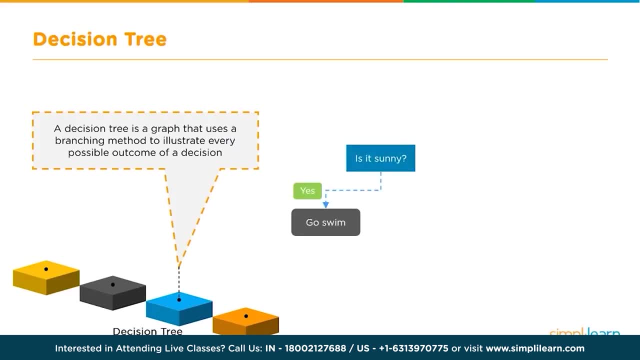 So that's your first condition. If the answer to that condition is yes, you go for a swim. If it's not sunny, then the next question you would ask yourself is if it's raining outside. So that's condition number two. If it's actually raining, you cancel the plan and stay indoors. 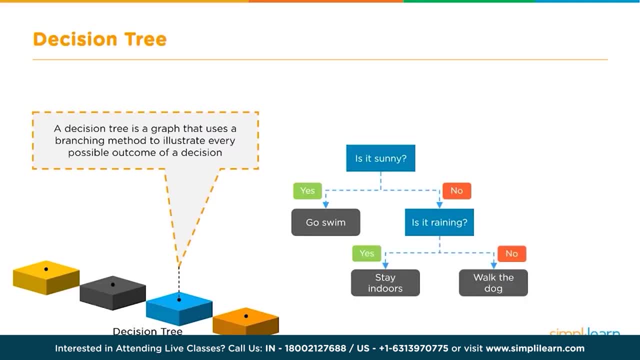 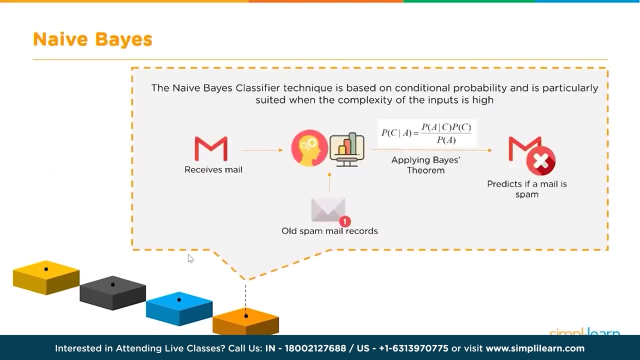 If it's not raining, then you would probably go outside and have a walk. That's the final node. That's how decision tree algorithm works. You probably use this every day. It realizes the problem and then takes the decisions based on the answers to every conditions. 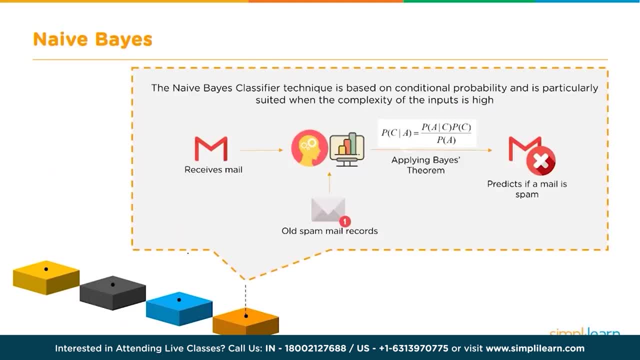 Naive-based algorithm is mostly used in cases where a prediction needs to be done on a very large dataset. It makes use of conditional probability. Conditional probability is the probability of an event, say A, happening given that another event B has already happened. 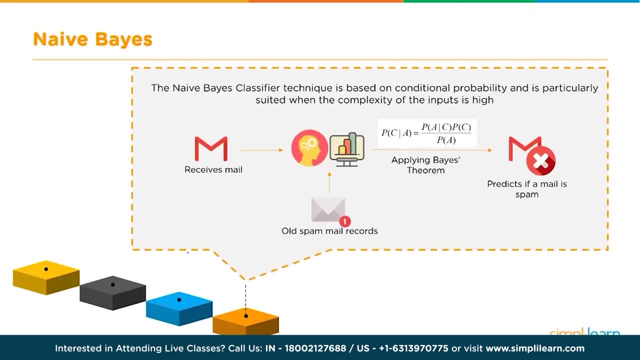 This algorithm is most commonly used in filtering spam mails in your email account. Let's say you receive a mail. The model goes through your old spam mail records, Then it uses Pace theorem to predict if the present mail is a spam mail or not. 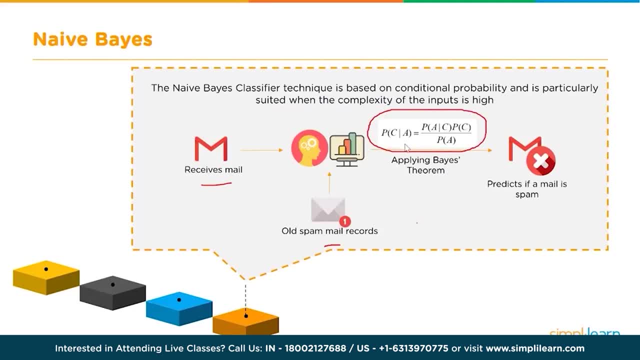 So PC of A is the probability of event C occurring when A has already occurred. PA of C is the probability of event A occurring when C has already occurred. PC is the probability of event C occurring. PA is the probability of event A occurring. 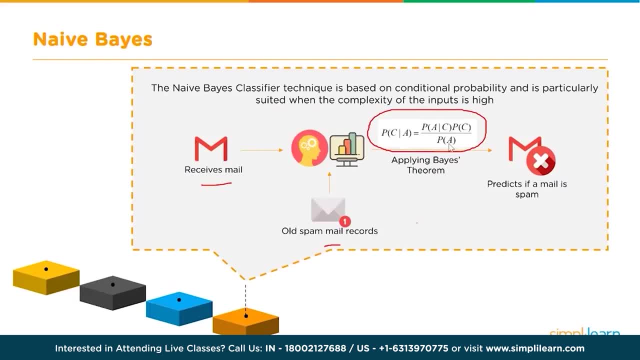 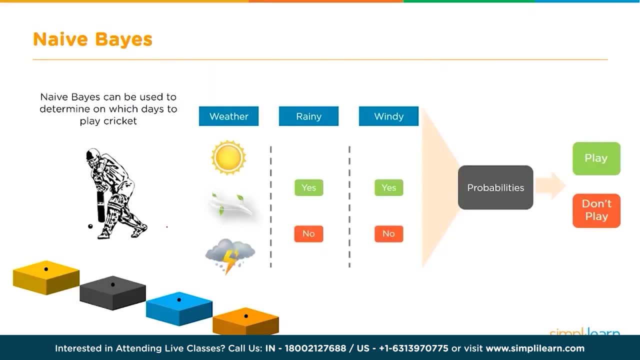 PC is the probability of event C occurring, event A occurring. Let's try to understand Knife Base with a better example. Knife Base can be used to determine on which days to play cricket. Based on the probabilities of a day being rainy, windy or sunny, the model tells us if a match is possible. If we consider 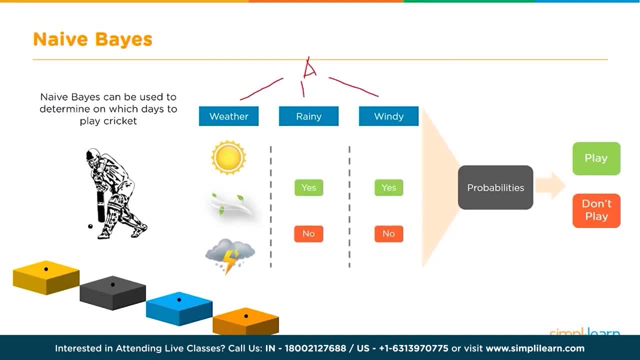 all the weather conditions to be, event A for us and the probability of a match being possible event C. so the model applies the probabilities of event A and C into the Bayes theorem and predicts if a game of cricket is possible on a particular day or not. In this case, 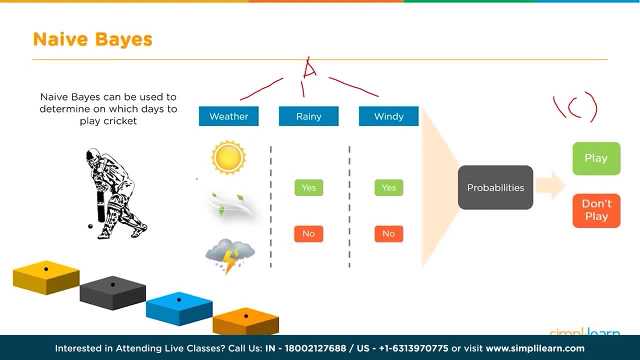 if the probability of C of A is more than 0.5, we can be able to play a game of cricket. If it's less than 0.5, we won't be able to do that. That's how Knife Base algorithm works. 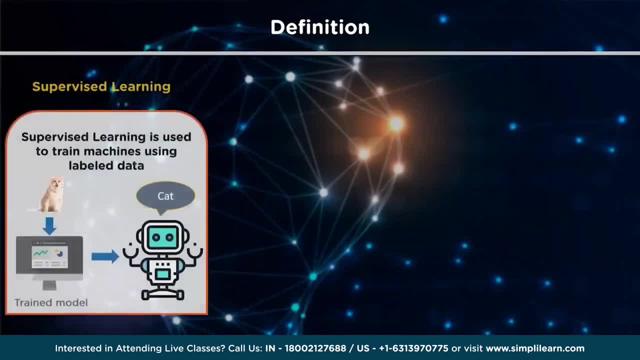 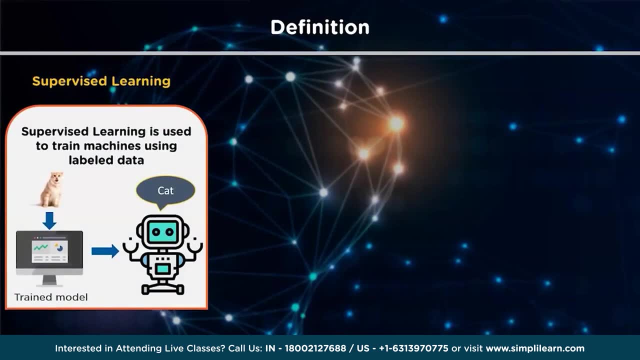 Let's look at the definition of each of these learning techniques. Superb- Unsupervised learning- uses labelled data to train machine learning models. Labelled data means that the output is already known to you. The model just needs to map the inputs to the outputs. An example of supervised learning can be to train a machine that identifies. 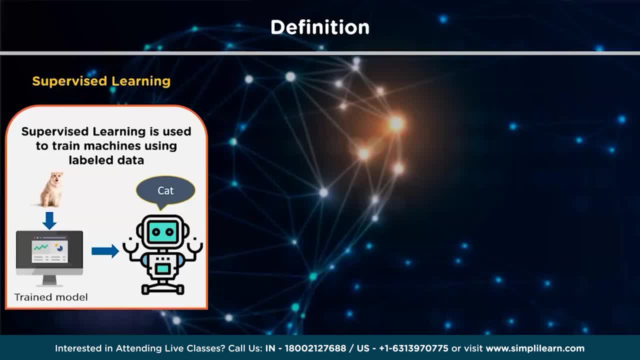 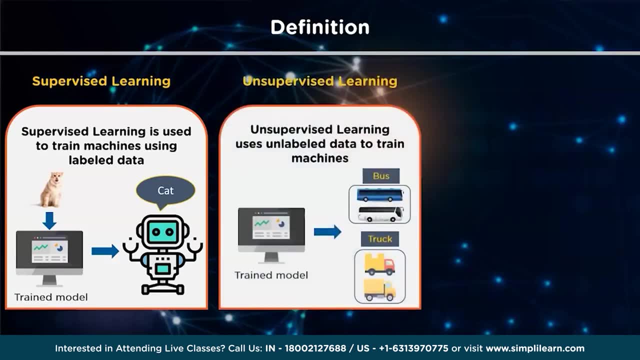 the image of an animal. Below you can see we have a trained model that identifies the picture of a cat. Unsupervised learning uses unlabelled data to train machines. Unlabelled data means there is no fixed output variable. The model learns. 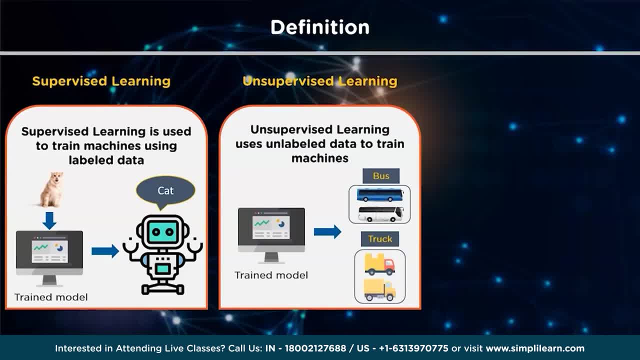 from the data, discovers patterns and features in the data and returns the output. Here is an example of an unsupervised learning technique that uses the images of vehicles to classify if it's a bus or a truck. So the model learns by identifying the parts of a vehicle such 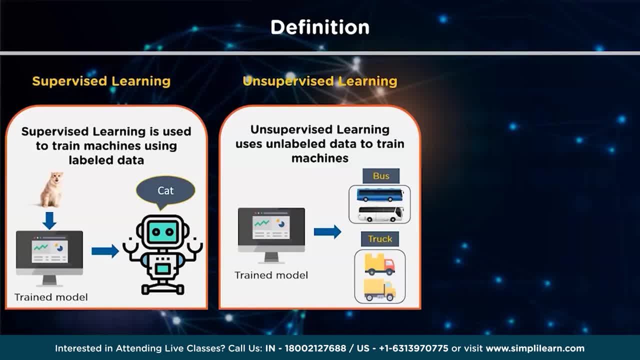 as the length and width of the vehicle, the front and rear end covers, roof hoods, the types of wheels used, etc. Based on these features, the model classifies if the vehicle is a bus or a truck. Reinforcement learning. 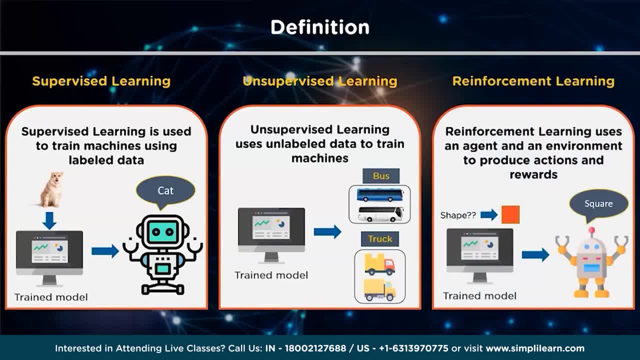 Trains a machine to take suitable actions and maximize reward in a particular situation. It uses an agent and an environment to produce actions and rewards. The agent has a start and an end state, but there might be different paths for reaching the end state, like a maze. 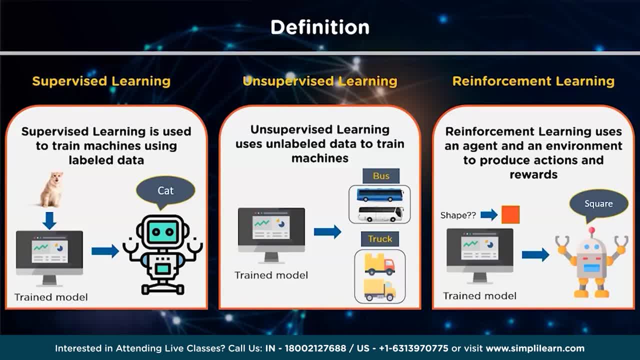 In this learning technique there is no predefined target variable. An example of reinforcement learning is to train a machine that can identify the shape of an object. given a list of different objects, such as square, triangle, rectangle, rectangle or a circle, In the example shown, the model tries to predict the shape of the object. 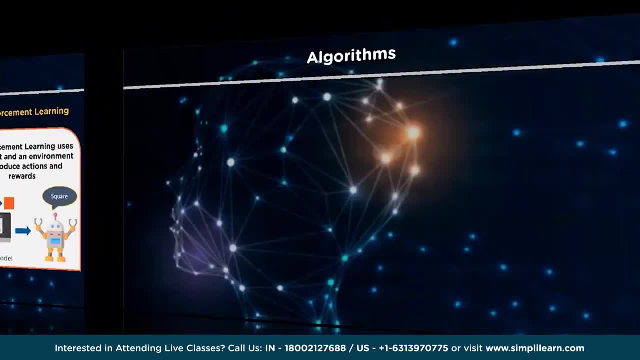 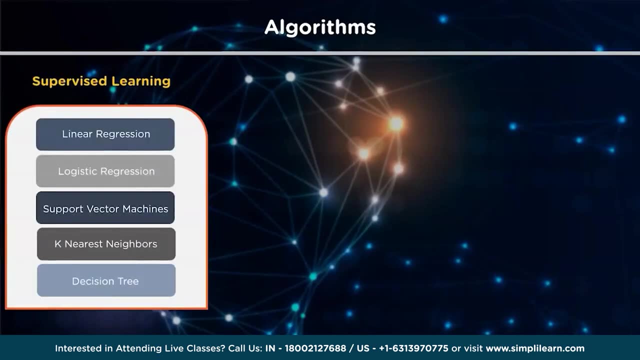 which is a square here. Now let's look at the different machine learning algorithms that come under these learning techniques. Some of the commonly used supervised learning algorithms are linear regression, logistic regression, support, vector machines, k-nearest neighbours, decision tree, random forest and knife base. Examples of unsupervised learning algorithms are k-means. 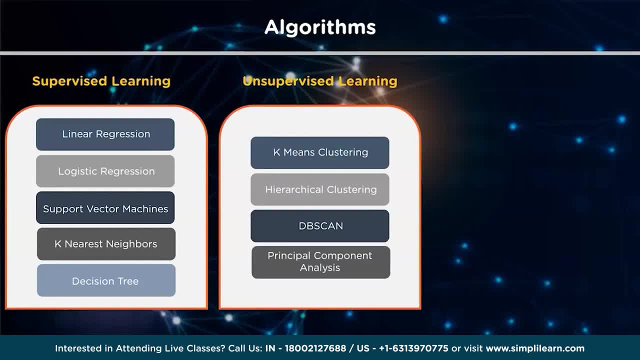 clustering and a few other. These are general mechanisms available in the problem system. In the example shown, an example of reinforcement learning is to teach a machine how to adapt hierarchical clustering, DB scan, principal component analysis and others. Choosing the right algorithm depends on the type of problem you are trying to solve. 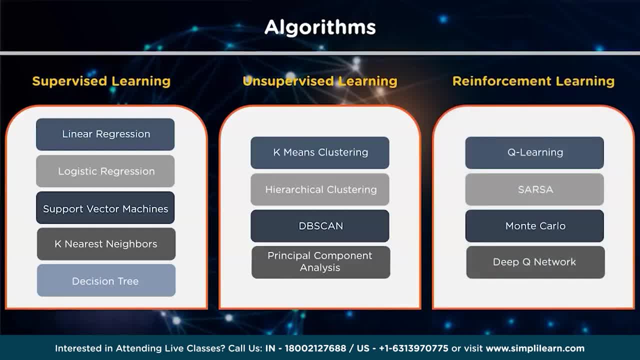 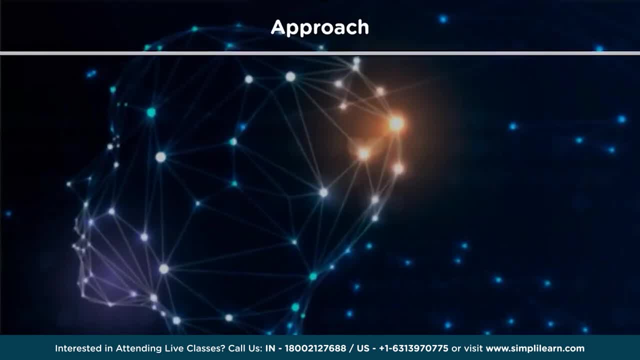 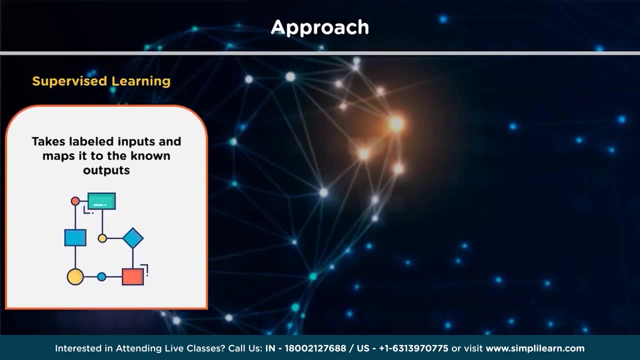 Some of the important reinforcement learning algorithms are Q-learning, Monte Carlo, SAR-SAR and Deep Q-network. Now let's look at the approach in which these machine learning techniques work. So supervised learning takes labeled inputs and maps it to known outputs, which means you already know the target variable. 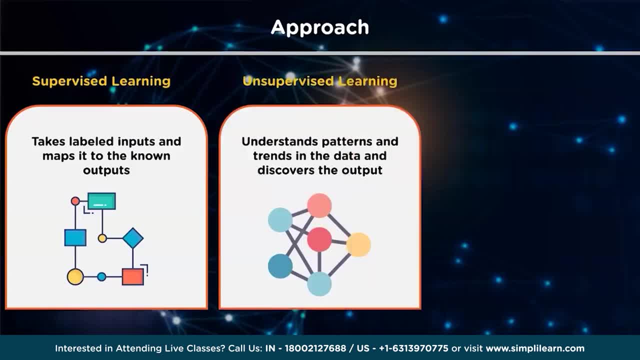 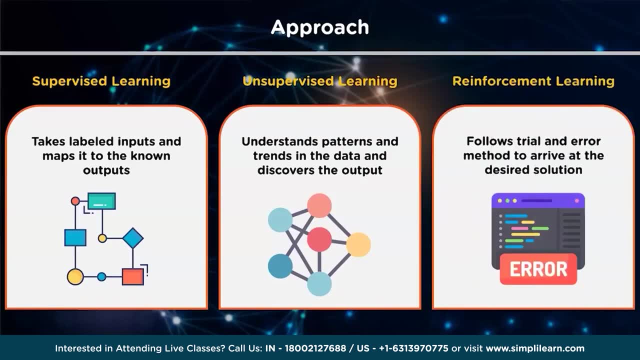 Unsupervised learning finds patterns and understands the trends in the data to discover the output. So the model tries to label the data based on the features of the input data, While reinforcement learning follows trial and error method to get the desired solution. After accomplishing a task, the agent receives an award. An example: 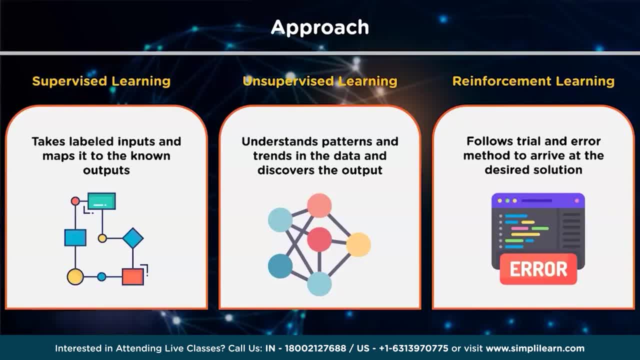 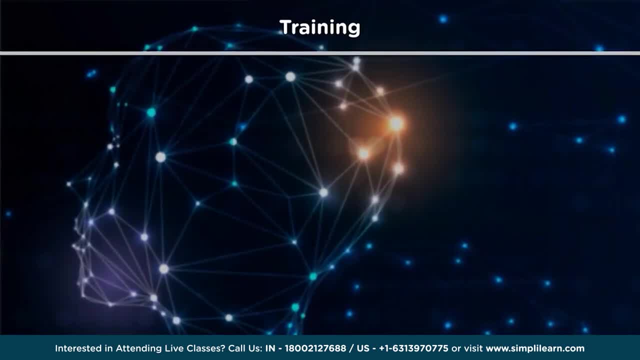 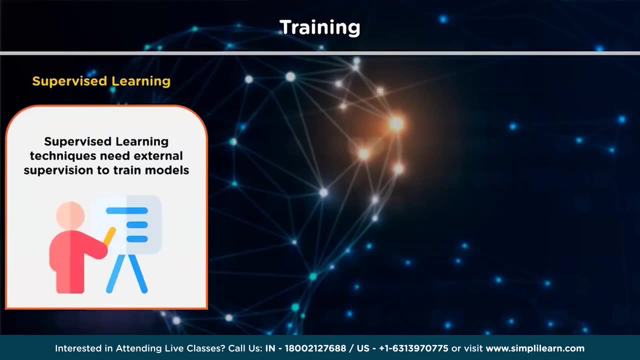 could be to train a dog to catch the ball. If the dog learns to catch a ball, you give it a reward, such as a biscuit. Now let's discuss the training process for each of these learning methods. So supervised learning methods need external supervision to train machine learning models, and hence the name supervised. 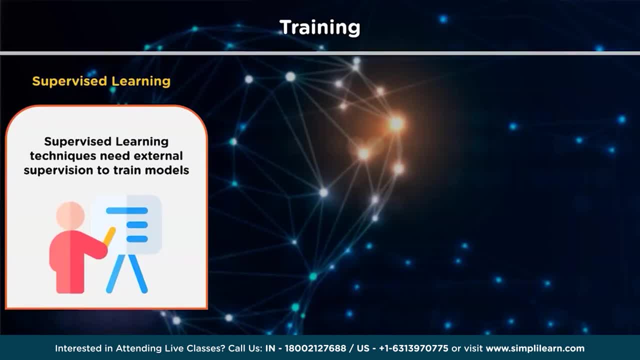 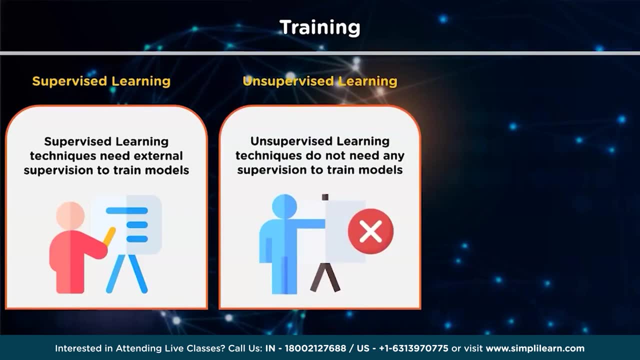 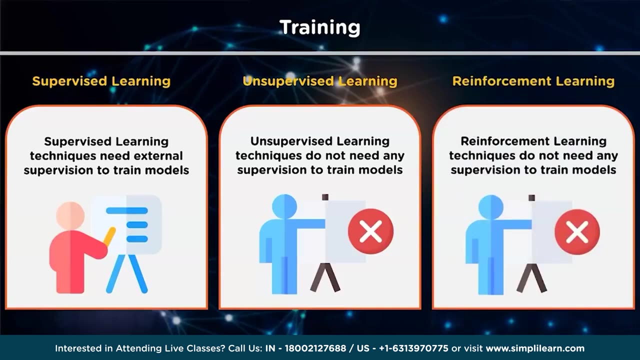 They need guidance and additional information to return the result. Unsupervised learning techniques do not need any supervision to train models. They learn on their own and predict the output. Similarly, reinforcement learning methods do not need any supervision to train machine learning models And with that, 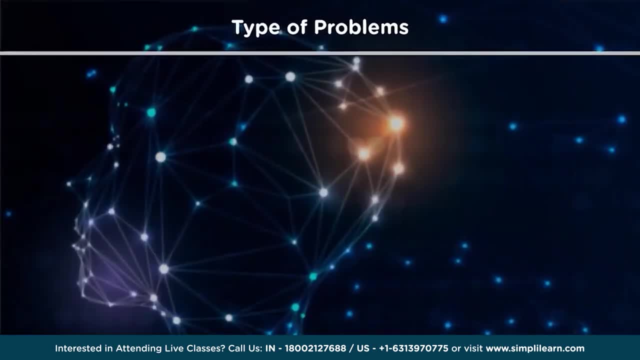 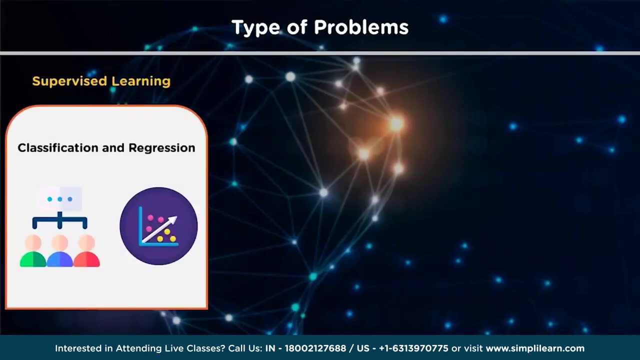 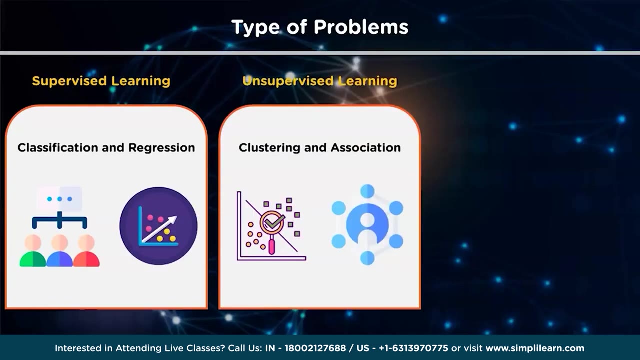 let's focus on the types of problems that can be solved using these three types of machine learning techniques. So supervised learning is generally used for classification and regression problems- We'll see the examples in the next slide- And unsupervised learning is used for clustering and association problems, While reinforcement learning 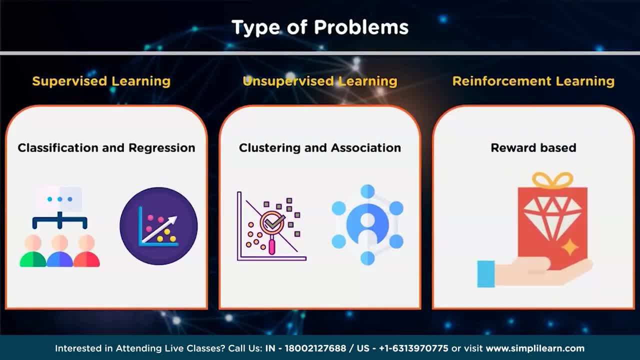 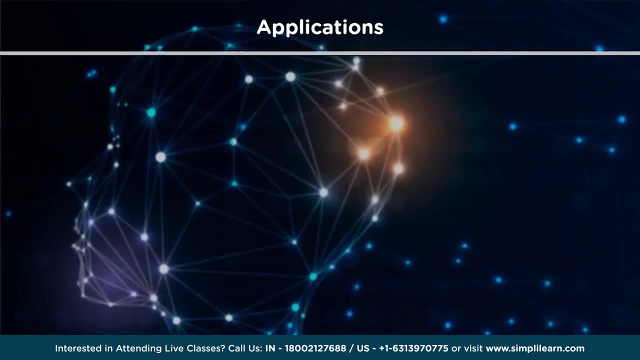 is reward based. So for every task or for every step completed, there will be a reward received by the agent, And if the task is not achieved correctly, there will be some penalty used. Now let's look at a few applications of supervised, unsupervised and reinforcement learning. 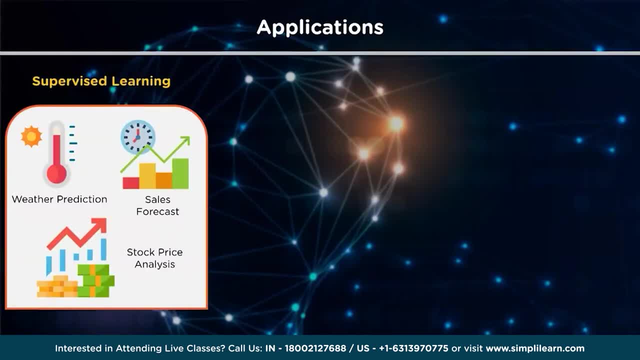 As we saw earlier, supervised learning are used to solve classification and regression problems. For example, you can predict the weather for a particular day based on humidity, precipitation, wind speed and pressure values. You can use supervised learning alone to use unsupervised learning algorithms to forecast sales for the next month or the next quarter for different products. 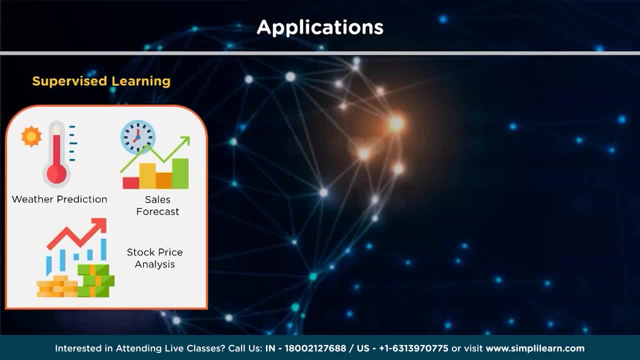 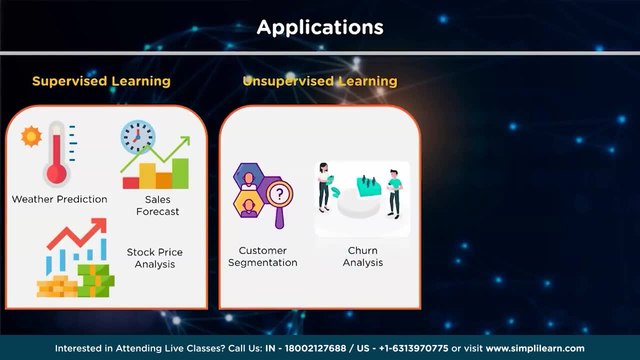 Similarly, you can use it for stock price analysis or identifying if a cancer cell is malignant or benign. Now, talking about the applications of unsupervised learning, we have customer segmentation. So, based on customer behavior, likes, dislikes and interests, you can segment and cluster similar customers into a group. Another. 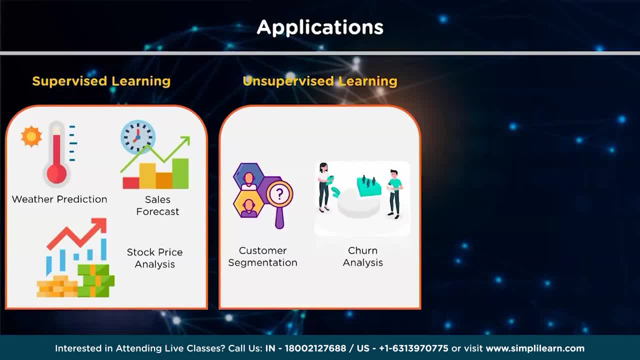 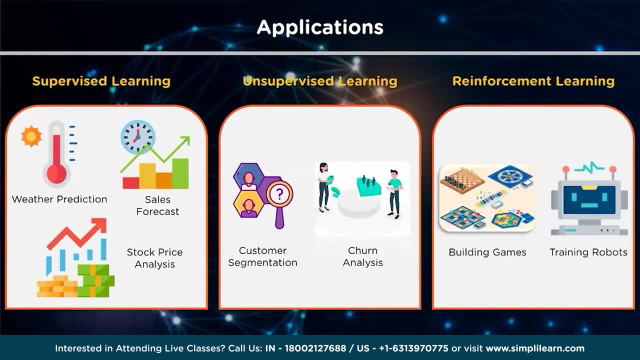 example where unsupervised learning algorithms are used is customer churn analysis. Now let's see what applications we have in reinforcement learning. So reinforcement learning algorithms are widely used in the gaming industries to build games. It is also used to train robots to perform human tasks. Profit estimation of a company. 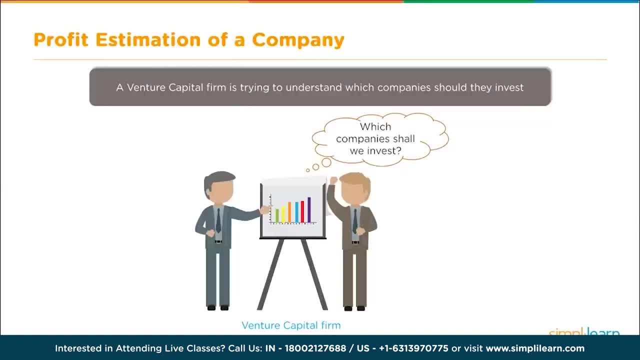 If I was going to invest in a company, I would like to know how much money I could expect to make. So we'll take a look at a venture capitalist firm and try to understand which companies they should invest in. So we'll take the idea that we need to decide the companies to invest in. 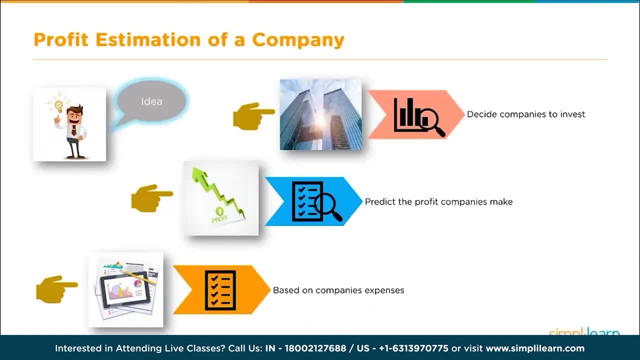 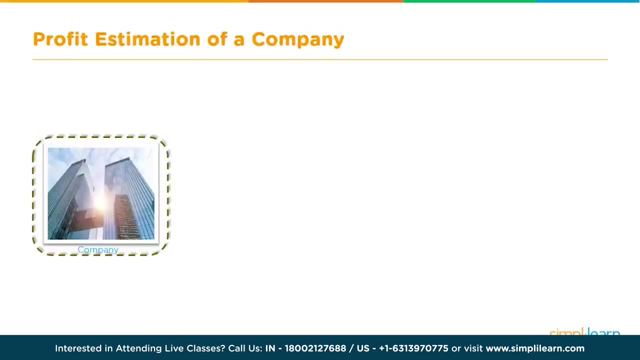 We need to predict the profit the company makes, and we're going to do it based on the company's expenses, and even just a specific expense. In this case, we have our company, We have the different expenses, So we have our R&D, which is your research and development. 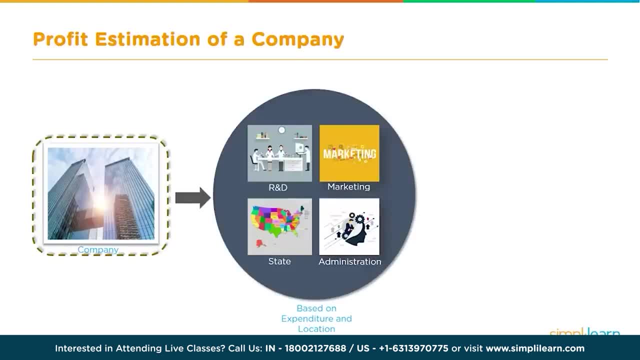 We have our marketing, We might have the location, We might have what kind of administration it's going through. Based on all this different information, we would like to calculate the profit. Now, in actuality, there's usually about 23 to 27 different markers that the company 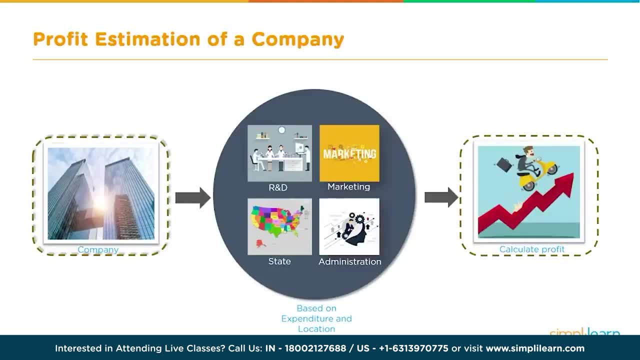 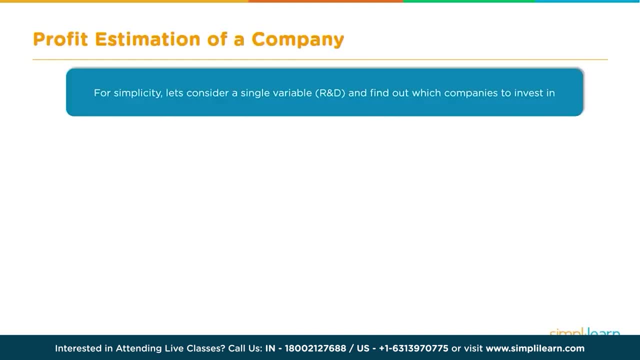 looks at if they're a heavy duty investor. We're only going to take a look at one basic one. We're going to come in and, for simplicity, let's consider a single variable R&D and find out which companies to invest in based on that. So we take our R&D, We're plotting the profit based on. 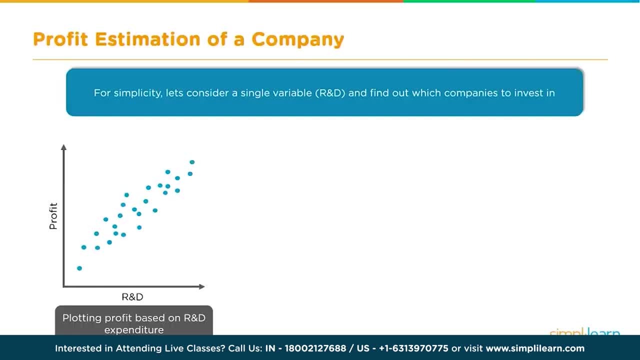 the R&D expenditure, how much money they put into the research and development, And then we look at the profit that goes with that. We can predict a line to estimate the profit. So we draw a line right through the data. When you look at that you can see how much they invest in. the R&D is a good 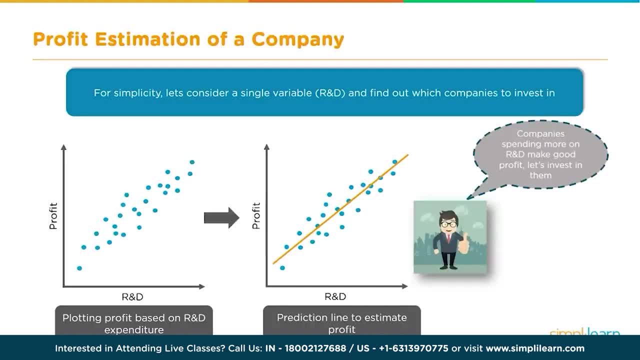 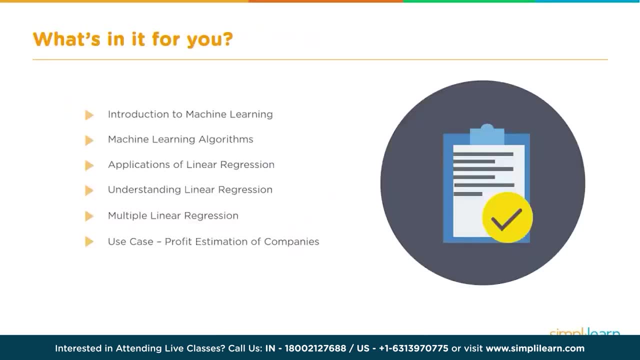 marker as to how much profit they're going to have. We can also note that companies spending more on R&D make good profit, So let's invest in the ones that spend a higher rate in their R&D. What's in it for you? First, we'll have an introduction to machine learning, followed by machine learning algorithms. 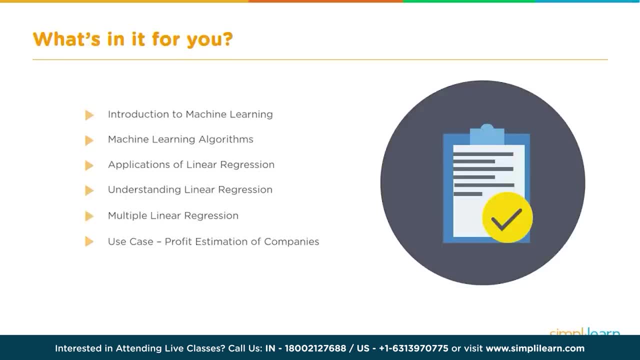 These will be specific to linear regression and where it fits into the larger model. Then we'll take a look at applications of linear regression, understanding linear regression and multiple linear regression. Finally, we'll roll up our sleeves and do a little programming in use case profit estimation of companies. Let's go ahead and jump in. 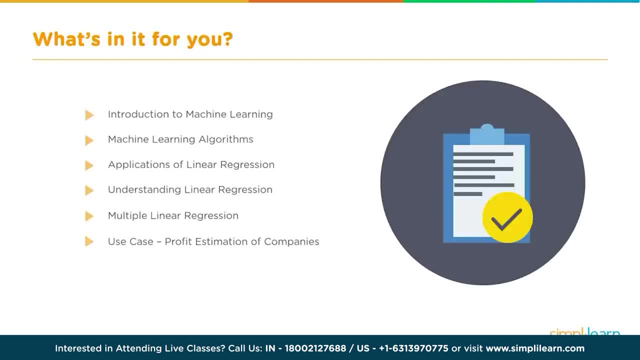 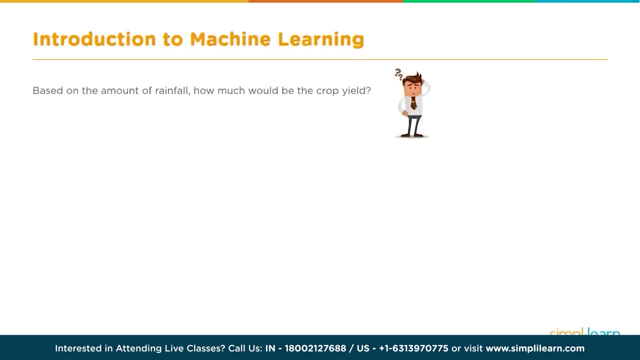 Let's start with our introduction to machine learning, along with some machine learning algorithms and, where that fits in, with linear regression. Let's look at another example of machine learning: Based on the amount of rainfall, how much would be the crop yield? So here we have our crops, we have our 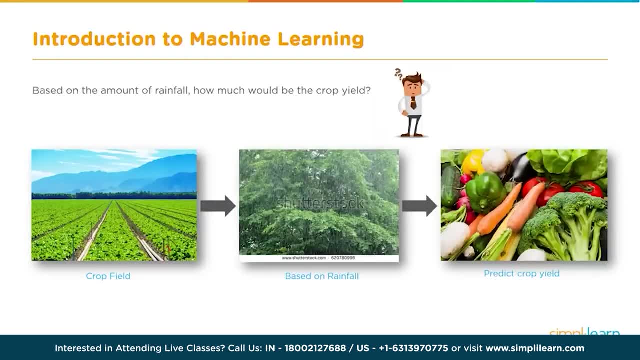 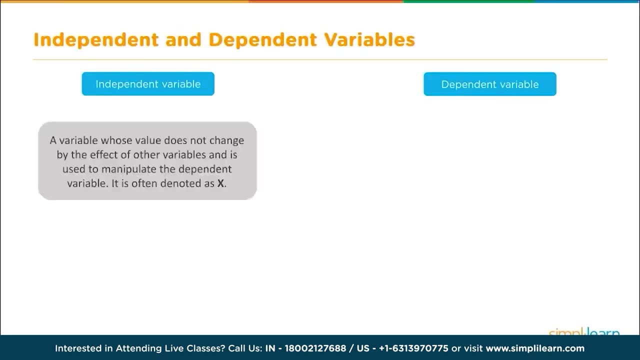 rainfall and we want to know how much we're going to get from our crops this year. So we're going to introduce two variables: independent and dependent. The independent variable is a variable whose value does not change by the effect of other variables and is used to manipulate the dependent. 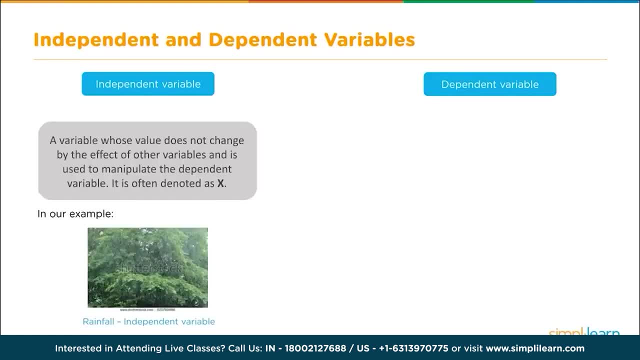 variable. It is often denoted as X. In our example, rainfall is the independent variable. This is a wonderful example, because you can easily see that we can't control the rain, but the rain does control the crop. So we talk about the independent variable, controlling the dependent. 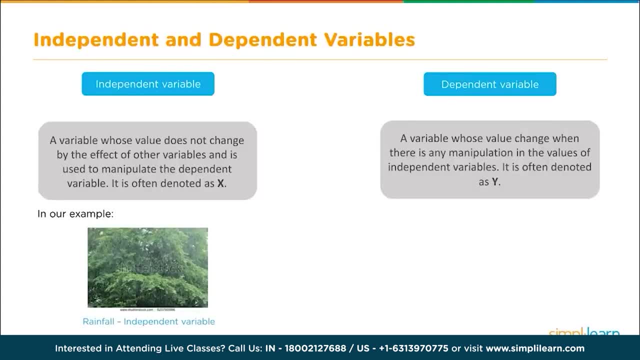 variable. Let's define dependent variable as a variable whose value change when there is any manipulation of the values of the independent variables. It is often denoted as Y And you can see here: our crop yield is dependent variable and it is dependent on the amount of rainfall. 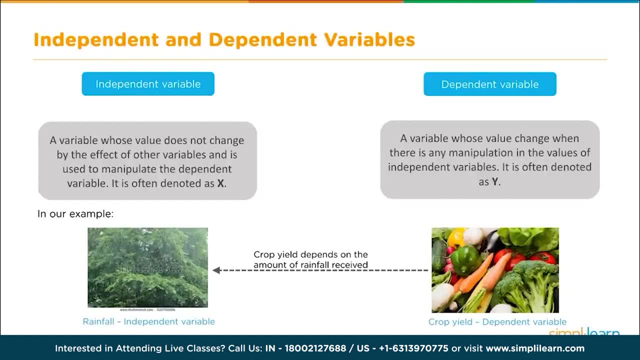 received. Now that we've taken a look at a real life example, let's go a little bit into the theory and some definitions on machine learning and see how that fits together with linear regression, Numerical and categorical values. Let's take our data. 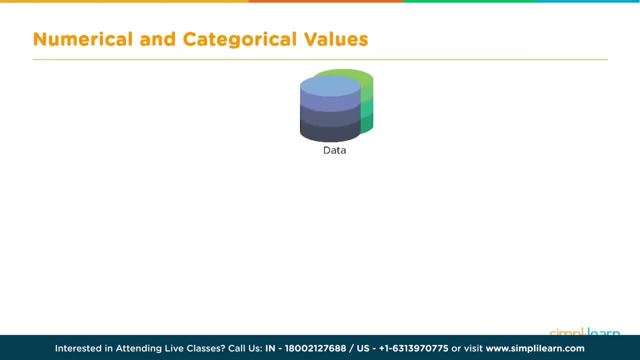 coming in. This is kind of random data from any kind of project. We want to divide it up into numerical and categorical. So numerical is numbers: age, calorie, height, where categorical would be a description, the color, a dog's breed, gender. Categorical is limited to very specific. 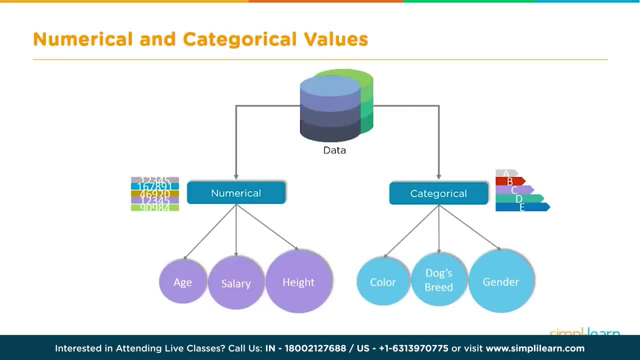 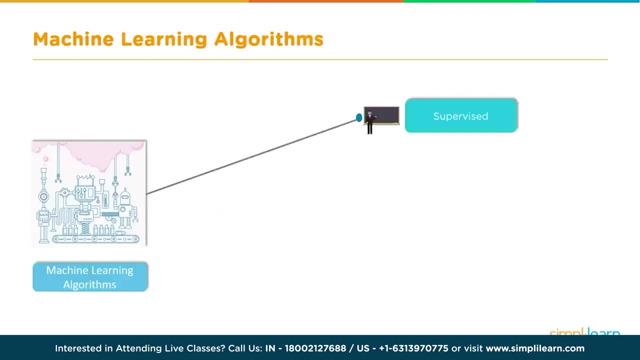 items where numerical is a range of information. Now that you've seen the difference between numerical and categorical data, let's take a look at some different machine learning definitions. When we look at our different machine learning algorithms, we can divide them into three areas: Supervised, unsupervised. 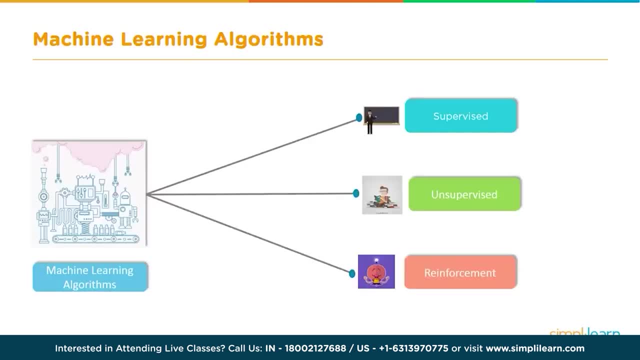 and reinforcement. We're only going to look at supervised today. Unsupervised means we don't have the answers and we're just grouping things. Reinforcement is where we give positive and negative feedback to our algorithm, to program it, and it doesn't have the information until after the 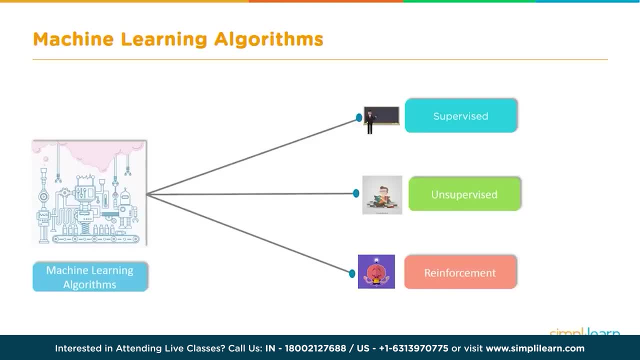 fact. But today we're just looking at supervised, because that's where linear regression fits in. In supervised data. we have our data already there and our answers for a group, and then we use that to program our model and come up with an answer. The two most common uses for that is through: 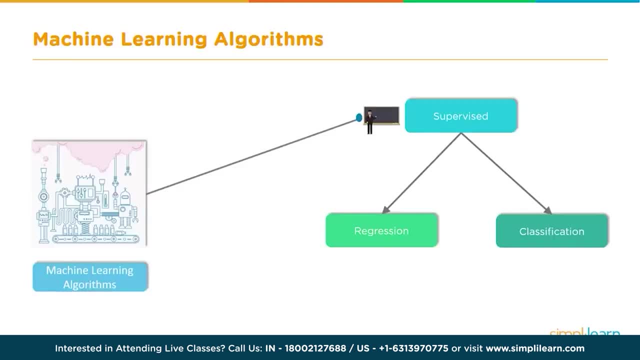 the regression and classification. Now we're doing linear regression, so we're just going to focus on the regression side. And in the regression we have simple linear regression, we have multiple linear regression and we have polynomial linear regression. Now, on these three, simple linear regression is the examples we've looked at so far where we have a lot. 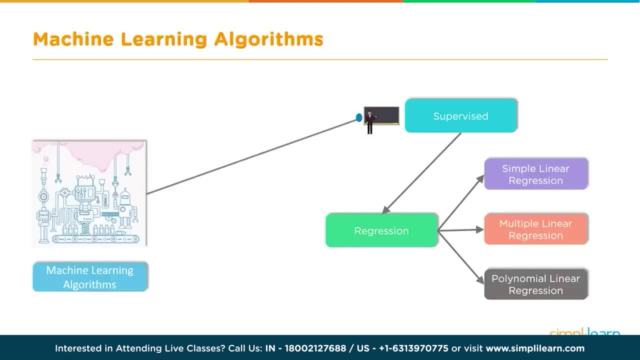 of data and we draw a straight line through it. Multiple linear regression means we have multiple variables. Remember where we had the rainfall and the crops. We might add a lot of additional variables in there, like: how much food do we give our crops? When do we harvest? 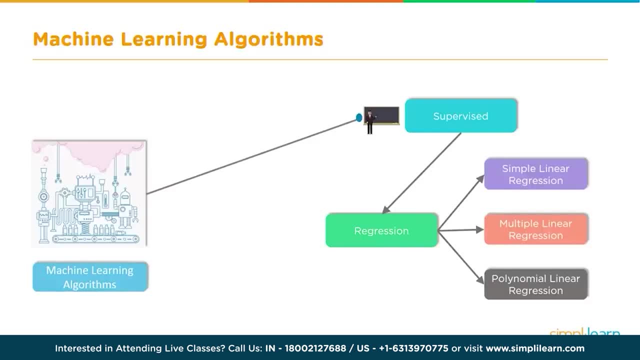 them. Those would be additional information added into our model and that's why it would be multiple linear regression. And finally, we have polynomial linear regression, That is, instead of drawing a line, we can draw a curved line through it. Now that you see where regression model fits into the 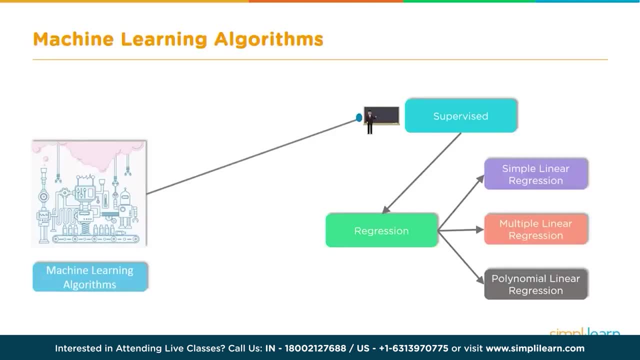 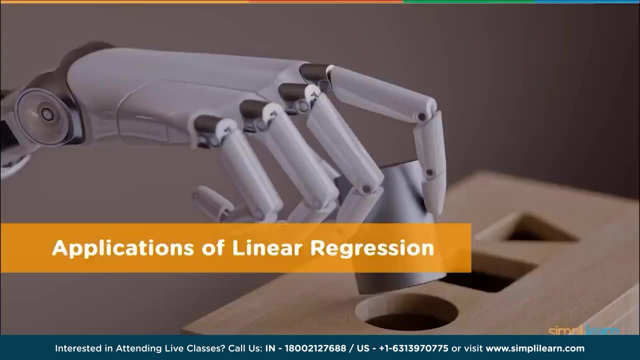 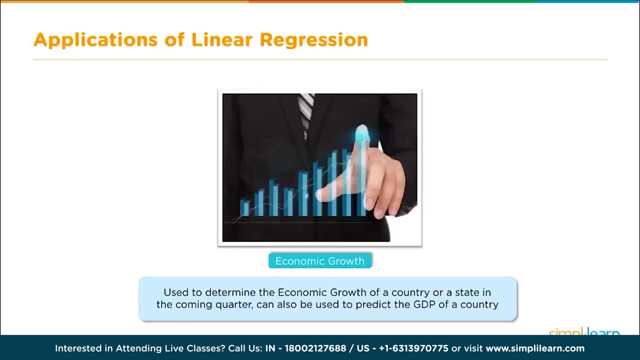 machine learning algorithms and we're specifically looking at linear regression. let's go ahead and take a look at applications for linear regression. Let's look at a few applications of linear regression. Economic growth, used to determine the economic growth of a country or a state in the coming quarter, can also be used to predict the GDP. 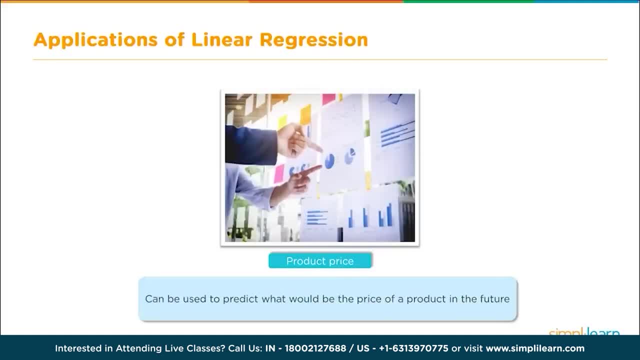 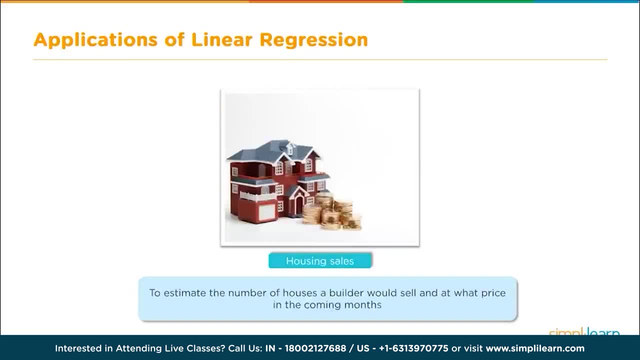 of a country. Product price can be used to predict what would be the price of a product in the future. We can guess whether it's going to go up or down. or should I buy today Housing sales to estimate the number of houses a builder would sell and what price in the coming months? Score predictions. 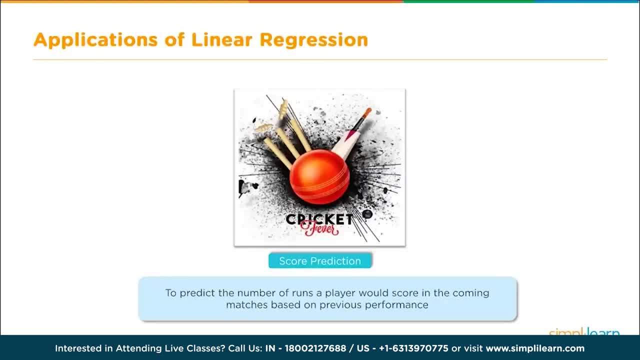 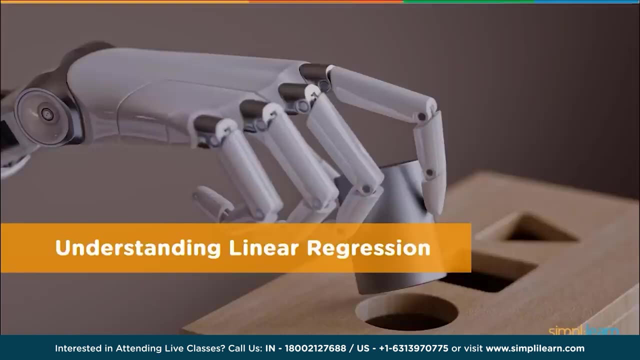 Cricket fever to predict the number of runs a player would score in the coming matches based on the previous performance. I'm sure you can figure out other applications you could use linear regression for. So let's jump in and let's understand linear regression and dig into the theory Understanding linear regression. Linear regression. 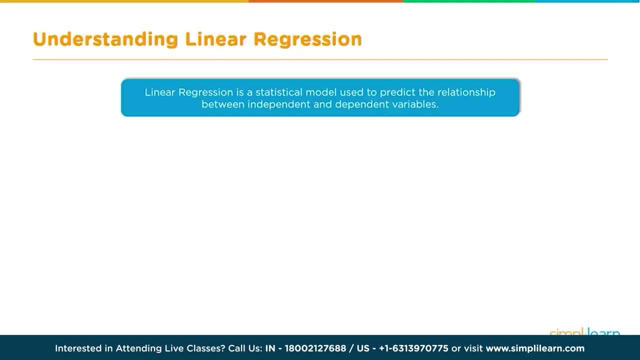 is a statistical model used to predict the relationship between independent and dependent variables by examining two factors. The first important one is which variables in particular are significant predictors of the outcome variable, And the second one that we need to look at closely is how significant is the regression line. 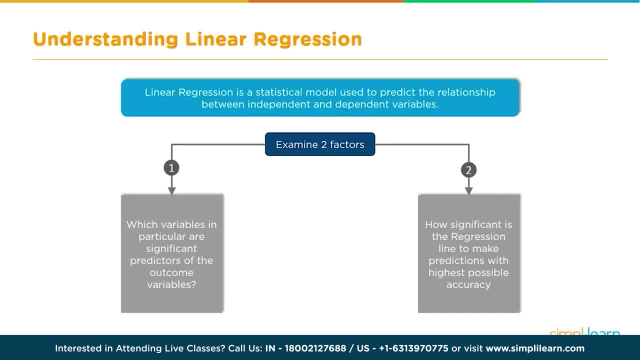 to make predictions with the highest possible accuracy. If it's inaccurate, we can't use it. So it's very important we find out the most accurate line we can get. Since linear regression is based on drawing a line through data, we're going to jump back and take a look. 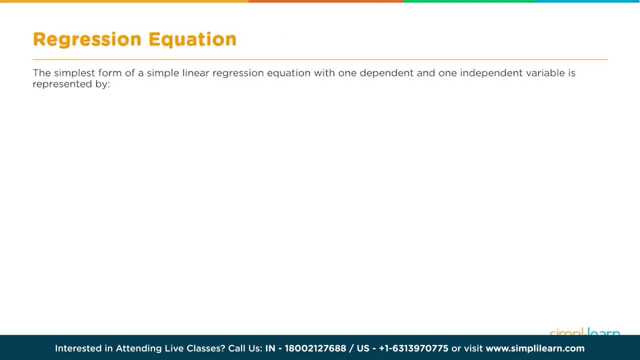 at some Euclidean geometry. The simplest form of a simple linear regression equation with one dependent and one independent variable is represented by: y equals m times x plus c. And if you look at our model here, we plotted two points on here: x1 and y1,, x2 and y2.. 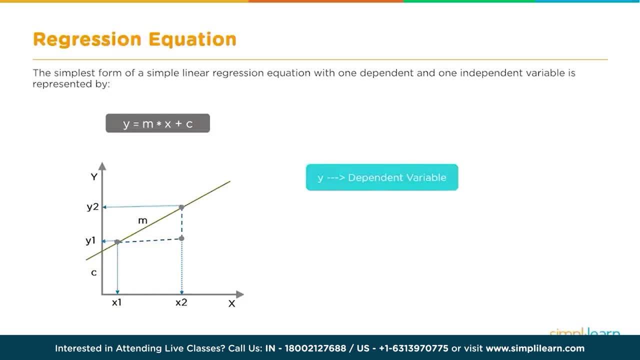 y being the dependent variable- Remember that from before- And x being the independent variable. So y depends on whatever x is. m, in this case, is the slope of the line where m equals the difference in the y2 minus y1 and x2 minus x1.. And finally, 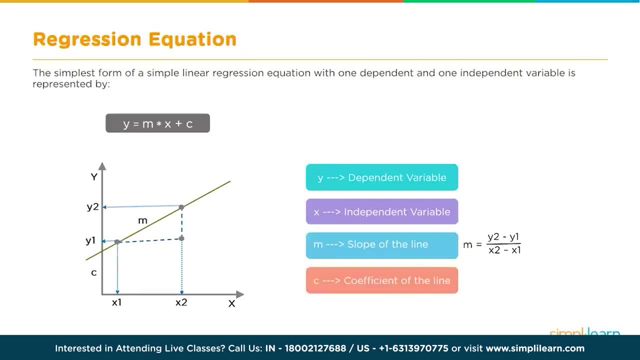 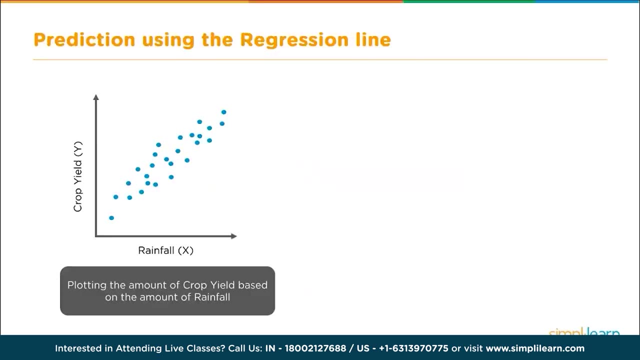 we have c, which is the coefficient of the line, or where it happens to cross the zero axes. Let's go back and look at an example we used earlier of linear regression. We're going to go back to plotting the amount of crop yield based on the amount of rainfall. 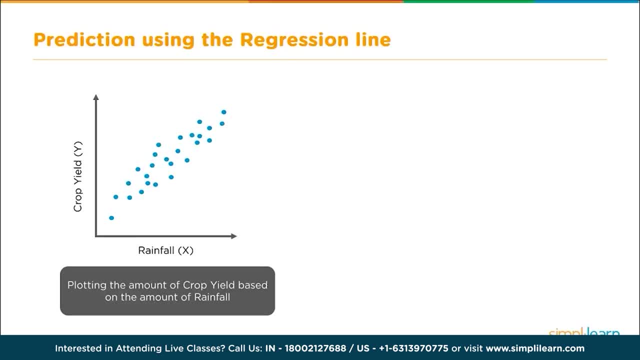 And here we have our rainfall- Remember, we cannot change rainfall- And we have our crop yield, which is dependent on the rainfall. So we have our independent and our dependent variables. We're going to take this and draw a line through it as best we can. 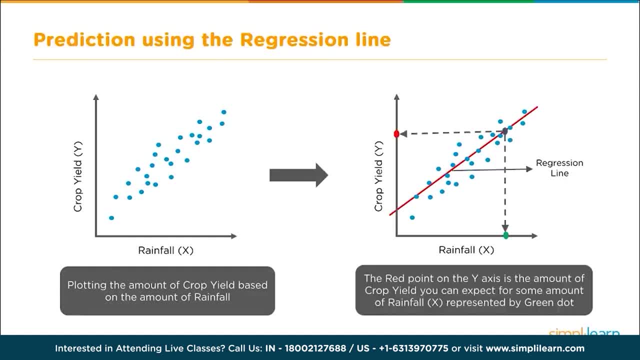 through the middle of the data And then we look at that. We put the red point on the y axes as the amount of crop yield you can expect for the amount of rainfall represented by the green dot. So if we have an idea what the rainfall is for this year and what's going on, then we can guess how. 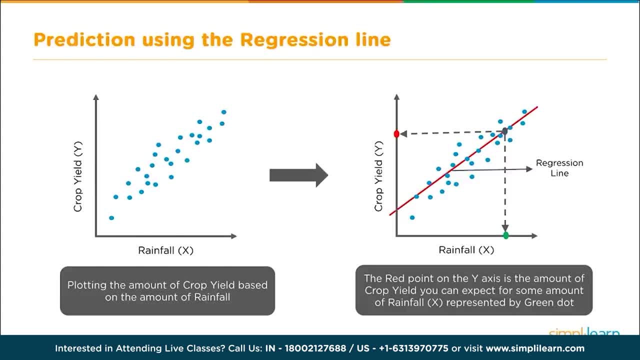 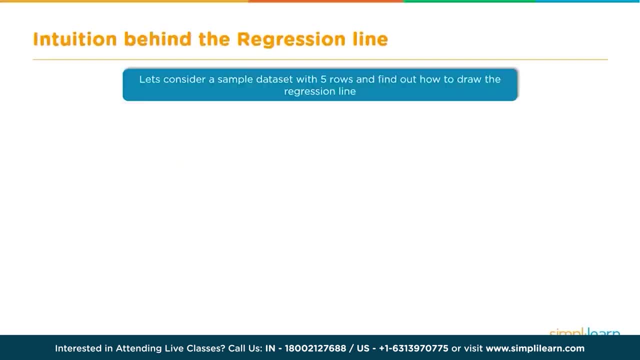 good our crops are going to be And we've created a nice line right through the middle to give us a nice mathematical formula. Let's take a look and see what the math looks like behind this. Let's look at the intuition behind the regression line. Now, before we dive into the math, 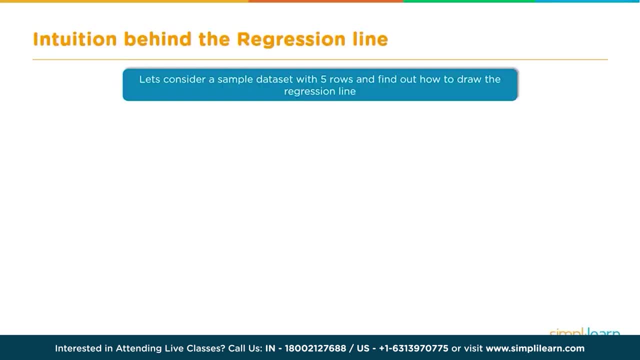 and the formulas that go behind this and what's going on behind the scenes. I want you to note that when we get into the case study and we actually apply some Python script, that this math that you're going to see here is already done automatically for you. 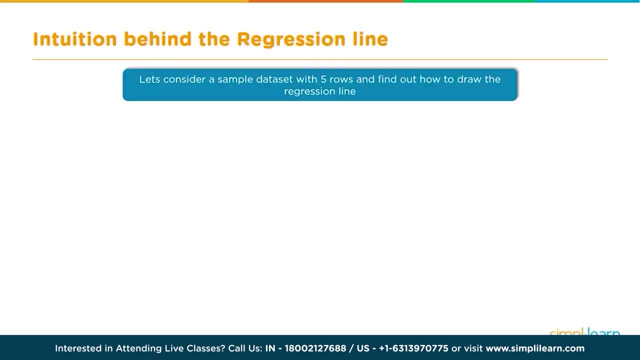 You don't have to have it memorized. It is, however, good to have an idea what's going on. so if people reference the different terms, you'll know what they're talking about. Let's consider a sample data set with five rows and find out how to draw the regression line. 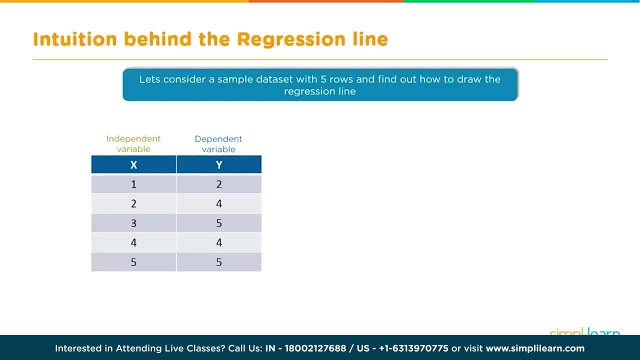 We're only going to do five rows because if we did like the rainfall, with hundreds of points of data, that would be very hard to see what's going on with the mathematics. So we'll go ahead and create our own two sets of data And we have our independent variable x and our dependent variable. 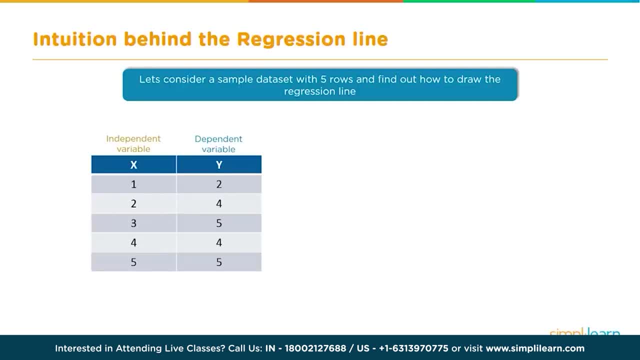 y, And when x was 1,, we got y equals 2.. When x was 2,, y was 4, and so on and so on. If we go ahead and plot this data on a graph, we can see how it forms a nice line through the middle. 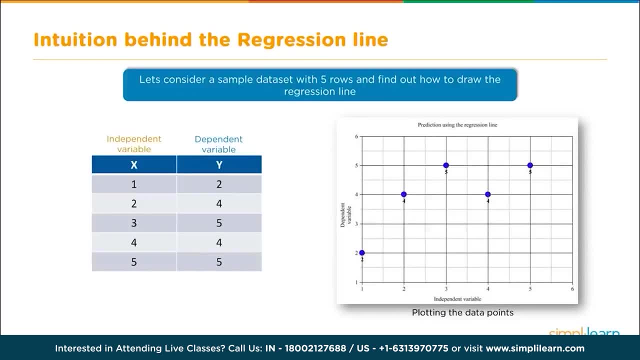 You can see where it's kind of grouped, going upwards to the right. The next thing we want to know is what the means is of each of the data coming in, the x and the y. The means doesn't mean anything other than the average, So we add up all the numbers and divide by the total. 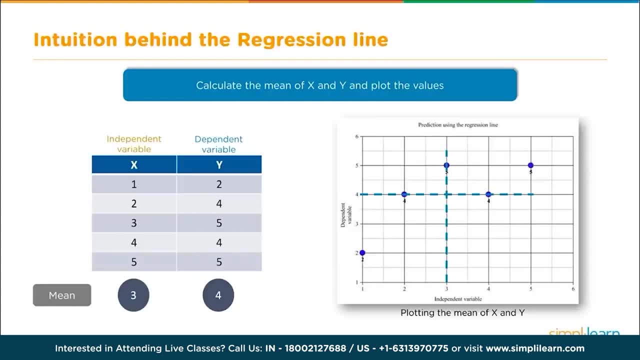 So 1 plus 2 plus 3 plus 4 plus 5 over 5 equals 3.. And the same for y: We get 4.. If we go ahead and plot the means on the graph, we'll see we get 3 comma 4, which draws a nice line down the middle. A good estimate. 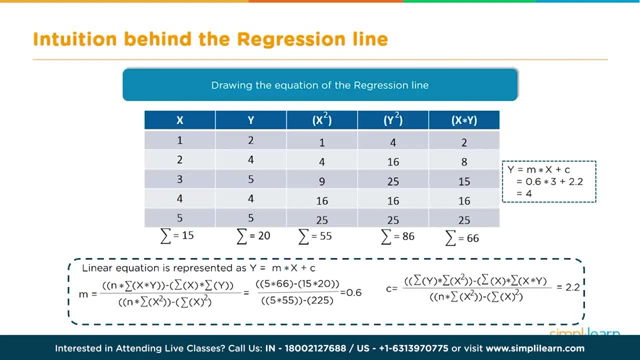 Here we're going to dig deeper into the math behind the regression line. Now remember before I said, you don't have to have all these formulas memorized or fully understand them, even though we're going to go into a little more detail of how it works. And if you're not a math whiz, 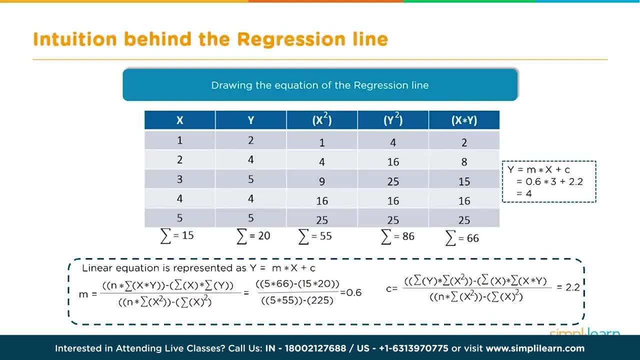 and you don't know if you've never seen the sigma character before, which looks a little bit like an e that's opened up. that just means summation, That's all that is. So when you see the sigma character, it just means we're adding everything in that row, And for computers, this is great. 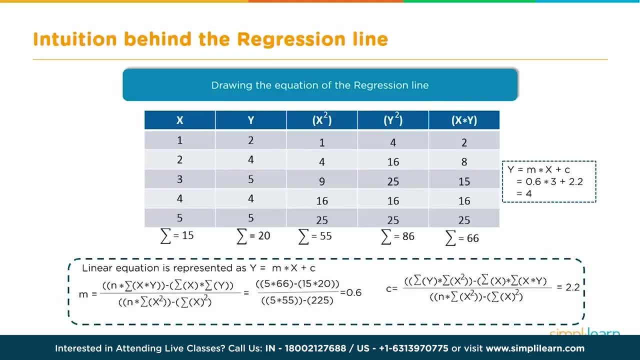 Because as a programmer you can easily iterate through each of the x- y points and create all the information you need. So in the top half you can see where we've broken that down into pieces And as it goes through the first two points it computes the squared value of x. the squared value. 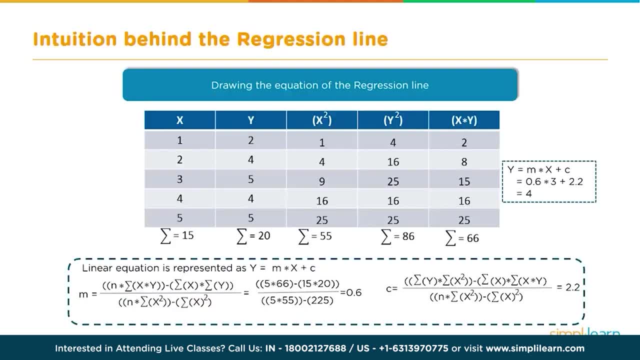 of y and x times y. And then it takes all of x and adds them up, All of y adds them up, All of x squared adds them up, And so on and so on, And you can see we have: the sum is equal to 15.. The sum is equal to 20.. All the way up to x times y, where the sum equals. 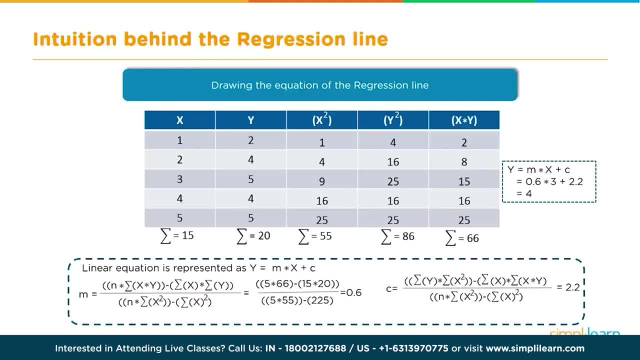 66. This all comes from our formula for calculating a straight line where y equals the slope times x plus the coefficient c. So we go down below and we're going to compute more like the averages of these And we're going to explain exactly. 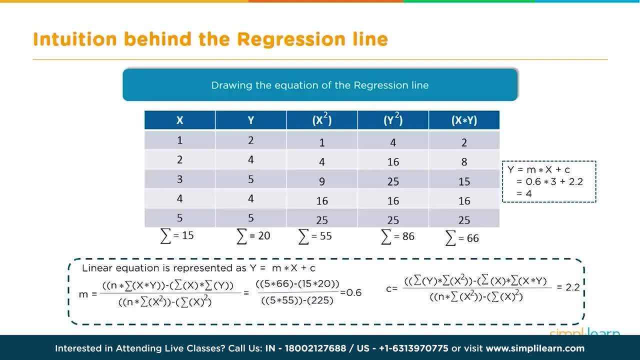 what that is in just a minute And where that information comes from is called. the square means error, But we'll go into that in detail in a few minutes. All you need to do is look at the formula and see how we've gone about computing it line by line, instead of trying to have a huge 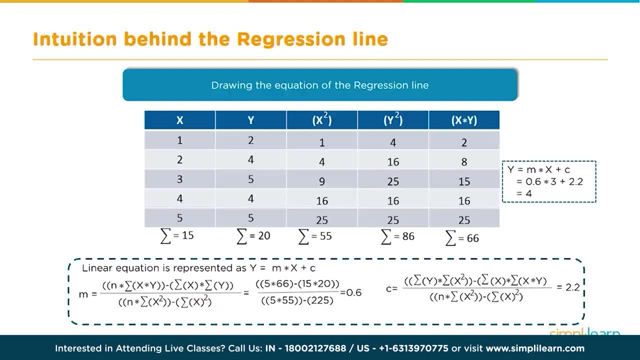 set of numbers pushed into it And down here you'll see where the slope m equals. and in the top part, if you read through the brackets, you have the number of data points times the sum of x times y, which we computed one line at a time there, And that's just the 66. And take all that and you subtract. 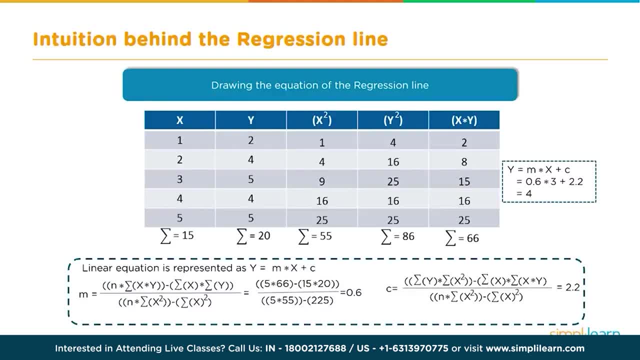 it from the sum of x times the sum of y, And those have both been computed, So you have 15 times 20.. And on the bottom we have the number of lines times the sum of x, squared, easily computed as 86, for the sum minus. 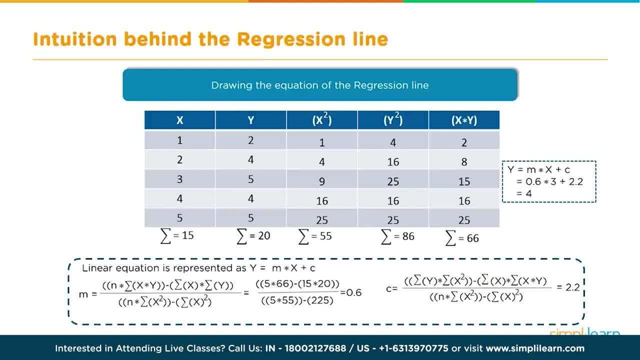 I'll take all that and subtract the sum of x squared And we end up, as we come across, with our formula. you can plug in all those numbers, which is very easy to do on the computer- You don't have to do the math on a piece of paper or calculator- And you'll get a slope of 0.6.. 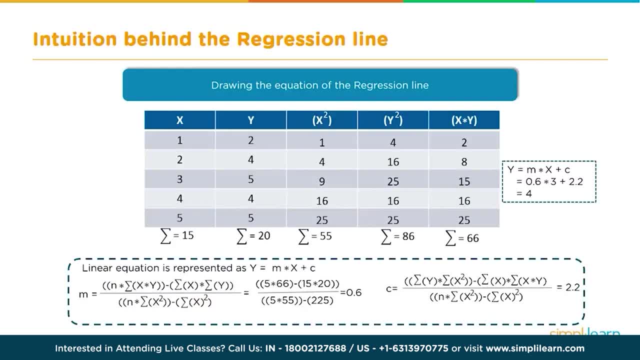 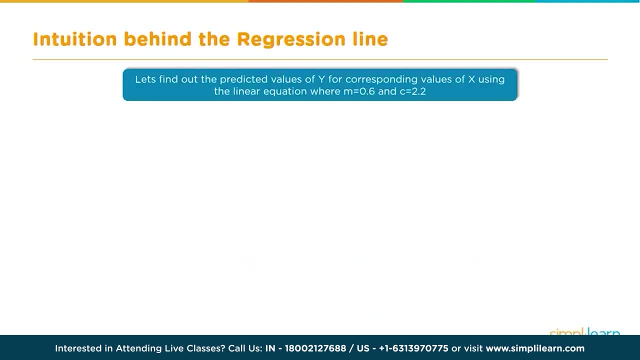 And you'll get your c coefficient. If you continue to follow through that formula, you'll see it comes out as equal to 2.2.. Continuing deeper into what's going behind the scenes, let's find out the predicted values of y for corresponding values of x using the linear. 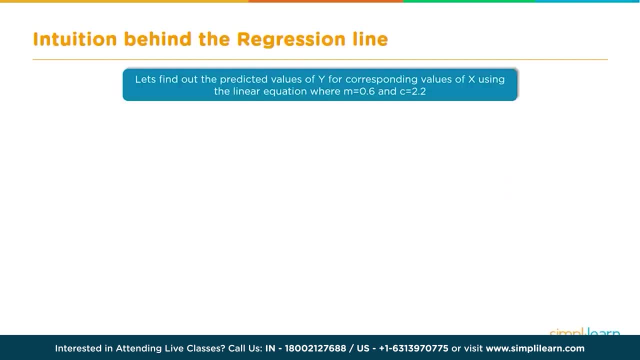 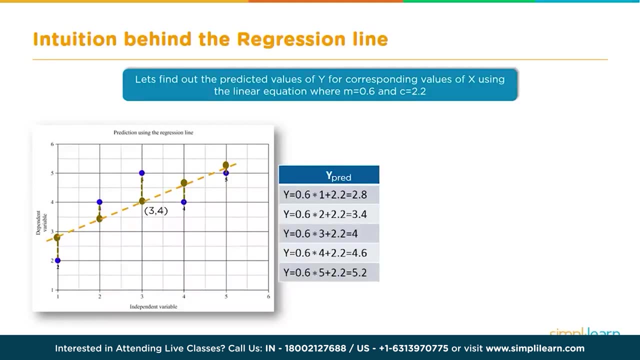 equation where m equals 0.6 and c equals 2.2.. We're going to take these values and we're going to go ahead and plot them, We're going to predict them. So y equals 0.6 times where x equals 1, plus 2.2 equals 2.8, so on and so on. 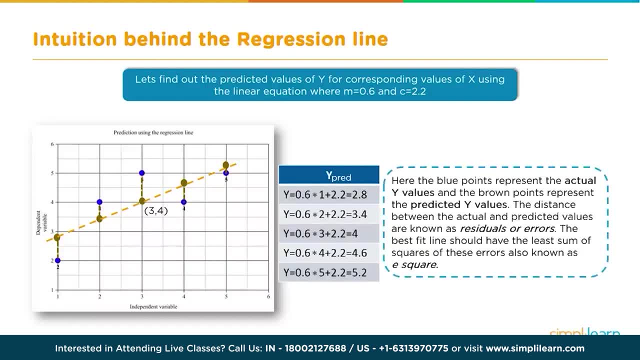 And here the blue points represent the actual y values And the brown points represent the predicted y values. based on the model we created, The distance between the actual and predicted values is known as residuals or errors. The best fit line should have the least sum of squares of these errors, also known as. 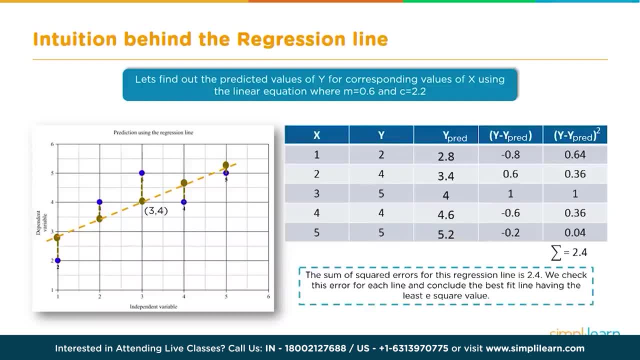 e squared. If we put these into a nice chart where you can see x and you can see y- what the actual values were, and you can see y predicted, you can easily see where we take y minus y predicted and we get an answer. What is the difference between those two? 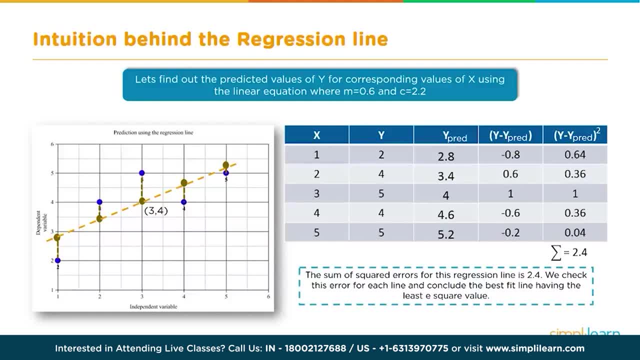 And if we square that y minus y- prediction squared, we can then sum those squared values. That's where we get the 0.64 plus the 0.36 plus 1, all the way down until we have a summation equals 2.4.. So the sum of squared errors 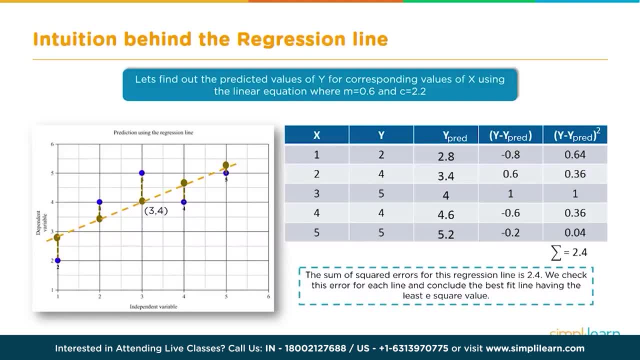 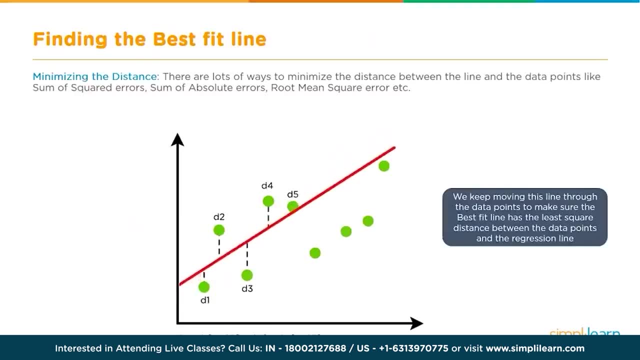 for this regression line is 2.4.. We check this error for each line and conclude the best fit line having the least e squared value In a nice graphical representation. we can see here where we keep moving this line through the data points to make sure the best fit line. 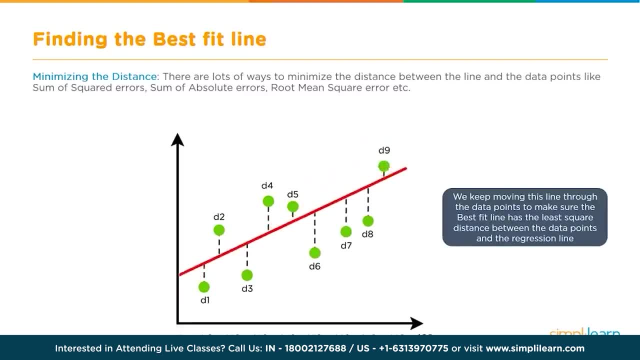 has the least squared distance between the data points and the regression line. Now we only looked at the most commonly used formula for minimizing the distance. There are lots of ways to minimize the distance between the line and the data points, like sum of squared errors, sum of absolute errors, root mean, square error, etc. 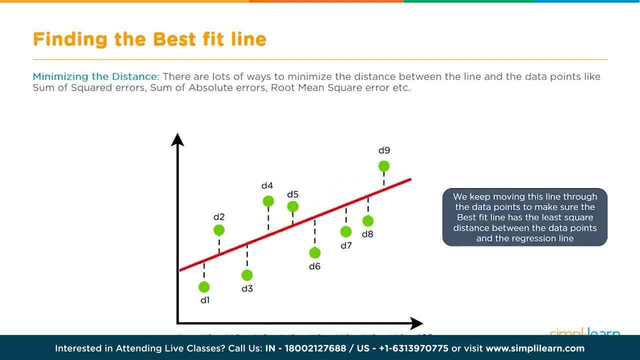 What you want to take away from this is, whatever formula is being used, you can easily, using computer programming and iterating through the data, calculate the different parts of it. That way, these complicated formulas you see, with the different summations and absolute values, are easily computed, one piece at a time, Up until this point. 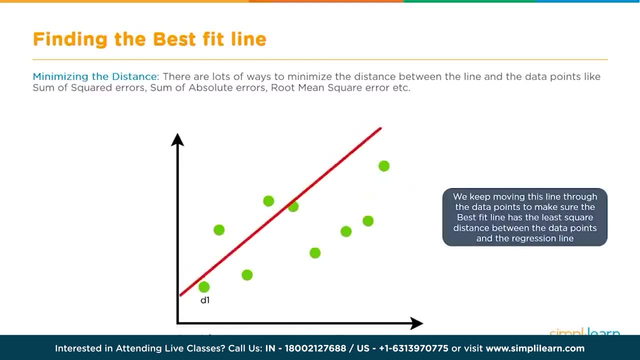 we've only been looking at two values: x and y. Well, in the real world, it's very rare that you only have two values when you're figuring out a solution. So let's move on to the next topic: multiple linear regression. Let's take a brief look at what happens when you 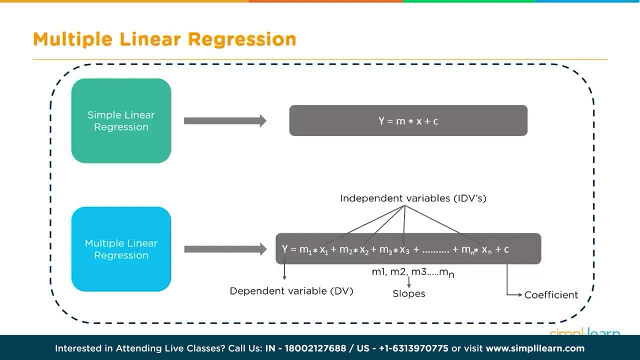 have multiple inputs. So in multiple linear regression we have. well, we'll start with the simple linear regression where we had y equals m plus x plus c And we're trying to find the value of y. Now, with multiple linear regression, we have multiple variables. 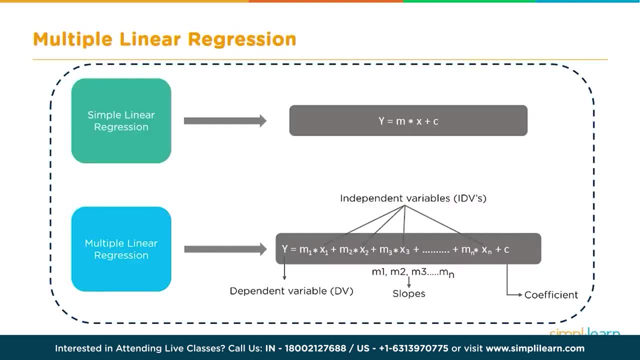 coming in. So instead of having just x, we have x1, x2, x3. And instead of having just one slope, each variable has its own slope attached to it. As you can see, here we have m1, m2, m3. And we still just have the single coefficient. So when you're 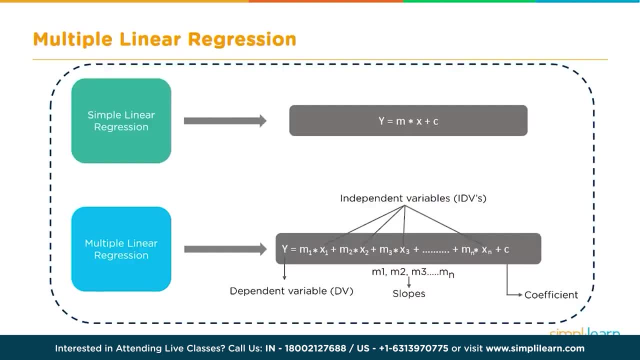 dealing with multiple linear regression. you basically take your single linear regression and you spread it out, So you have y equals m1 times x plus c, And you're adding x1 plus m2 times x2.. So on all the way to m to the nth, x to the nth, And then 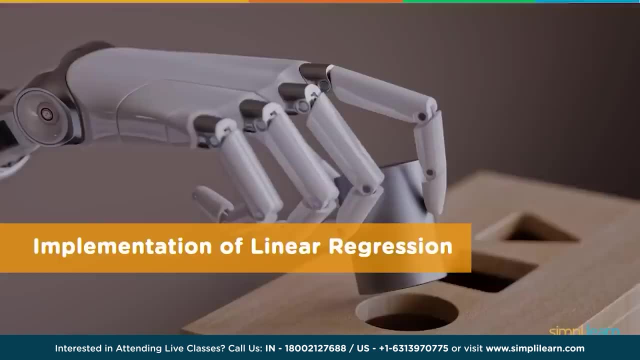 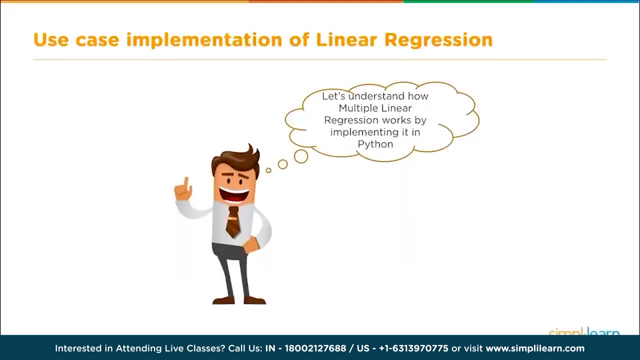 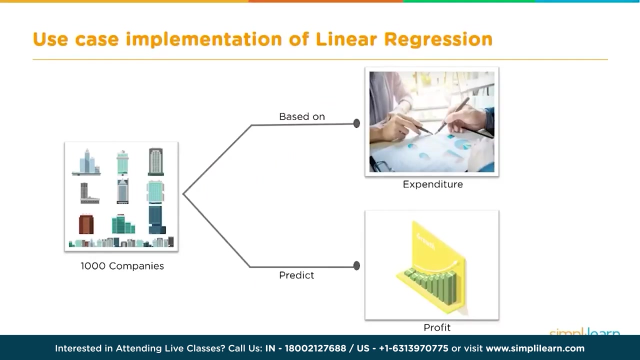 you add your coefficient on there. Implementation of linear regression: Now we get into my favorite part. Let's understand how multiple linear regression works by implementing it in Python. If you remember, before we were looking at a company and, just based on its R&D, trying to figure out its profit. We're going to start looking at the expenditure. 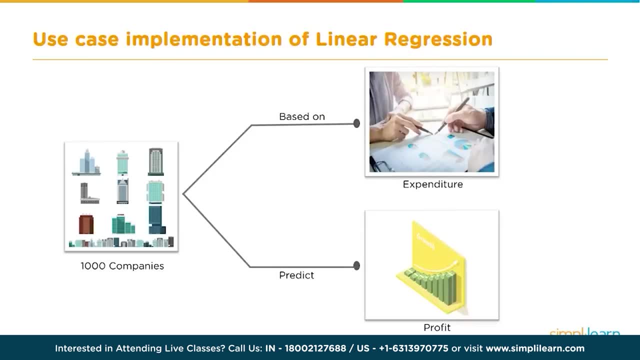 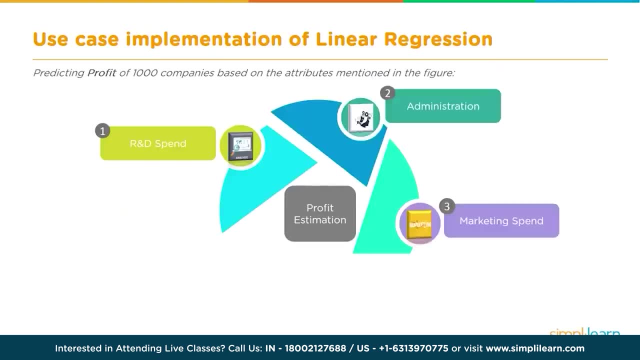 of the company. We're going to go back to that. We're going to predict its profit. But instead of predicting it just on the R&D, we're going to look at other factors like administration costs, marketing costs and so on, And from there we're going to see. 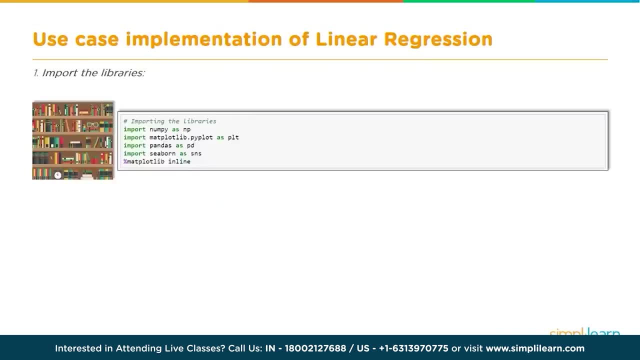 if we can figure out what the profit of that company is going to be. To start our coding, we're going to begin by importing some basic libraries And we're going to be looking through the data before we do any kind of linear regression. We're going to take a 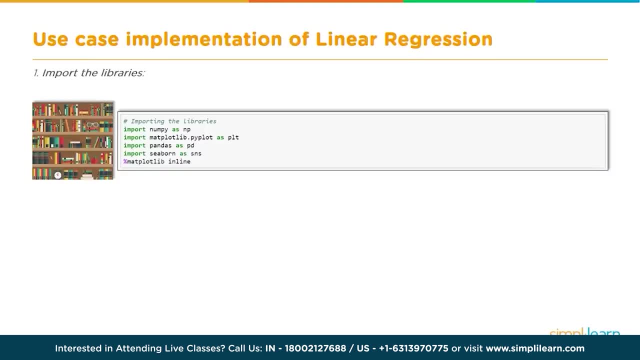 look at the data to see what we're playing with. Then we'll go ahead and format the data to the format we need to be able to run it in the linear regression model And then from there we'll go ahead and solve it and just see how valid our solution is. So let's 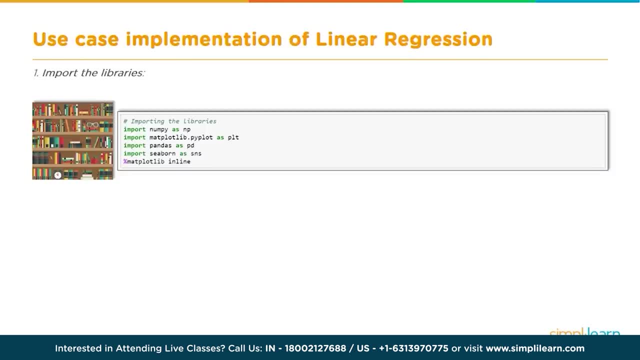 start with importing the basic libraries. Now I'm going to be doing this in Anaconda Jupyter Notebook, a very popular IDE. I enjoy it because it's such a visual to look at and it's so easy to use. Just any IDE for Python will work just fine for this. So break out. 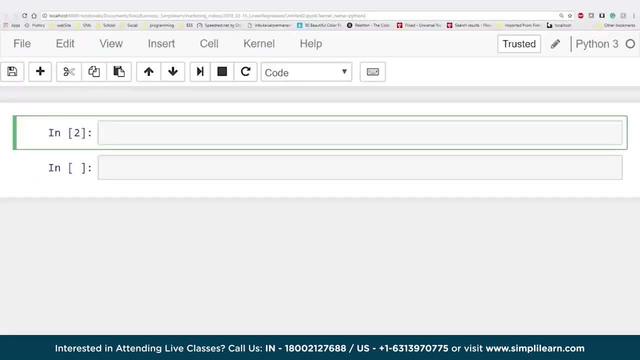 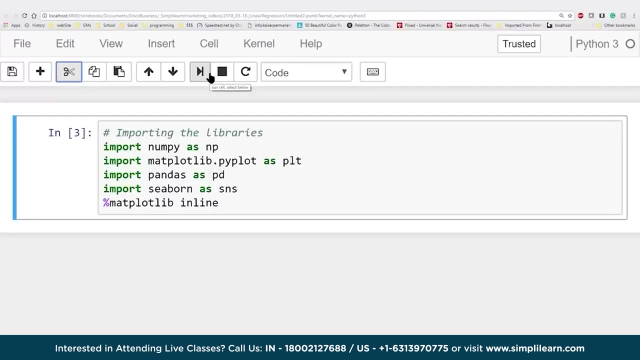 your favorite Python IDE. So here we are in our Jupyter Notebook. Let me go ahead and paste our first piece of code in there And let's walk through what libraries we're importing. First we're going to import numpy as np, And then I want you to skip one line and look. 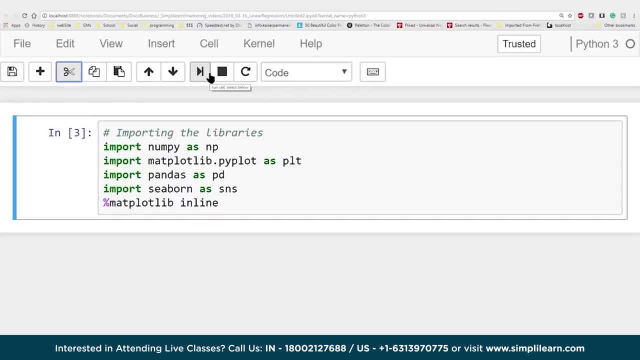 at import pandas as pd. These are very common tools that you need with most of your linear regression. The numpy, which stands for number Python, is usually denoted as np And you have to almost have that for your sklearn toolbox. You always import that right off the. 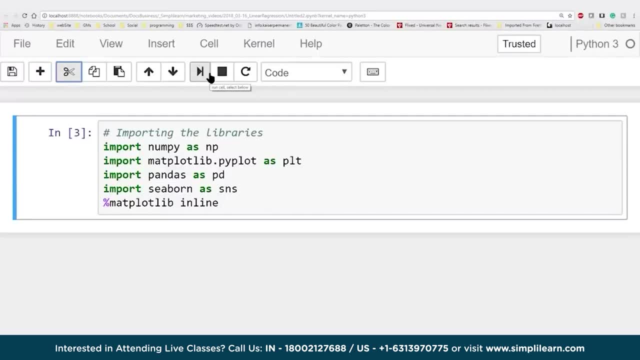 beginning Pandas. although you don't have to have it for your sklearn libraries, it does such a wonderful job of importing data, setting it up into a data frame so we can manipulate it rather easily, And it has a lot of tools also in addition to that, So we usually like to use the pandas. 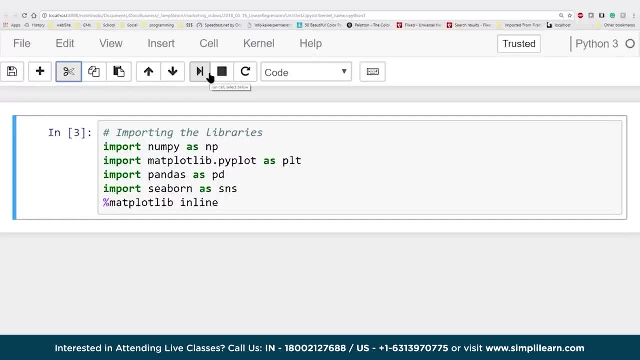 when we can, And I'll show you what that looks like. The other three lines are for us to get a visual of this data and take a look at it. So we're going to import matplotlibrarypyplot as plt And then seaborn as sns. Seaborn works with the matplot library, So you have to always 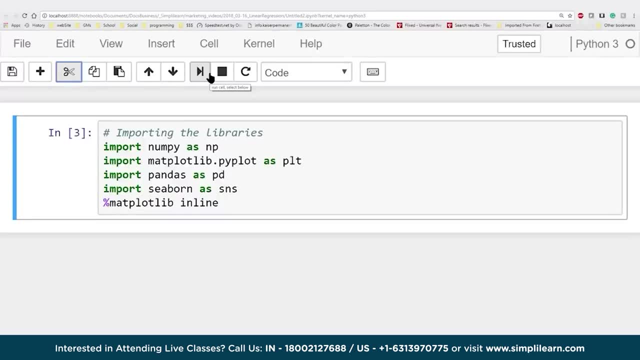 import matplotlibrary and then seaborn sits on top of it, And we'll take a look at what that looks like. You could use any of your own plotting libraries you want. There's all kinds of ways to look at the data. These are just very common ones, and the 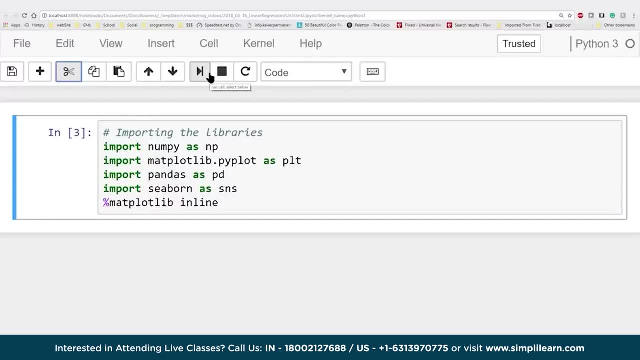 seaborn is so easy to use that it just looks beautiful. It's a nice representation that you can actually take and show somebody. And the final line is the amberson matplotlibrary inline. That is only because I'm doing an inline IDE, My interface in the Anaconda Jupyter Notebook. 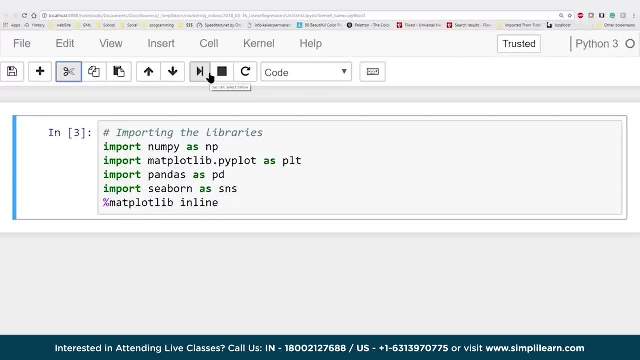 requires. I put that in there, or you're not going to see the graph when it comes up. Let's go ahead and run this. It's not going to be that interesting because we're just setting up variables. In fact, it's not going to do anything that we can see, but it is importing these. 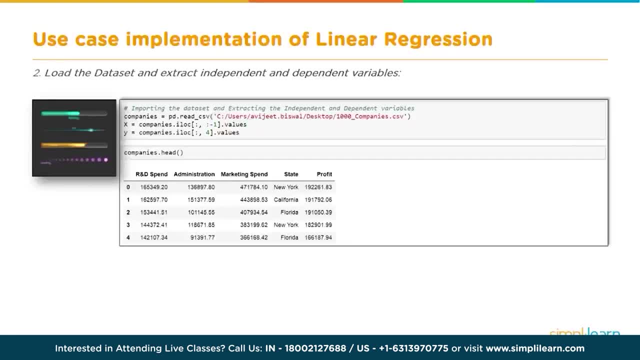 different libraries and setup. The next step is load the dataset and extract independent and dependent variables. Now here in the slide you'll see companies equals pdreadcsv and it has a long line there with the file at the end 1000companiescsv. You're going to have to change this. 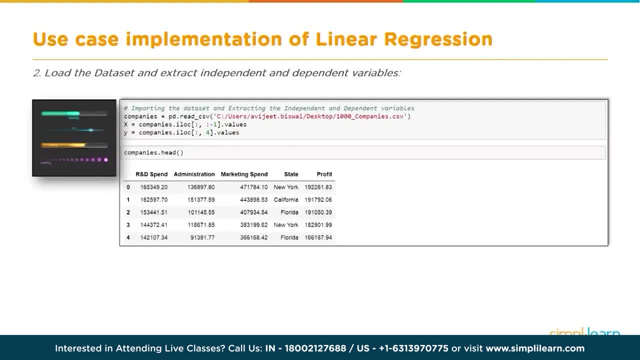 to fit whatever setup you have And the file itself you can request. Just go down to the commentary below this video and put a note in there and SimplyLearn will try to get in contact with you and supply you with that file so you can try this coding yourself. So we're going to add this code in here. 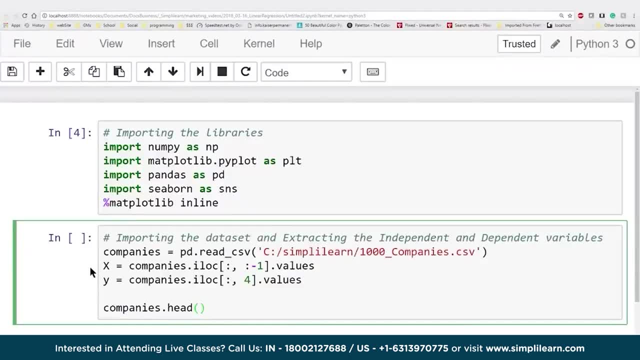 and we're going to see that I have companies equals pdreadercsv and I've changed this path to match my computer C colon slash SimplyLearn. slash 1000 underscore companies dot, csv, And then below there we're going to set the x equals to companies under the i location and because this is companies is a. 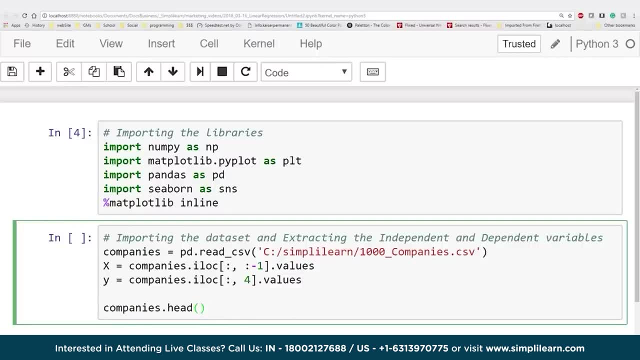 pd dataset. I can use this nice notation that says: take every row, that's what the colon, the first colon, is comma, except for the last column. That's what the second part is, where we have a colon minus one And we want the values set into there. So x is no longer a dataset, a pandas dataset. But we can easily. 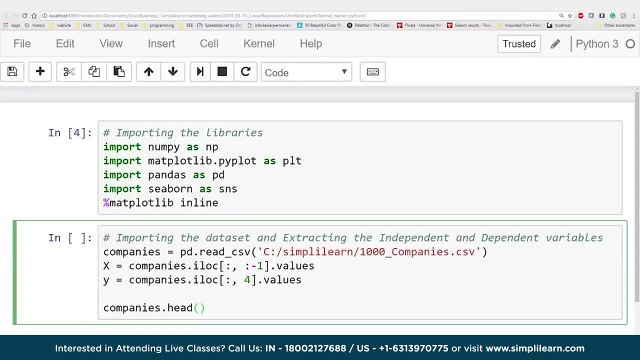 extract the data from our pandas dataset with this notation, And then y we're going to set equal to the last row. Well, the question is going to be: what are we actually looking at? So let's go ahead and take a look at that. 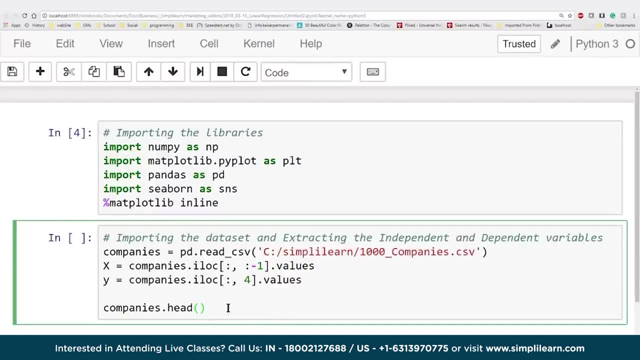 And we're going to look at the companies dot head, which lists the first five rows of data, And I'll open up the file in just a second so you can see where that's coming from. But let's look at the data in here. as far as 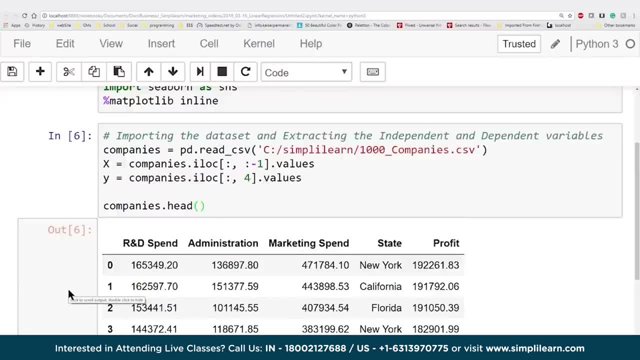 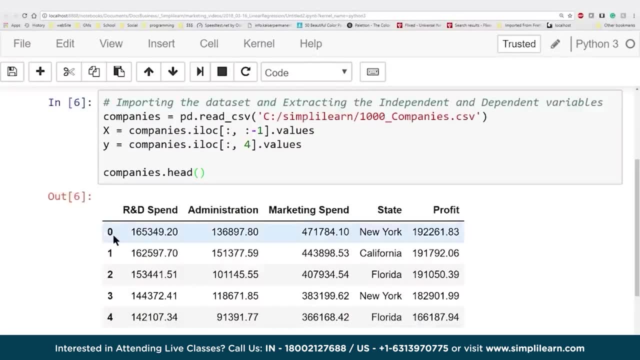 the way the pandas sees it. When I hit run, you'll see it breaks it out into a nice setup. This is what pandas. one of the things pandas is really good about is it looks just like an Excel spreadsheet. You have your rows and remember, when we're programming, we always start with zero, We don't start with one, So it shows the first. 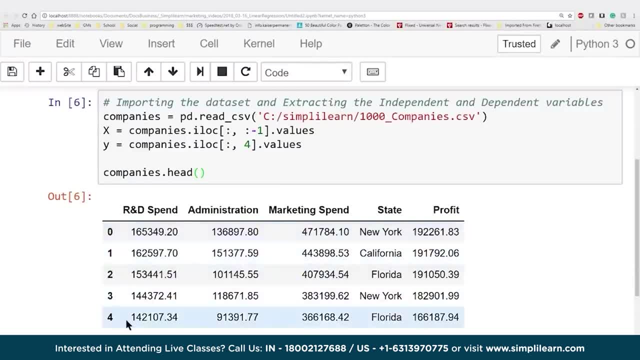 five rows: Zero, one, two, three, four, And then it shows your different columns: R&D spend, administration, marketing spend, state profit. It even notes that the top are column names. It was never told that, but pandas is able to recognize a lot of things that. 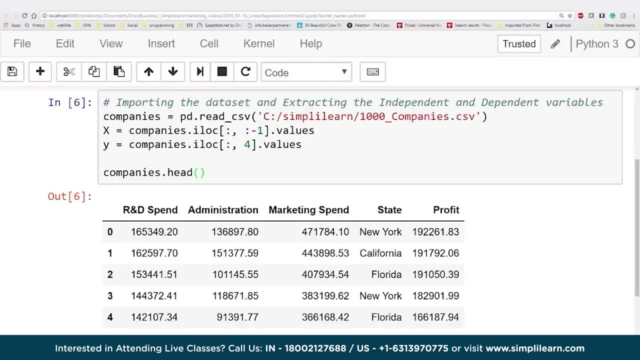 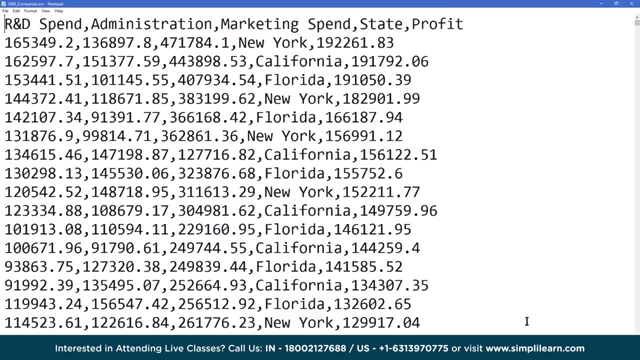 they're not the same as the data rows. Why don't we go ahead and open this file up in a CSV so you can actually see the raw data? So here I've opened it up as a text editor And you can see at the top we have R&D spend. 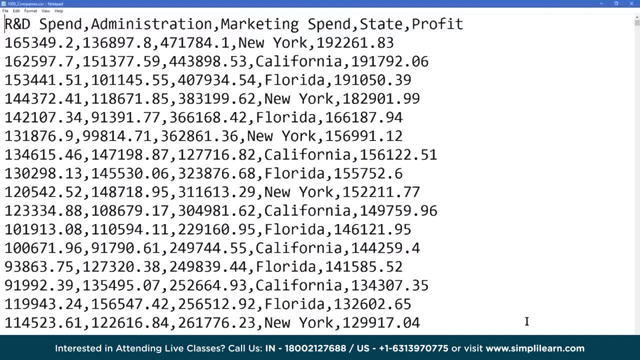 administration, marketing, spend, state profit. Can you see that? Yeah, And you can see that it carries return. I don't know about you, but I'd go crazy trying to read files like this. That's why we use the pandas. You could also open this up in an Excel and it would separate it, since it is a comma separated. 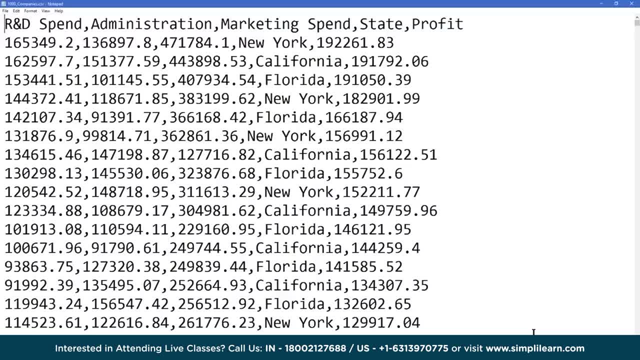 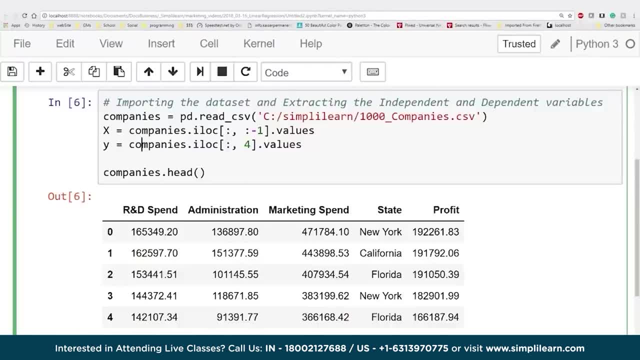 variable file. But we don't want to look at this one. We want to look at something we can read rather easily. So let's flip back and take a look at that top part, the first five rows. Now, as nice as this format is where I can see the data, to me it 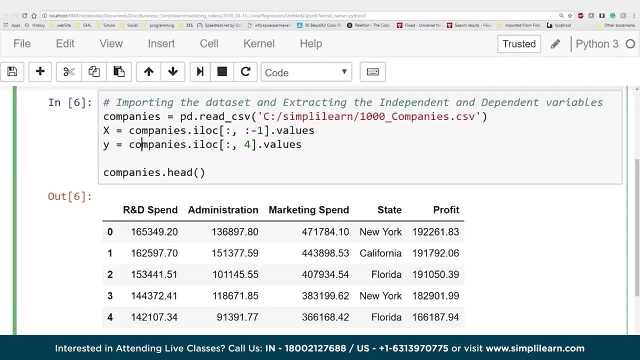 doesn't mean a whole lot. Maybe you're an expert in business and investments and you understand what: 165,340 dollars and 20 cents compared to the administration cost of 136,897 dollars and 80 cents, so on and so on. 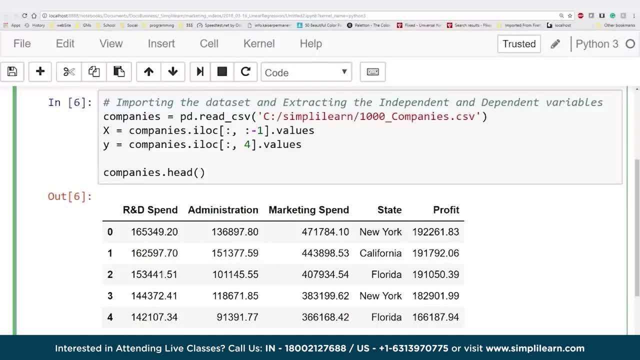 It helps to create the profit of 192,261 and 83 cents. That makes no sense to me whatsoever, No pun intended. So let's flip back here and take a look at our next set of code, where we're going to graph it so we can get a better. 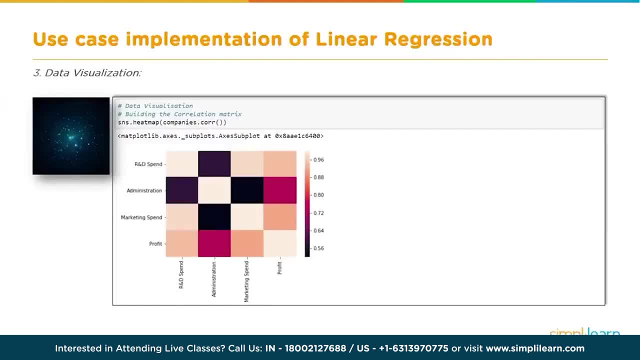 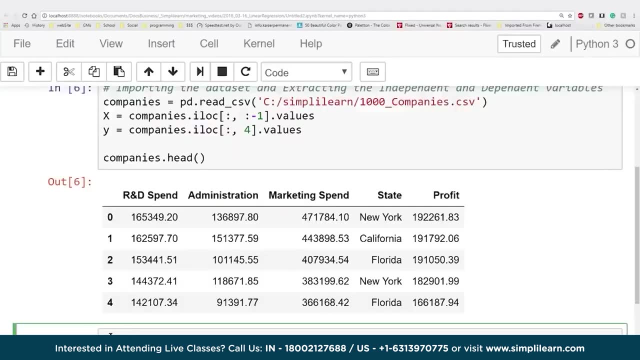 understanding of our data and what it means. So at this point we're going to use a single line of code to get a lot of information. So we can see where we're going with this. Let's go ahead and paste that into our notebook and see what we got going. 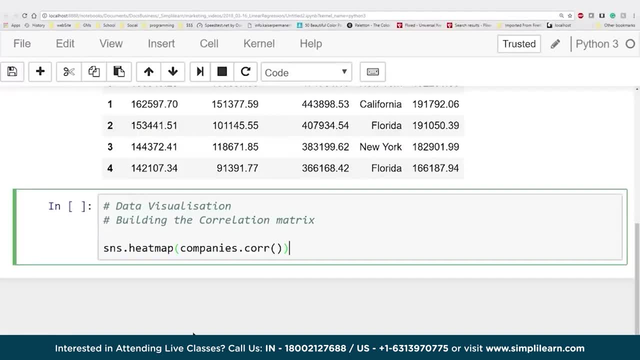 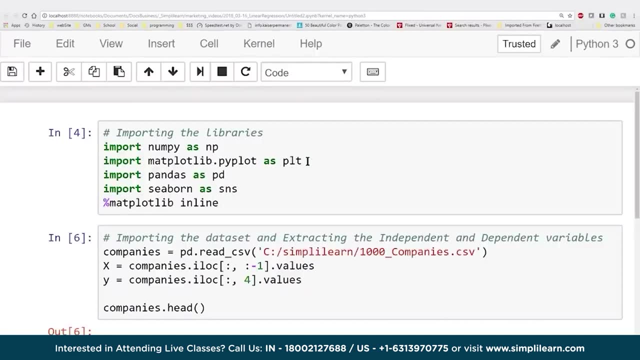 So we have the visualization and again we're using SNS, which is pandas. As you can see, we imported the matplotlibrarypyplot as plt, which then the seaborn uses, And we imported the seaborn as sns, And then that final line of code helps us show this in our inline coding. 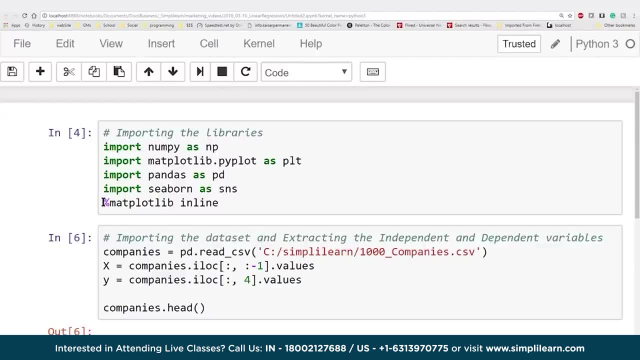 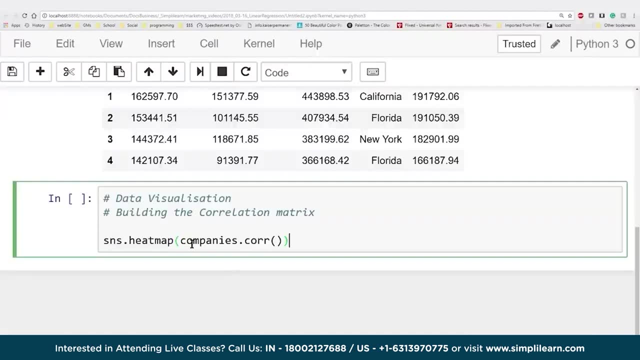 Without this it wouldn't display and you could display it to a file and other means And that's the matplotlibrary inline with the amber sign at the beginning. So here we come down to the single line of code. Seaborn is great because it actually recognizes the panda data frame. 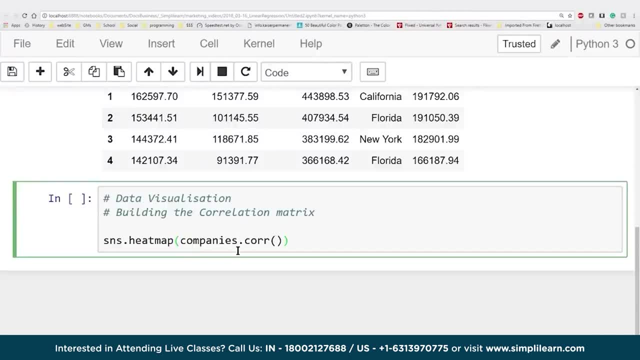 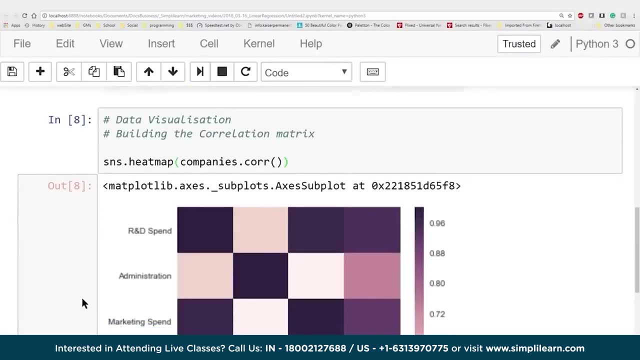 So I can just take the companiescore for coordinates and I can put that right into the seaborn. And when we run this we get this beautiful plot. And let's just take a look at what this plot means. If you look at this plot on mine, the colors are probably a little bit more purplish and blue than the original one. 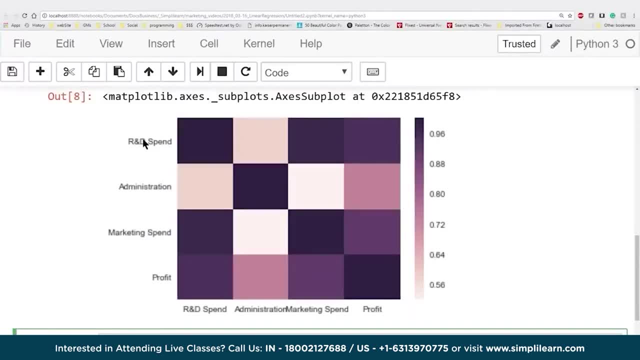 We have the columns and the rows, We have R&D spending, We have administration, We have marketing spending and profit. And if you cross index any two of these- since we're interested in profit- If you cross index profit with profit, it's going to show up. if you look at the scale on the right way up in the dark. 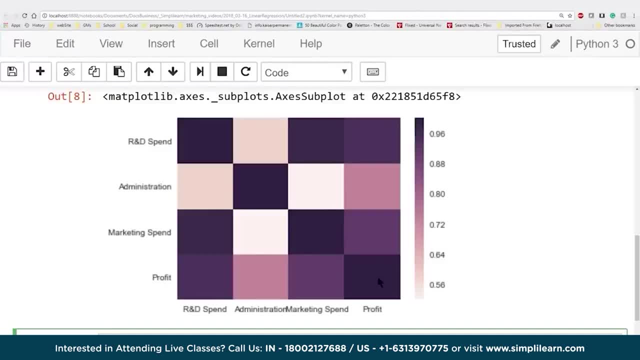 Why? Because those are the same data. They have an exact correspondence. So R&D spending is going to be the same as R&D spending and the same thing with administration costs. So right down the middle you get this dark row or dark column. 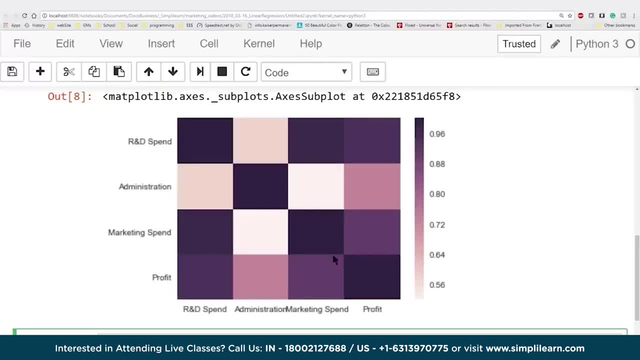 A diagonal row that shows that this is the highest corresponding data. that's exactly the same. And as it becomes lighter there's less connections between the data. So we can see: with profit, obviously profit is the same as profit. And next, it has a very high correlation with R&D spending, which we looked at earlier. 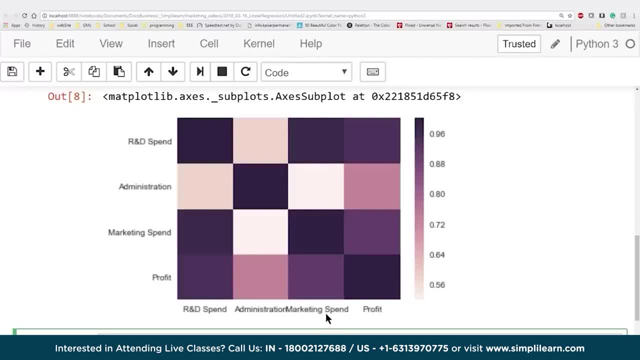 And it has a slightly less connection to marketing spending and even less to how much money we put into the administration. So now that we have a nice look at the data, Let's go ahead and dig in and create some actual useful linear regression models. 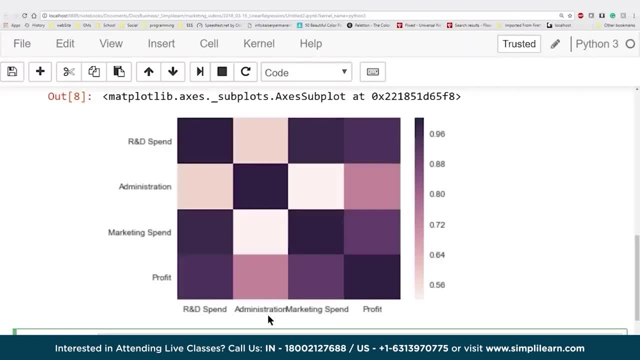 So that we can predict values and have a better profit. Now that we've taken a look at the visualization of this data, We're going to move on to the next step. Instead of just having a pretty picture, We need to generate some hard data. 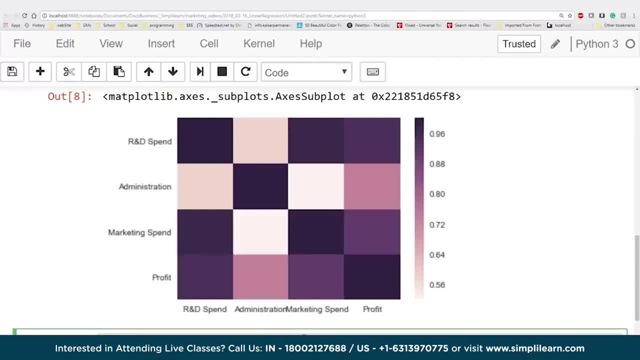 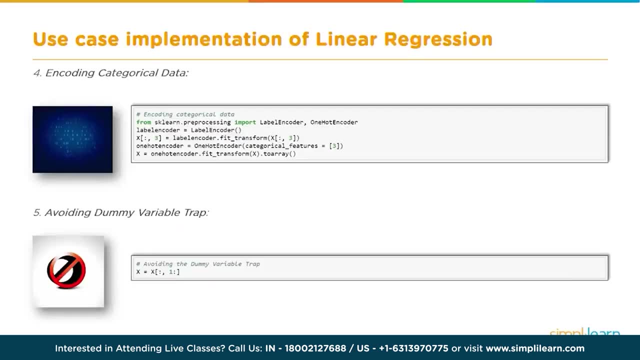 Some hard values. So let's see what that looks like. We're going to set up our linear regression model in two steps. The first one is we need to prepare some of our data so it fits correctly. Let's go ahead and paste this code into our Jupyter notebook. 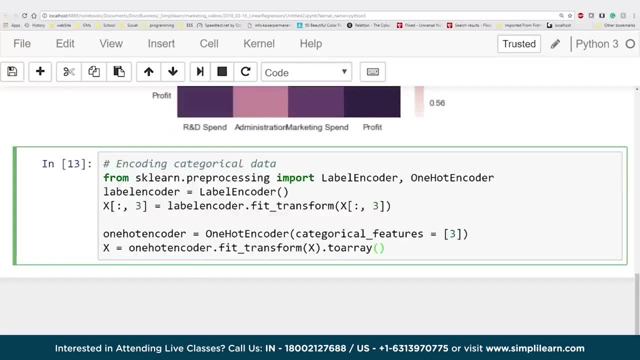 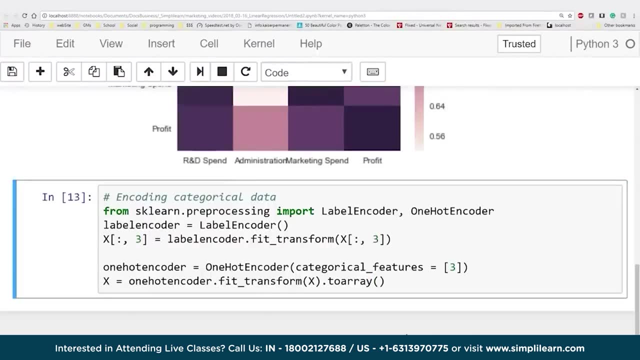 And what we're bringing in is we're going to bring in the sklearn preprocessing, Where we're going to import the label encoder and the one hot encoder To use the label encoder. we're going to create a variable called label encoder And set it equal to capital L label, capital E encoder. 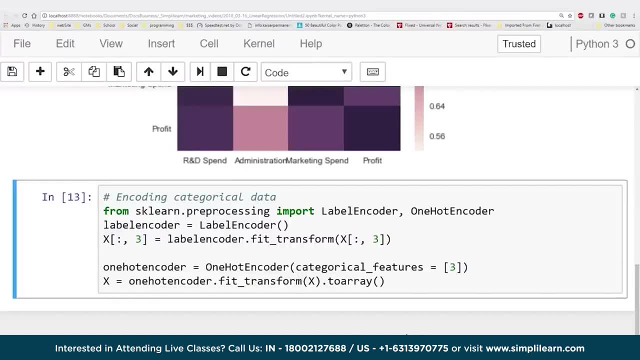 This creates a class that we can reuse for transferring the labels back and forth. Now about now, you should ask: what labels are we talking about? Let's go take a look at the data we processed before And see what I'm talking about here. 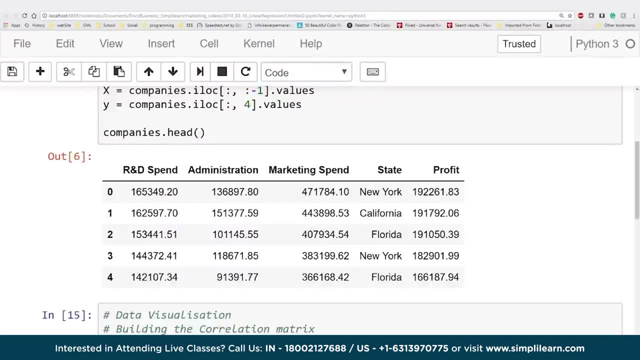 If you remember when we did the companieshead And we printed the top five rows of data, We have our columns going across. We have column zero, which is R&D spending, Column one, which is administration, Column two, which is marketing spending, And column three is state. 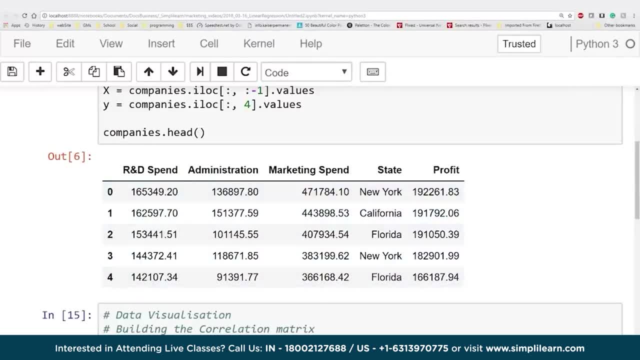 And you'll see, under state we have New York, California, Florida. Now to do a linear regression model, it doesn't know how to process New York. It knows how to process a number. So the first thing we're going to do is we're going to change that: New York, California and Florida. 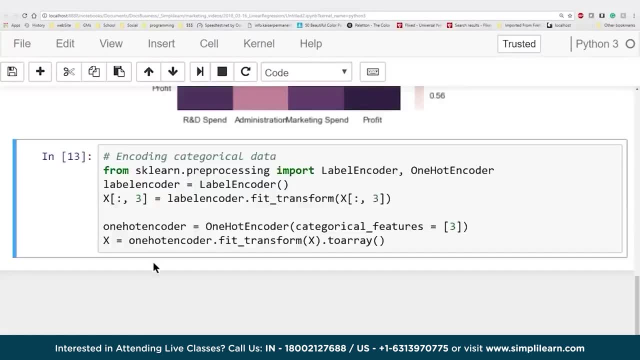 And we're going to change those to numbers, And that's what this line of code does here. X equals, and then it has the colon comma, three in brackets: The first part. the colon comma means that we're going to look at all the different rows. 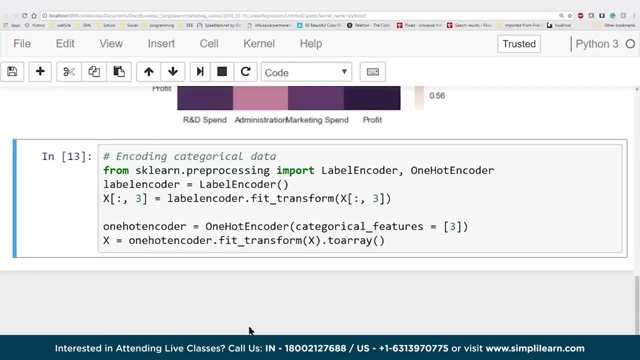 So we're going to keep them all together. But the only row we're going to edit is the third row And in there we're going to take the label coder And we're going to fit and transform the X. also the third row. 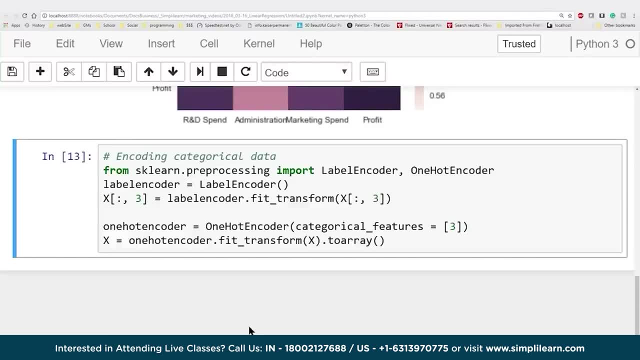 So we're going to take that third row and we're going to set it equal to a transformation, And that transformation basically tells it that instead of having a New York, It has a zero or a one or a two. And then, finally, we need to do a one hot encoder. 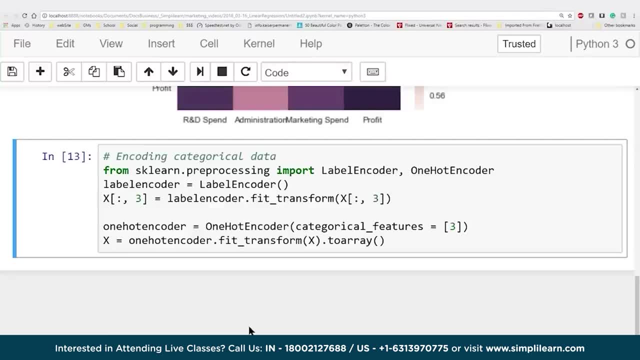 Which equals one hot encoder, categorical features equals three. And then we take the X and we go ahead and do that: equal to one hot encoder. fit. transform X to array. This final transformation preps our data for us. so it's completely set the way we need it. 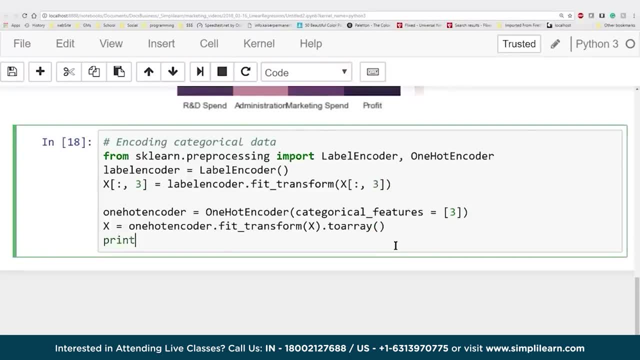 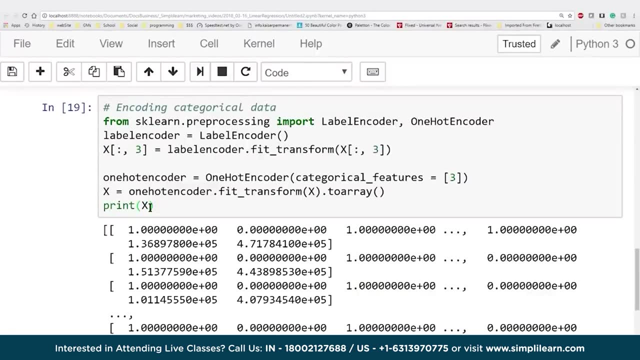 It's just a row of numbers. Even though it's not in here, let's go ahead and print X And just take a look at what this data is doing. You'll see you have an array of arrays And then each array is a row of numbers. 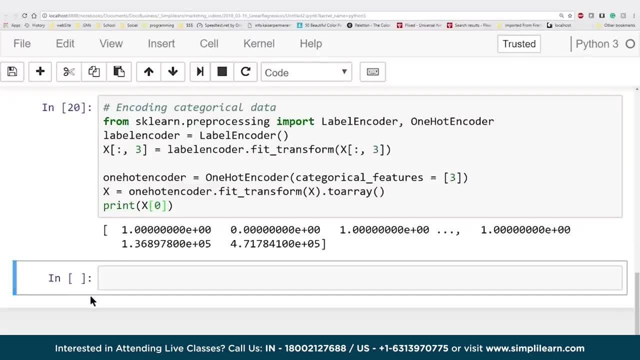 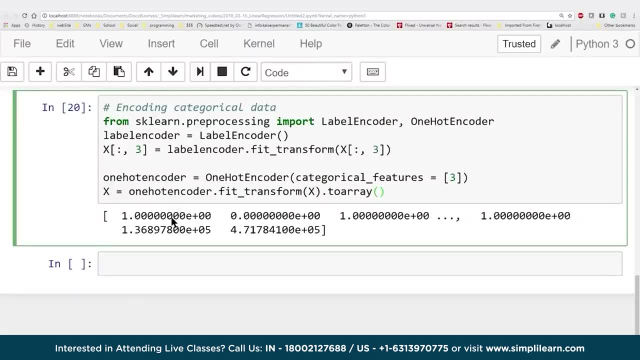 And if I go ahead and just do row zero, You'll see I have a nice organized row of numbers that the computer now understands. We'll go ahead and take this out there, because it doesn't mean a whole lot to us, It's just a row of numbers. 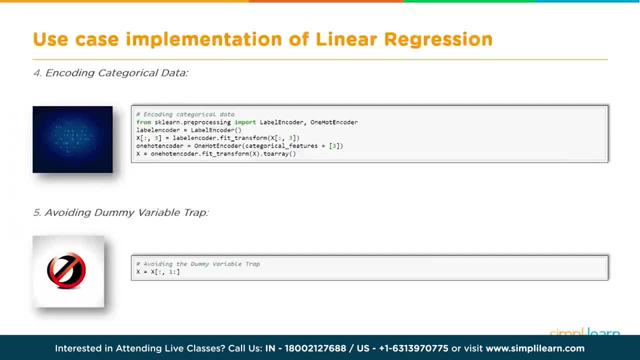 Next, on setting up our data, we have avoiding dummy variable trap. This is very important. Why? Because the computer has automatically transformed our header into the setup And it's automatically transformed all of our data, So we have all these different variables. So when we did the encoder, 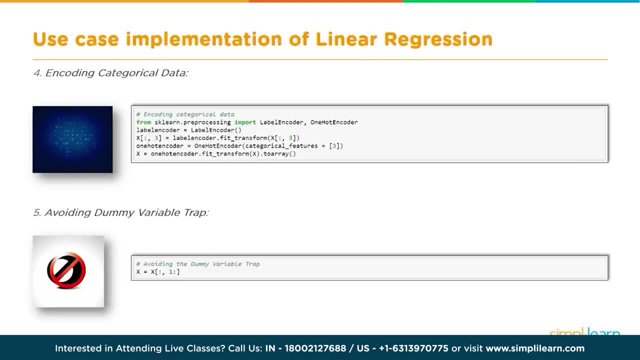 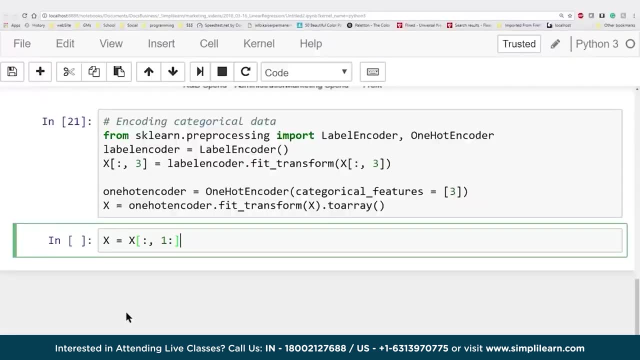 The encoder created two columns, And what we need to do is just have the one, Because it has both the variable and the name. That's what this piece of code does here. Let's go ahead and paste this in here And we have X equals X, colon, comma one colon. 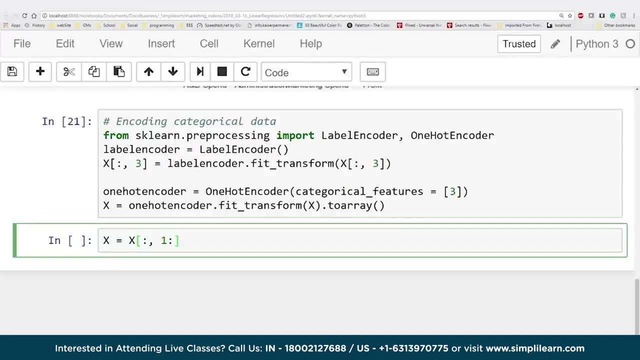 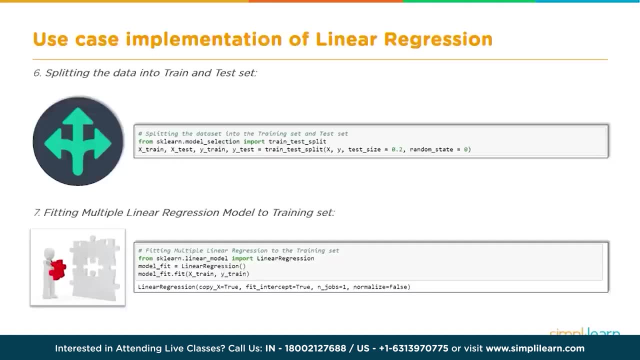 All this is doing is removing that one extra column we put in there when we did our one hot encoder and our label encoding. Let's go ahead and run that And we're going to create our linear regression model And let's see what that looks like here. 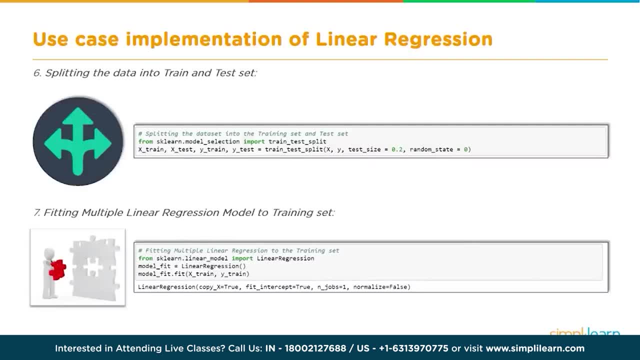 And we're going to do that in two steps. The first step is going to be in splitting the data. Now, whenever we create a predictive model of data, We always want to split it up. so we have a training set and we have a testing set. 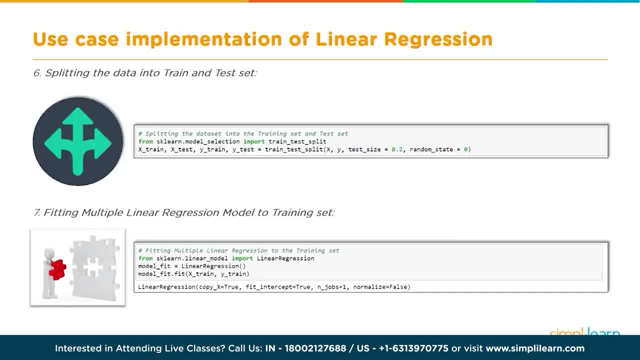 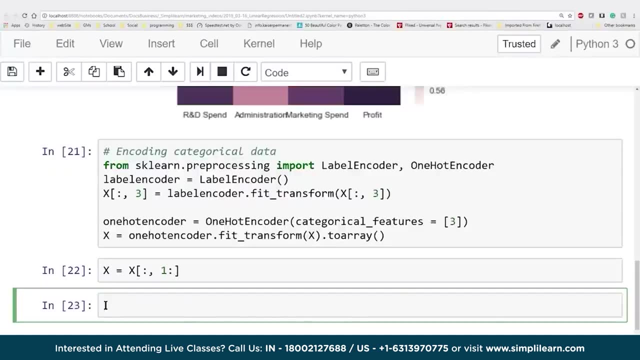 That's very important, Otherwise we'd be very unethical without testing it to see how good our fit is, And then we'll go ahead and create our multiple linear regression model and train it and set it up. Let's go ahead and paste this next piece of code in here: 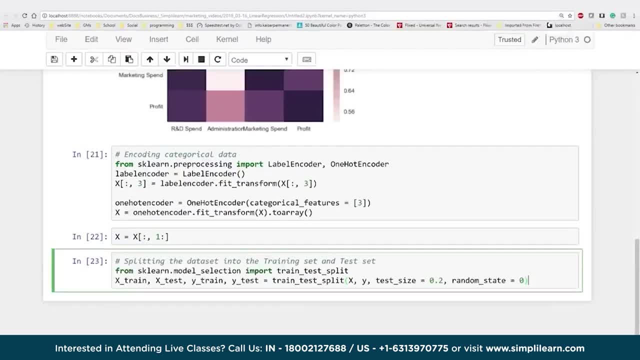 And I'll go ahead and shrink it down a size or two so it all fits on one line. So from the sklearn module selection we're going to import train test split And you'll see that we've created four completely different variables. We have capital X train. capital X test. smaller case y train. smaller case y test. 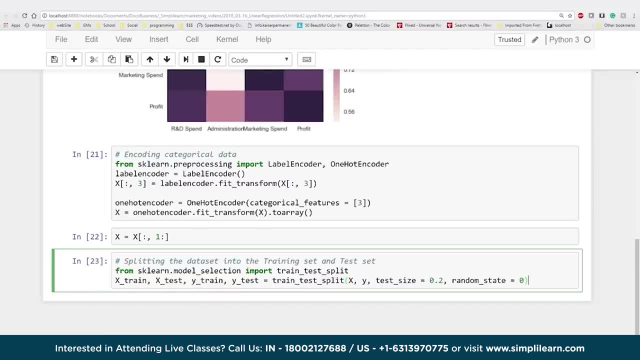 That is the standard way that they usually reference these. when we're doing different models, You'll usually see that A capital X. You see the train and the test and the lower case y. What this is is X. is our data going in? 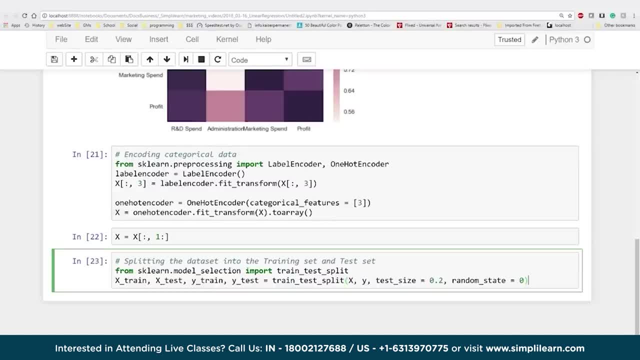 That's our R&D spin, our administration, our marketing, And then Y, which we're training, is the answer. That's the profit, Because we want to know the profit of an unknown entity. That's what we're going to shoot for in this tutorial. 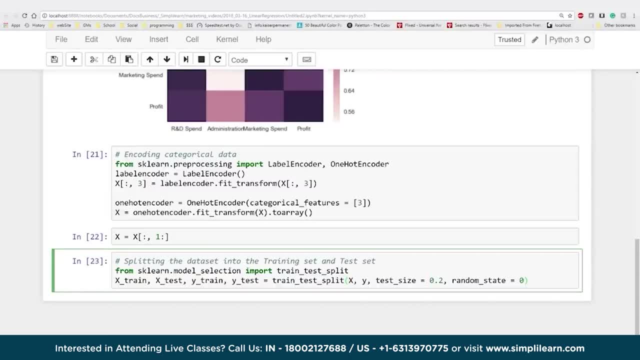 The next part, train test split. We take X and we take Y. We've already created those. X has the columns with the data in it And Y has a column with profit in it, And then we're going to set the test size. 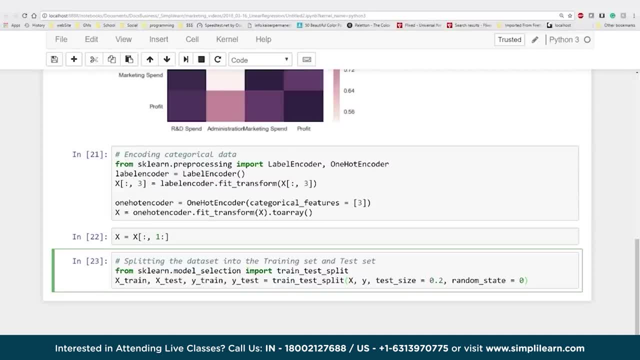 We're going to set it to 0.2.. That basically means 20%. So 20% of the rows are going to be tested. We're going to put them off to the side. So since we're using 1,000 lines of data, that means that 200 of those lines we're going to hold off to the side to test for later. 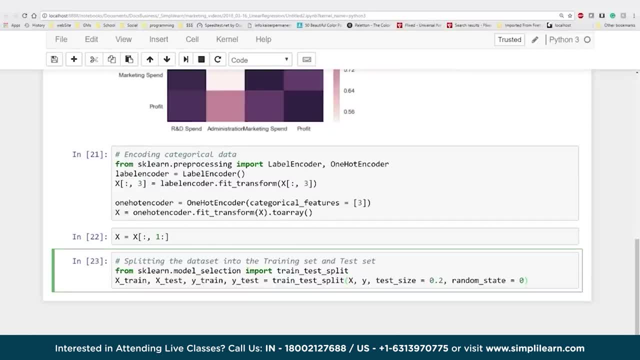 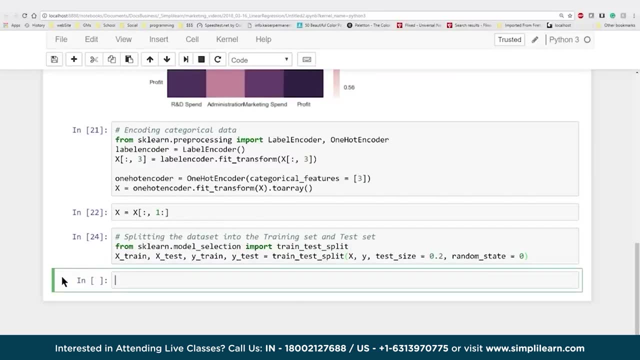 And then the random state equals 0.. We're going to randomize which ones it picks to hold off to the side. We'll go ahead and run this. It's not overly exciting because it's setting up our variables, But the next step is the next step. we actually create our linear regression model. 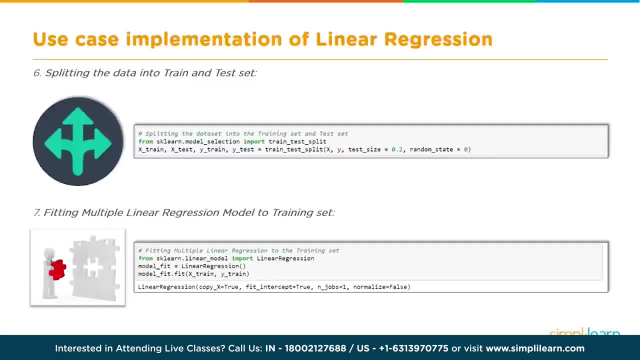 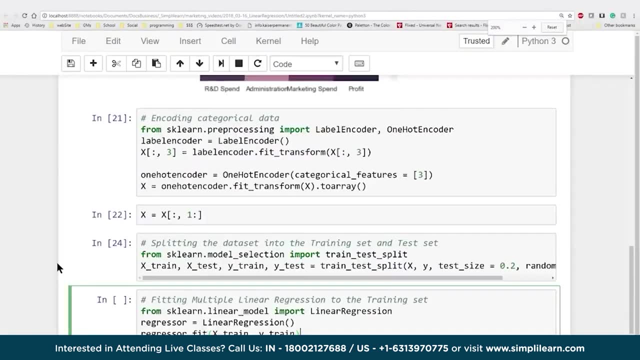 Now that we got to the linear regression model, we get that next piece of the puzzle. Let's go ahead and put that code in there and walk through it. So here we go, We're going to paste it in there And let's go ahead. and since this is a shorter line of code, let's zoom up there so we can get a good look. 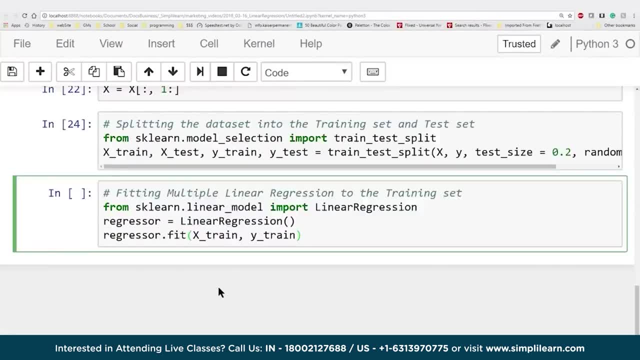 And we have from the sklearn the linear underscore model. We're going to import linear regression Now. I don't know if you recall from earlier when we were doing all the math. Let's go ahead and flip back there and take a look at that. 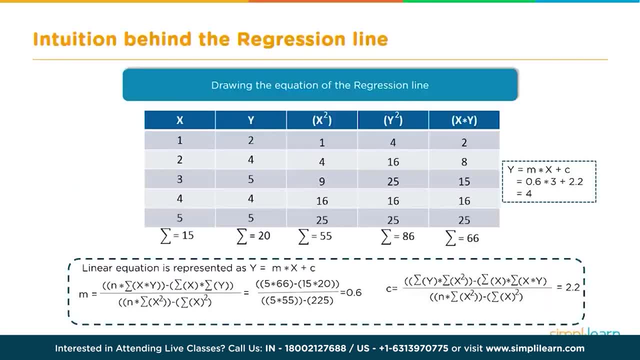 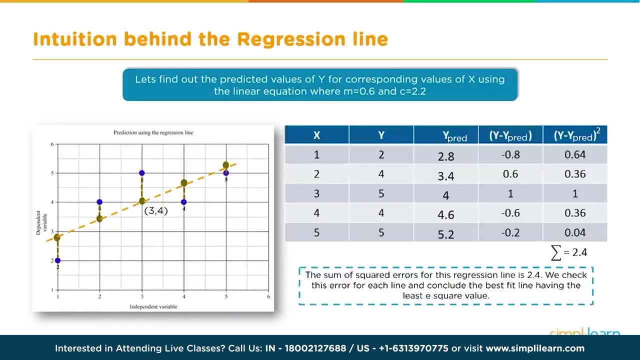 Do you remember this, where we had this long formula on the bottom and we were doing all this sumization, And then we also looked at setting it up with the different lines, And then we also looked all the way down to multiple linear regression Where we're adding all those formulas together. 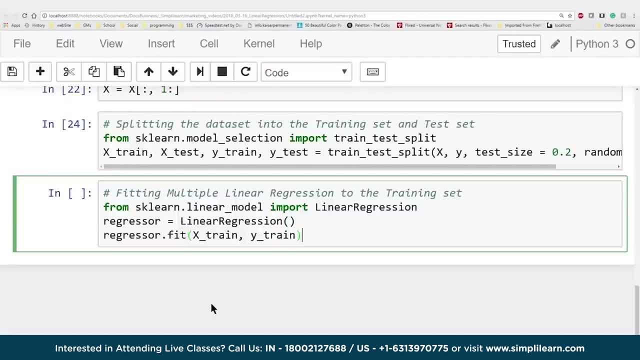 All of that is wrapped up in this one section. So what's going on here is I'm going to create a variable called regressor, And the regressor equals the linear regression. That's the linear regression model that has all that math built in. 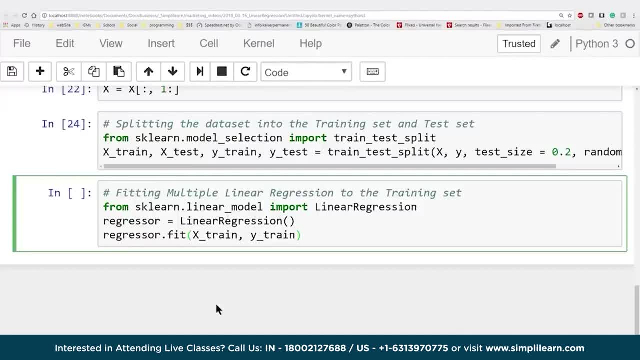 So we don't have to have it all memorized or have to compute it individually. And then we do the regressorfit. In this case, we do x And y Because we're using the training data, X being the data in and y being profit. 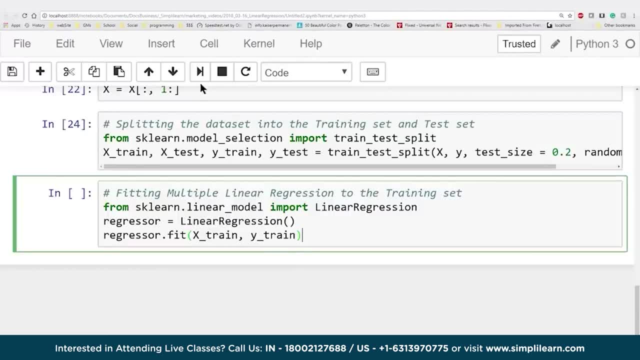 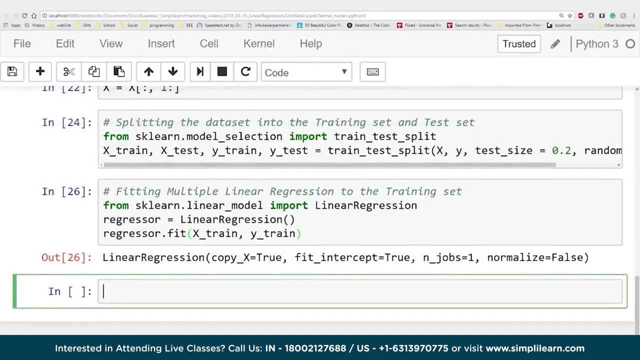 What we're looking at And this does all that math for us. So within one click and one line we've created the whole linear regression model And we fit the data to the linear regression model And you can see that when I run the regressor it gives an output. 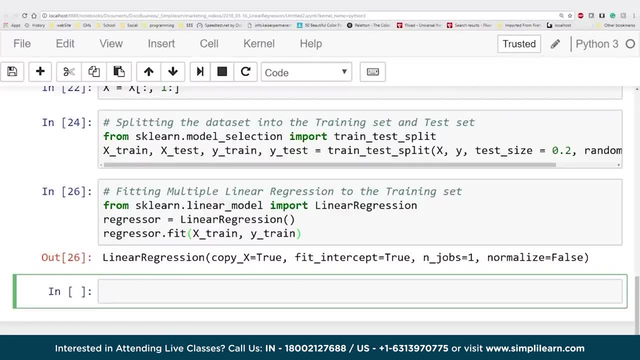 Linear regression. It says: copy x equals true, Fit intercept equals true, In jobs equals one, Normalize equals false. It's just giving you some general information on what's going on with that regressor, Now that we've created our linear regression model. 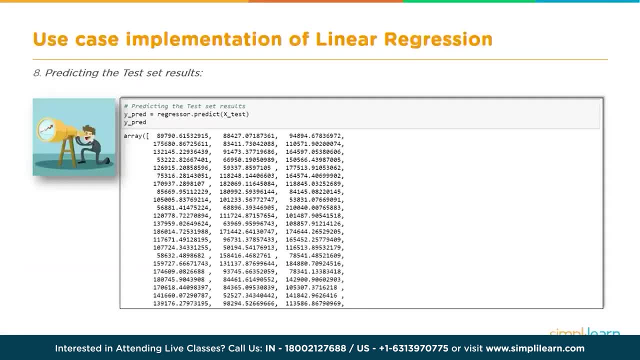 Let's go ahead and use it And, if you remember, we kept a bunch of data aside. So we're going to do a y predict variable And we're going to put in the x test And let's see what that looks like. 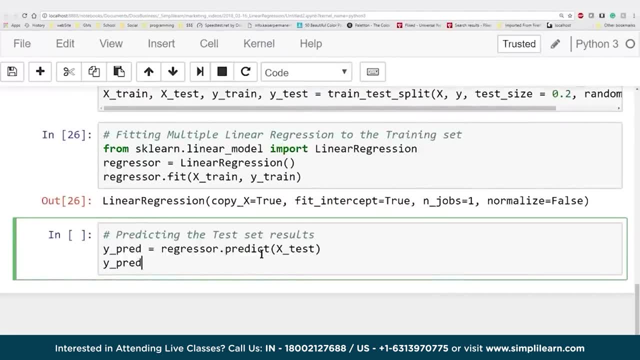 Scroll up a little bit. Paste that in here Predicting the test set results. So here we have y predict equals regressor dot predict X test going in And this gives us y predict Now because I'm in Jupyter inline. 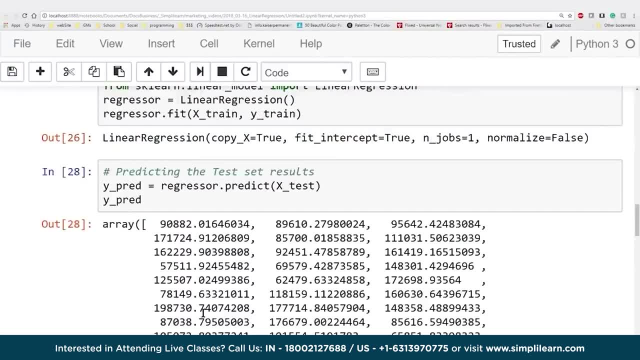 I can just put the variable up there And when I hit the run button It will print that array out. I could have just as easily done print y, predict. So if you're in a different IDE, that's not an inline setup Like the Jupyter notebook. 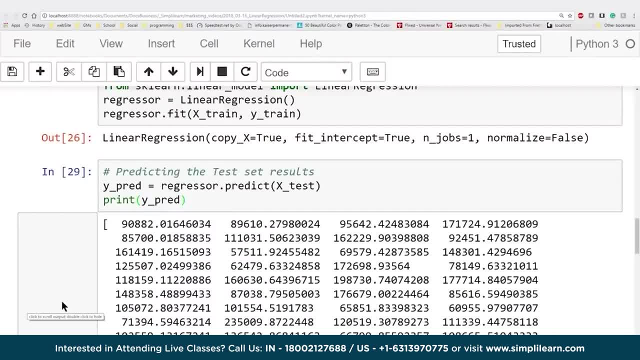 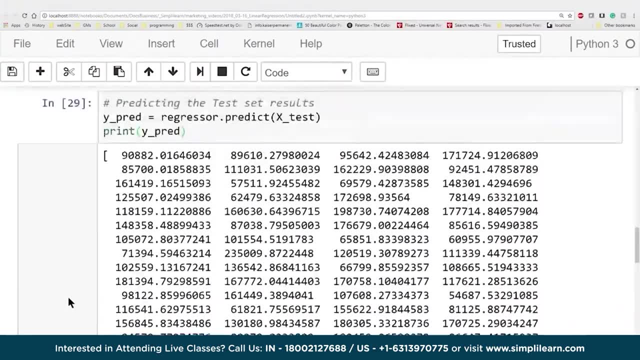 You can do it this way: Print y predict And you'll see that for the 200 different test variables we kept off to the side, It's going to produce 200 answers. This is what it says the profit are for those 200 predictions. 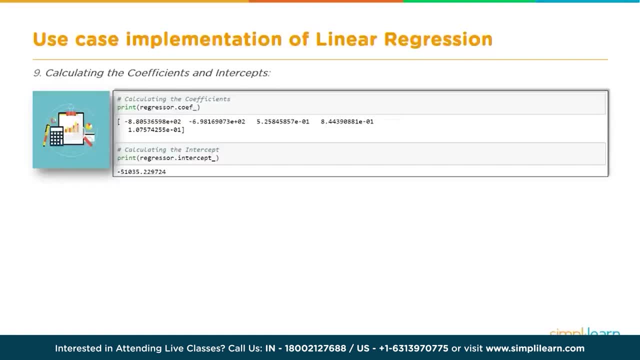 But let's don't stop there. Let's keep going And take a couple look. We're going to take just a short, deep look At the detail here And calculating the coefficients and the intercepts. This gives us a quick flash at what's going on behind the line. 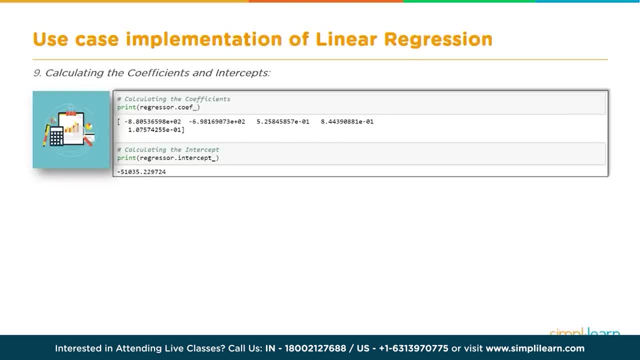 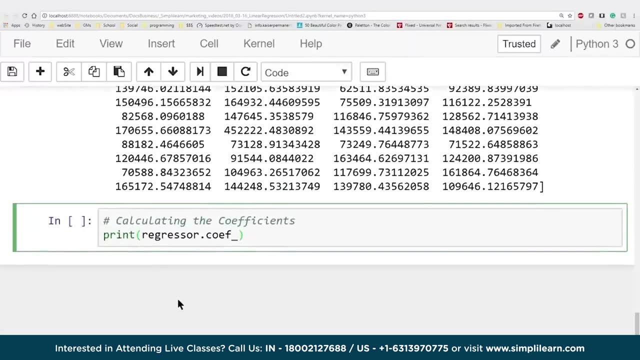 We're going to take a short detour here And we're going to be calculating the coefficient and intercepts So you can see what those look like. What's really nice about our regressor we created Is it already has a coefficients for us. 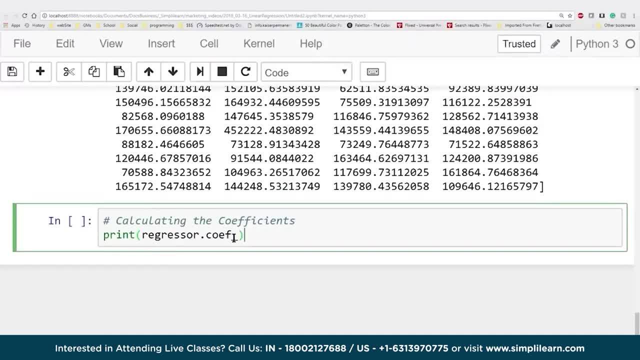 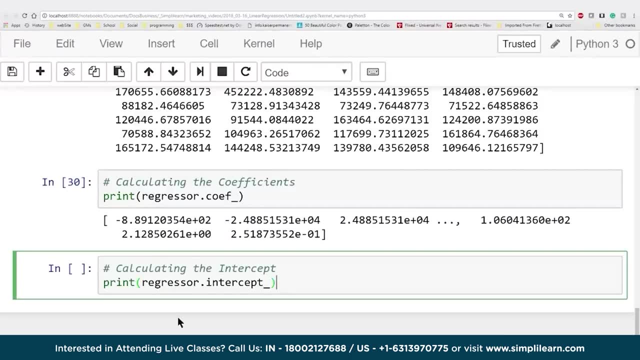 We can simply just print regressor dot coefficient underscore. When I run this You'll see our coefficients here. And if we can do the regressor coefficient, We can also do the regressor Intercept. And let's run that And take a look at that. 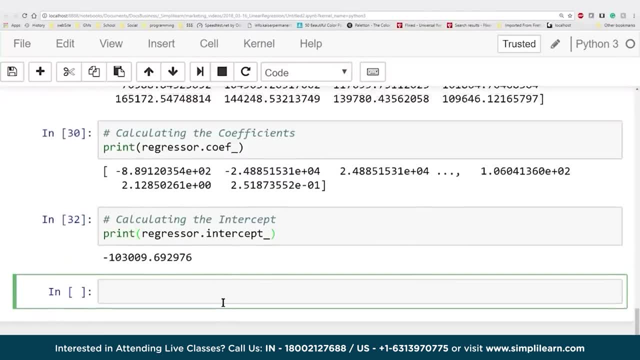 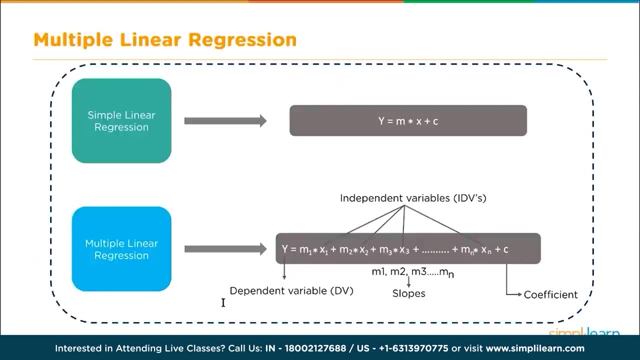 This all came from the multiple regression model And we'll flip over so you can remember where this is going into And where it's coming from. You can see the formula down here, Where y equals m1 times x1.. Plus m2 times x2.. 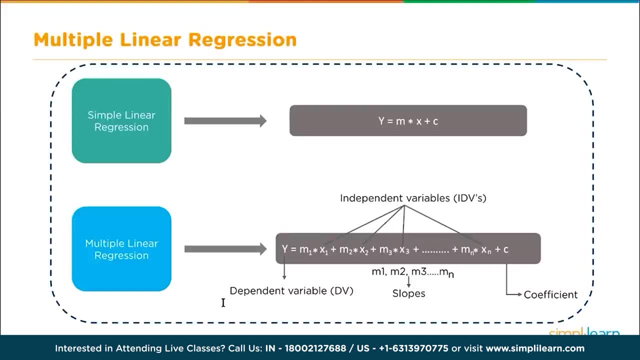 And so on and so on, Plus c the coefficient, So these variables fit right into this formula. Y equals slope 1 times column 1 variable, Plus slope 2 times column 2 variable, All the way to the m, into the n. 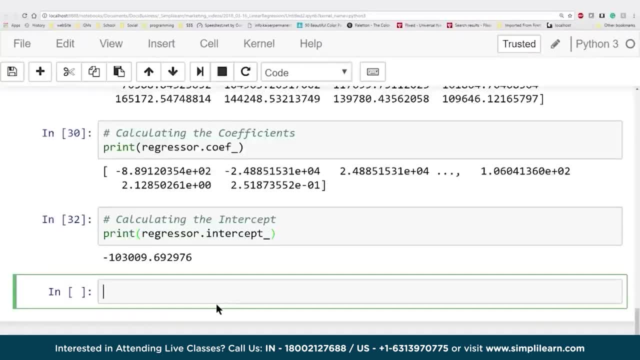 And x to the n plus c the coefficient, Or in this case You have minus 8.89 to the power of 2. Etc, Etc Times, the first column And the second column And the third column, And then our intercept is the minus 103009 point. 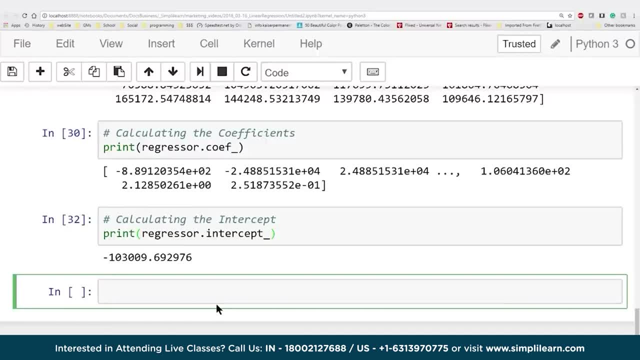 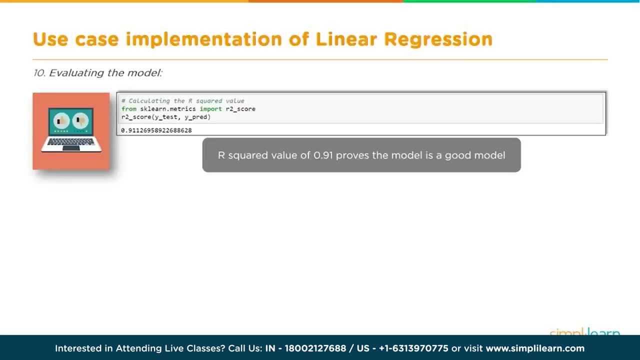 Boy, it gets kind of complicated when you look at it. This is why we don't do this by hand anymore. This is why we have the computer To make these calculations easy to understand and calculate. Now, I told you that was a short detour. 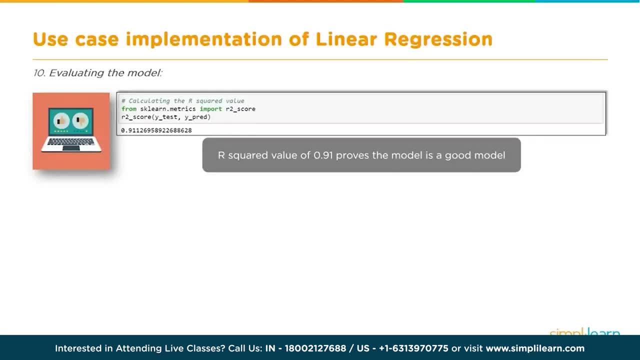 And we're coming towards the end of our script. As you remember, from the beginning I said: if we're going to divide this information, We have to make sure it's a valid model, That this model works, And understand how good it works. 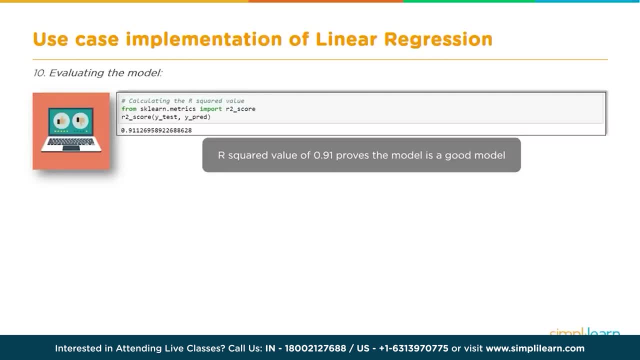 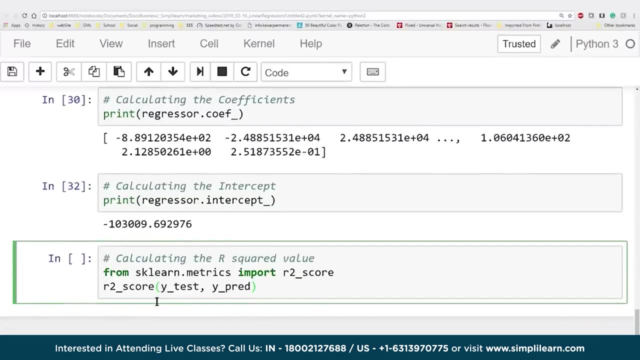 So calculating the r squared value. That's what we're going to use To predict how good our prediction is, And let's take a look at what that looks like in code. And so we're going to use this From sklearnmetrics. 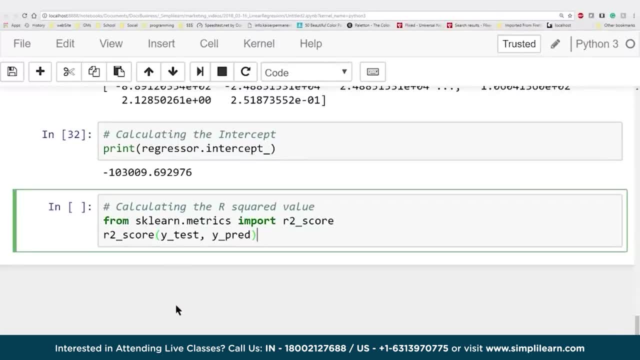 We're going to import r2 score. That's the r squared value And we're looking at the error. So in the r2 score We take our y test Versus our y. predict Y test is the actual values we're testing. 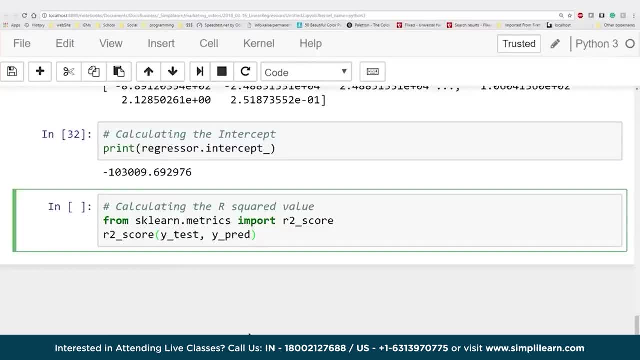 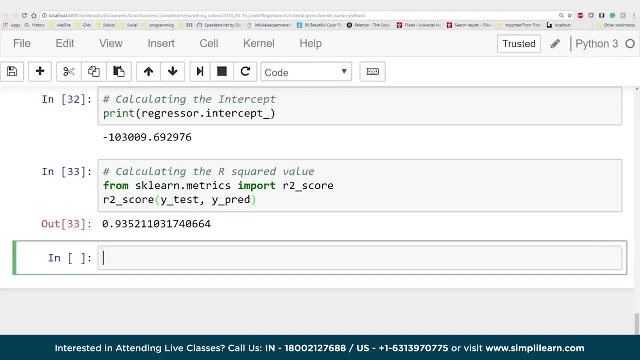 That was the one that was given to us. That we know are true. The y predict of those 200 values Is what we think it was true And when we go ahead and run this We see we get a .9352.. 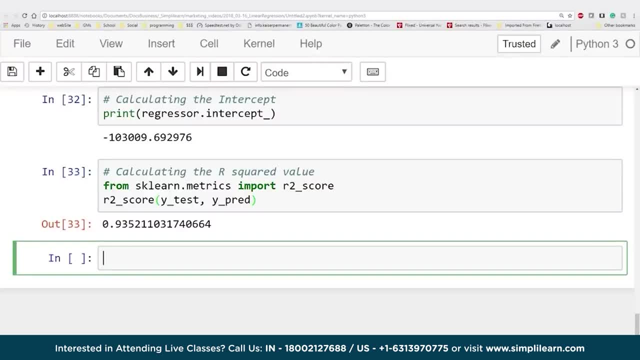 That's the r2 score. Now, it's not exactly a straight percentage, So it's not saying it's 93% correct, But you do want that in the upper 90s. Oh and higher Shows that this is a very valid prediction. 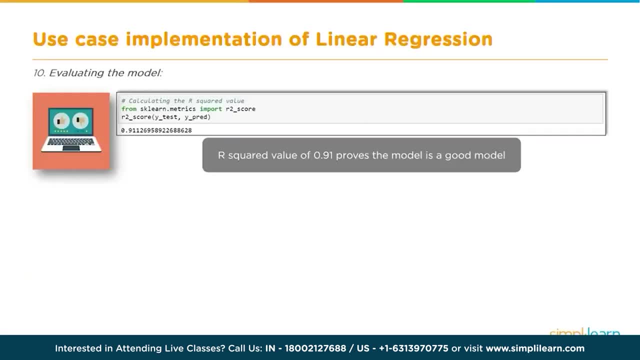 Based on the r2 score And if r squared value of .91.. Or 92 as we got on our model, Because, remember, it does have a random generation involved. This proves the model is a good model, Which means success. Yay. 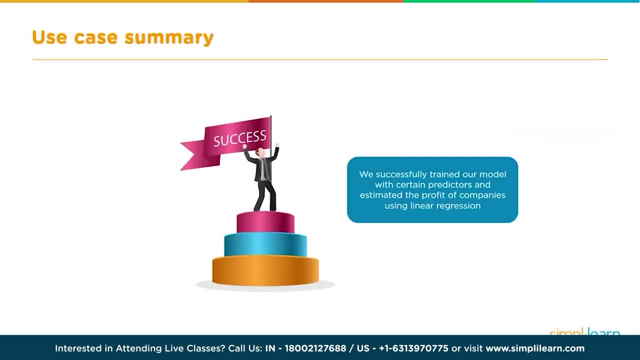 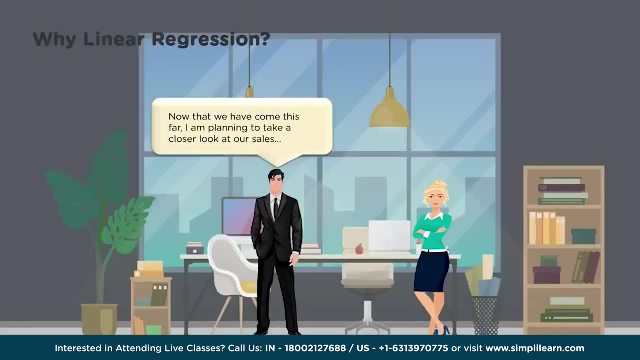 We successfully trained our model With certain predictors and estimated the profit Of the companies using linear regression, The y linear regression. Now that we have come this far, I'm planning to take a closer look at our cells So that we can estimate cells in the future. 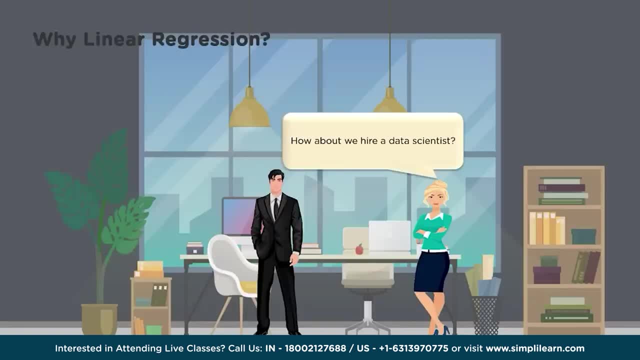 How about we hire a data scientist? You can see our two corporate individuals. Looks more like they should be agents Or secret agents some place Discussing how to better forward their company, And so they're going to come in And ask the data scientist to come in. 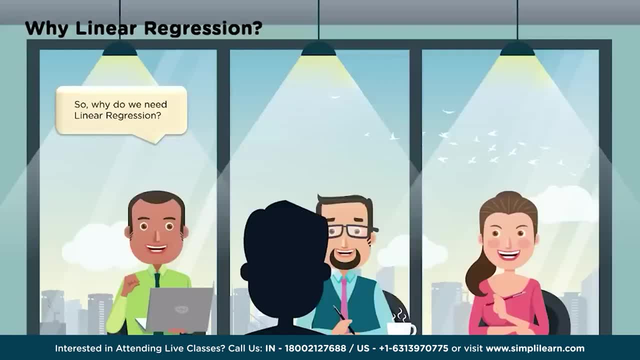 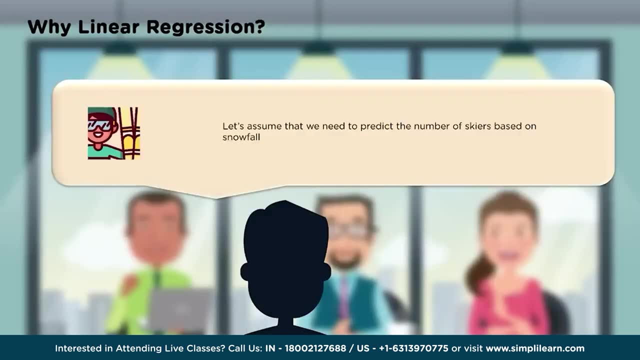 Good idea. This will help us to keep a constant track of our cells. So why do we need linear regression? Let's assume that we need to predict the number of skiers Based on snowfall. So this happens to be. We've kind of jumped one business to the next. 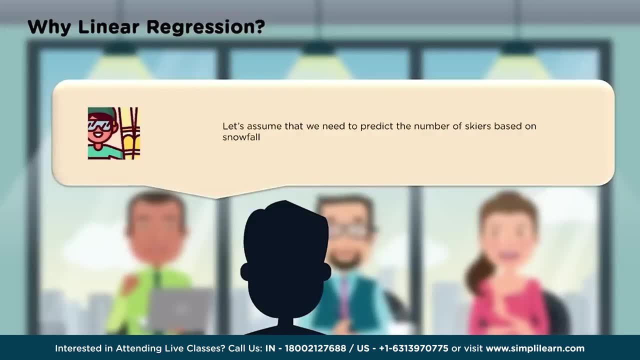 So we're looking at the skiing business, Very popular in a lot of areas. A lot of times You figure you don't have snow, You don't have skiers, But can we actually use something more specific Instead of look it's snowing? 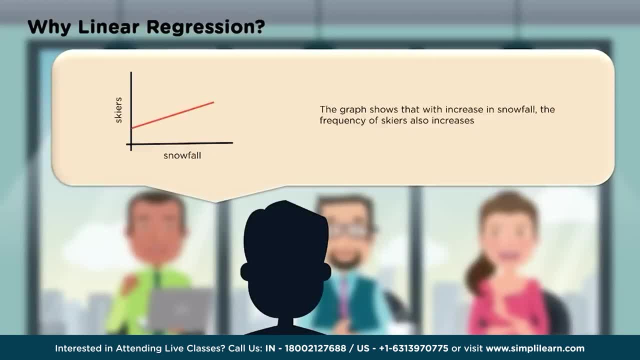 And instead of saying hey look, it's snowing, We can actually start drawing graphs. And the graph shows that with an increase in snowfall, The frequency of skiers also increases. So and there's a pretty direct correlation If you've ever been up to ski areas. 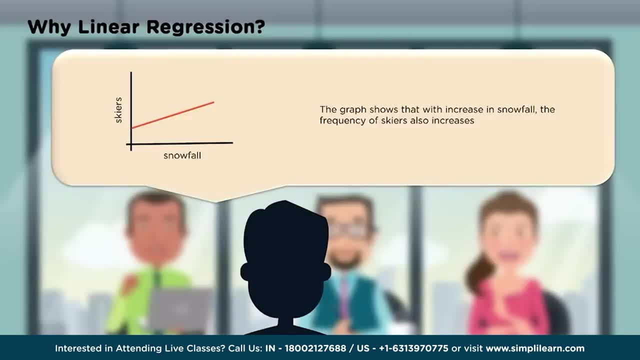 When there's a lot of snowfalls, The skiers all show up Because they know it's going to be better skiing right afterward. So it's kind of easy to see why And you can easily predict How many skiers. And that way you can also predict. 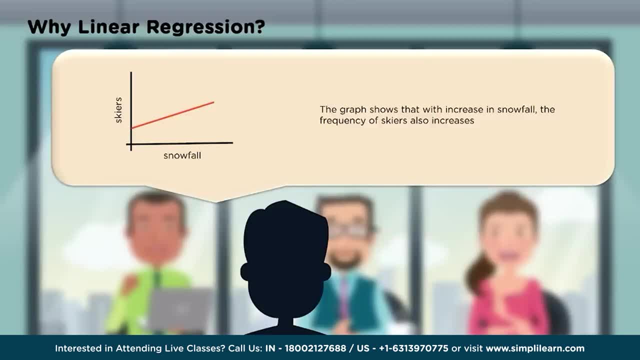 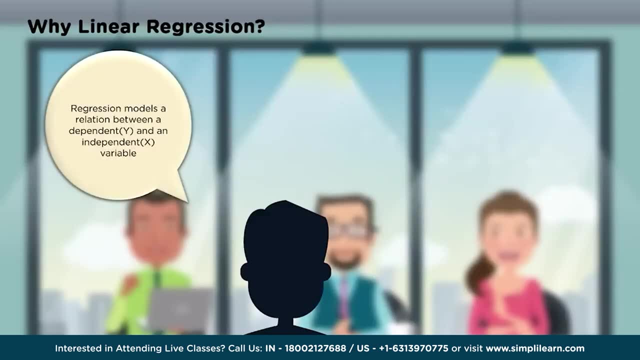 How many people you need to service them, How many lifts to have up and running And all the stuff that goes with running a ski area. Thus we see that the number of skiers Are directly proportional to the amount of snowfall. Regression models. 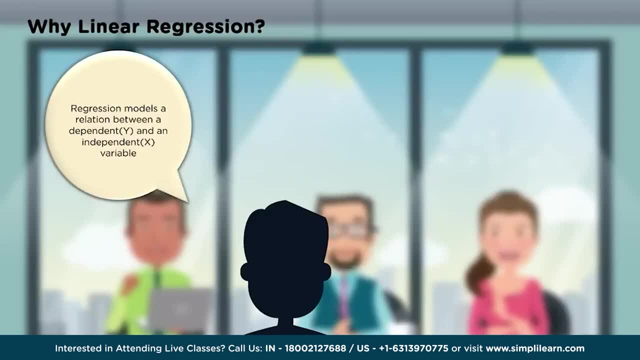 A relation between a dependent y And an independent x variable. This is real important to understand regression, Because when we talk about linear regression, It's the basis of almost all our machine learning Algorithms out there. It's the underlying part of the math. 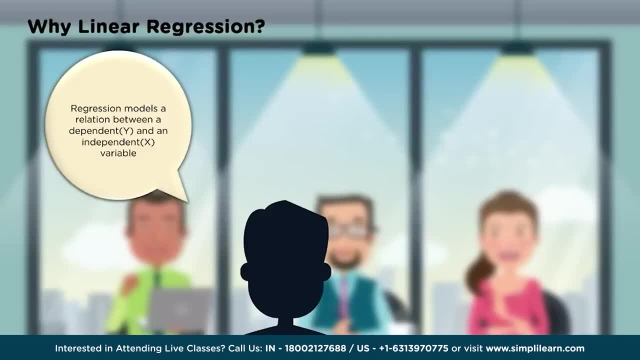 In our deep learning. So it all starts here with linear regression And when we talk about a dependent y And an independent x variable, These are numbers. We're usually talking about floats, So we want to have an actual number value coming out. 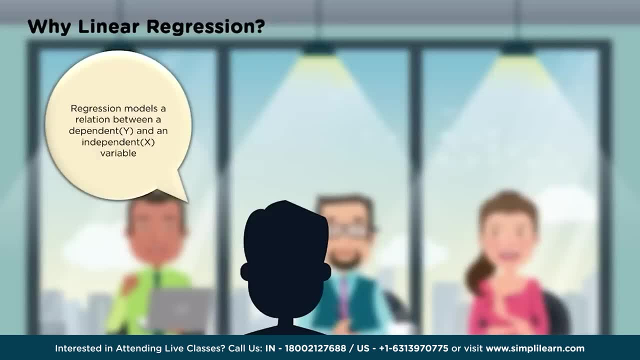 And that's different than something that's categorical, Where we want to know yes or no, True or false. So regression means we're looking for a number. The independent variable is known as predictor variable And dependent variable is known as the response variable. 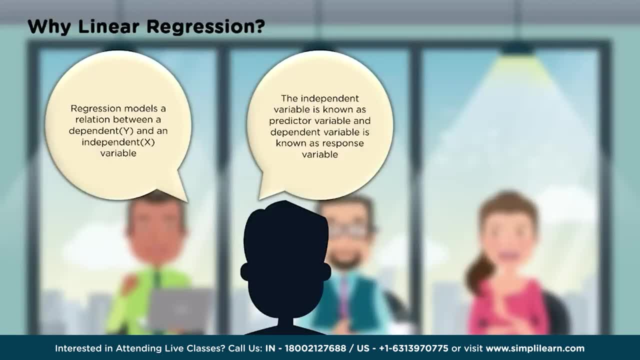 So we have one predictor variable- The amount of snowfall- And one response variable- How many skiers are going to show up- And then we can take this relationship And it can be expressed as: y equals beta. We're going to use the Greek letter beta. 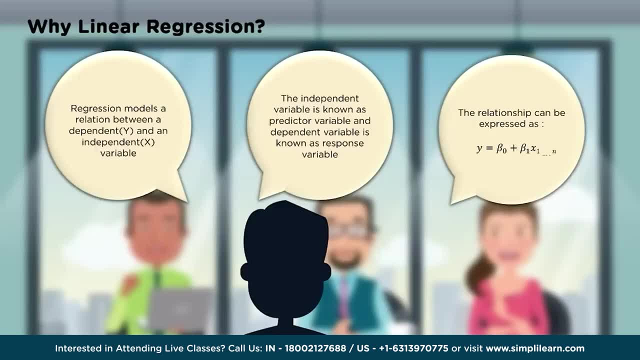 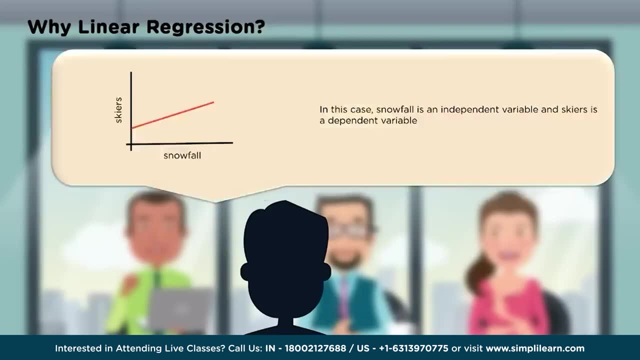 And we have beta naught Plus beta one x one, And if you continue out It would be plus beta two x two, And so on until the nth degree. In this case, snowfall is an independent variable And skiers is a dependent variable. 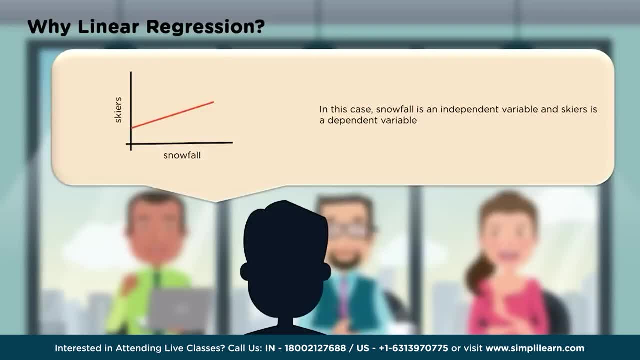 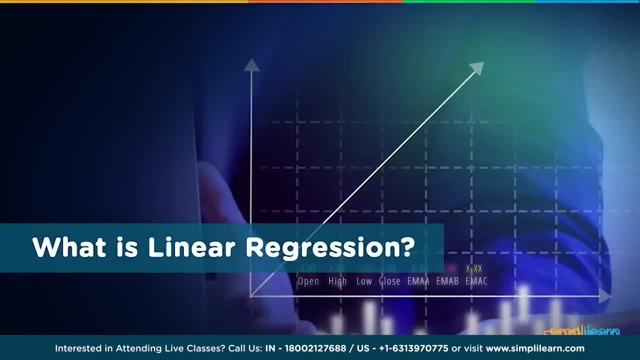 So we kind of had a little quick overview. Let's go ahead and talk a little bit more. What is linear regression? So we're going to go from y Predicting a number of skiers for snowfall, And we looked at the formula a little bit. 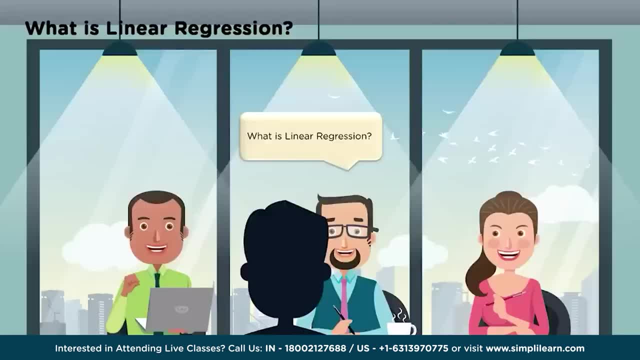 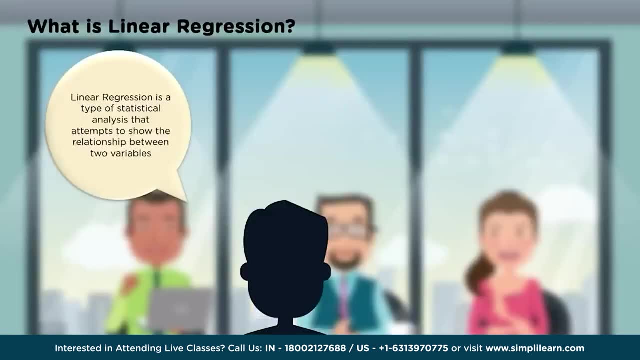 But let's look a little bit closer At what exactly is going on with linear regression- And the question is going to come up in an interview: What is linear regression? Linear regression is a type of statistical analysis That attempts to show the relationship between two variables. 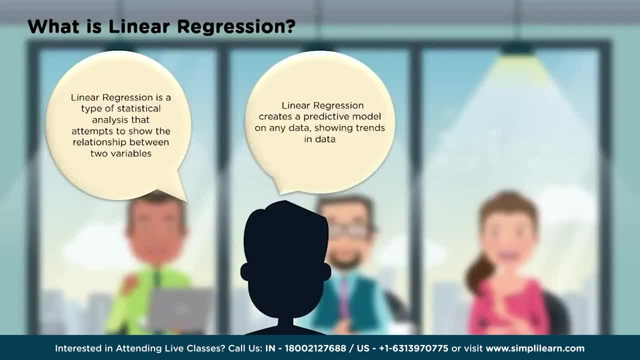 Linear regression creates a predictive model On any data showing trends in data. The model is found by using the least square method. There are other methods. The least square method happens to be the most commonly used out there And we usually start with the least square method. 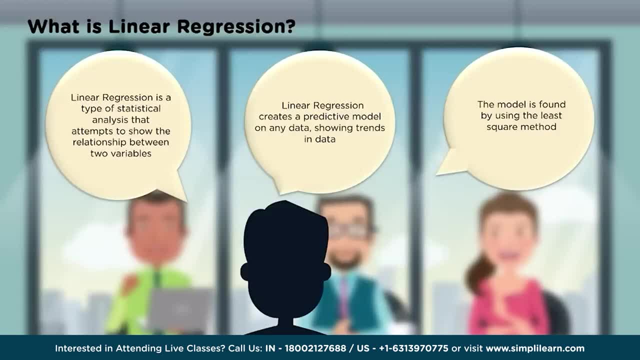 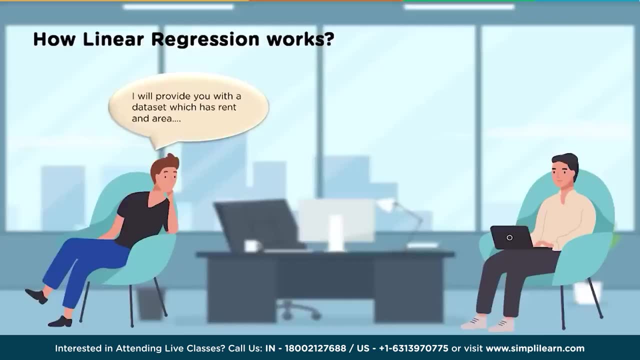 Since it's the most common And usually works the best on most models. And we're already looking at how linear regression works. But let's dig deeper into it And let's take a closer look How linear regression works. I will provide you with a data set. 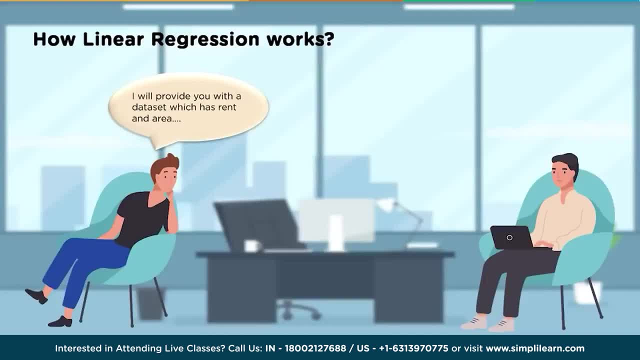 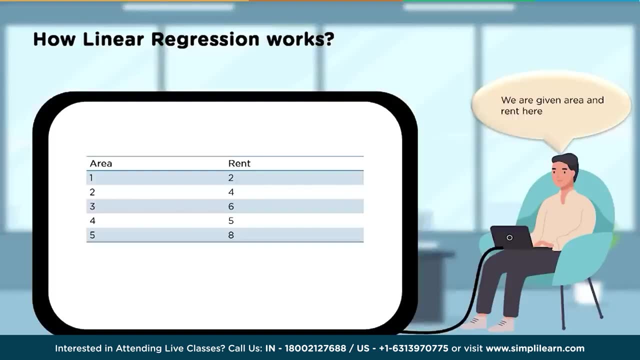 Which has rent area other information in it. It looks like our secret agents have put on their casual wear for this one. You need to predict rent accordingly. We are given area and rent here, So you can do linear regression with more variables. 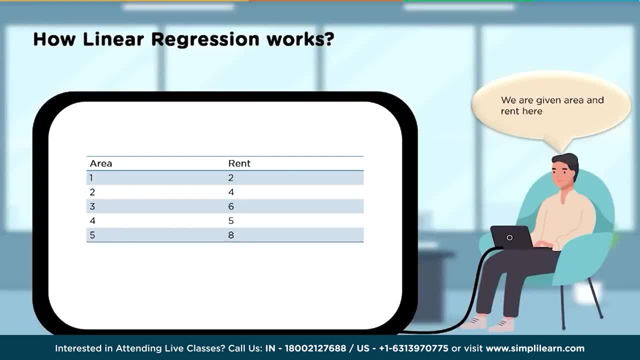 But we're just going to look at the area And then from that Try to figure out what the rent should be. We plot the graph And if you look at it here You can see that the graph is kind of a linear pattern. 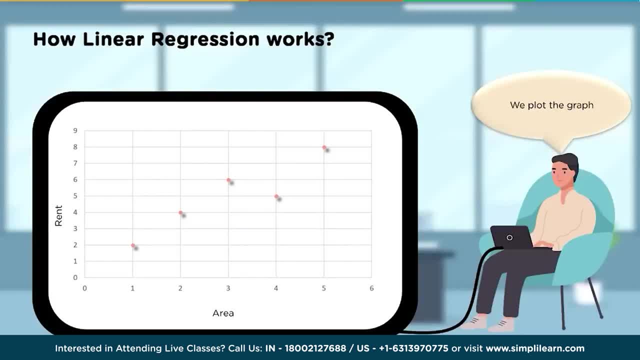 With a little dip in it. So the rent seems to be based on the area. In most of our work As data scientists, We usually try to start with a physical graph, If we can, So we can actually look at it and say: 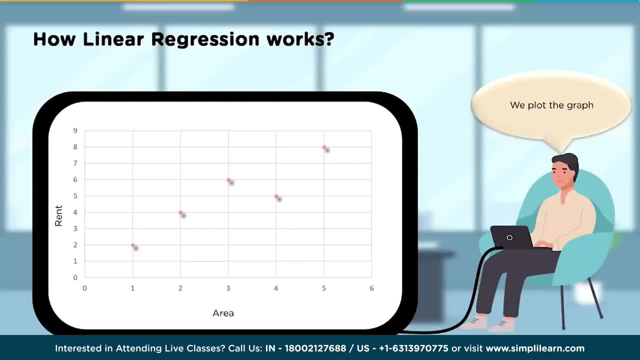 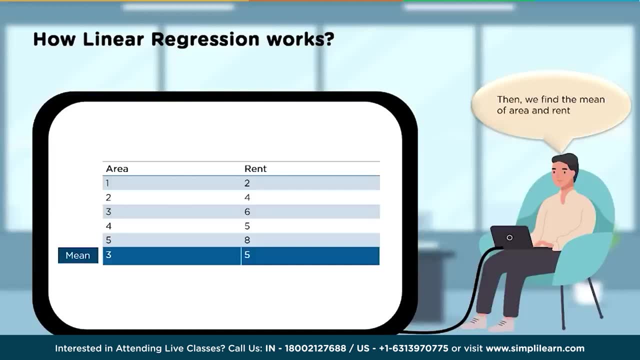 It doesn't look right. You can solve a lot of problems that arise By looking at the graph and saying, No, that doesn't look right at all, Or oh, I should be looking over here for this. Then we find the mean of area and rent. 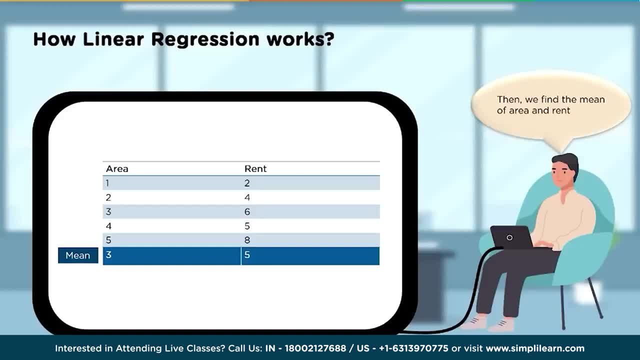 So the mean just means average, And if you take one, two, three, four, five And add them all together And divide by- in this case there's five areas- You get three, And the rent is two, four, six, five and eight. 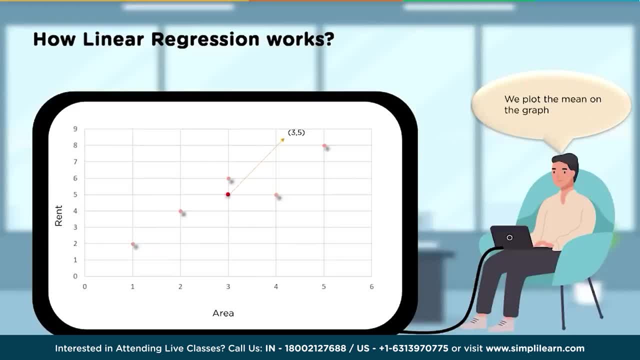 If you add them all together and divide by five, You get five And we plot the mean on the graph On the area. It's kind of a very central point, Which is what we're looking for: The average of everything in there. 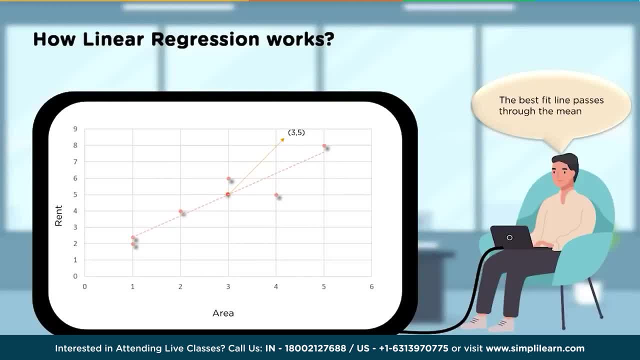 The best fit line passes through the mean. This is real important When you're eyeballing it. As humans, we can do this fairly easy If it's a straight line through a bunch of data. It gets more complicated mathematically When you start adding multiple variables. 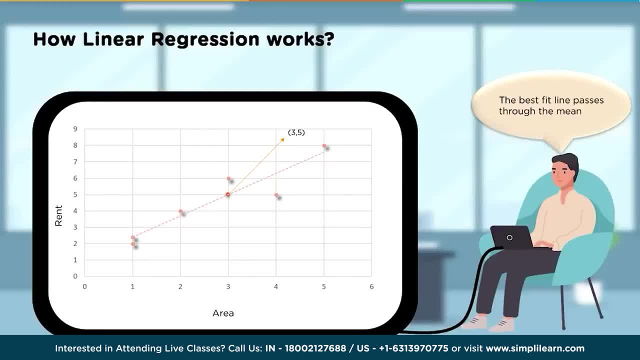 And instead of a line you have a curve. But for basic linear regression We're going to draw a line through the data And the line should go through the means. So depending on how you look at it, You can kind of wiggle the line around back and forth. 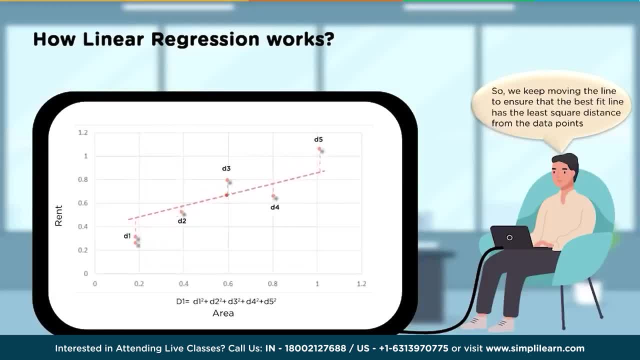 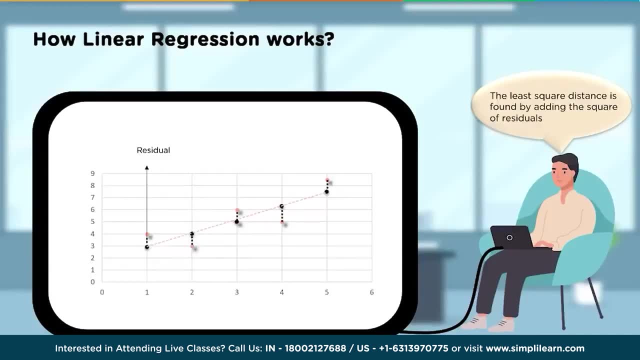 So we keep moving the line To ensure that the best fit line Has the least squared distance from the data points And this is, You can see right here, residual. We have our data point And then we look at the distance between them. 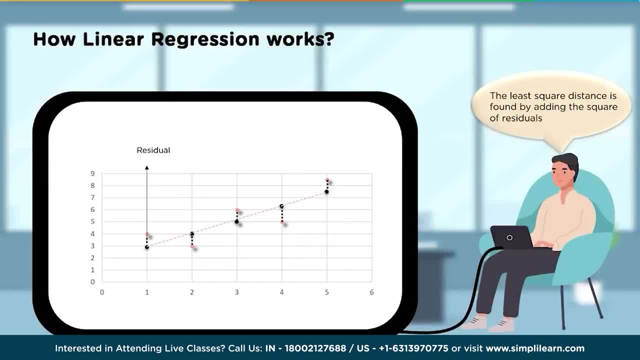 And we square that distance, And that's what they mean by the least squared distance. We want all those distances to add up To the smallest amount we can. When we talk about that distance, We call it the residual And that's the Y predicted. 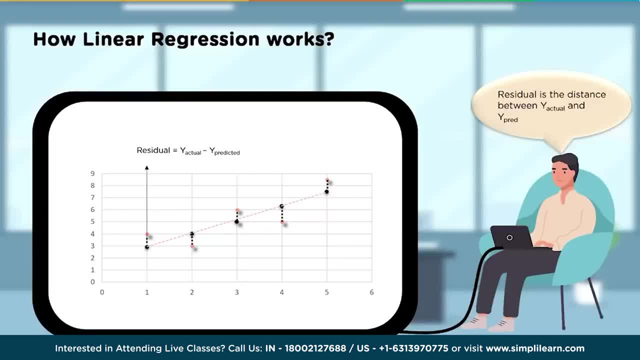 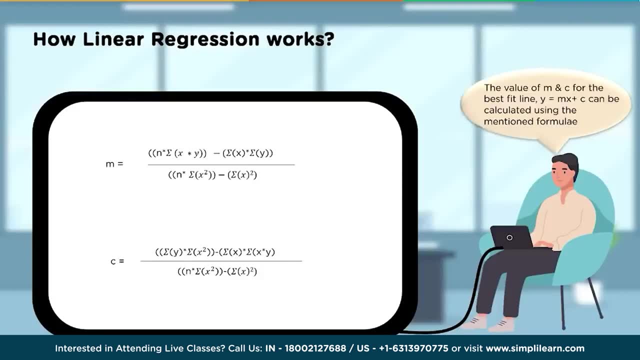 Very straight forward. Just looking at the distance, You can accidentally switch these And it will come out the same Because we're going to square it. But when you're working with other sets of linear regression, You want to make sure you do the Y actual. 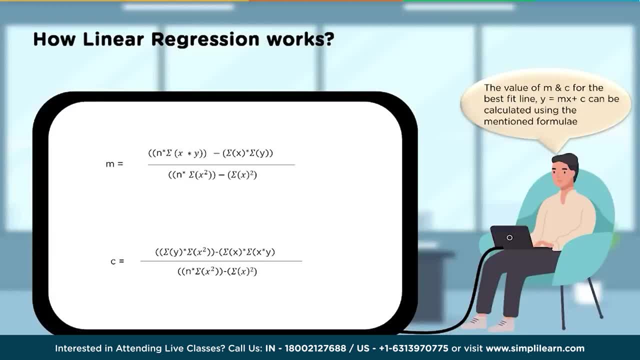 Minus the Y predicted. The value of M and C for the best fit line- Y equals MX plus C- Can be calculated using the mentioned formula And you can see here we have M equals the number of points. That's what N stands for. 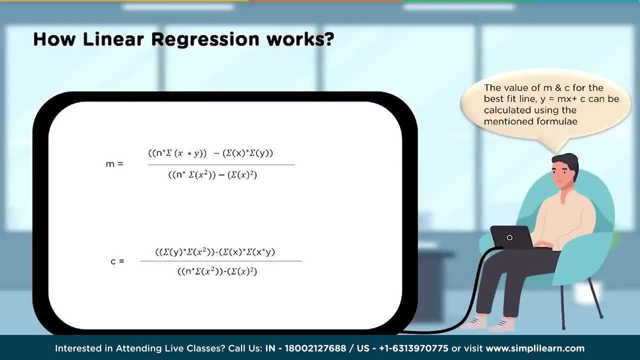 M equals Y Minus the summation of X Times the summation of Y Over the number of the summation of X squared Minus the summation of X squared Of X, all of it squared. That can be confusing trying to say that. 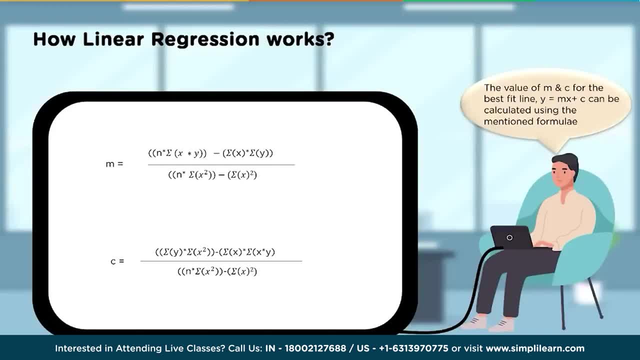 And then, of course, your C value Is going to be the summation of Y Times the summation of X squared Minus the summation of X times the sumation of X times Y Over the total count Of the summation X squared minus the summation of X squared. 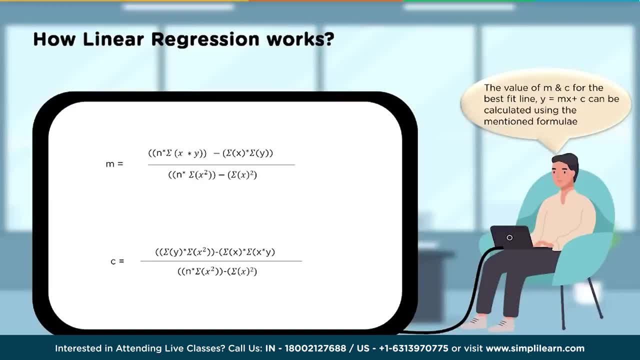 That's a mouthful. Normally we don't worry too much much about these formulas, other than to know they're there. Now, if you're a mathematician, you might go back in there and work on those And those people who originally started to. 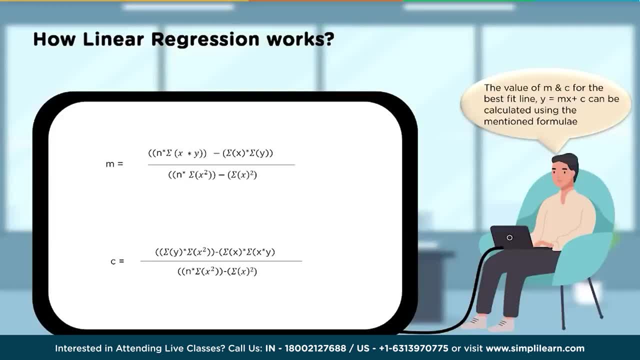 put together the different models in R, of course had to know all this math to build them and had to test it out. That's one of the nice things about R. What is important is that you know about these formulas so that you know where it's coming from. So if you're 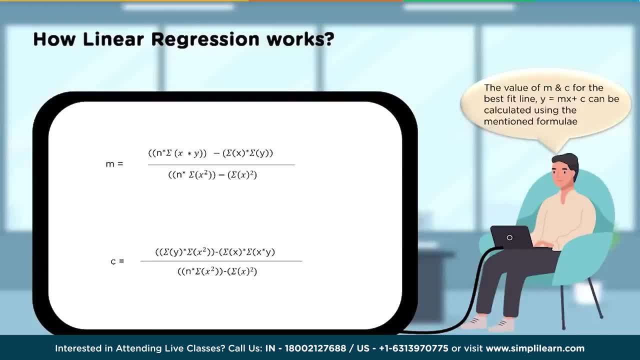 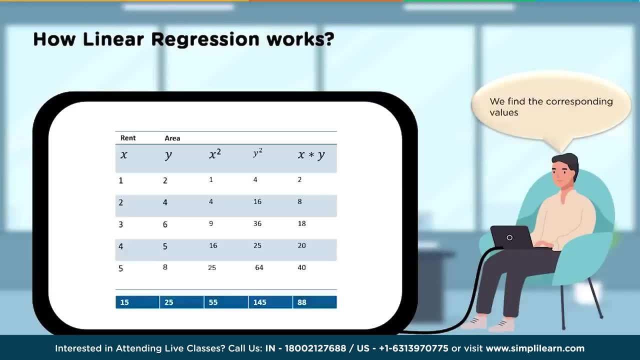 using one linear regression model. this is how this one works. There's other linear regression models based on different math, And so you'd have to be aware when that math changes and how that changes the model, We find the corresponding values. So in this case, if you're going to 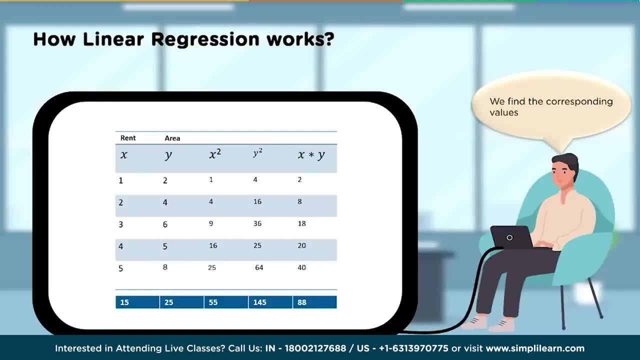 break this up and you're building your own model instead of using the one in R. you would have your rent, you would have your area, you would find your rent squared, your area squared and your rent times area, And if we go back one, we can see that that's all. 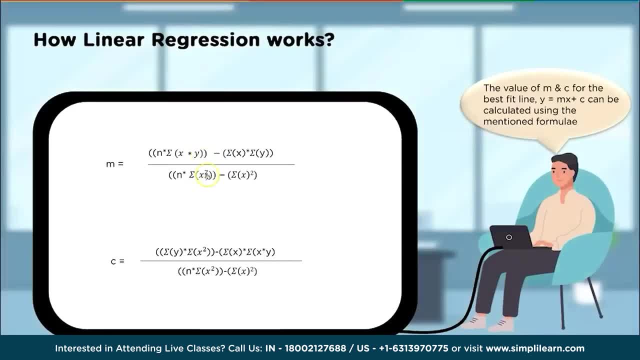 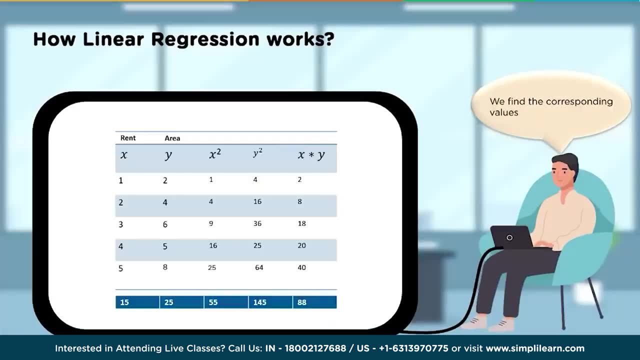 the different little pieces in this model. We have x times y. we have x squared, we have the sum of x which is going to be squared. we have the sum of x, the sum of y. This is the same. These are all the little pieces in here. 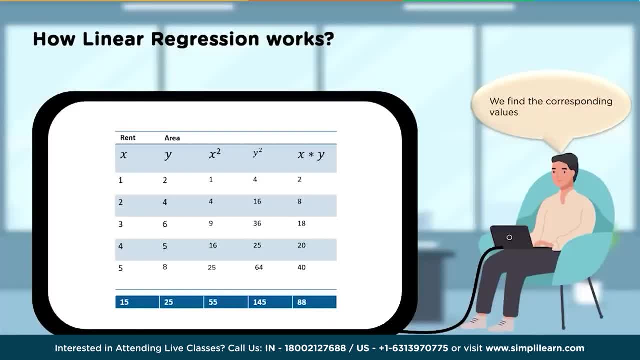 That we see for m equals and c equals, And so once we compute all these, we have 15,, 25,, 55,, 145,, 88.. Very easy to do on a computer. thankfully, You could have millions of these. 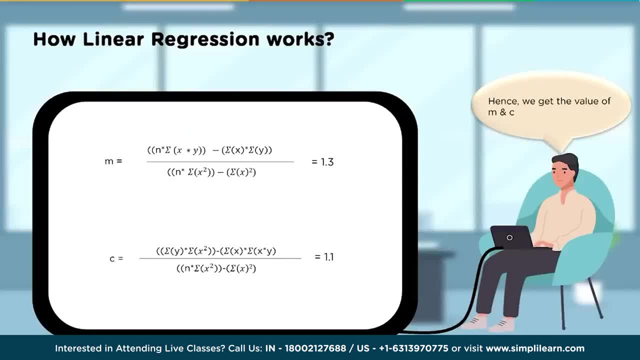 points and it would do it in a very short period. We can then plug in those values very easily into this formula and get a final answer, And we'll see that m equals 1.3 and c equals 1.1.. And then when we take this for the y predicted equals m of i, x of i plus c, we 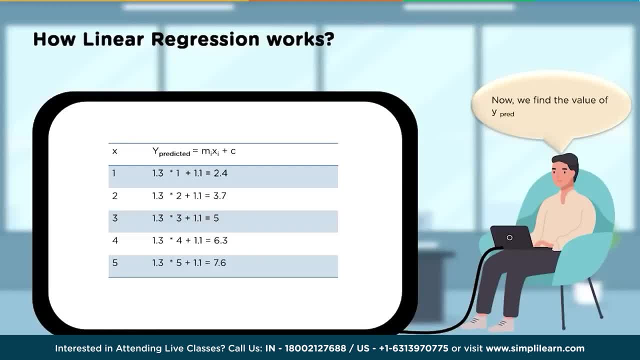 can actually run the data we have. So we're going to see how it predicts. So now we find the value of y predicted, So we have our x in and we want to know what we think y will be based on. our formula- we generated the linear regression formula And so when we 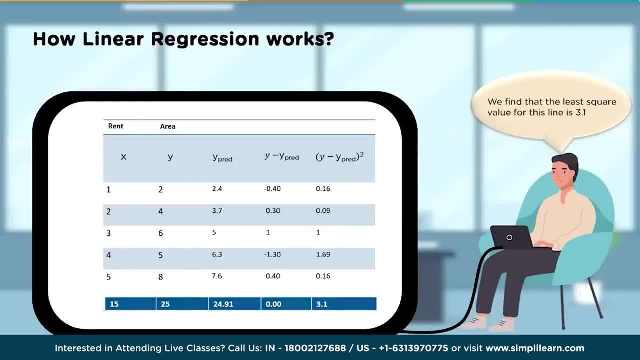 come in here. we have our x, we have our actual y, then we have our y predict- what we think it's going to be. And then we take y minus y predict and we get those values minus 0.4,. 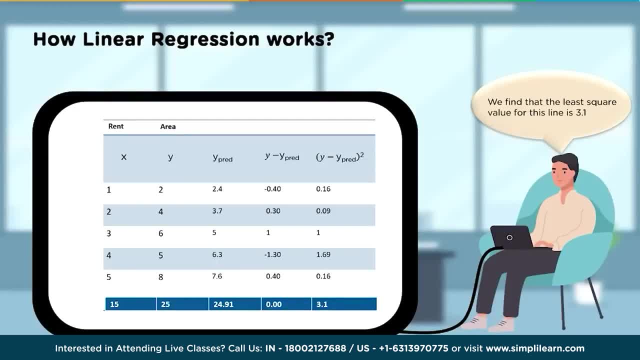 it's off by 0.3.. This one's off by 1, this one's off by minus 1.3, by 0.4. And we go ahead and square that and then we can sum that square and average it out and we'll get a value. This is just. 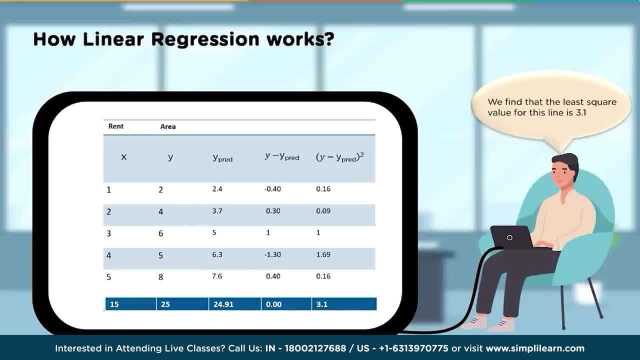 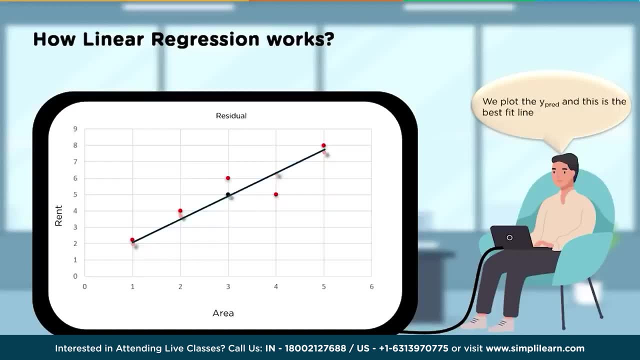 a summation down here of y minus y, predicted square is 3.1. And we call that the least square value for this line is 3.1. And we go ahead and divide that by 5.. So when we plot the y predict and this is the best fit line, and you can see that it. 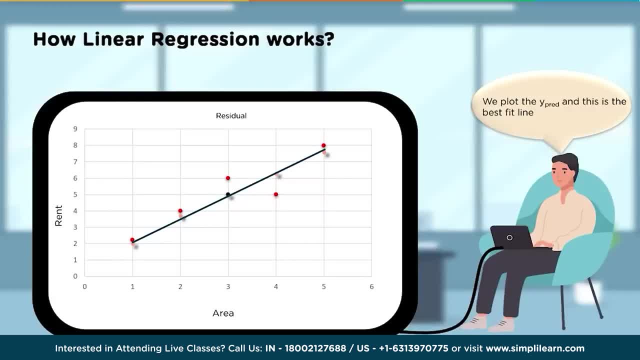 does a pretty good job going right through the middle of lines And in something like rent versus area. if you're trying to figure out how much rent to charge or how many people are allowed to be in the area, that's going to work. But if you're looking for the rent, 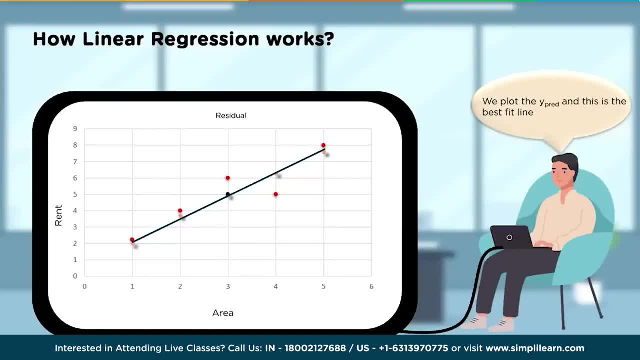 value compared to the area. this gives you a good idea based on the area of what you should rent the place for. It's close enough that in the business world this would work. You're not computing something down to the millimeters or micrometers or nuclear physics. We're just charging people. 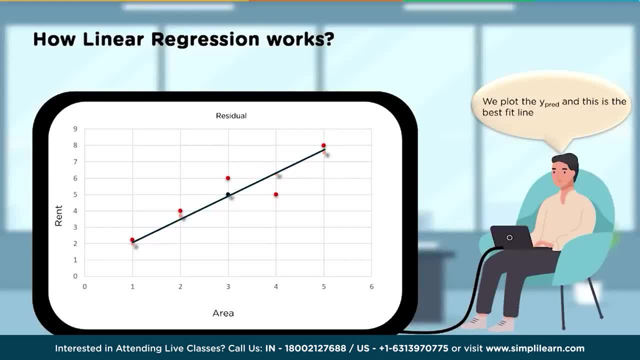 And so if you're off by a couple of dollars, it's not a big deal. You'll be pretty close to what you think it's worth and get the right value for your property, In this case, predicting the revenue using linear regression. Now that you have a good 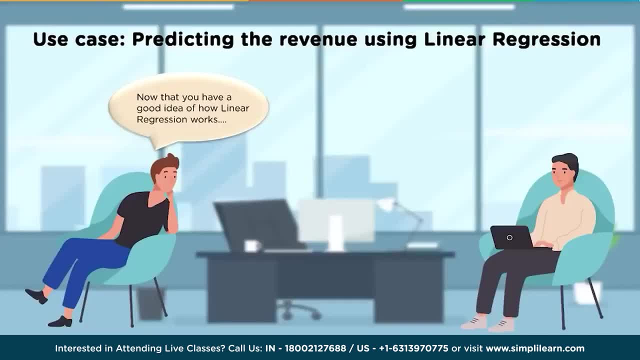 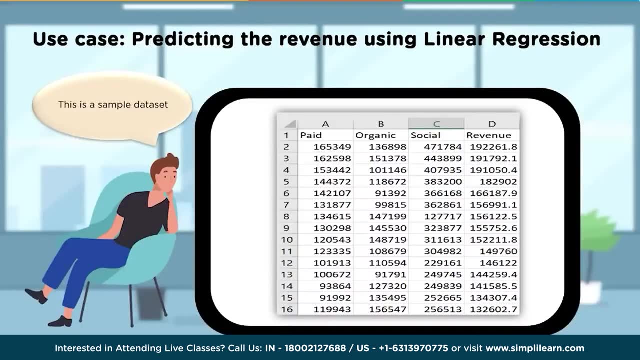 idea of how linear regression works and we're kicking back on our lounging sofa today. let's work on a real life scenario where you have to predict the revenue. So we're going to take a data set and we'll pull this up in just a minute. We'll have 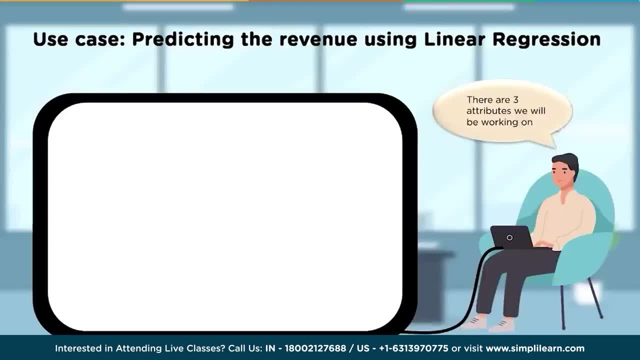 paid, organic, social and revenue. There are three attributes we'll be working on. The first one is our paid traffic. So all the traffic through the advertisement that comes in, The non-paid traffic from search engines. So these are people coming to the. 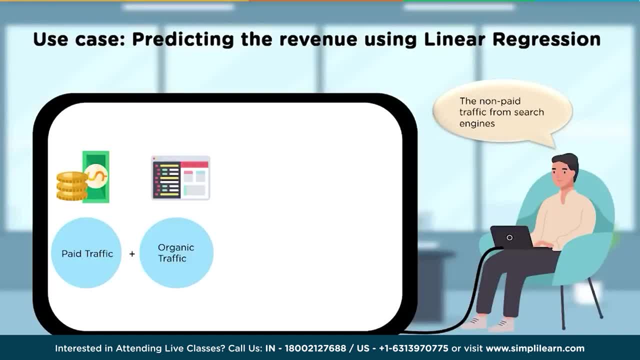 website. They're doing so because they did a search for something specific, So it's pulling it from your website- All the traffic coming from social networking sites. So we want to know what's coming from Twitter and Facebook and somehow they've linked into your website and coming into your. 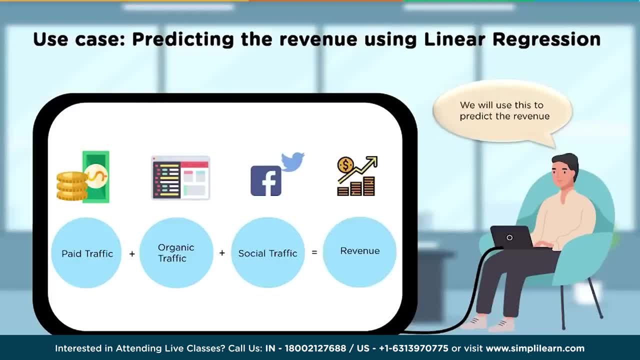 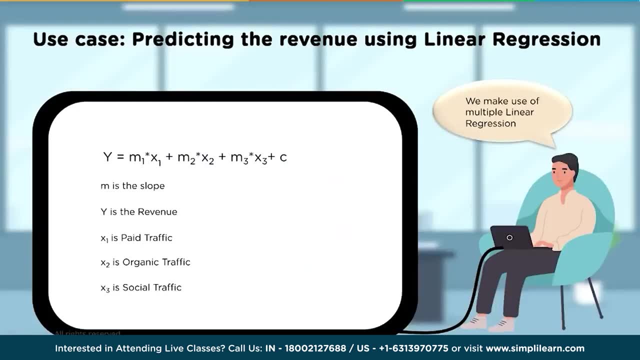 marketing area to buy something, And we'll use this to predict the revenue. So we want to know how all this traffic comes together and how it's going to affect our sales. if the traffic's coming in, We're going to make use of the multiple linear regression model. So you'll see that this 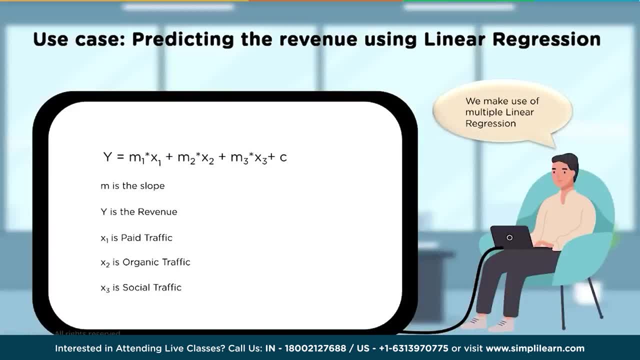 is very similar to what we had before. We had Y equals M times X plus C, But instead we have Y equals M1X1 plus M2X2 plus M3X3 plus C. M is the slope. So you have M1, M2, M3.. The three different slopes, or three different. 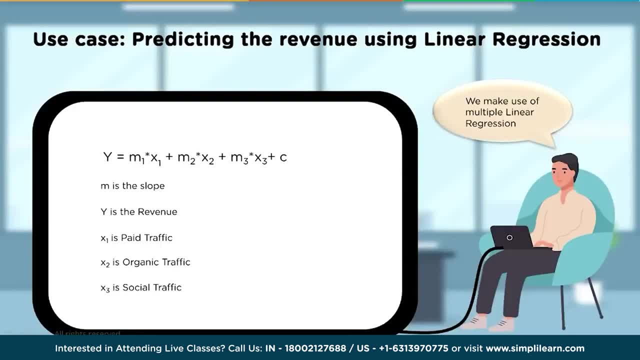 lines. Y is the revenue, So we're only looking for one variable And remember, this is regression. so we're looking for a number: X1 is going to be the paid traffic And, of course, M1, the corresponding slope, X2, the organic traffic And X3, the social traffic. We will follow. 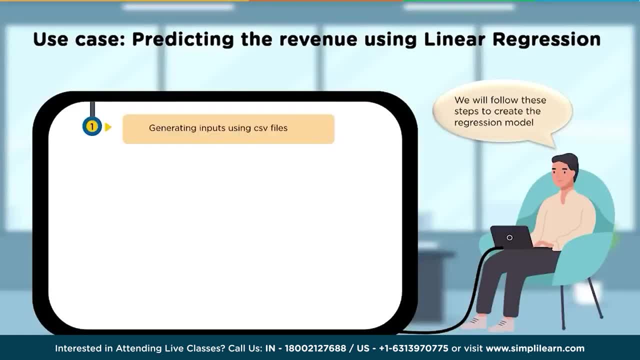 these steps to create the regression model. We're going to start with the pay traffic. We're going to use the regression model. We'll start by generating inputs using the CSV files. We'll then import the libraries, Splitting the data into train and test Very 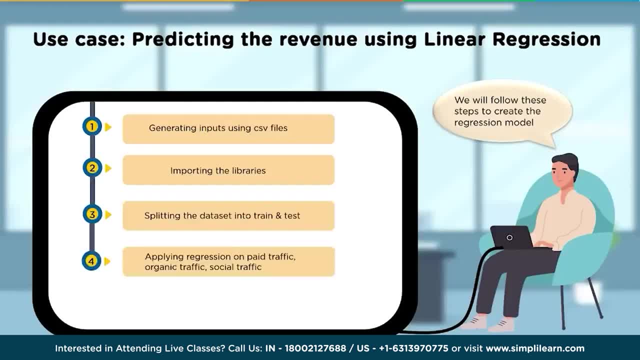 important whenever you're doing any kind of data science, Applying regression on paid traffic, organic traffic, social traffic. So we're going to apply a regression model on them And then we're going to validate the model. That's the whole reason we split. 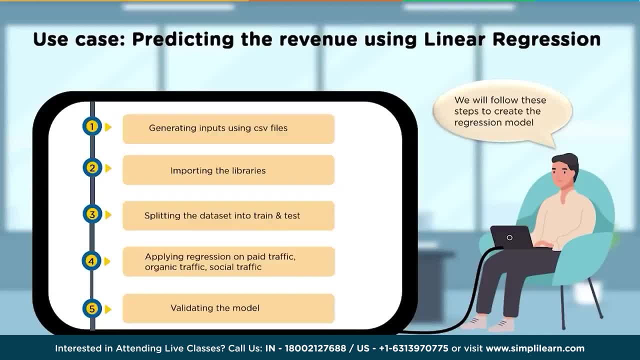 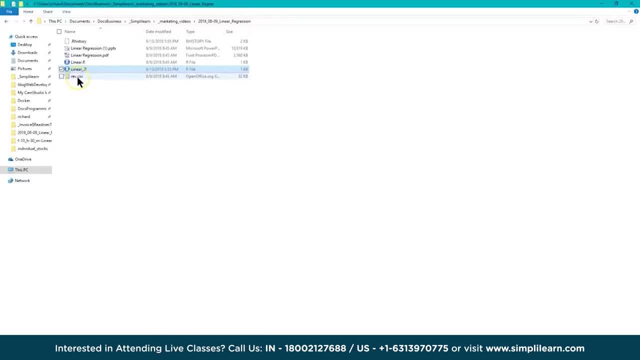 it to a training and testing is so we can now validate to see just how good our model is. Now, before we open up R, I always like to just take a quick look at the data. It's going to show us the data itself, And we're using the revcsv file And this is a cs file. 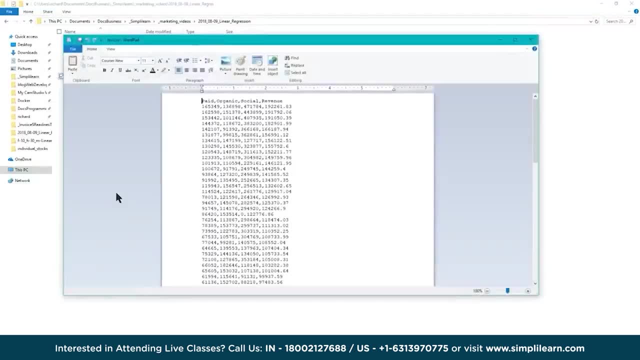 or a comma separated variable file. We'll just open that with WordPad. Any kind of text editor would be nice to show you what's going on And you can see we have paid organic, social and revenue across the top. So those are your titles for your columns And the 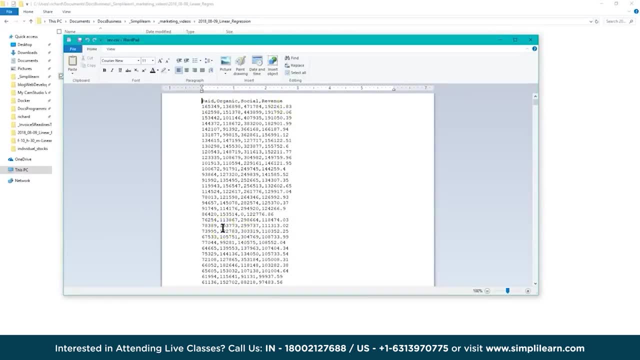 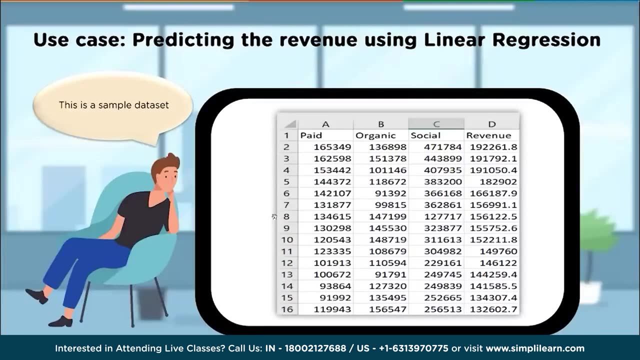 value is going down, And this is the same as what we saw on the slide just a minute ago: Paid, organic, social and then revenue from them. They probably have it in more of a spreadsheet than just a WordPad. In the newer version of RStudio, which already has a nice layout, It automatically opens. 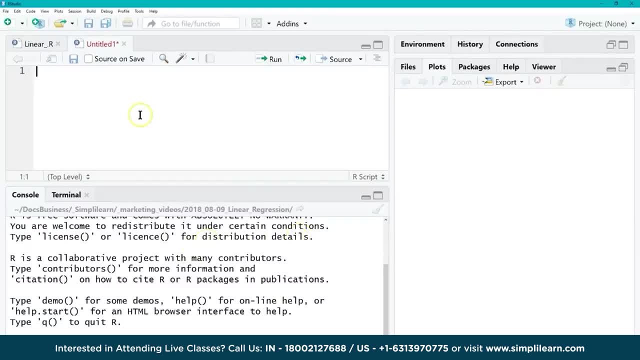 up with your console and terminal window. down and left You have your script And we'll run it in script And then when I run it line by line in script, you'll see it show up on the console bottom left. I could type it straight into the console and it would do the same. 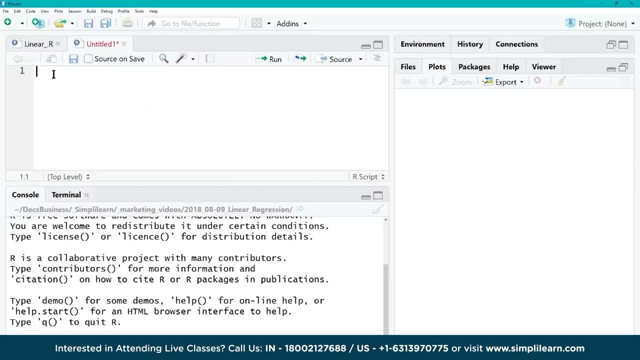 thing, And then on the right we have our environment, And under the environment we'll see plots. If you're in an older version, the plots will pop up And you usually are running just in the console And then you have to open up a different window to run. 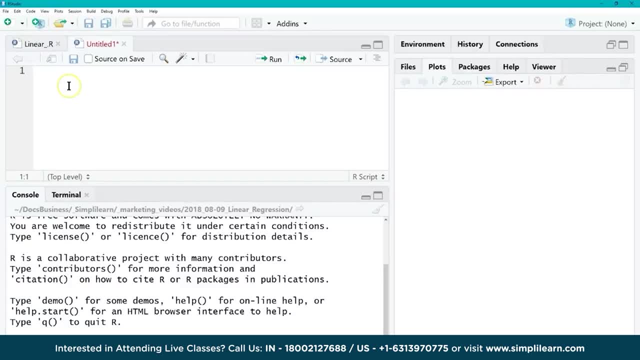 the script And you can run the script from there. This opens up everything at the same time when you use the new RStudio setup, And the first thing we want to do is we want to go ahead and generate a variable- We'll call it cells- And we want to load this with our data set. And so in R we use the less. 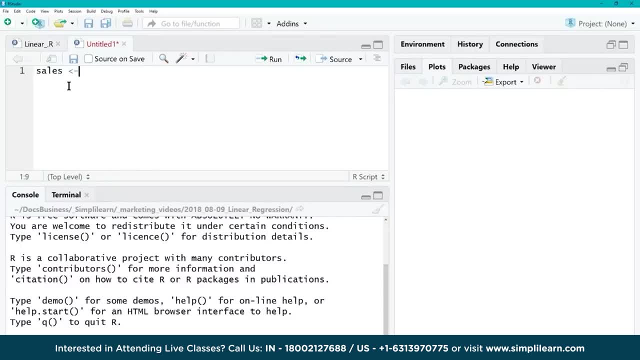 than minus sign. That's the same as assigned to. It's like an arrow pointing at cells And it says: whatever it goes past here is going to be assigned to cells And we want to read in our CSV file. And then I went ahead and fixed the CSV file up a little bit. 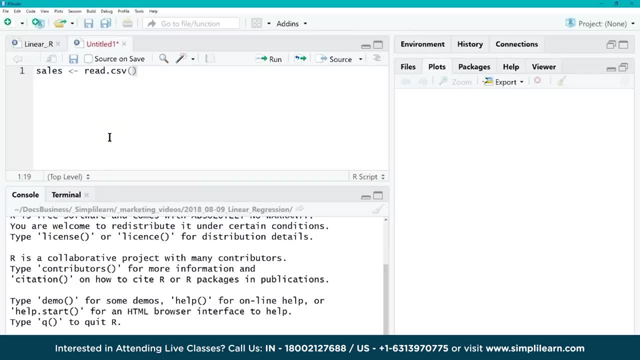 When I say the CSV file, I mean the path to it, And we'll go ahead and just paste that in there. And this is my edited version And you'll see I took: wherever we had the backward slash, I switched it for a forward slash, Because a backward slash is an escape character. 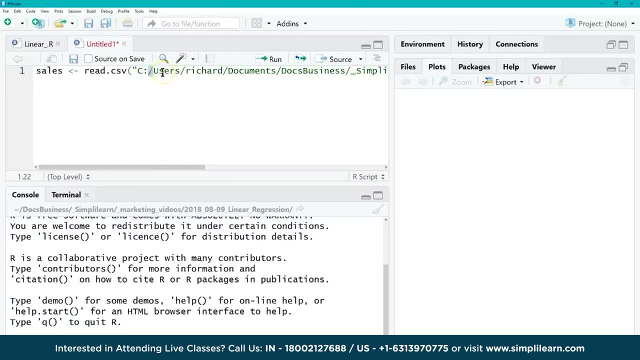 And whenever you're programming in just about any scripting language, you want to do the forward slash instead. So, like a good chef, I prepped this and copied it into my clipboard And we can see the full path here. And the full path ends in our revcsv file And we'll 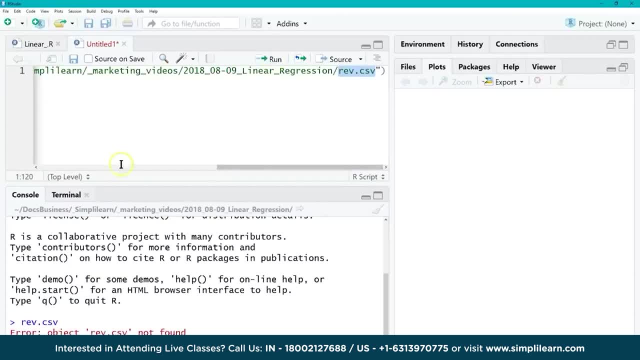 get that CSV file. So that's the path on my machine And then I'm going to run that And now we have down here. you see it appear right here. Uh-oh, must have an error in my path. It says: object: rev not found. Let me fix that real quick And run it again, And 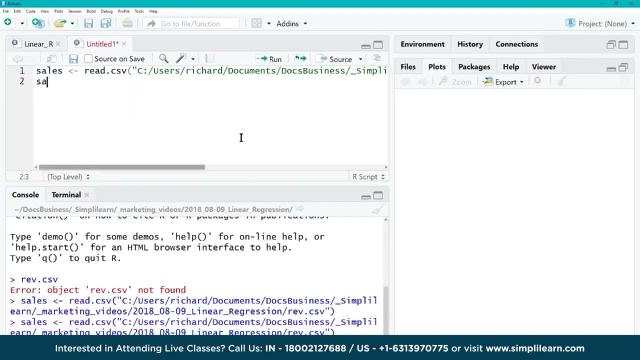 this time it does assign the cells, the data set, And then we'll just type in cells And this is the same as printing it. So if you work in other languages you'll do like print and then cells, or maybe print cells dot head if you're in Pandas and Python or something. 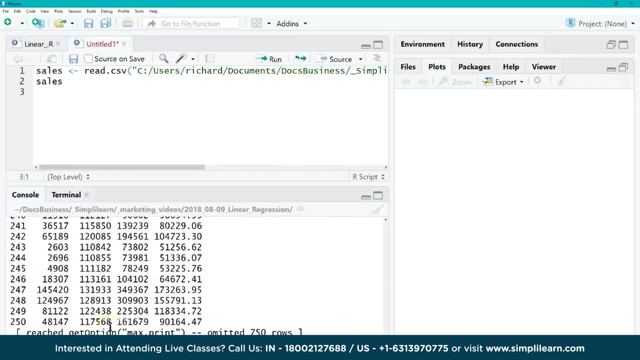 like that. But in R you just type in the variable We'll run this And you can see it printed out, all those columns. So that's the same thing we just looked at And it says max print. So it omitted 750 rows, So it has a total. 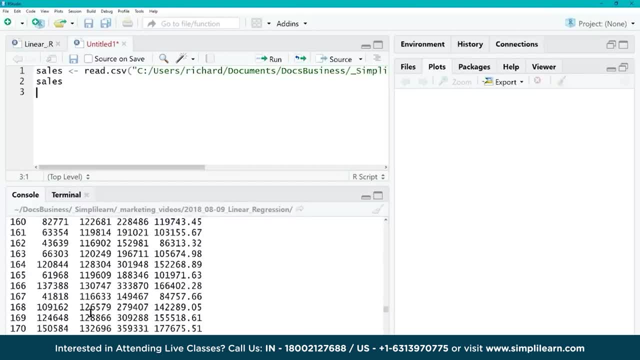 of 1,000 rows And we can scroll up here on our console where the answer came in. And if I scroll up to the top, whoop way up to the top, There we go, You'll see paid organic. 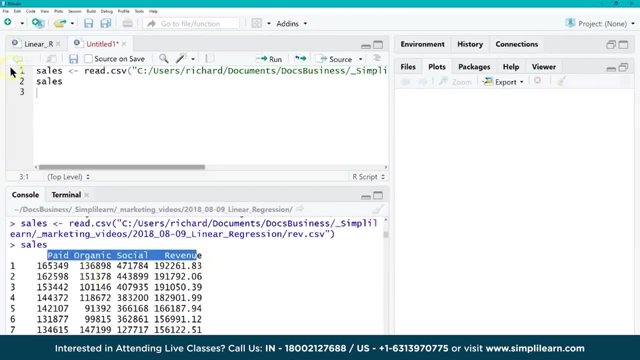 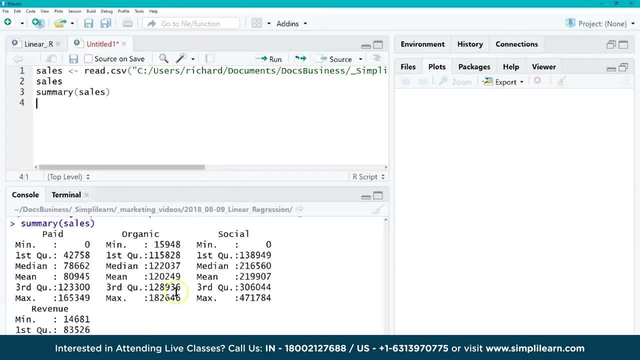 social and revenue. So everything looks good on this And there's a lot of cool things we can do with it. One of the things we can do is I can summary it. So let's do a summary of cells And we'll run that And the summary of cells. 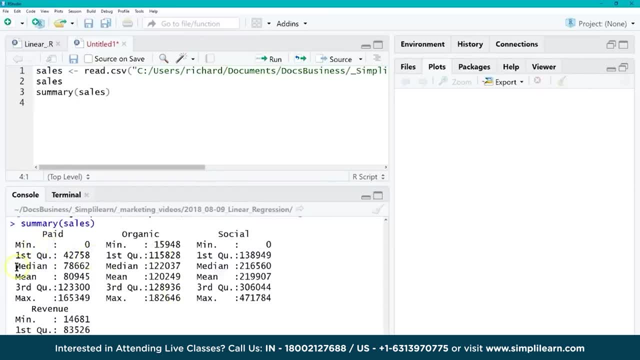 it comes in. It tells you your min. first quarter median mean third quarter max for paid organic social. It breaks it up And you can actually get kind of a quick view as to what the data is doing. You can take more time to study this. A lot of people look. 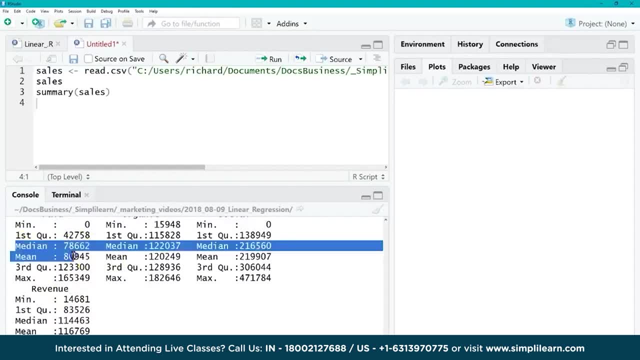 at this And you can see from the median the mean. that tells you a lot And it's divided into quarters, So you have your first quarter value and your third quarter set up on there and the max. It just gives you a quick idea of what's going on in the data. A summary: 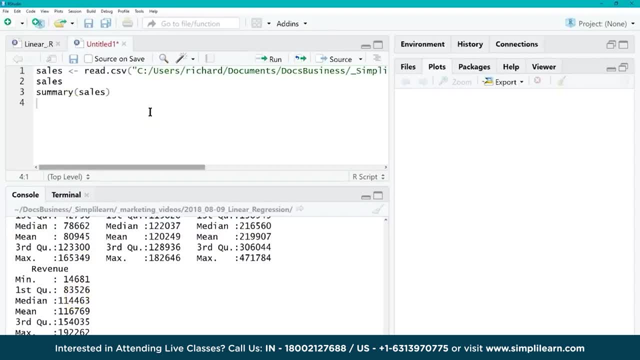 is a really wonderful tool. One of the reasons I like to jump into R before I might do a major project in something else, or you could run everything in R And let's take a look at the head- head of cells And let me run this And you can see it just. 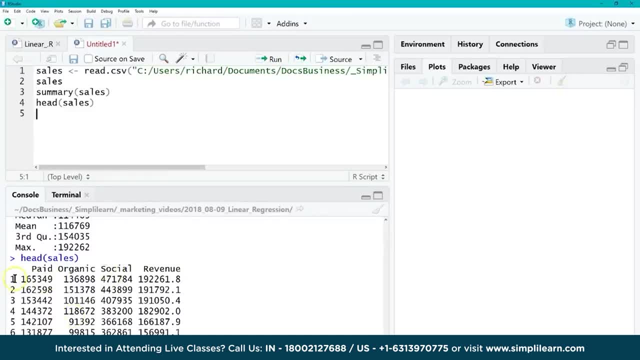 shows the head of our data, the first six rows in this case, And it starts with one Important to know. Other different systems start with zero and go up. R is one that starts with the first as one, And then, if we want to do a plot, I'll go ahead and do a plot: cells, Another, really. 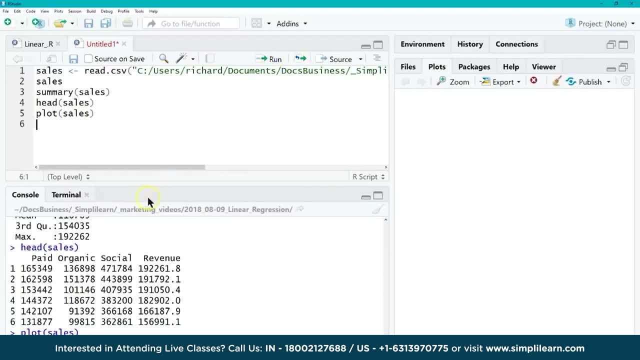 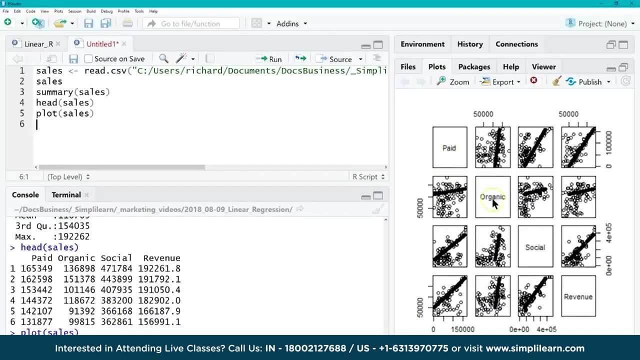 powerful tool that you can just jump right into with R once you have your data in here And you'll see that the plot comes over on the right hand side And what it does is it compares them. So if I look at my paid and my organic and you cross the two, you'll see there's a nice line down the 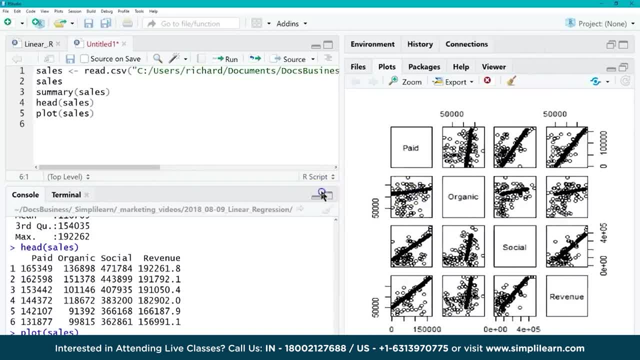 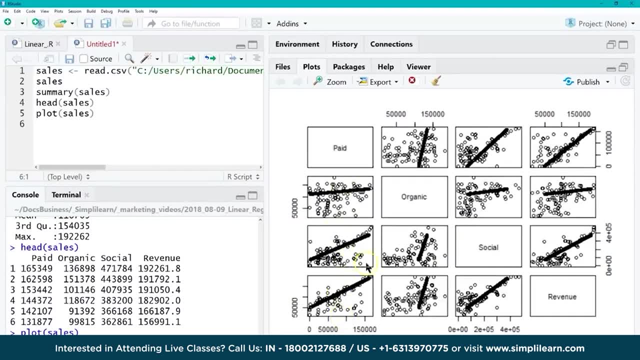 middle Big black line where it plots the two together. Let me just widen this a little bit so we can see more of it. There we go The same thing with paid and social paid and revenue. So each one of these has a clear connection to each other. So that's a good. 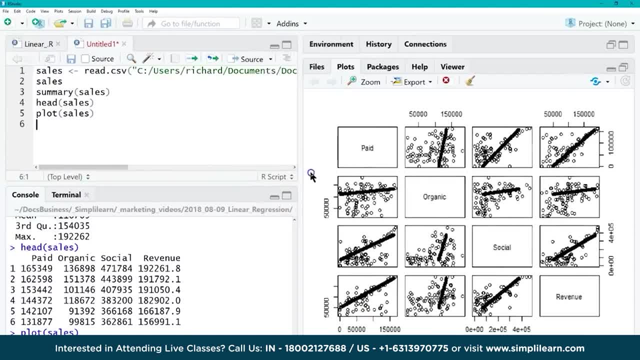 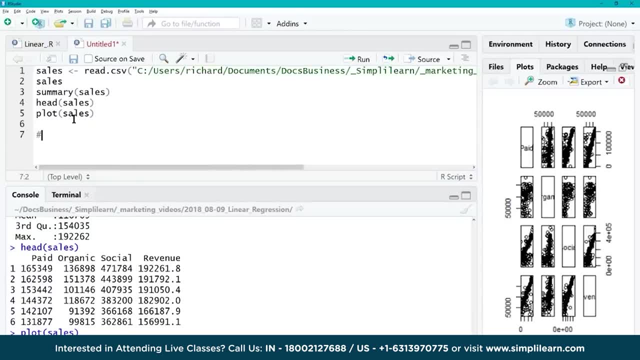 sign. We have a nice correlation between the data and you can just eyeball that. That's a good way to jump in and explore your data rather quickly and see what's going on. So we'll go ahead and I'll put a pound sign there. 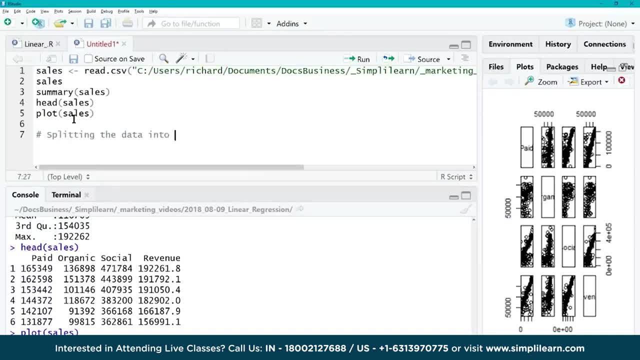 a hashtag and splitting the data into training and test data, And we want to split it so that we have something to work with to train our data set. And when we do our data set, you do this with any data set because you want to make sure you have a good model And 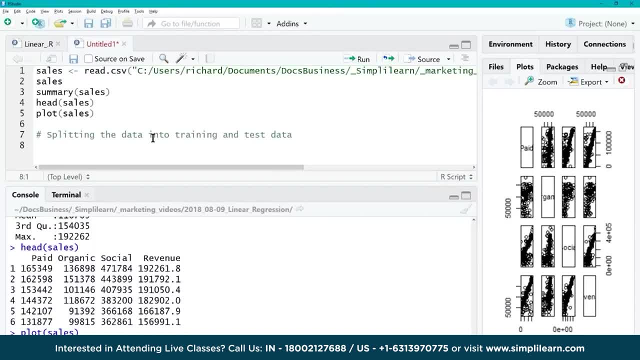 then, once we've trained it, we're going to take the other set of data we pulled off to the side and we'll test it to see how good it is. If you test it with the training data, it's already got that memorized and should give you a really good answer. In fact, when 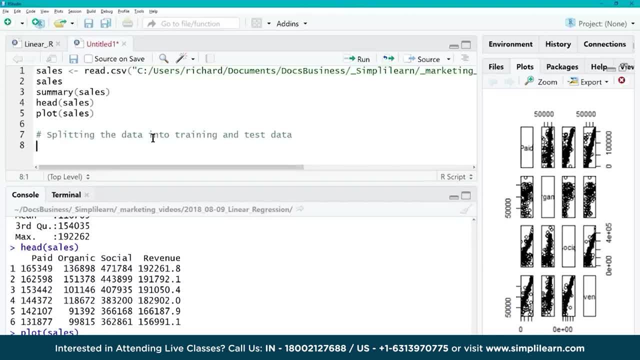 you get into more advanced machine learning tools. you watch those very closely. You watch your training set and how it does versus your testing set, And if your training set starts doing better than your testing set, then you're starting to overtrain it. Now, that's more. 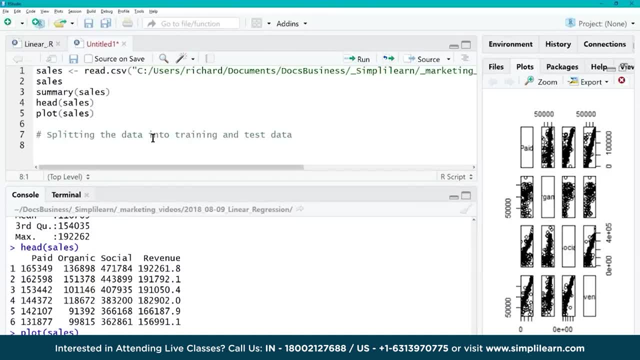 with deep learning and some other packages that are beyond what we're working with today. But, yeah, this is important. It's very important to understand that that test and that training correlate with each other and gives you an idea of what's going on And to make sure. 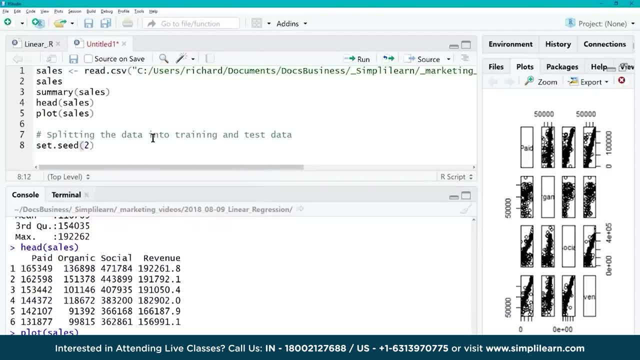 you're doing that correctly, And we'll go ahead and set a seed of two And that's for our random generators, So that when we run them you can seed them with just a. there's always to randomize a number or you can do like date and stuff like that, But that way 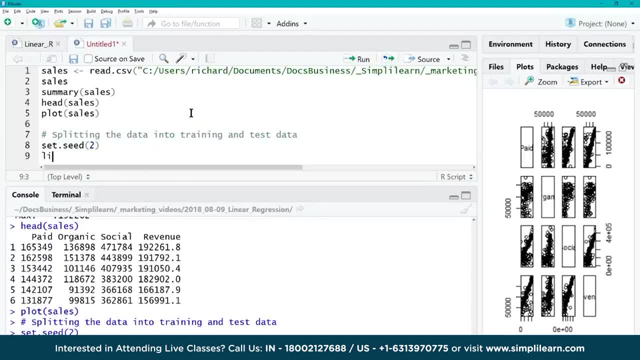 we always use the same random numbers, So we'll seed it with two, And then we're going to need a library. In this case, we're going to import the library And we want to import caTools, And caTools has our split function, So we're going to be able to split our data. 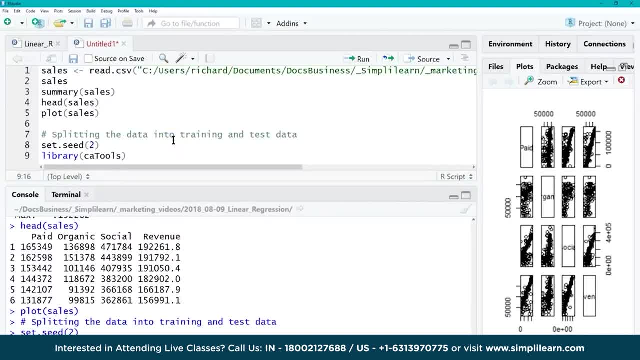 along with many of the other tools we're going to need for this example. So we're going to import caTools, So they're all built into the caTools. That's why we need to import that. A lot of times they call them library, or sometimes you hear them referred to as 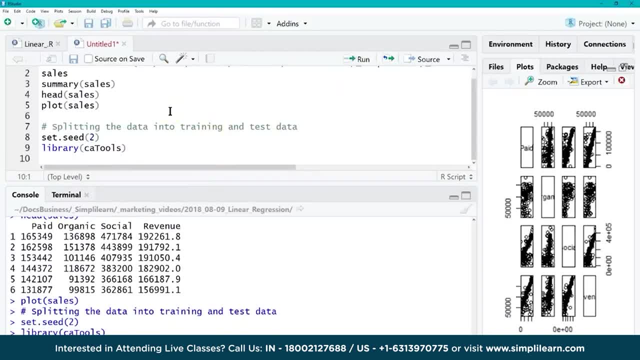 packages. So let's go ahead and run that line And that brings the library in. So now we can use all those different tools that are in there. And then I'm going to do a split And we're going to assign to the split that's going to be our variable sample split. Okay, 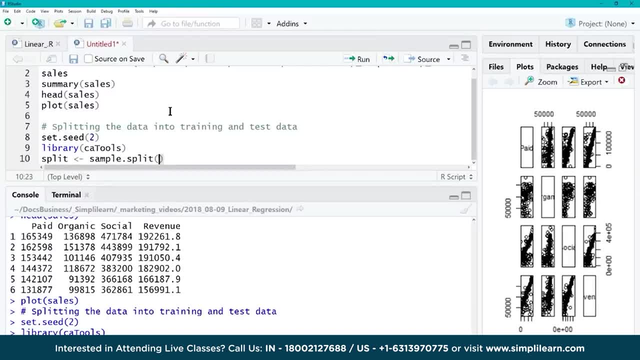 So that's one of the tools we just brought in- is to sample. is the actual keyword or the function word samplesplit? And we're going to take our cells and we're going to go ahead and do a split ratio equals to 0.7.. And let's do 0.7 so we make sure it knows it's a decimal. 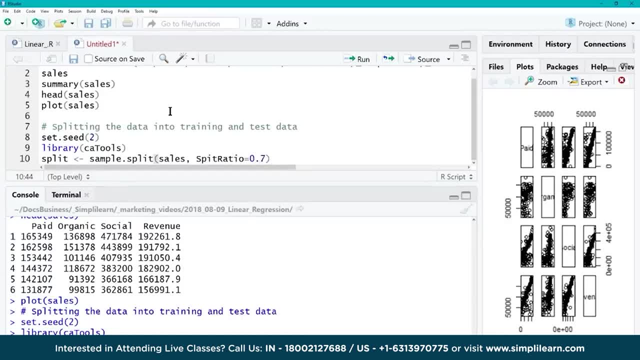 point or float, And what this is saying is that we're going to take our cells data, the variable we created called cells. it has the data in there And I want to split it, And I'm going to split it so that 70% of it goes in one side. We'll use that for training. 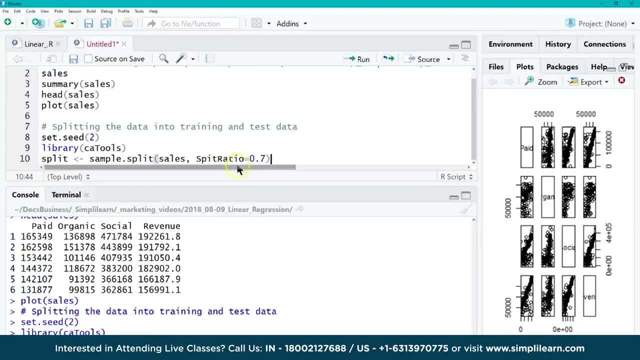 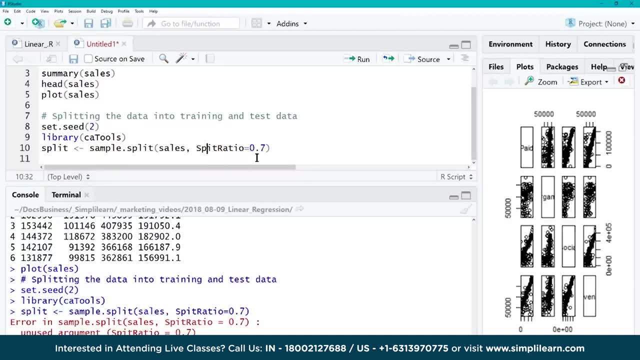 And 30% will go into the other side, which we'll use then for testing out our model. Let me go ahead and run that And hold on one second. Got an error there. Spit is definitely very different than split. I don't think we want. 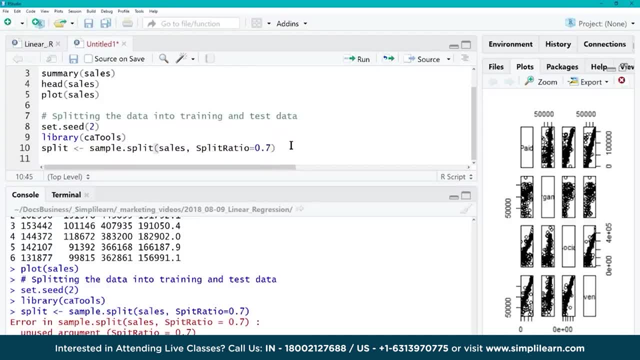 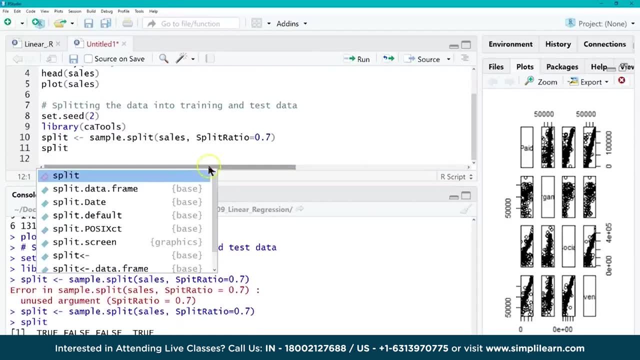 to spit our data out, which is actually kind of what we're doing is spitting it out, But we want to split. We want to split the data. Let me get that spelled correctly, And then, when I type in split, we can just run that, because that's now a variable. You'll see. 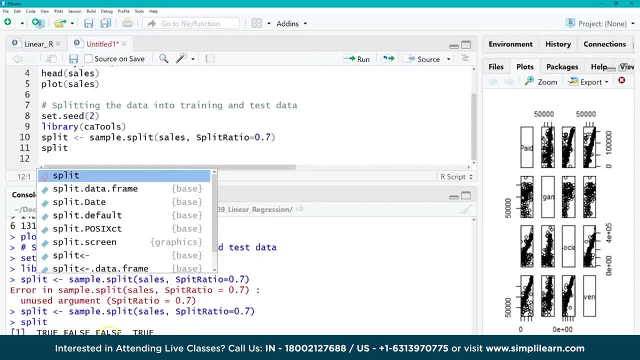 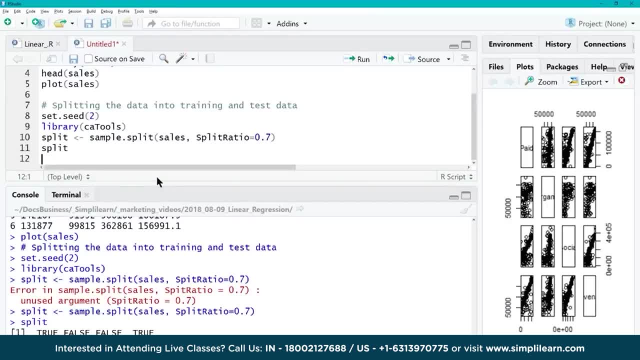 means down there, And then true, false, false, true. That means that's how we are looking at the data. We are splitting all those different pieces of data in line 1 in different directions, And so we now want to create our train set And we're going to assign that And when we 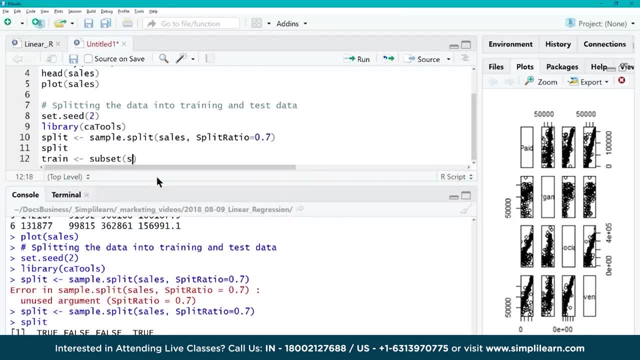 take it and we assign to the train set a subset of cells And then the subset of cells is going to be based on split equal. and I put this in brackets, true, So you can see the down here is capital T, capital R, capital U, capital E. so I just want to reflect. 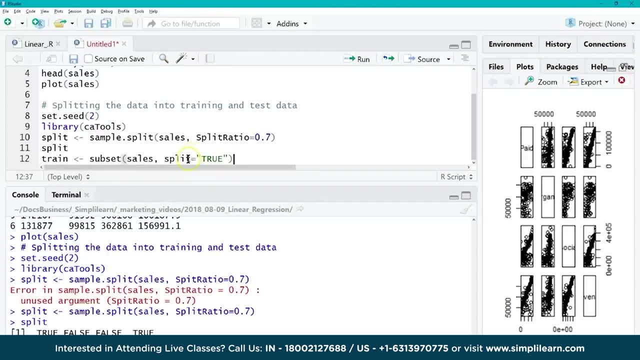 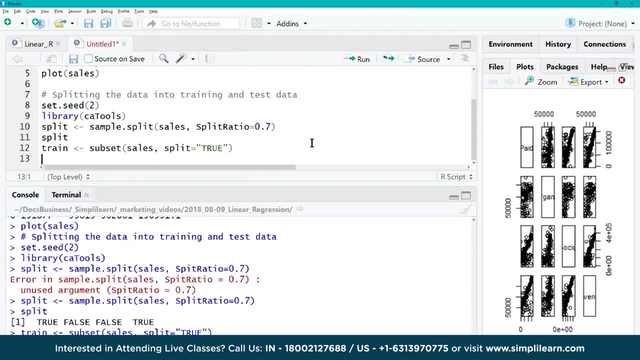 that on the train and this is going to take everything where our split variable is equal to true and it's going to set cells equal to that and we'll go ahead and run that, and then we're going to set our test variable as a subset of cells. 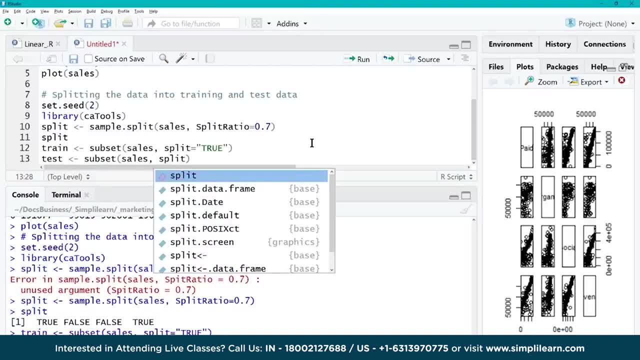 and if we assign the true to the train set, then we want to assign the false to our test set. so now we'll have this will have 30% of the variables in it and train will have 70%. we'll go ahead and run that. so we've now created both our. 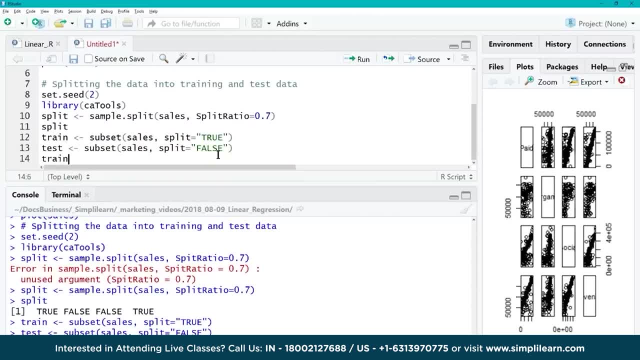 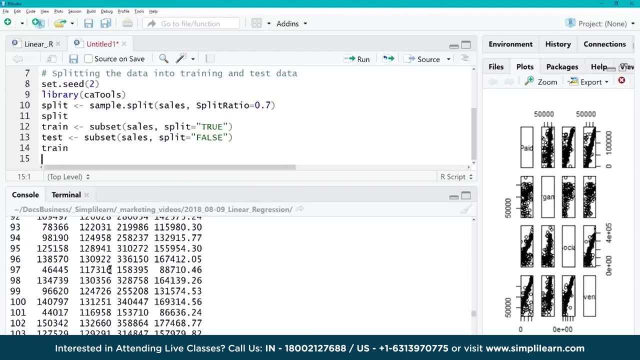 training set and our test set and we can just real quickly type in train hit the run on there and you can see our train set. if I scroll way up to the top, I'll have the column names on there, which should match what we had before paid. 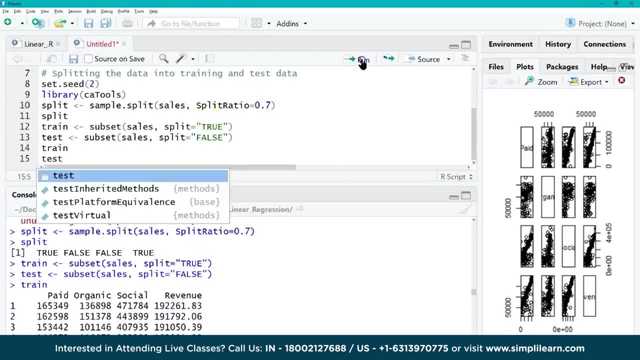 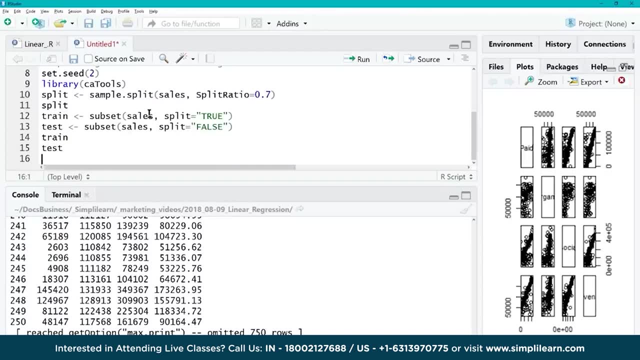 organic, social and revenue, and then we'll type in test. when I hit run on there, that's going to do the same thing. it'll spit out all the test variables going out. so now that we have the test and train variables, we want to go ahead and create the model. 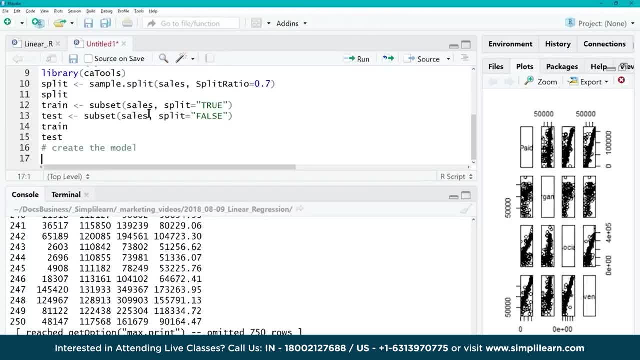 and we're going to go ahead and create the model. and we're going to go ahead and create the model, and you'll see this in any of the machine learning. and we're going to create the model, and you'll see this in any of the machine. 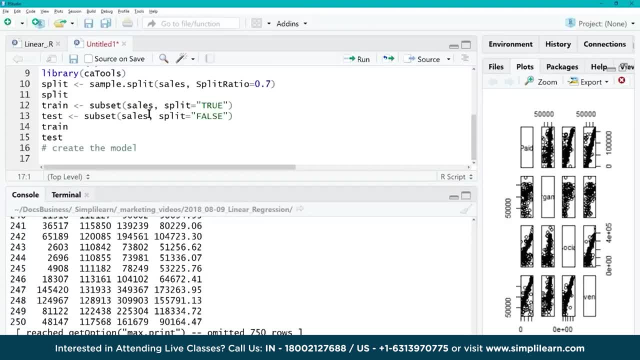 tutorials they always refer to them as models for modeling, a function of some kind on the data to fit the data. and then we're gonna put the test data through there to see how well it does, and so we're going to create the variable called models and I'm going to assign that LM. that is our linear. 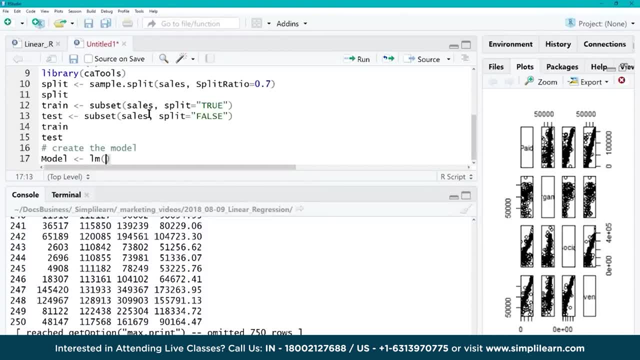 regression model I left out. simplified R makes it just LM- linear regression- and then model em. I guess it dates back because the linear regression models, like one of the first major models used so they kept it easy on there and revenue happens to be the main variable that we want to track. so if you remember correctly from our formula, Y is the 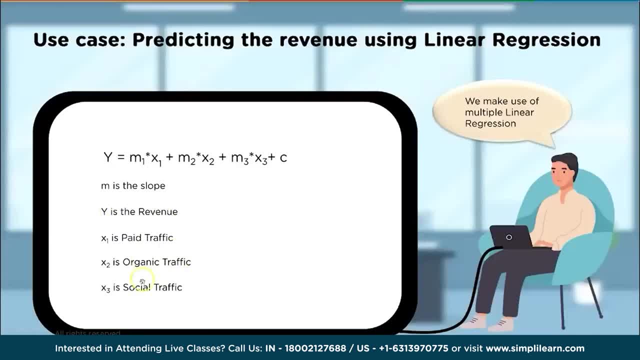 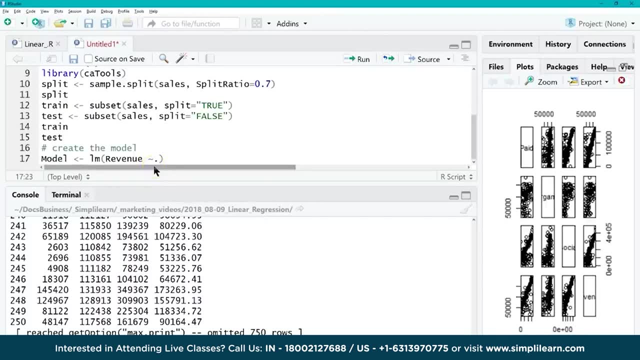 revenue and then we have X is our paid traffic, X to organic traffic, and x3 our social traffic. so Y is what we want to predict in here, and then you'll see this notation where we have our squiggle and the period, which means we're gonna match up the revenue lines with the lines of the data we're. 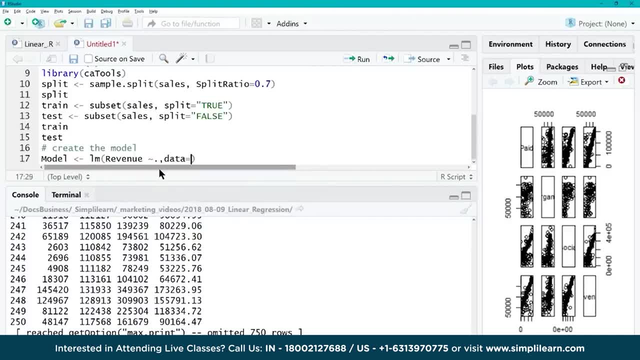 putting in here and then I'll put comma and then our data equals train and of course that's the training data that we creative. so when I hit the run, remember we did all that discussion about all those different functions and formulas to compute our model and how that set up when it comes down. 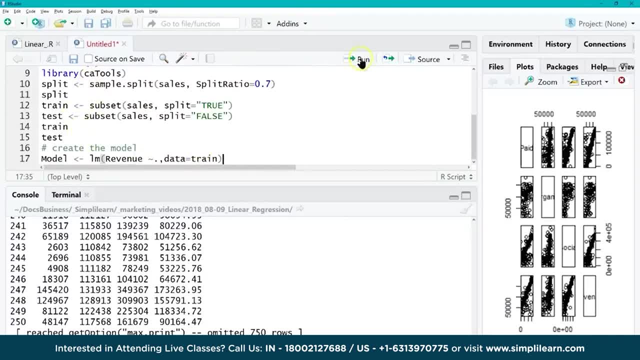 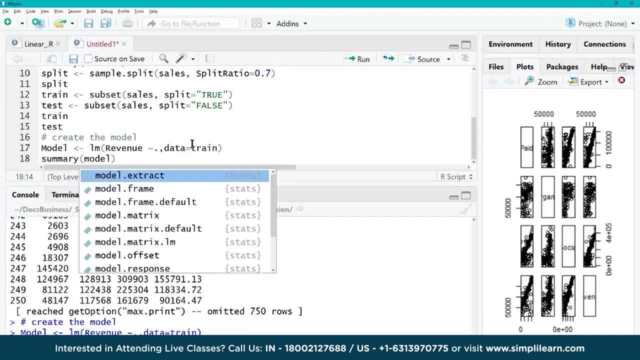 to it. we spend all our time setting up our data and then I hit the run button on the single line and our models been trained. so we now have a trained model here and we can do a summary of the model. summary is such a wonderful command because you can do that on our. that works on. 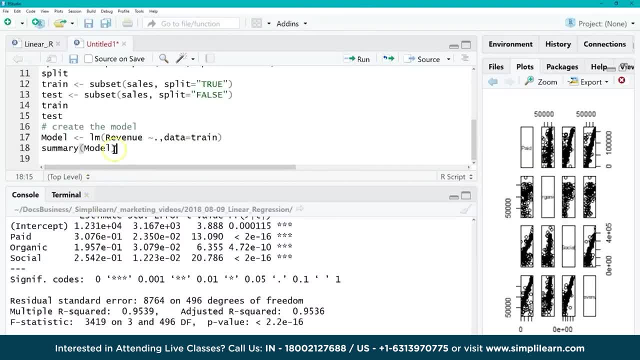 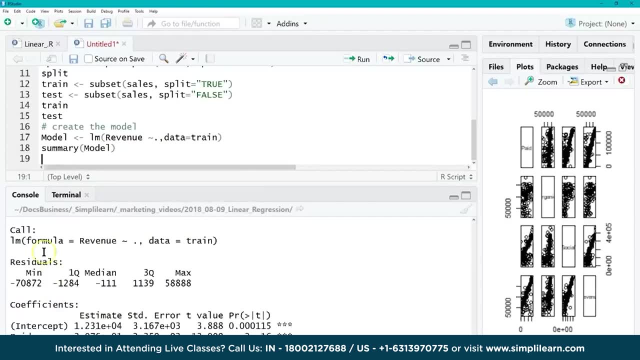 all kinds of different things on there. oops, and of course it does help if I remember that my model has a capital N when I run it and you'll see right here tells you a little bit about the model. use a summary on there, comes down here: 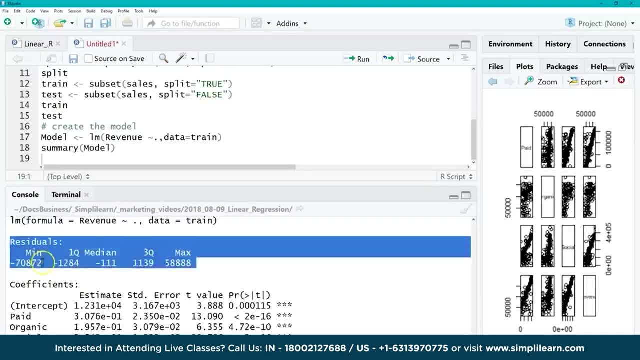 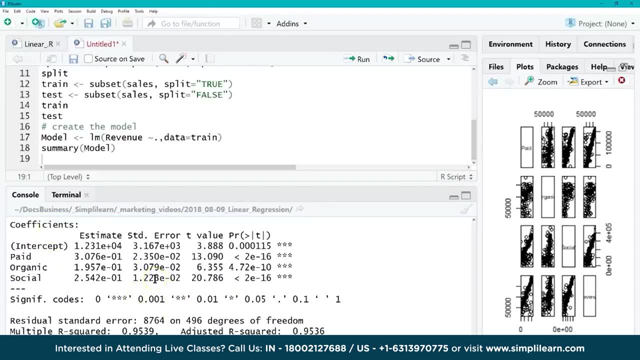 it has our residuals. this is all the information on there. as far as, like, the minimum, the median, the max has all our coefficients in there. if you remember correctly from our formula, let's just go ahead and switch back over to that. we have m1, x1, m2, x2, m3, x3 plus C. well, that's right here. here's. 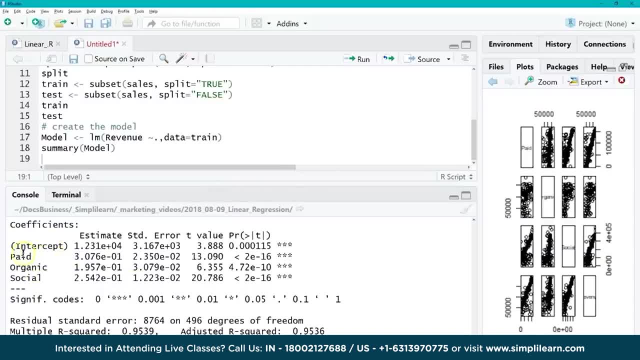 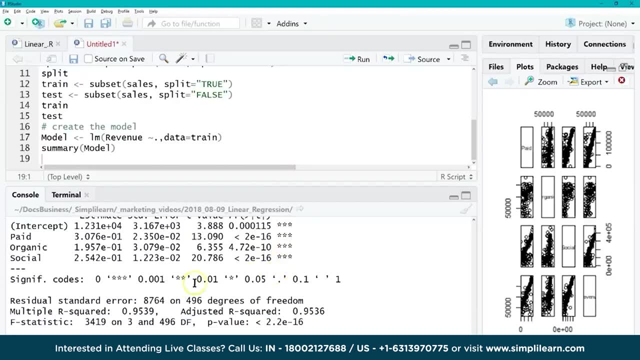 our intercept and then we have our different values for each of those and then we have our refresher values. so we have these again. we have our intercept, our paid, organic and social, and then it also shows us error and information on the air and the really nice things about when. 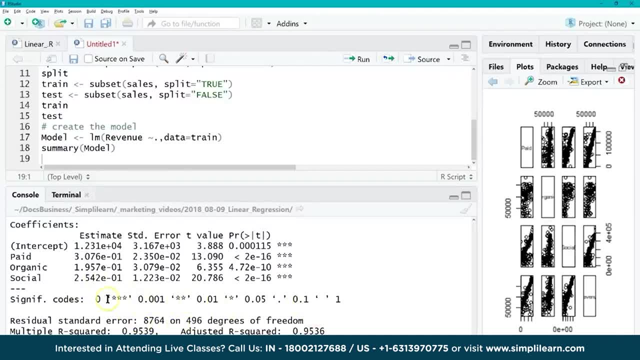 you're working with our and come down here and you see where we have our stars down here and it says 3 stars. really good, two stars maybe. one star, probably no correlation and we can see with all of these three stars on them. so out of three stars we get three stars. in all these there's no four. 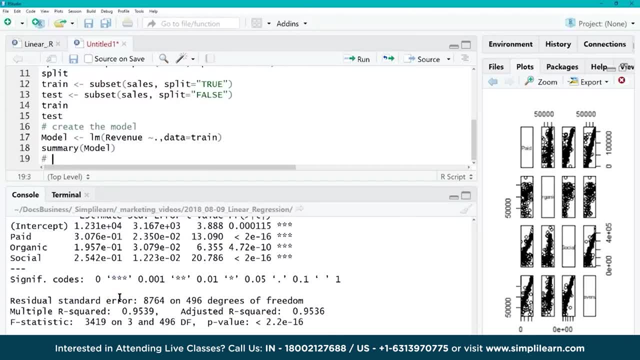 stars. four stars would mean that you have the exact same same data going in as coming out, and then, if we're going to do this, we want to actually run a prediction on here, and that's what we saved our test data for. so let's come down here. we'll do. 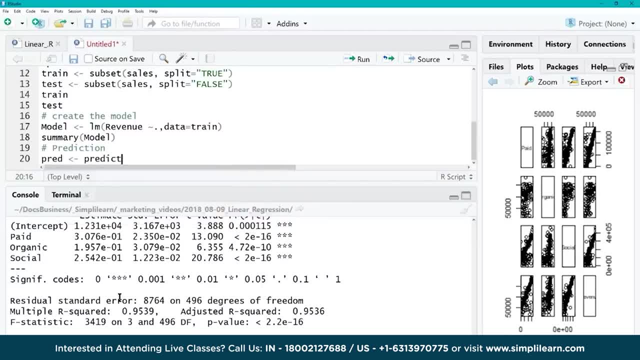 our prediction. we'll take this variable and we'll assign it predict model. remember the predict comes from when we imported that package, the ca tools. that's all part of the ca tools in there. so we're going to predict, we're going to use the model and then we're going to use our test data. pretty, 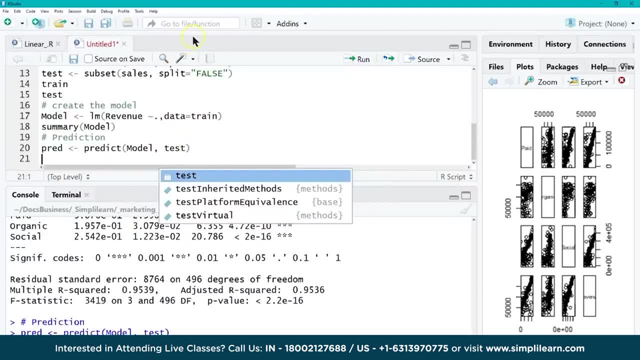 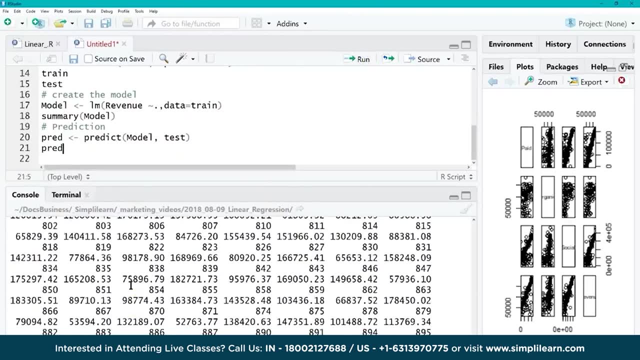 straightforward, quick and easy. we'll run this and then, if we go ahead and type in the predict, it'll print out what's in that variable and you'll see down here the predicted values it expects to come out. it's going to see our revenue is and it goes through and it gives it both the 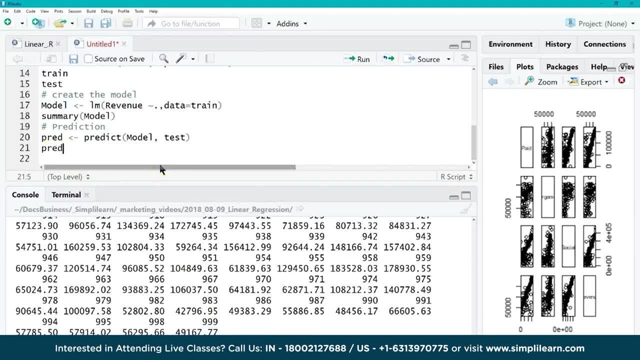 line number and the actual revenue value. so that's quick and easy boy. we got a prediction really fast and this is also how you would do it if you had new data coming in after this. you could predict the revenue based on these other factors. so now that we have a training model, which are we trained? 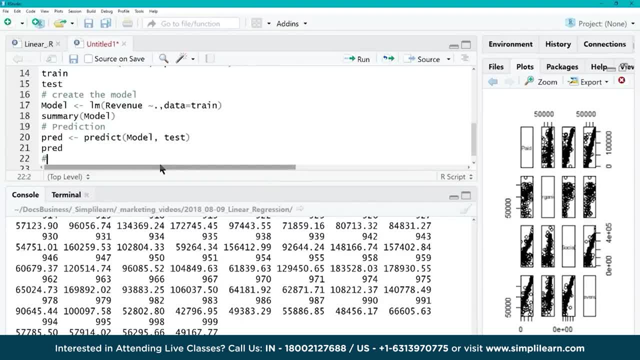 the data with our training data, or we trained the model with our training data and we've done a prediction on our model with our test data. we want to look this up and we took a quick glance from our training thing. our training said it trained really well. but that's not the final. 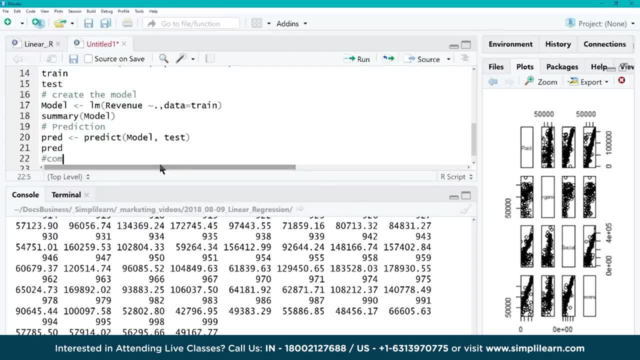 word on it. the final word is going to be comparing it. so we want to go ahead and do comparing predicted versus actual values. what I'm going to do is I'm going to do a plot and I'm going to do our test and we're going to do test: revenue: dot type equals. we're going to put this in as a type. 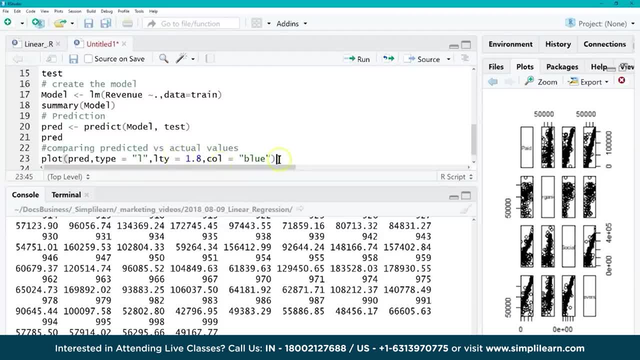 one and or L, and then we have lty equals 1.8 and we're going to set it for column blue. that's a lot of stuff in there. let's go ahead and just run that so you can see what that looks like and what. 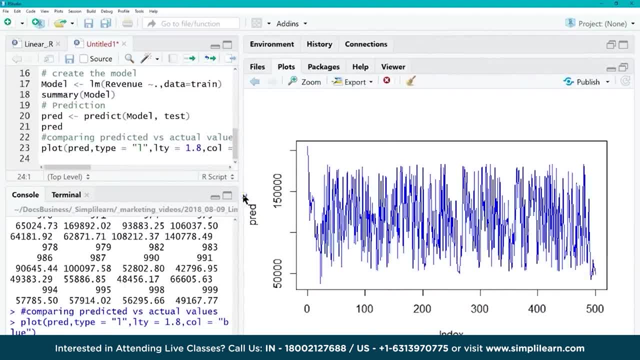 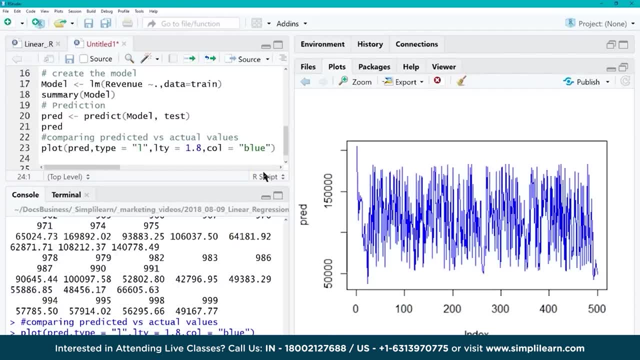 that's doing. it's going to generate this nice graph. we see on the right, there's our graph. you can see the data comes up and down. we're plotting the prediction on there. so this is the values we predicted, and then let's go ahead and do lines- and I actually did this backwards, so let me try. 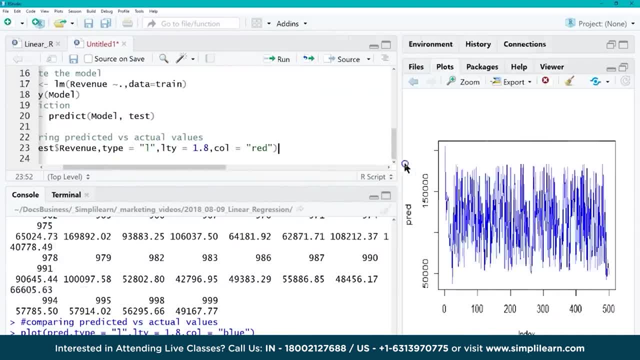 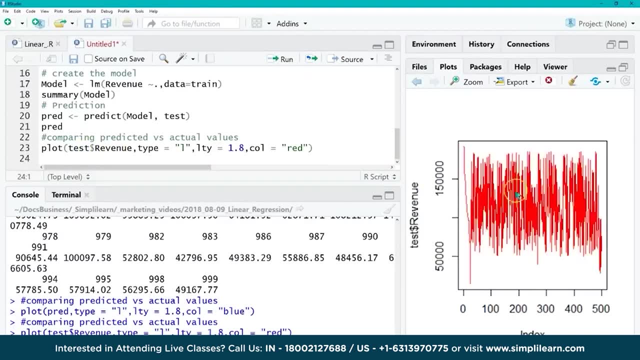 that again and we'll start with the red one. we're going to do the first one in red and I want to start with the actual test revenue. so here's our test revenue and we'll go ahead and run this, and so we have our red plot over here in red. go ahead and take a look at that, pull that over, you can see. 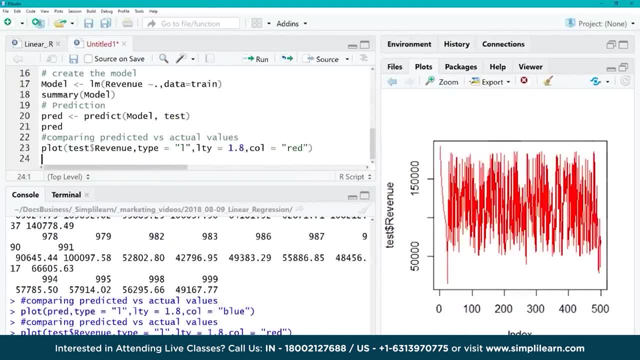 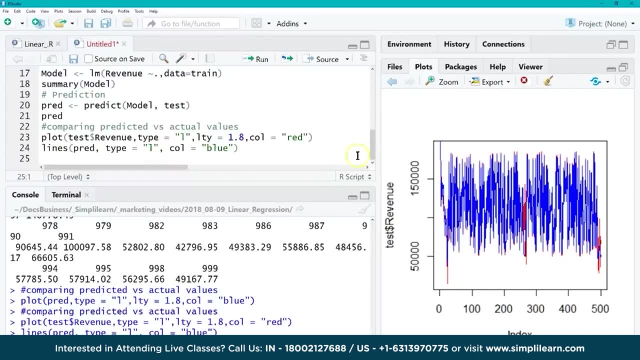 how that looks. it goes up and down, hard to track there, and then we're going to do a couple things here. we'll plot our test revenue and then we'll make it a little pretty, although it's kind of hard to say. see the way I was scrunched up here on the right, as far as size and sizing and 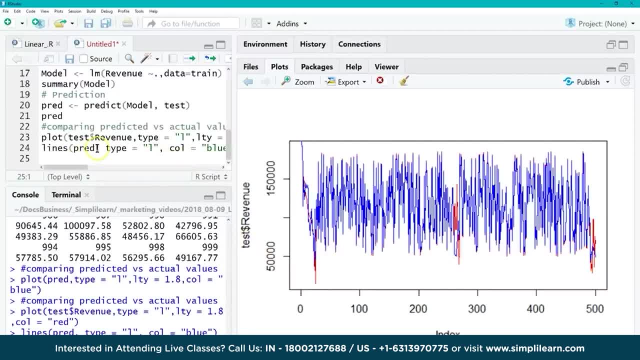 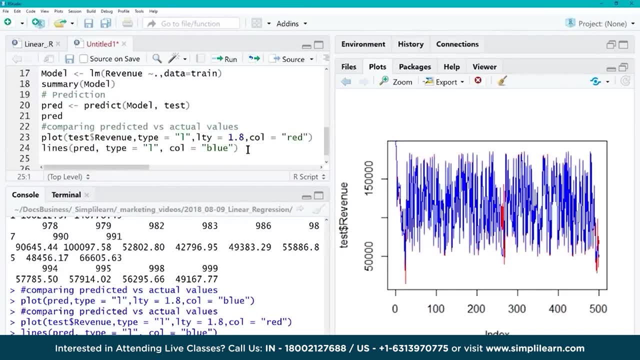 everything, but we'll go ahead and have our columns in blue and run our prediction on there too. you can see they overlap the two graphs. so we have our test revenue and our prediction, and then, finally, what I started with is we'll go ahead and plot the prediction. 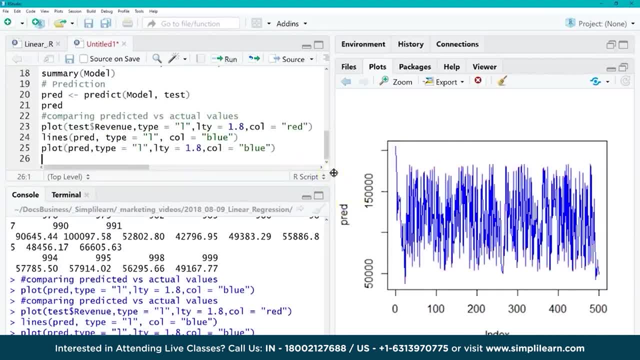 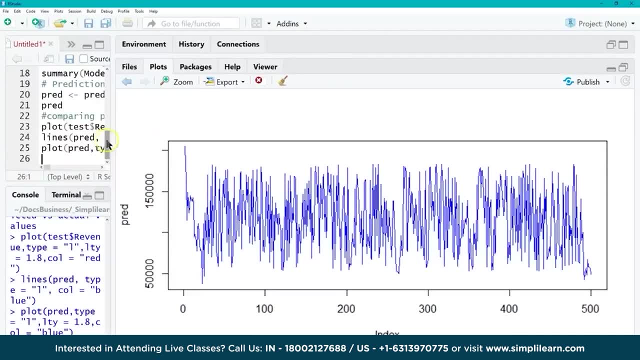 fully on the bottom and run that. and if you look over here on the graph, we put the blue lines over the red lines and so you'll see a couple spots where there's red underneath there, but for the most part our prediction is pretty right on. so it looks really tight, looks like a good set of 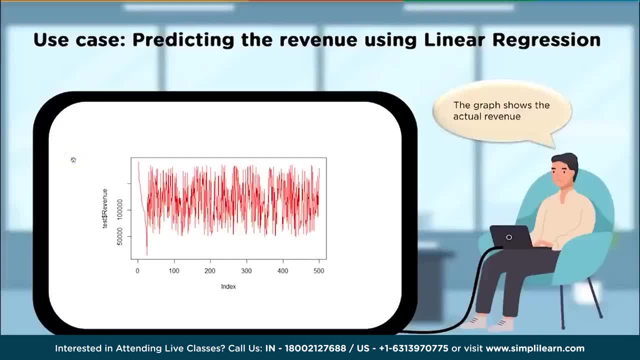 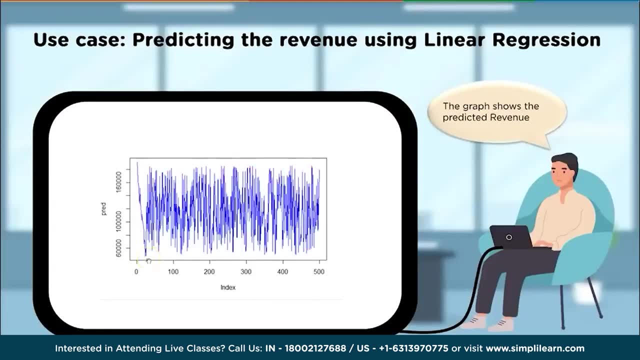 predictions for what we're working on and this is what we were looking at the slide right before we did RStudio. we can see in the slide here. here's a red- this is a little bit better spread out than what I have on my screen from my RStudio- and the graph shows a predicted revenue. we see that the 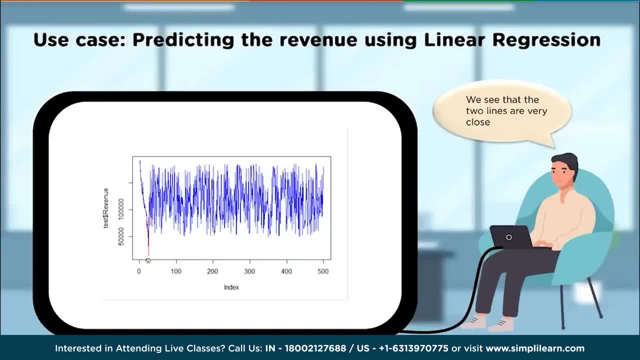 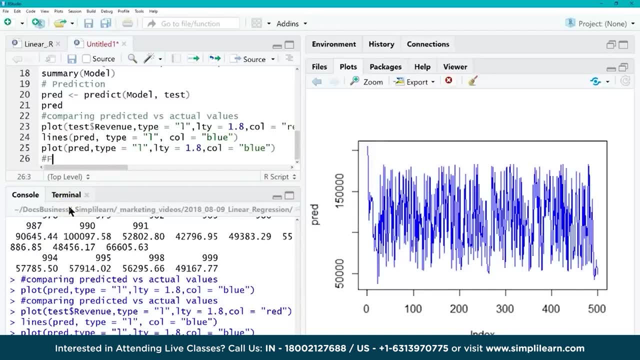 two lines are very close, so again they're tight. it's right on. this is what we're looking for in our prediction model. but it's not good enough just having a graph and you always do both. and the reason we do both is you want to have a visual of it, because sometimes you look at these, you get to. 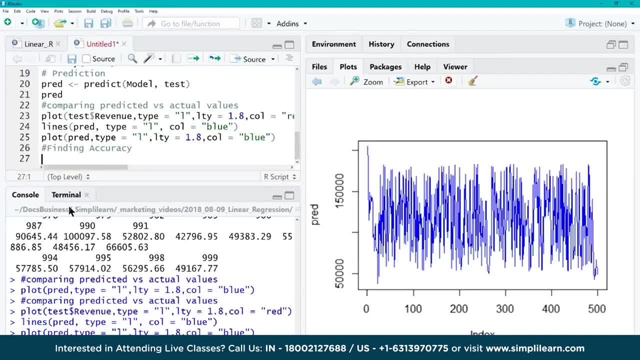 the graph, you're like, oh my gosh, what is that? and then sometimes you look at the graphic, oh that's right on. how come my accuracy doesn't look right. so we're going to go ahead and do that, and we're going to do that right, and you realize that your accuracy might be off or you're plotting it incorrectly. so 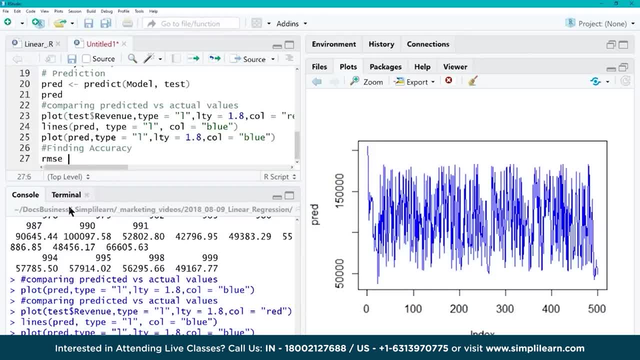 let's go ahead and look up the accuracy and we'll use RMSE- that's going to be the variable name we're going to give it- and sqrt the square root of the mean, and mean just means average. and then we want prediction minus cells revenue, and then we're going to take this whole thing and we're going 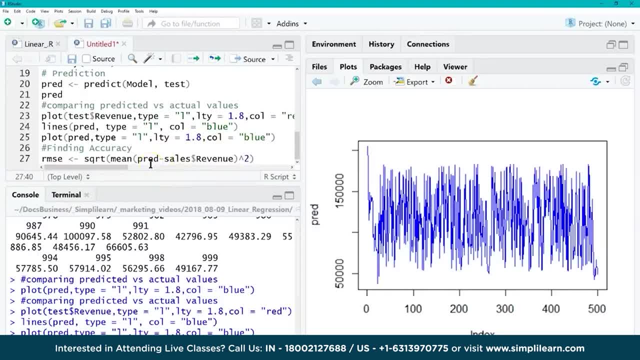 to square it. so what we've got here is we're going to go through. let's just explain this formula. we're going to look at the- what I predict it for to be, and what the actual cells. what's our prediction versus our cells, comparison to the revenue, and we compare those two. we're going to find the average. 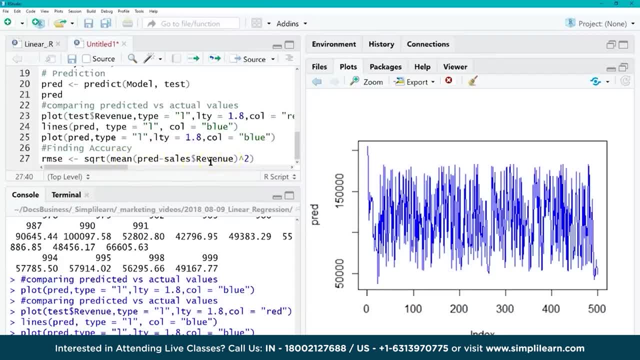 and then I'm going, or we're going to square each one of those values and then we're going to average the square and then find the square root of that. and that's quite a mouthful. the reason we do it this way, the reason we square the value and then we find the means, is to generate an answer based. 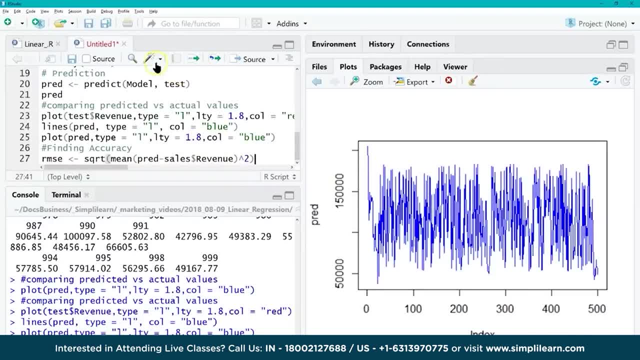 on. doesn't matter whether it's plus or minus. there's a lot of other formulas you can use there to check your accuracy and all kinds of other things you can do. but a quick, straightforward way of doing it is just like this: and then let's go ahead and run. 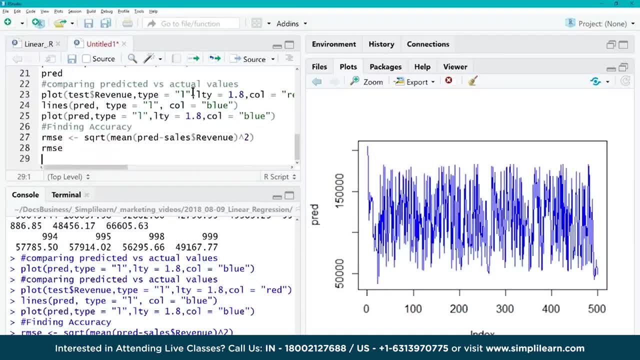 this and then we type in the RMSE and they'll give us an actual printed value out. let's just see what that looks like. and so we have 866.6338 for our accuracy. and so we look at the 866.63 and we 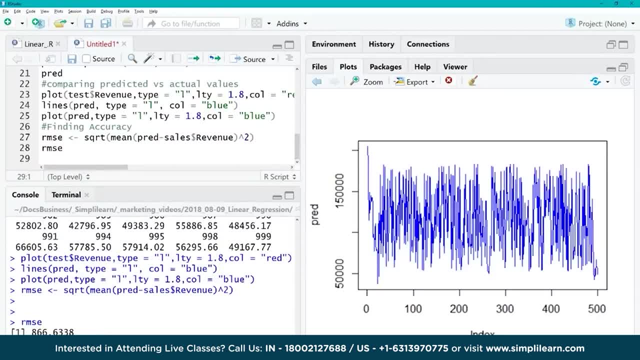 compare that to say, uh, 50 000.. that's pretty close, that's. that's actually a pretty good accuracy, given this model takes a little bit more when you're playing with accuracies and start dividing out other different aspects of it to get something you can communicate better with, but you 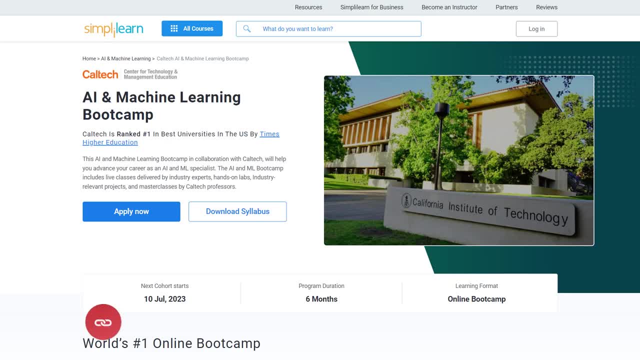 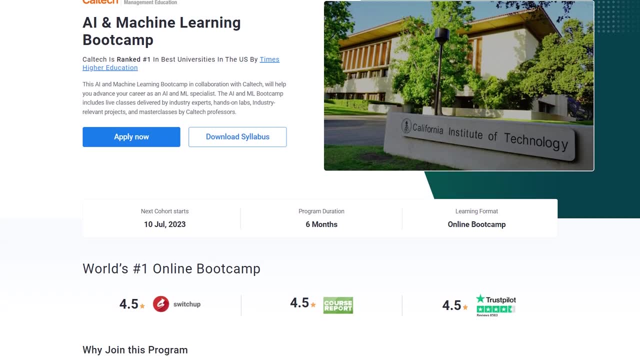 always start with the square root means it's always a good place to start, and now we are thrilled to present our AI bootcamp that is designed to equip you with the knowledge and skills you need to thrive in this fast-paced and ever-evolving field. in this six months intensive 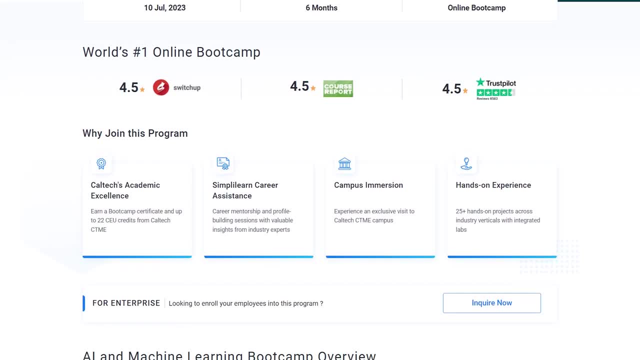 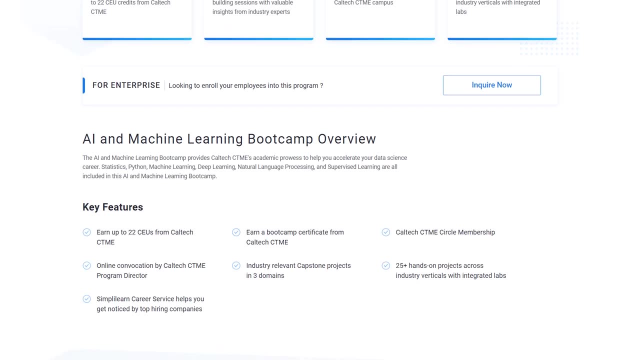 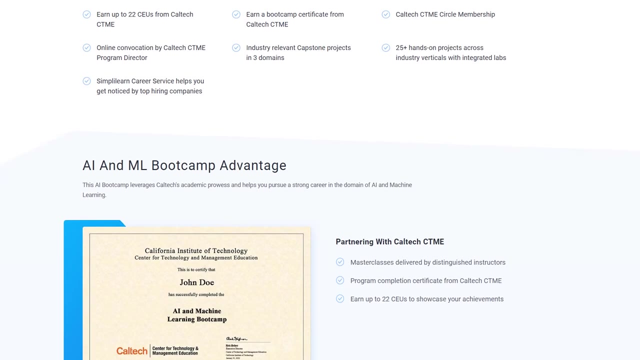 and immersive learning experience. you will have the opportunity to dive headfirst into the subject and building a strong foundation in AI. we believe in a practical approach where you will work on 25 plus hands-on projects across various industry verticals, providing you with real world experience. 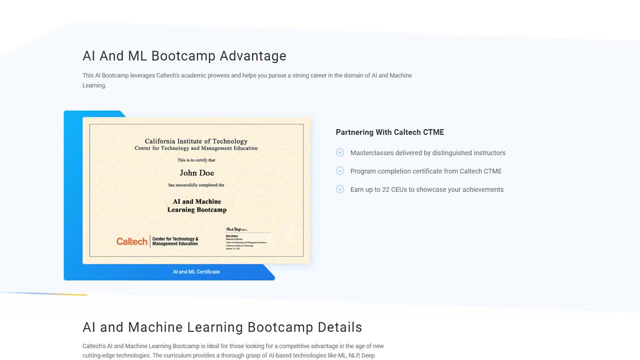 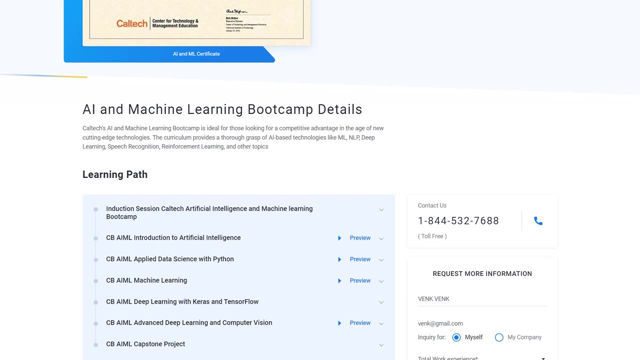 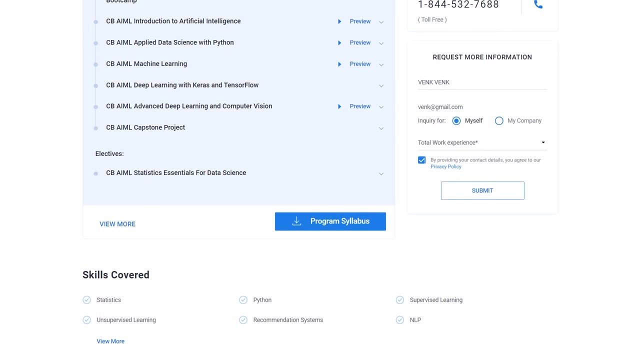 what sets our bootcamp apart is our partnership with caltech cdme, ensuring academic excellence and industry recognition. by successfully completing the bootcamp, you will earn a prestigious certificate and up to 22 cu credits from caltech ctm, validating your expertise in the field. so are you ready to? 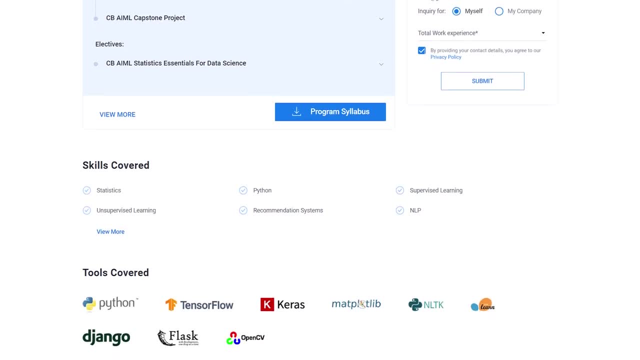 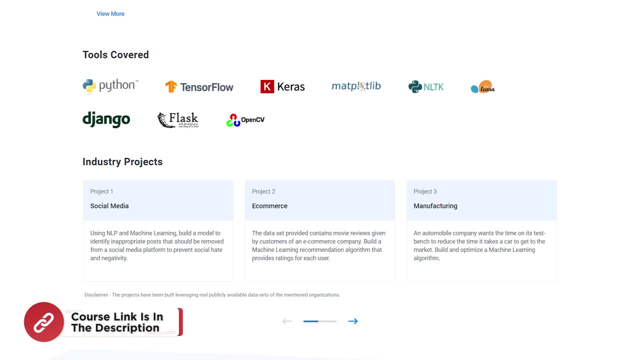 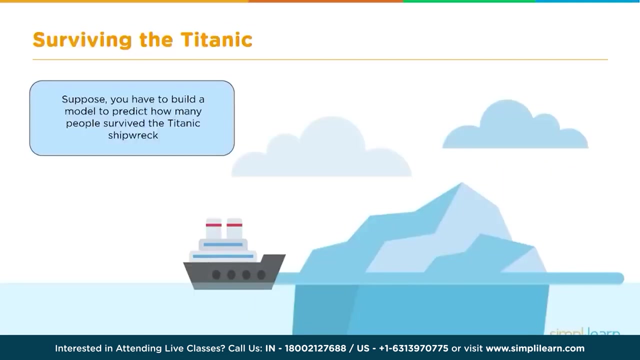 embark on this transformative Journey. are you ready to unlock the power of AI and take your career to new heights? if so, and roll in our AI bootcamp today and become part of the AI revolution. the course link is mentioned in the description box below. what is logistic regression? let's say we have to build a predictive model, or? 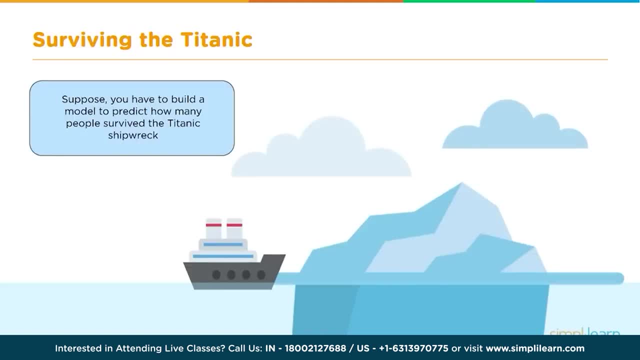 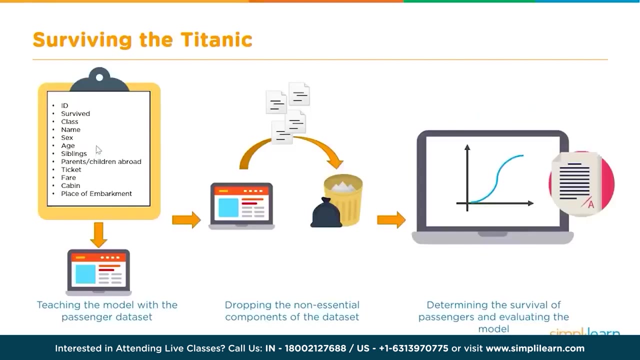 a machine learning model to predict whether the passengers of the Titanic ship have survived or not. the ship right. so how do we do that? so we use logistic regression to build a model for this. how do we use logistic regression? so we have the information about the passengers, their ID, whether. 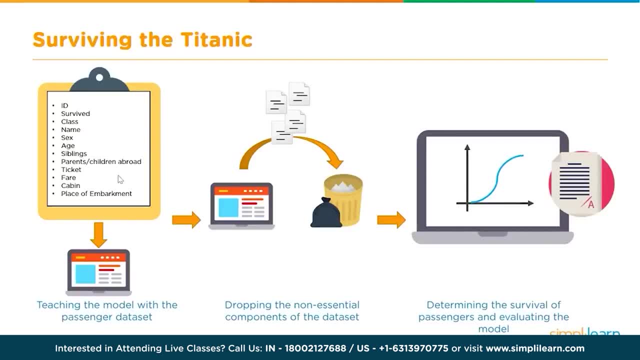 they have survived or not, their class and name and so on and so forth, and we use this information where we already know whether the person has survived or not. that is the labeled information, and we help the system to train based on this information with based on this labeled data. this 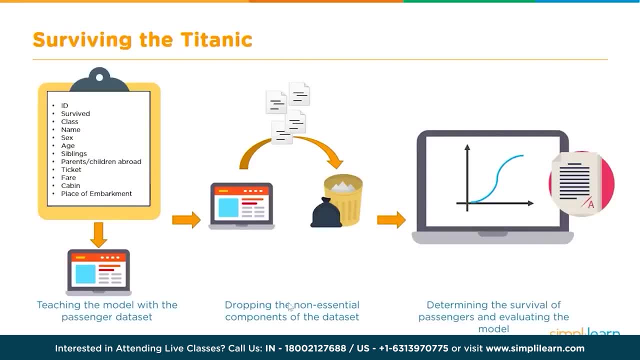 is known as labeled data, and during the process of building the model, we probably remove some of the non-essential parameters or attributes. here we only take those attributes which are really required to make these predictions, and once we train the model, we run new data through it whereby the model will predict whether the passenger has survived or not. let's start with. 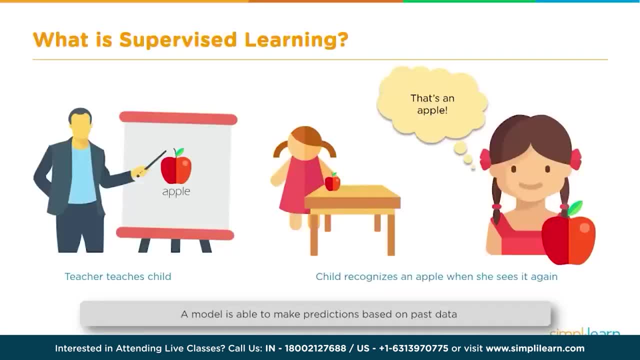 what is supervised learning? supervised learning is one of the two main types of machine learning methods. here we use what is known as labeled data to help the system learn. this is very similar to how we human beings learn. so let's say, you want to teach a child to recognize an apple. how do we do that? we never tell the child: okay, this is an apple has a. 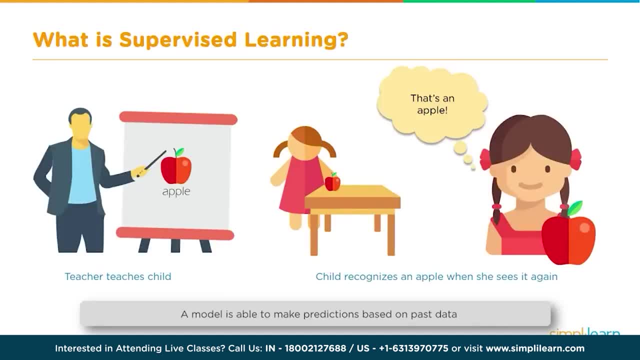 certain diameter on the top, a certain diameter at the bottom and this has a certain RGB color. no, we just show an apple to the child and tell the child: this is Apple. and then next time when we show an Apple, child immediately recognizes: yes, this is an Apple. supervised learning. 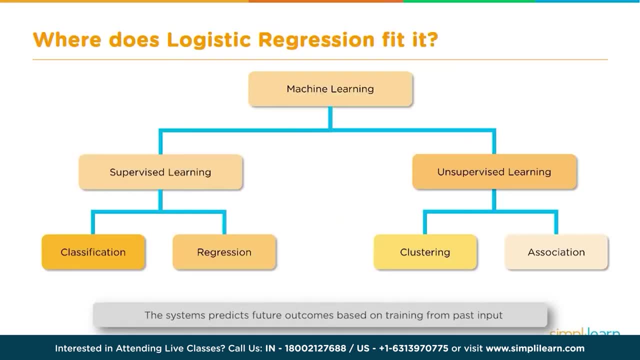 works very similar on the similar lines. so where does logistic regression fit into the overall machine learning process? machine learning is divided into two types, mainly two types. there is a third one called reinforcement learning, but we will not talk about that right now. so one is supervised learning and the other is unsupervised learning. unsupervised learning uses techniques. 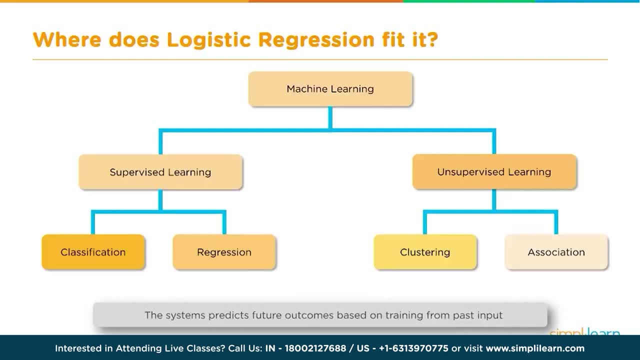 like clustering and association, and supervised learning uses techniques like classification and regression. now, supervised learning is used when you have labeled data- you have historical data, then you use supervised learning. when you don't have labeled data, then you used unsupervised learning. it's it's supervised learning. there are two types of techniques that are used: classification, 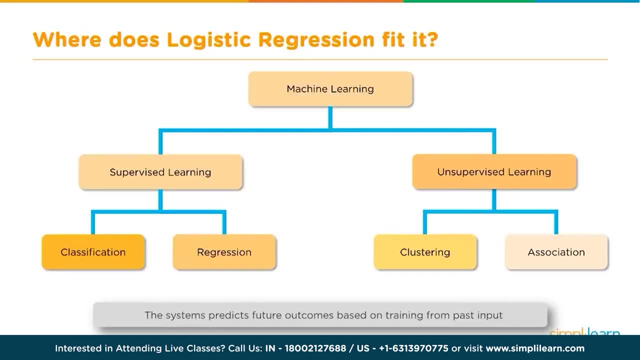 and regression based on what is the kind of problem we are solving. let's say we want to take the data and classify it. it could be binary classification like a zero or a one. an example of classification: we have just seen whether the passenger has survived or not survived- like a zero or one. that 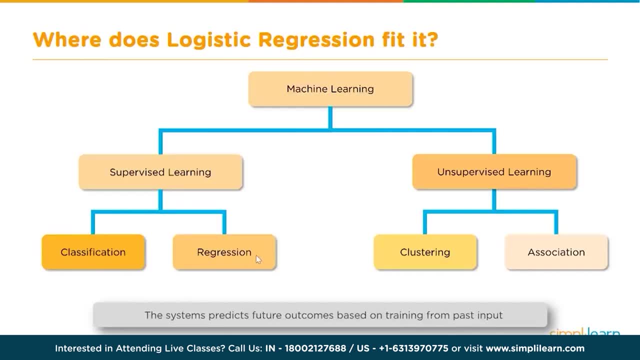 is known as binary classification. regression, on the other hand, is you need to predict a value, what is known as a continuous value. classification is for discrete values. regression is for continuous values. let's say you want to predict a share price or you want to predict the temperature that will be. 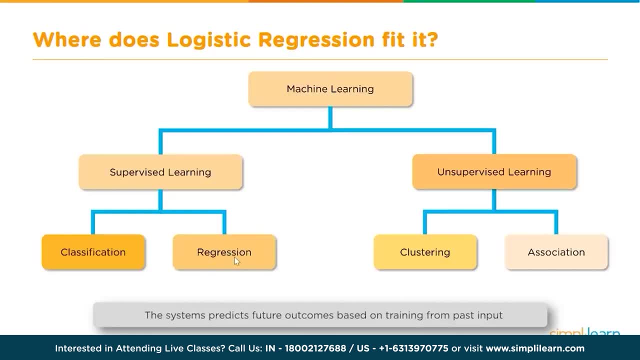 there. what will be the temperature tomorrow? that is where you use regression, whereas classification are discrete values- is: will customer buy the product or will not buy the product? will you get a promotion or you will not get a promotion? I hope you're getting the idea, or it could be multi-class classification as well. let's 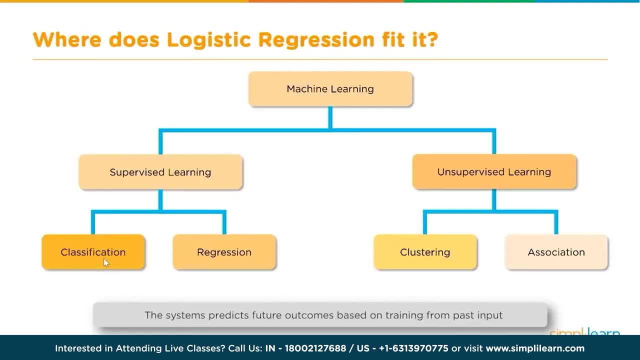 say you want to build an image classification model. so the image classification model would take an image as an input and classify into multiple classes whether this image is of a cat or a dog or an elephant or a tiger. so there are multiple classes, so not necessarily binary. 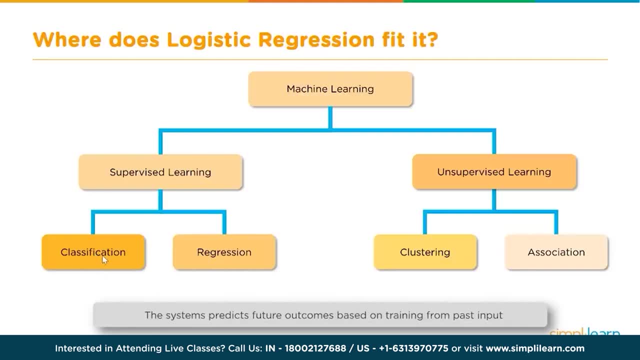 classification is known as a multi-class classification. so we are going to focus on classification, because logistic regression is one of the algorithms used for classification. now, the name may be a little confusing. in fact, whenever people come across logistic regression, it always causes confusion because the name has regression in it, but we are actually using this for performing classification. 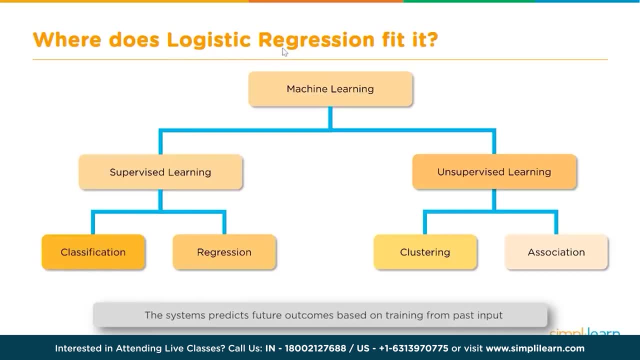 okay. so yes, it is logistic regression, but used for classification. And in case you are wondering, is there something similar for regression? Yes, For regression we have linear regression, Keep that in mind. So linear regression is used for regression, Logistic regression is used for classification. So in this video, we are going to focus on supervised learning and, within supervised learning, we are going to focus on classification and then, within classification, we are going to focus on logistic regression algorithm. 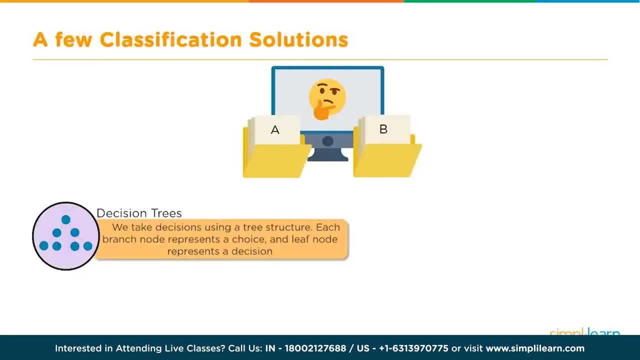 So, first of all, classification. So what are the various algorithms available for performing classification? The first one is decision tree. There are, of course, multiple algorithms, but here we will talk about a few. Decision trees are quite popular and very easy to understand, and therefore they are used for classification. Then we have k: nearest neighbors. This is another algorithm for performing classification. And then there is logistic regression, And this is what we are going to focus on in this video. 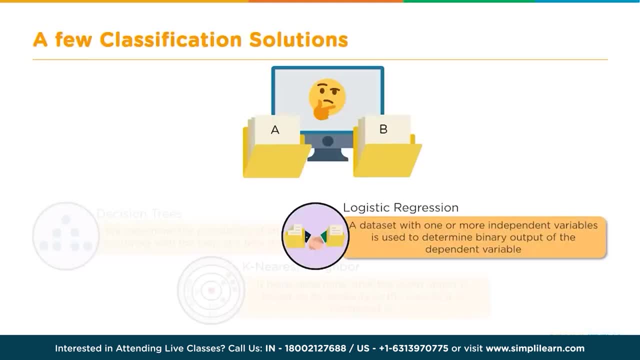 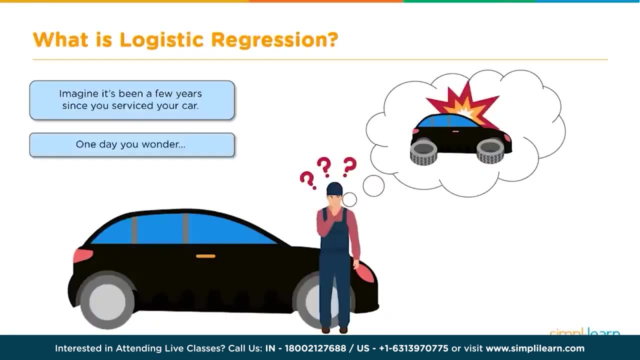 And we are going to go into a little bit of details about logistic regression. All right, What is logistic regression? As I mentioned earlier, logistic regression is an algorithm for performing binary classification. So let's take an example and see how this works. Let's say your car has not been serviced for quite a few years and now you want to find out if it is going to break down in the near future. So this is like a classification problem: Find out whether your car will break down or not. 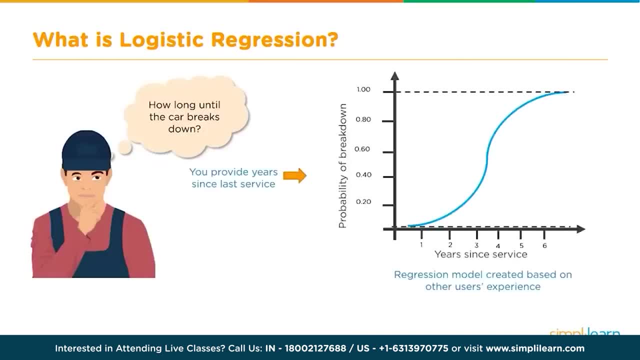 So how are we going to perform this classification? So here's how it looks: If we plot the information along the x and y axis, X is the number of years since the last service was performed and y is the probability of your car breaking down. And let's say, this information was, this data rather, was collected from several car users. It's not just your car, but several car users. So that is our labeled data. So the data has been collected. 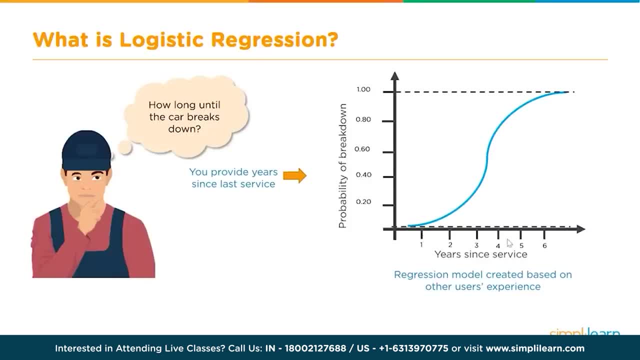 And for the number of years and when the car broke down and what was the probability, And that has been plotted along x and y axis. So this provides an idea. from this graph We can find out whether your car will break down or not. We'll see how. So, first of all, the probability can go from 0 to 1.. As you are aware, probability can be between 0 and 1. And, as we can imagine it is. 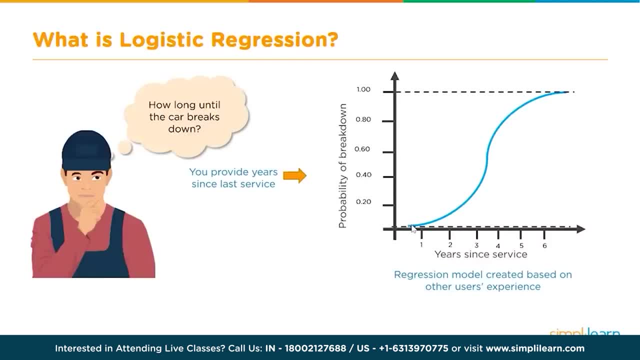 intuitive as well As the number of years are on the lower side. Maybe one year, two years or three years still after the service, The chances of your car breaking down are very limited. So, for example, chances of your car breaking down, The probability of your car breaking down within two years of your last service are 0.1 probability. Similarly, three years is maybe 0.3 and so on. But as the number of years increases, Let's say, if it was, 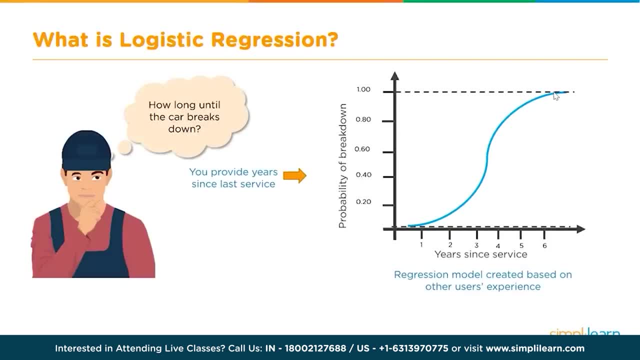 six or seven years, there is almost a certainty that your car is going to break down. That is what this graph shows. So this is an example of an application of the classification algorithm, And we will see in little details how exactly logistic regression is applied here. One more thing needs to be added here is that the dependent variables outcome is discrete. So if we are talking about whether the car is going to break down or not, So that is a discrete value. The white 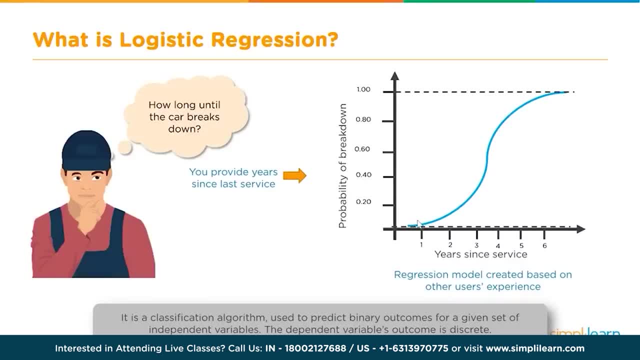 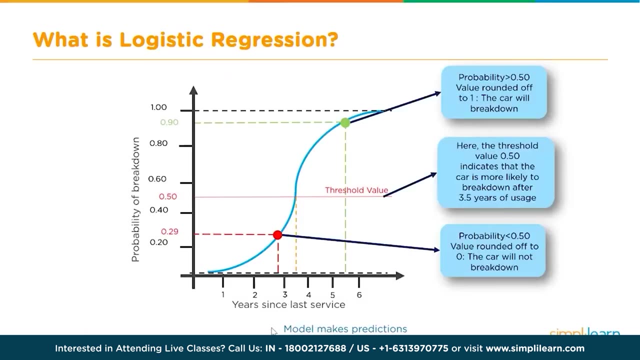 that we are talking about. the dependent variable that we are talking about. What we are looking at is whether the car is going to break down or not, Yes or no? That is what we are talking about. So here the outcome is discrete and not a continuous value. So this is how the logistic regression curve looks. Let me explain a little bit what exactly, how exactly we are going to determine the class outcome. rather So for a logistic regression curve, a threshold has to be. 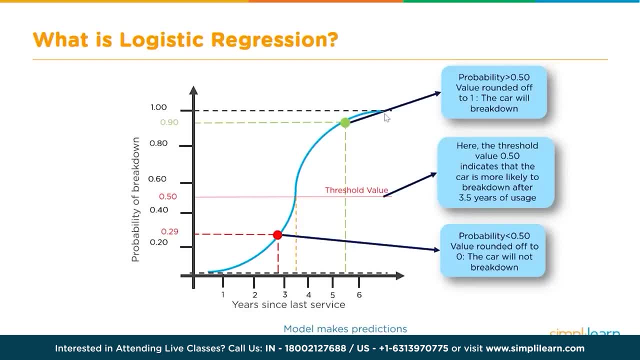 set saying that because this is a probability calculation- Remember, this is a probability calculation and the probability itself will not be 0 or 1.. But based on the probability we need to decide what the outcome should be. So there has to be a threshold, Like, for example, 0.5 can be the threshold, Let's say in this case: So any value of the probability below 0.5 is considered to be 0.. And any value above 0.5 is considered to be 0. 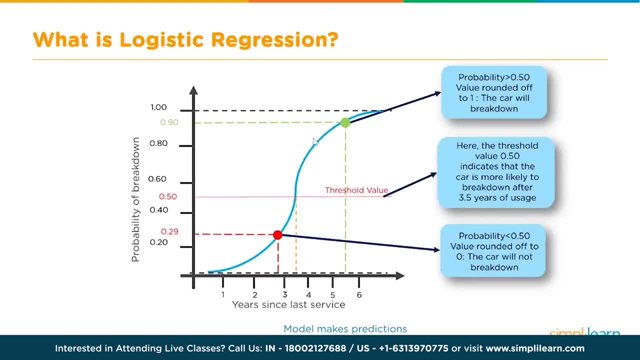 So an output of, let's say, 0.8 will mean that the car will break down. So that is considered as an output of 1.. And let's say an output of 0.2 is considered as 0, which means that the car will not bottom. 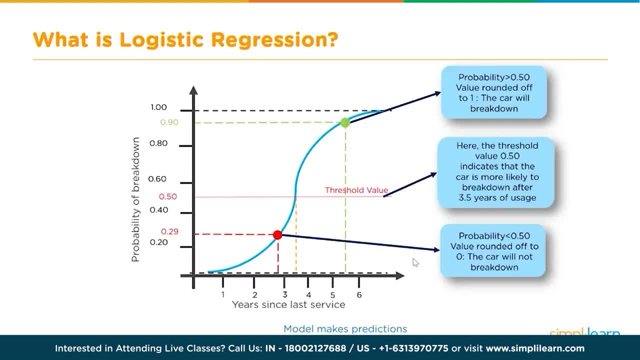 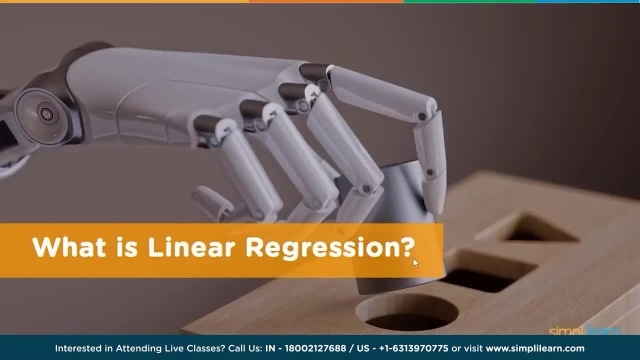 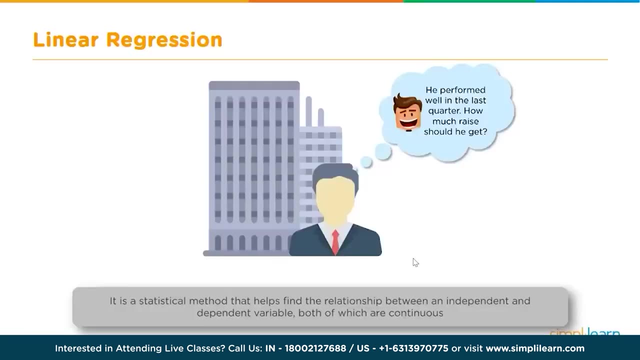 So that's the logistic regression works. Now let's do a quick comparison between logistic regression and linear regression, Because they both have the term regression in that, so that can cause confusion, So let us try to use it to remove that confusion. so what is linear regression? linear regression is a process. 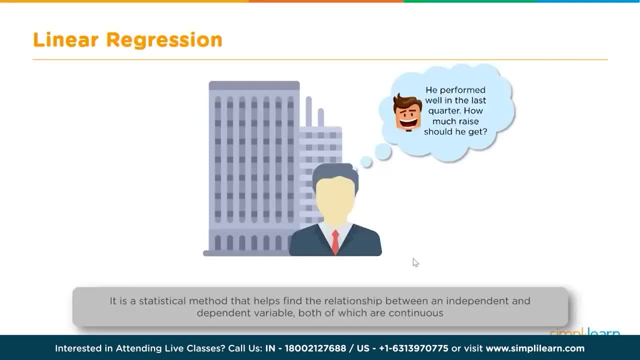 is once again an algorithm for supervised learning. however, here you're going to find a continuous value. you're going to determine a continuous value. it could be the price of a real estate property, it could be your hike- how much height you're going to get, or it could be a stock. 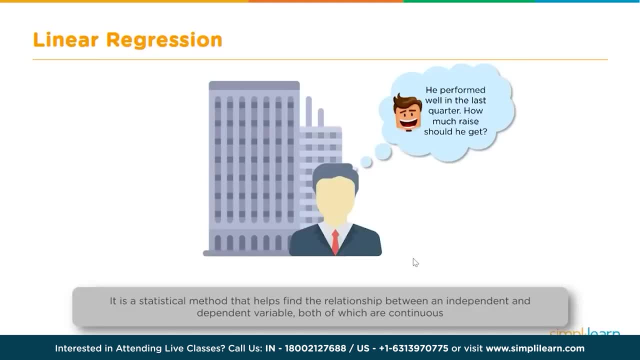 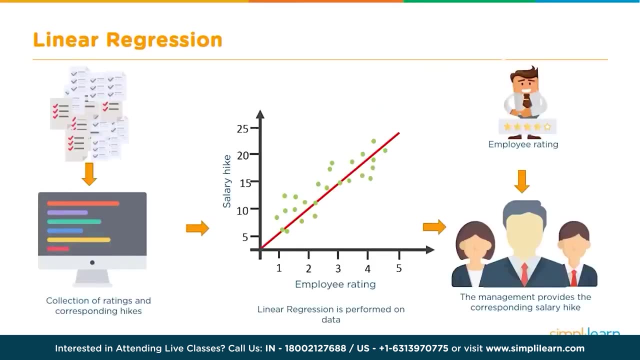 price. these are all continuous values. these are not discrete compared to a yes or a no kind of response that we are looking for in logistic regression. so this is one example of a linear regression. let's say the hr team of a company tries to find out what should be the salary hike. 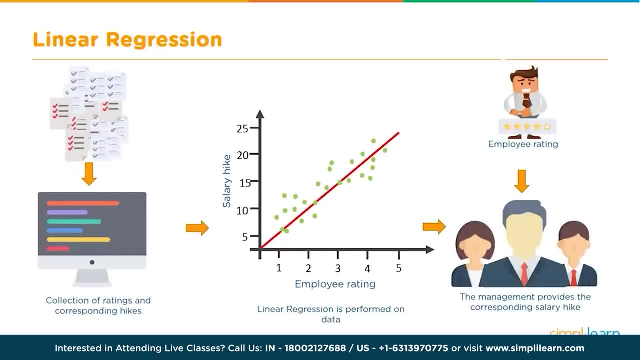 of an employee, so they collect all the details of their existing employees, their ratings and their salary hikes. what has been given, and that is the labeled information that is available, and the system learns from this, it is trained and it learns from this labeled information so that, when a new employees 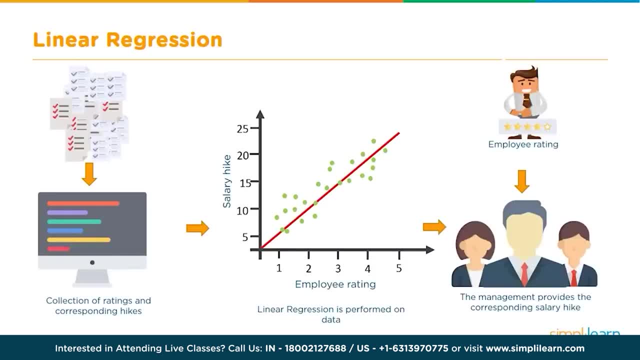 is fed. based on the rating, it will determine what should be the high. so this is a linear regression problem and a linear regression example. now, salary is a continuous value. you can get five thousand, five thousand, five hundred, five thousand, six hundred. it is not discrete, like a cat or a dog, or an apple or a 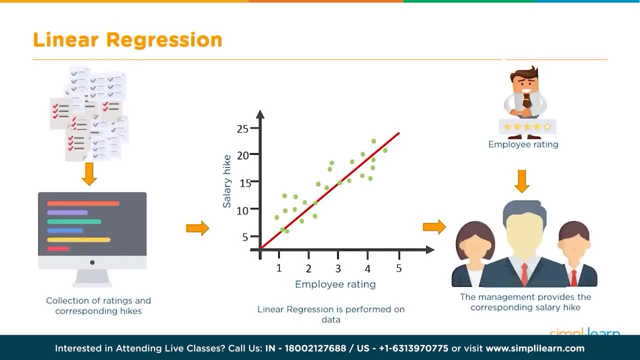 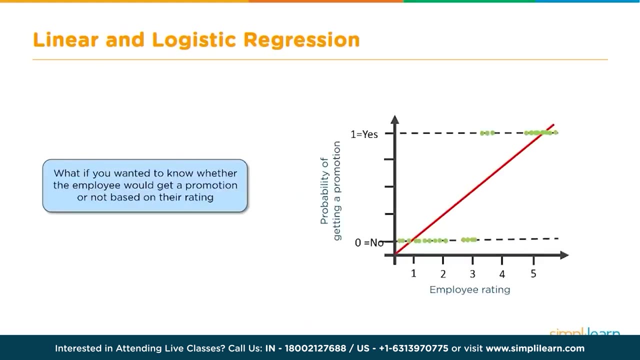 banana. these are discrete, or a yes or no, these are discrete values, right? so this way you're trying to find continuous values is where we use linear regression. so let's say, just to extend on this scenario, we now want to find out whether this employee is going to get a promotion or not. so we want to find out. 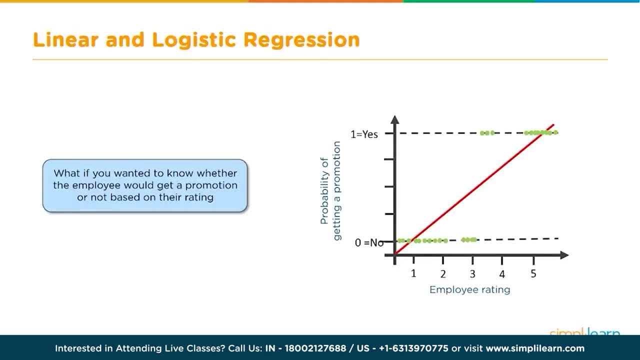 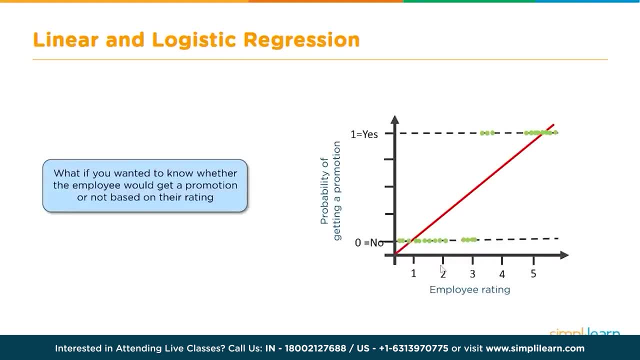 the employee rating. these are the ratings. and then some people got the promotion and this is the ratings for which people did not get promotion. that is a no and this is the rating for which people got promotion. we just plotted the data about whether a person has got an employers got promotion or not. yes, no. 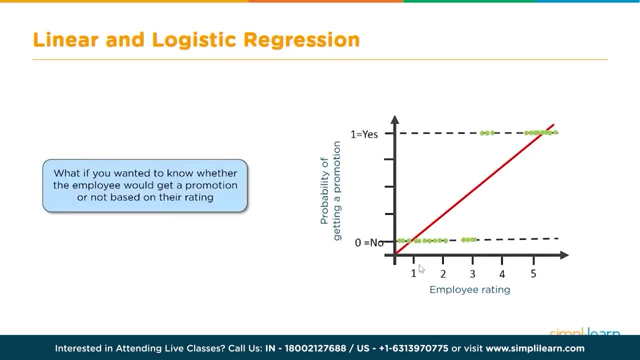 right, so there is nothing in between. and what is the employees rating? okay, and ratings can be continuous. that is not. but the output is discrete in this case, whether employee got promotion or not. so this is the ratings for which people get promotion: yes, no, okay. so if we try to plot that and we try to find a 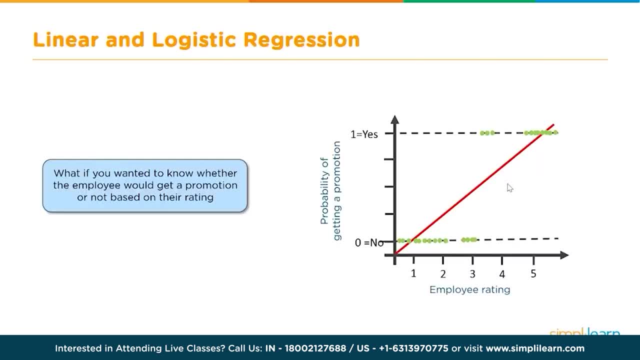 straight line. this is how it would look and, as you can see, doesn't look very right because looks like there will be a lot of errors. this root mean square error, if you remember, for linear regression would be very, very high, and also the the values cannot go beyond zero or beyond one, so the graph should 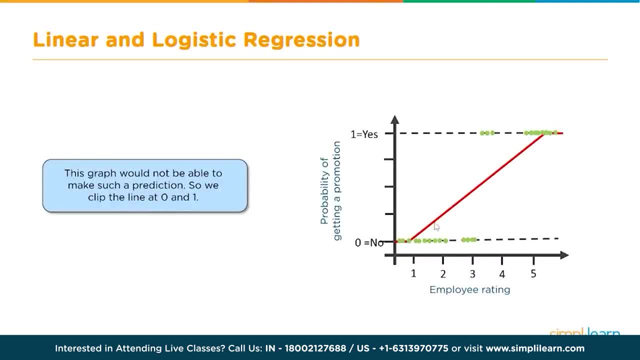 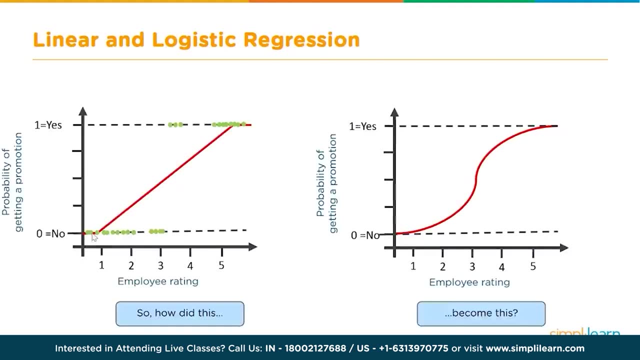 probably look somewhat like this: clicked at zero and one, but still the straight line doesn't look right. therefore it's refusing a linear equation. we need to come up with something different and therefore the logistic regression model looks somewhat like this: so we calculate the probability and if we thought that probability not in the form of a straight? 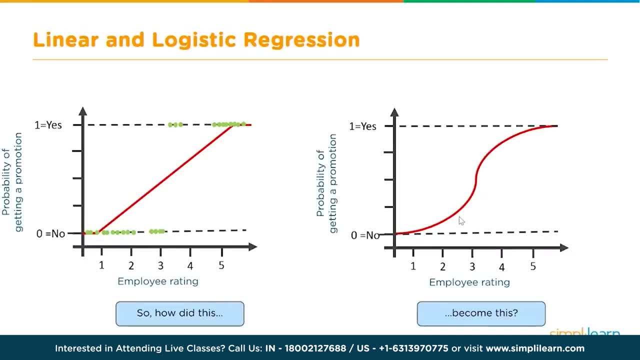 line, but we need to use some other equation. we will see very soon what the equation is then. it is a gradual process, right? so you see here, people, that some of these ratings are not any promotions, and then slowly, at certain rating, they get promotion. so that is a gradual process. 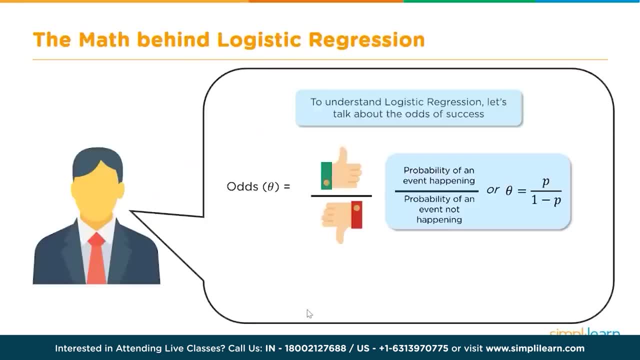 and this is how the math behind logistic regression looks. so we are trying to find the odds for a particular event happening. and this is the formula for finding the odds. so the probability of an event happening divided by the probability of the event not happening, so p if it is the. 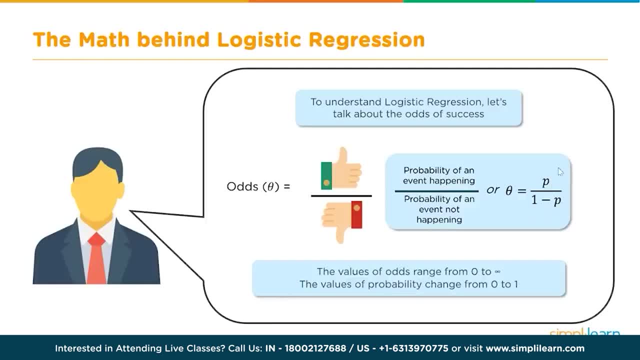 probability of the event happening, probability of the person getting a promotion, and divided by the probability of the person not getting a promotion, that is one minus p. so this is how you measure the odds. now, the values of the odds range from zero to infinity, so when this probability 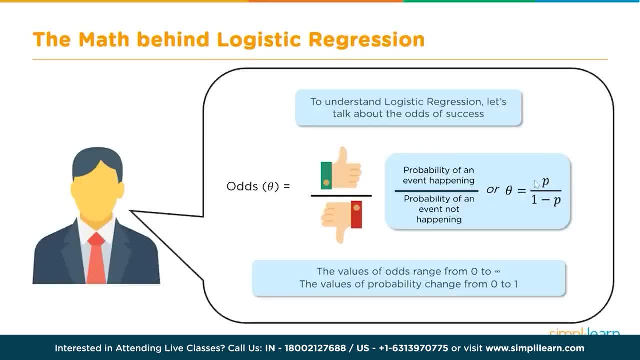 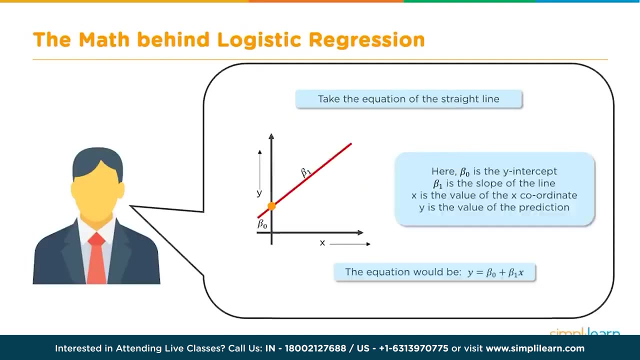 is zero, then the odds will. the value of the odds is equal to zero, and when the probability becomes one, then the value of the odds is one by zero. that is be infinity, but the probability itself remains between zero and one. now this is how an equation of a straight line looks. so y is equal to beta 0 plus beta 1 x, where beta 0 is the y intercept. 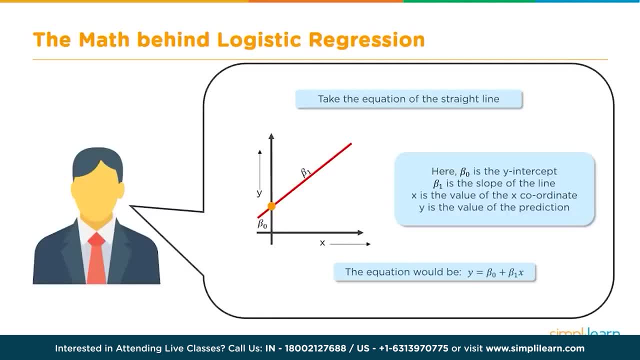 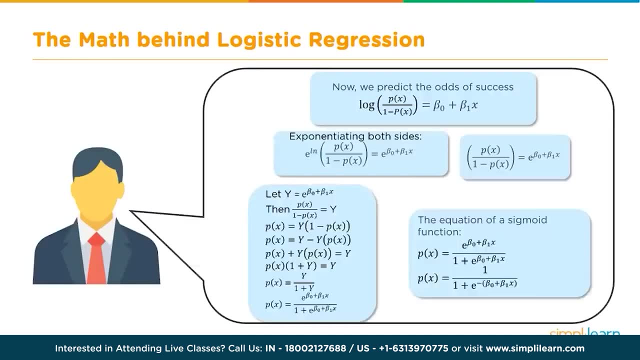 and beta 1 is the slope of the line. if we take the odds equation and take a log of both sides, then this would look somewhat like this, and the term logistic is actually derived from the fact that we are doing this. we take a log of px by 1 minus px. this is an extension of the calculation of. 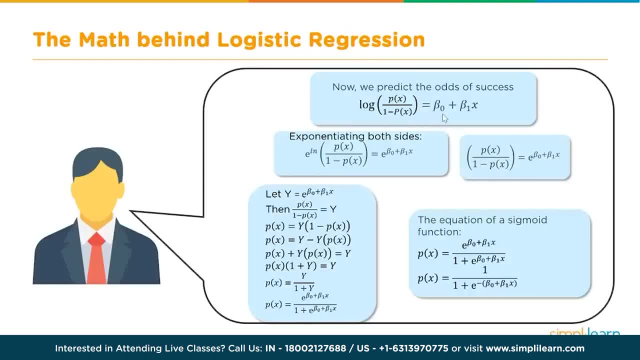 odds that we have seen right, and that is equal to beta 0 plus beta 1 x, which is the equation of the straight line. and now from here, if you want to find out the value of px, you will see we can take the exponential on both sides and then, if we solve that equation, we will get the. 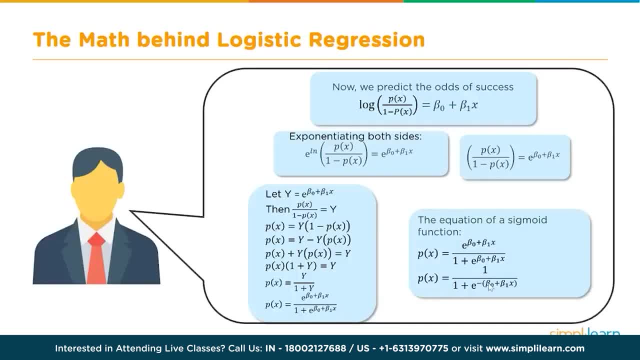 equation of px like this: px is equal to 1 by 1 plus e, to the power of 1 minus px, to the power of minus beta 0 plus beta 1 x. and recall, this is nothing but the equation of the line which is equal to y. y is equal to beta 0 plus beta 1 x, so that this is the equation also known. 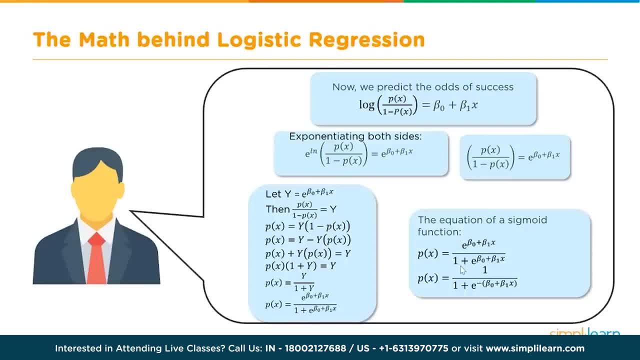 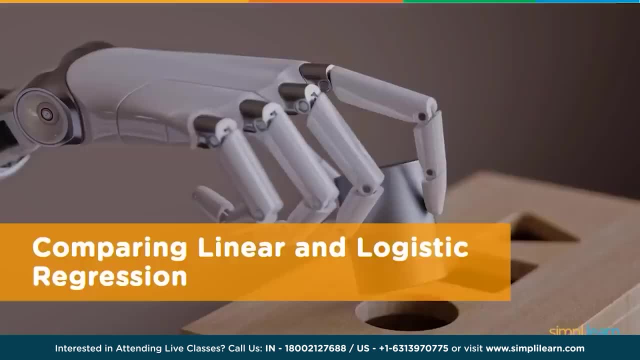 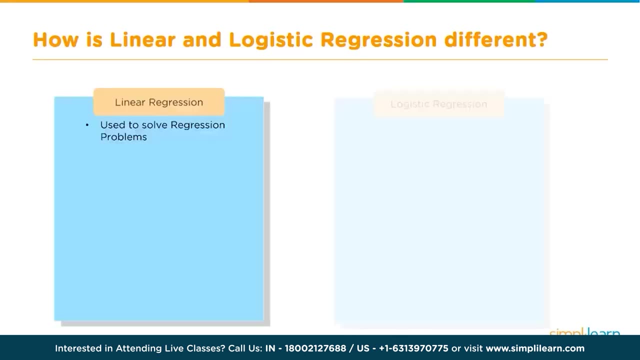 as the sigmoid function and this is the equation of the logistic regression. all right, and if this is plotted, this is how the sigmoid curve is obtained. so let's compare linear and logistic regression, how they are different from each other. let's go back. so linear regression is solved or used to solve regression problems, and logistic regression is. 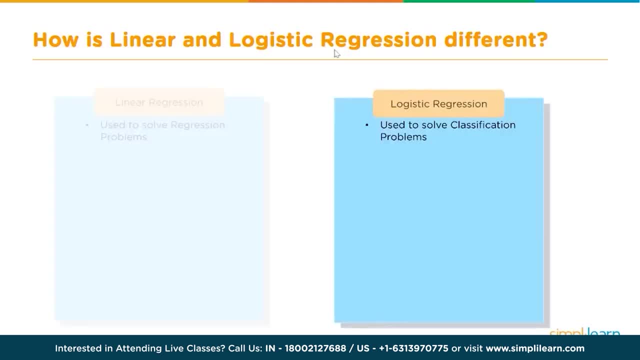 used to solve classification problems, so both are called regression. but linear regression is used for solving regression problems where we predict continuous values, whereas logistic regression is used for solving classification problems where we have had to predict discrete values. the response variables in case of linear regression are continuous in nature. 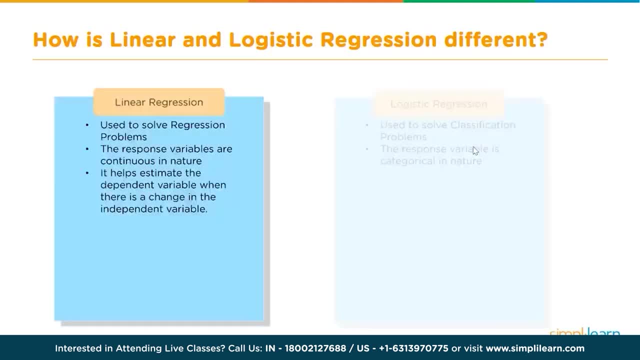 whereas here they are categorical or discrete in nature, and linear regression helps to estimate the dependent variable when there is a change in the independent variable, whereas here, in case of logistic regression, it helps to calculate the probability or the possibility of a particular event happening, and linear regression, as the name suggests, is a straight line. that's why it's called. 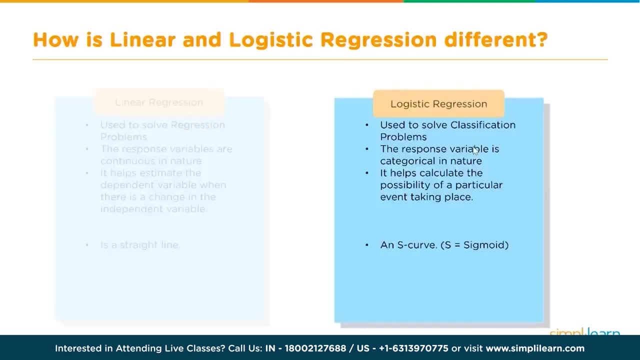 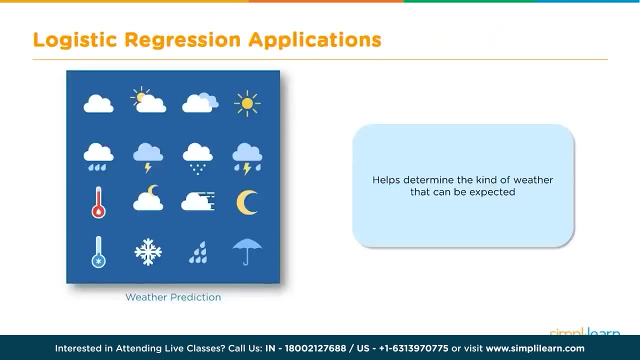 linear regression, whereas logistic regression is a sigmoid function and the curve is. the shape of the curve is s, it's an s-shaped curve. this is another example of application of logistic regression in weather prediction- that it's going to rain or not rain. now, keep in mind both are used. 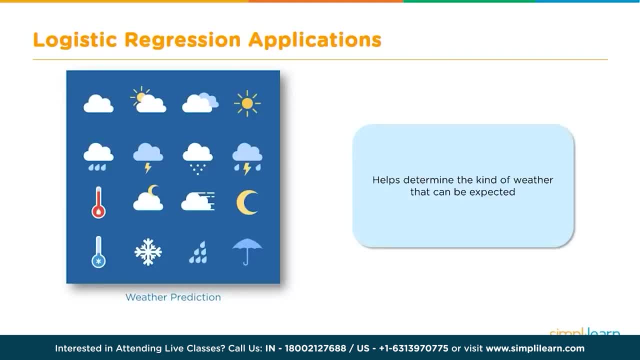 in weather prediction. if we want to find the discrete values, like whether it's going to rain or not rain- that is a classification problem- we use logistic regression. but if we want to determine what is going to be the temperature tomorrow, then we use linear regression. so just keep in mind that. 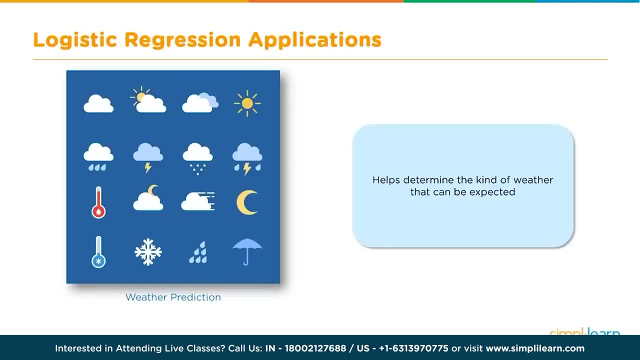 in weather prediction we actually use both. but these are some examples of logistic regression. so we want to find out whether it's going to rain or not, it's going to be sunny or not, it's going to snow or not. these are all logistic regression examples. a few more examples: classification of 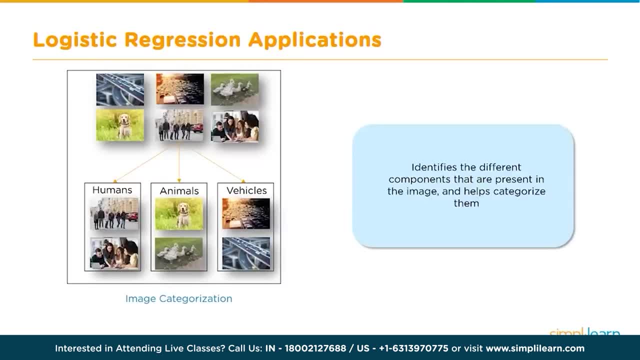 objects. this is a again another example of logistic regression now here. of course, one distinction is that these are multi-class classification, so logistic regression is not used in the original form, but it is used in a slightly different form. so we say: whether it is a dog or not. 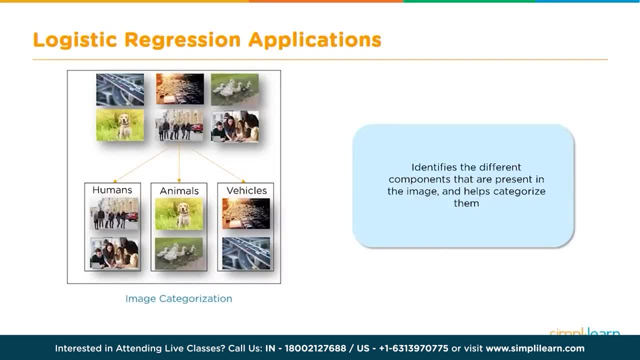 a dog. i hope you understand. so instead of saying is it a dog or a cat or elephant, we convert this into saying so, because we need to keep it to binary classification. so we say: is it a dog or not a dog, is it a cat or not a cat? so that's the way logistic regression can be used for. 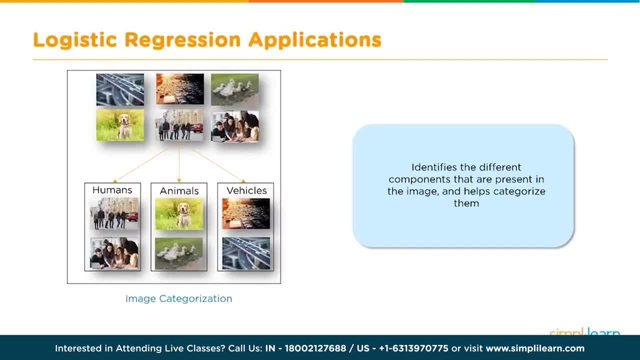 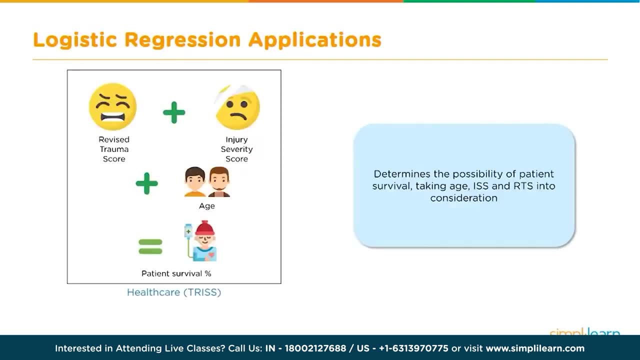 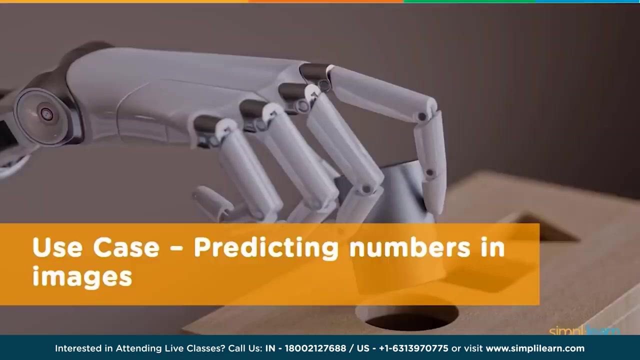 classifying objects. otherwise, there are other techniques which can be used for classification. in healthcare, logistic regression is used to find the survival rate of a patient. so they take multiple parameters like trauma score and age and so on and so forth, and they try to predict the rate of survival. all right now, finally, let's take an example and see how we can apply. 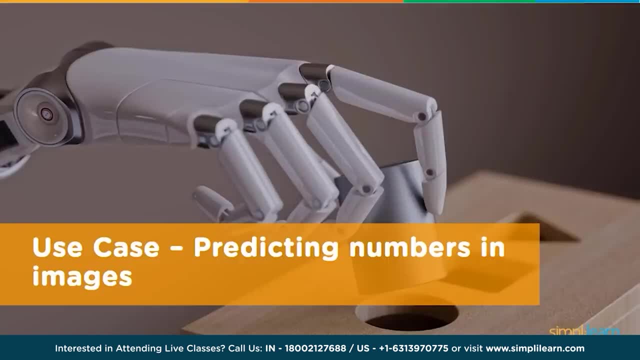 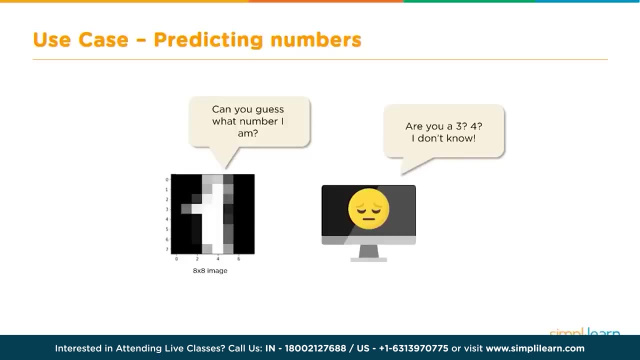 logistic regression to predict the number that is shown in the image. so this is actually a live demo. i will take you into jupiter notebook and, uh, show the code. but before that let me take you through a couple of slides to explain what we are trying to do. so let's say you have an 8x8 image and there the image has a number. 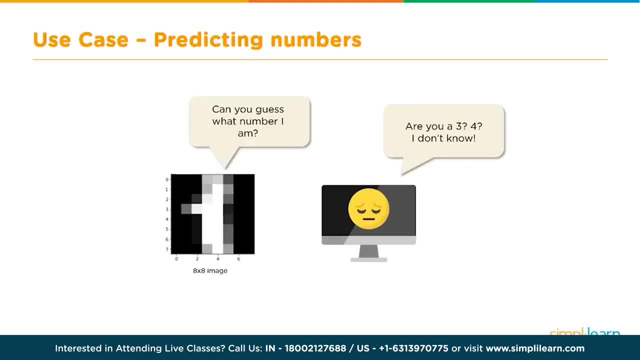 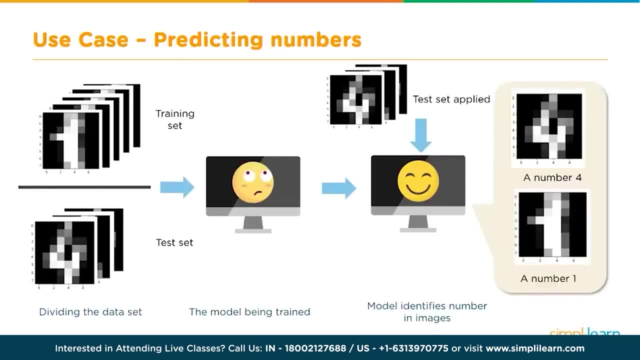 one, two, three, four, and you need to train your model to predict what this number is. so how do we do this? so the first thing is, obviously, in any machine learning process, you train your model. so in this case, we are using logistic regression, so, and then we provide a training set to train the 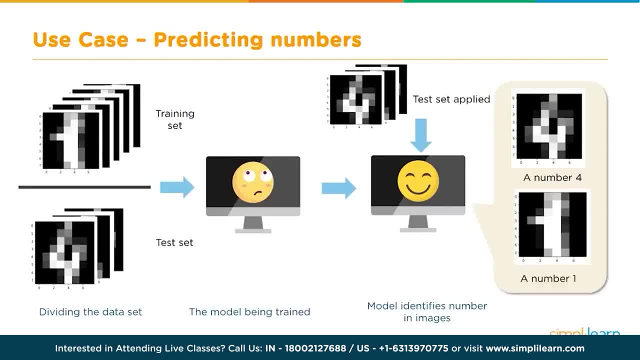 model and then we test how accurate our model is with the test data, which means that, like any machine learning process, we split our initial data into two parts: training set and test set. with the training set, we train our model and then, with the test set, we test the model till we get. 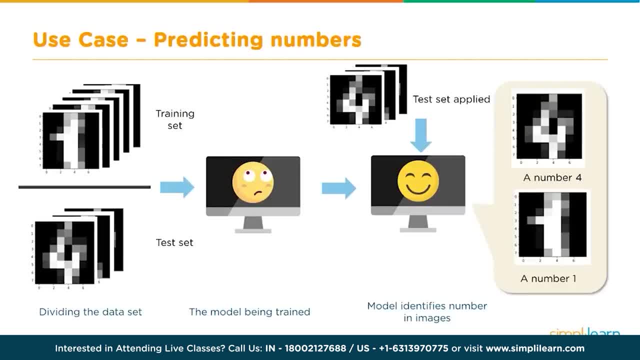 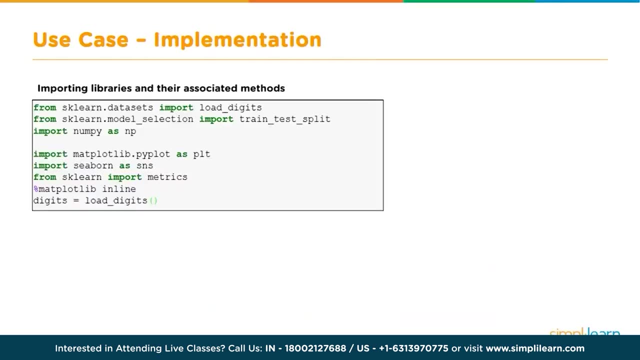 good accuracy and then we use it for for inference, right? so that is typical methodology of training, testing and then deploying of machine learning modules. so let's uh, take a look at the code and see what we are doing. so i will not go line by line, but just take you through. 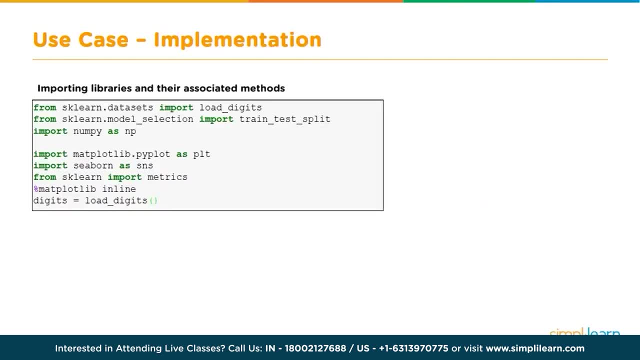 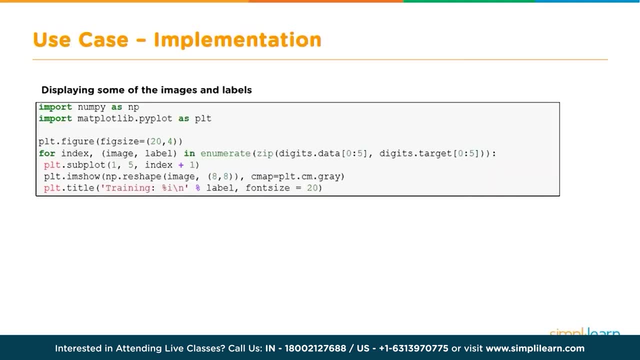 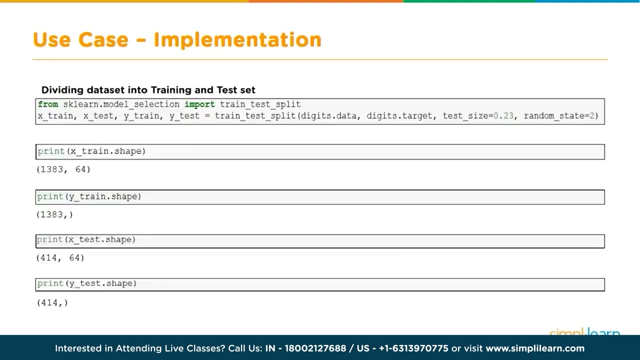 some of the blocks. so first thing we do is import all the libraries and then we basically take a look at the images and see what is the total number of images we can display using matplotlib- some of the images are a sample of these images, and then we split the data into training and 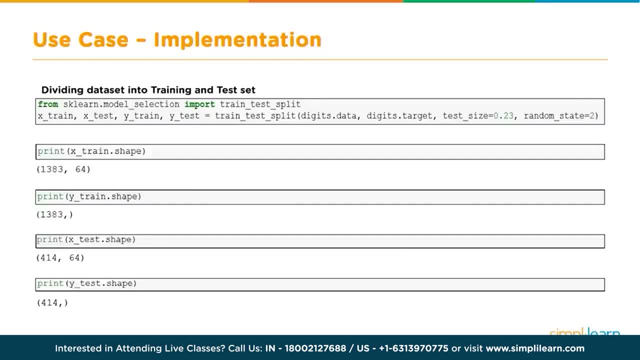 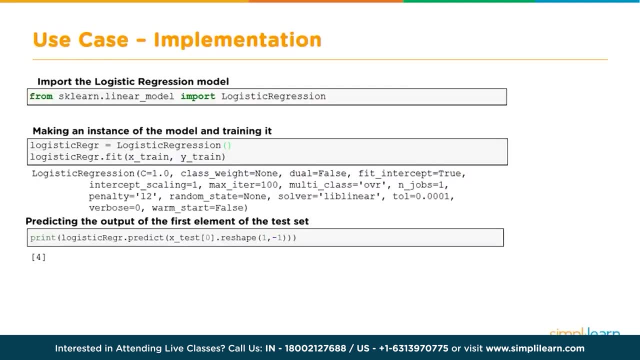 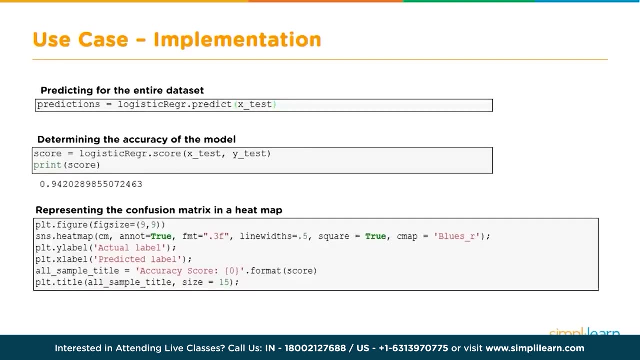 test, as i mentioned earlier, and we can do some exploratory analysis, and then we build our model, we train our model with the training set and then we test it with our test set and find out how accurate our model is using the confusion matrix, the heat map and use. 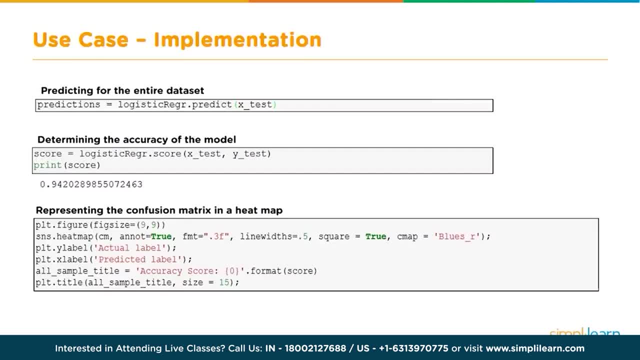 heatmap for visualizing this and i will show you in the code what exactly is the confusion matrix and how it can be used for finding the accuracy. in our example we got we get an accuracy of about 0.94, which is pretty good, or 94 percent, which is pretty good. 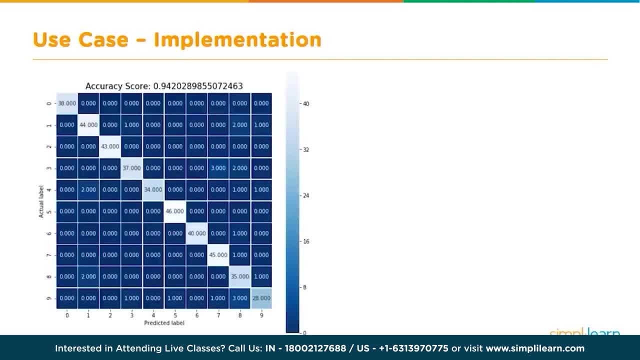 so what is the confusion matrix? this is an example of a confusion matrix, and this is used for identifying the accuracy of a classification model like a logistic regression model. so the most important part in a confusion matrix is that, first of all, this: as you can see, this is a matrix, and the size of the matrix depends on how many. 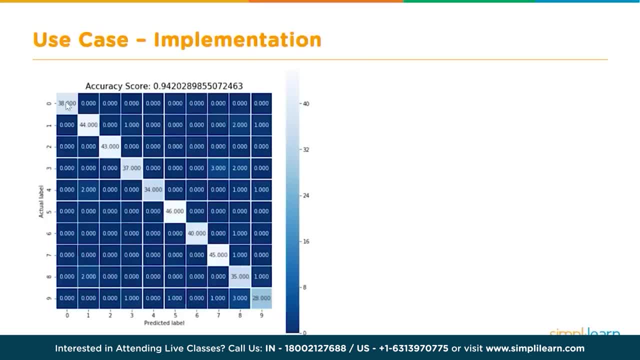 outputs we are expecting right. so the most important part here is that the model will be accurate when we have the maximum numbers in its diagonal, like in this case. that's why it has almost 93, 94 percent, because the diagonals should have the maximum numbers and the others other than. 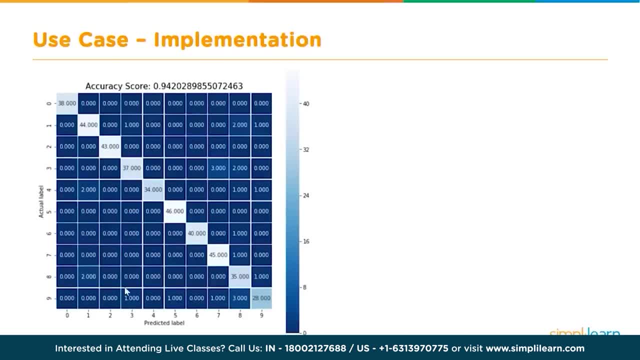 diagnose. the cells other than the diagonal should have very few numbers. so here that's what is happening. so there is a two here, there are, there's a one here, but most of them are along the diagonal this. what does this mean? this means that the number that has been fed is zero and the number that has been detected is also zero. 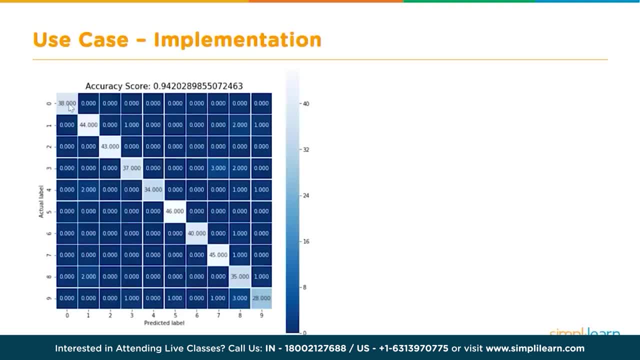 so the predicted value and the actual value are the same. so, along the diagonals, that is true, which means that, let's, let's take this diagonal right. if the maximum number is here, that means that, like here in this case, it is 34, which means that 34 of the images that have been fed, or? 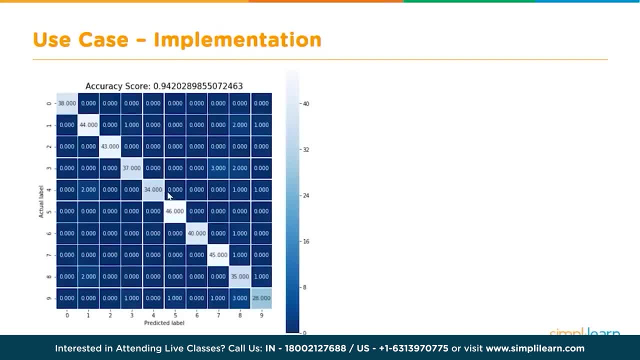 rather, actually there are two misclassifications in there. so 36 have been fed which have number four, and out of which 34 have been predicted correctly as number four and one has been predicted as number eight and another one has been predicted as number nine. so these are two misclassifications. okay, so that is the meaning of saying that the maximum number 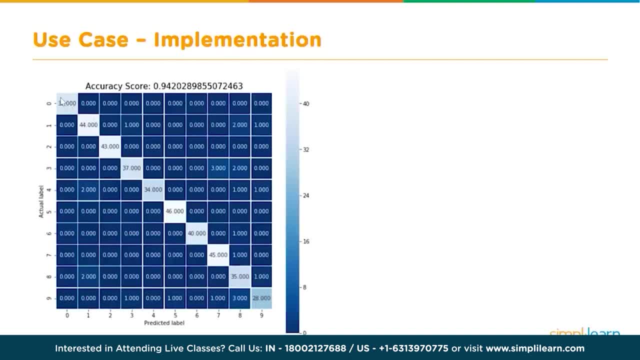 should be in the diagonal. so if you have all of them, so for an ideal model which has, let's say, hundred percent accuracy, everything will be only in the diagonal. there will be no numbers other than zero in all other cells. so that is like a hundred percent accurate model. okay, so that's. 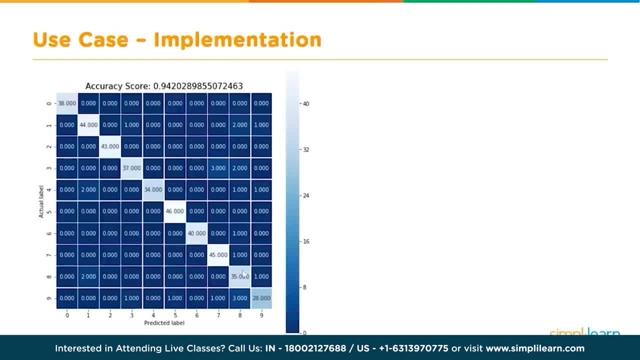 just of how to use this matrix. uh, how to use this, uh, confusion matrix. i know the name uh is a little funny sounding- confusion matrix, but actually it is not very confusing, it's very straightforward. so you are just plotting what has been predicted and what is the labeled information or what is. 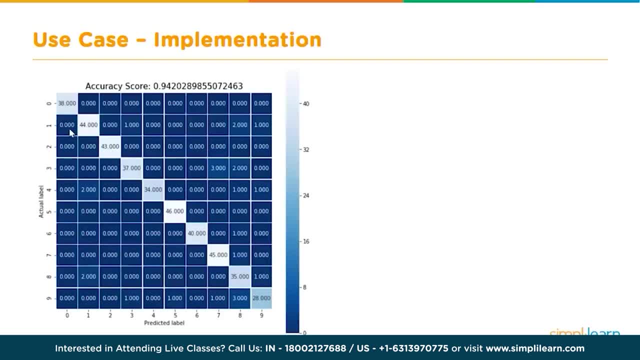 the actual data, that's also known as the ground truth sometimes, okay, these are some fancy terms. so predicted label and the actual name, that's all that is okay. yeah, so we are showing a little bit more information here. so 38 have been predicted, and here you will see that all of them have been. 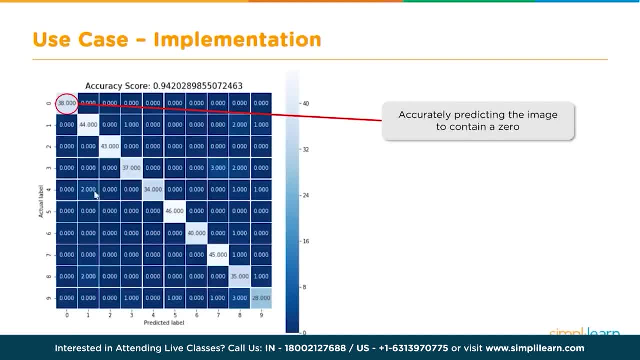 predicted correctly, there have been 38 zeros and the predicted value- and the actual value is- is exactly the same, whereas in this case- right it has. uh, there are i think 37 plus five. yeah, 42 have been fed the images. 42 images are of digit 3 and the accuracy is only 37 of them have been. 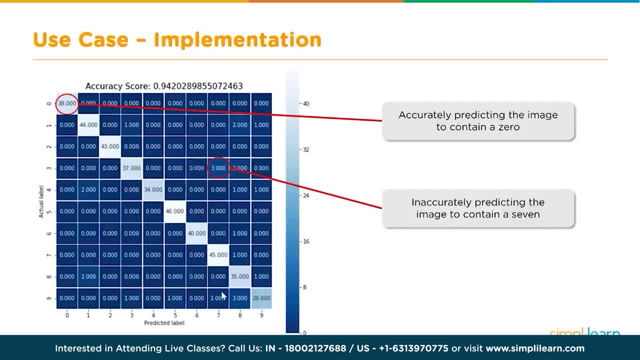 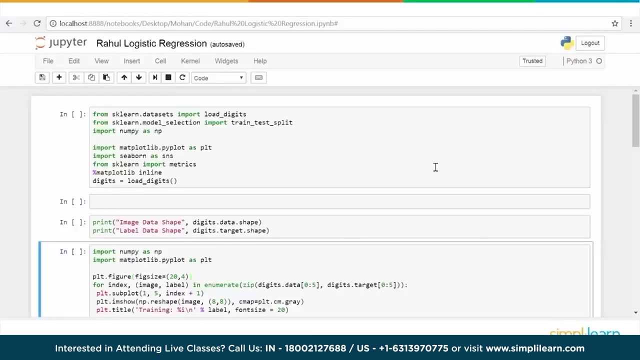 accurately predicted. three of them have been predicted as number seven, and two of them have been predicted as number eight, and so on and so forth. okay, all right. so with that, let's go into jupyter notebook and see how the code looks. so this is the code in in jupyter notebook. 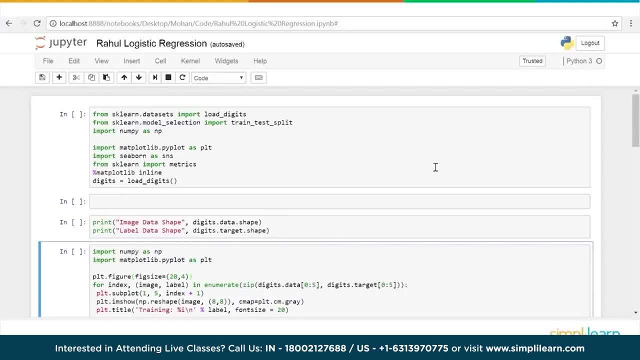 for logistic regression. in this demo, what we are going to do is train our model to recognize digits, which are the images which have digits from, let's say, 0 to 5 or 0 to 9, and and then we will see how well it is trained and whether it is able to predict these. 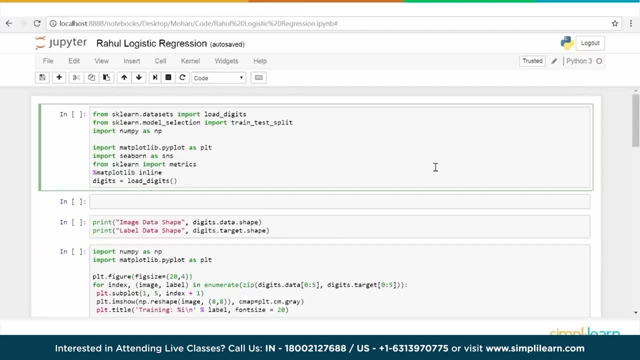 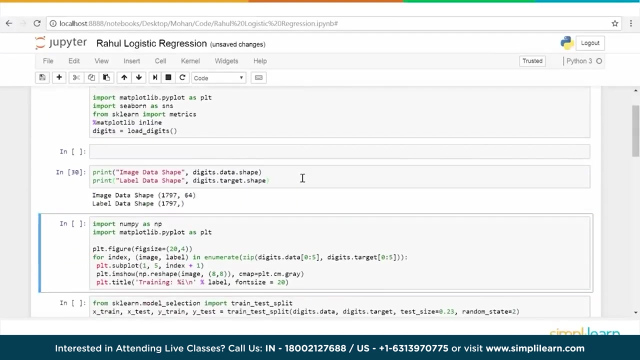 numbers correctly or not. so let's get started. so the first part is as usual. we are importing some libraries that are required, and then the last line and this block is to load the digits. so let's go ahead and run this code. then here we will visualize the shape of these digits so we can see here if we take a look, and 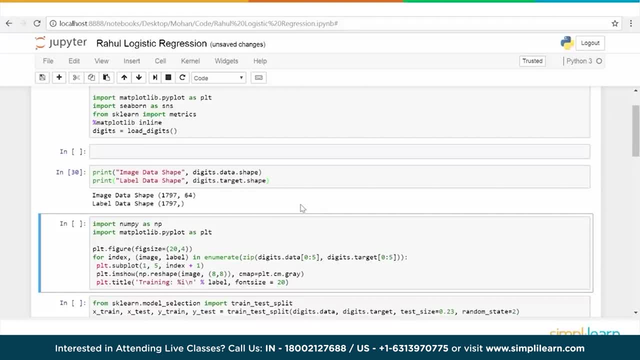 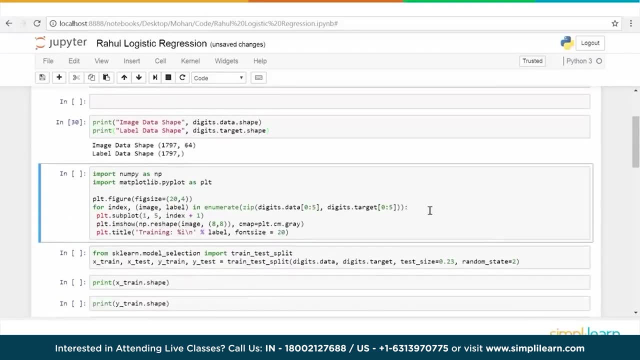 this is how the shape is: 1797 by 64. these are like 8 by 8 images. so that's that's what is reflected in this shape. now, from from here onwards, we are basically once again importing some of the libraries that are required, like numpy and matplot, and we will take a look at some of the sample. 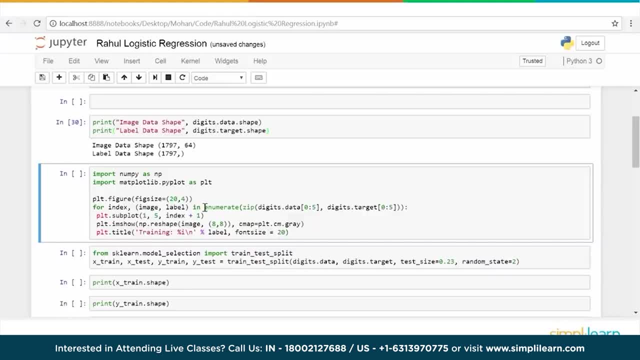 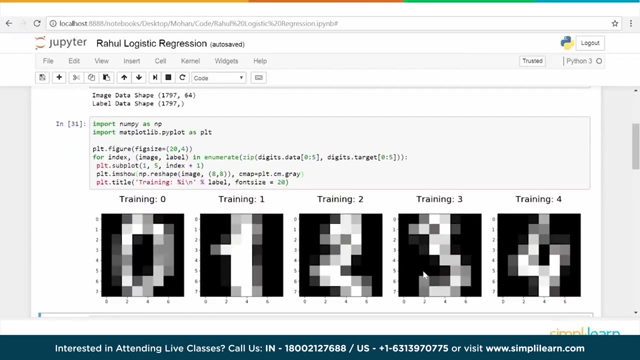 images that we have loaded. so this one, for example, creates a figure and then we go ahead and take a few sample images to see how they look. so let me run this code and so that it becomes easy to understand. so these are about five images, sample images that we are looking at. 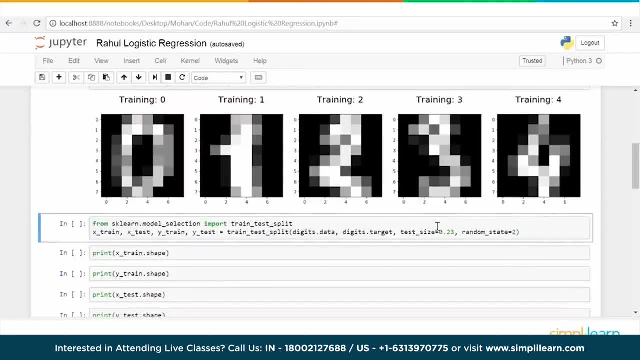 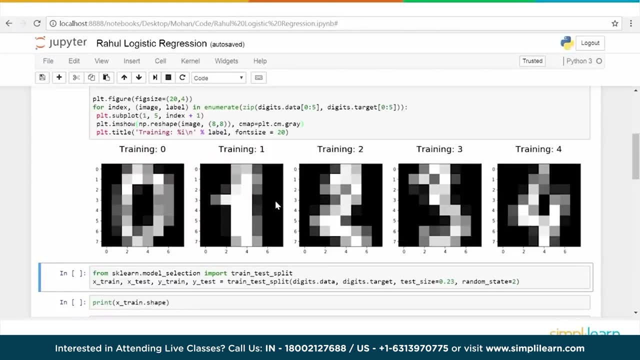 one, two, three, four. so this is how the image is, this is how the data is. okay, and based on this, we will actually train our logistic regression model and then we will test it and see how well it is able to recognize. so the way it works is: 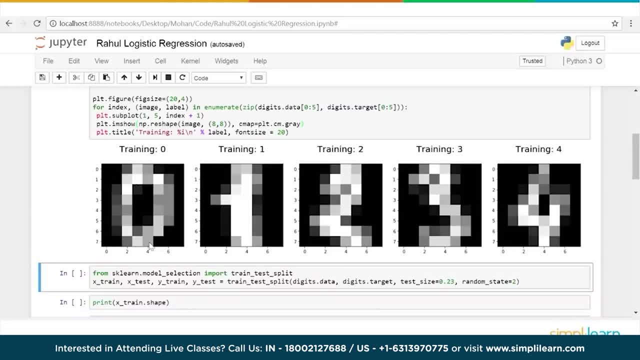 the pixel information. so, as you can see here, this is an eight by eight pixel kind of a image and the each pixel, whether it is activated or not activated, that is the information available for each pixel now, based on the pattern of this activation and non-activation. 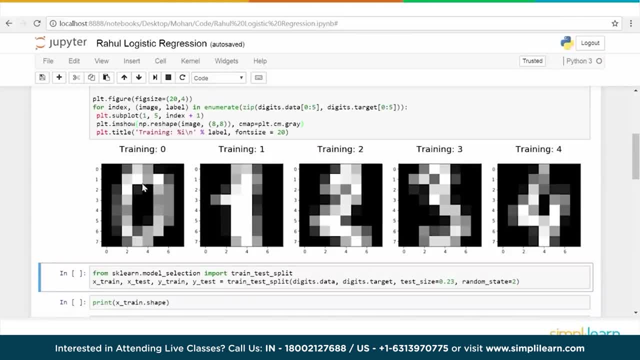 of the various pixels. this will be identified as a zero, for example, right, similarly as you can see. so, overall, each of these numbers actually has a different pattern of the pixel activation, and that's pretty much that our model needs to learn. for which a number, what is the pattern of the? 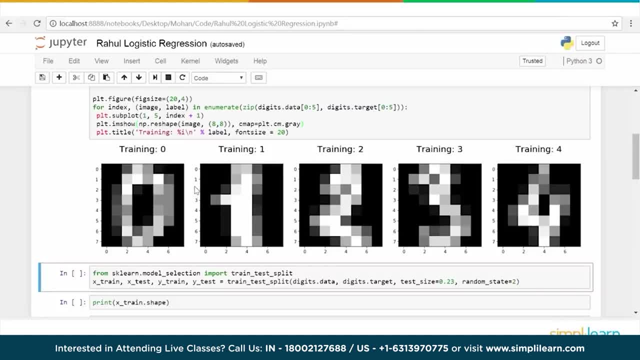 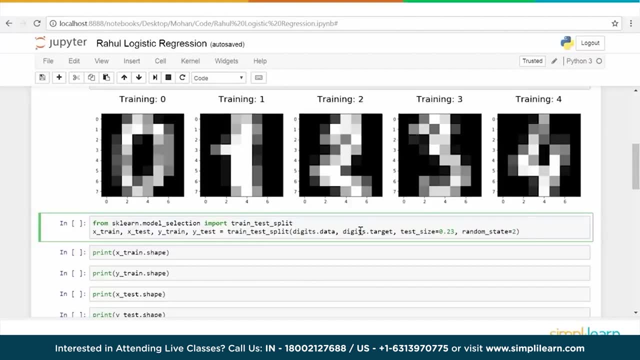 activation of the pixels. right, so that is what we are going to train our model. okay, so the first thing we need to do is to split our data into training and test data set, right? so whenever we perform any training, we split the data into training and tests so that the training data set is used to train the system. so we pass this. 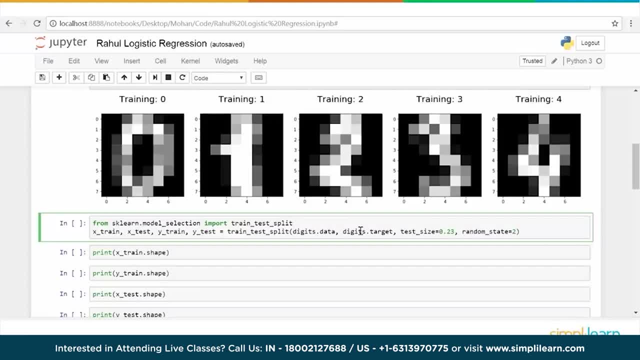 probably multiple times, and then we test it with the test data set and the split is usually in the form of there, and there are various ways in which we can split this data. it is up to the individual preferences. in our case here we are splitting in the form of 23 and 77. so when we say test size as 20.23, that means 23 percent of that entire data is. 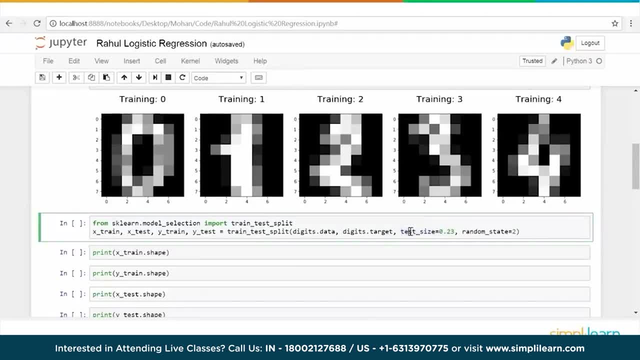 used for testing and the remaining 77 percent is used for training. so there is a readily available function which is uh called train test split. so we don't have to write any special code for the splitting. it will automatically split the data based on the proportion that we give here, which is test size. so we just give the test size automatically: training. 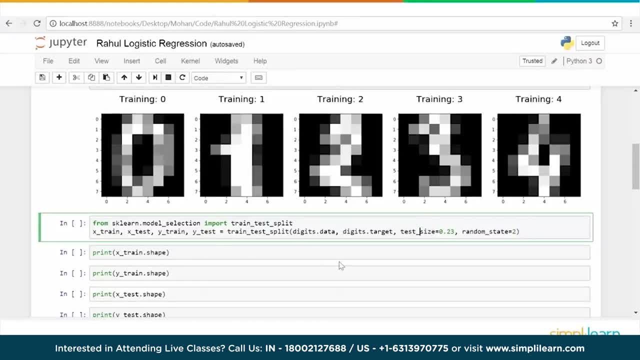 size will be determined and we pass the data that we want to split and the. the results will be stored in x underscore train and y underscore train for the training data set. and what is x underscore train? this are, these are the features, right, which is like the independent variable. 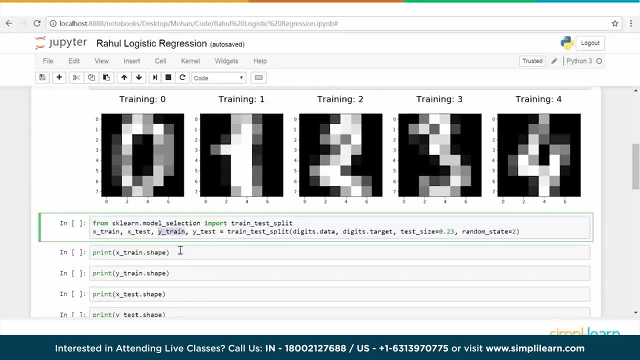 and y underscore train, is the label right. so in this case, what happens is we have the input value, which is, or the features value, which is in x underscore train, and since this is the labeled data for each of them, each of the observations, we already have the label information saying whether 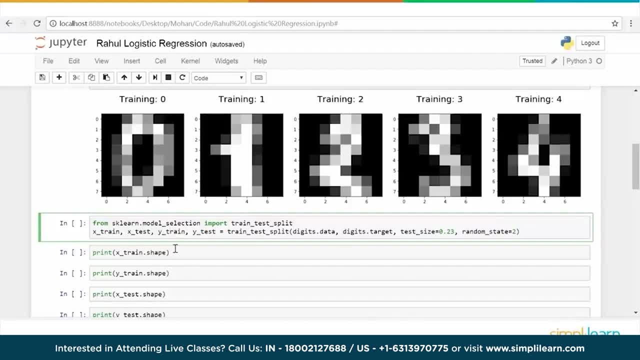 this digit is a zero or a one or a two, so that that's, this is what will be used for comparison to find out whether the the system is able to recognize this it correctly or there is an error. for each observation, it will compare with this right. so this is the label, so the 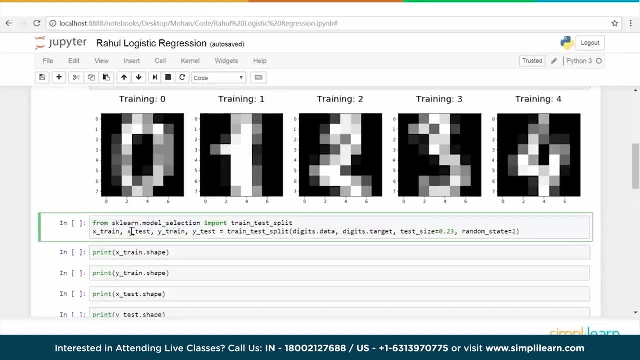 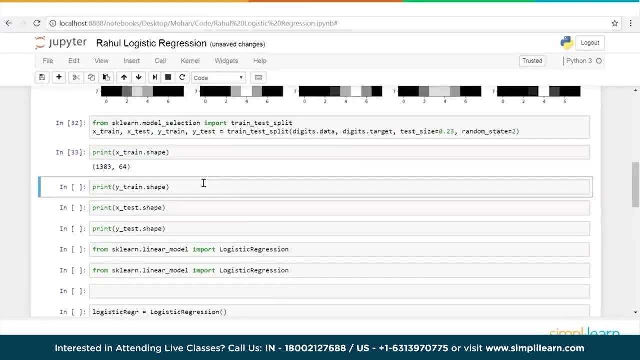 same way. x underscore train. y underscore train is for the training data set. x underscore test. y underscore test is for the test data set. okay, so let me go ahead and execute this code as well, and then we can go and check quickly what is the. how many entries are there and in each of this? so x. 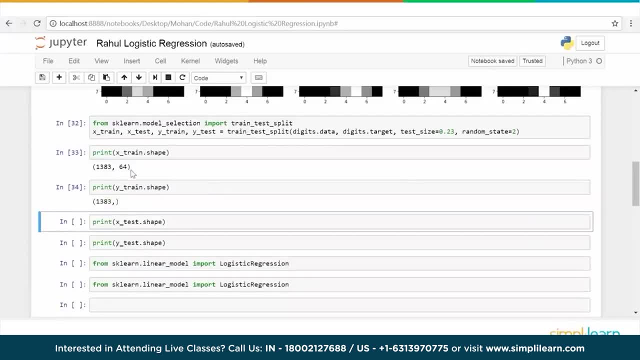 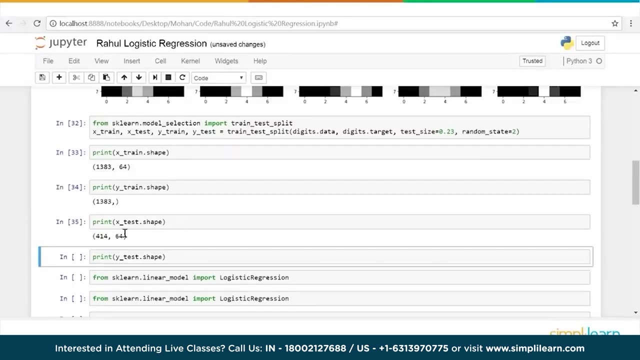 underscore train the shape is 13, 83 by 64 and y underscore train has 1383, because there is nothing like the second part is not required here. and then x underscore test shape we see is 414. so actually there are 414 observations in test and 1383. 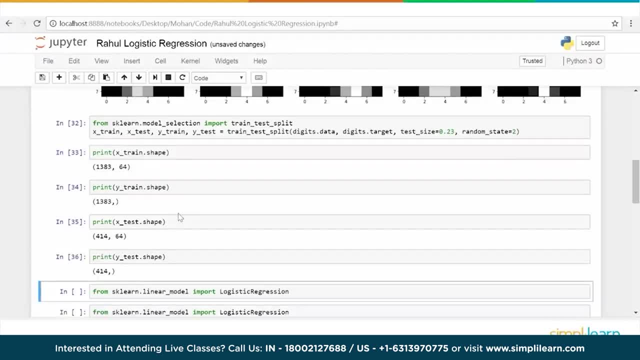 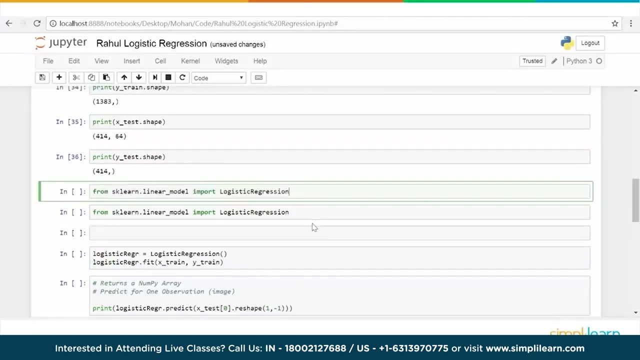 observations in train. so that's basically what these four lines of code are saying. okay, then we import the logistic regression library and which is a part of scikit-learn. so we we don't implement the logistic regression process itself, we just call these the function. and let me go ahead. 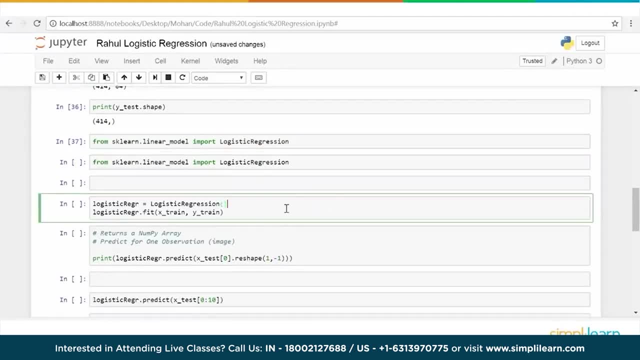 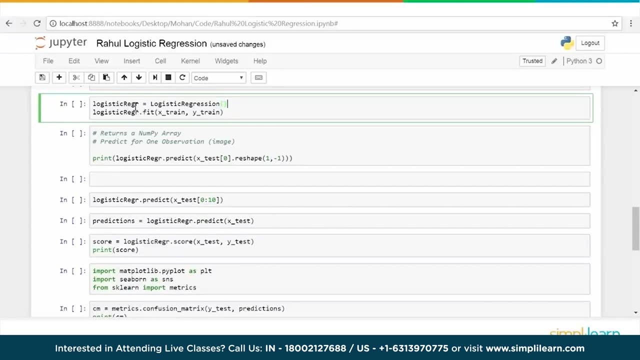 and execute that so that we have the logistic regression library imported. now we create an instance of logistic regression, right? so logistic regr is a is an instance of logistic regression, and then we use that for training our model. so let me first execute this code, so these two lines, so 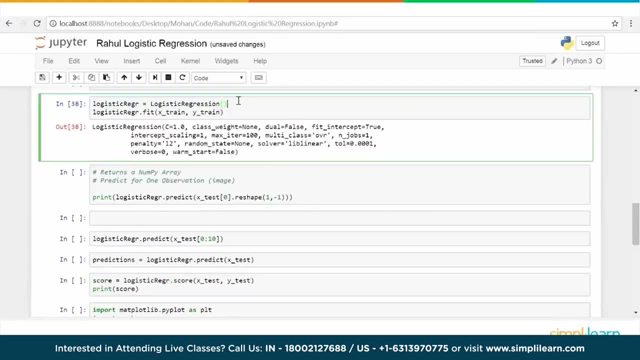 the first line basically creates an instance of logistic regression model, and then the second line way is where we are passing our data, the training data set, and this is our, the predictors, and this is our target. we are passing this data set to train our model. all right, so once we do this, in this case the data is not large, but by 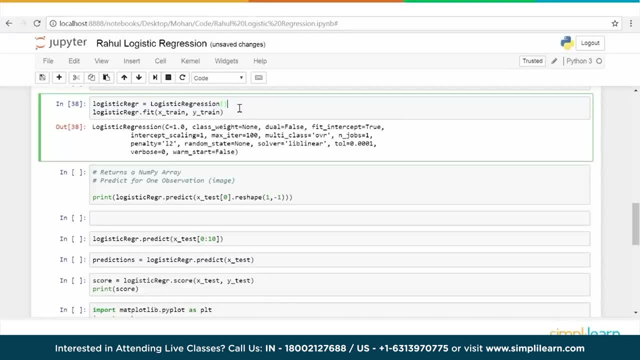 and large. the training is what takes usually a lot of time. so we spend in machine learning activities, in machine learning projects, we spend a lot of time for the training part of it. okay, so here the data set is relatively small, so it was pretty quick. so all right. so now our model has been trained using the training data set and 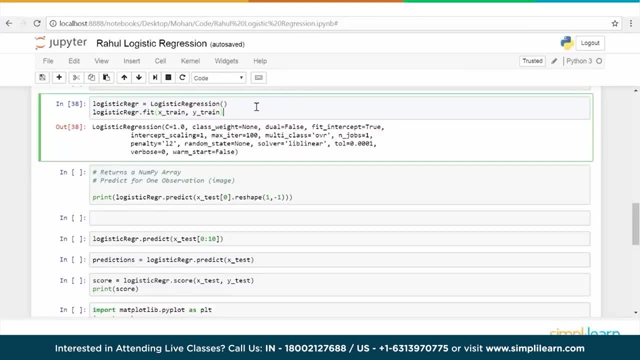 we want to see how accurate this is, so what we'll do is we will test it out in probably faces, so let me first try out how well this is working for one image. okay, I will just try it out with one image- my the first entry in my test data set- and see if it works or not. I will just try it out with one image- my the first entry in my test data set- and see if it works or not. 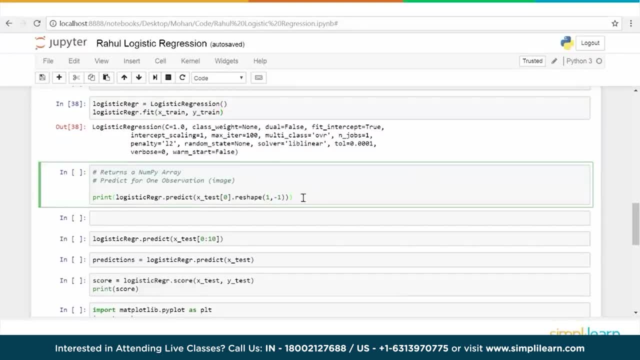 whether it is correctly predicting or not. so, and in order to test it, so for training purpose, we use the fit method. there is a method called fit, which is for training the model, and once the training is done, if you want to test for a particular value, new input- you use the predict. 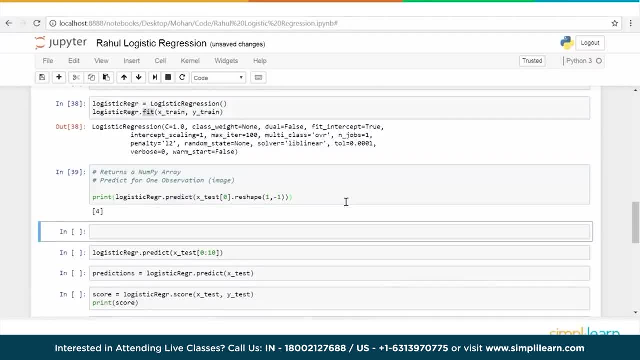 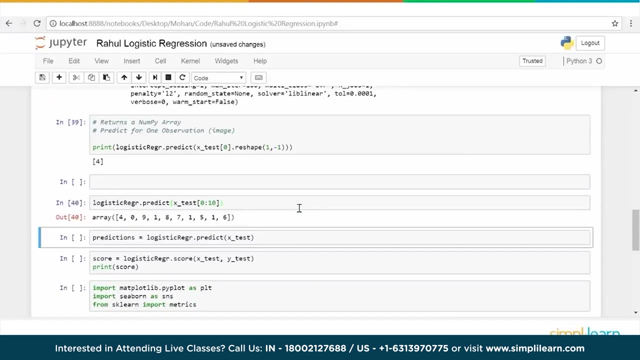 method. okay, so let's run the predict method and we pass this particular image and we see that the shape is, or if the prediction is four. so let's try a few more. let me see for the next 10. seems to be fine, so let me just go ahead and. 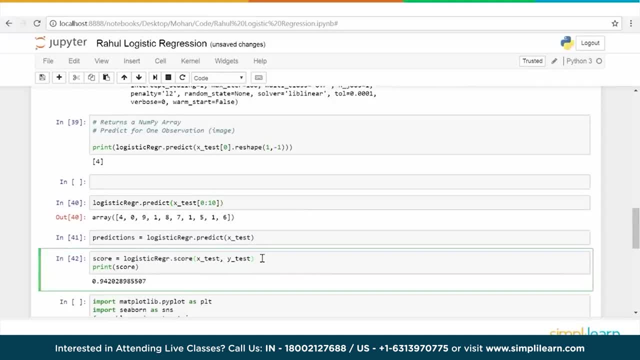 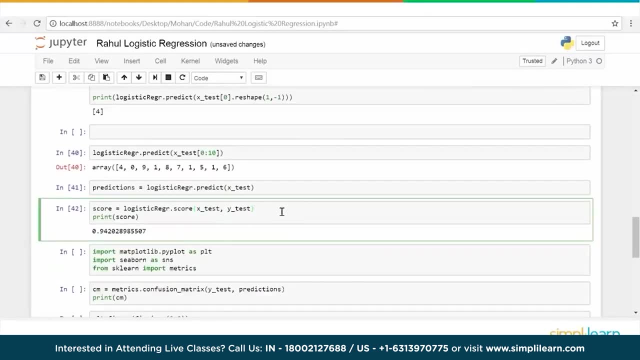 test the entire data set. okay, that's basically what we will do. so now we want to find out how accurately this has performed. so we use the score method to find what is the percentages of accuracy, and we see here that it has performed up to 94 accurate. okay, so that's, on this part, now, what we 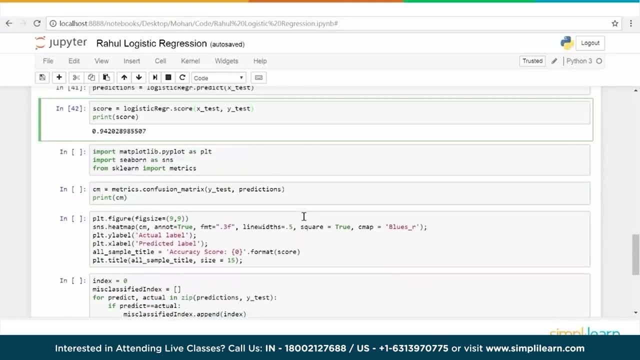 can also do is we can um also see this accuracy using what is known as a confusion Matrix. so let us go ahead and try that as well, so that we can also visualize how well this model has done. so let me execute this piece of code, which will basically import some of the libraries that are required, and we, we basically 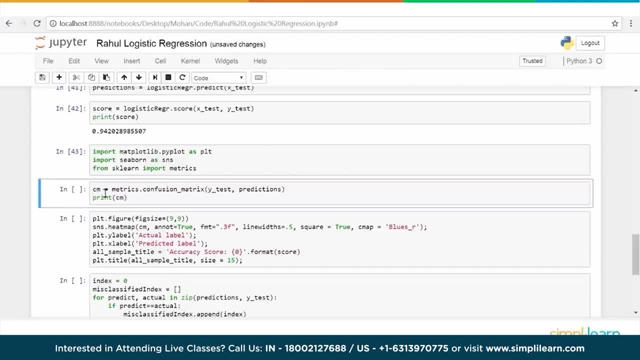 create a confusion Matrix, an instance of confusion Matrix, by running confusion Matrix and passing these values. so we have. so this confusion underscore Matrix method takes two parameters: one is the y underscore test and the other is the prediction. so what is the y underscore test? these are the labeled values which we already know for the test. data set and predictions are what the 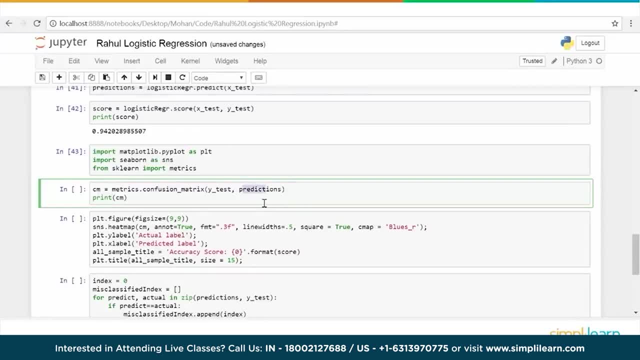 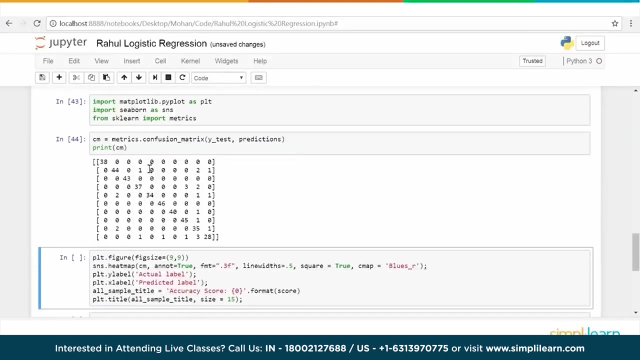 system has predicted for the test data set. okay, so this is known to us and this is what the system has that model has generated. so we kind of create the confusion Matrix and we will print it and this is how the confusion Matrix looks. as the name suggests, it is a Matrix and the key point out here is that 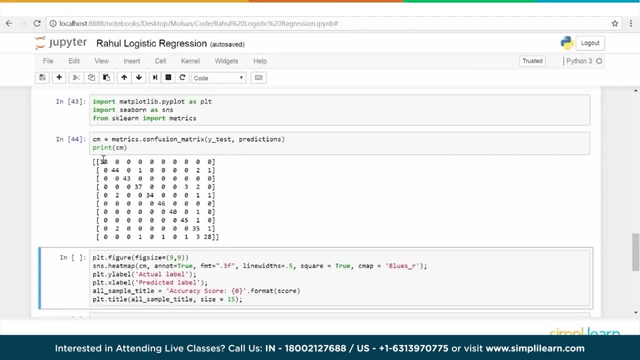 the accuracy of the model is determined by how many numbers are there in the diagonal. the more the numbers in the diagonal, the better. the accuracy is okay. and first of all, the total sum of all the numbers is equal to the number of observations in the test data set. that is the first thing, right? so 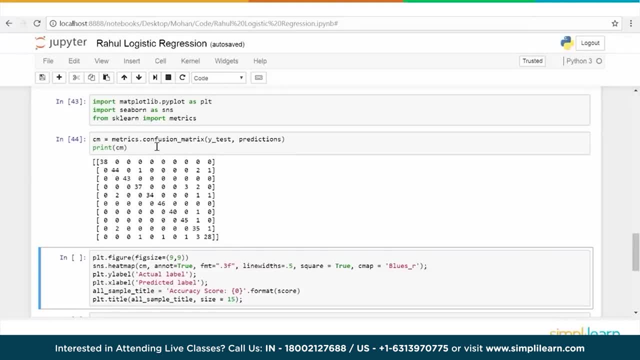 if you add up all these numbers that will be equal to the number of observations in the test data set, and then out of that the maximum number of them should be in the diagonal. that means the accuracy is pretty good if the the numbers in the diagonal are less, and in all other places there are a lot. 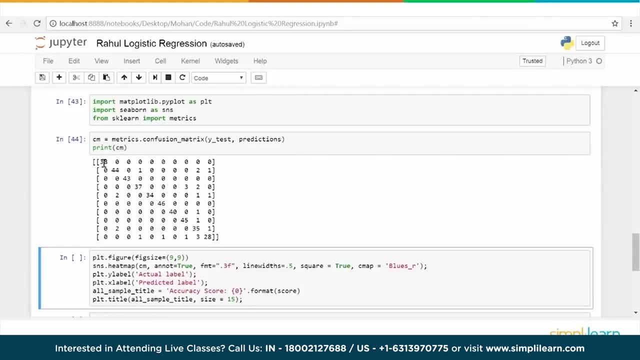 of numbers, which means the accuracy is very low. the diagonal indicates a correct prediction, that the actual value is same as the predicted value. here again: actual value same as the predictive value, and so on. right, so the moment you see a number here, that means the actual value is. 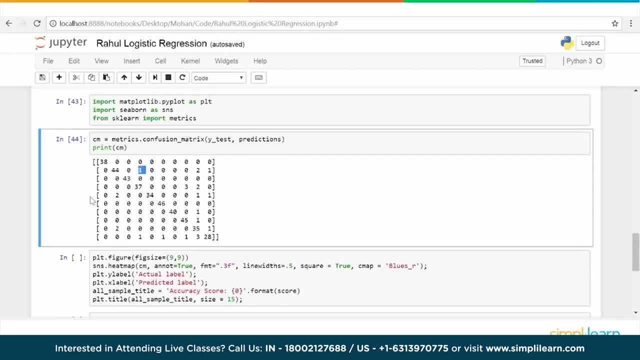 something and the predicted value is something else. right? similarly here, the actual value is something and the predicted value is something else. so that is basically how we read the confusion Matrix. now, how do we find the accuracy? you can actually add up the total values in the diagonal. 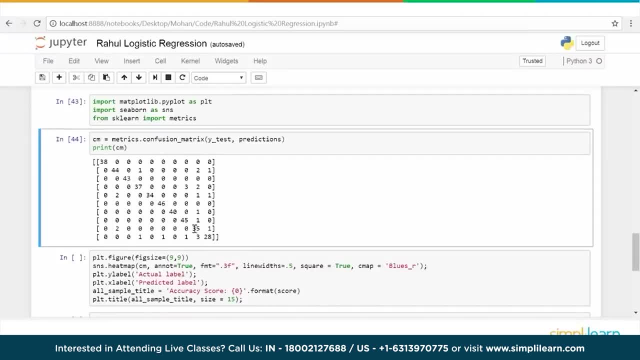 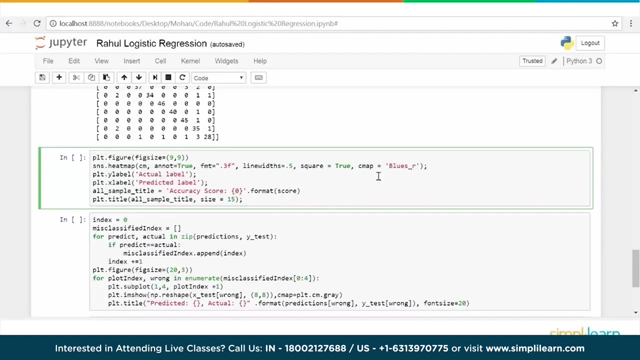 so it's like 38 plus 44 plus 43 and so on, and divide that by the total number of test observations. that will give you the percentage accuracy using a contribution Matrix. now let us visualize this confusion Matrix in a slightly more sophisticated way using a heat map. so we will create a heat map. 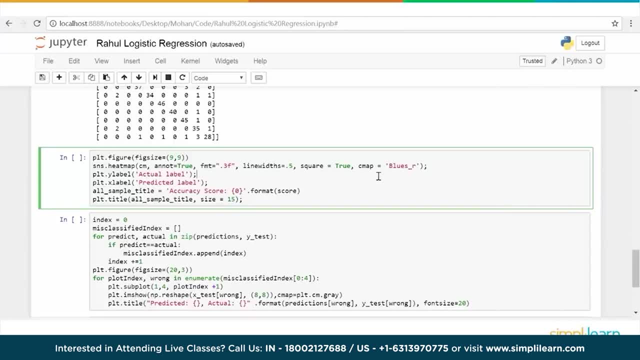 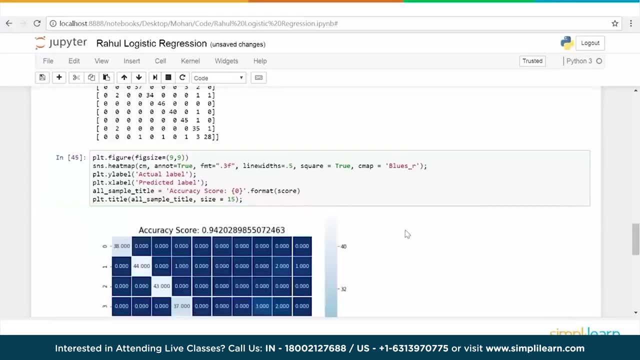 with some, we'll add some colors as well. it's uh, it's like a more visually, visually more appealing. so that's the whole idea. so if we run this piece of code and this is how the heat map looks and, as you can see here, the diagonals: 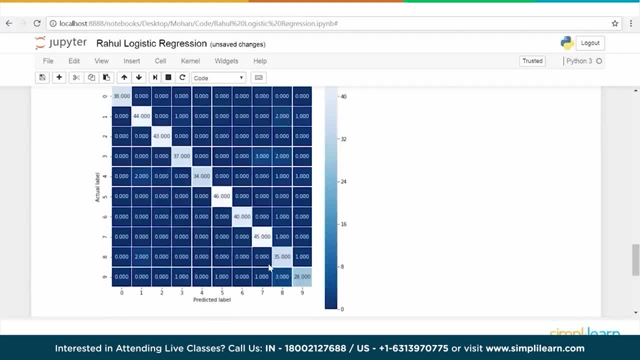 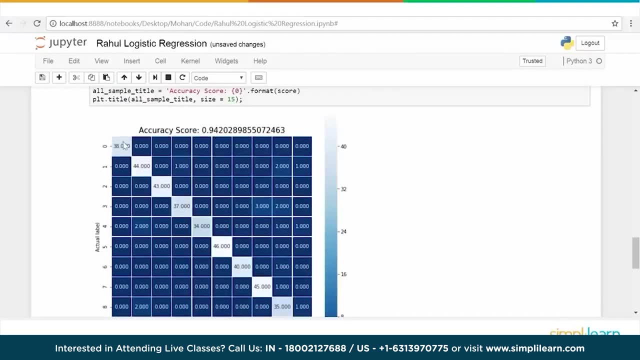 again, are all the values, are here most of the values, so, which means reasonably. this seems to be reasonably accurate and, yeah, basically the accuracy score is 94. this is calculated, as I mentioned, by adding all these numbers divided by the total test values, or the total number of. 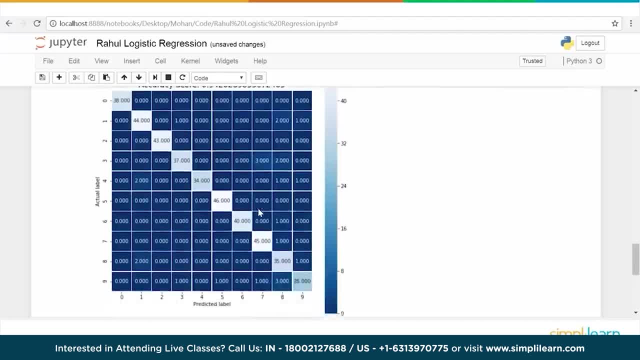 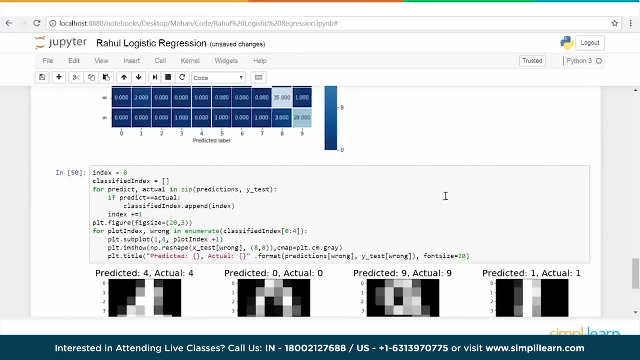 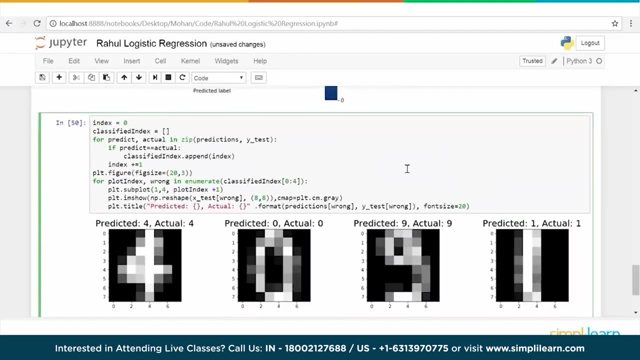 observations in test data set. okay, so this is the confusion Matrix for logistic regression. all right, so now that we have seen the confusion Matrix, let's take a quick sample and see how well the system has classified and we will take a few examples of the data. so if we see here, we picked up randomly a few of them. so this is number four. 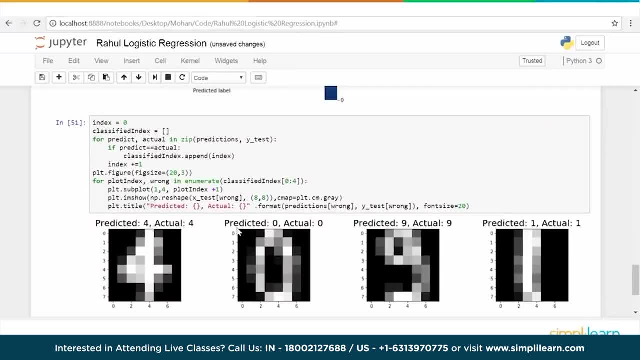 which is the actual value and also the predicted value. both are four. this is an image of zero, so the predicted value is also zero. actual values, of course zero. then this is the image of nine, so this has also been predicted correctly: nine and actual value is nine. and this is the image of one. 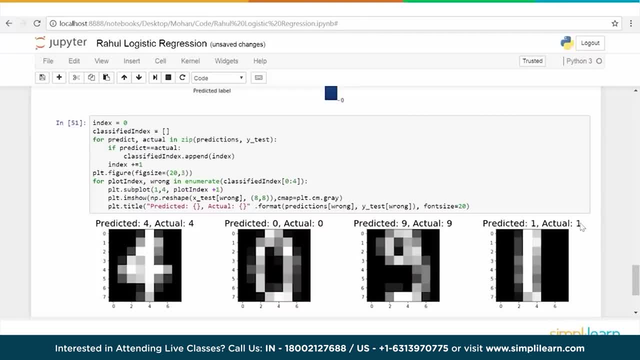 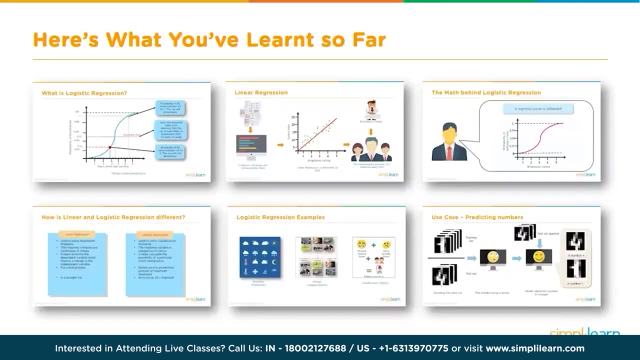 and again this has been predicted correctly as like the actual value. okay, so this was a quick demo of logistic regression- how to use logistic regression to identify images. okay, so let's get started. in this video, we discussed about what is logistic regression and how it fits into the 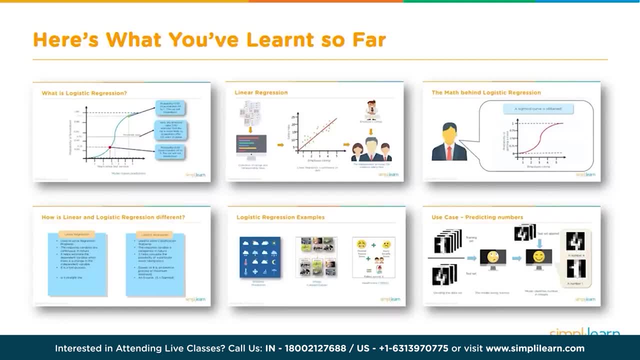 overall machine learning. we discussed about the different types of machine learning and how logistic regression is one of the algorithms for classification, and then we compared logistic regression with linear regression, because the names may be sounding similar, but these are completely different algorithms. linear regression is used for predicting continuous values, whereas 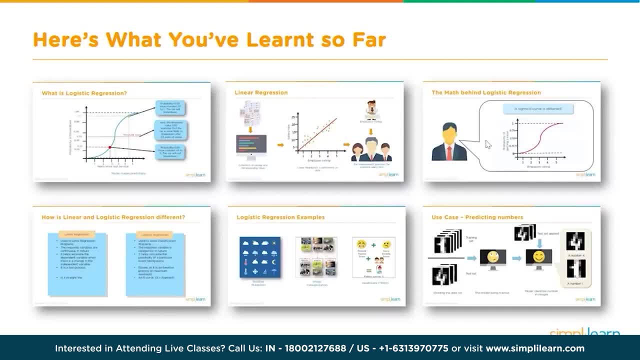 regression is used for finding discrete values. and then we talked about the math behind logistic regression and we derived that function as well, the sigmoid function. we did a quick tabular comparison between linear and logistic regression. we saw some examples of day-to-day life, how logistic regression is used for some of the class for solving some of the classification problems and 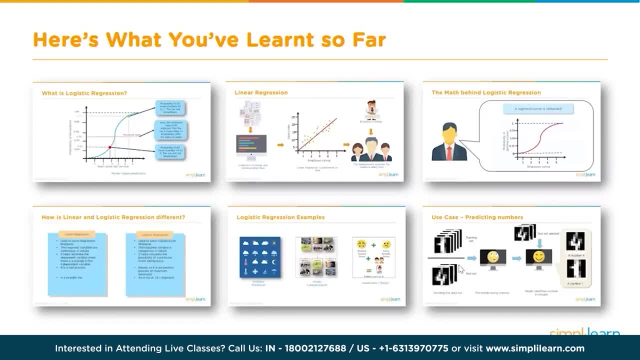 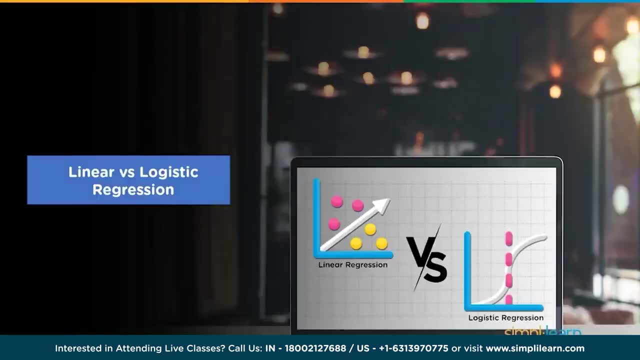 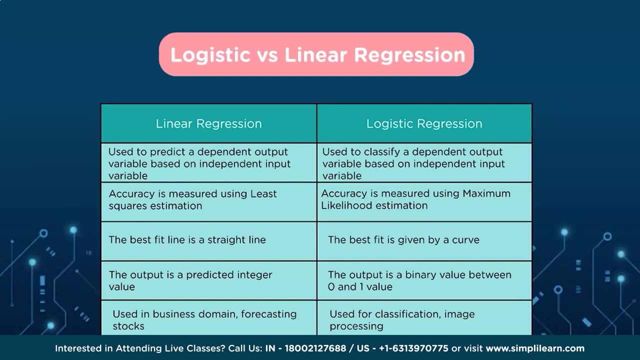 then in the end we looked at the code to see how we can implement logistic regression to train the model to identify images. there's all kinds of regression models that come out of this, so we put them side to about side. we have our linear regression, which is a predictive number used to predict a dependent output variable. 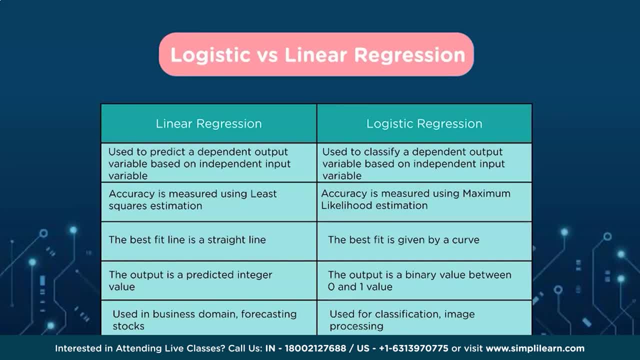 based on independent input. variable accuracy is a measured using least squares estimation, so that's where you take it. you can also use absolute value. the least squares is more popular. there's reasons for that, mathematically, and also you can use the least squares method to calculate the least squares. 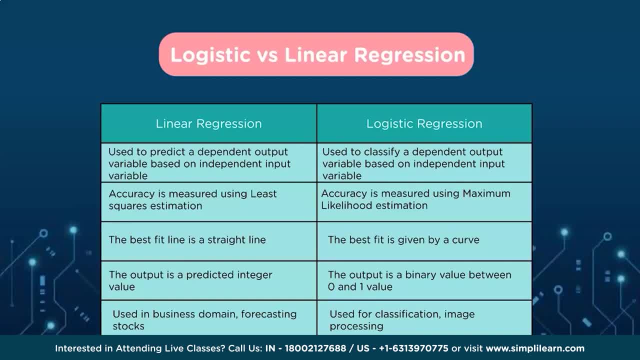 so for computer run time, but it does give you an accuracy based on the least square estimation. the best fit line is a straight line and clearly that's not always used in all the regression models. there's a lot of variations on that. the output is a predicted integer value. again this: 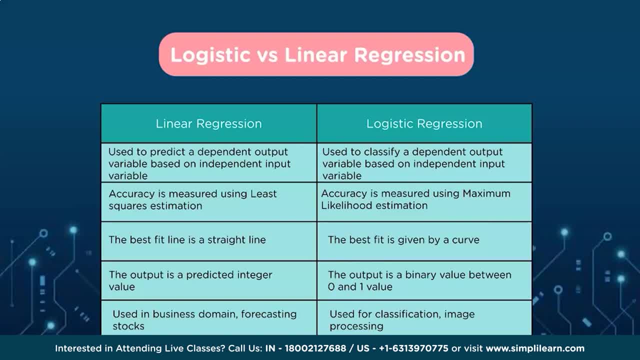 is what we're talking about. we talk about linear regression and we're talking about regression. it means the numbers coming out. linear usually means we're looking for that line versus a different model and it's used in business domain forecasting stocks. it's used as a basis of almost predictions with 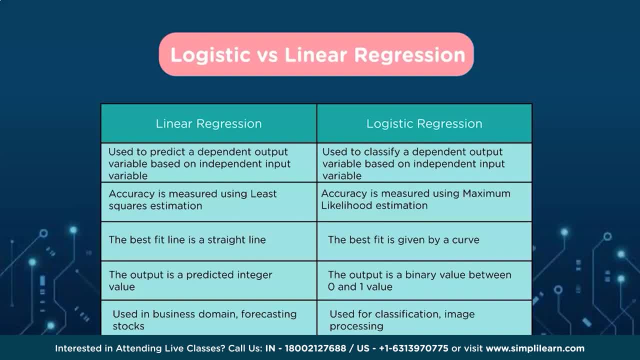 numbers. so if you're looking at a lot of numbers, you're probably looking at a linear regression model. for instance, if you do just the high-lowz of the stock exchange and you're going to take a lot more of that if you want to make money off the stock, you'll find that the linear regression model. 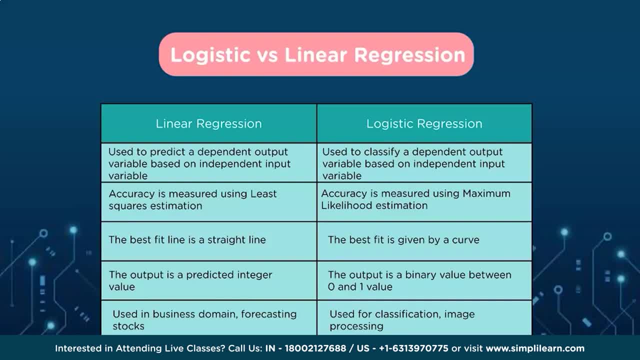 fits, probably better than almost any of the other models: das, 19 percent of theкретickmencom models, even high-end neural networks and all these other different machine learning and AI models, because they're numbers, They're just a straight set of numbers. You have a high value. 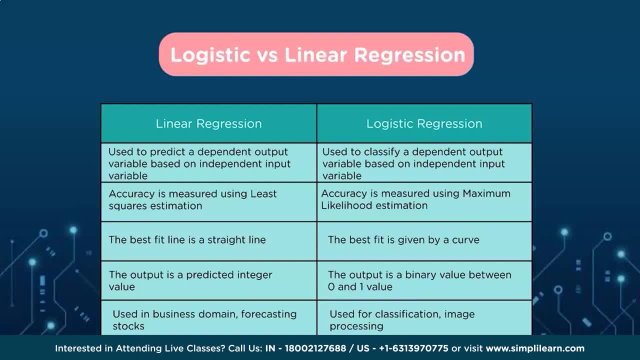 a low value volume, that kind of thing. So when you're looking at something that's straight numbers and are connected in that way, usually you're talking about a linear regression model and that's where you want to start A logistic regression model used to classify dependent 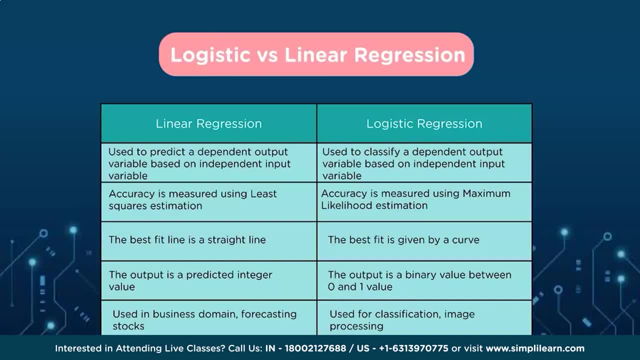 output variable based on independent input variable. So, just like the linear regression model and like all of our machine learning tools, you have your features coming in, And so in this case you might have an image or something like. that is probably the very popular thing right now: labeling broccoli and vegetables, or whatever Accuracy is measured using. 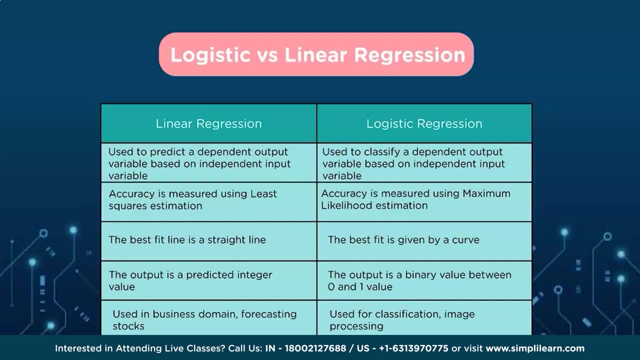 maximum likelihood estimation, The best fit is given by a curve and we saw that when we're talking about linear regression, you definitely are talking about a straight line, although there is other regression models that don't use straight lines, And usually when you're looking at a logistic regression, the math, as you saw, was still 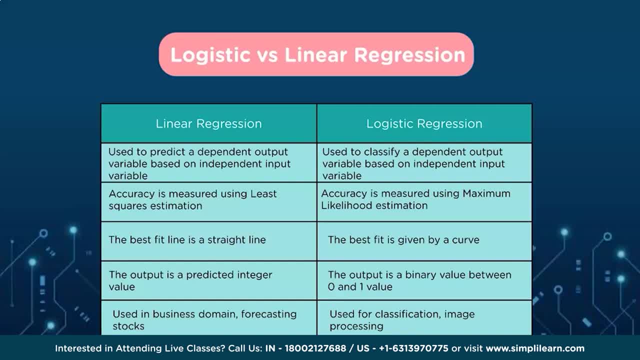 kind of a Euclidean line, but it's now got that sigmoid activation which turns it into a heavily weighted curve And the output is a binary value between 0 and 1. And it's used for classification. image processing, as I mentioned, is what people usually think of, although they use it for. 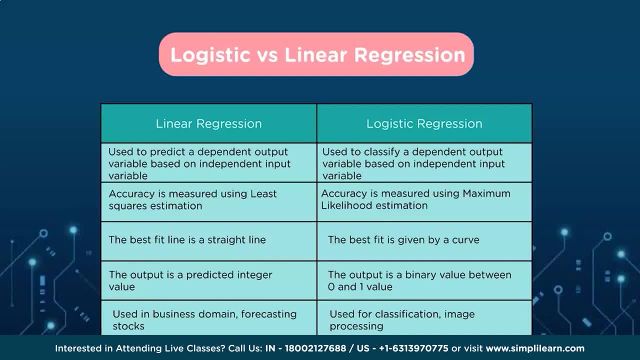 classification of like a window of things. So you could take a window of stock history and you could generate classifications based on that and separate the data that way. If it's going to be that this particular pattern occurs, it's going to be upward trending or downward trending, In fact, a number 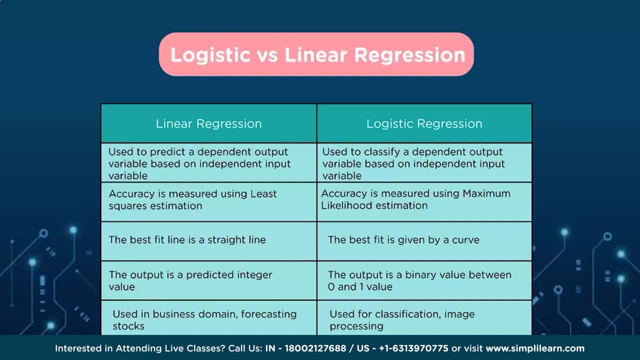 of stock traders use that not to tell them how much to bid or what to bid, but they use it as to whether it's worth looking at the stock or not. whether the stock is going to go down or go up, It's just a 0 or 1.. Do I care, or do I even want to look at it? 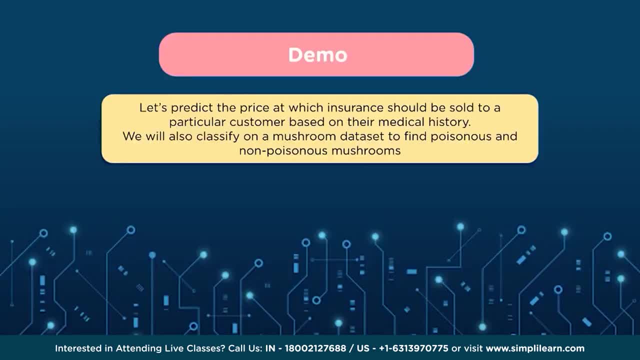 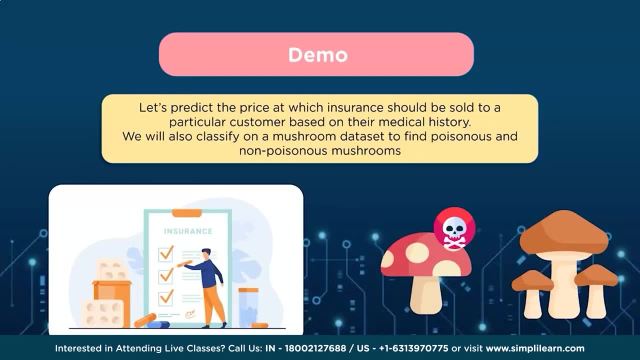 So let's do a demo so you can get a picture of what this looks like in Python code. Let's predict the price at which insurance should be sold to a particular customer based on their medical history. We will also classify on a mushroom data set to find the poisonous. 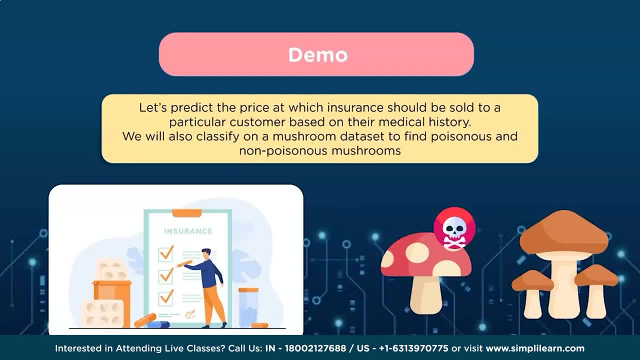 and non-poisonous mushrooms. And when you look at these two data, the first one, we're looking at the price. So the price is a number, So let's predict the price, So let's predict the price. So let's predict the price. 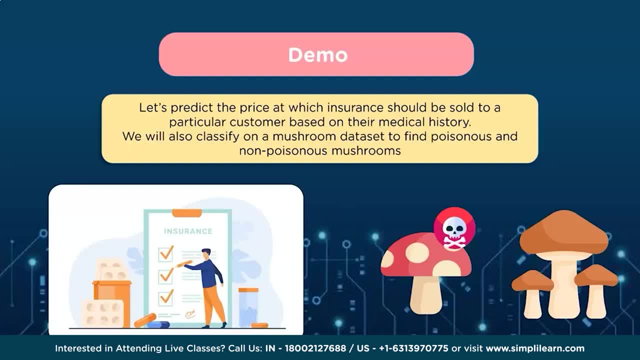 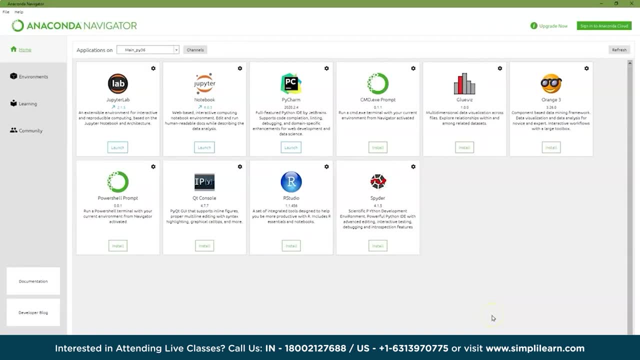 Which the insurance should be sold to. And the second one is we're looking at either it's poisonous or it's not poisonous. So first off, before we begin the demo, I'm in the Anaconda Navigator. In this one I've loaded the Python 3.6 and using the Jupyter Notebook, And you can. 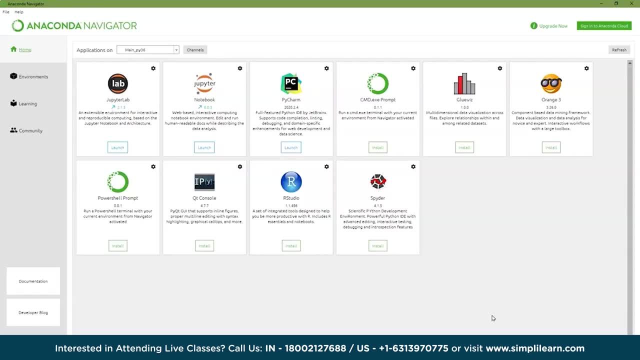 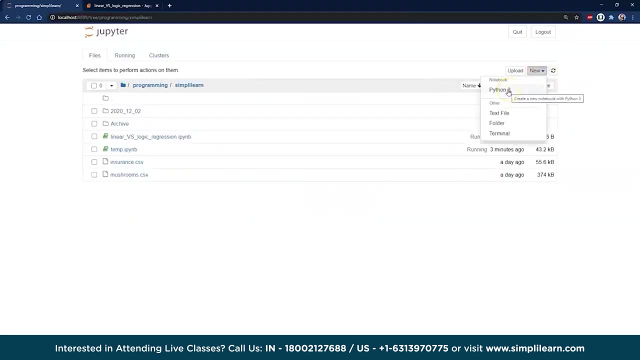 use Jupyter Notebook by itself. You can use the Jupyter Lab, which allows multiple tabs. It's basically the notebook with tabs on it. But the Jupyter Notebook is just fine and it'll go into Google Chrome, which is what I'm using for my Internet Explorer, And from here we open up new and you'll see. 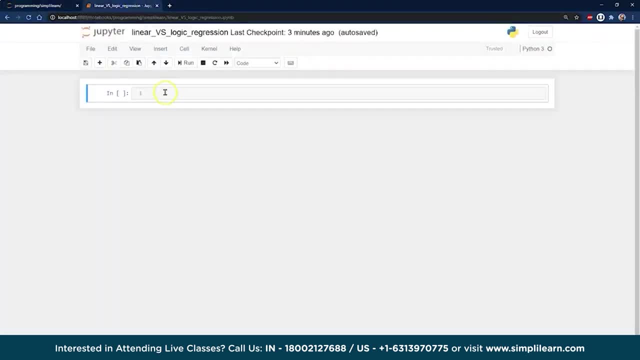 Python 3.. And again, this is loaded with Python 3.6.. And we're doing the linear versus logic regression or logit. You'll see, L-O-G-I-T is one of the names that kind of pops up when you do a search on here, But it is a logic. 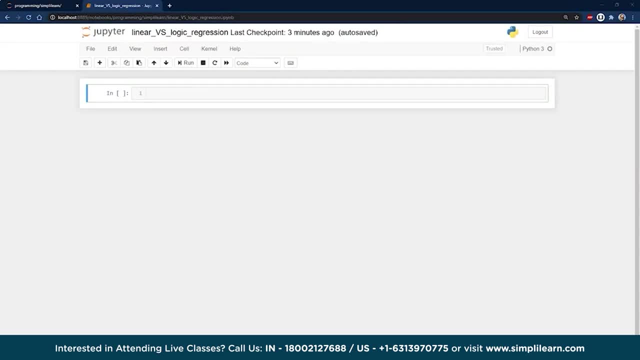 We're looking at the logistic regression models And we'll start with the linear regression because it's easy to understand. You draw a line through stuff And so in programming, we got a lot of stuff to unfold here in our startup. as we preload all of our different parts, Let's go ahead and 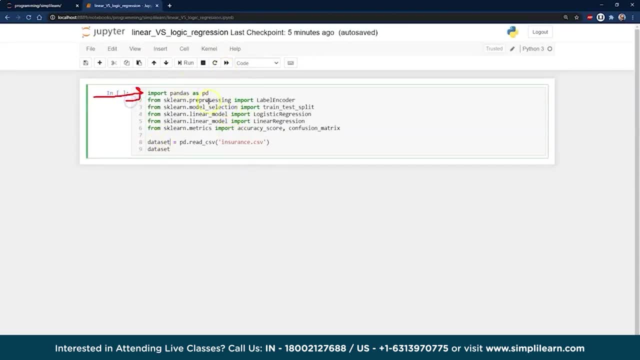 break this up. We have, at the beginning, import pandas, So this is our data frame. It's just a way of storing the data. Think of a…. when you talk about a data frame, think of a spreadsheet. You have rows and columns. It's a nice way of viewing the data. 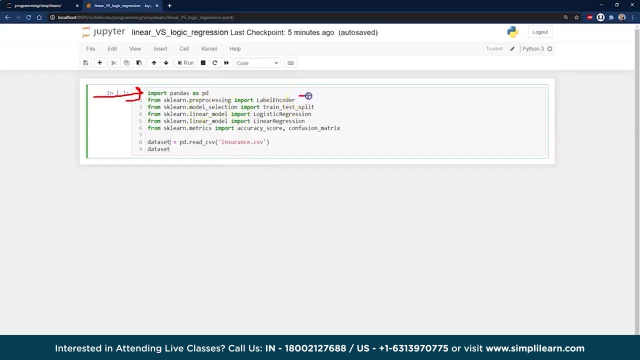 And then we have- we're going to be bringing in- our pre-processing label encoder. I'll show you what that is. When we get down to it, it's easier to see in the data, But there's some data in here, like sex. It's male or female, So it's not like an actual number. 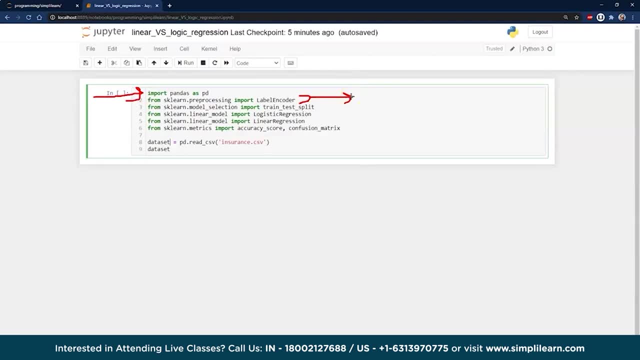 It's either your one or the other, That kind of stuff ends up being encoded. That's what this label encoder is. right here We have our test split model. If you're going to build a model, you do not want to use all the data. You want to use some of the data and then test it to see how. 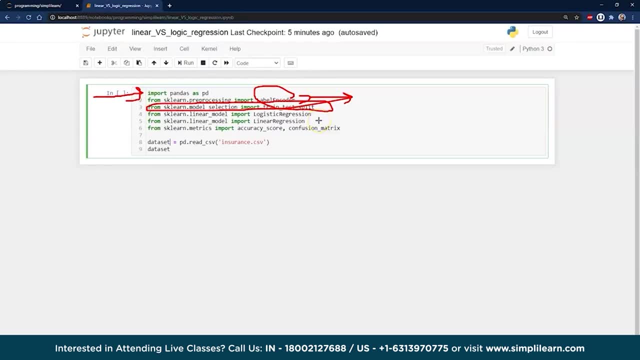 good it is, And it can't have seen the data you're testing on until you're ready to test it on there and see how good it is. And then we have our logistic regression model, our categorical one, and then we have our linear regression model. These are the two, these right here. let me just 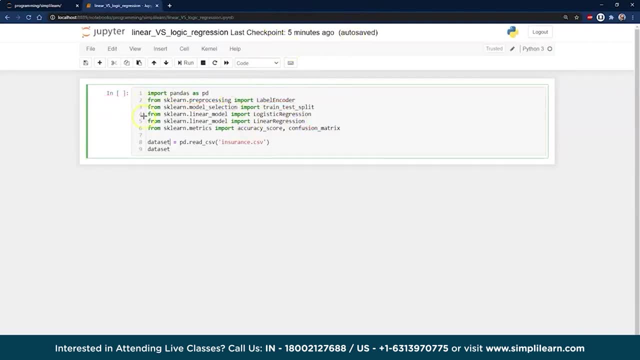 clear all that. There we go. These two right here are what this is all about: logistic versus linear. Is it categorical? Are we looking for a true, false, Or are we looking for a specific number? And then finally, usually at the very end, we have to take and just ask how accurate. 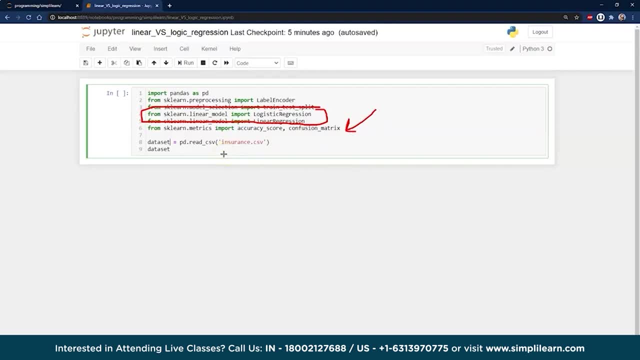 is our model. Did it work? If you're trying to predict something, in this case we're going to be doing a insurance costs- How close to the insurance cost does it measure that we expect it to be? If you're an insurance company, you don't want to promise to pay everybody's medical bill and not 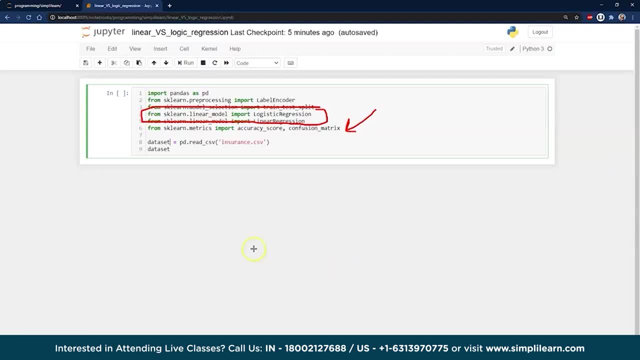 be able to, And, in the case of the mushrooms, you probably want to know just how much at risk you are for following this model as to far as whether you're going to eat a poisonous mushroom and die or not. So we'll look at both of those and we'll get to talk a little bit more about the. 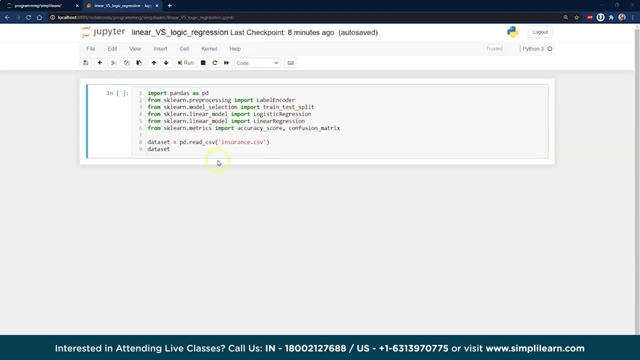 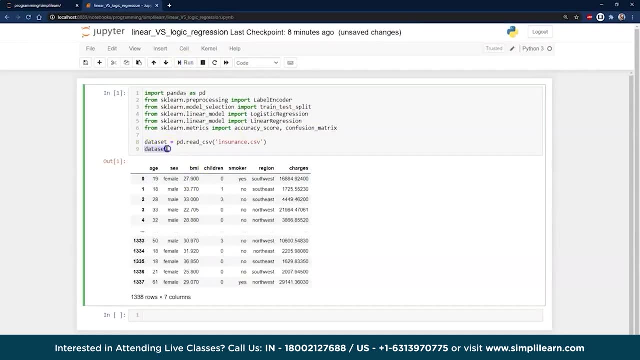 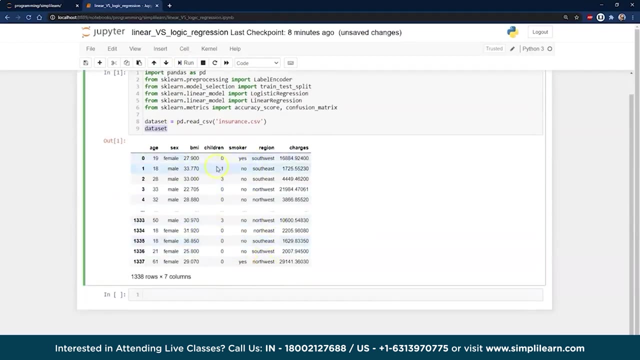 shortcomings and the value of these different processes. So let's go ahead and run this. This is loaded, the data set on here, And then, because we're in Jupyter Notebook, I don't have to put the print on there. We just do data set and by, and it prints out all the different data on here And you. 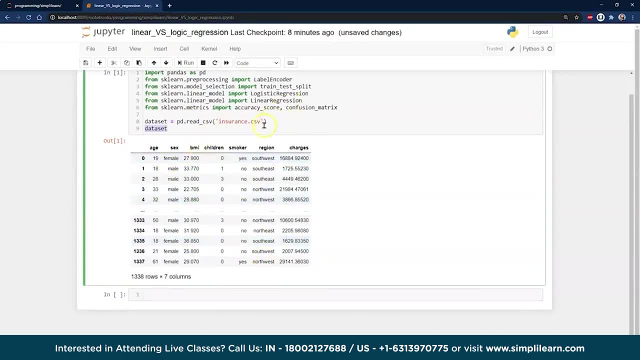 can see here for our insurance, because we're starting with, we're loading that with our pandas and it printed in a nice format where you can see the age, sex, body mass index, number of children, smoker. so this may be something that the insurance company gets from the doctors. 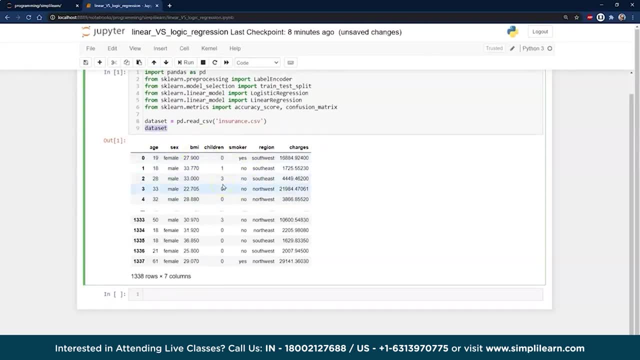 to say: we're going to, this is what we need to know, to give you a quote for what we're going to charge you for your insurance. and you can see that it has 1338 rows and seven columns. you can count the columns one, two, three, four. 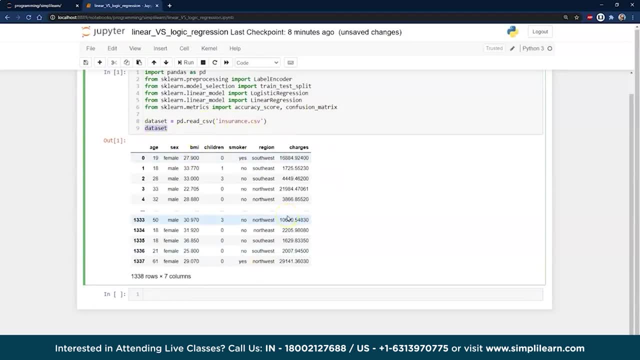 five, six, seven, so there's seven columns on here, and the column we're really interested in is charges. I want to know what the charges are going to be. what can I expect? not a very good arrow drawn what to expect them to charge on there. so is this going to be, you know, is this person going to cost me sixteen thousand? 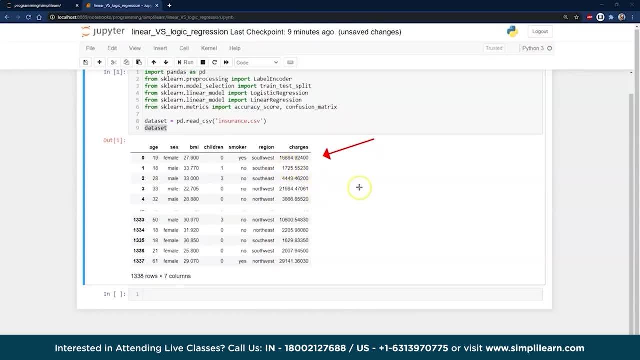 eight hundred eighty four dollars, or is this person only going to cost me three thousand eight hundred sixty six? how do we guess that, so that we can guess what the minimal charge is for their insurance? and then there's one other thing you really need to notice on. 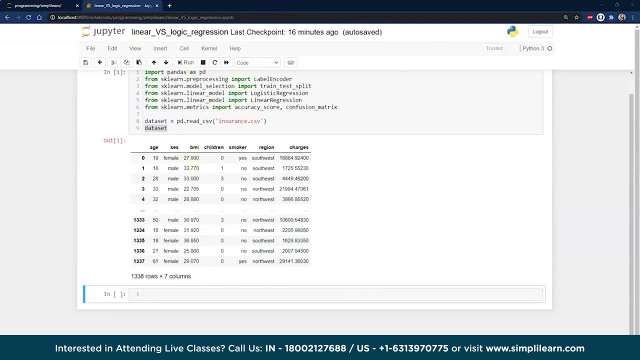 this data and I mentioned it before, but I'm going to mention it again because pre-processing data is so much of the work in data science. sex- well, how do you? how do you deal with female versus male? are you a smoker, yes or no? what does that? 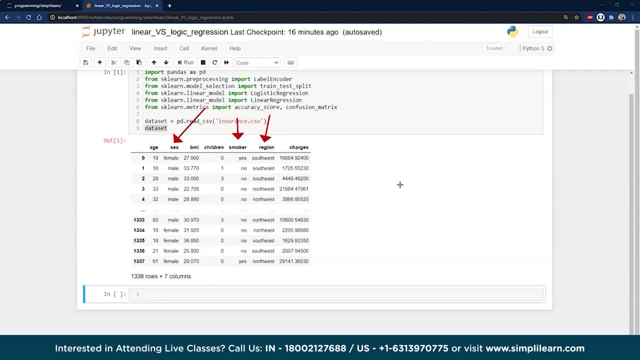 mean region. how do you look at region? it's not a number. how do you draw a line between southwest and northwest? you know they're objects. it's either your southwest or your northwest, it's not like I'm southwest. I guess you could do longitudinal attitude, but the data doesn't come in like that. it comes in as. 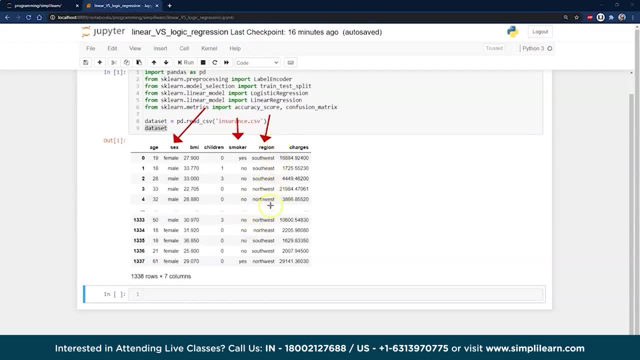 true, false or whatever. you know it's either your southwest or your northwest, so we need to do a little bit of pre-processing of the data on here to make this work. oops, there we go. okay, so let's take a look and see what we're. 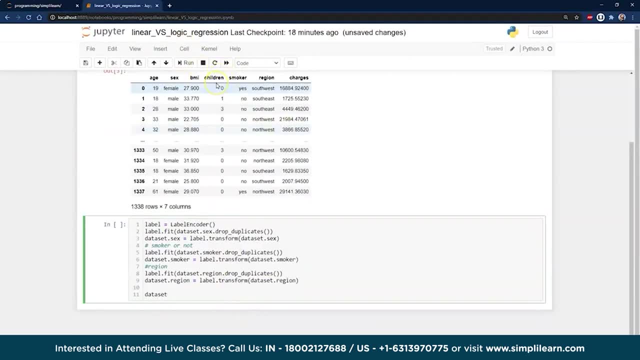 doing with pre-processing, and again, this is really where you spend a lot of time with data science is trying to understand how and why you need to do that, and so we're going to do- you'll see right up here- label, and then we're going to do the do a label encoder. 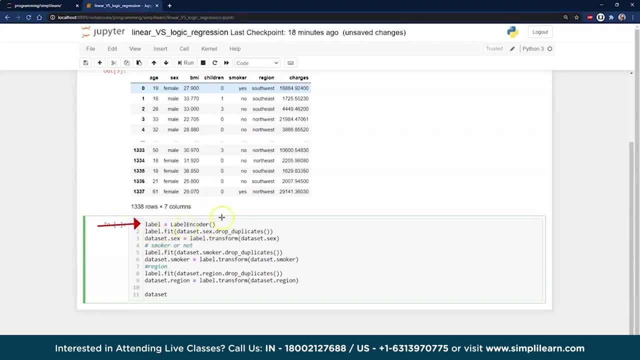 one of the modules we brought in. so this is SK learns label encoder. I like the fact that it's all pretty much automated, but if you're doing a lot of work with the label encoder, you should start to understand how that fits. and then we have a label dot fit right here where we're going to go ahead and do. 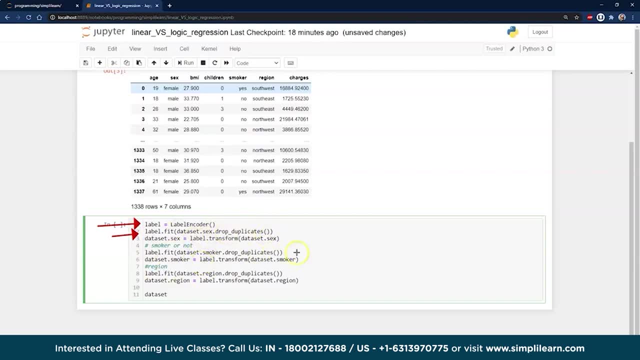 the data set dot sex, dot, drop duplicates. and then for data set sex, we're going to do the label transform the data set sex, and so we're looking right here at male or female, and so it usually just converts it to a zero one, because there's only two choices on here. same thing with the smoker: it's zero or one. 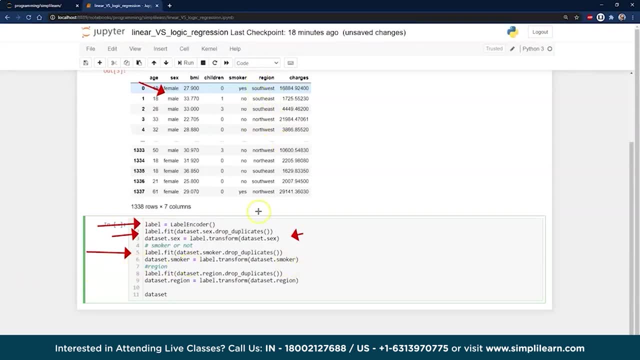 so we're going to transfer the transfer, change the smoker: 0, 1 on this. and then, finally, we did region down here. region does it a little bit different? we'll take a look at that and it's- I think in this case it's probably going to do it because we did it on this label- transform with. 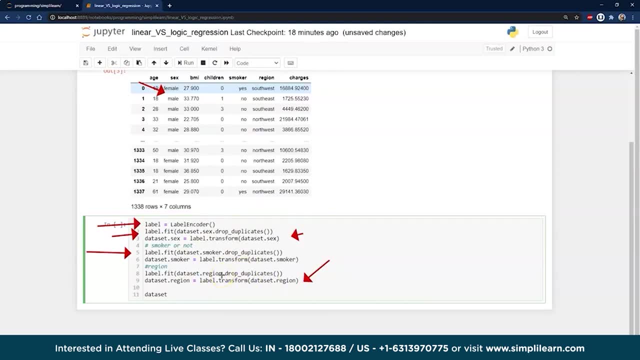 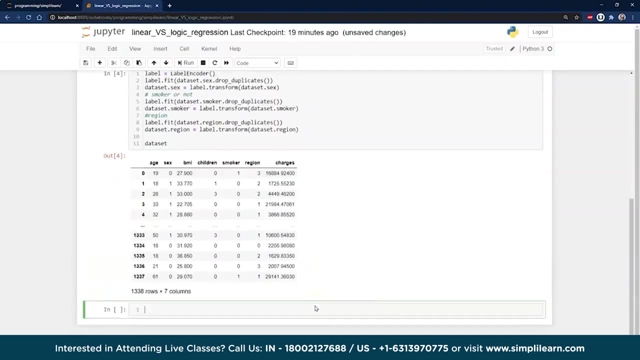 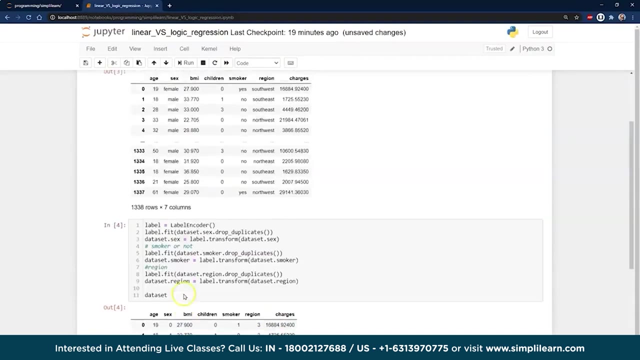 this particular setup. it gives each region a number like 0, 1, 2, 3. so let's go ahead and take a look and see what that looks like. go and run this and you can see that our new data set has age. that's still a number. sex is 0 or 1, so 0 is female, 1 is male. number of children: we left that. 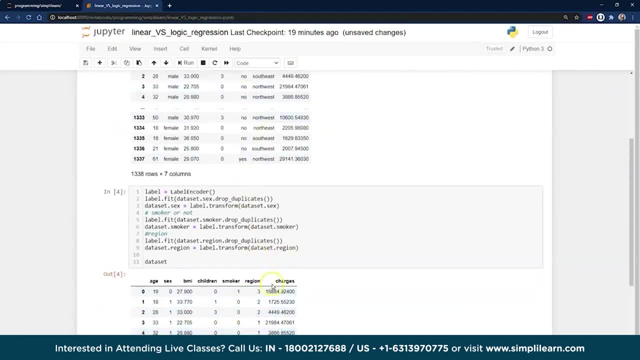 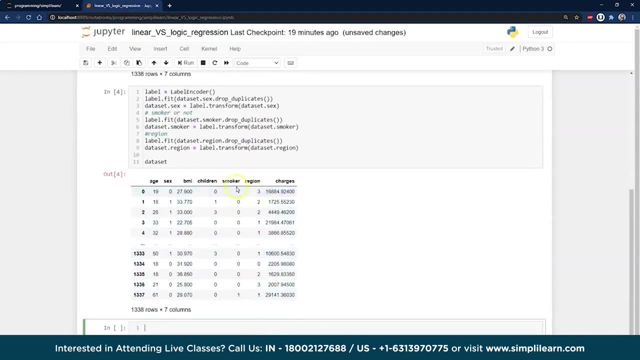 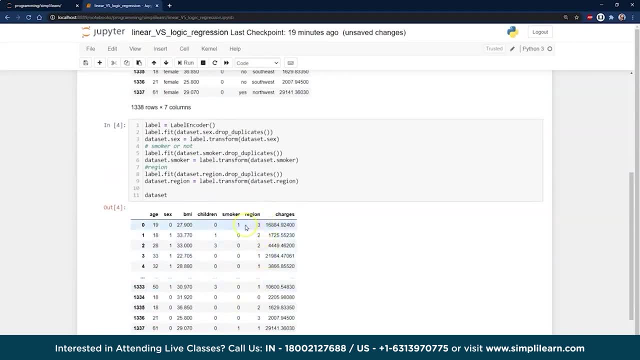 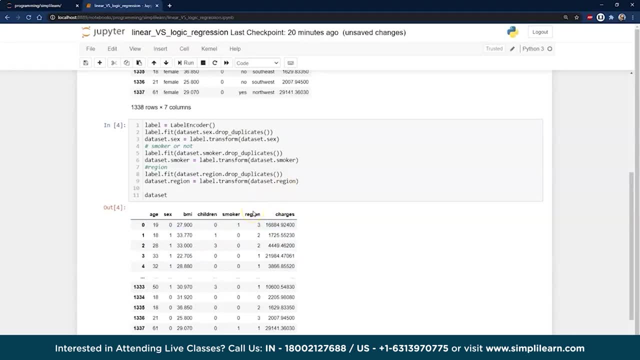 working with data science and you're dealing with regions or even word analysis. instead of doing one column and labeling it- 0, 1, 2, 3- a lot of times you increase your features and so you would have: region Northwest would be one column, yes or no. region Southwest would be one column, yes or no, true, or? 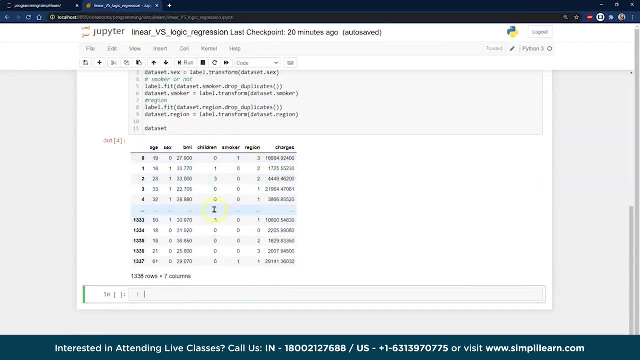 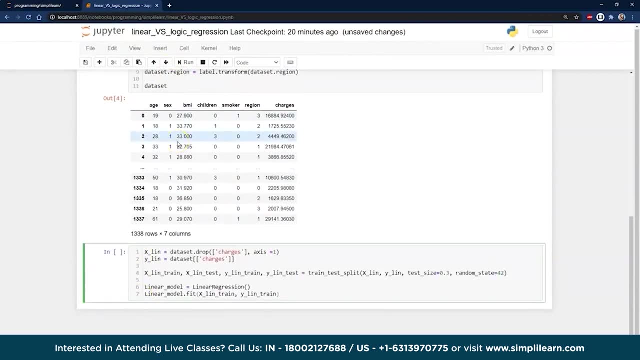 01. but for this, this, this particular setup. this will work just fine on here, now that we spent all that time getting it set up. here's the fun part. here's the part where we're actually using our setup on this and you'll see, right here we have our y linear regression data set. drop the charges. 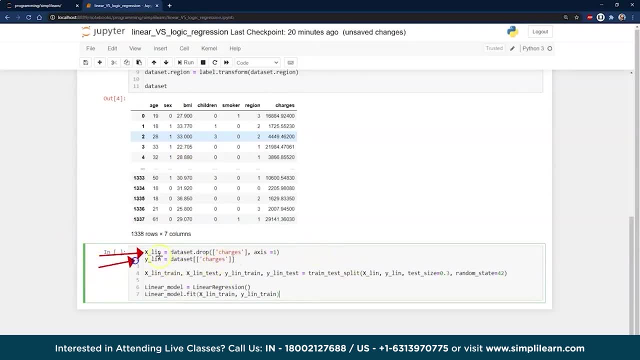 because that's what we want to predict. and so our x- i'm sorry, our x- linear data set drop the charges, because that's what we're going to predict. we're predicting charges right here, so we don't want that as our input for our features and our y output is charges. that's what we want to guess. 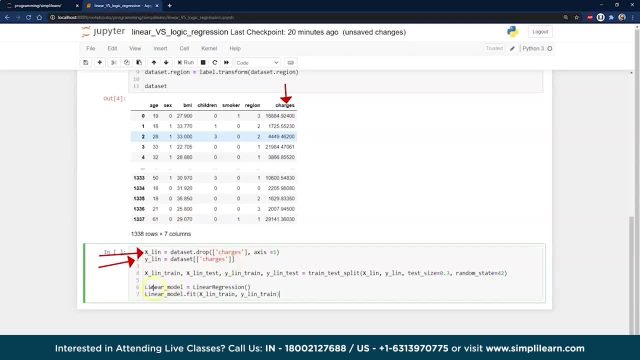 we want to guess what the charges are. and then what we talked about earlier is we don't want to do all the data at once, so we're going to take 0.3 means 30 percent. we're going to take 30 percent of our data and it's going to be as the train as the testing site. so here's our y test and our x. 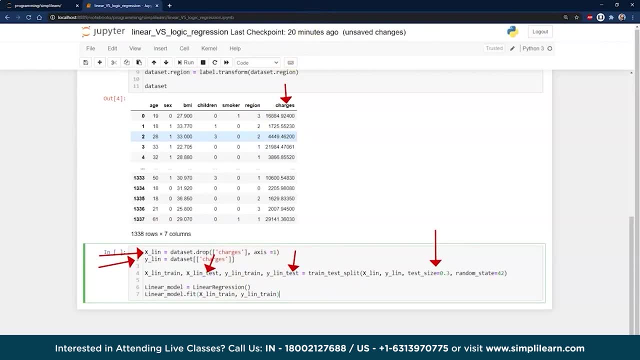 test down there. and so that part, our model, will never see it until we're ready to test to see how good it is. and then, of course, right here you'll see our training set, and this is what we're going to train it. we're going to trade it on seventy percent of the data. and then, finally, the big. 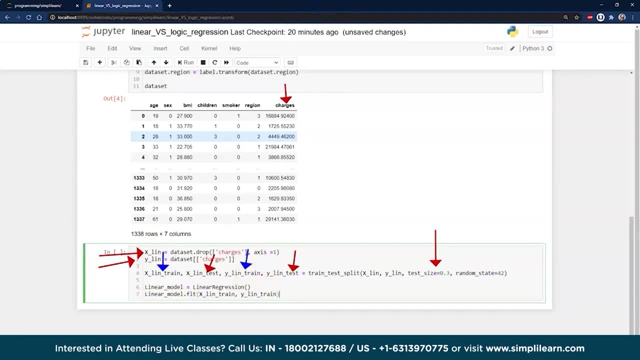 ones. this is where all the magic happens. this is where we're going to create our magic setup and that is, right here, our linear model. we're going to set it equal to the linear regression model and then we're going to fit the data on here. and then, at this point, I always like to pull up if you hit. 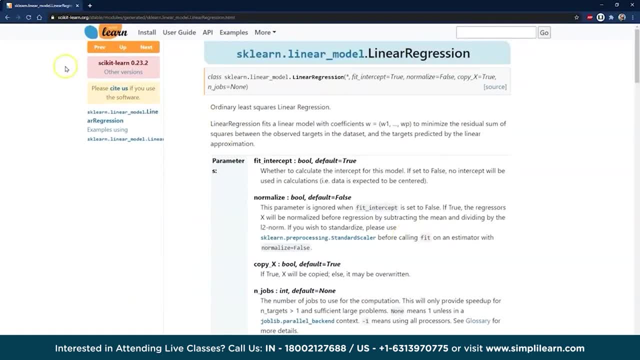 if you're, if you're working with a new model, it's good to see where it comes from. this comes from the psykit learn and this is the sk learn linear model, the your regression that we imported early and you can see they have different parameters. the basic parameter works great. if you're dealing. with just numbers. I mentioned that earlier with stocks. the basic country works great if you're dealing with just numbers. I mentioned that earlier with stocks. back in the day it wasn't just three rooms, it didn't even require three rooms, it was a Ookabara linear regression and you get a little bit. 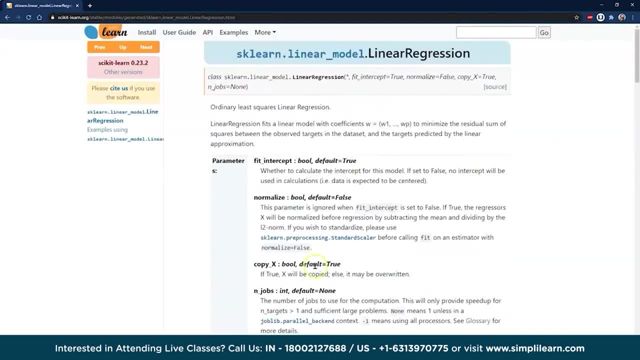 Oak trained in digital modeling and I know we've got something for just our numbers okay. so we're going to do easier面- Zoom basic parameters out here, so we're going to go over to our E website for some high lows. this model will do as good as any other model out there for do, if 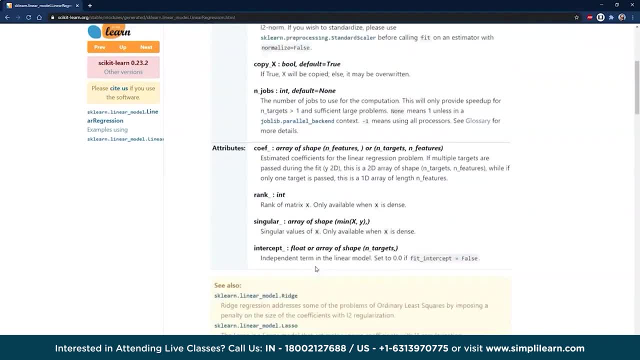 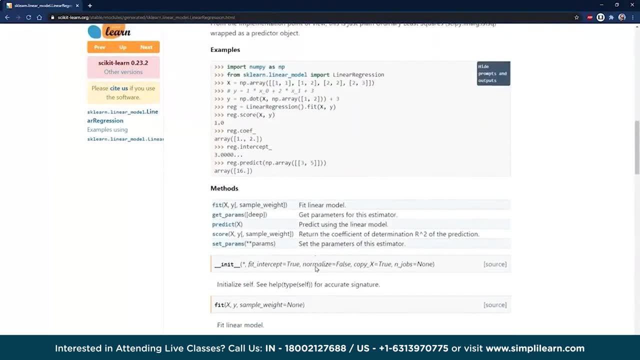 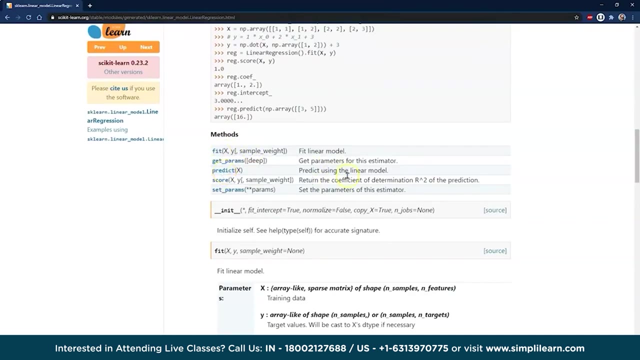 you're doing just the very basic high lows and looking for a linear fit, a regression model fit, and would you? one of the things when I'm looking at this is they look for methods and you'll see, here's our fit that we're using right now and here's our predict, and we'll actually do a little bit in the middle. 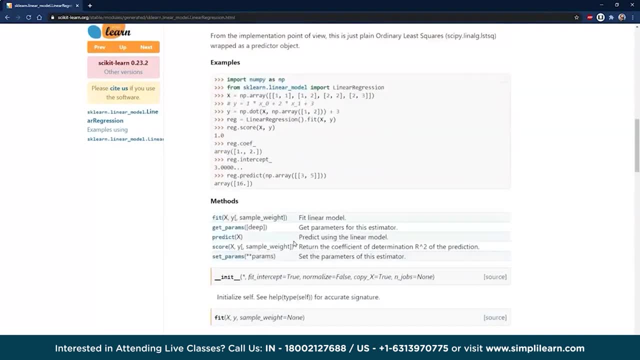 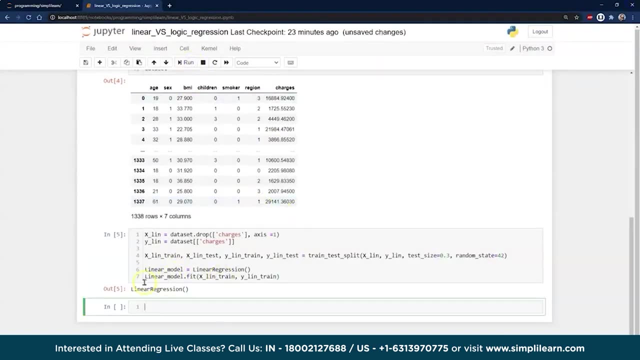 here as far as looking at some of the parameters hidden behind it, the math that we talked about earlier, and so we go in this, we go ahead and run this. you'll see it loads the linear regression model and just has a nice output that says hey, I loaded the linear regression model. and then the second. 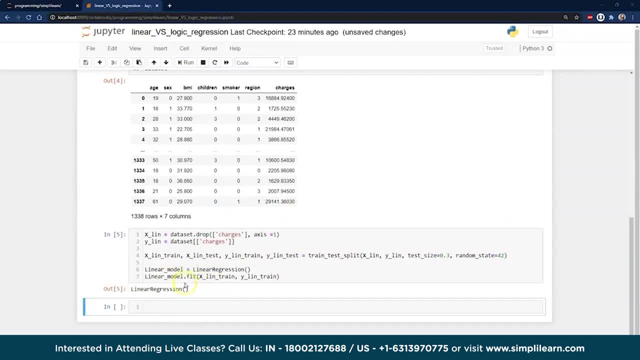 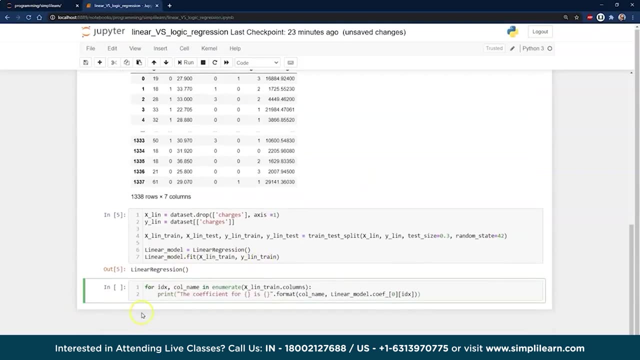 part is: we did the fit, and so this model is now trained. our linear model is now trained on the training data, and so one of the things we can look at is the for ID X and call a name and enumerate X linear training model and then we can look at the fit, and so this model is now trained. 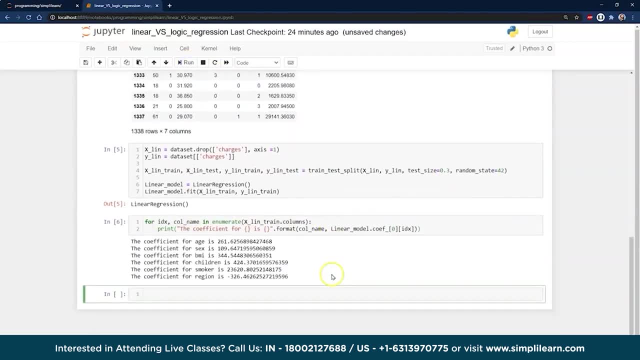 for ID X and call a name and enumerate X linear training model and then we can look at the fit and so this model is now trained columns come. an interesting thing: this prints out the coefficients. so when you're looking at the back end of the data you remember we had that formula B. 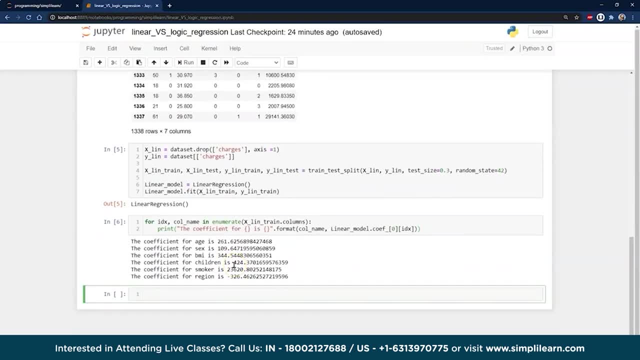 X X 1 plus B X X 2, plus the inner, plus the intercept and so forth. these are the actual coefficients that are in here. this is what it's actually. multiplying these numbers by and you can see like region gets a minus value. so when it. 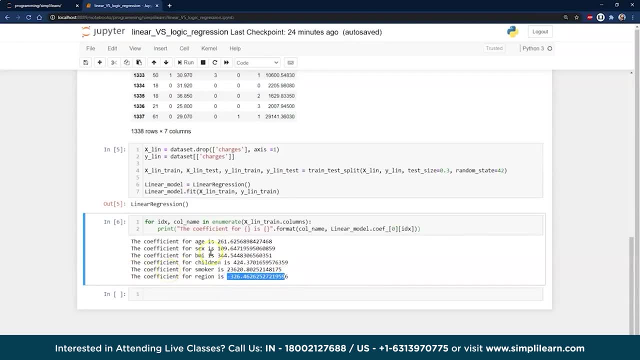 heads it up, I guess region. you can read a lot into these numbers. it gets very complicated. there's ways to mess with them. if you're doing a basic linear regression model, usually don't look at them too closely. but you might start looking in these and saying: 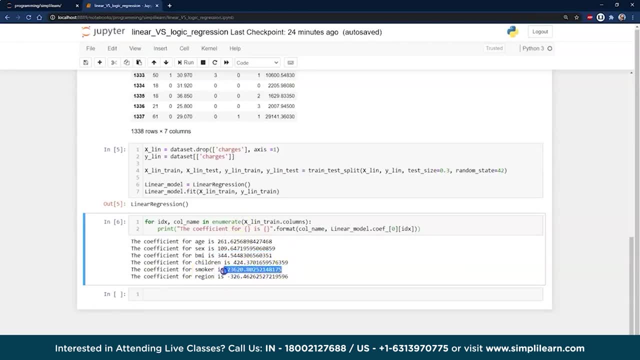 hey, you know what smoker? look how smoker impacts the cost. it's just massive. so this is a flag that, hey, the value of the smoker really affects this model. and then you can see here with a body mass index index: so somebody who is overweight is probably less healthy and more likely to 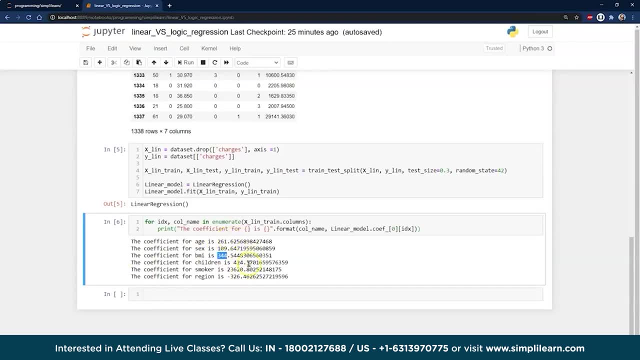 have cost money and then of course age is a factor and then you can see down here we have sexes than a factor also. it just it changes as you go in there negative number, it probably has its own meaning on there again. it gets really complicated when you dig into the workings and how the linear model works. 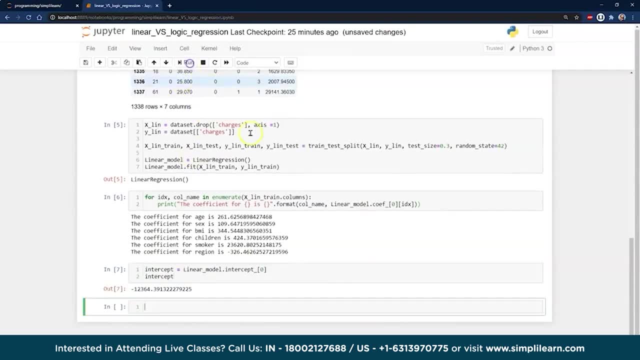 on that and so we can also look at the intercept. this is just kind of fun. so it starts at this negative number, then adds all these numbers to it. that's all that means. that's our intercept on there and that fits the data we have on that, and so you can see, right here we can go back and just a. 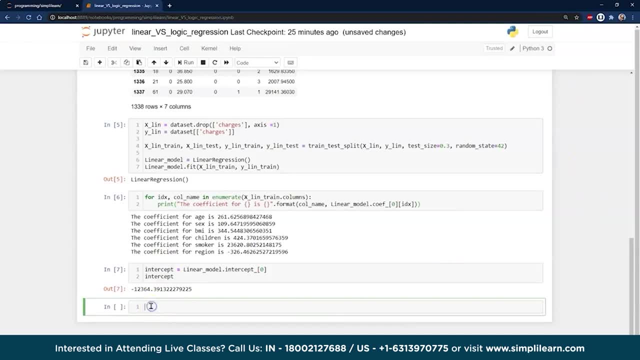 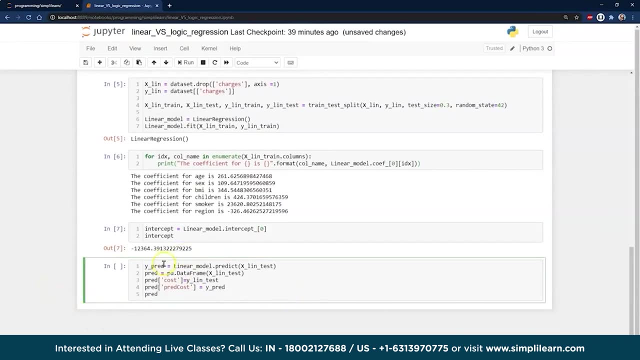 second, there we go. we can go ahead and predict the unknown data and we can print that out. and if you're going to create a model to predict something, we'll go ahead and predict it. here's our Y prediction value: linear model predict. and then we'll go ahead and create a new data frame, in this case from our X. 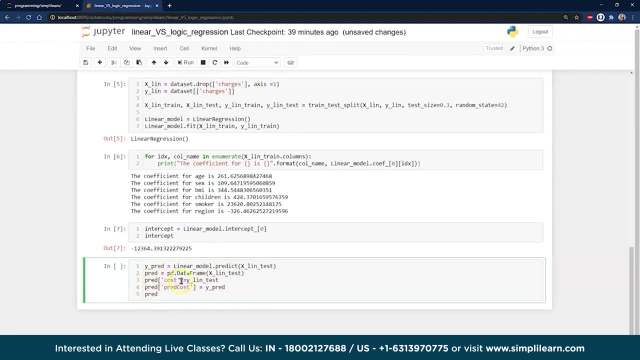 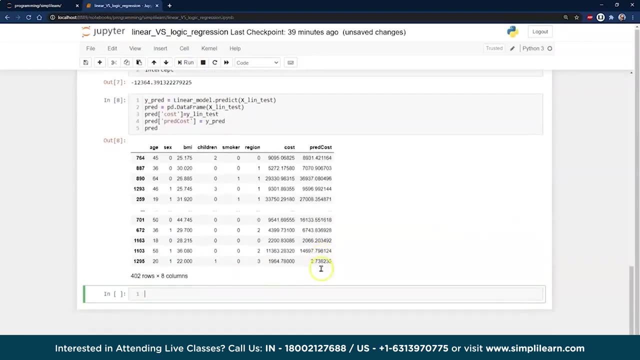 linear test group. we'll go ahead and put the cost back into this data frame and then they predicted cost. we're going to make that equal to our Y prediction and so when we pull this up, you can see here that we have the actual cost and what we 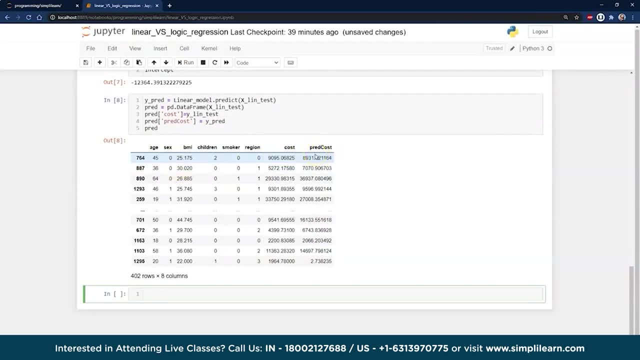 predicted the cost is going to be. there's a lot of ways to measure the accuracy on there, but we're going to go ahead and jump in to the data frame and then we're going to go ahead and create a new data to our mushroom data, and so in this, you can see here we've run our basic model. 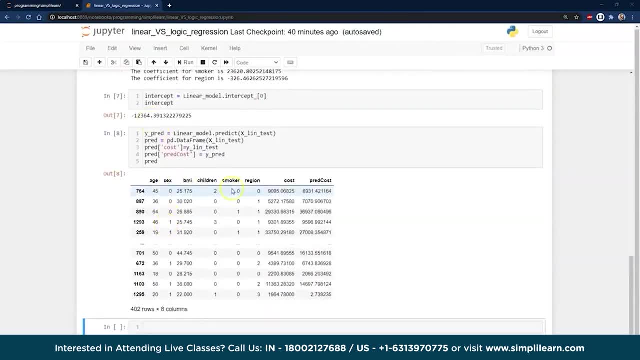 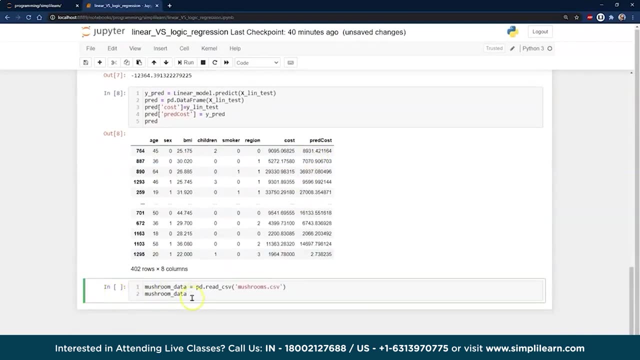 we built our coefficients. you can see the intercept, the back end. you can see how we're generating a number here now with mushrooms, we want a yes or no, we want to know whether we can eat them or not, and so here's our mushroom file. we're going to go ahead and run this. take a look at the data and again you 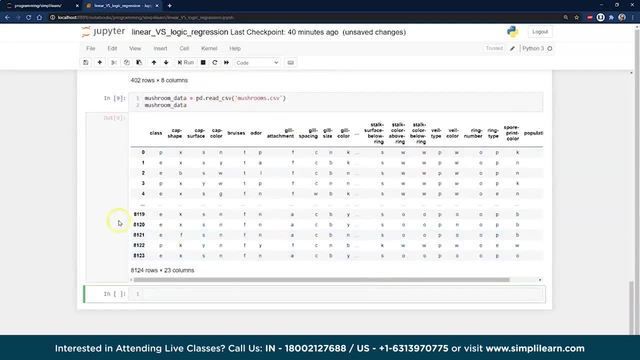 can ask for a copy of this file, send a note over to simply learn comm, and you can see here that we have a class, the cap shape, cap surface and so forth, so there's a lot of feature. in fact. there's 23 different columns in here going across, and when you look at this I'm not even sure what these 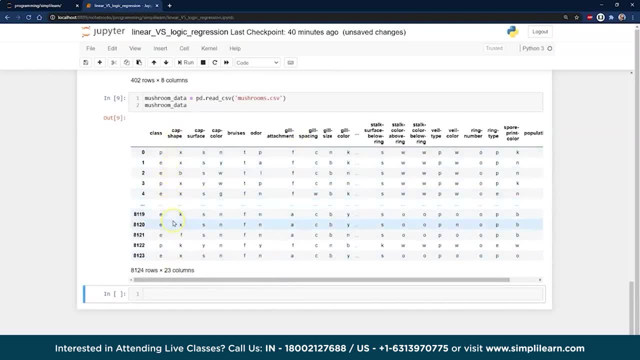 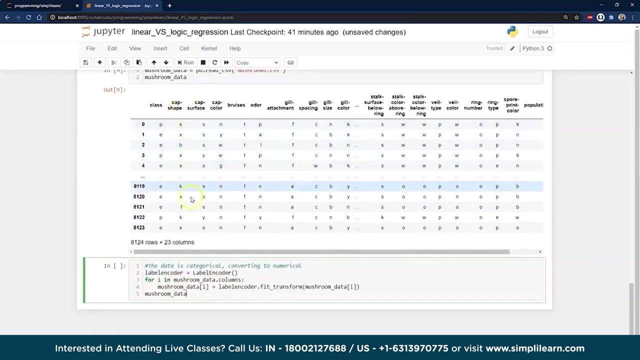 particular like PE, PE. I don't even know what the class is on this. I'm going to guess by the notes that the class is poisonous or edible. so, if you remember, before we had to do a little pre coding on our data. same thing with here. we have our cap shape, which is B or X or K. we have cap color, these: 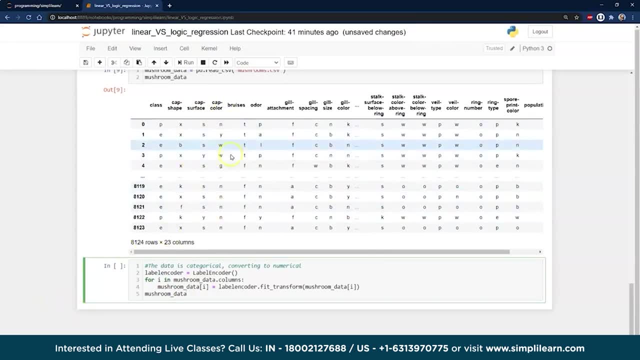 really aren't numbers, so it's really hard to do anything with just a single number. so we need to go ahead and turn those into a label encoder, which again there's a lot of different encoders. with this particular label encoder it's just switching it to zero: one, two, three and so forth. 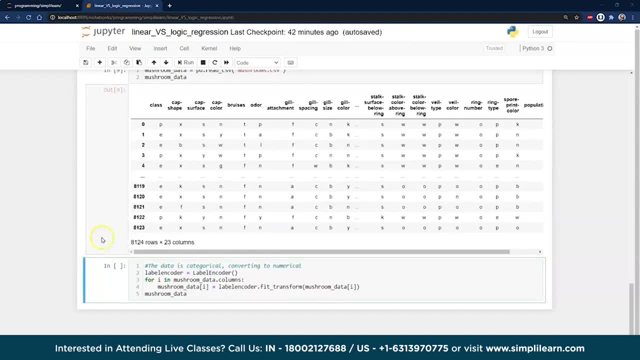 giving it an integer value. in fact, if you look at all the columns, all of our columns are labels and so we're just going to go ahead and loop through all the columns in the data and we're going to transform it into a label encoder, and so when we run this, you can see. 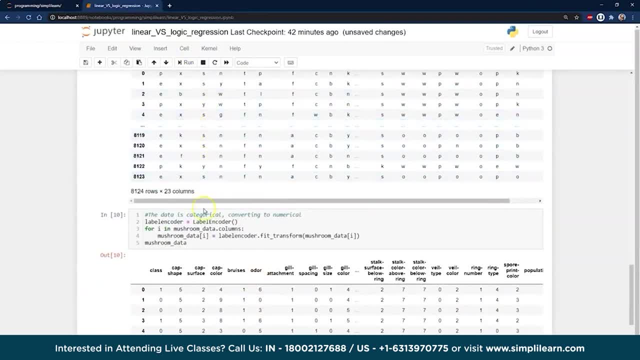 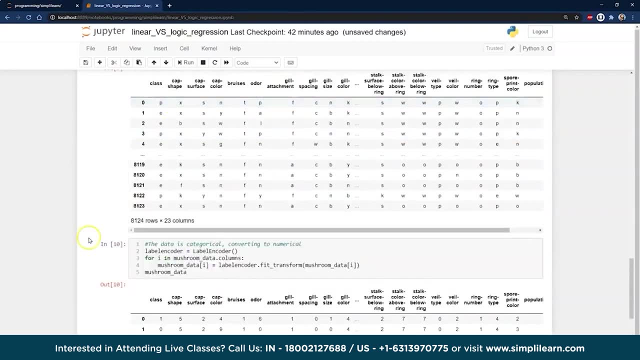 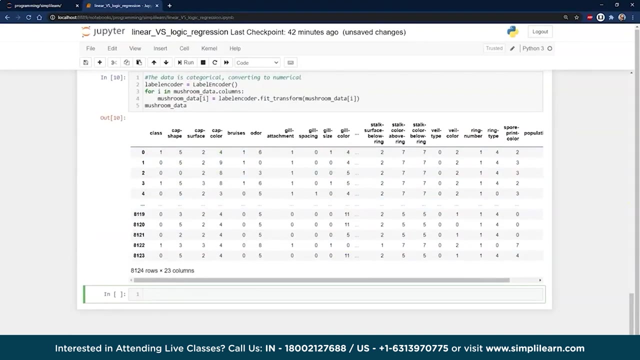 how this gets shifted from x b, x, x k to 0, 1, 2, 3, 4, 5 or whatever it is. class is 0, 1, 1 being poisonous. 0 looks like it's editable and so forth on here, so we're just encoding it. if you were doing this. 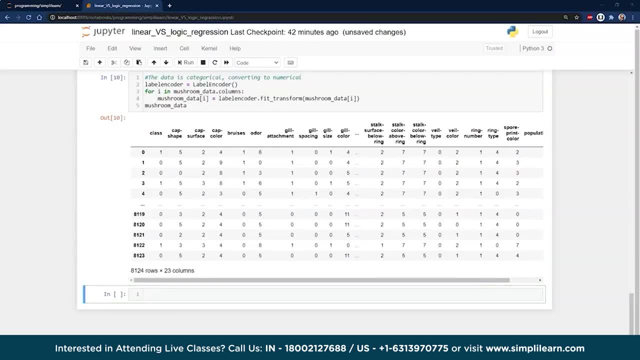 project. depending on the results, you might encode it differently. like i mentioned earlier, you might actually increase the number of features as opposed to laboring at zero. one, two, three, four, five. in this particular example, it's not going to make that big of a difference how we encode it. 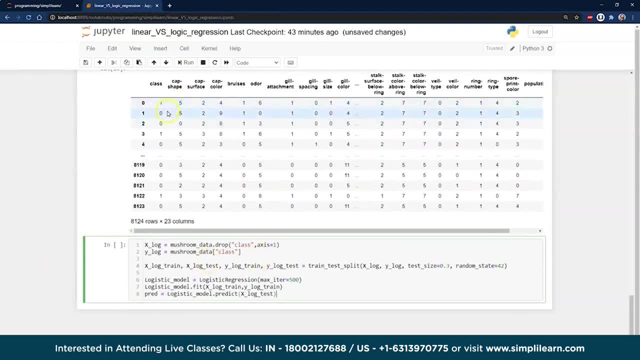 and then, of course, we're looking for the class whether it's poisonous or edible. so we're going to drop the class in our x logistics model and we're going to create our y logistics model is based on that class. so here's our x- y and, just like we did before, we're going to go ahead and 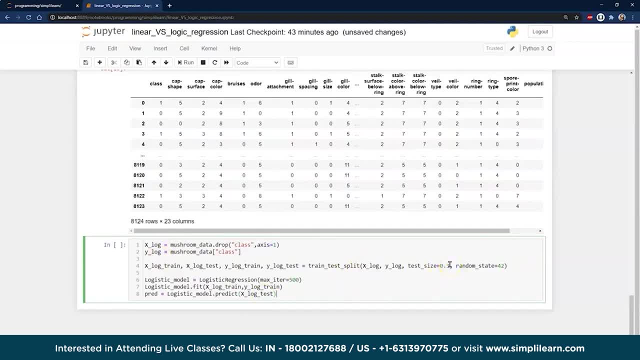 split it using 30 percent for test 70 to program the model on here. and that's right here. whoops, there we go, there's our train and test, and then you'll see here on this next setup. this is where we create our model, all the. 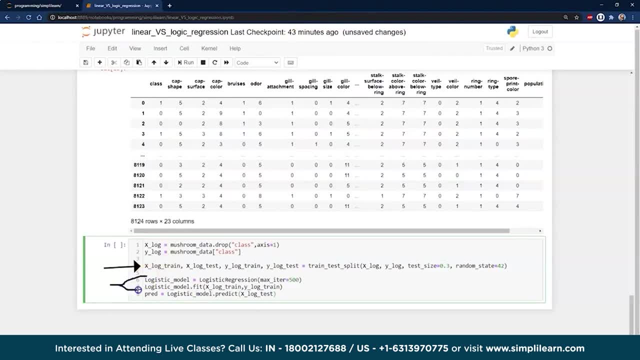 magic happens right here. we go ahead and create a logistics model. i've upped the max iterations. if you don't change this for this particular problem, you'll get a warning that says this has not converged. because that that's what it does is. it goes through the math and it goes. hey, can we? 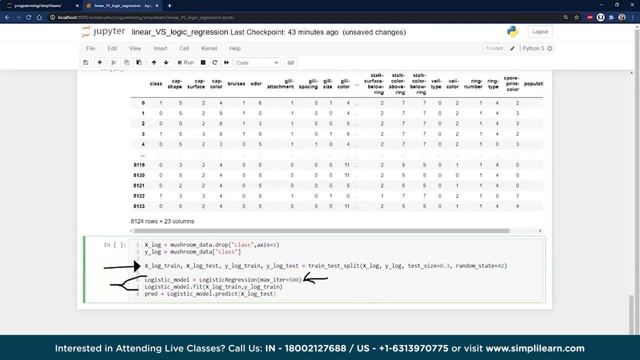 minimize the error and it keeps finding a lower and lower error and it still is changing that number. so that means it hasn't conversed yet, it hasn't find the lowest amount of error it can and the default is 100.. there's a lot of settings in here, so when we go in here to let me pull that, 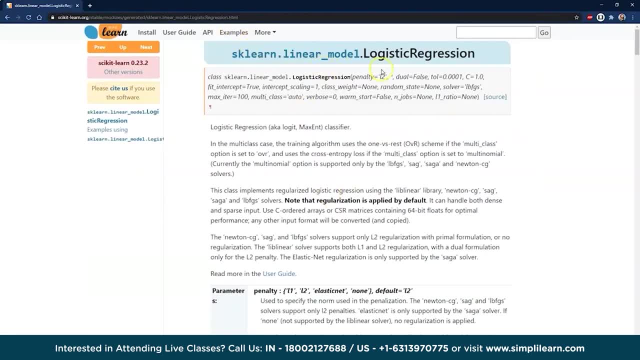 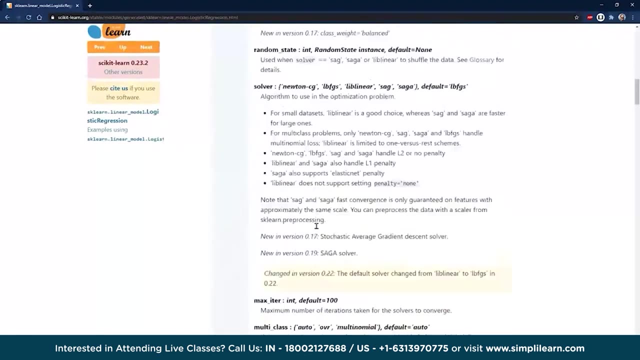 up from the sk learn, so we pull that up from the sk learn model. you can see here we have our logistic. it has our different settings on here that you can mess with. most of these work pretty solid on this particular setup so you don't usually mess a lot. usually i find myself adjusting. 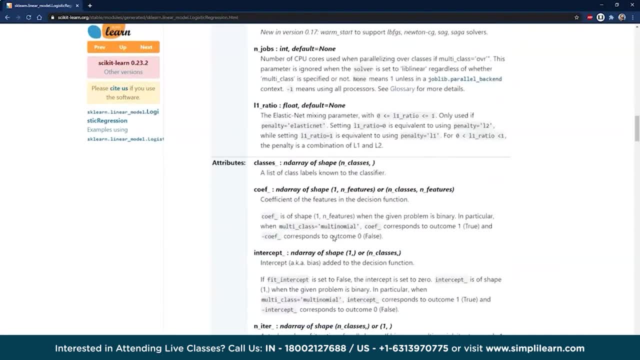 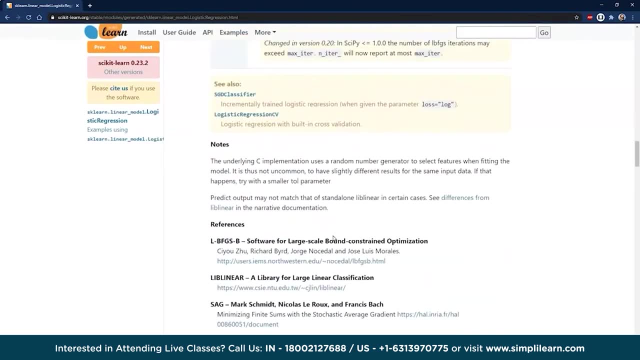 the iteration and i'll get that warning and then increase the iteration on there and, just like the other model, you go. just like you did with the other model. we can scroll down here and look for our methods and you can see there's a lot of methods in here, so i'm going to go ahead and go. 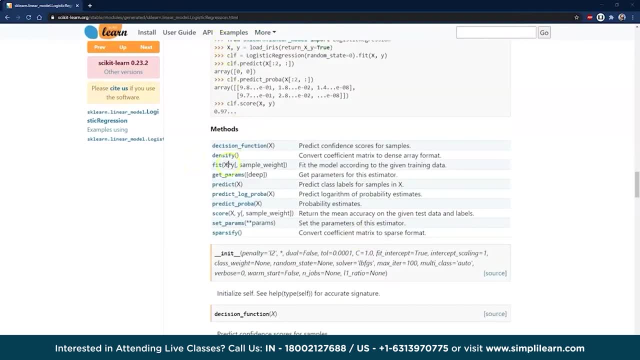 a lot of methods available on here and certainly there's a lot of different things you can do with it, but the most basic thing we do is we fit our model, make sure it's set right and then we actually predict something with it. so those are the two main things we're going to be looking at. 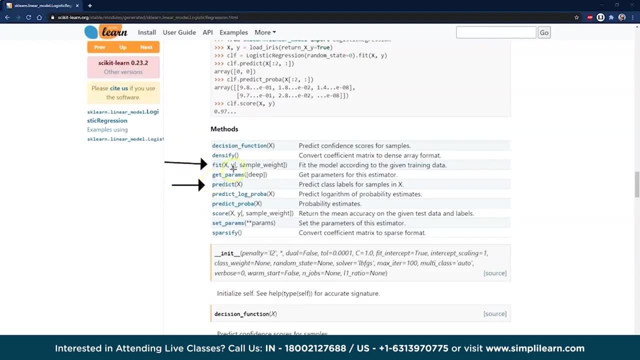 on this model is fitting and predicting. there's a lot of cool things you can do that are more advanced, but for the most part, these are the two which i use when i'm going into one of these models and setting them up. So let's go ahead and close out of our sklearn setup on there. 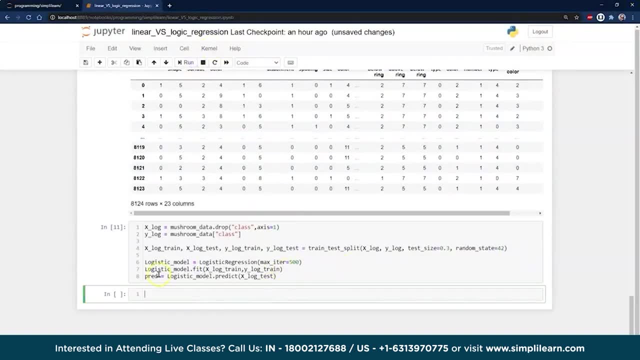 And we'll go ahead and run this And you can see here it's now loaded this up there. We now have a logistic model And we've gone ahead and done a predict here also, just like I was showing you earlier. So here is where we're actually predicting the data. 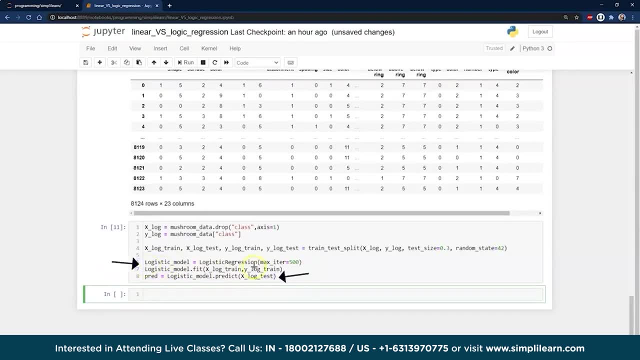 So we've done our first two lines of code. as we create the model, We fit the model to our training data And then we go ahead and predict for our test data. Now, in the previous model we didn't dive into the test score. 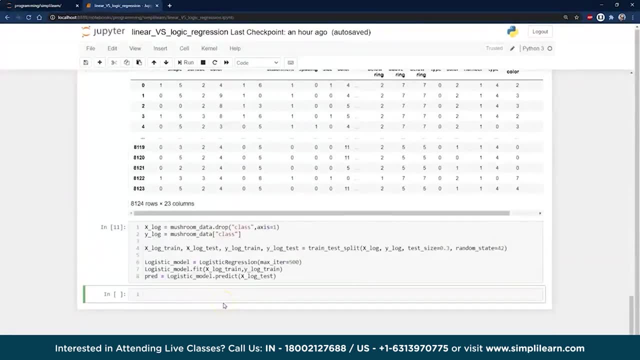 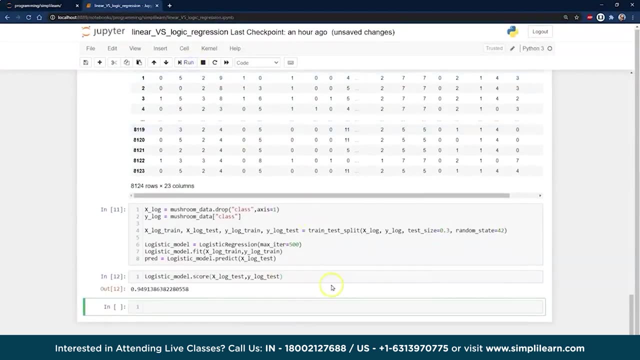 I think I just showed you a graph And we can go in there and there's a lot of tools to do this. We're going to look at the model score on this one And let me just go ahead and run the model score. 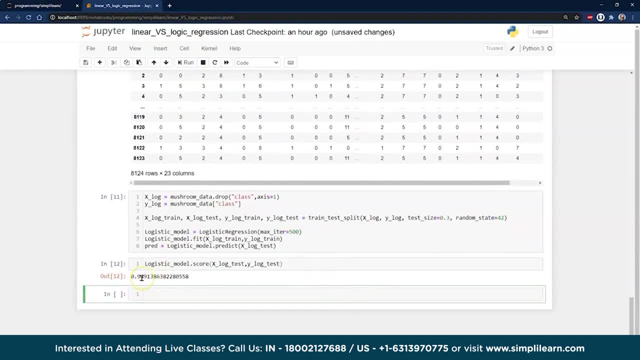 And it says that it's pretty accurate. We're getting roughly 95% accuracy. Wow, that's good 95% accuracy. 95% accuracy might be good for a lot of things, But when you look at something as far as whether you're going to pick a mushroom, 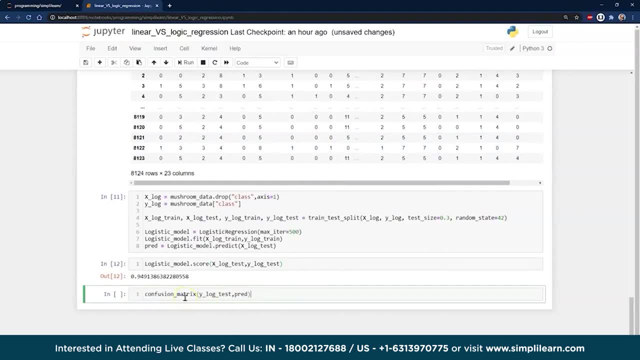 on the side of the trail and eat it. we might want to look at the confusion matrix And for that we're going to put in our Y logistic test the actual values of edible and unedible And we're going to put in our prediction value. 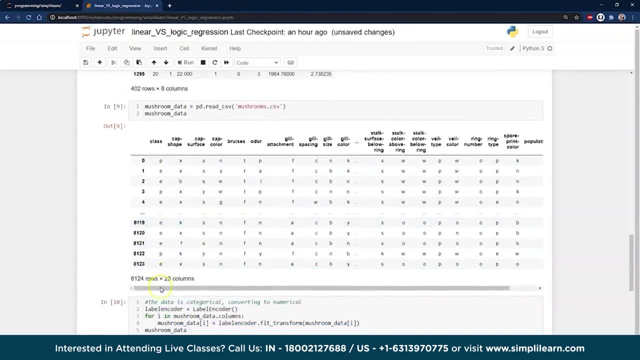 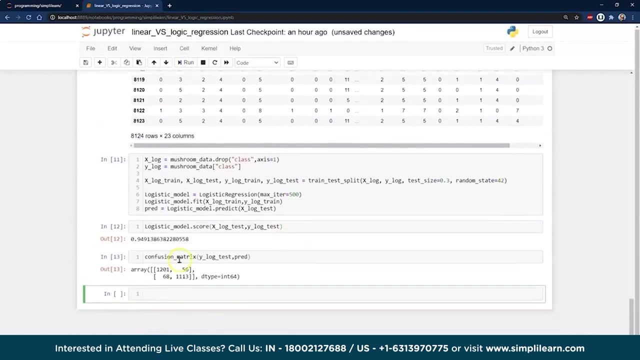 And if you remember on here, let's see- I believe it's poisonous- was one Zero is edible, So let's go ahead and run that zero. one Zero is good, Zero is good. So here is a confusion matrix. 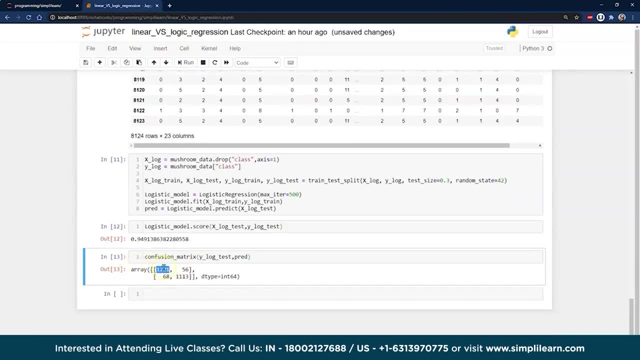 And this is if you're not familiar with these- we have true, true, true, false, true, false, false, false. So it says, out of the edible mushrooms we correctly labeled, 1,201 mushrooms edible that were edible. And we correctly measured 1,113 poisonous mushrooms as poisonous. But here's the kicker: I labeled 56 edible mushrooms as being poisonous. Well, that's not too big of a deal, We just don't eat them. But I measured 68 mushrooms as being edible that were poisonous. 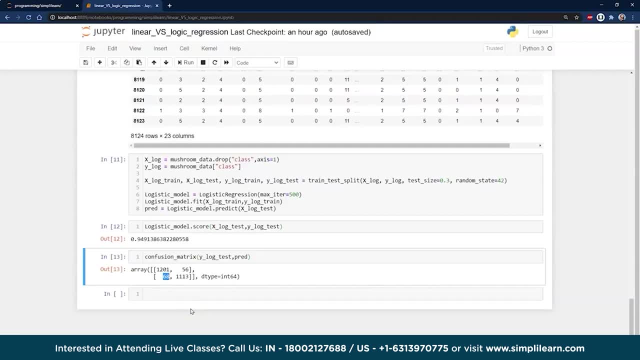 So probably not the best choice to use this model to predict whether you're going to eat a mushroom or not, And you'd want to dig a little deeper before you start picking mushrooms off the side of the trail. So a little warning there When you're looking at any of these. 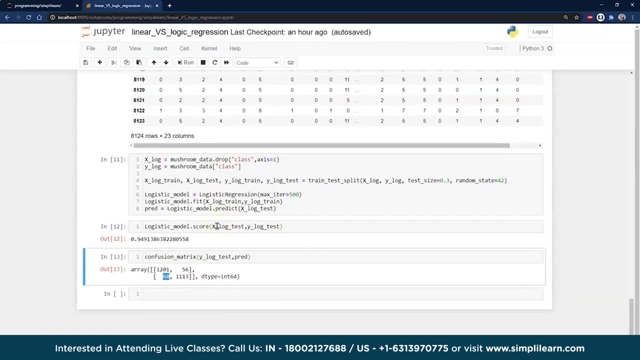 these data models, looking at the error and how that error fits in with what domain you're in, domain in this case being edible mushrooms. be a little careful, make sure that you're looking at them correctly. So we've looked at edible or not edible. 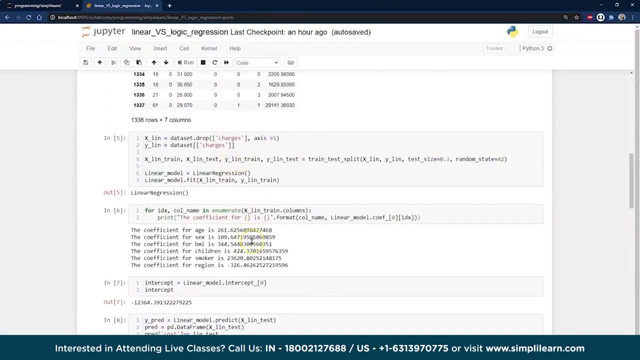 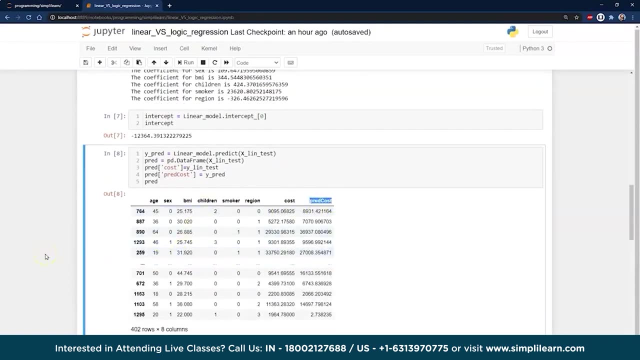 We've looked at a regression model as far as the end values, what's going to be the cost and what our predicted cost is, So we can start figuring out how much to charge these people for their insurance. And so these really are the fundamentals of data science when you pull them together. when I say data science, 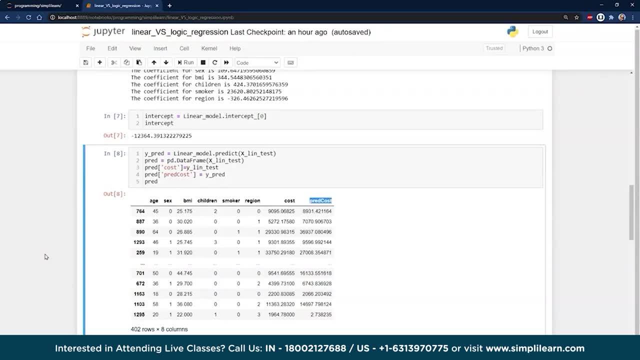 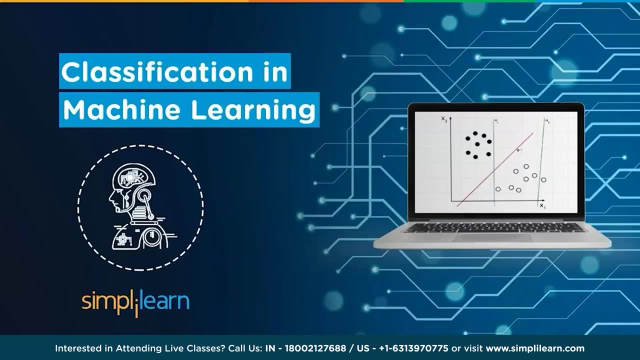 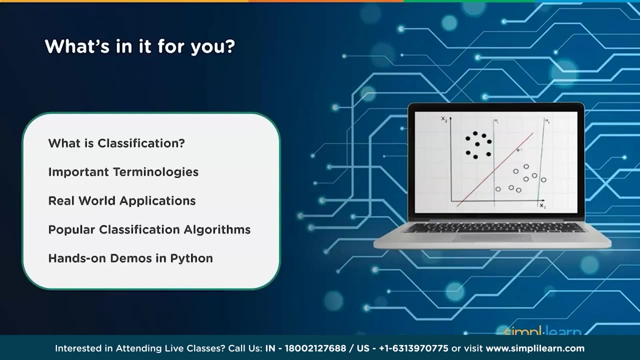 talk about your machine learning code and hopefully you got a little. classification is probably one of the most widely used tools in machine learning in today's world. It is also one of the simpler versions to start understanding how a lot of machine learning works. We're going to start by taking a look at what exactly is classification. 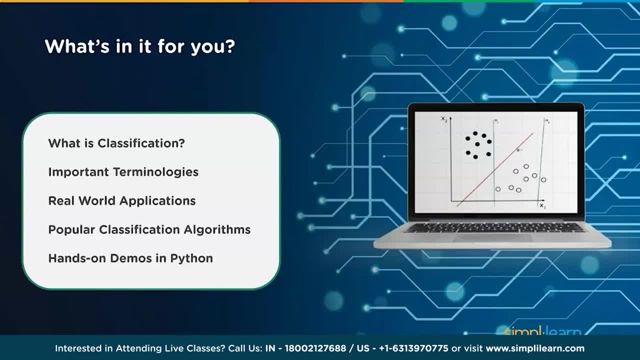 The important terminologies around classification. We'll look at Some real world applications, my favorite popular classification algorithms- and there are a lot out there, so we're only going to touch briefly on a variety of them so you can see how the different flavors work. 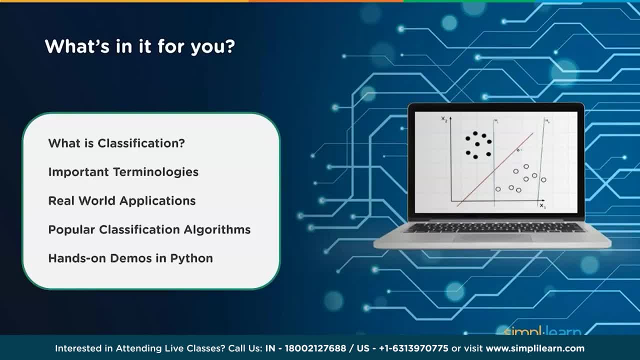 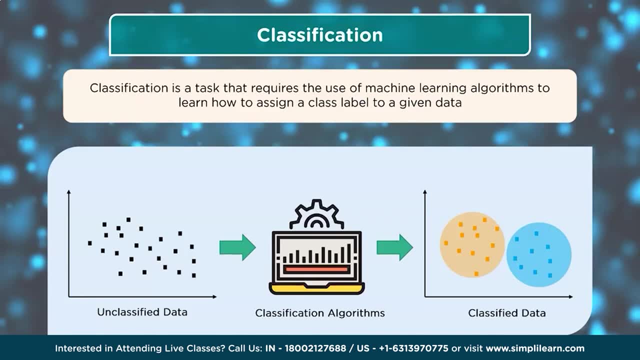 And we'll have some hands on demos in python embedded throughout the tutorial: classification Classification is a task that requires the use of machine learning algorithms to learn how to assign a class label to a given data. You can see in this diagram we have our unclassified 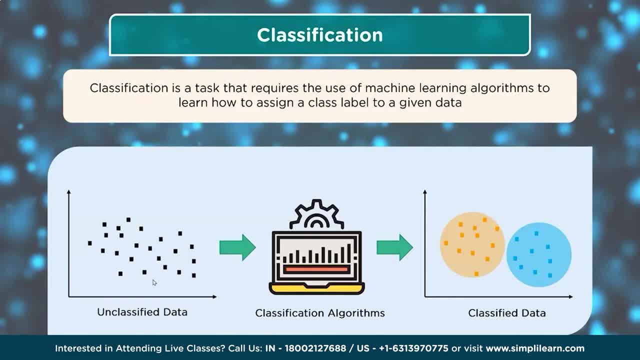 unclassified. unclassified data that goes through a classification algorithms and then you have classified data. It's hard to just see it as data and that really is where you kind of start and where you end when you start running these machine learning algorithms. and classification and the classification algorithms is a little black box in a lot of respects and we'll look into that. 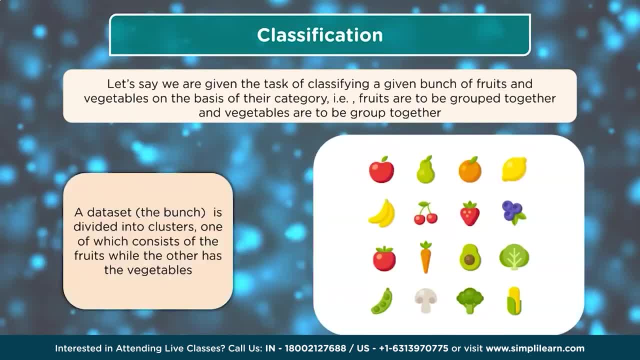 You can see what I'm talking about when we start swapping in and out different models. Let's say, we are given the task of classifying a given bunch of fruits And vegetables on the basis of their category I. fruits are to be grouped together and vegetables are to be grouped together. 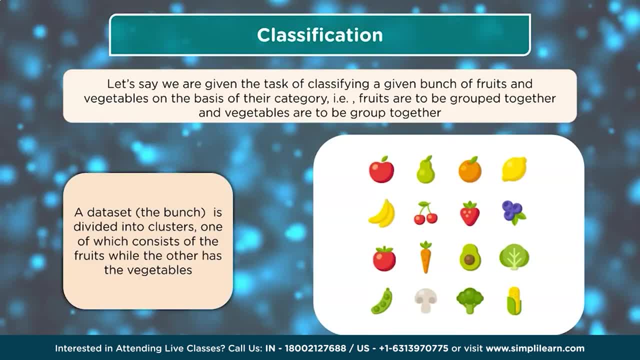 And so we have a data set. We'll call it. the bunch is divided into clusters, one of which consists of the fruits, while the other has the vegetables. You can actually look at this as any kind of data When we talk about breast cancer. 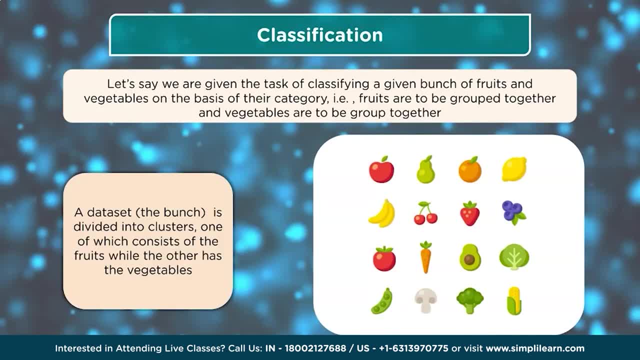 can we sort out in images to see what is malignant, What is benign? Very popular one. Can you classify flowers, The iris data set, Certainly in wildlife. can you classify different animals and track where they're going? Classification is really the bottom starting point or the baseline for a lot of machine learning and setting it up and trying to figure out how we're going to break the data up so we can use it in a way that is beneficial. 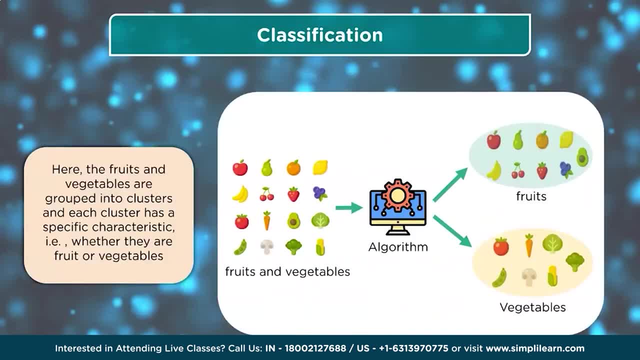 So here the fruits and the vegetables are grouped into clusters and each clusters has a specific characteristic, ie whether they are a fruit or a vegetable, And you can see we have a pile of fruits and vegetables. We feed it into the algorithm. 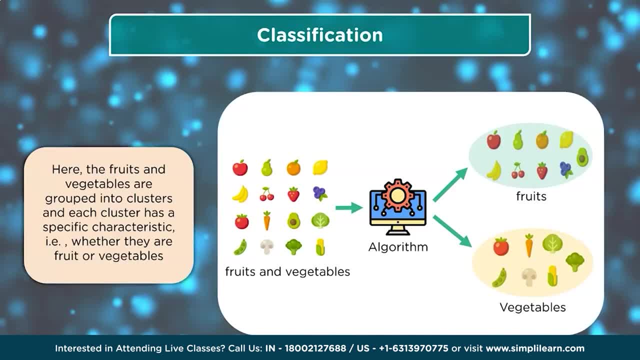 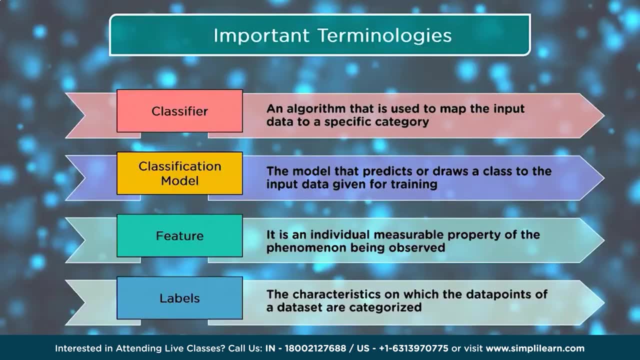 And the algorithm separates them out and you have fruits and vegetables. So some important terminologies before we dig into how it sorts them out and what that all means. When we look at the terminologies, you have a classifier. That's the algorithm that is used to map the input data to a specific category. 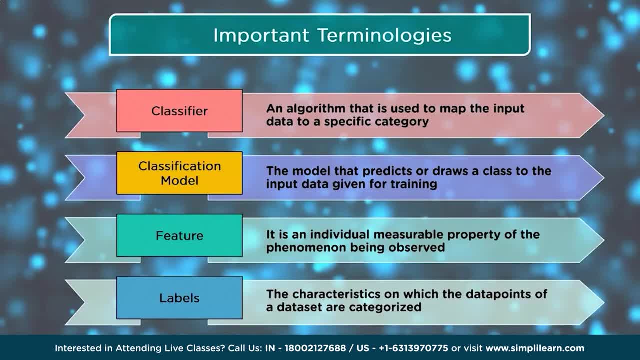 The classification model, The model that predicts or draws a class to the input data given for training Feature. It is an individual measurable property of the phenomena being observed And labels The characteristics on which the data points of a data set are categorized. 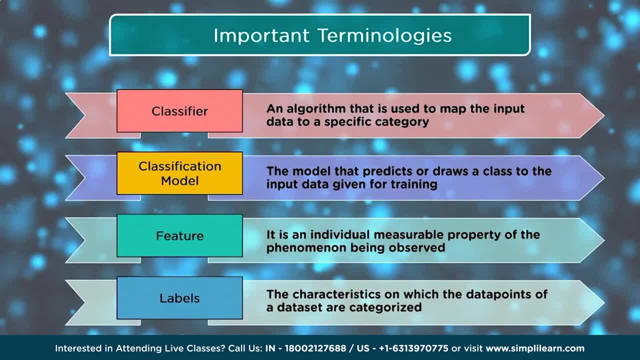 The classifier and the classification model go together. A lot of times the classifier is part of the classification model And then you choose which classifier you use after you choose which model you're using. Where features are what goes in, labels are what comes out. 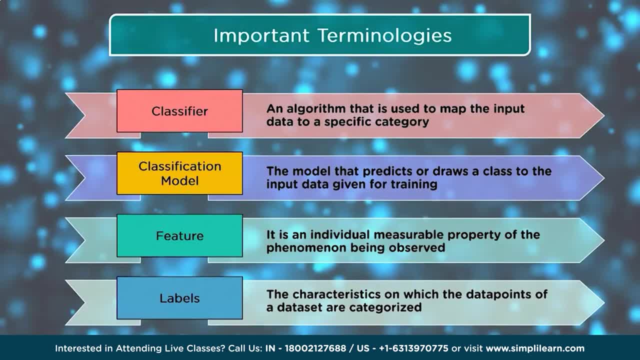 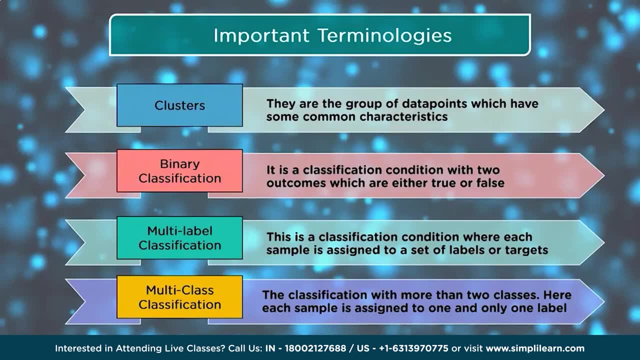 So your classifier model is right in the middle of that. That's that little black box we were just talking about Clusters. They are a group of data points which have some common attributes, Characteristics. Binary classification: It is a classification condition with two outcomes, which are either true or false. 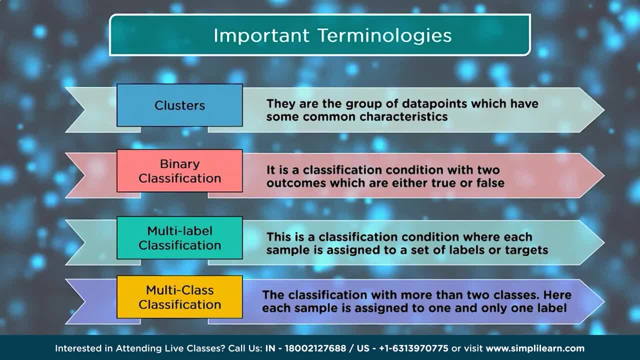 Multi-label classification: This is a classification condition where each sample is assigned to a set of labels or targets. Multi-class classification: The classification with more than two classes. Here, each sample is assigned to one and only one label. When we look at this group of terminologies, 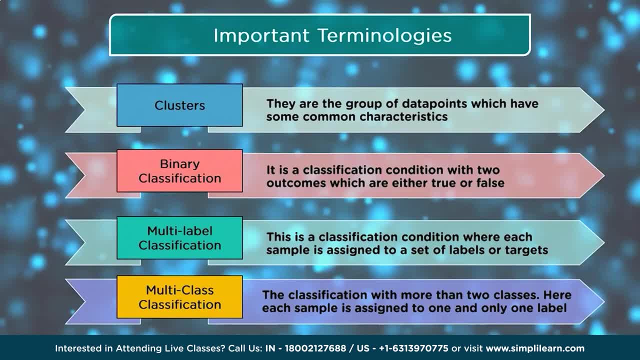 A few important things to notice Going from the top Clusters. When we cluster data together, we don't necessarily have to have an end goal. We just want to know what features cluster together. These features, then, are mapped to the outcome we want. 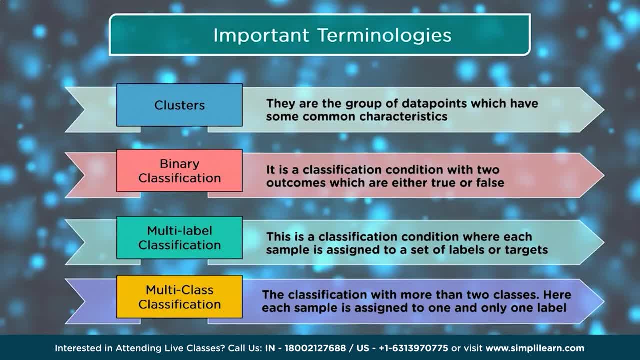 In many cases, the first step might not even care about the outcome, Only about what data connects with other data, And there's a lot of clustering algorithms out there that do just the clustering part. Binary classification: It is a classification condition with two outcomes, which are either true or false. 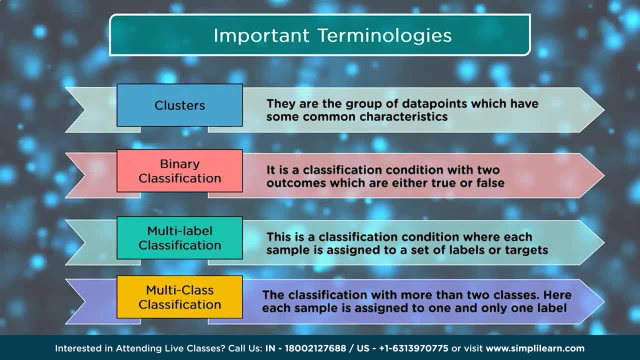 We're talking. usually it's either a cat or it's not a cat. It's either a dog or it's not a dog. That's the kind of thing we talk about, binary classification, And then that goes into multi-label classification. Think of label, as you can have an object that is brown. 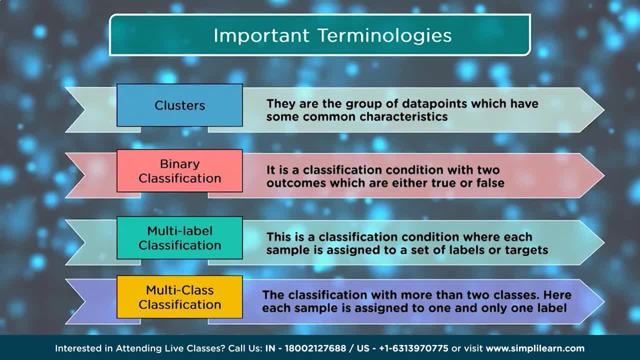 You can have an object that is labeled as a dog, So it has a number of different labels. That's very different than a multi-class classification where each one is a binary. You can either be a cat or a dog. You can't be both a cat and a dog. 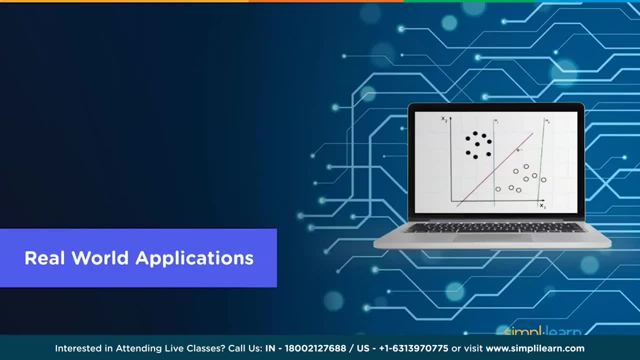 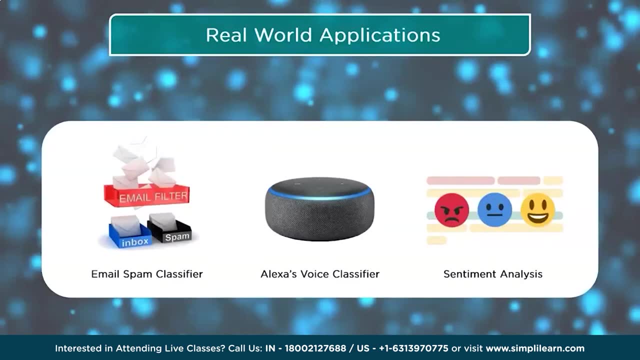 Real world applications. So to make sense of this, of course, the challenge is always in the details- Is to understand how we apply this in the real world. So in real world applications, we use this all the time. We have email spam classifier, So you have your email inbox coming in. 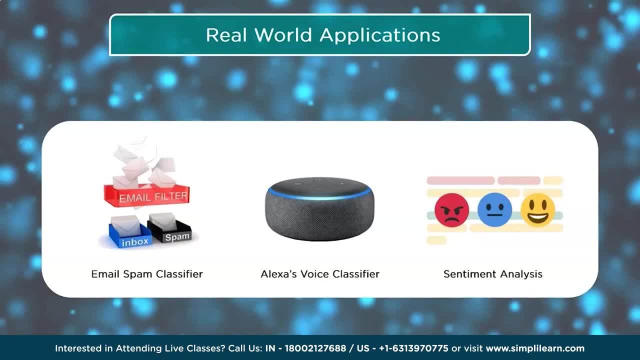 It goes through the email filter that we usually don't see in the back And it goes: this is either valid email or it's a spam And it puts it in the spam filter if that's what it thinks it is. Alexa's voice classifier. 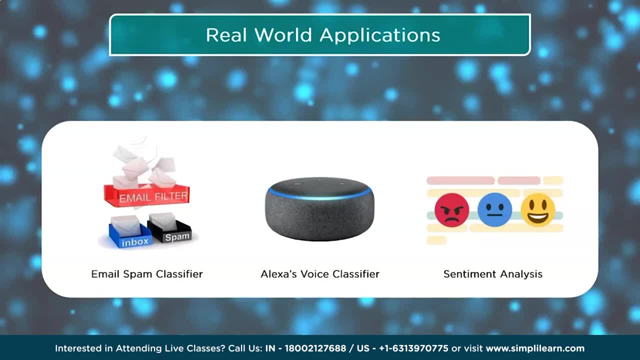 Google voice Any of the voice classifiers. they're looking for points, So they try to group words together And then they try to find those groups of words trigger a classifier. So it might be that the classifier is to open your tasks program Or open your text program. 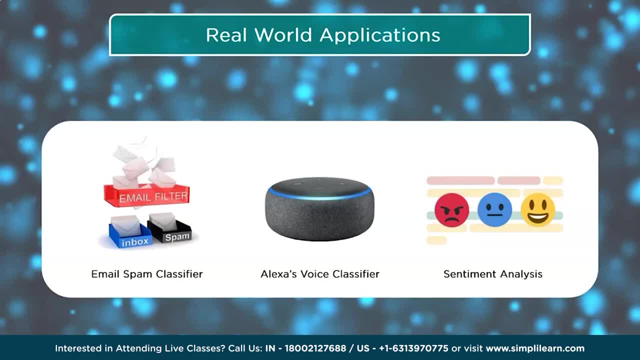 So that you can start sending a text. Sentiment analysis is really big When we're tracking products. We're tracking marketing. Trying to understand whether something is liked or disliked is huge. That's like one of the biggest driving forces in sales nowadays. 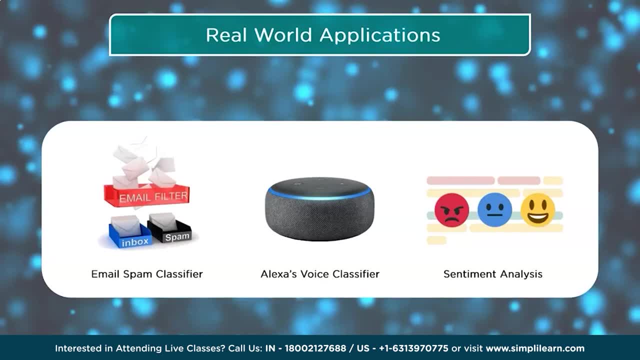 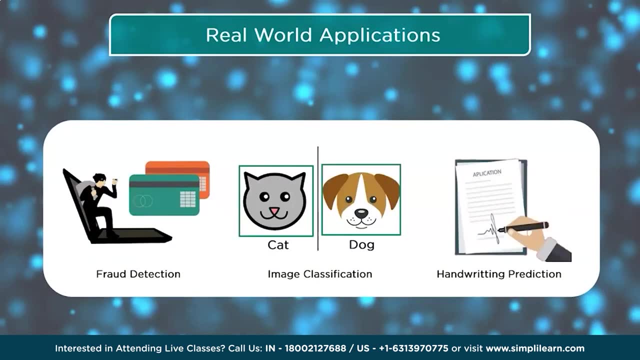 And you almost have to have these different filters going on. If you're running a large business of any kind, Fraud detection- You can think of banks. They find different things on your bank statement And they detect that there's something going on there. 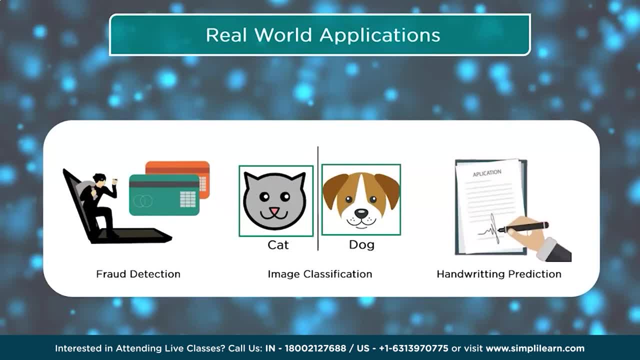 They have algorithms for tracking the logs on computers. They start finding weird logs on computers. They might find a hacker. I mentioned cat and dog, So here's our image classification. We have a neighbor who runs an outdoor webcam And we like to have it come up with a classification when the wild animals in our area are out. 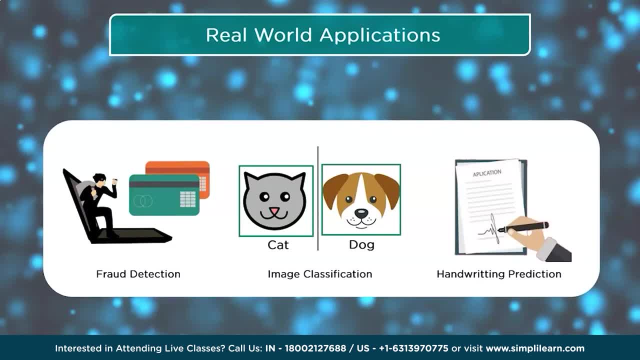 Like foxes. We actually have a mountain lion that lives in the area, So it's nice to know when he's here. Handwriting prediction Classifying A, B, C, D And then classifying words to go with that. 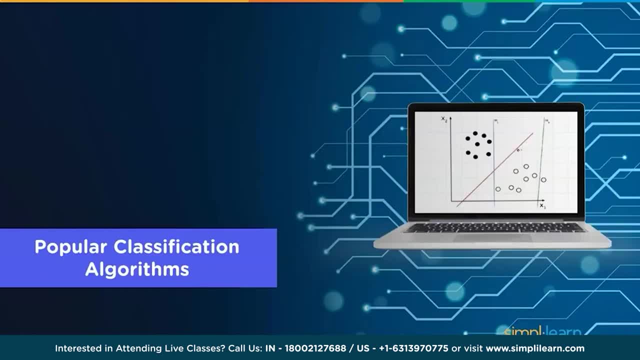 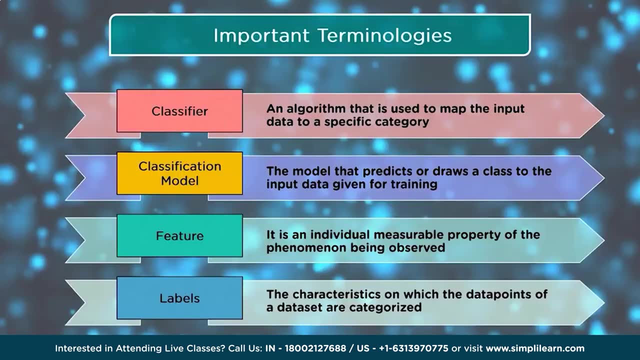 So let's go ahead and roll our sleeves up And take a look at some popular classification algorithms. Before we look at the algorithms, Let's go back and take a look at our definitions. We have a classifier and a classification model, So we're looking at the classifier. 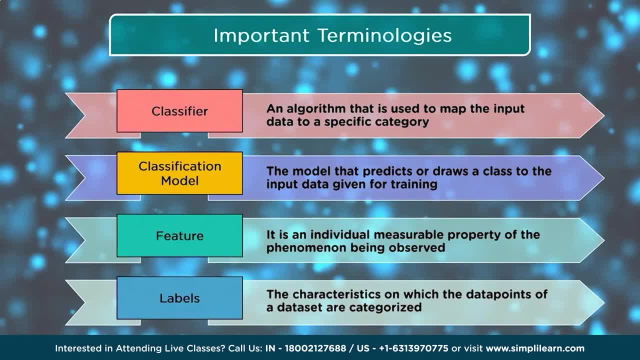 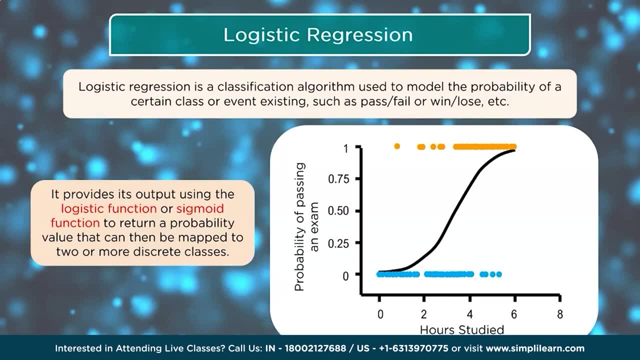 An algorithm that is used to map the input data to a specific category. One of those algorithms is a logistic regression. The logistic regression is a classification algorithm used to model the probability of a certain class or event existing, Such as pass, fail Or win, lose, etc. 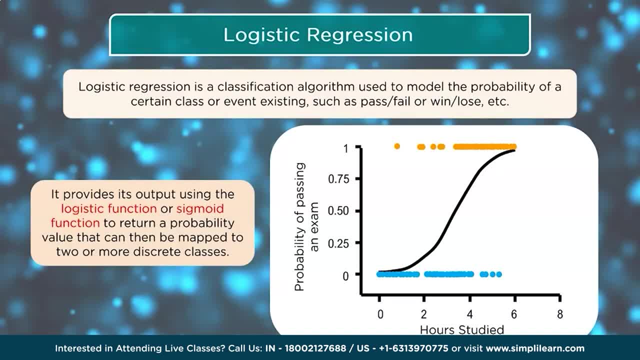 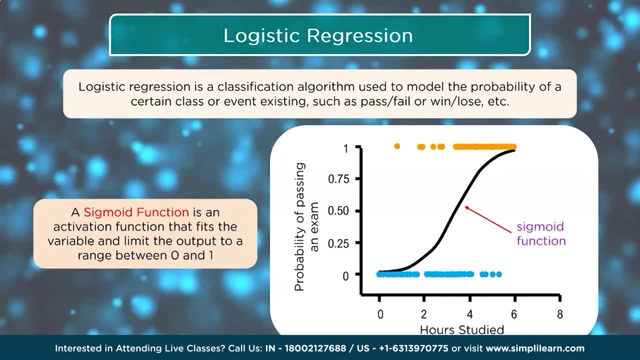 It divides its output using the logistic function or sigmoid function to return the probability value. that can then be mapped to two or more discrete classes. A sigmoid function is an activation function that fits the variable and limits the output to a range between 0 and 1.. 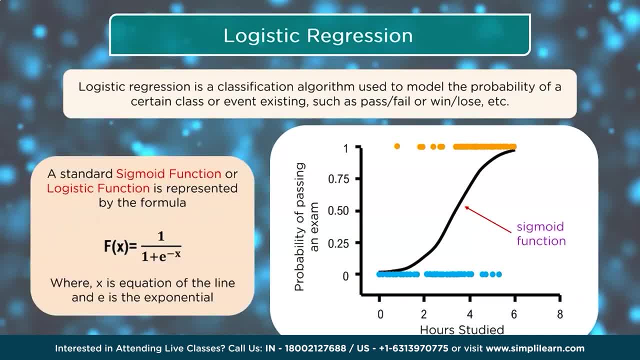 A standard sigmoid function or logistic function is represented by the formula: fx equals 1 over 1 plus e to the minus x, Where x is the equation of the line and e is the exponential. Just taking a quick look at this, You can think of this as being a point of uncertainty. 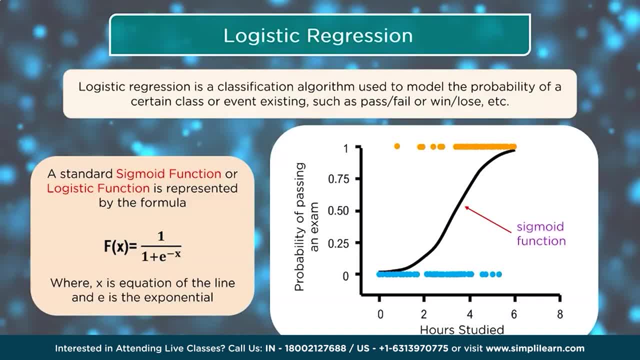 And so as we get closer and closer to the middle of the line, It's either activated or not, And we want to make that just shoot way up, So you'll see a lot of the activation formulas kind of have this nice s-curve. 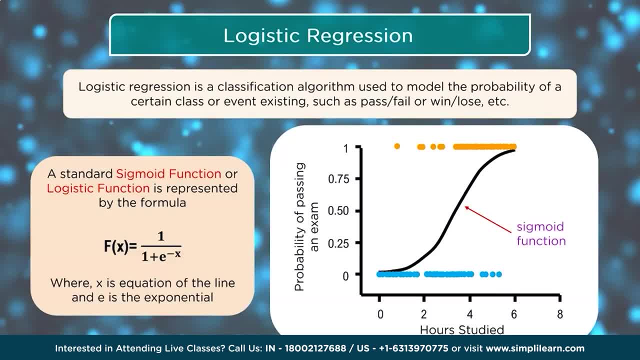 Where it approaches 1 and approaches 0. And based on that, there's only a small region of error. And so you can see in the sigmoid logistic function The 1 over 1 plus e minus x to the minus x. You can see it frames that nice s-curve. 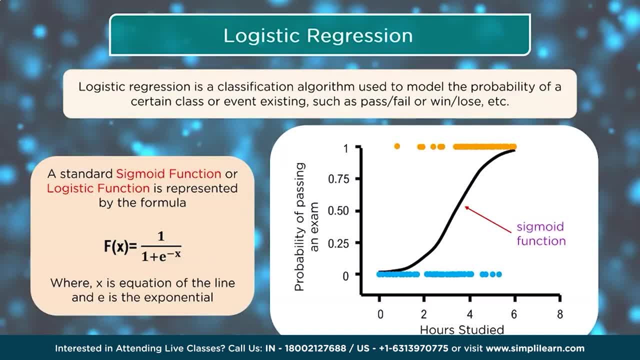 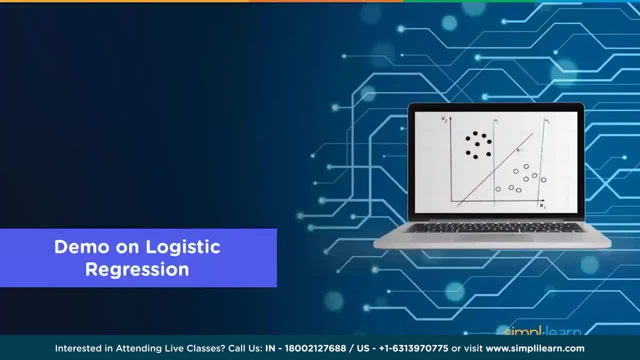 We also can use a tangent variation. There's a lot of other different models here. as far as the actual algorithm, This is the most commonly used one. Let's go ahead and roll up our sleeves and take a look at a demo that is going to use a logistic regression. 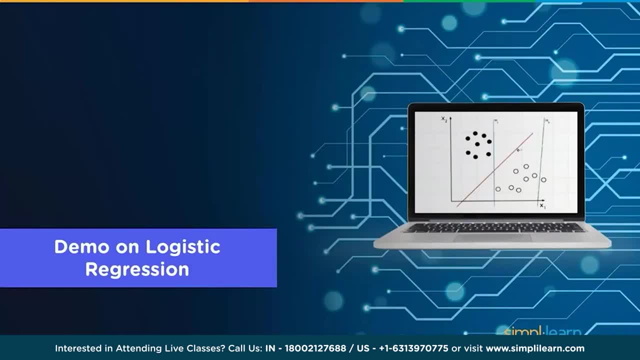 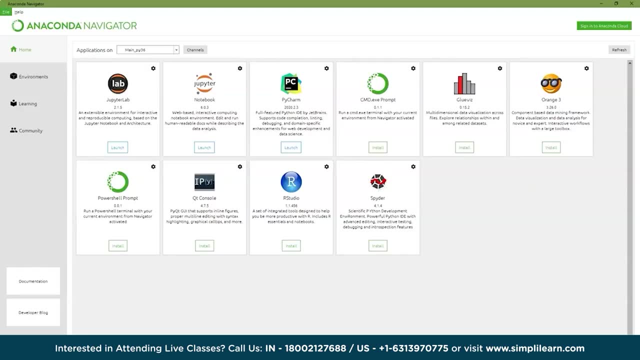 So we're going to have the activation formula and the model, Because you have to have both. For this we will go into our Jupyter notebook Now. I personally use the Anaconda Navigator to open up the Jupyter notebook To set up my IDE as a web-based. 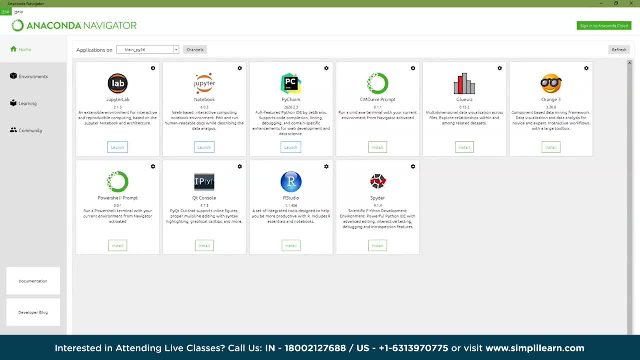 It's got some advantages that it's very easy to display in, But it also has some disadvantages in that if you're trying to do multi-threads and multi-processing, You start running into single git issues with Python. And then I jump to PyCharm. 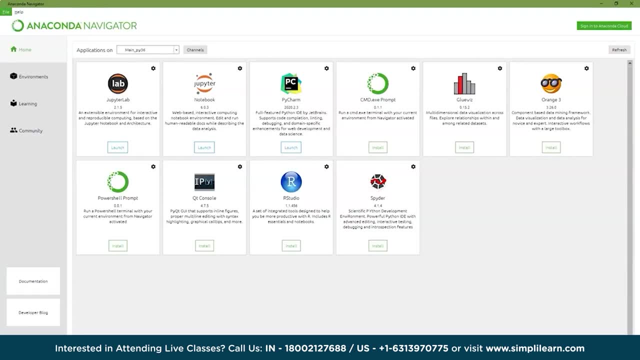 It really depends on whatever IDE you want. Just make sure you've installed NumPy and the sklab So that you can actually learn modules into your Python In whatever environment you're working in, So that you'll have access to that for this demo. 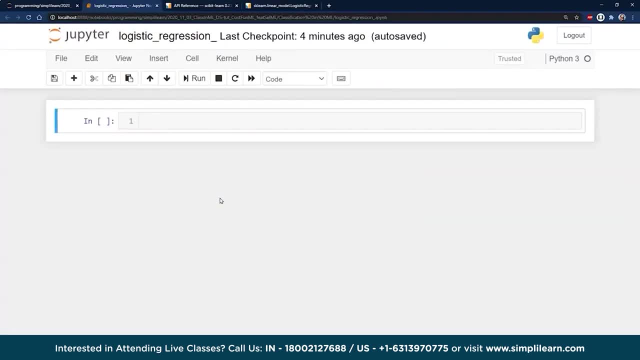 Now the team in the back has prepared my code for me, Which I'll start bringing in one section at a time So we can go through it Before we do that. It's always nice to actually see where this information is coming from. 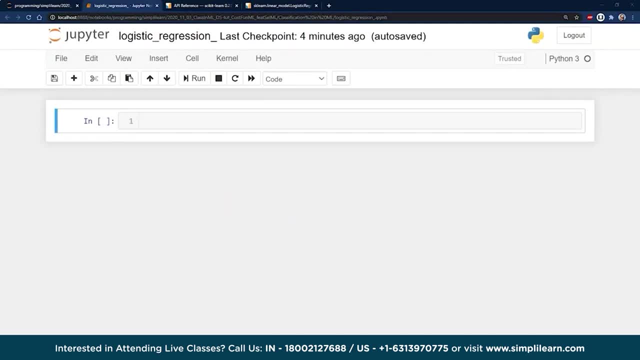 And what we're working with. So the first part is we're going to import our packages, Which you need to install into your Python, And that's going to be your NumPy. We usually use NumPy as in P From sklearn. 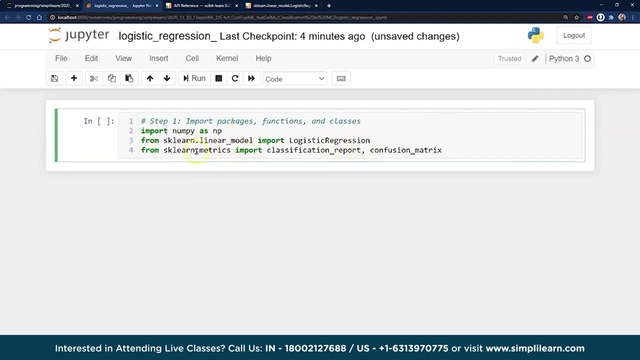 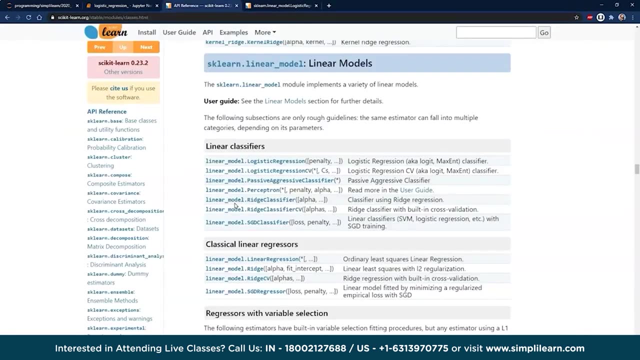 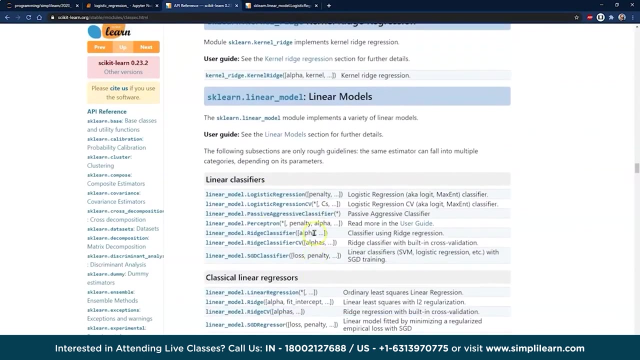 The learn model We're going to use a logistic regression And from sklearn metrics We're going to import the classification report, confusion, matrix. And if we go ahead and open up the scikit-learnorg And go under their API, You can see all the different features and models they have. 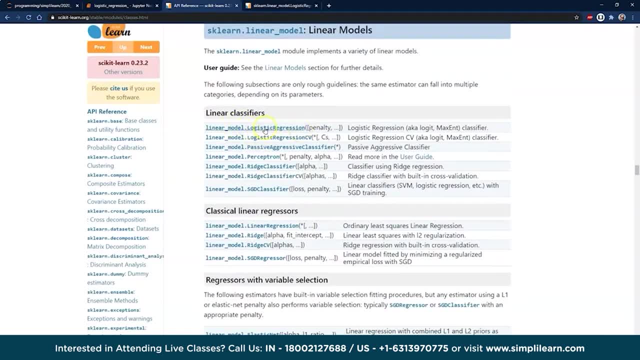 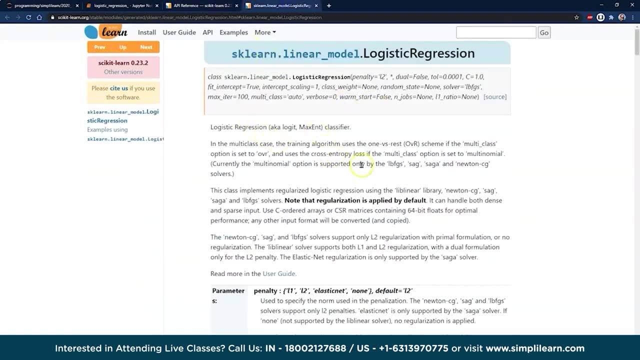 And we're looking at the linear model, logistic regression, One of the more common classifiers out there, And if we go ahead and go into that And dig a little deeper, We'll see here where they have the different settings And it even says right here: 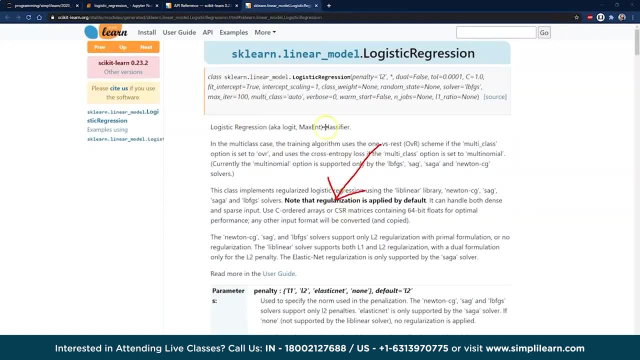 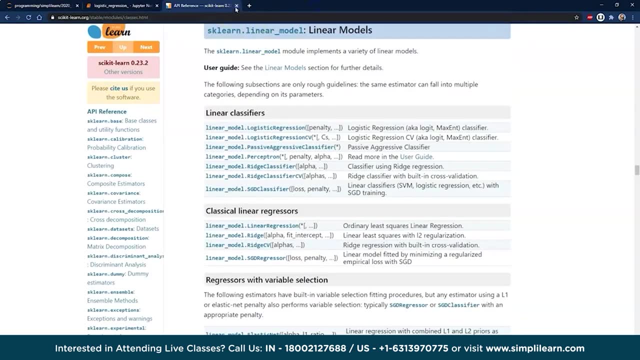 Note: the regularization is applied by default, So by default, that is the activation formula being used. Now we're not going to spend. We might come back to this. Look at some of the other models, Because it's always good to see what you're working with. 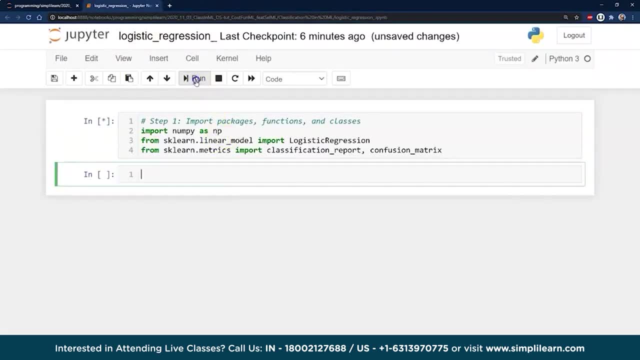 But let's go ahead and jump back in here And we have our imports. We're going to go ahead and run those. So these are now available to us As we go through our Jupyter notebook script And they put together a little piece of data for us. 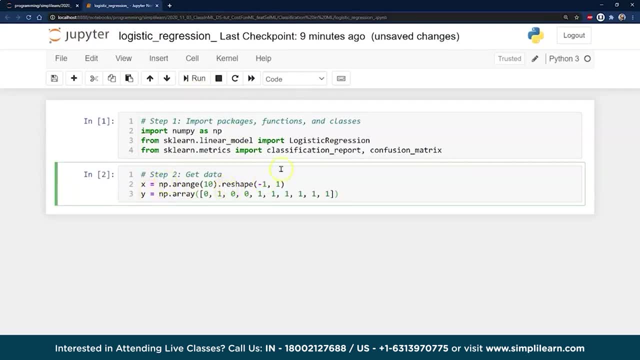 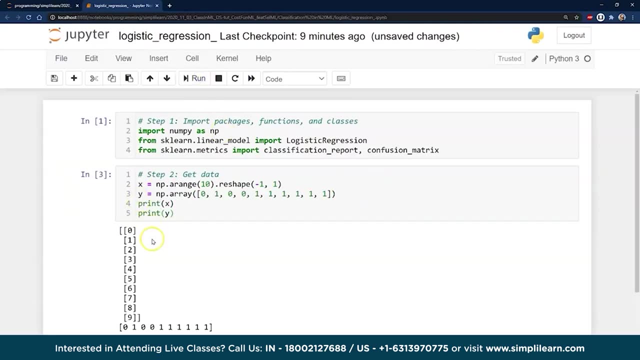 This is simply Going through 0 to 1.. Actually, let's go ahead and print this out over here. We'll go ahead and print x, Just so you can see what we're actually looking for And when we run this, You can see that we have our x is 0,, 1, 2 through 9.. 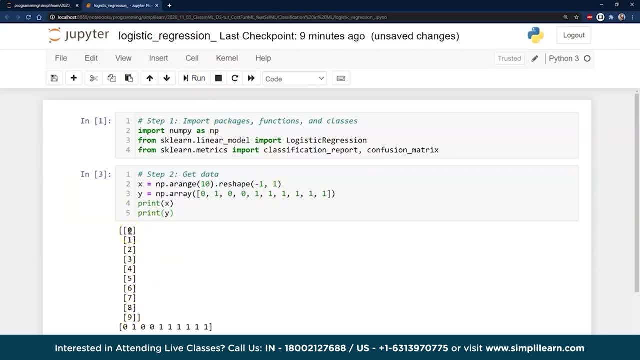 We reshaped it. The reason for this is just looking for a row of data. Usually we have multiple features. We just have the one feature, which happens to be 0 through 9.. And then we have our 10 answers right down here. 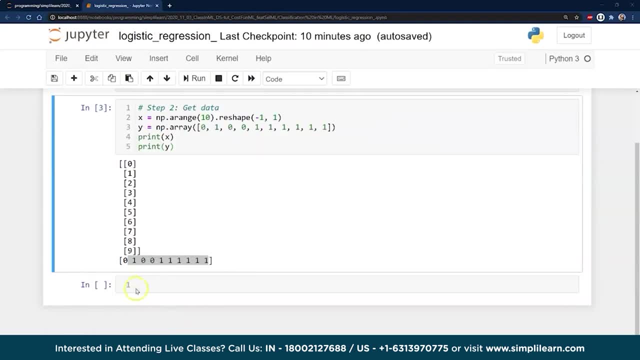 0, 1, 0, 0, 1, 1, 1, 1, 1, 1.. Bring in a lot of different data. depending on what you're working with, You can make your own. 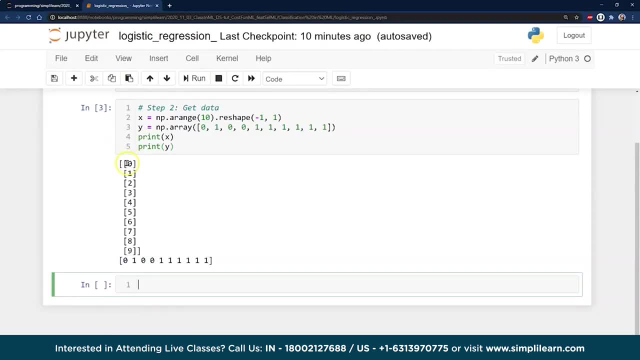 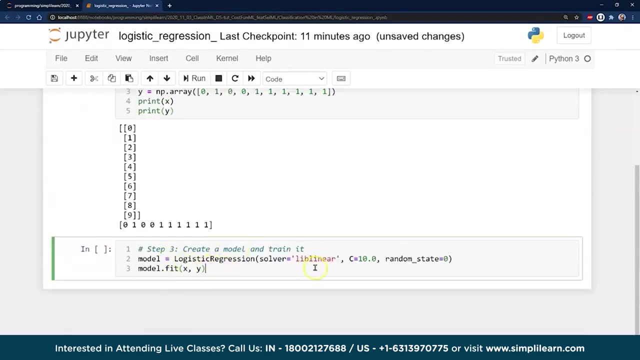 You can. instead of having this as just a single, You could actually have like multiple features in here, But we just have the one feature for this particular demo, And this is really where all the magic happens, right here, And I told you, it's like a black box. 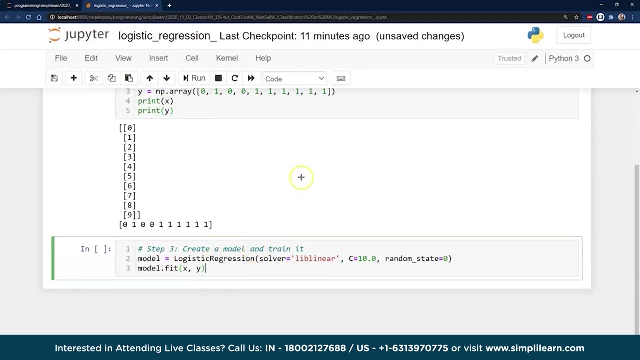 That's the part that is kind of hard to follow, And so if you look, right here We have our model, We talked about the model right there And then we went ahead and set it for library linear, Because I showed you earlier, that's actually default. 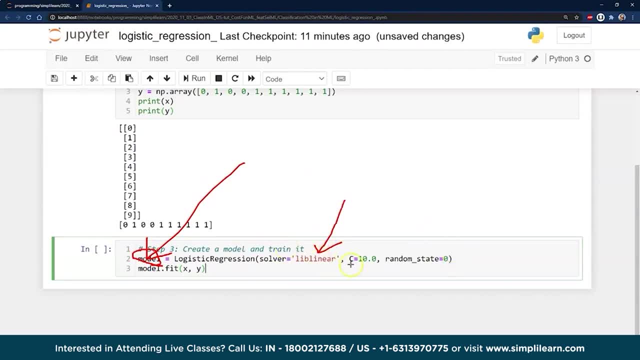 So it's not that important. Random state equals 0. This stuff you don't worry too much about And then with the scikit learn You'll see the model fit. This is very common to scikit. They use similar stuff in a lot of other different packages. 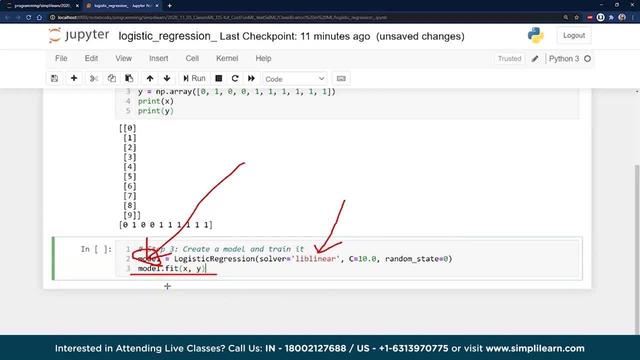 But you'll see that that's very common. You have to fit your data And that means we're just taking the data And we're fitting our x right here, Which is our features. That's our x And here's y. 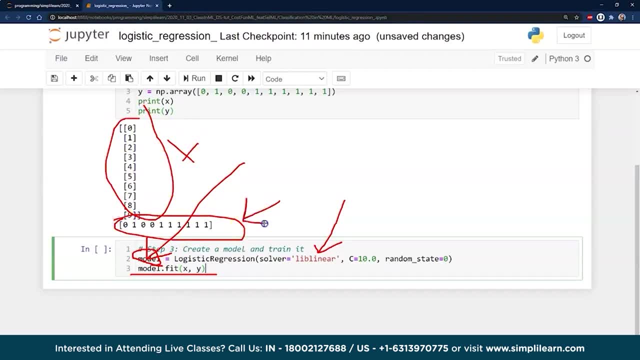 These are the labels we're looking for. So before we were looking at, Is it fraud? Is it not? Is it cat? Is it not That kind of thing? And this is looking at 0, 1.. So we want to have a binary setup on this. 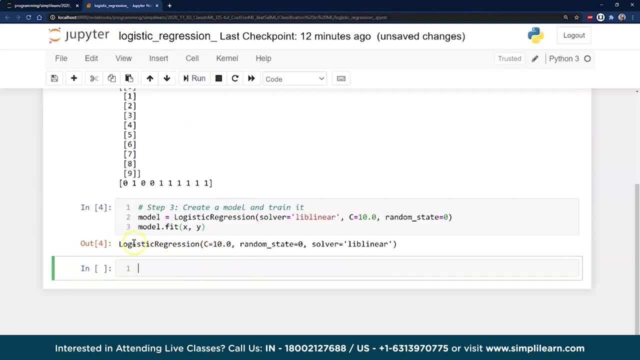 And we'll go ahead and run this. You can see right here. It just tells us what we loaded it with as our defaults And that this model has now been created And we've now fit our data to it. And then comes the fun part. 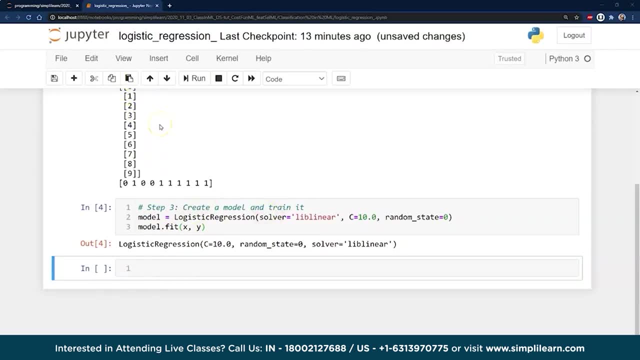 You work really hard to clean your data, To bake it and cook it. There's a lot of stuff. There's all kinds of. I don't know why they go with the cooking terms. As far as how we get this data formatted, 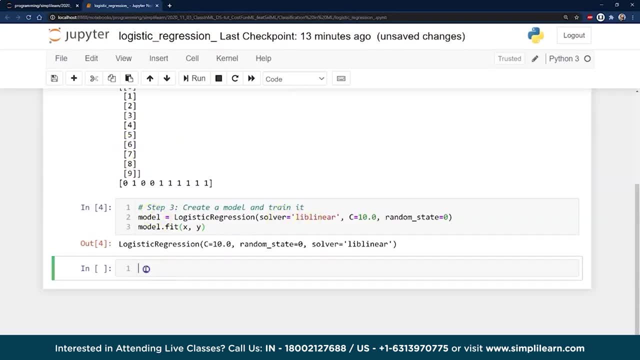 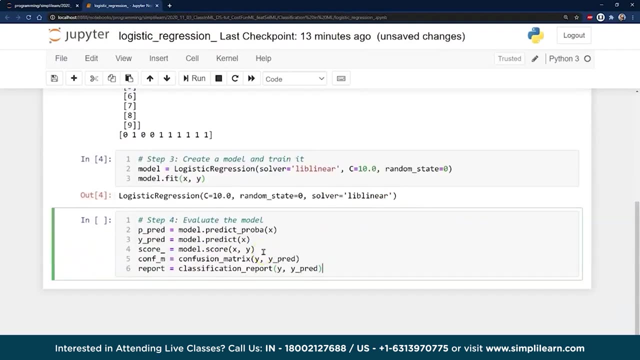 Then you go through and you pick your model, You pick your solver And you have to test it to see, Hey, which one's going to be best. And so we want to go ahead and evaluate the model, And you do this. Is that, once you've figured out which one is going to work the best for you? 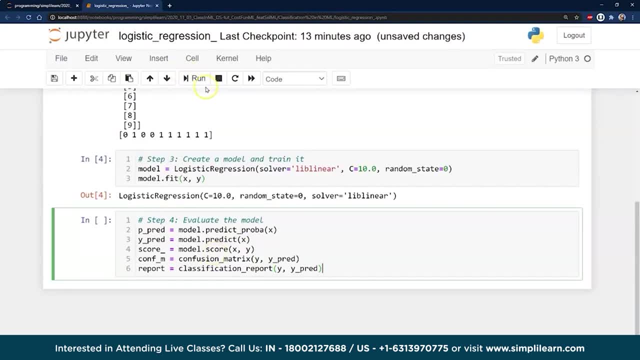 You want to evaluate it So you can compare it to your last model And you can either update it to create a new one Or maybe change the solver to something else. I mentioned tangent. That's one of the other common ones That's commonly used with language. 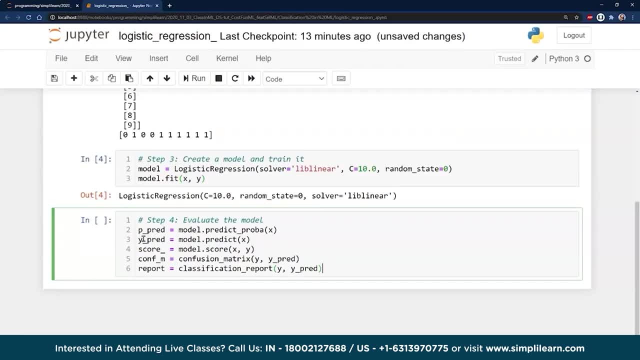 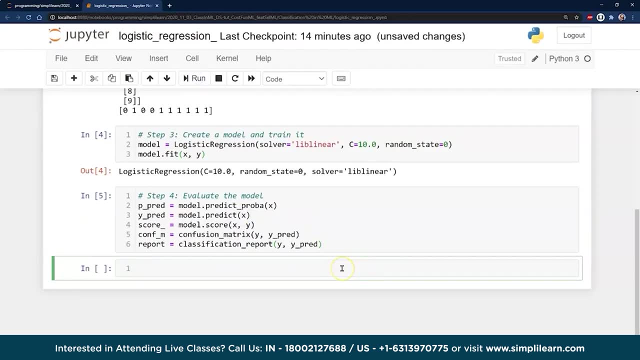 For some reason the tangent, Even though it looks almost to me identical to the one we're using With the sigmoid function. For some reason it activates better with language, Even though it's a very small shift In the actual math behind it. 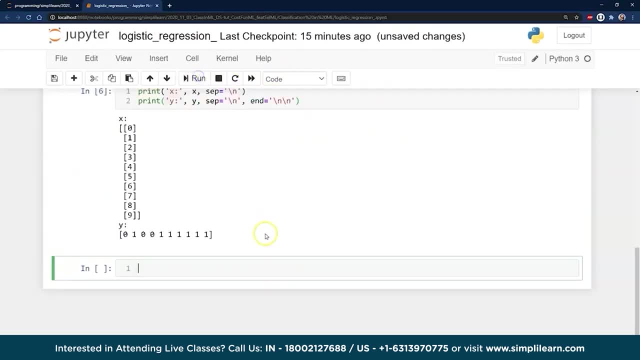 We already looked at the data early, But we'll go ahead and look at it again, Just so you can see what we look at. We have our rows of zero- It only has one entity- And we have our output that matches these rows. 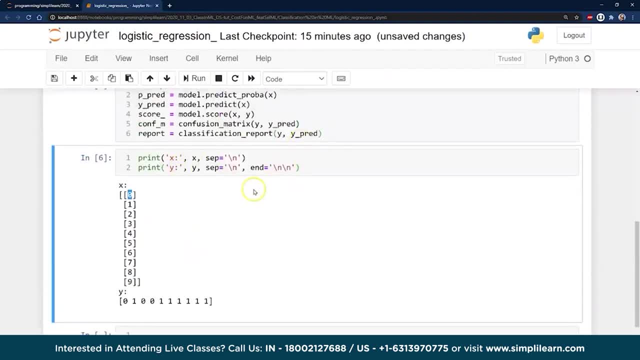 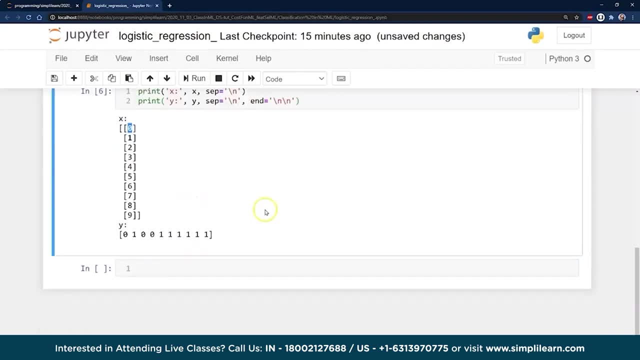 And these do have to match. You'll get an error if you put in Something with a different shape. So if you have ten rows of data and nine answers, It's going to give you an error Because you need to have ten answers for it. 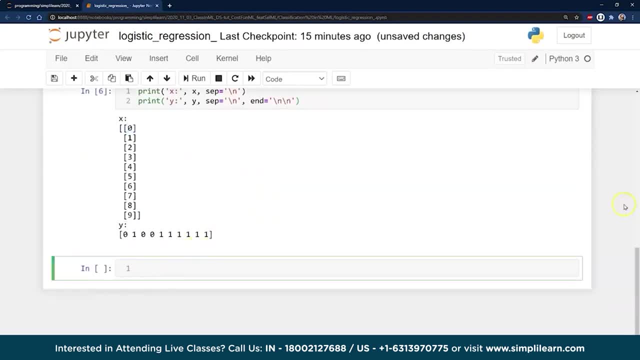 A lot of times you separate this too When you're doing larger models, But for this we're just going to take a quick look at that. The first thing we want to start looking at is the intercept, One of the features inside our linear regression model. 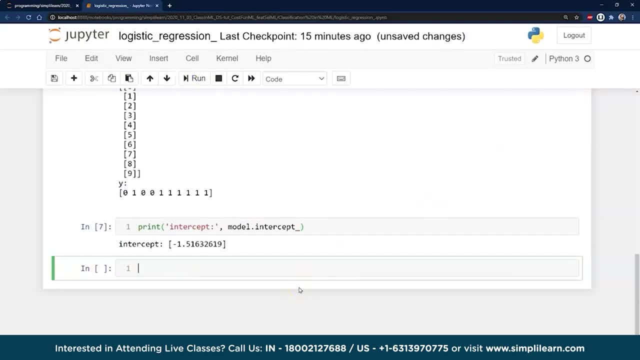 We'll go ahead and run that and print it. You'll see, here we have an intercept of minus 1.516.. And if we're going to look at the intercept, We should also look at our coefficients. And if you run that, 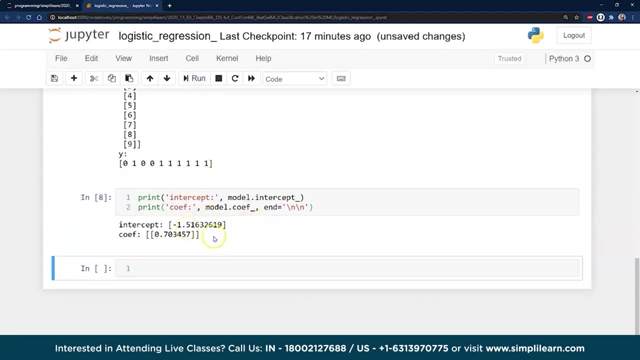 You'll see that our coefficient is the .7035.. You can just think of this as your Euclidean geometry For a very basic model like this, Where it intercepts the y at some point And we have a coefficient multiplying by it. 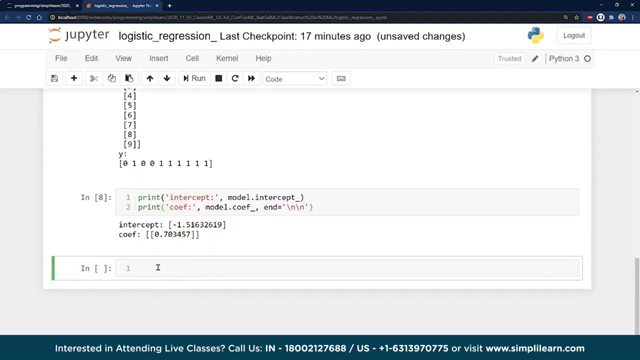 A little more complicated in the back end. But that is just this simple model With just the one feature in there, And we'll go ahead and reprint the y, Because I want to put them on top of each other With the y: predict. 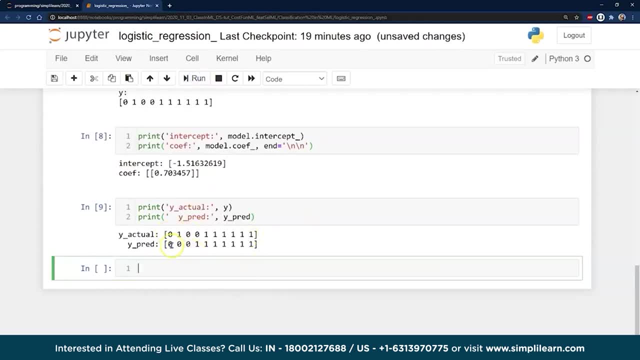 And so these were the y values we put in And this is the y predict we had coming out. And you can see, Here we go. There's the y actual And there's what the prediction comes in Now. keep in mind. 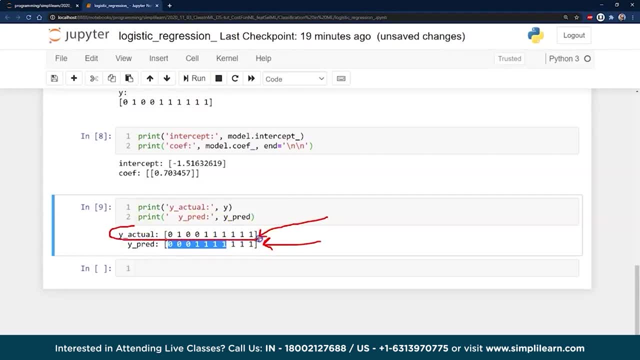 That we used the actual complete data As part of our training. That is, if you're doing a real model, A big stopper right there, Because you can't really see how good it did Unless you split some data off To test it on. 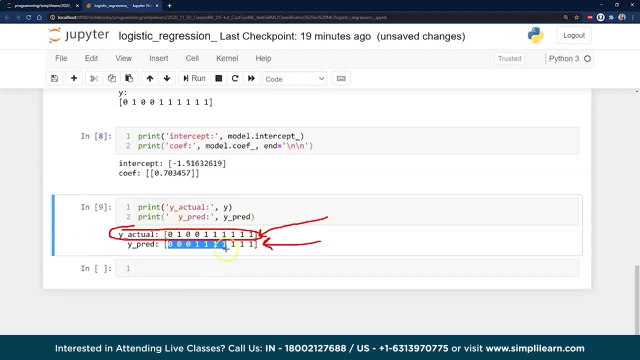 This is the first step. Is you want to see how your model actually Tests on the data you trained it with? And you can see here. There is this point right here Where it has it wrong And this point right here Where it also has it wrong. 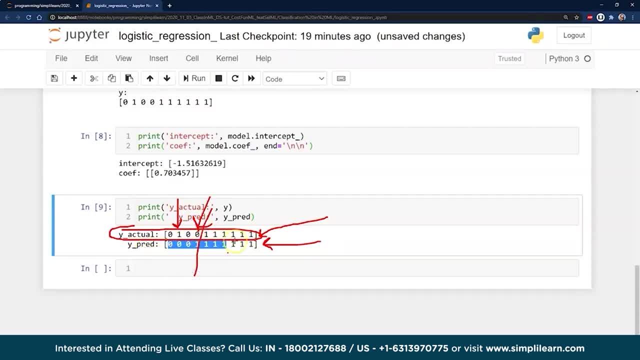 And it makes sense Because we're going, Our input is zero through nine And it has to break it somewhere, And this is where the break is. So it says this: half the data is going to be zero, Because that's what it looked like to me. 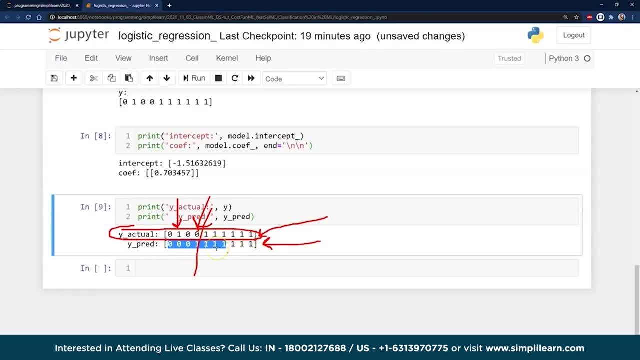 If I was looking at it Without an algorithm, And this data is probably going to be one, And I didn't. I forgot to point this out, So let's go back up here. I just kind of glanced over this window here. 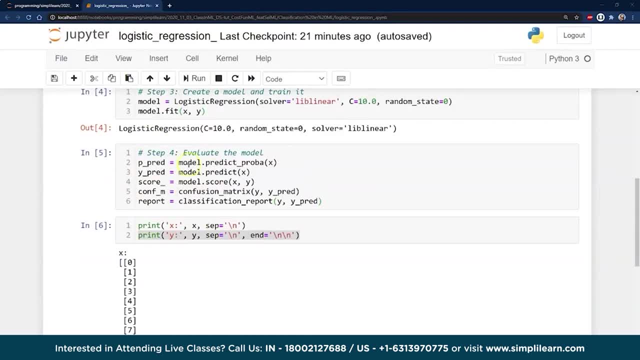 Where we did a lot of stuff. Let's go back and just take a look at that. What was done here Is: we ran a prediction, So this is where our predict comes in. Is our model dot predict? So we had a model fit. 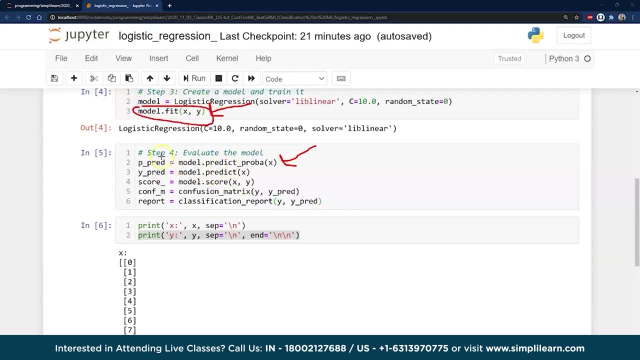 We created the model, We programmed it to give us the right answer. Now we go ahead and predict What we think it's going to be. There's our model: dot predict probability of x. And then we have our y predict, Which is very similar. 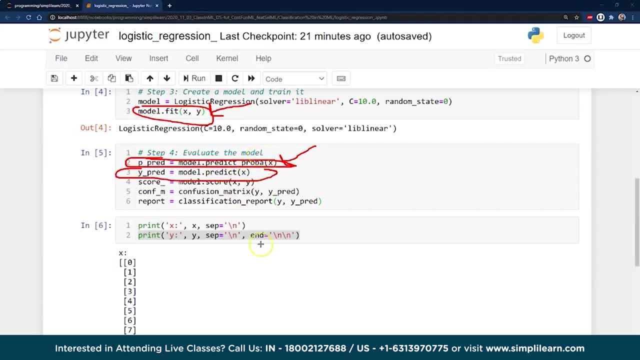 But this has to do more with the probability numbers. So, if you remember, down below We had the setup where we're looking at that sigmoid function. That's what this is returning And the y predict is returning a zero or a one, And then we have our confusion matrix. 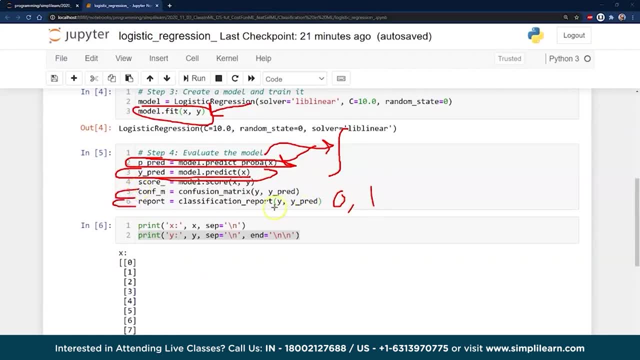 We'll look at that And we have our report Which just basically compares our y to our y predict, Which we just did. It's kind of nice. It's simple data, So it's really easy to see what we're doing. 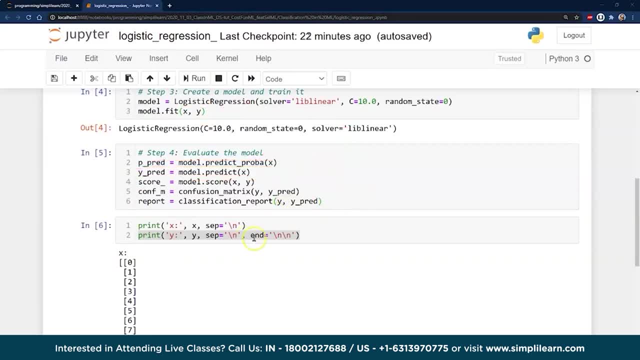 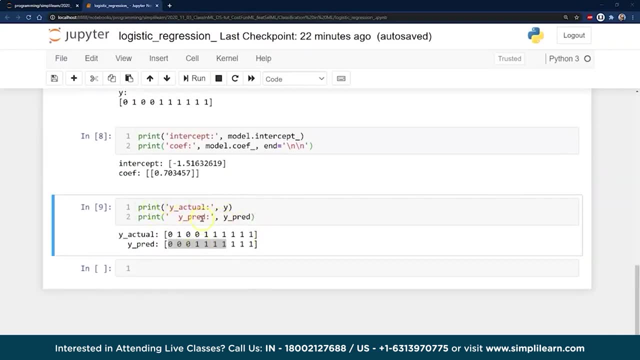 That's why we use the simple data. This can get really complicated when you have a lot of different features And things going on And splits. So here we go. We've had our. I printed out our actual and our prediction. So this is the actual data. 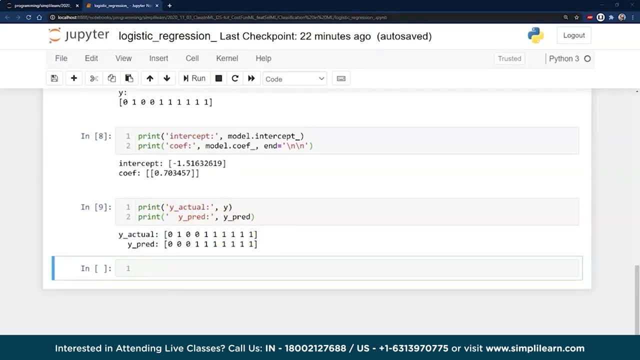 This is what the predict ran, And then we'll go ahead and do We're going to print out the confusion matrix. We were just talking about that. This is great if you have a lot of data to look at, But you can see right here. 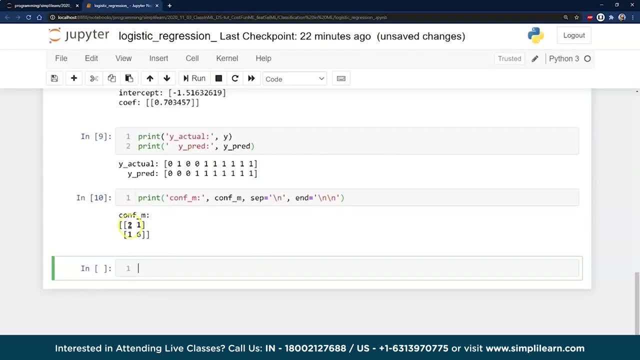 Our confusion matrix says: If you remember from the confusion matrix, We have the two. This is two, correct, One, two. And it's been a while since I looked at a confusion matrix. There's the two, And then we have this one. 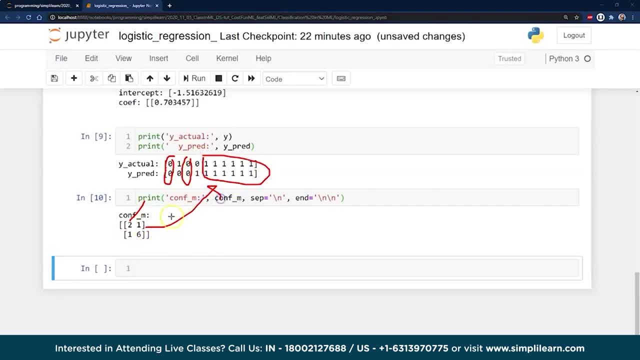 Which is our six. That's where the six comes from, And then we have this one, Which is the one false. This is the two ones. So we have this one here And this one here, Which is misclassified. This really depends on what data you're working with. 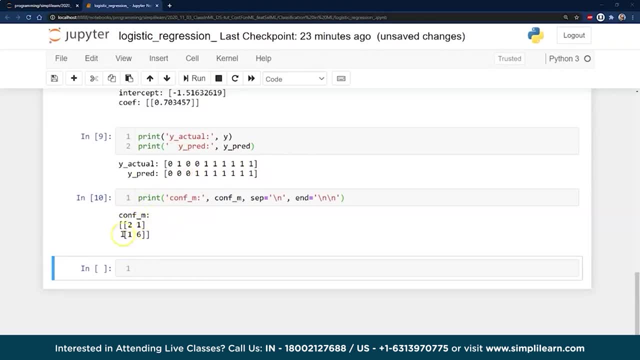 As to what is important. You might be looking at this model And if this model, This confusion matrix, comes up And says that you misclassified even one person As being non-malignant cancer, That's a bad model. I wouldn't want that classification. 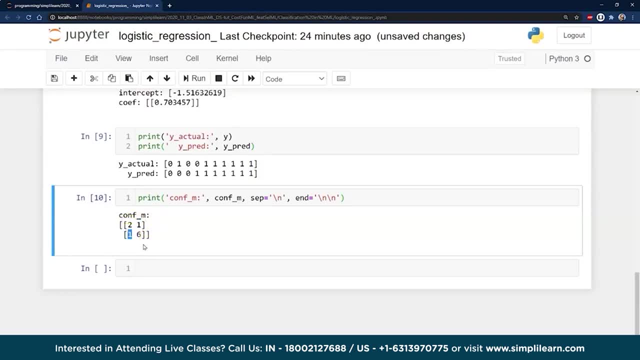 I'd want this number to be zero. I wouldn't care if this false positive was off by a little bit more, As long as I knew that I was correct on the important factor That I don't have cancer. So you can see that this confusion matrix. 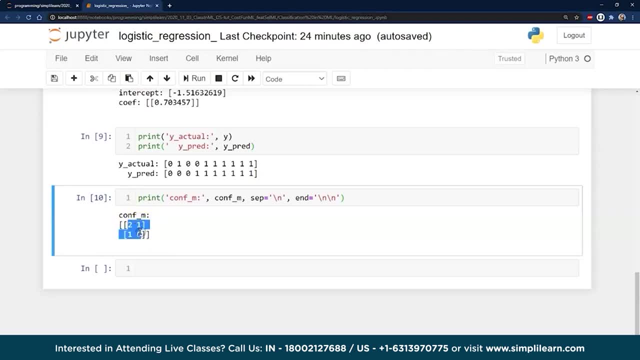 Really aims you in the right direction Of what you need to change in your model, How you need to adjust it. And then there's, of course, a report. Reports are always nice. If you notice we generated a report earlier. We'll go ahead and just print the report up. 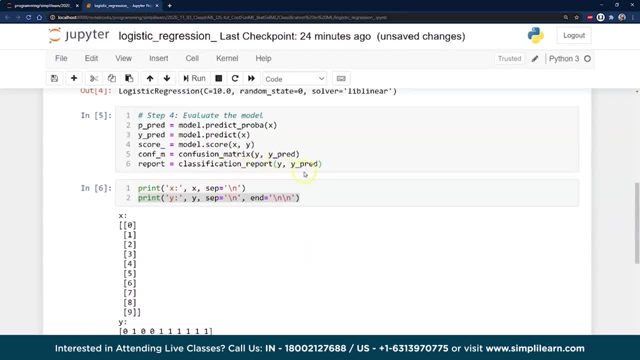 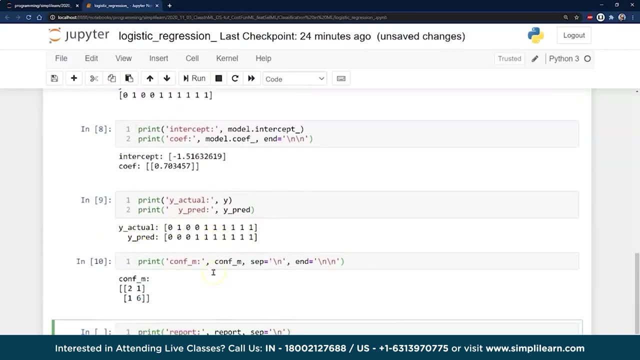 And you can remember, this is our report, It's a classification report: Y comma, Y predict. So we're just putting in our two values, Basically what we did here visually With our actual and our predicted value, And we'll go ahead and run the report. 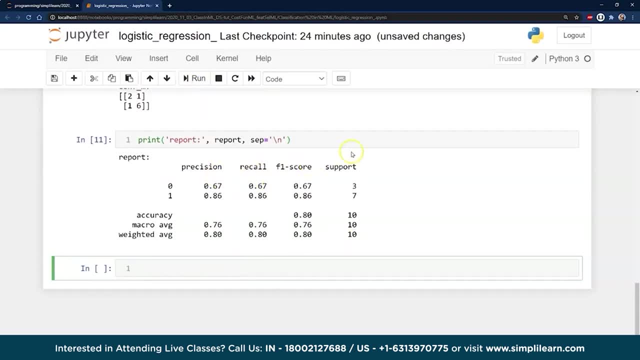 And you can see. it has the precision, The recall, Your F1 score, Your support, Translated into accuracy, Macro average And weighted average, So it has all the numbers. A lot of times when working with clients Or with the shareholders in the company, 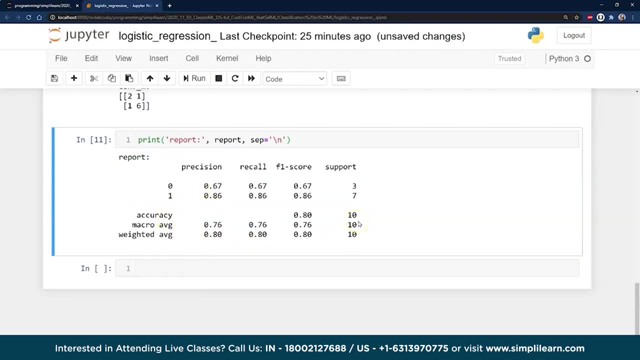 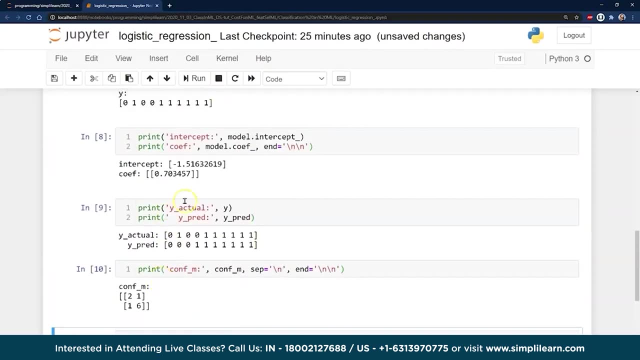 This is really where you start, Because it has a lot of data And they can just kind of stare at it And try to figure it out. And then you start bringing in, like the confusion matrix. I almost do this in reverse As to what they show. 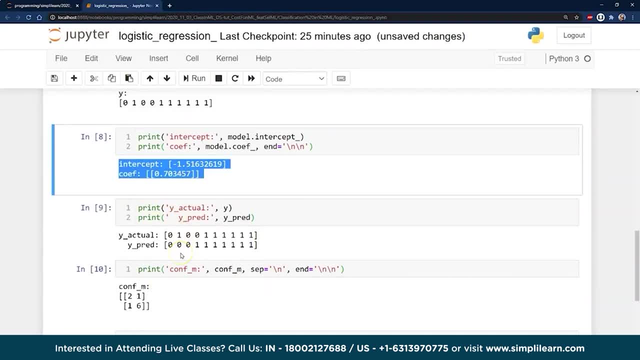 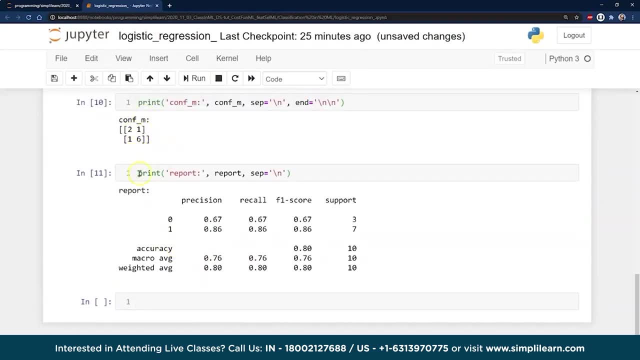 I would never show your shareholders The intercept or the coefficient That's for your internal team only Working on machine language. But the confusion matrix And the report are very important. Those are the two things you really want to be able to show on these. 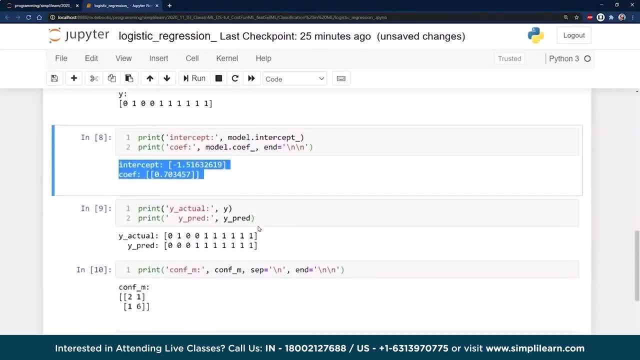 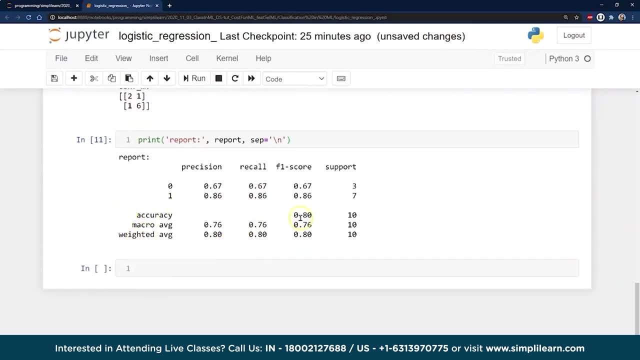 And you can see here we did a decent job Of classifying the data, Managed to get a significant portion of it correct. We had our was it accuracy. here Is a .80 F1 score, That kind of thing. So you know it's a pretty accurate model. 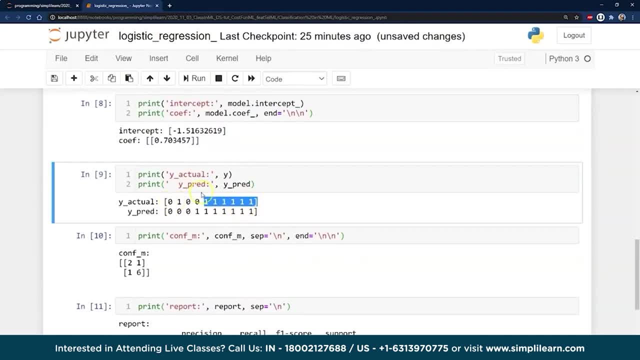 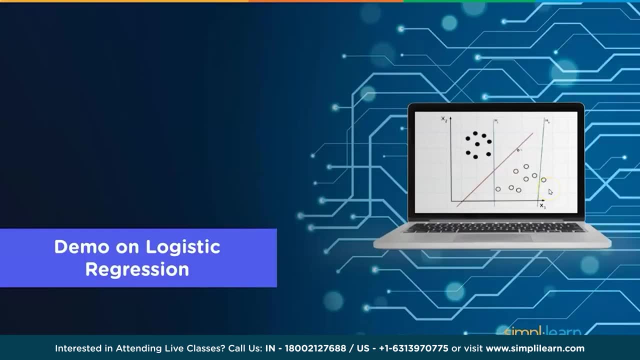 Of course, this is pretty goofy Because it's a very simple model And it's just splitting the model between 1s and 0s. So that was our demo of the logistic regression on there. Let's go ahead and take a look at k nearest neighbors. 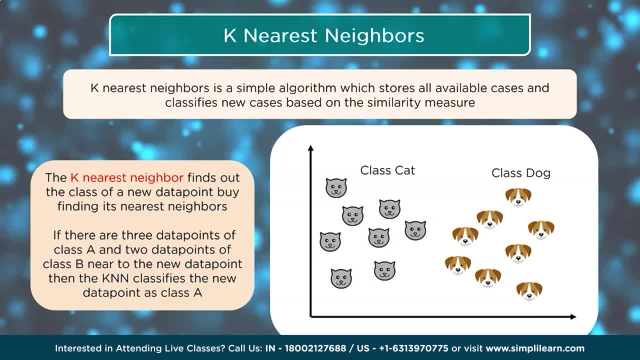 This one is another very highly used And important algorithm to understand K nearest neighbors is a simple algorithm Which stores all available cases And classifies new cases based on the similarity measure. The k nearest neighbor Finds out the class of the new data point. 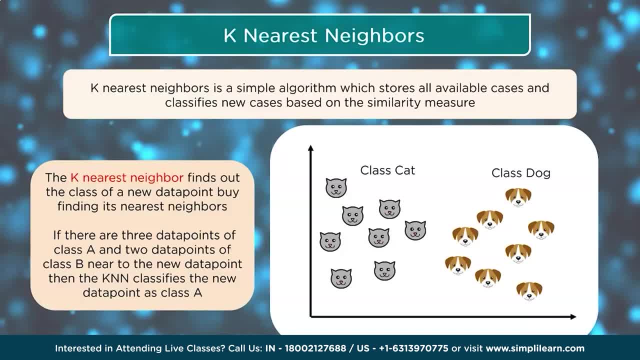 By finding its nearest neighbors. If there are 3 data points of class A And 2 data points of class B Near to the new data point, Then the KNN classifies the new data point as class A, The k in k- nearest neighbors. 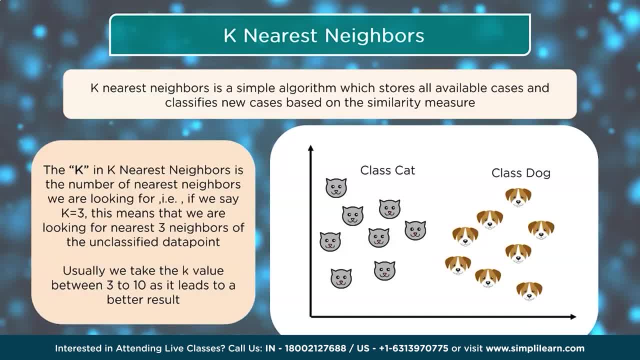 Is the number of nearest neighbors we are looking for. Ie, if we say k equals 3. This means that we are looking for Nearest 3 neighbors of unclassified data point. Usually we take the k value between 3 to 10.. 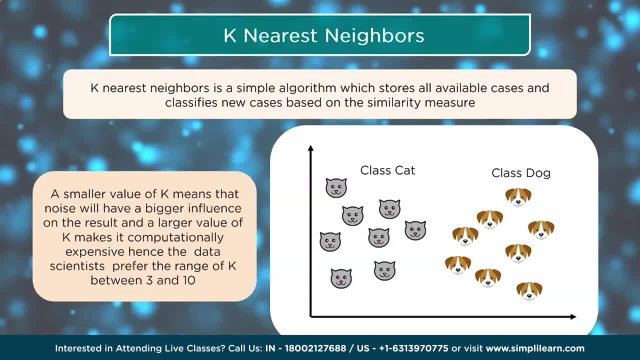 As it leads to a better result. A smaller value of k Means that noise will have a bigger influence on the result, And a larger value of k Makes it computationally expensive. Hence the data scientists prefer the range of k between 3 and 10.. 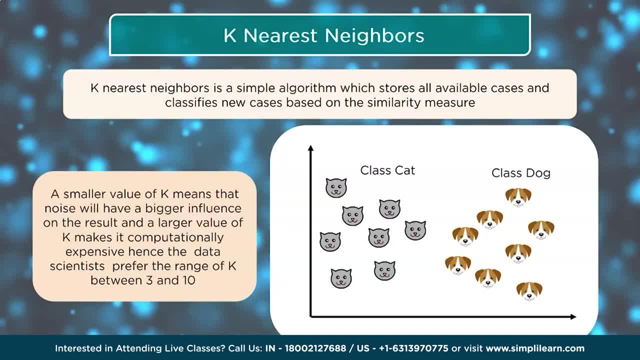 When we talk about noise, Remember the data we just looked at Was 0, 1, 1, 0, 0. It had some values where it cut it And said: everything to the right is a 1.. Everything to the left is a 0. 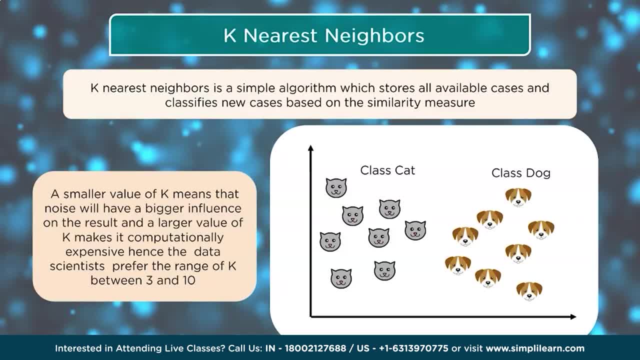 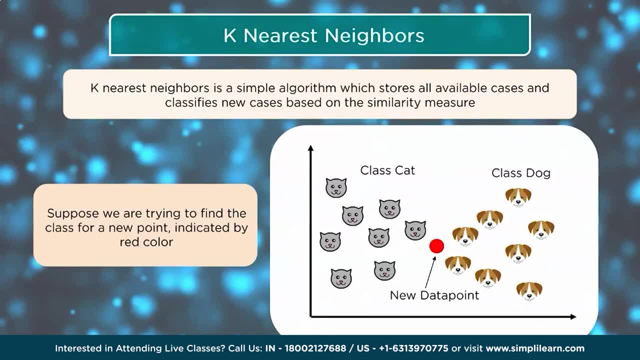 But it had some 1's and 0's mixed in there. That's called noise. That's what they are talking about. There are some things that are right in the middle in the classification Which makes it very hard to classify, So suppose we are trying to find the class for a new point. 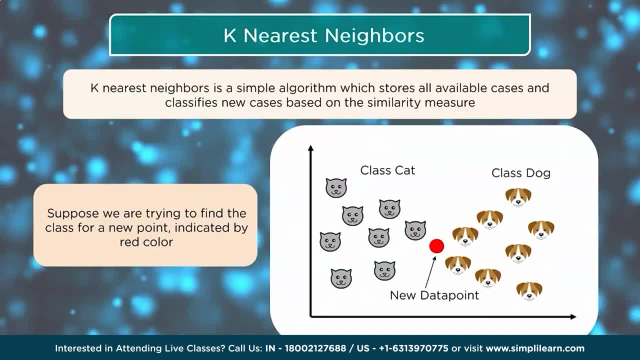 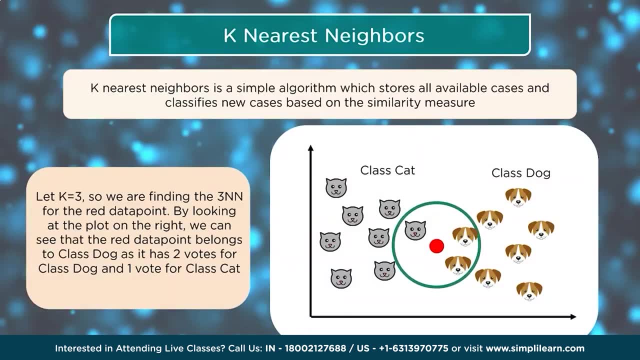 Indicated by the red color And you can see it's kind of right between the cat, Right between the dogs. Let k equal 3.. So we are finding the 3 and n for the red data point By looking at the plot on the right. 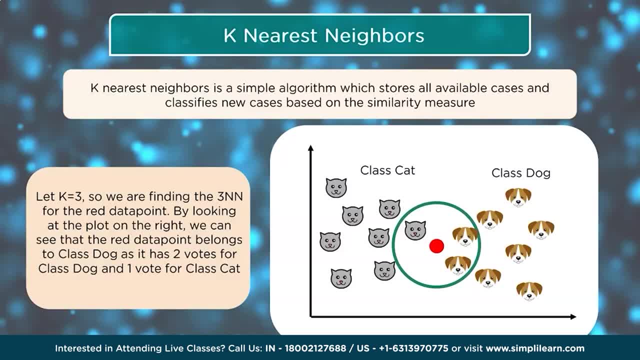 We can see that the red data point belongs to the class dogs, As it has 2 votes for class dogs And 1 vote for class cat. And if you ask the question, Well, what are you measuring the distance? What is that distance? 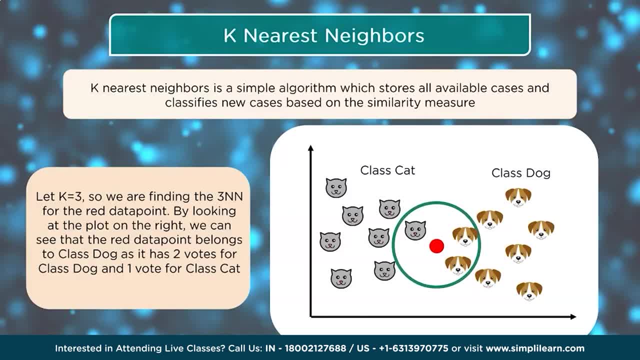 It could be the measurements of the ears, Whether they are pointed or floppy. That might be. one of the features you are looking at Is how floppy the ears are. Another one might be the whiskers Versus the nose, And then you take those measurements. 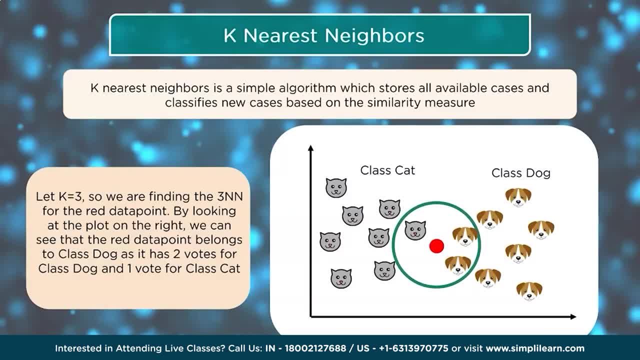 And using one of the most common things in k means measurement Is the Euclidean geometry. You can figure out the distance between those points. There is a lot of different algorithms for that, But you can think about it that you do have to have some kind of solid data to measure. 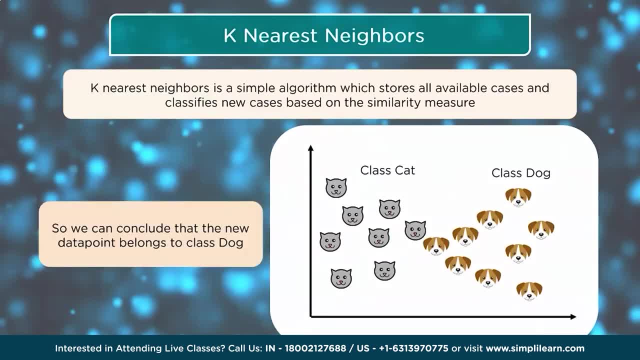 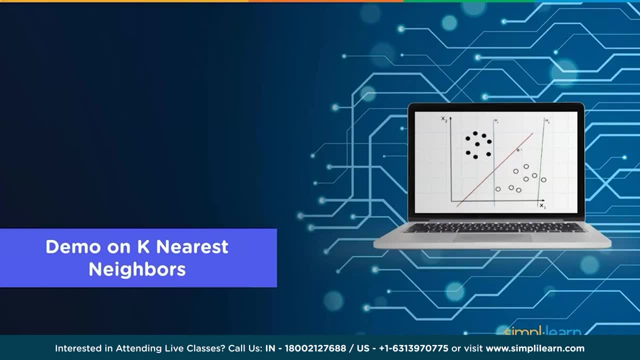 And so we can conclude that the new data point belongs to the class dog. So let's go ahead and see what this looks like in code And do a demo on the k nearest neighbors in here, And we will go right back into our Jupyter notebook. 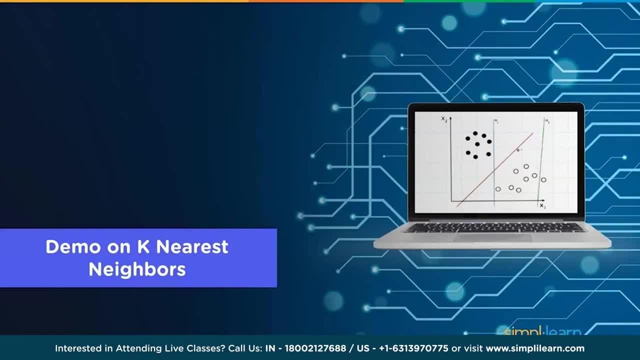 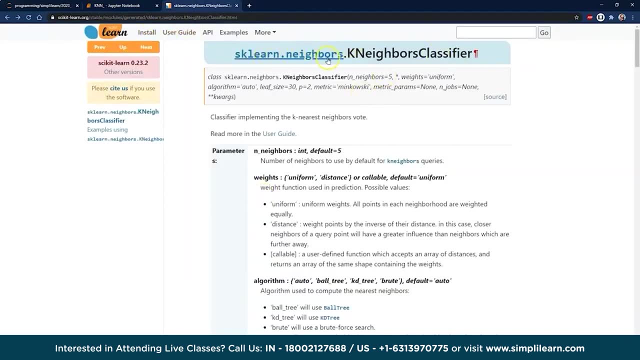 And open up a new Python programming script page. Of course, once we are in here, We are going to look at the scikit-learn. I did just a quick search for skneighbors- knneighbors classifier. This actually is the older version. .023 is the one we want. 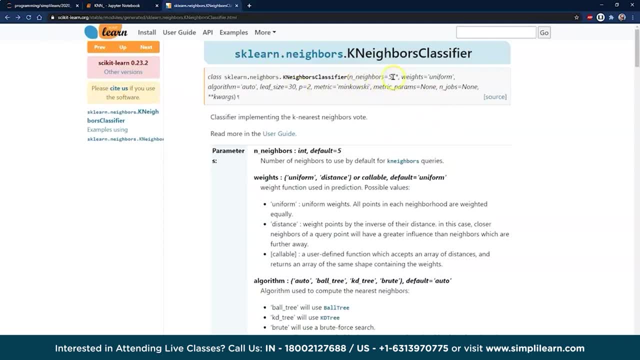 And you will see here that we have all their defaults. nneighbors equals 5. At defaults- we were talking about that- between 3 and 10.. There are different ways to weigh it. There is an algorithm based on it. I mentioned Euclidean geometry. 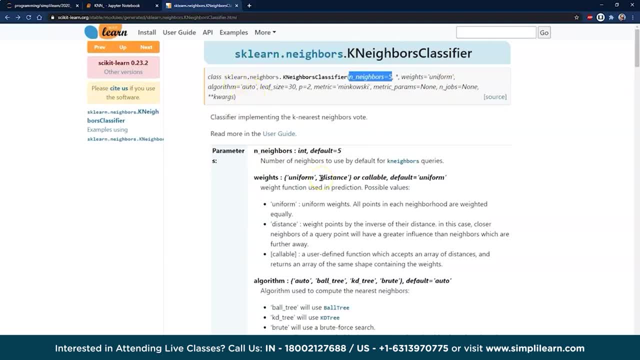 Finding the distance. There are other algorithms for figuring out what that distance is And how to weight those. There are a lot of other parameters you can adjust. For the most part, The k means basic setup is a good place to start. Just let the defaults go. 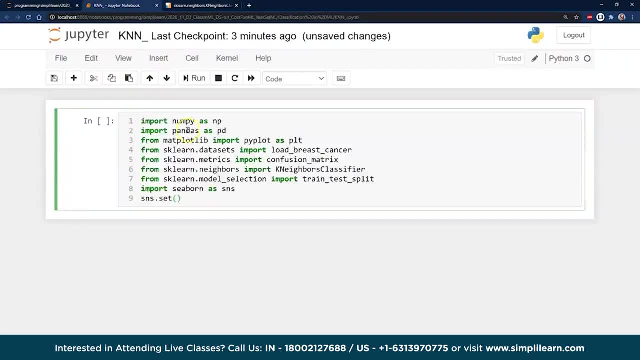 We might play with some of those. We will see what the guys in the back did And from here we are going to import numpy. We are going to use pandas, If you haven't been running pandas. Pandas is our data frame which sits on top of numpy. 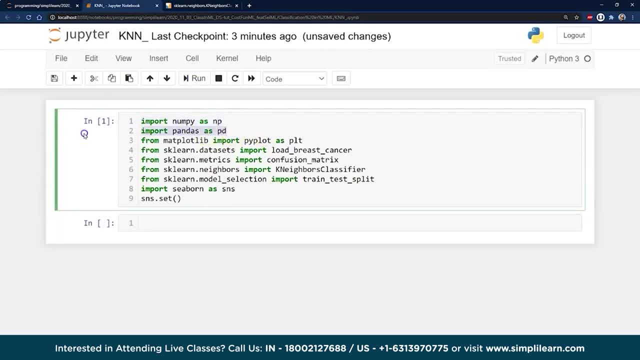 Data frames are: numpy is our number array? Pandas is our data frame. We are going to use matplotlib. We are going to plot some graphs. Everybody likes some pretty pictures. It makes it a lot easier to see what is going on When you have a nice display. 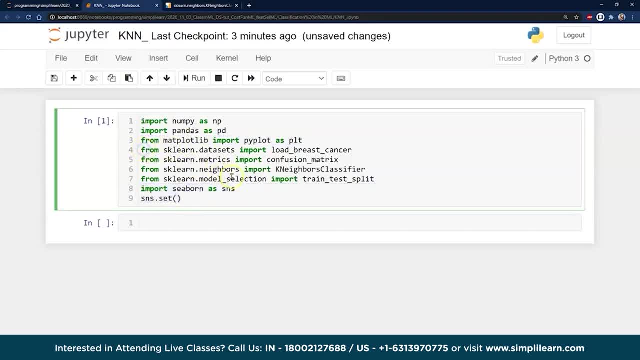 That is also what the seaborn is in here In the setup that sits on top of the matplotlib. The ones we really want to look at right here Are what we are bringing in from sklearn. These ones right here From sklearn we are going to load. 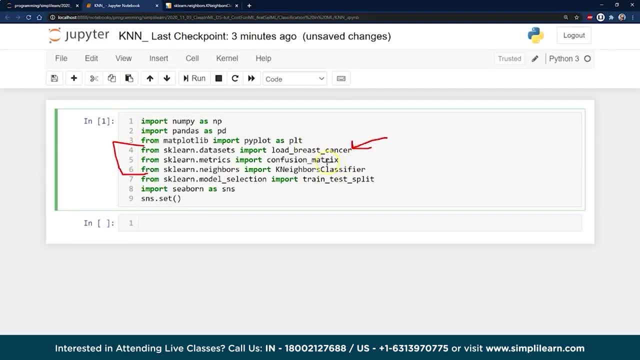 I mentioned the breast cancer. That is a very popular one Because it has 36 measurements. So there are 36 features. Unless you are an expert, You are not going to know what any of those features really mean. You can sort of guess. 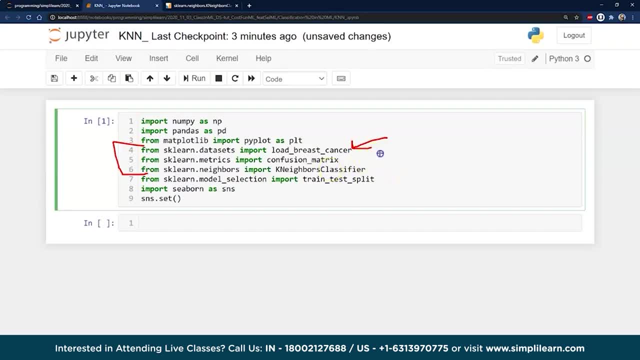 But there are special measurements they take of When they take an image And, of course, our confusion matrix, So that we can take a look and see what the data looks like And how good we did. And then we have our kn at neighbors classifier on here. 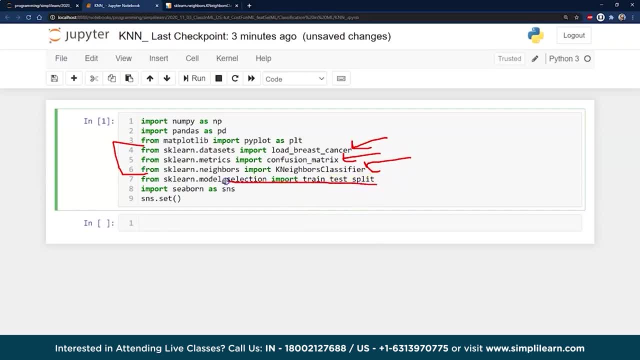 And then I mentioned that whenever you do training and testing, You want to split the data up. You don't want to train the data And then test it on the same data. That just tells you how good your training model is. It doesn't tell you whether it actually works on unknown data. 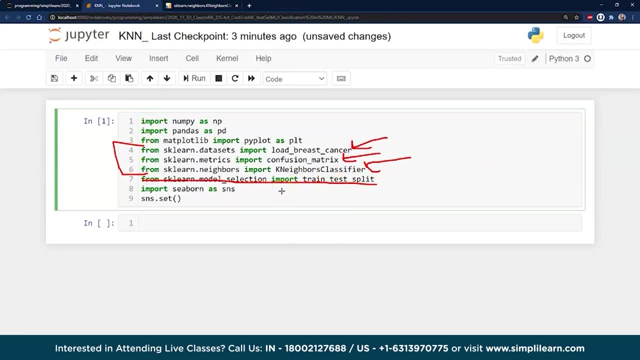 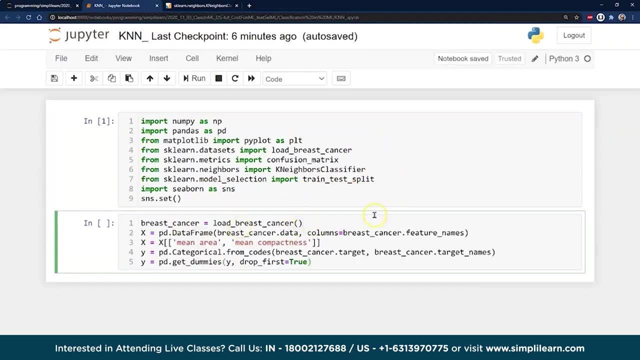 And so this just splits it off So that we can train it, And then we can take a look at data we don't have in there And see how good it did, And we will go ahead and load our data up. So here is our setup on that. 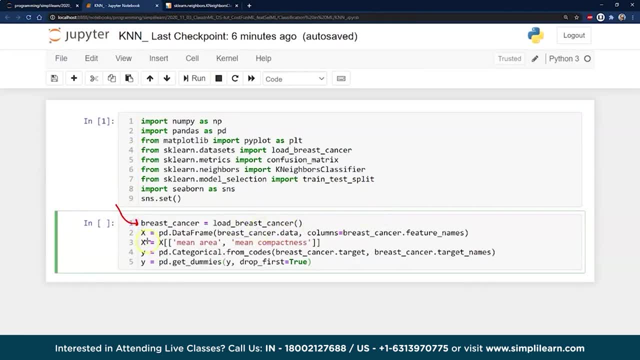 There we go. So we are going to go ahead and load the data up. We have our x value And that is going to come from our Breast cancer dot data And column breast cancer feature names. So there is our actual, All our different features. 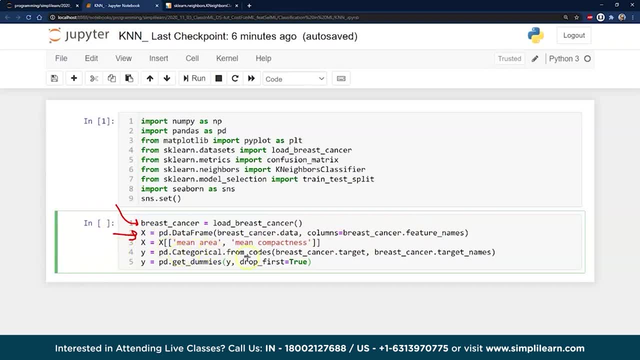 We will print that out here in a second, And then we have our mean area, Mean compactness. So I guess we are going to take the data And we are only going to use a couple of the columns. This just makes it easier to read. 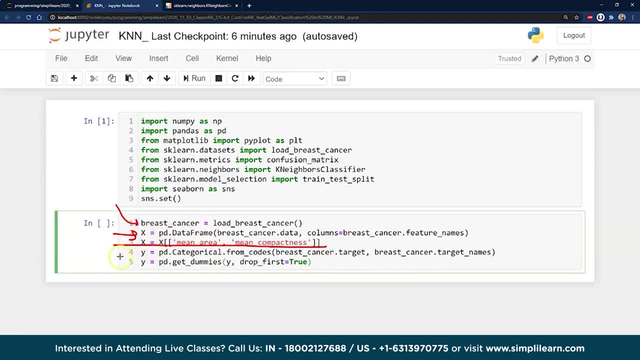 Of course, when you actually were going to do this, You would want to use all your columns. And then we have our y, And this is simply: Either it is malignant or benign, And then we want to go ahead and drop the first line. 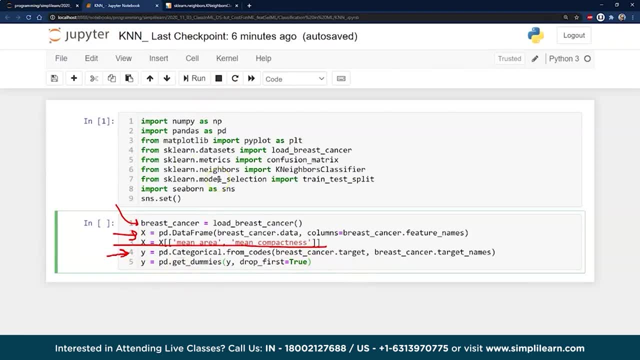 Because that is how it came in on there And we will go ahead. Let's just take a look at this a little closer here. Let's go ahead and run this real quick, And just because I like to see my data before I run it. 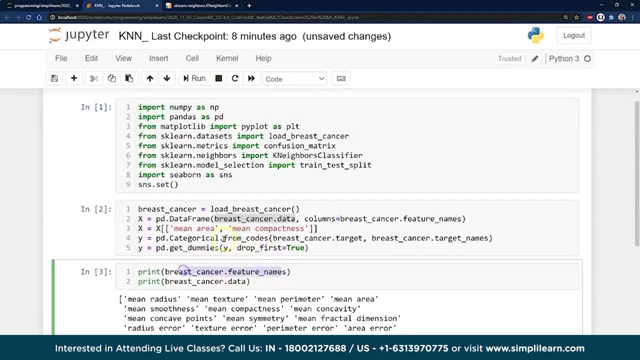 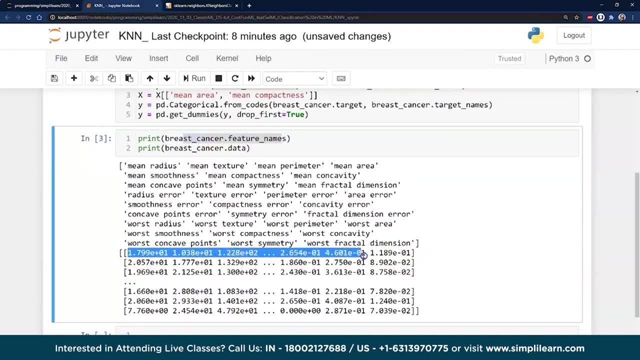 We can look at this And we can look at the original features. Remember, we are only going to use two features off of here, Just to make it a little easier to follow. And here is the actual data And you can see that this is just. 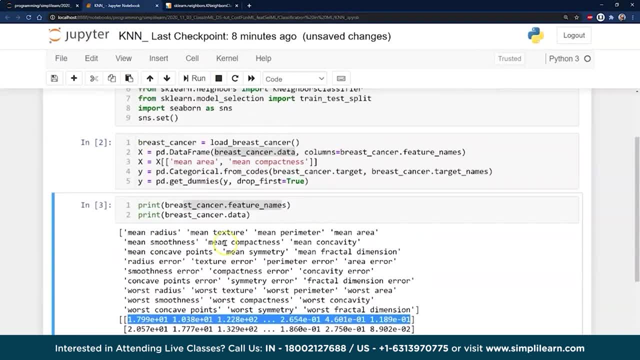 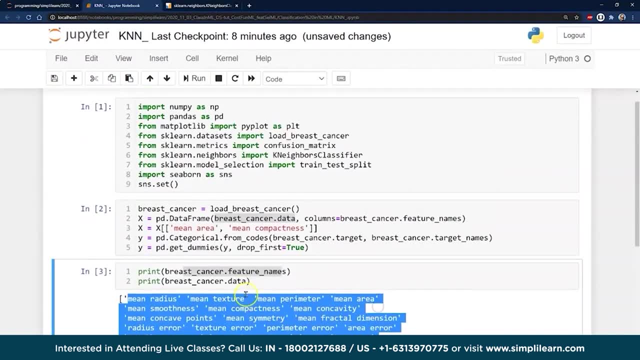 This massive stream of data coming in here. It is going to just skip around Because there is so much in there to set up. I think there is like 500. If I remember correctly. And you can see here is all the different measurements they take. 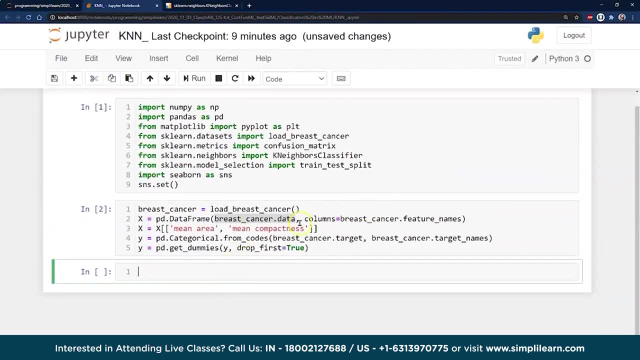 But we don't really need to see that on here. We are just going to take a look at just the two columns And then also our solution. We will go ahead and just do a quick print Y on here So you can see what the y looks like. 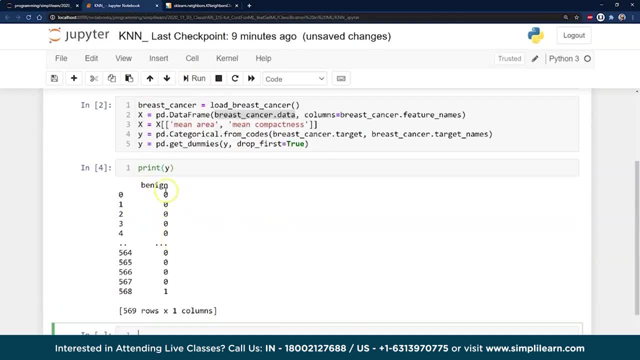 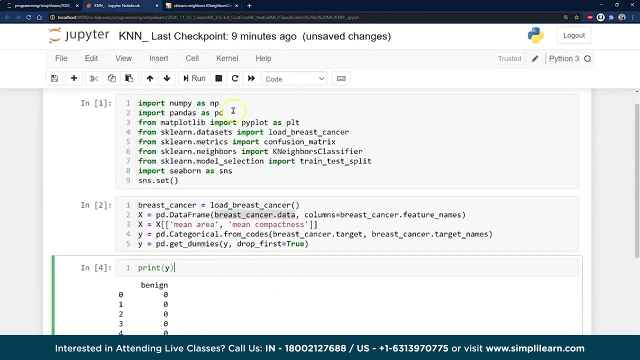 And it is simply just 000.. You know b90001.. So a 1 means it is benign, A 0 means it is malignant. That is what we are looking at on that. Go ahead and cut that out of there. The next stage is to go ahead and split our data. 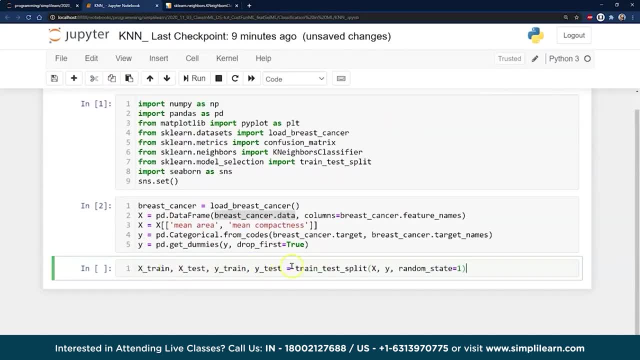 I mentioned that earlier. We will just go ahead and let them do the splitting for us. We have xtrain, xtest, ytrain, ytest, And so we go ahead and train test. split xy, random state equals 1.. It makes it nice and easy for us. 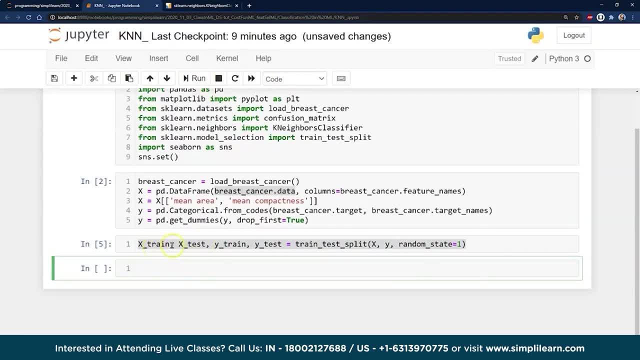 We will go ahead and run that. And so now we have our training and our testing. Train means we are going to use that to train the model, And then we are going to use the test To see how good our model does, And then we will go ahead and create our model. 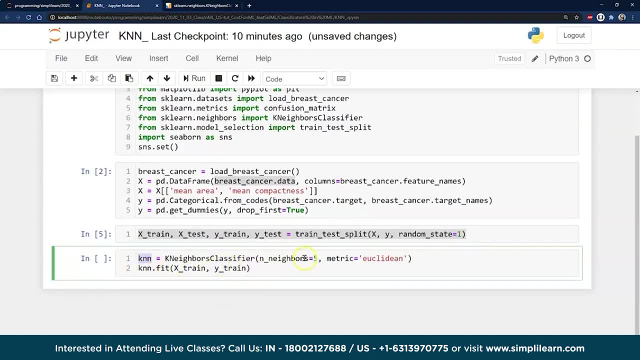 Here is our knn model: The k-neighbors classifier, n-neighbors equals 5.. The metrics is Euclidean. Remember I talked about Euclidean? This is simply your c squared equals a squared plus b squared plus a squared equals b squared plus c squared plus c squared plus d squared. 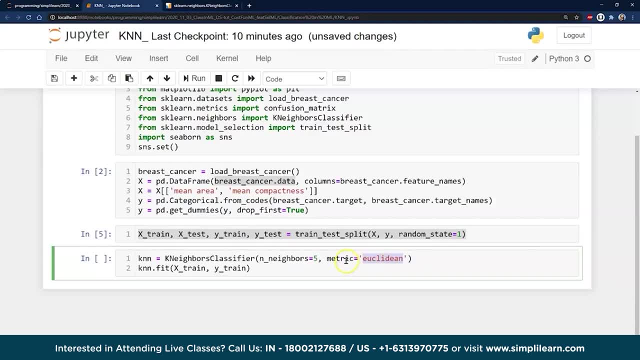 And then you take the square root of all that. That is what they are talking about here. It is just the length of the hypotenuse of a triangle, But you can actually do that in multiple dimensions, Just like you do in two dimensions with a regular triangle. 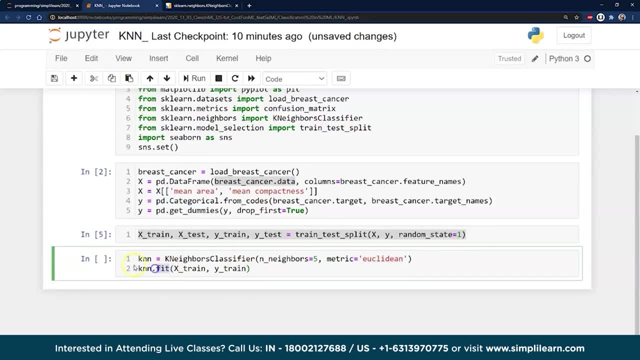 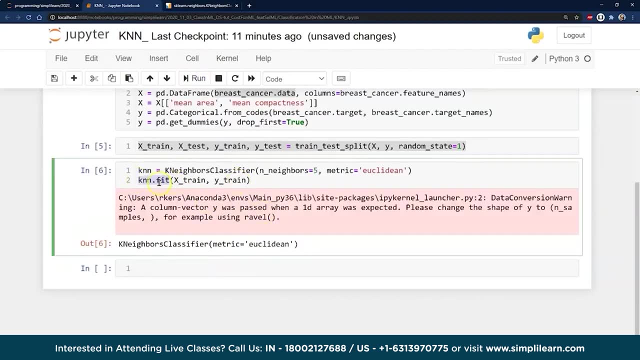 And here we have our fit. This should start to look familiar, Since we already did that in our last example. That is very standard for scikit And any other one, Although sometimes the fit algorithms look a little bit more complicated Because they are doing more things on there. 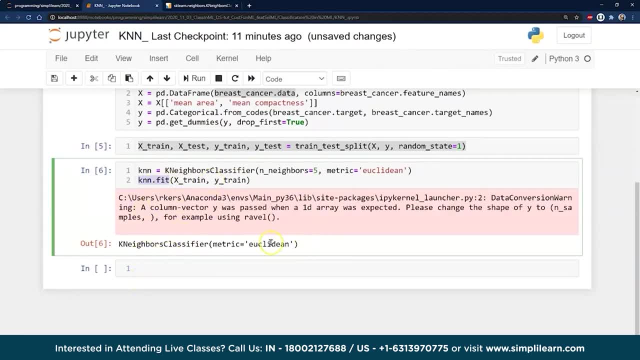 Especially when you get into neural networks And then you have your k-neighbors, It just tells you: we created a k-neighbors setup. They kind of wanted us to reformat the y, But it is not that big of a deal for this. 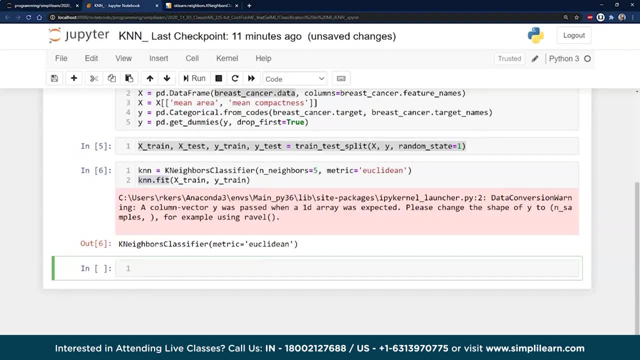 And it comes out: It shows you that we are using the Euclidean metric for our measurement. So now we have created a model. Here is our live model. We have fitted the data to it. We say, hey, here is our training data. 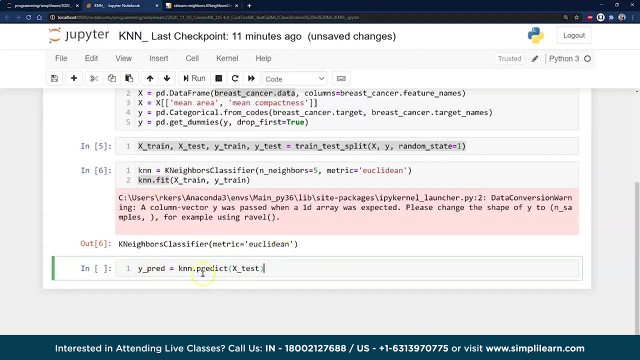 Let us go ahead and predict it. So we are going to take our y predict equals k and n predict y test. So this is data we have not. This model has not seen this data, And so we are going to create a whole new set of data off of there. 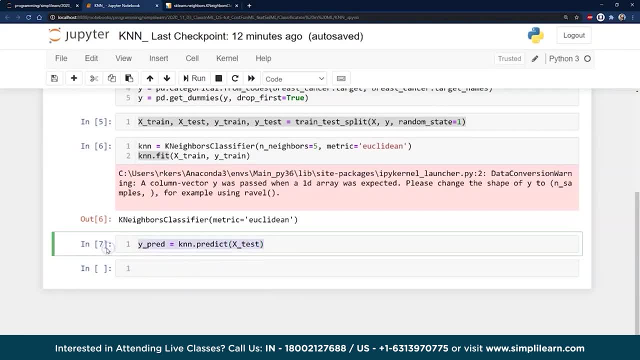 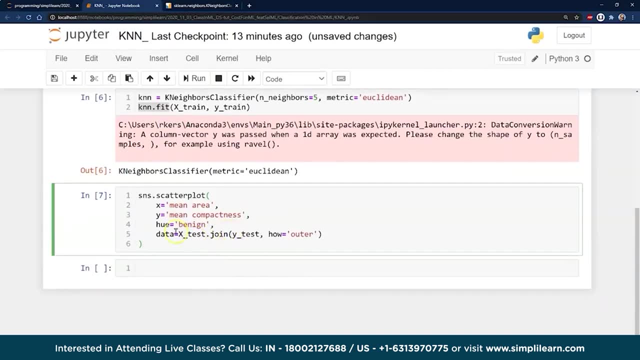 Now, before we look at our prediction- In fact, I am going to bring this down and put it back in here later- Let us take a look at our x test data. versus the y test, What does it look like? And so we have our mean area. 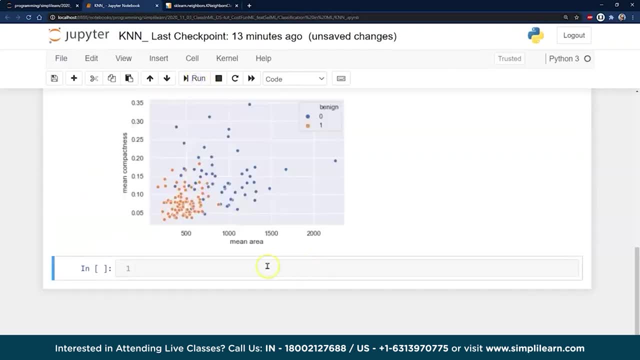 We are going to compare it to our mean compactness. We are going to go ahead and run that And we can see here the data. if you look at this, Just eyeballing it. We put it in here. We have a lot of blue here. 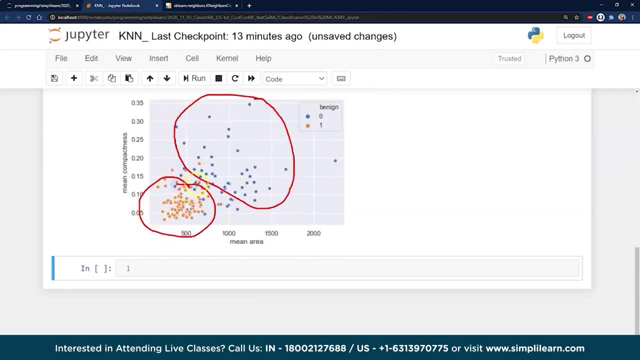 And we have a lot of orange here, And so these dots in the middle, Especially like this one here And these here, These are the ones that are going to give us false negatives, And so we should expect. this is your noise. This is where we are not sure what it is. 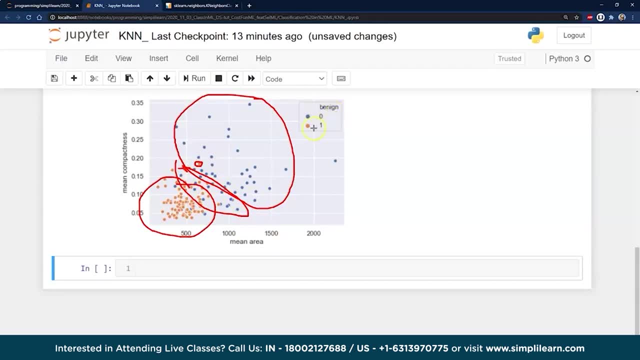 And then b9, in this case, is done in blue And malignant is done in one. So if you look at it, there are two points based on these features, Which makes it really hard to have 100% where the 100% is down here. 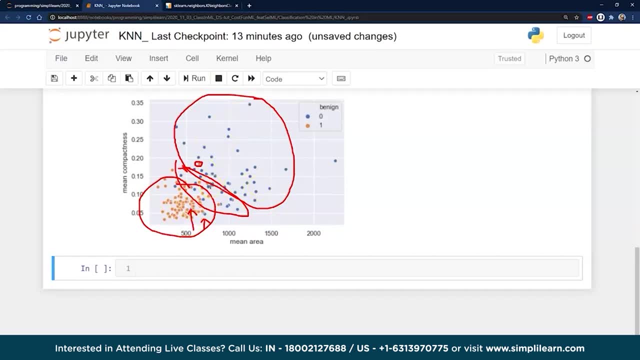 Or up here. That is kind of the thing I would be looking for when we are talking about cancer and stuff like that, Where you really do not want any false negatives, You want everything False positive. Great, You are going to go in there and have another set up in there. 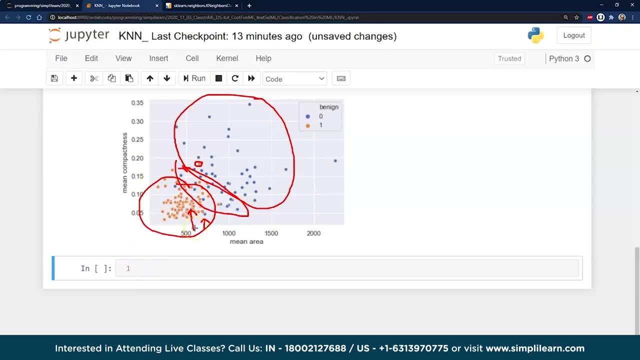 Where you might get an autopsy or something like that done on it. Again, that is very data specific on here. So now let us go ahead and pull in and get our prediction in here And we will create our Y prediction. We will go ahead and run that. 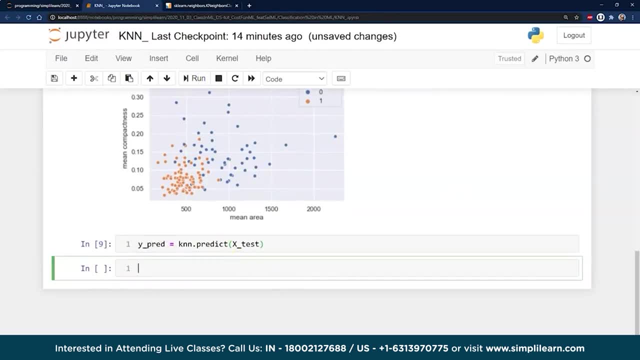 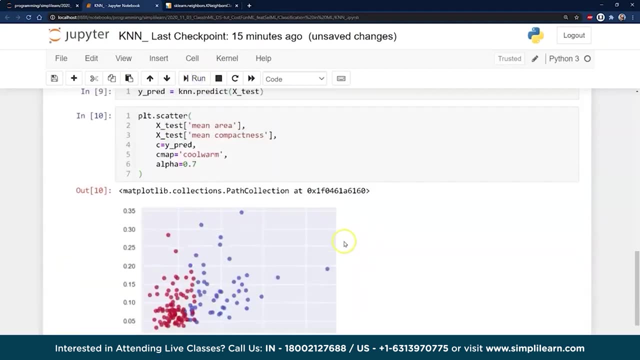 So now this is loaded with what we think the unknown data is going to be, And we can go ahead and take that And go ahead and plot it, Because it is always nice to have some pretty pictures And when we plot it we are going to do the mean area versus mean compactness. 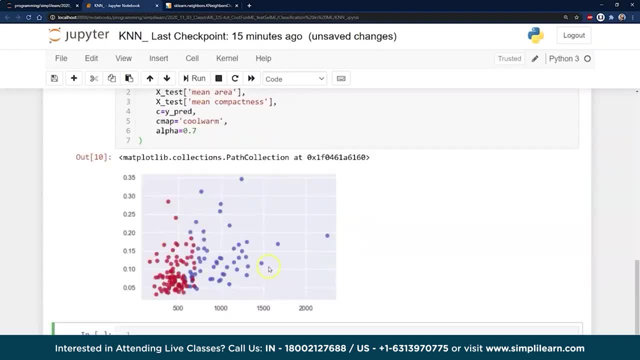 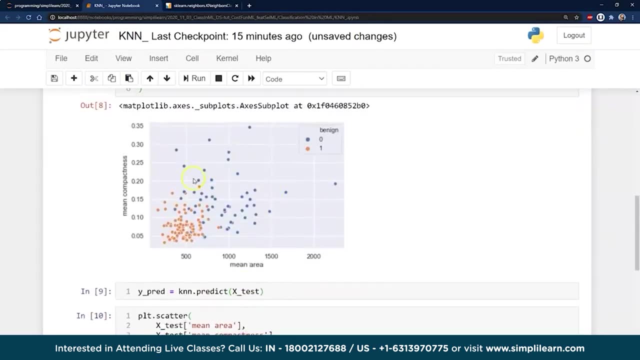 Again, you look at this map and you can see that there is some clear division here. We can clearly see on some of this stuff that our Y prediction- If we look at this map up here And this map down here, We probably got some pretty good deal. 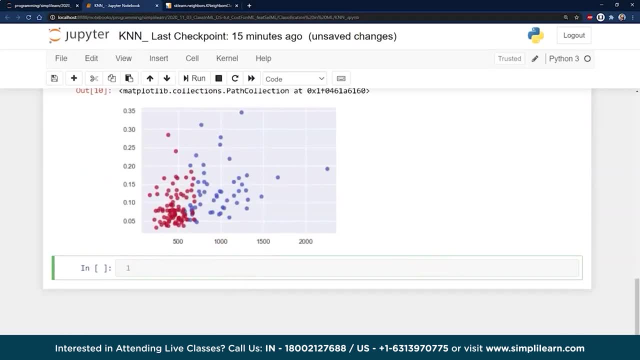 It looks pretty good, like they match a lot. This is, of course, just eyeballing it. Really, you do not want to eyeball these things. You want to show people the pictures So that they can see it And you can say, hey, this is what it looks like. 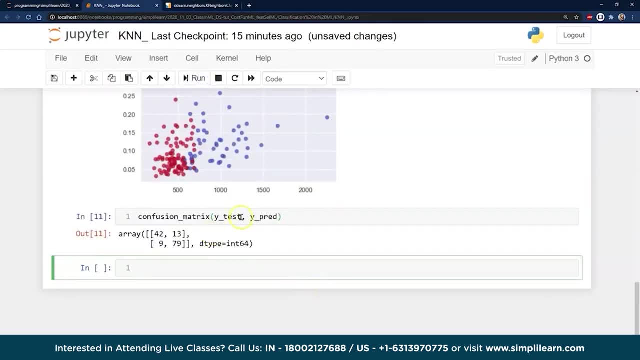 But we really want the confusion matrix And when we do the Y test and the Y predict, We can see in the confusion matrix here It did pretty good And we will just go ahead and point that out real quick. Here is our 42, which is positive. 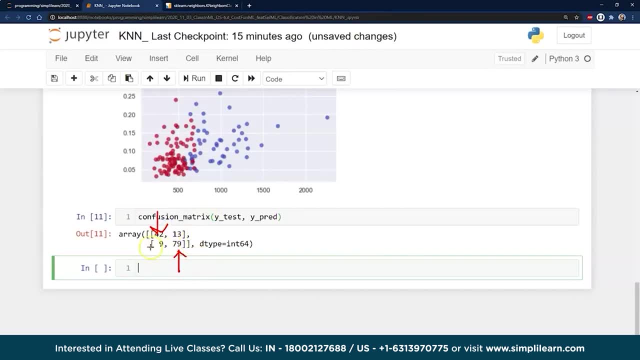 And our 79. And, if I remember correctly, I would have to look at the data. which one of these is a false negative? I believe it is the 9.. That is scary. I would not want to be one of those nine people. 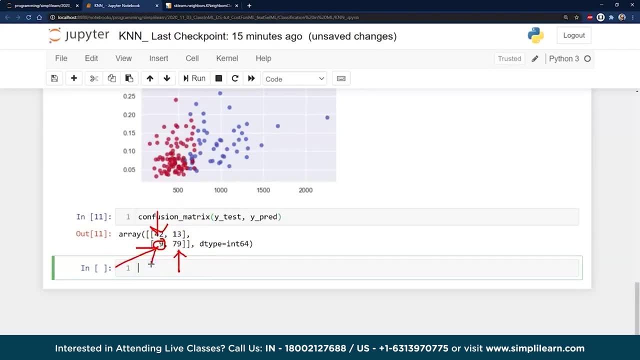 Told that I do not have cancer And then suddenly find out I do. So we would need to find a way to sort this out, And there is different ways to do that. A little bit past this, But you can start messing with the actual Euclidean geometry. 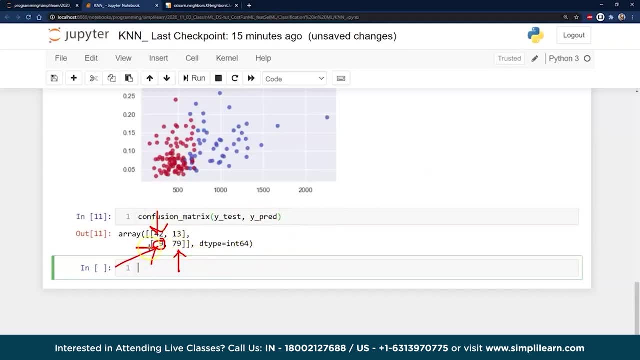 And the activation measurements And start changing those and how they interact. But that is very advanced. There is also other ways to classify them Or to create a whole other class right here of we do not knows. Those are just a couple of the solutions you might use for that. 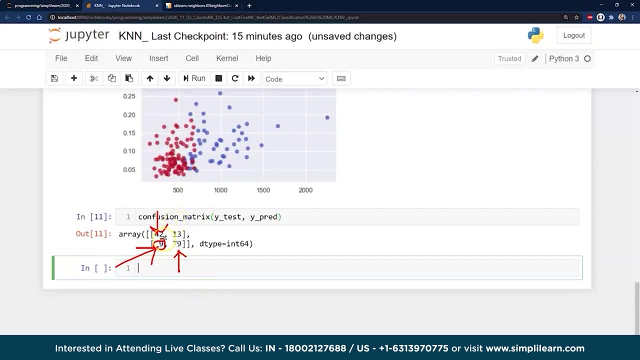 But for a lot of things this works out great. You can see here, maybe you are trying to sell something. Well, if this was not life dependent- And this was- if I display this ad, 42 of these people are going to buy it. 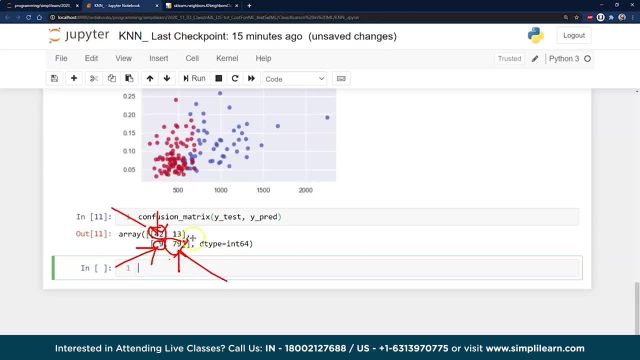 And if I display this other ad, If I do not display it, 79 people are going to go a different direction Or whatever it is. So maybe you are trying to display whether they are going to buy something If you add it on to the website. 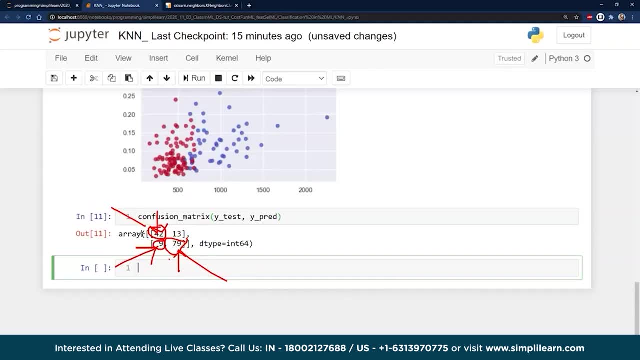 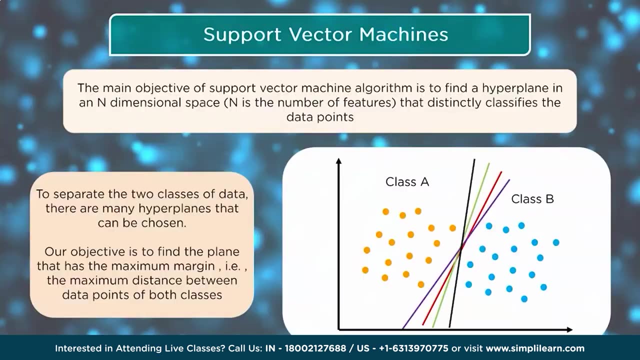 In which case that is really a good number. You have just added a huge number of sales to your company. So that was our K nearest neighbors. Let us go ahead and take a look at support vector machines. So support vector machines is the main objective of a support vector machine algorithm. 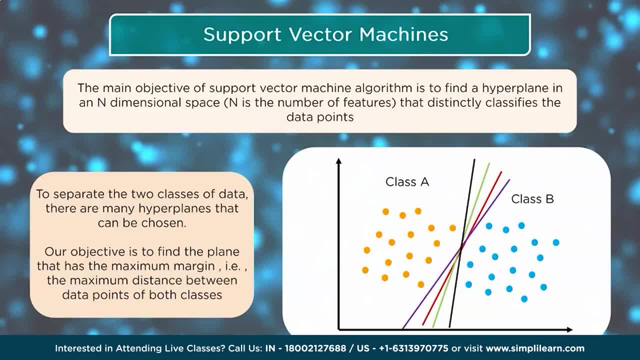 Is to find a hyperplane in an N dimensional space. N is the number of features That distinctly classifies the data points. If you remember, we were just looking at those nice graphs we had earlier, In fact, let me go ahead and flip back on over there. 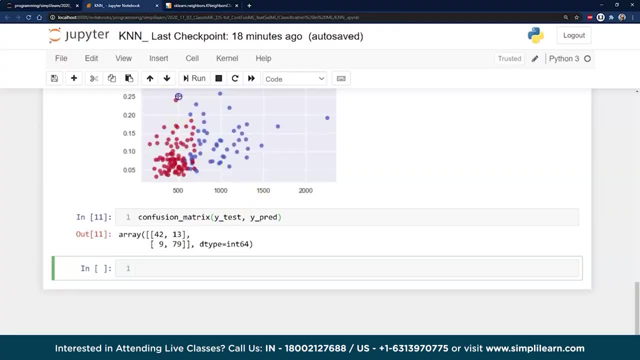 If we were looking at this data here, We might want to try to find A nice line through the data, And that is what we are talking about with this next setup. So the main objective of a support vector machine algorithm Is to find a hyperplane in an N dimensional space. 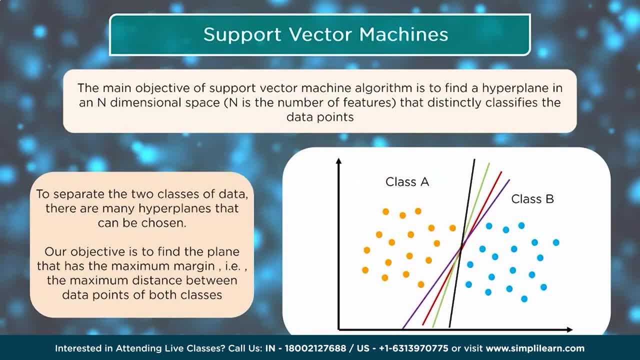 N is the number of features that distinctly classifies the data points. To separate the two classes of data, There are many hyperplanes that can be chosen. Our objective is to find the plane that has the maximum margin, IE the maximum distance between data points of both classes. 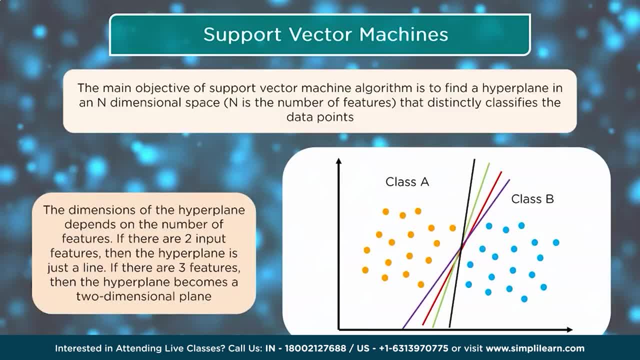 The dimensions of the hyperplane depends on the number of features. If there are two input features, Then the hyperplane is just a line. If there are three features, Then the hyperplane becomes a two dimensional plane, The line that separates the data into two classes. 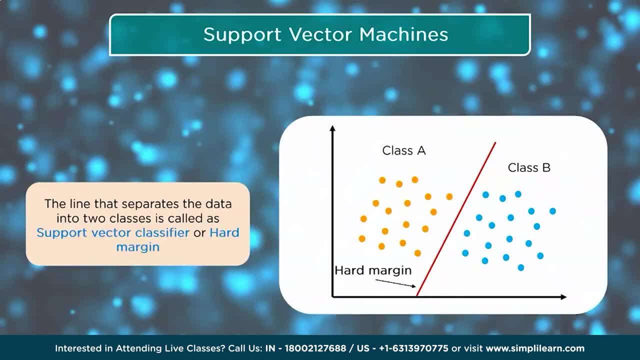 Is called as support vector classifier Or hard margin, And that is why I just showed you on the other data You can see here we look for a line that splits the data evenly. The problem with hard margin Is that it doesn't allow outliers. 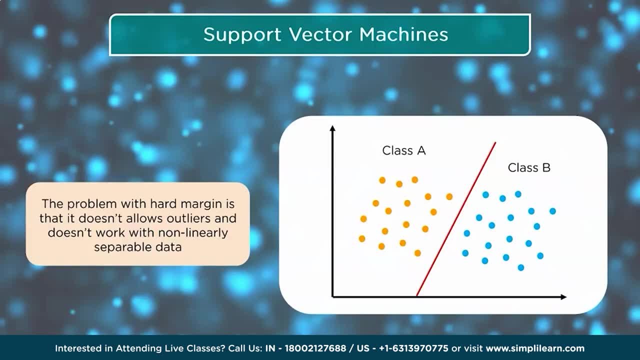 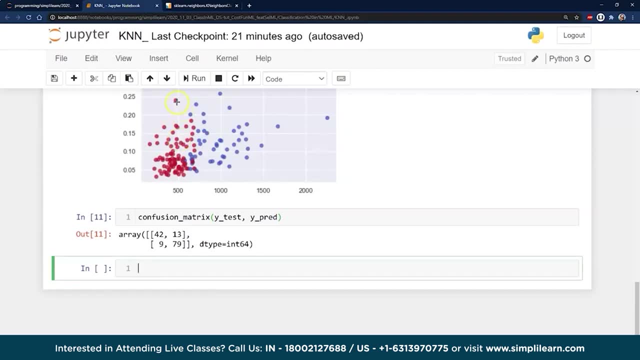 And doesn't work with non-linearly separable data, And we just were looking at that. Let me flip back on over here. And when we look at this setup in here And we look at this data, Here we go: Look how many outliers are in here. 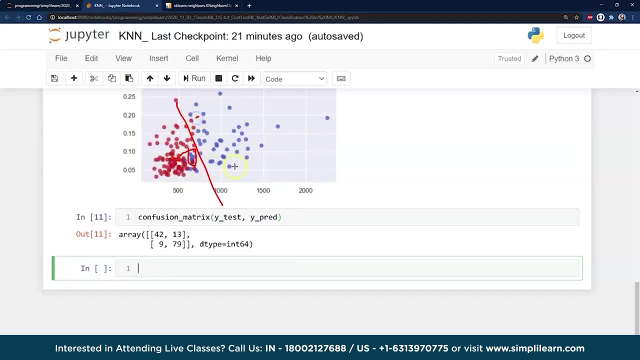 These are all with all these blue dots on the wrong side of the line Would be considered outlier, And the same with the red line, And so it becomes very difficult to divide this data, Unless there's a clear space. There we go. 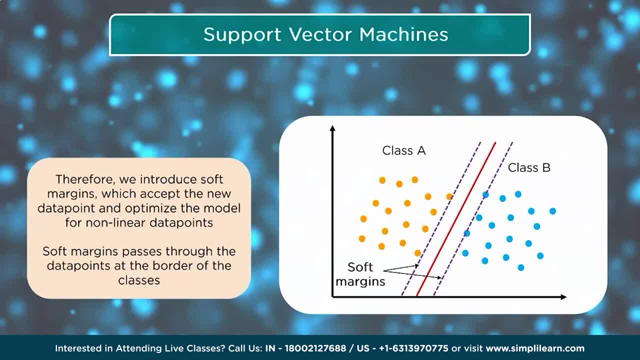 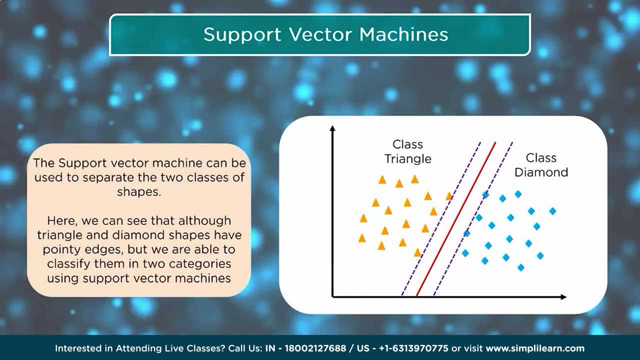 Therefore we introduce soft margins Which accept the new data point And optimize a model for non-linear data points. Soft margins pass through the data points at the border of the classes. The support vector machine can be used to separate the two classes of shapes. 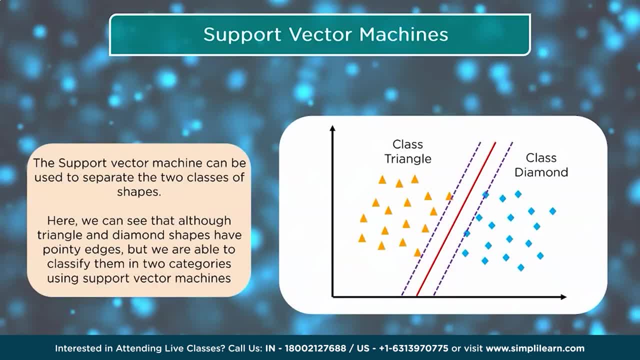 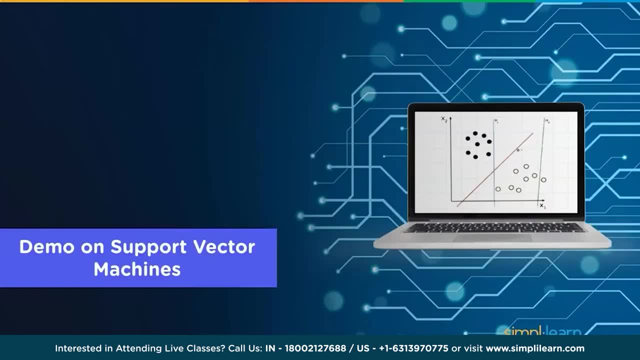 Here we can see that although triangles and diamond shapes have pointy edges, But we are able to classify them in two categories using a support vector machine. Let's go ahead and see what that looks like in a demo And flip back on over to our Jupyter notebook. 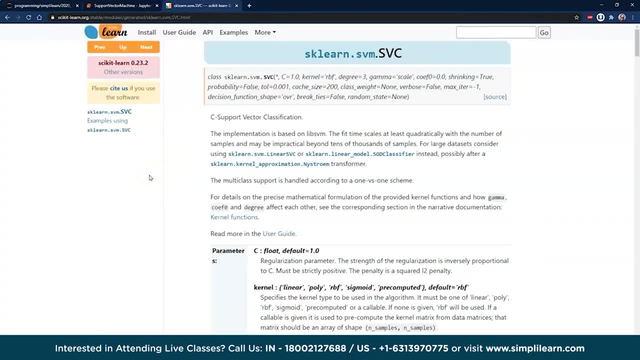 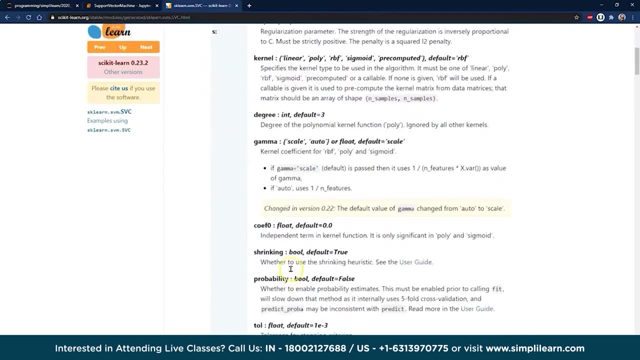 We always want to start with taking a look at the sklearn API, In this case the SVM, SVC. There is a significant number of parameters Because the SVM has been a lot of development in the recent years And it's become very popular. 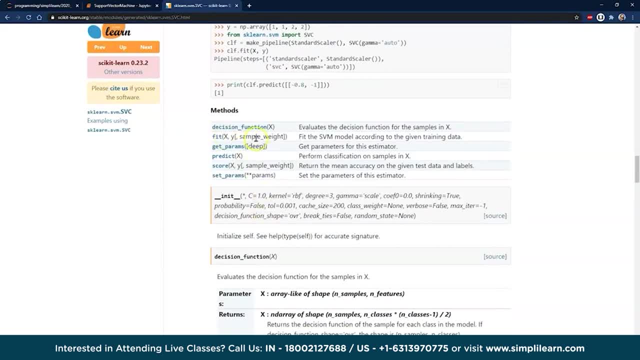 If we scroll all the way down to methods, You'll see right here is our fit And our predict. That's what you should see in most of the scikit-learn packages, So this should look very familiar to what we've already been working on. 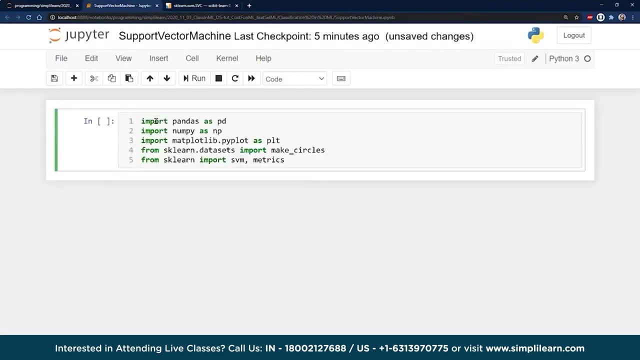 And we'll go ahead and bring in our import And run that. We should already have pandas, numpy, our matplot library, Which we're going to be using to graph some of the things A little bit different right here. You'll see that we're going to go ahead and bring in 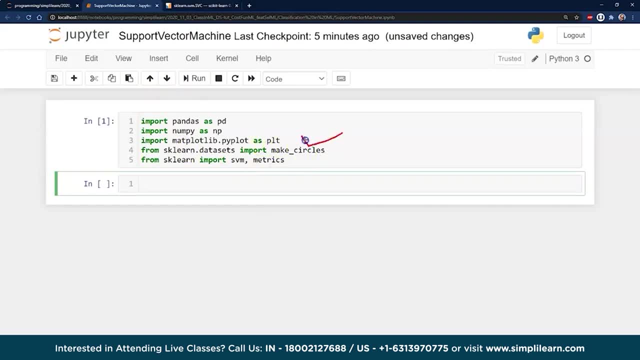 One of the fun things you can do with test data is make circles. Circles are really hard to classify. You have a ring on the inside and a ring on the outside And you can see where that can cause some issues, And we'll take a look at that a little closer in a minute. 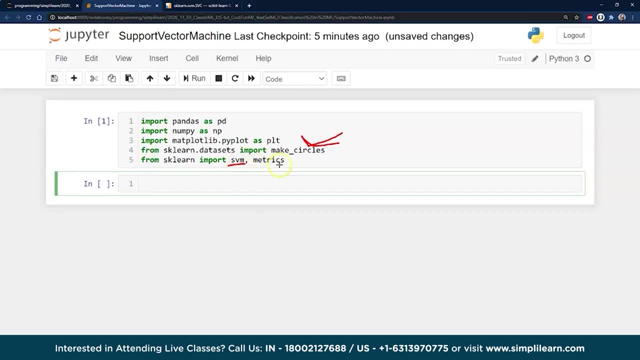 Here's our SVM setup on there And then, of course, our metrics, Because we're going to use that to take a closer look at things. So we go ahead and run this. Whoops already did Once. we've gone ahead and done that. 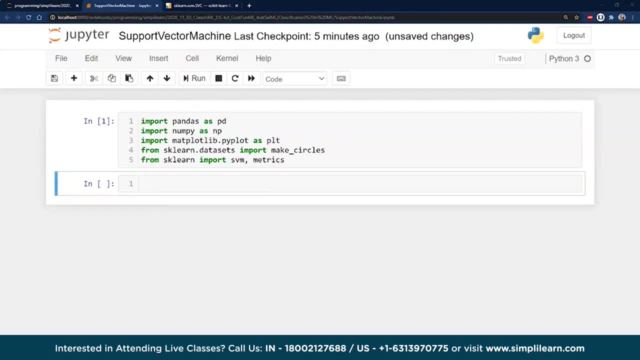 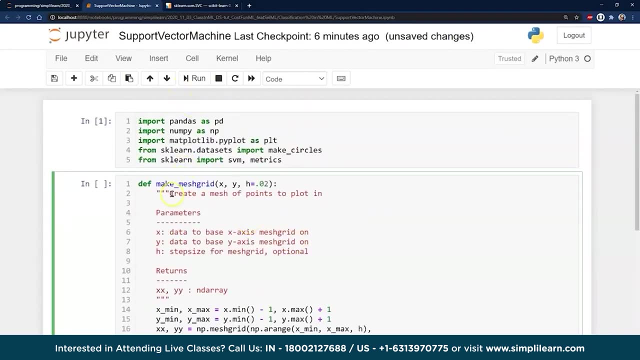 We're going to go ahead and start making ourselves some data, And this part probably a little bit more complicated than we need. I'm not going to go too much in detail on it. We're going to make a mesh grid And we'll see what that looks like in a minute. 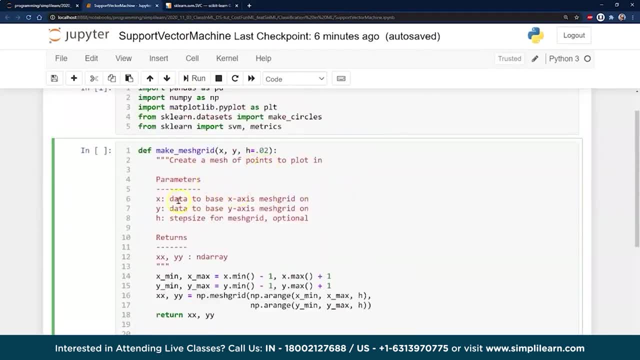 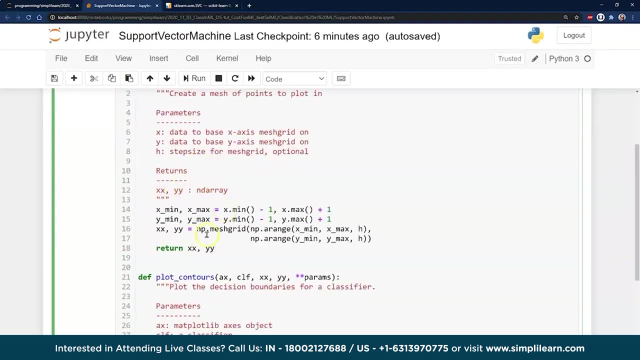 We're defining the minimums You can see in here. create a mesh grid of points. Here's our parameters of x, y and h. It's going to return X, x, y, y. You can also send a note to us. 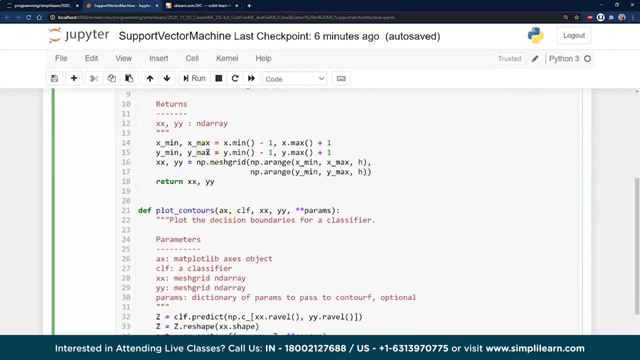 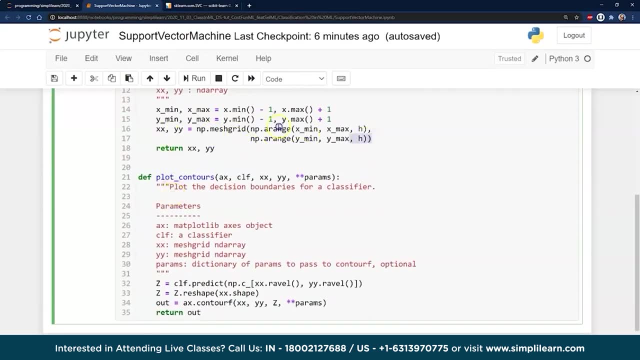 Make sure you get a copy of this if you want to dig deeper into this particular code especially. And we have a y min y max, Y min y max Plus one. Here's our mesh grid we're actually going to make. 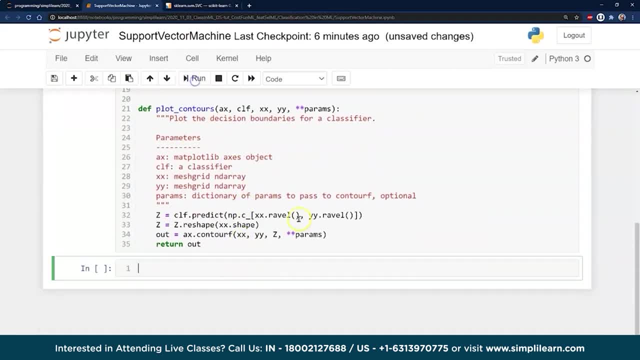 X, x and y, y Plot the contours all the way through And this is just a way of creating data. It's kind of a fun way to create some data. We go plot contours ax, clf, x, x, y, y. 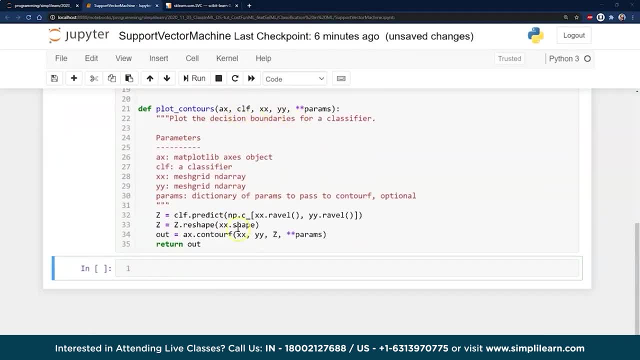 And return it out And some perimeters here, so that when we're doing it we have our setup on there Train property And then we'll go ahead and make our data. Just throw that right in there too, in the same setup. 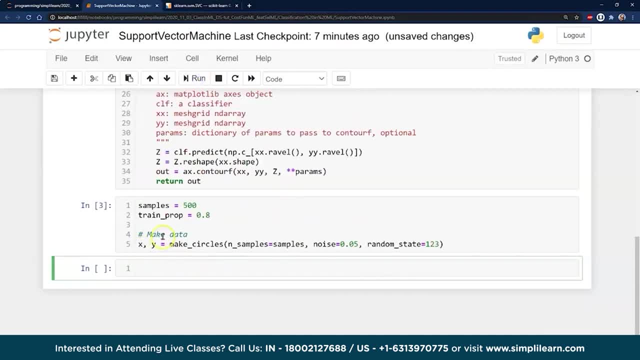 And run that. So now we have x and y. We're going to make our circles. We have n samples, equals samples. In this case, we're going to have 500 samples. We went ahead and gave it noise of 0.05.. 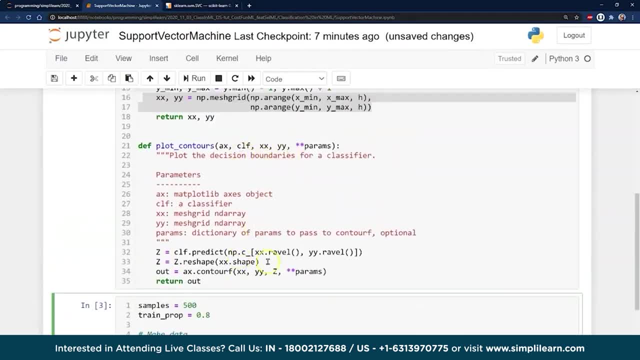 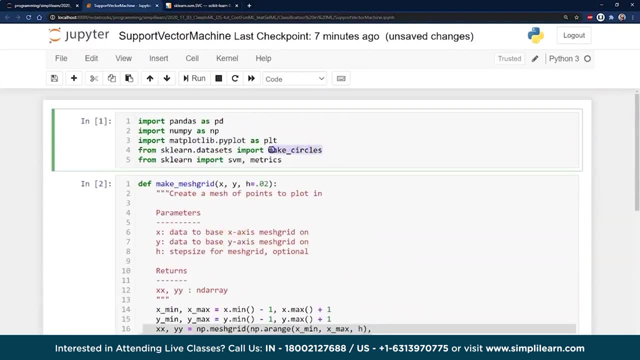 Random state 123.. These are all going into. Let's go back up Here we go Make our mesh grid, Make circles. There it is. So this is going into our make circles up here And this is part of that setup on this. 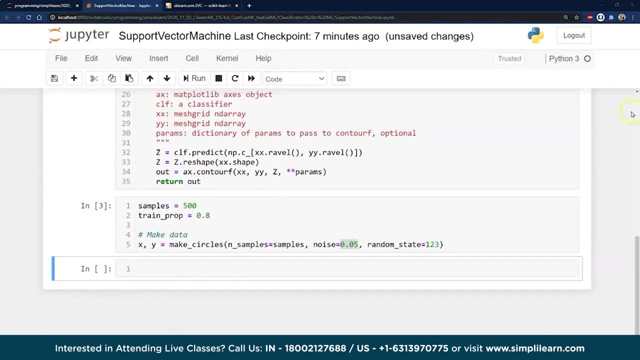 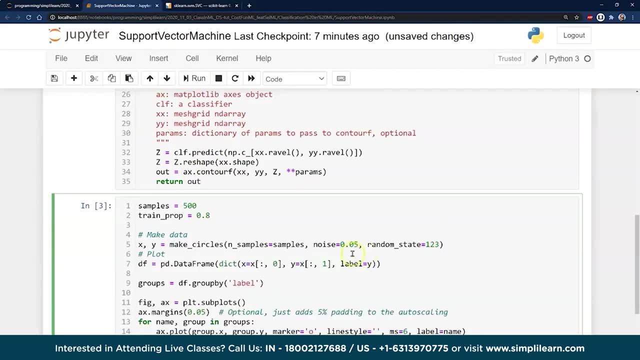 And then, once we've gone ahead and make the circle, let's go ahead and plot it. That way you can see what we're talking about. Right now. what I'm saying is really confusing, because without a visual it doesn't really mean very much what we're actually doing. 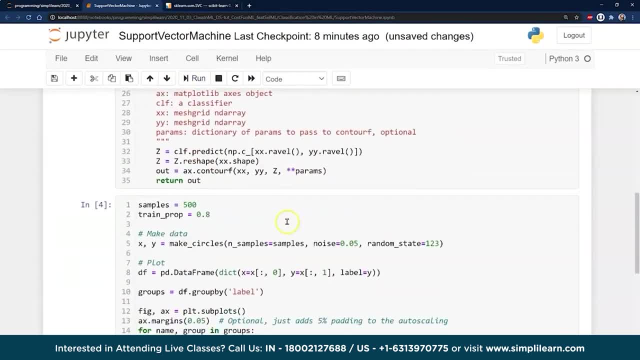 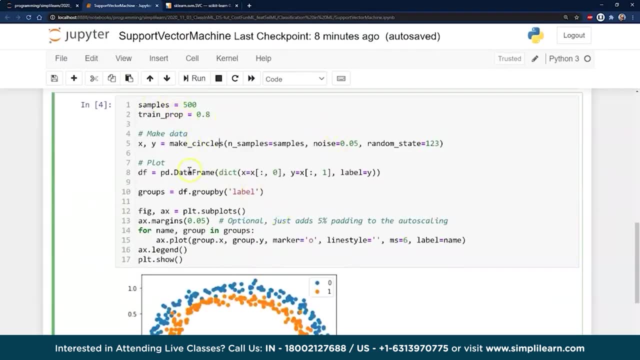 So I'm going to go ahead and run this with the plot. Let's go back up here and just take a look. We've made our circle. We have our n samples equals samples. We're going to have 500.. We're going to have training property 0.8.. 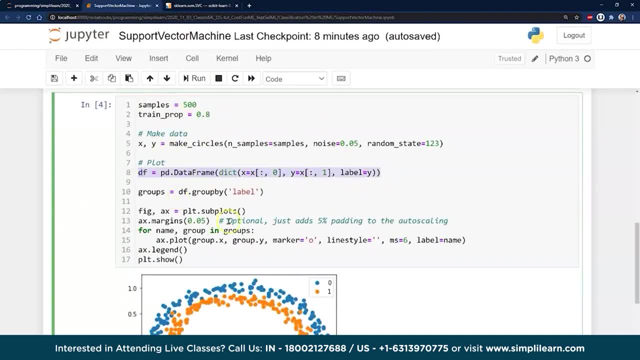 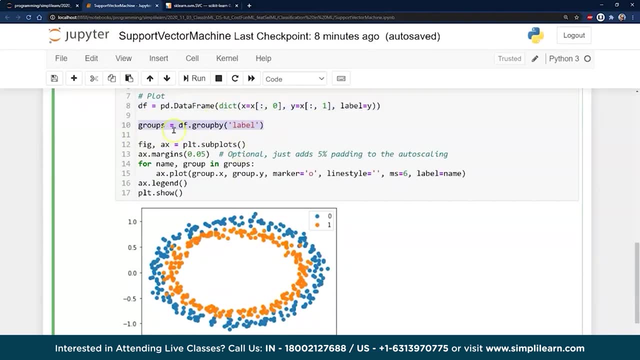 Here's our data frame. We go and load it into the data frame so we can plot it. Groups Df, Group by label. This is kind of a fun way. if you have multiple columns you can really quickly pull whatever setup is in there. 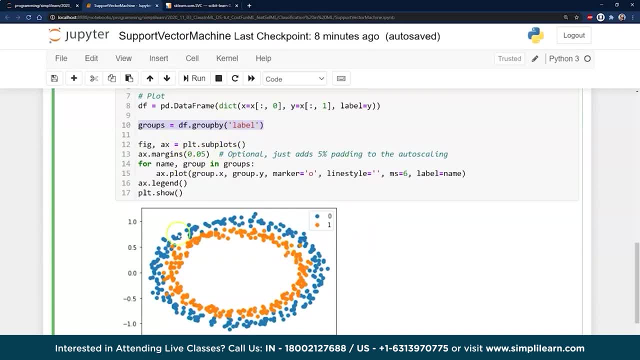 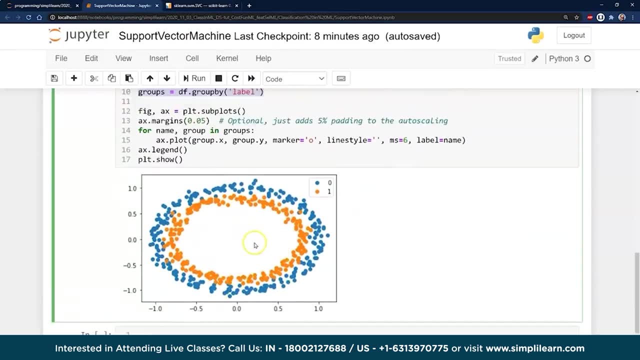 And then we go ahead and plot it And you can see, here we have two rings that are formed, And that's all this is doing is just making this data for us. This is really hard data to figure out. A lot of programs get confused in this. 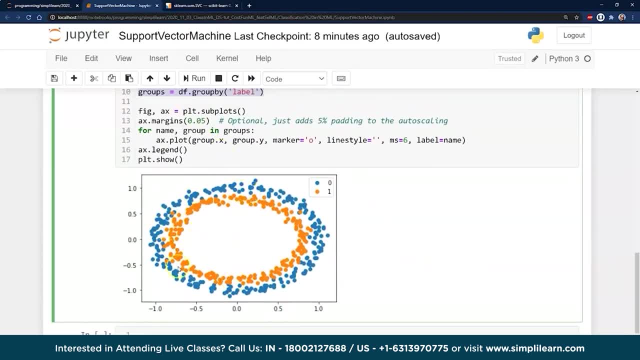 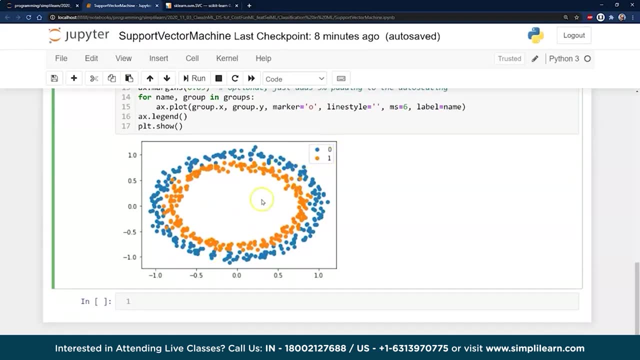 because there's no straight line or anything like that. But we can add planes and different setups on here, And so you can see we have some very interesting data. We have our 0s in blue and our 1s in the yellow in the middle. 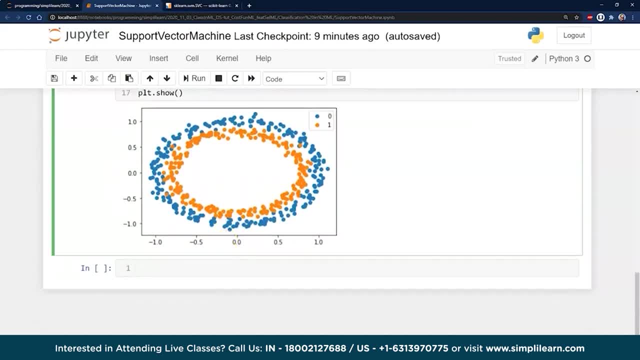 And the data points are an xy coordinate plot on this. One of the things we might want to do on here is go ahead and find the min to max ratio setup in there, And we can even do. let's just do a print x. 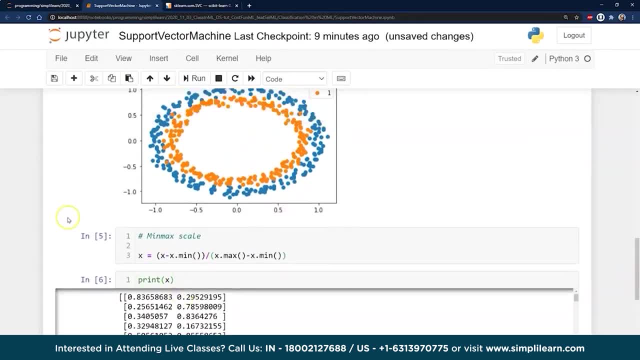 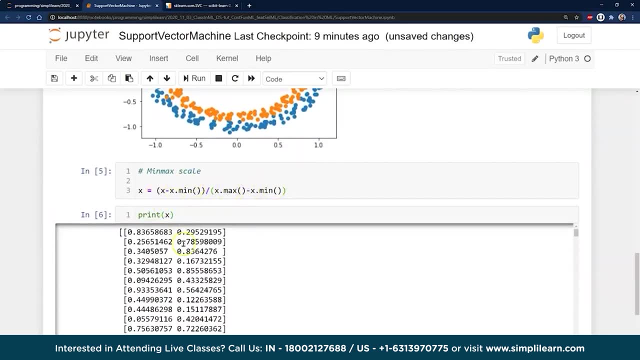 You can see what the data looks like that we're producing on this. There we go. So x equals x minus x min over x max minus x min. All we're doing is putting this between 0 and 1.. Whatever this data is, we want a 0 to 1 setup on here. 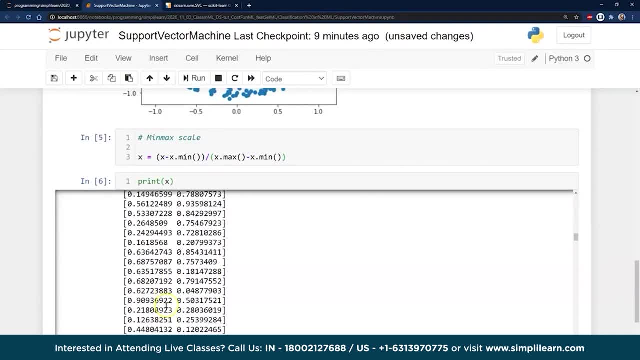 And if you look at this, all our data is 0.8, 0.5.. That's what this particular line is doing. That's a pretty common thing to do in processing data, especially in neural networks. Neural networks don't like big numbers. 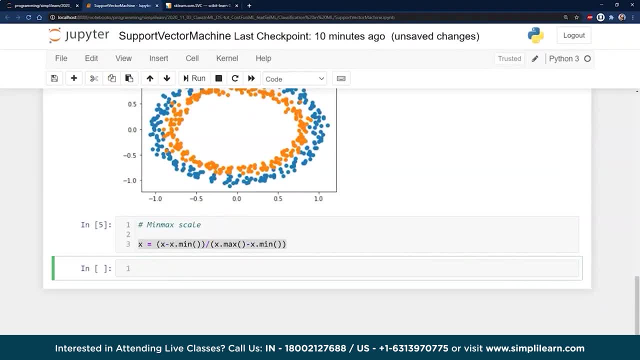 They create huge biases and cause all kinds of problems. And that's true in a lot of our models, Some of the models it doesn't really matter, But when you're doing enough of these, you just start doing them, You just start putting everything between 0 and 1.. 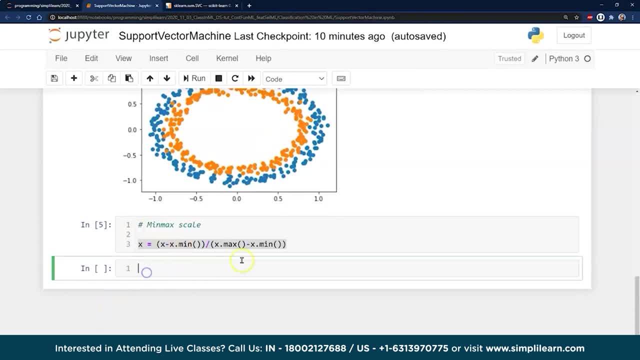 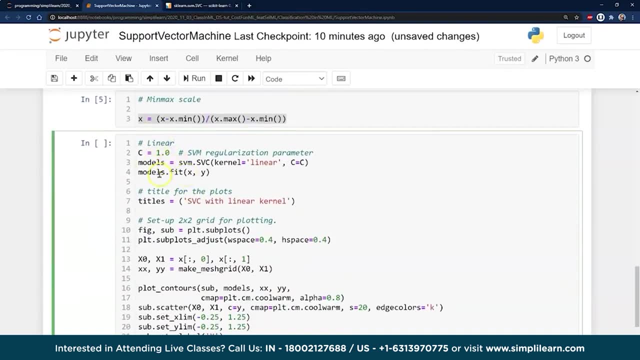 There's even some algorithms to do that in the sklearn, Although, as you can see, it's pretty easy to do it here. So let's go ahead and jump into the next thing, which is a linear kind of setup. C equals 1.0.. 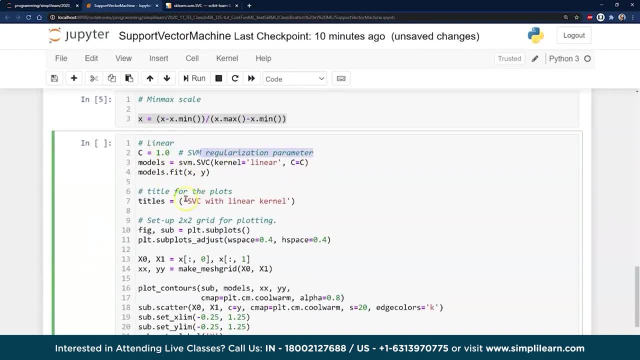 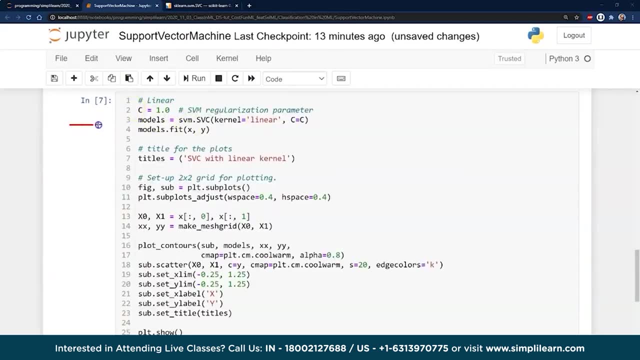 This is the SVM regularization parameter. we're going to use Models. here's our SVM And let's go ahead and scroll up just a notch. There we go. So here we are with our model. We're going to create the setup with the SVC. 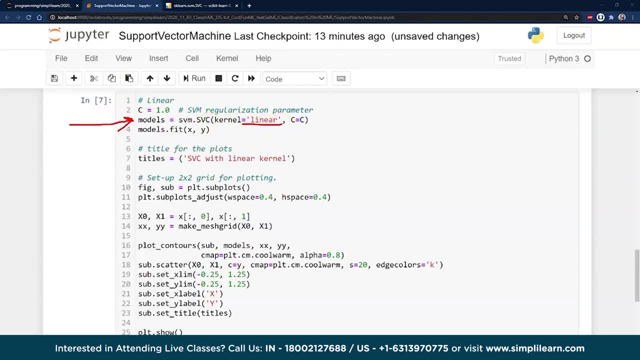 Kernel is linear And we'll come back to that because that's an important setup in there as far as what our kernel is- And you'll see why that's so important here in a minute because we're going to look at a couple of these- 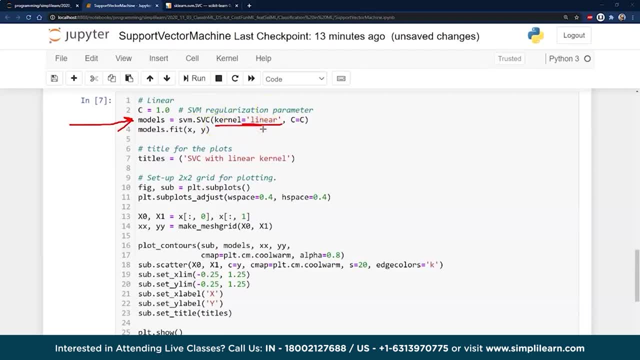 And so this one, we're actually going to be changing how that processes it. And then our C, here's our 0.0.. And then the rest of this is plotting. We're just adding titles, making the contours. so it's a pretty graph. 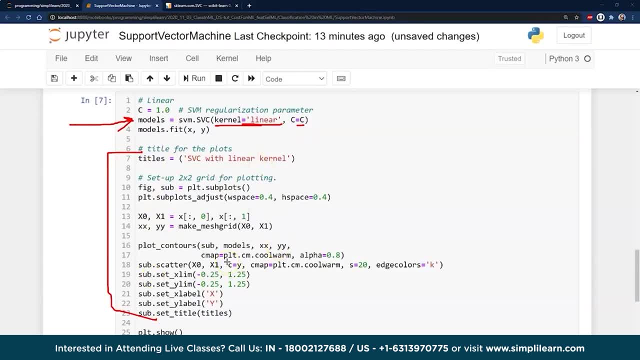 You can actually spend. this would be a whole class just to do all the cool things you can do with scatter plots and regular plots and colors and things like that. In this case, we're going to create a graph with a nice white line down the middle. 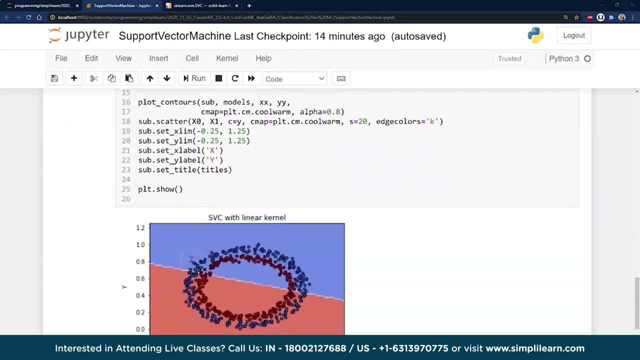 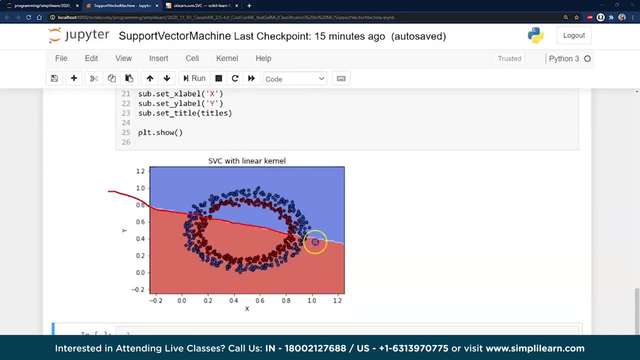 so that you can see what's going on here And when we do this, you can see that as it split the data, the linear did just that. It drew a line through the data And it says: this is supposed to be blue and this is supposed to be red. 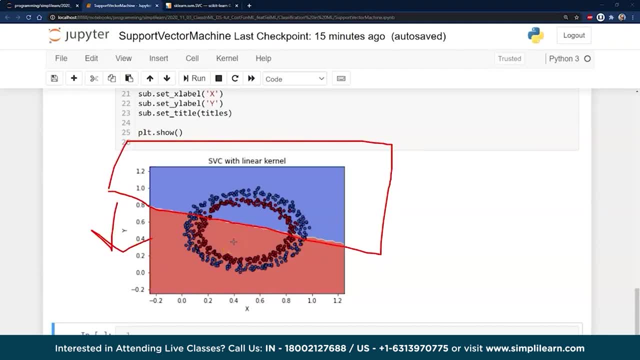 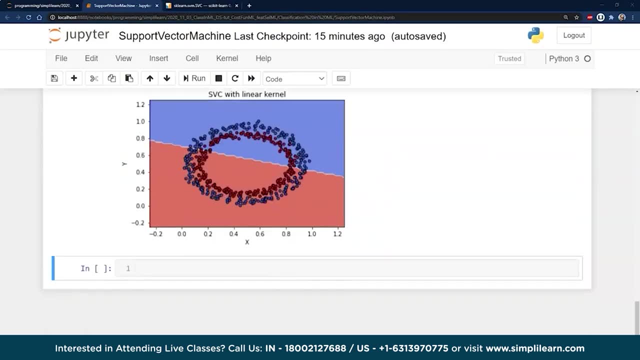 And it doesn't really fit very well, And that's because we used a linear division of the data And it's not very linear data, It's anything but linear. So when we look at that it's like, well, okay, that didn't work. 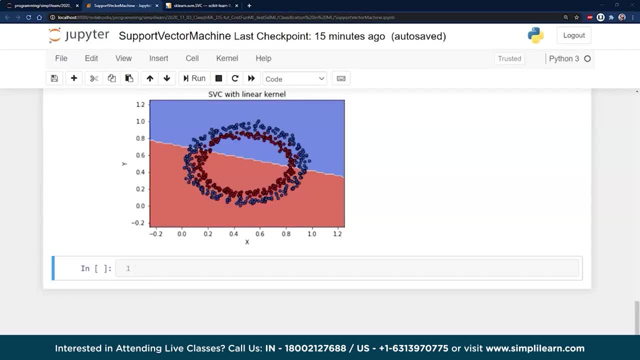 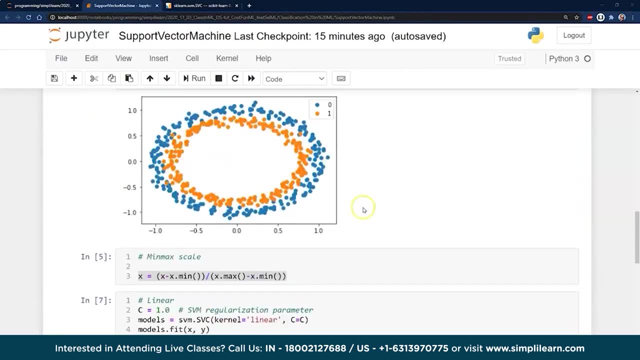 What's the next option? Well, there's a lot of choices in here. One of them is just simply: we can change this from the kernel being linear to poly, And we'll just go back up here and use the same chart. Oops, here we go. 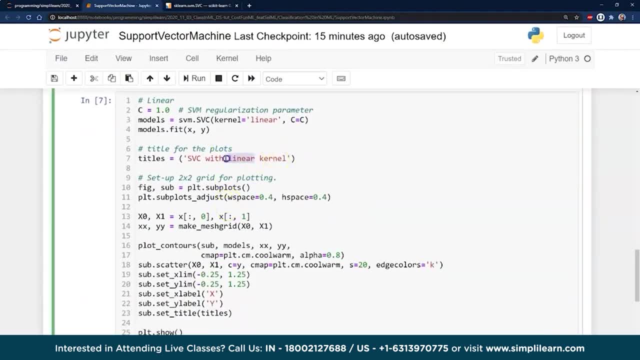 So here we go: linear kernel, We'll change this to poly, And then when we come in here and create our model- here's our model up here, linear- We can actually just go right in and change this to the poly model. 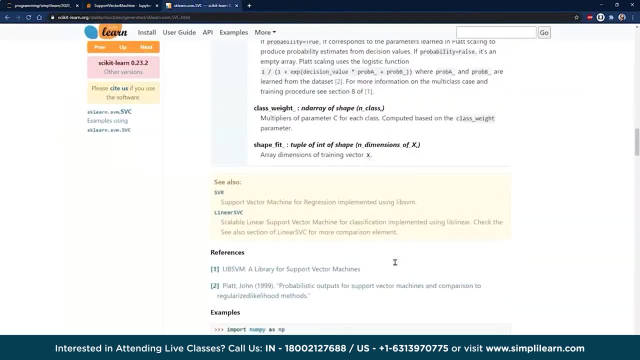 And, if you remember, when we go back over here to the SVC and let's scroll back up here, there's a lot of different options. Oops, even further. Okay, So when we come up here and we start talking about the kernel, 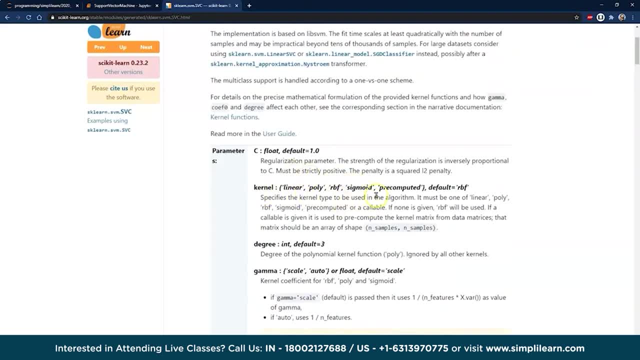 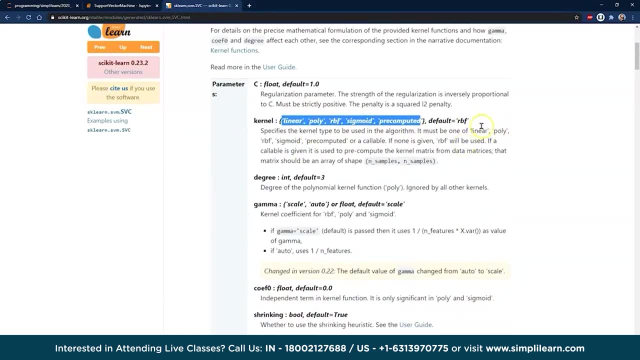 here's the kernel. There's linear, there's poly, RBF, sigmoid, precomputed. There's a lot of different ways to do this setup And their actual default is RBF. Very important to note that. So when you're running these models, 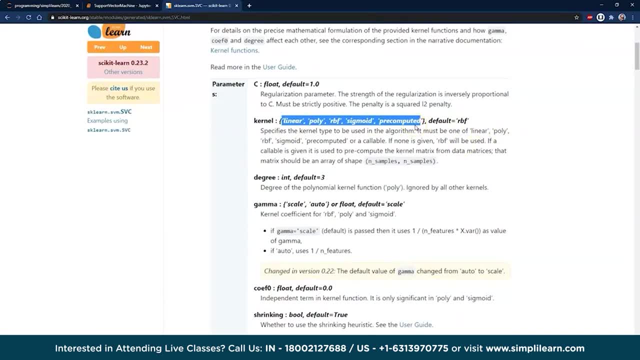 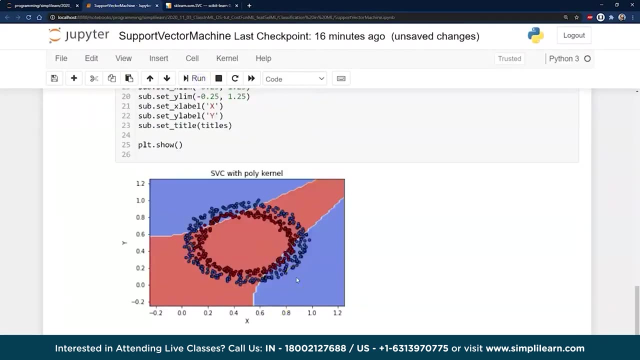 understanding which parameter really has a huge effect on what's going on. In this particular one with the SVM, the kernel is so important- You really need to know that. And we switched our kernel to poly And when we run this you can see it's changed a little bit. 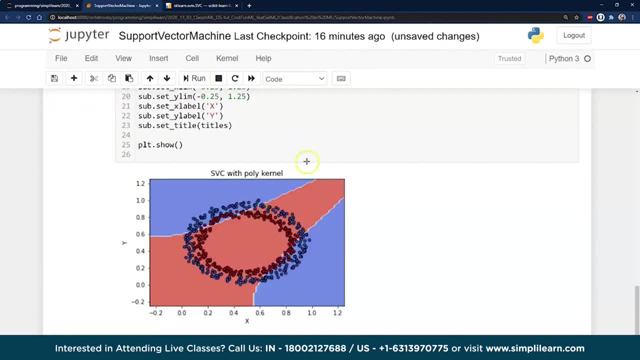 We now have quite an interesting looking diagram And you can see on here. it now has these classifications Correct, But it messes up in this blue up here And it messes up on. this blue is correct And this blue is supposed to be red. 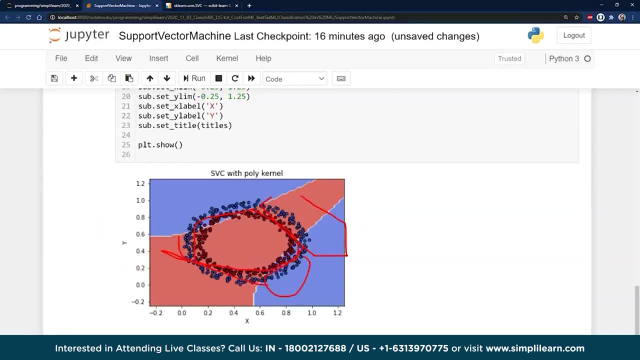 You can see that it still isn't quite fitting on there, And so that is when we do a poly fit. you can see if you have a split in data where there's a group in the middle- that's one kind of data- and the groups on the outside are different. 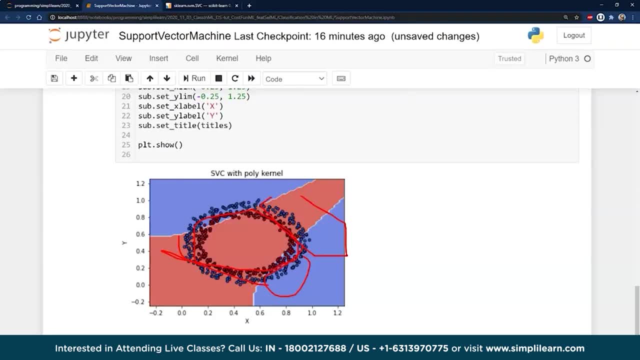 the poly fit or the poly kernel is what's going to be fit for that. So if that doesn't work, then what are we going to use? Well, they have the RBF kernel And let's go ahead and take a look and see what the RBF is. 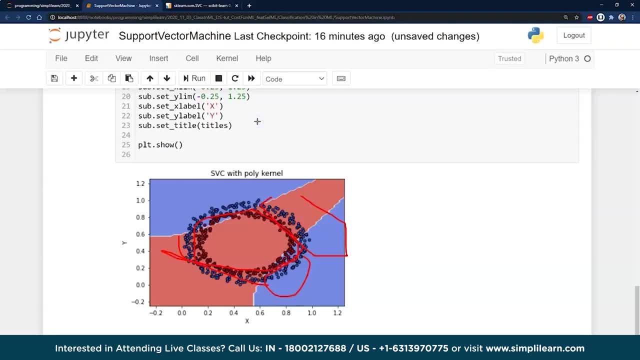 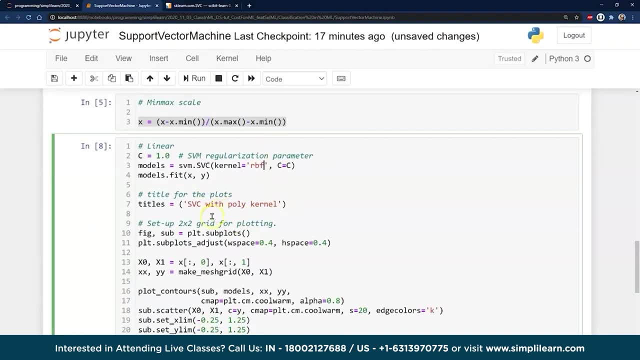 Let's see what the RBF looks like- And let me go ahead and turn my drawing off- And the RBF kernel: Oops, there we go, RBF. And then, of course, for our title. it's always nice to have it match with the RBF kernel. 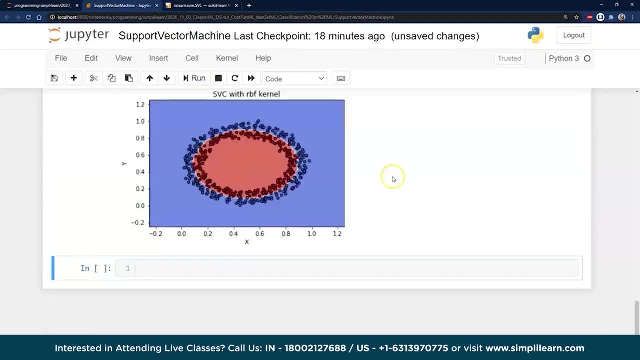 Let me go ahead and run this And you can see that the RBF kernel does a really good job. It actually has divided the data up on here And this is the kind of what you expect. here was that ring. Here's our inner ring. 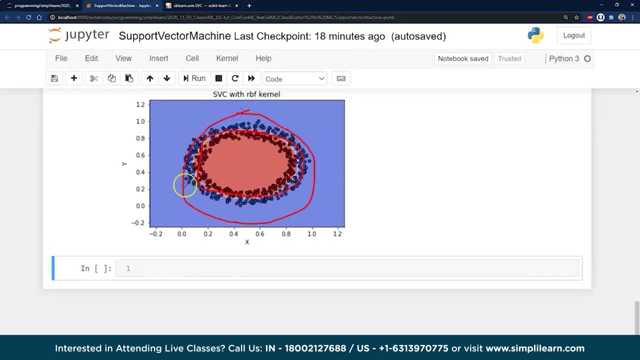 Here's an outer ring of data, So the RBF fits this data package quite nicely And that we're talking about SVM. It really is powerful in that it has this kind of sorting feature to it in its algorithms. This is something that is really hard to get. the SK means to do, or the K means set up. 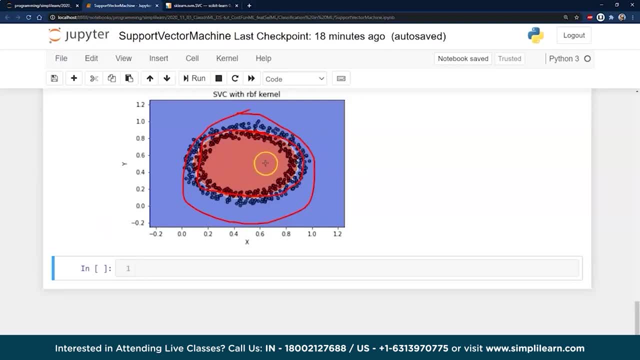 And so when you start looking at these different machine learning algorithms, understanding your data and how it's grouped is really important. It makes a huge difference as far as what you're computing and what you're doing with it. So that was a demo on the support vector. 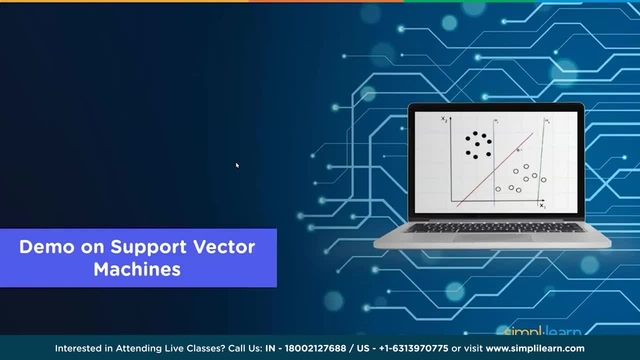 Certainly you could have continued on that and done like a confusion matrix and all that kind of fun stuff to see how good it was, and split the data up to see how it vectorizes. The visual on. that is so important. It makes a big difference just to see what it looks like and that giant donut. 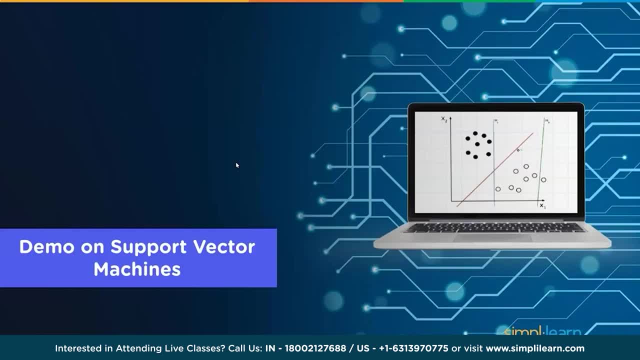 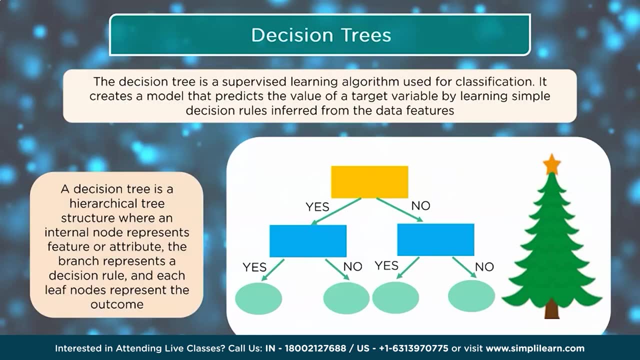 and why it does circles so well, or your poly version or your linear version. So we've looked at some very numerical kind of setups where there's a lot of math involved- Euclidean geometry, that kind of thing. A totally different machine learning algorithm for approaching this is the decision trees. 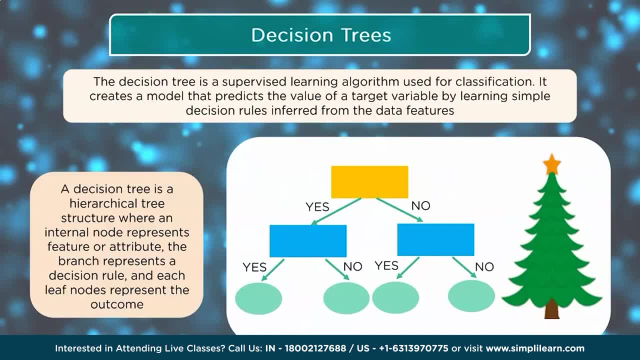 And there's also forests that go with the decision trees. They're based on multiple trees combined. The decision tree is a supervised learning algorithm used for classification. It creates a model that predicts the value of a target variable by learning simple decision rules inferred from the data features. 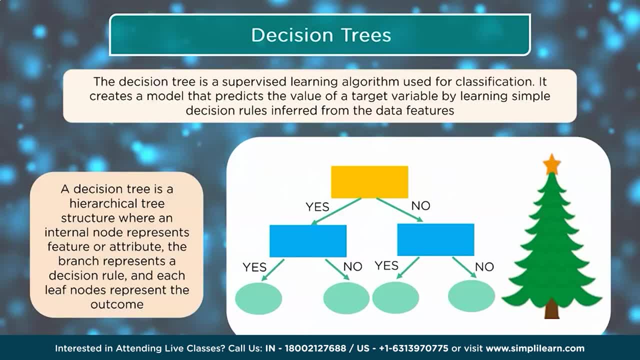 A decision tree is a hierarchical tree structure where an internal node represents features or attribute, The branch represents a decision rule and each leaf node represents the outcome. And you can see here where they have the first one- yes or no- And then you go either left or right, and so forth. 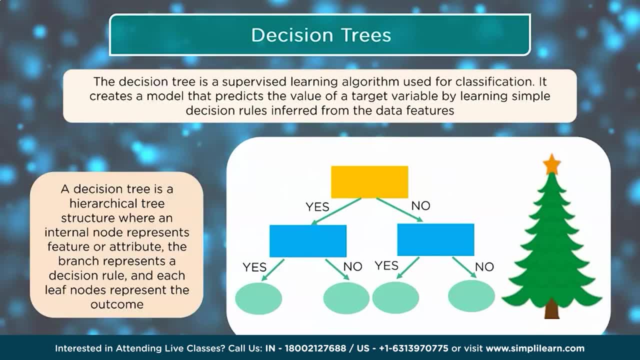 One of the coolest things about decision trees- and I'll see people actually run a decision tree, even though their final model is different- because the decision tree allows you to see what's going on. You can actually look at it and say: did you go right or left? 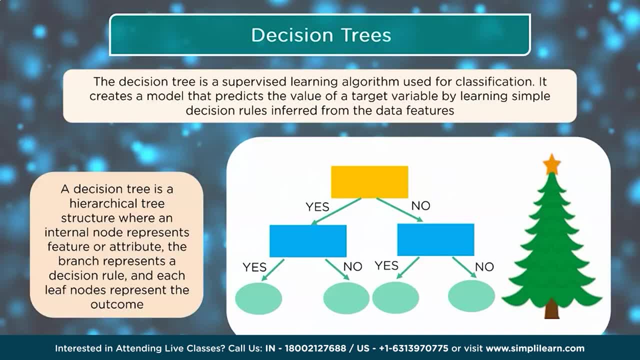 What was the choice? Where's that break? And that is really nice if you're trying to share that information with somebody else as to why, When you start getting into the why this is happening, decision trees are very powerful, So the topmost node of a decision tree is known as the root node. 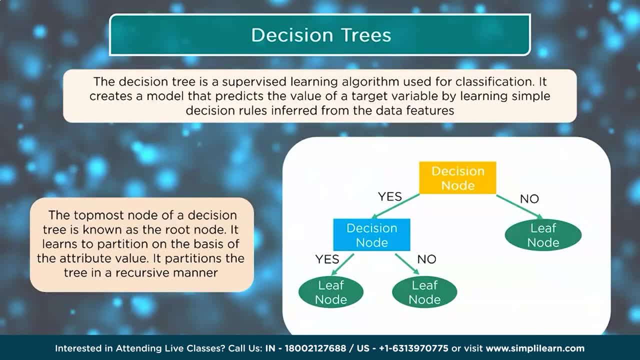 It learns to partition on the basis of the attribute value. It partitions the tree in a recursive manner, So you have your decision node. If you get yes, you go down to the next node. That's a decision node. And either yes, you go to if it ends on a leaf node. 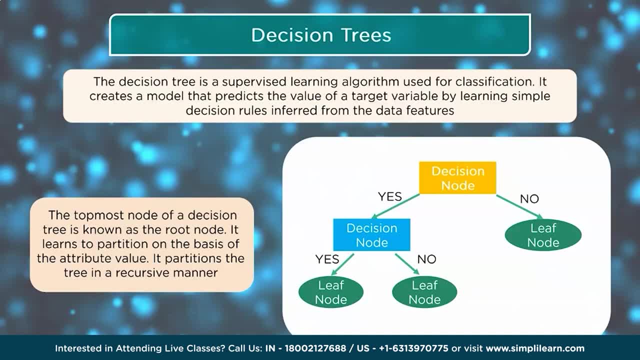 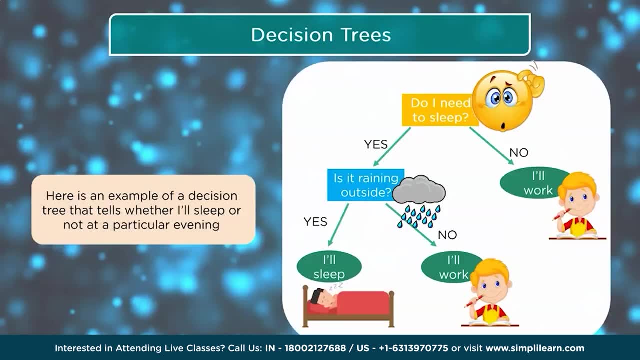 then you know your answer, which is yes or no. So there's your end classification set up on there. Here's an example of a decision tree that tells whether I'll sleep or not at a particular evening. Mine would be depending on whether I have the news on or not. 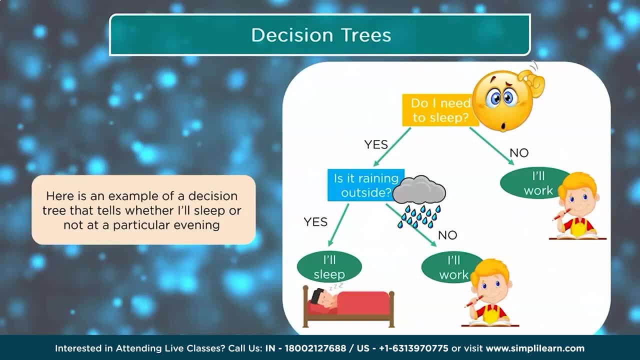 Do I need to sleep? No, Okay, I'll work, Yes. is it raining outside? Yes, I'll sleep. No, I'll work. So I guess if it's not raining outside it's harder to fall asleep where you have that nice rain. 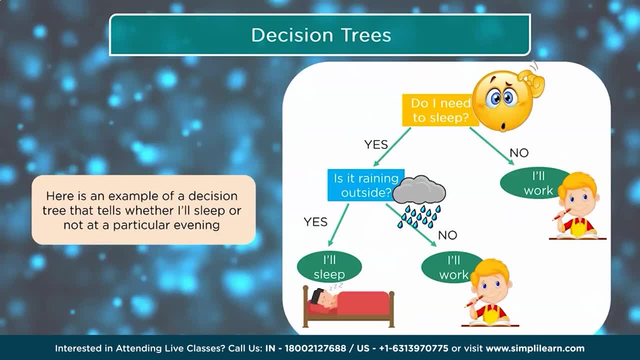 And again, this is really cool about a decision tree is I can actually look at it and go, oh, I like to sleep when it rains outside. So when you're looking at all the data, you can say, oh, this is where the switch comes in. 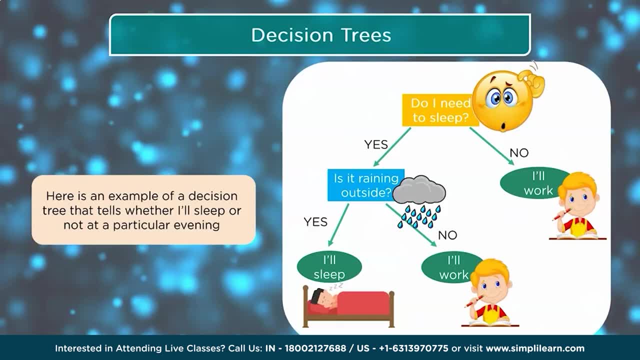 When it rains outside, I'll sleep really good. If it's not raining, or if I don't need sleep, then I'm not going to sleep, I'm going to go work. So let's go ahead and take a look at what that looks like in the code. 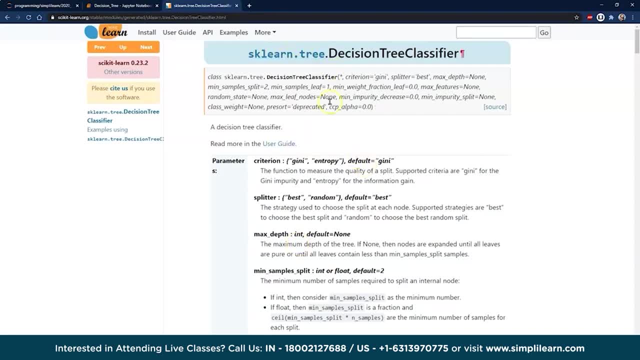 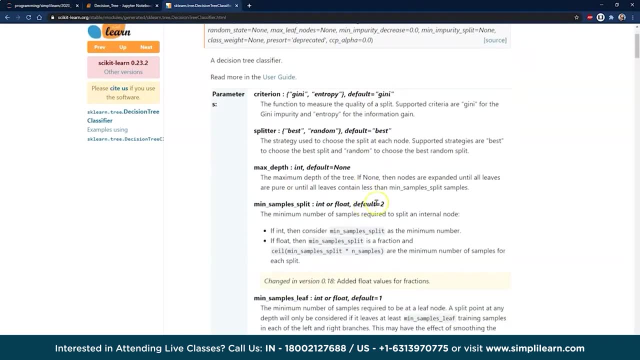 Just like we did before we go ahead and open up the site kit set up just to say what the decision tree classifier has. You have your parameters, which will look a little bit more interesting. We're in depth that as we write the code. 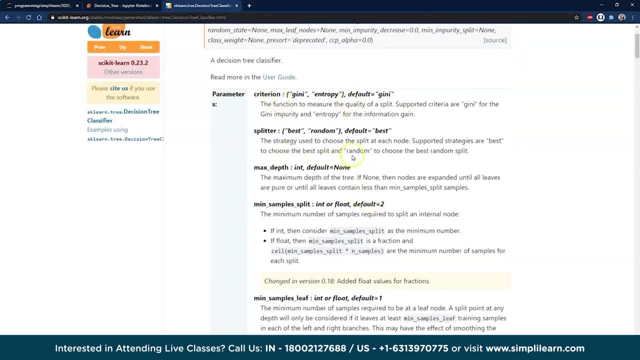 It has different ways of splitting it. The strategy used to choose a split at each node. criterion: max depth. Remember the tree. how far down do you want it? Do you want it to take up the space of your whole computer and map every piece of data? 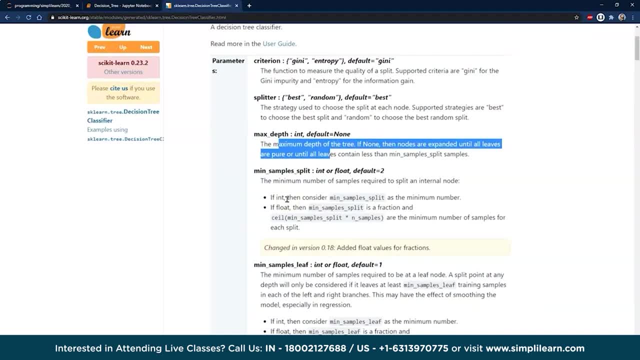 Or the smaller that number is, the smaller the level of the tree is and the less processing it takes. But it's also more general, so you're less likely to get as in-depth an answer. And then, of course, minimal samples. 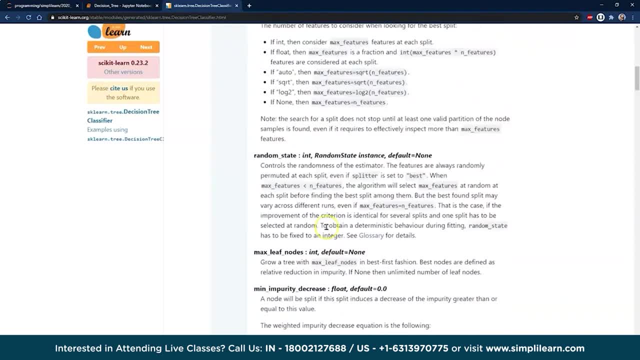 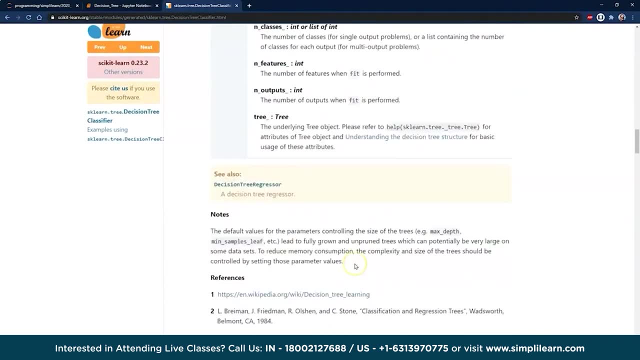 You need for it to split samples for the leaves. There's a lot of things in here as far as how big the tree is and how to define it and when do you define it and how to weight it, And they have their different attributes. 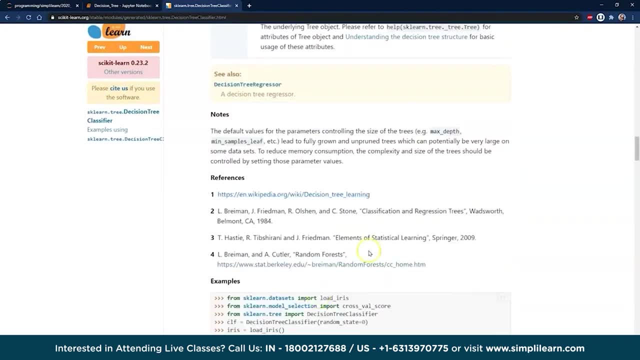 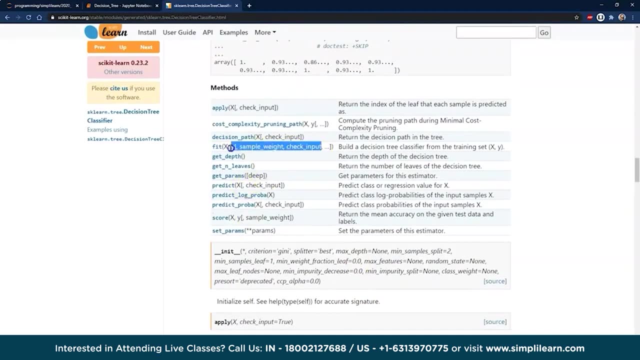 which you can dig deeper into. that can be very important if you want to know the why of things. And then we go down here to our methods and you'll see, just like everything else, we have our fit method- very important- and our predict. 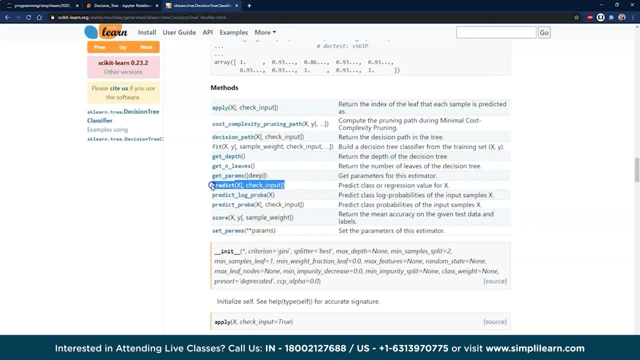 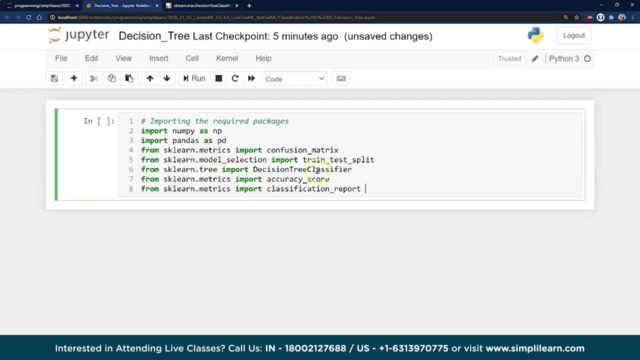 the two main things that we use. What are we going to predict our x to be equal to? We'll go ahead and go up here and start putting together the code. We're going to import our numpy, our pandas. there's our confusion- matrix. 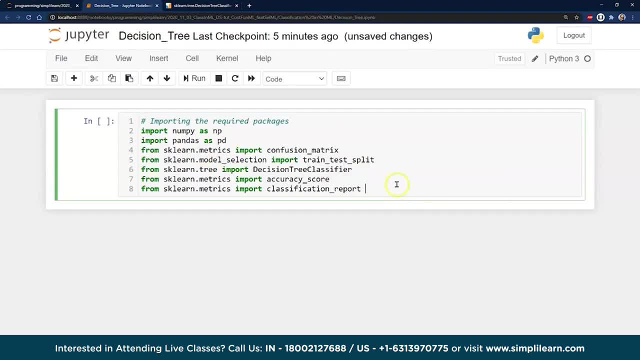 our train test split decision tree classifier. that's the big one that we're actually working with. That's the line right here where we're going to be. oops, decision tree. there it is Decision tree classifier. that's the one I was looking for. 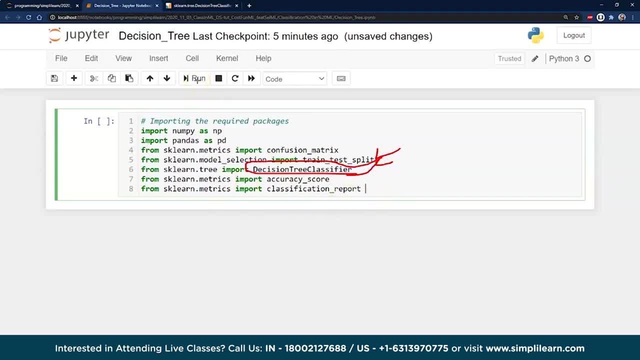 And of course we want to know the accuracy and the classification report on here And we're going to do a little different than we did in the other examples. There's a reason for this. Let me go ahead and run this and load this up here. 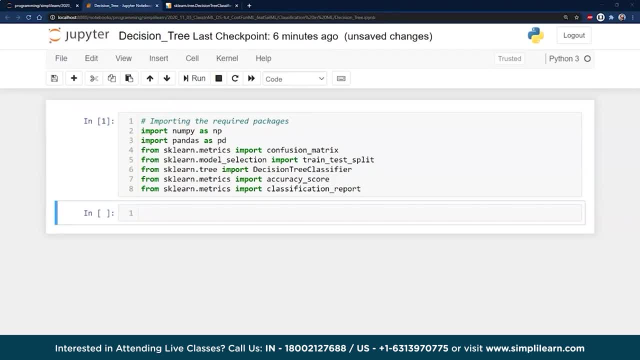 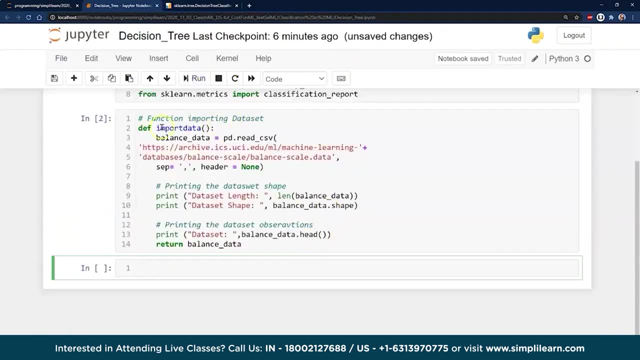 We're going to go ahead and build things on functions, And this is when you start splitting up into a team. this is the kind of thing you start seeing a lot more, Both in teams and for yourself, because you might want to swap one data. 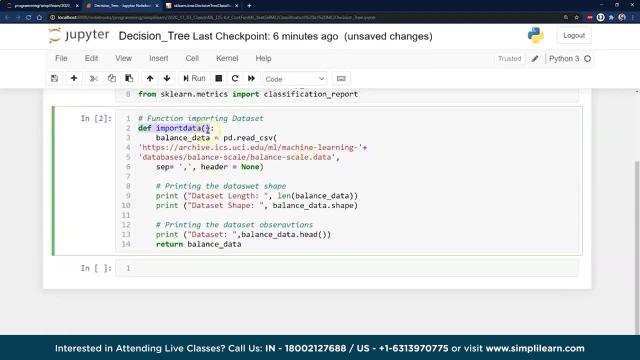 to test it on a different data depending on what's going on. So we're going to have our import data here: the data set, length, the balance and so forth. This just returns balance data. Let me just go ahead and print some materials as to what this looks like. 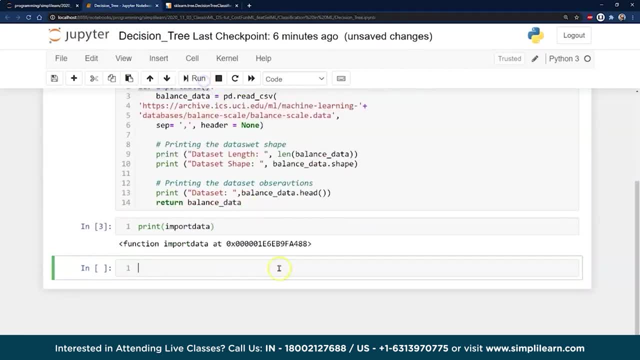 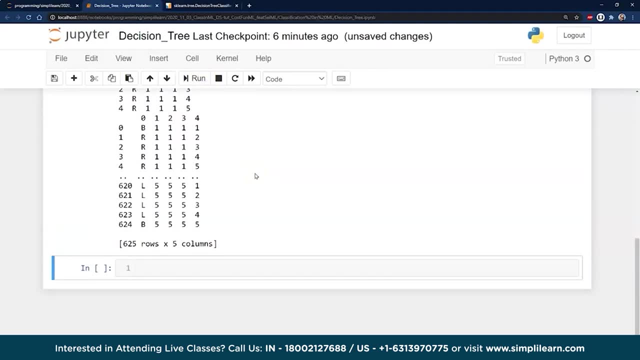 Import data And it's going to return the balance data. So if I run that, if we go ahead and print this out here and run that, you can see that we have a whole bunch of data that comes in there and some interesting setup on here has. 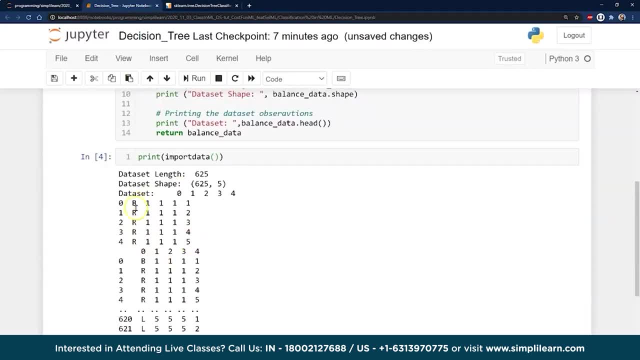 let's see BRR- I'm not sure exactly what that represents- on here 111,, 112, and so forth. So we have a different set of data here. The shape is five columns: one, two, three, four, five. 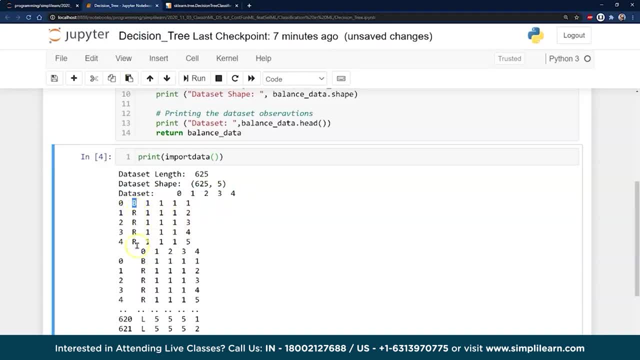 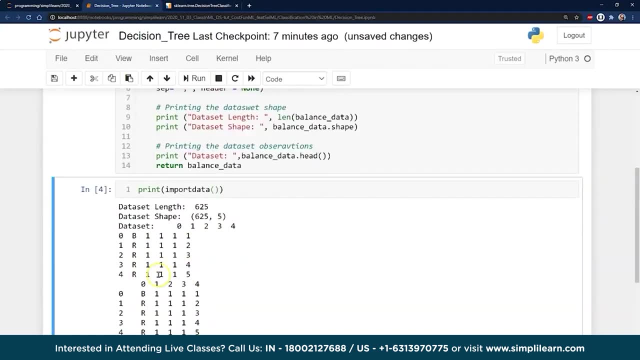 It seems to have a number at the beginning, which I'm going to guess- BRL, a letter I mean, And then a bunch of numbers in there: 1111,. let's see down here we've got 555.. Setup on this. 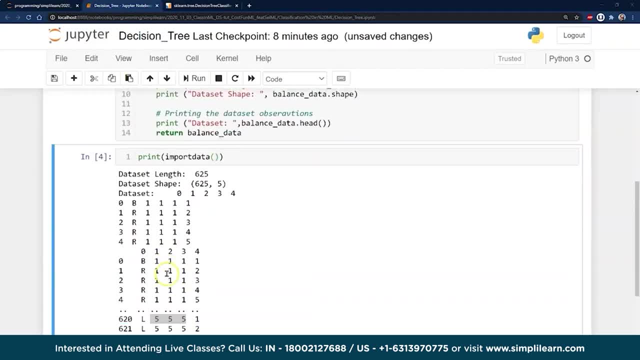 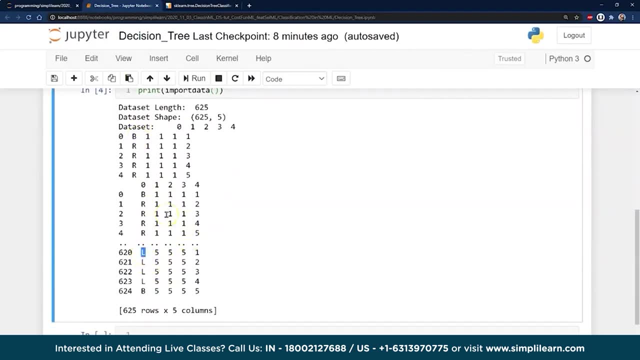 And let's see balance data. And since it said balance data, I'm going to guess that B means balanced, R means you need to move it right and L means it needs to be moved left or skewed to the left. I'm not sure which one. 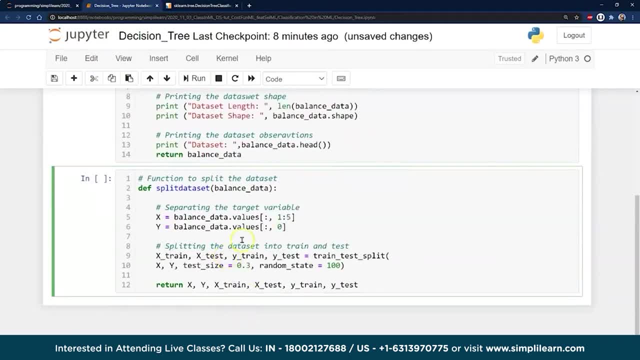 Let's go ahead and close that out. We have a function to split the data set. X balance data equals data values. Y balance equals data values of zero. There's that letter, Remember left, right and balance. Then we're looking for the values of one through five. 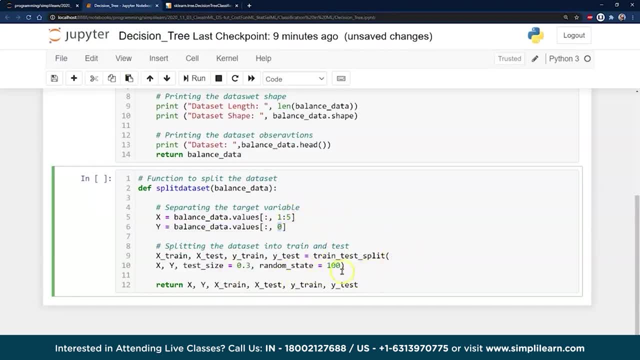 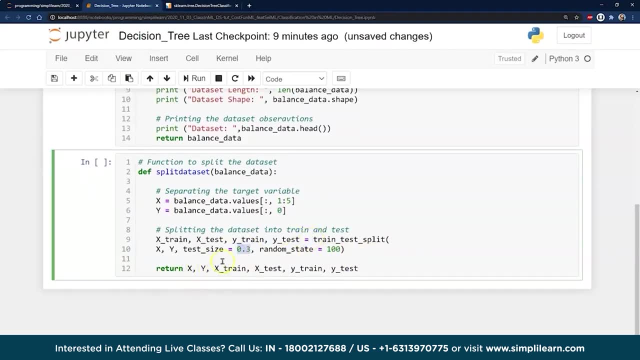 And we go ahead and split it just like you would: X, train, Y train set, random state 100.. Test size is .3, so we're taking 30% of the data And it's going to return your X, your Y, your Y train your. 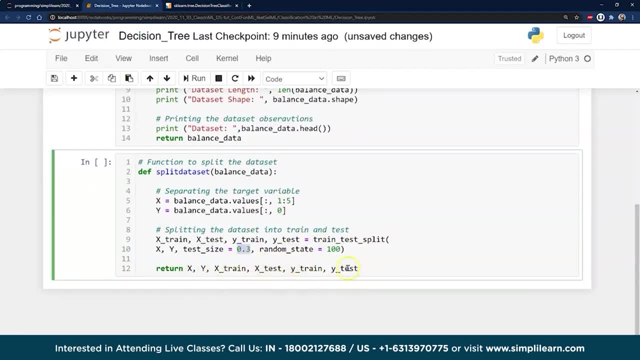 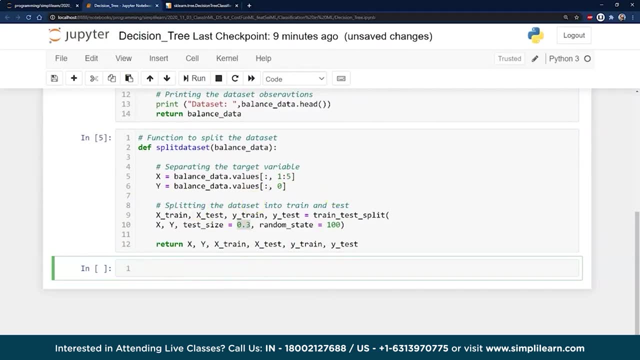 X. train your X test your Y. train your Y test Again. we do this because if you're running a lot of these, you might want to switch how you split the data and how you train it. I tend to use a bifold method. 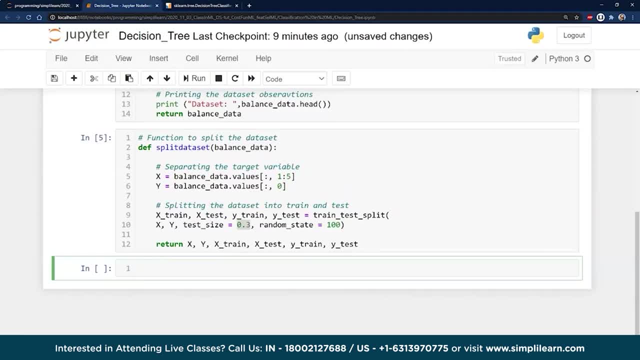 I'll take a third of the data and I'll train it on the other two thirds and test it on that third and then I'll switch it. I'll switch which third is the test data And then I can actually take that information and correlate it. 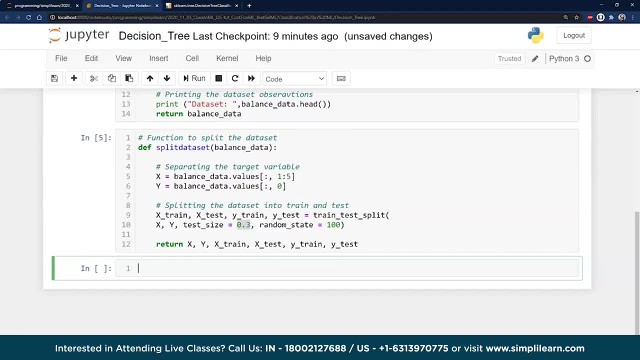 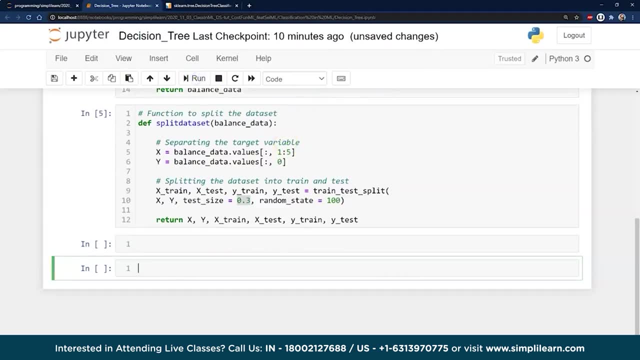 and it gives me a really robust package for figuring out what the complete accuracy is. But in this case we're just going to go ahead. this is our function for splitting data, And this is where it kind of gets interesting, because, remember, we were talking a little bit about. 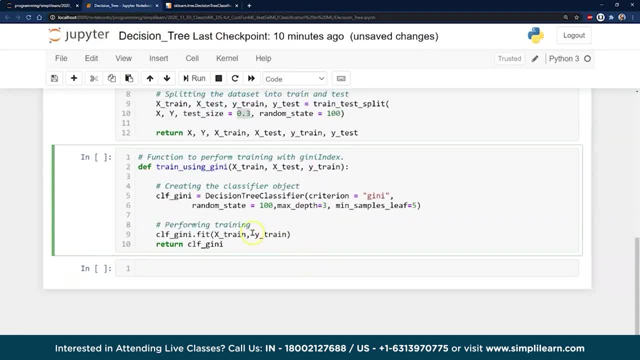 the different settings in our model, And so in here we're going to create a decision tree, but we're going to use the genie setup. And where did that come from? What's the genie on here? So if we go back to the 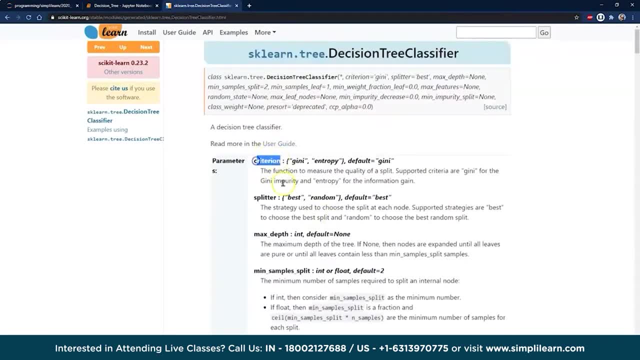 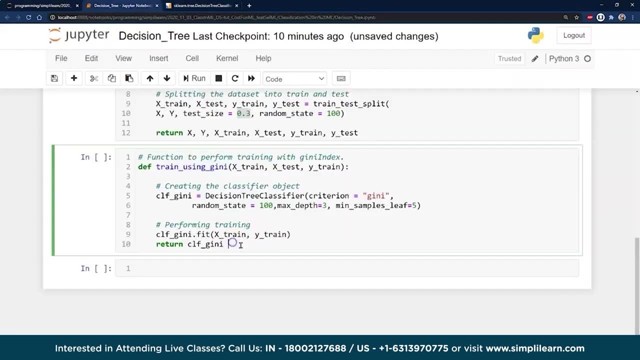 top of their page and we have: what criterion are we going to use? We're going to use genie. They have genie and entropy. Those are the two main ones that they use for the decision tree. So this one's going to be genie. 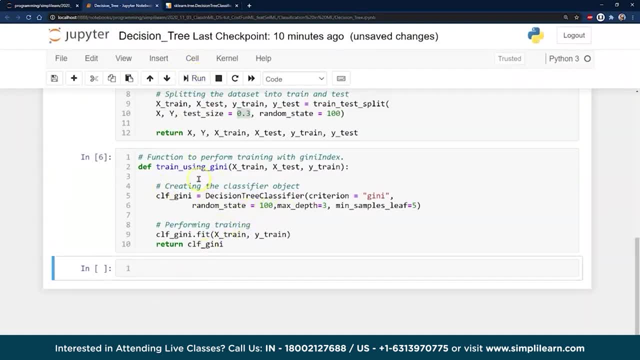 and if we're going to have a function that creates the genie model- and it even goes down here and here's our fit train of the genie model- we'll probably also want to create one for entropy. Sometimes I even- just I- might even make this just one function. 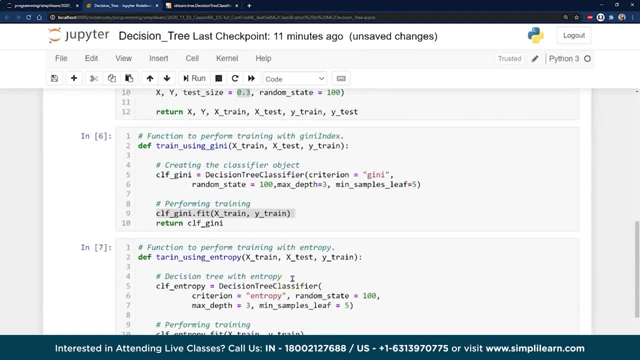 with the different setups, and I know one of the things I worked on recently: I had to create one that tested across multiple models, And so I would send the parameters to the models, or I would send this part right here where it says decision tree classifier. 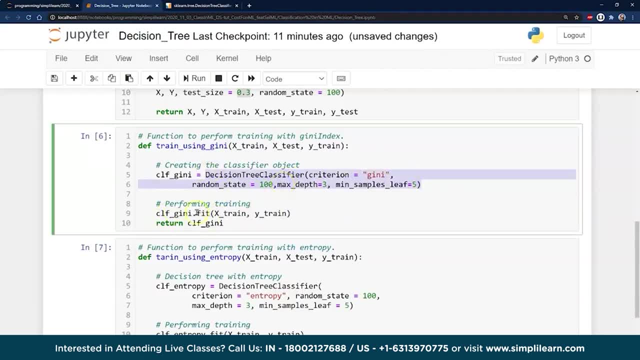 That whole thing might be what I send to create the model and I know it's going to fit. We're going to have our x train and we're going to have our predict and all that stuff is the same, So you can just send that. 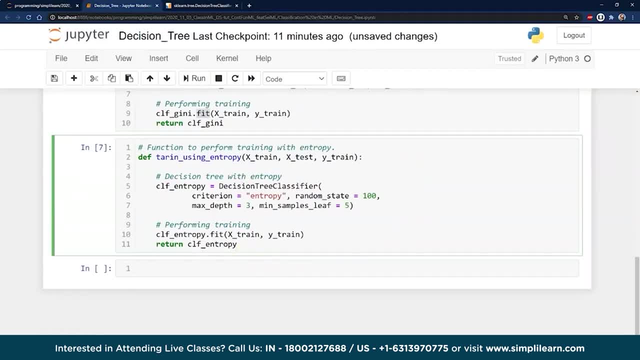 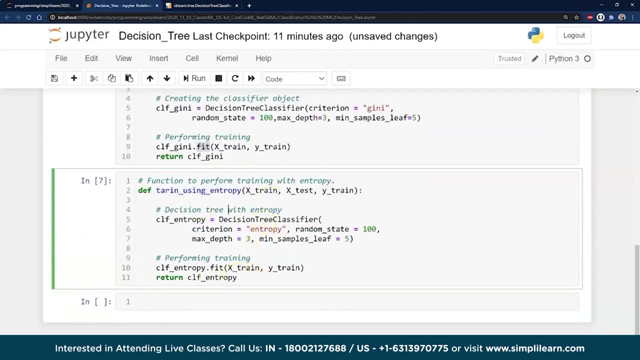 model to your function for testing different models. Again, this just gives you one of the ways to do it And you can see, here we're going to train with the genie and we're also going to train with the entropy to see how that works. 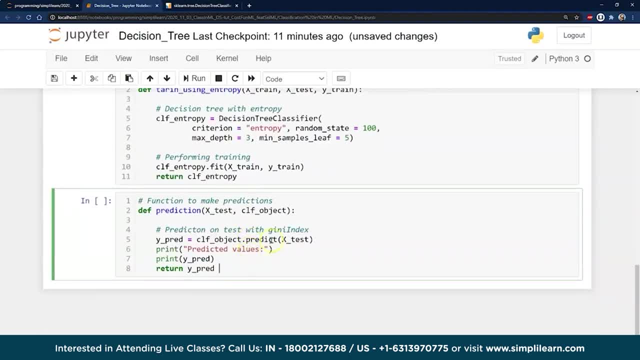 And if you're going to have your models going, two separate models you're sending there- we'll go ahead and create a prediction. This simply is our y predict equals our whatever object we sent, whatever model we sent here, the CLF object, and predict against our x test. 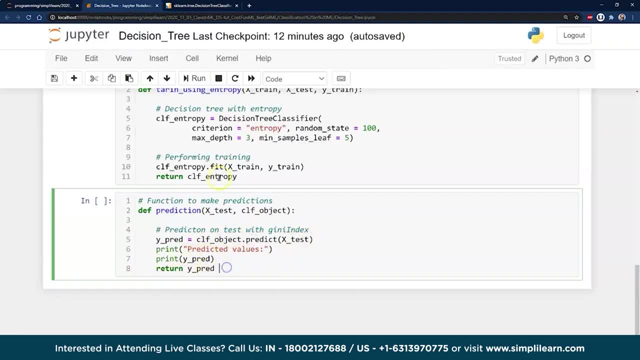 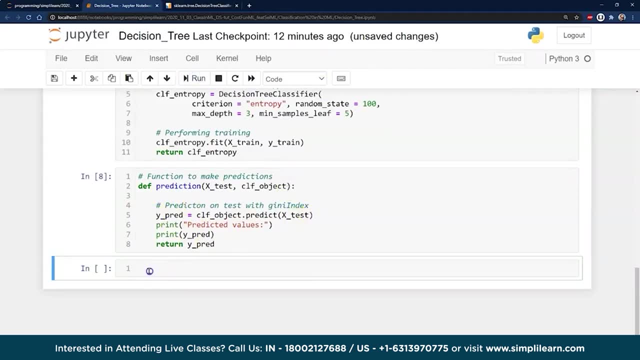 And you can see here: print y predict and return y predict set up on here. We'll load that definition up And then if you're going to have a function that runs a predict and prints some things out, we should also have our accuracy function. 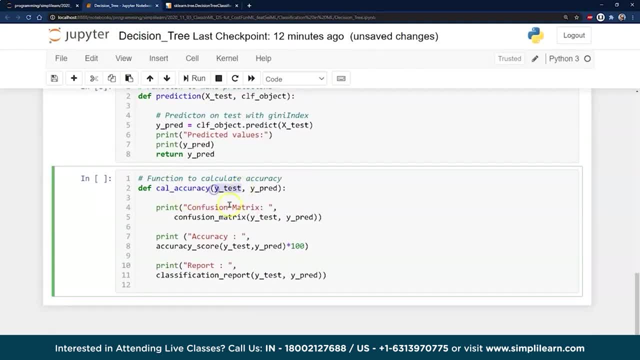 So here's our calculate the accuracy. what are we sending? We're sending our y test data. This could also be y actual and y predict- And then we'll print out a confusion matrix. then we'll print out the accuracy of the score on here and print a report. 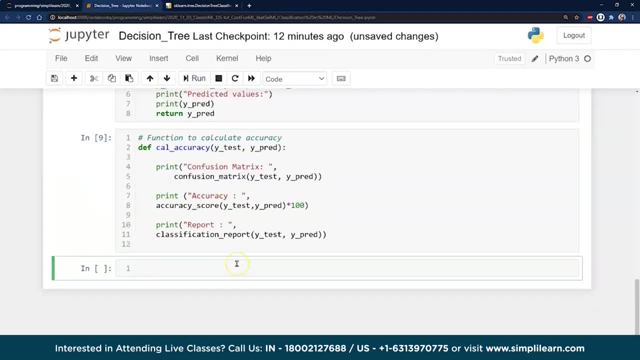 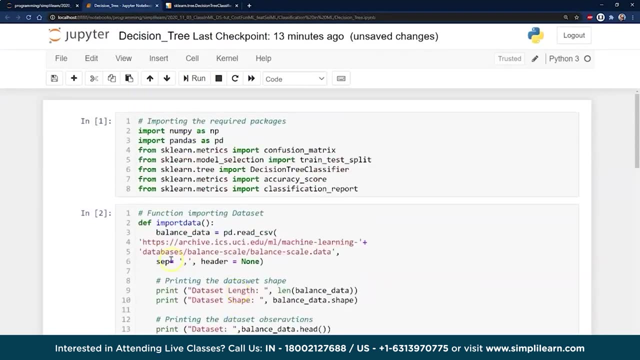 classification report. Bundle it all together there. So if we bring this all together, we have all the steps we've been working towards, which is importing our data. by the ways, you'll spend 80% of your time importing data in most machine learning setups and cooking it and burning it. 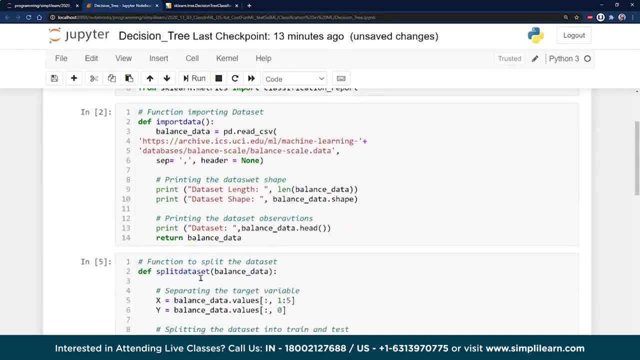 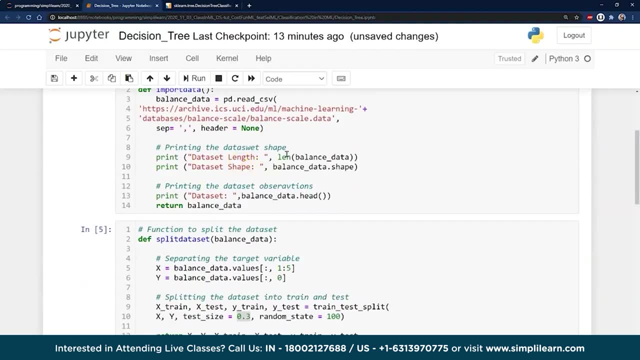 and getting it formatted so that it works with whatever models you're working with. The decision tree has some cool features in that if you're missing data, it can actually pick that up and just skip that and says: I don't know how to split this, there's no way of knowing whether it rained or didn't. 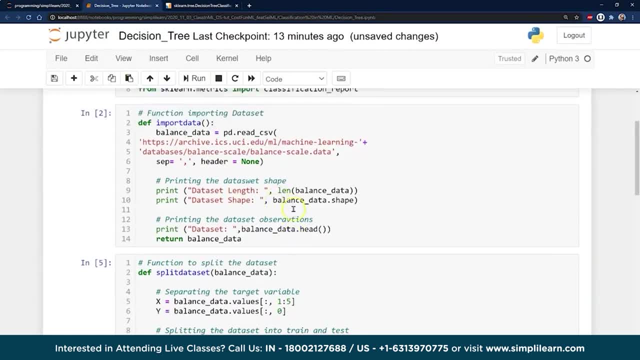 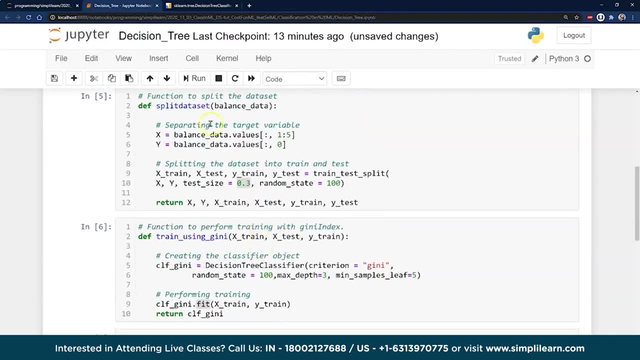 rain last night, so I'll look at something else, like whether you watched TV after 8 o'clock. you know that blue screen thing. So we have our function, importing our data set, We bring in the data, we split the data, so we have. 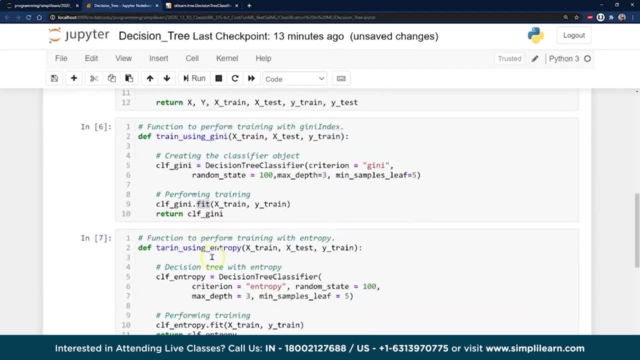 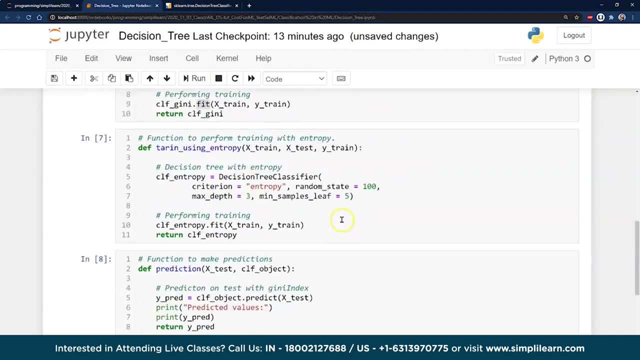 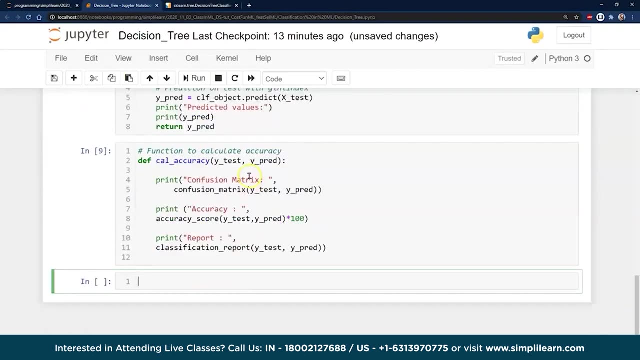 our xtest test and ytrain and then we have our different models, our clf genie, so it's a decision tree classifier using the genie setup and then we can also create the model using entropy. And then, once we have that, we have our function for making the prediction and we 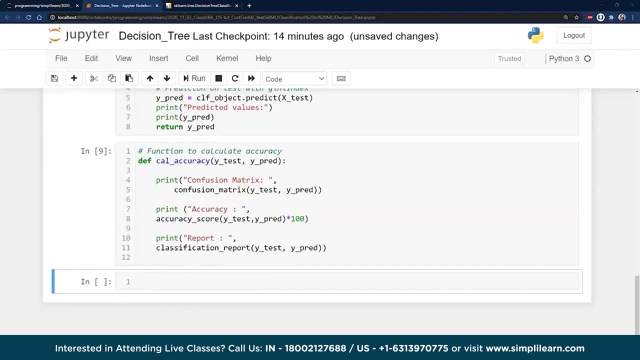 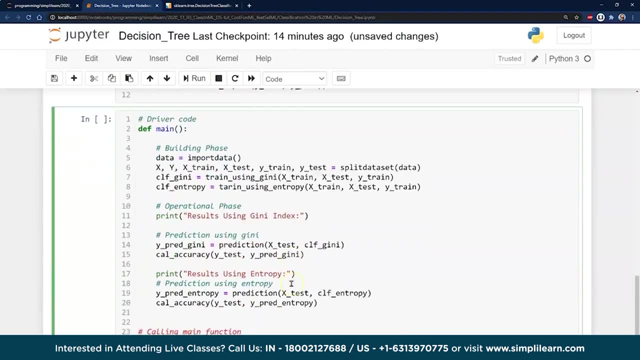 have our function for calculating the accuracy And then, if we're going to have that, we should probably have our main code involved here. This probably looks more familiar if you're depending on what you're working on. if you're working on like a PyCharm, then you would see this in throwing. 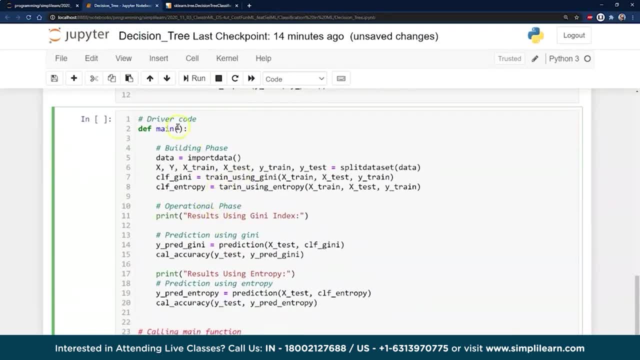 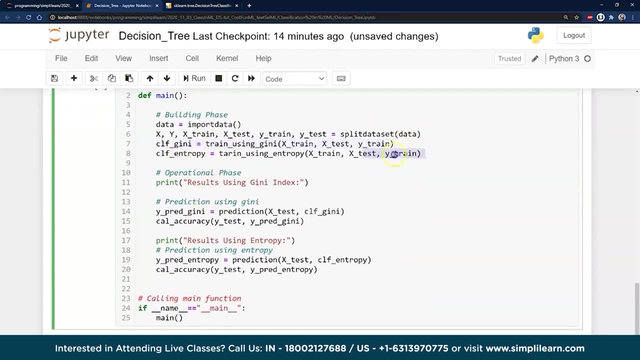 something up real quick in Jupyter Notebook. So here's our main data import, which we've already defined. We get our split data, we create our genie, we create our entropy. so there's our two models going on here. There's our two models. So these are two separate. 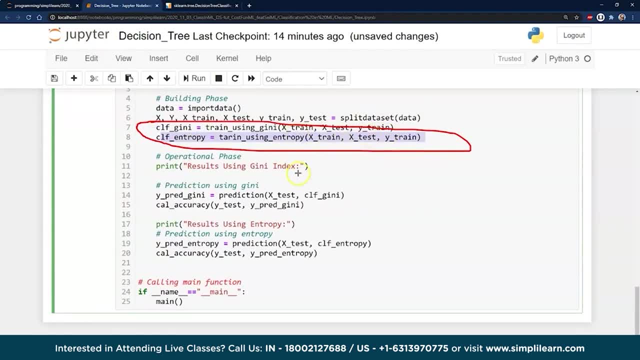 data models. We've already sent them to be trained. Then we're going to go ahead and print the results using genie index. So we'll start with the genie and we want to go ahead with the genie and print our predictions. Y, X. 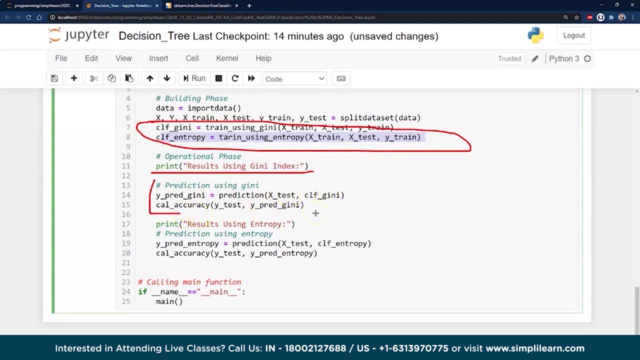 test to the genie and calculate the accuracy on here, And then we want to print the results using entropy. So this is just the same thing coming down. like we did with the genie, We're going to put out our Y- predict entropy- and our calculations. So let's. 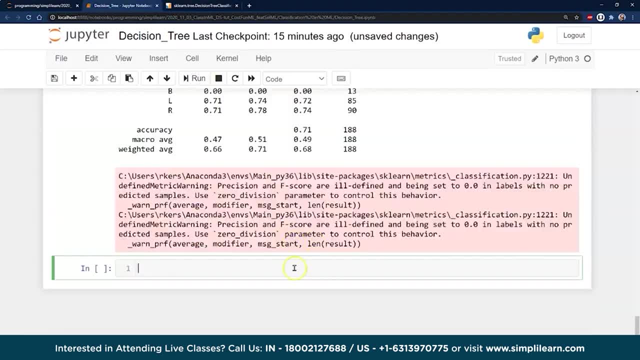 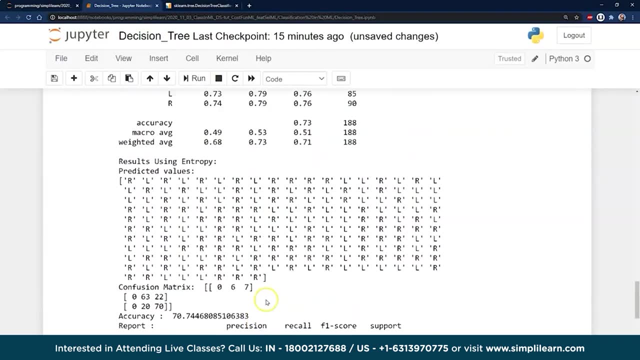 go ahead and run that and just see what this piece of code does. We do have like one of our data needs to be getting a warning on there. That's nothing major because it's just a simple warning. Probably an update of a new version is coming out. 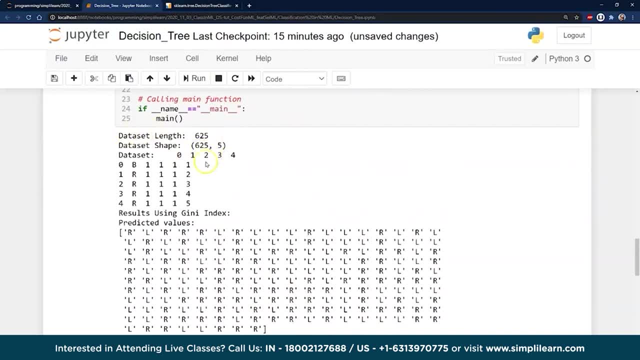 And so here we are, We have our data set. It's got 625.. You can actually see an example of the data set B meaning balanced, I guess, And here's our five data points- 1111 means it's balanced. 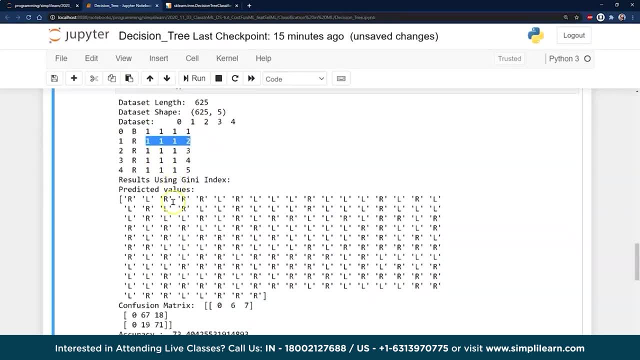 It's skewed to the right, with 1112 and so forth on here, And then we're going to go ahead and predict from our prediction whether it's to the right or to the left. You can think of a washing machine that's banging on one side of the 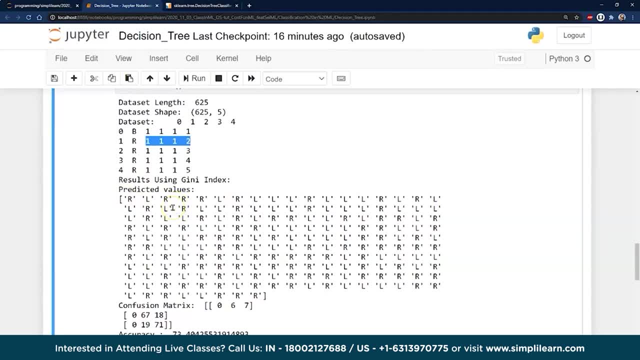 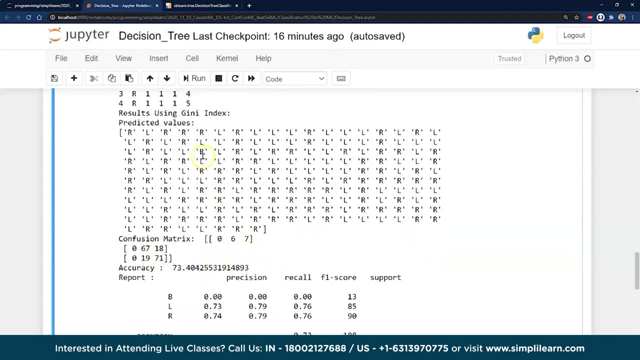 thing. or maybe it's an automated car, where we're down the middle of the road that's in balance and it starts going, veering to the right, so we need to correct for it. And when we print out the confusion matrix, we have three different variables. 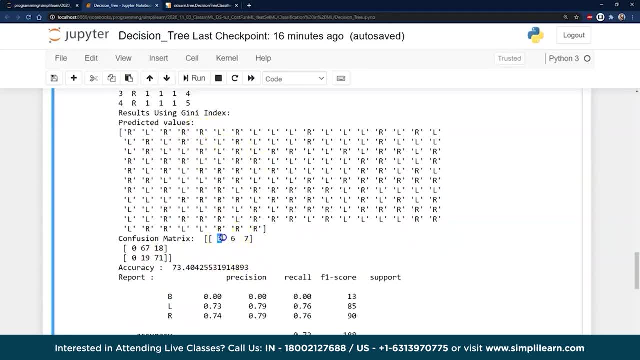 R, L and B. So we should see the three different variables on here And you have as far as whether it predicts, in this case, the balance. There's not a lot of balanced loads on here And didn't do a good job guessing whether it's balanced. 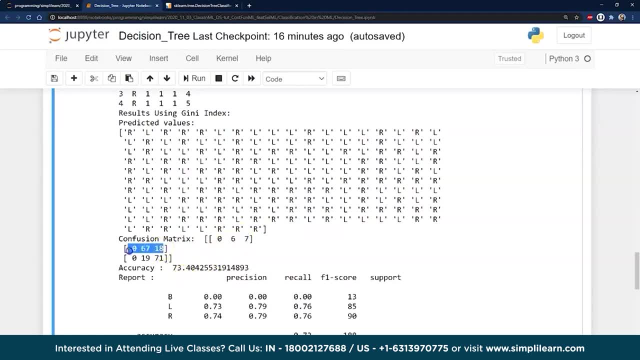 or not. That's what I took from this first one. The second one I'm guessing is the right. So it did a pretty good job guessing the right balance. You can see that a bunch of them came up left unbalanced- Probably not good for an automated car. 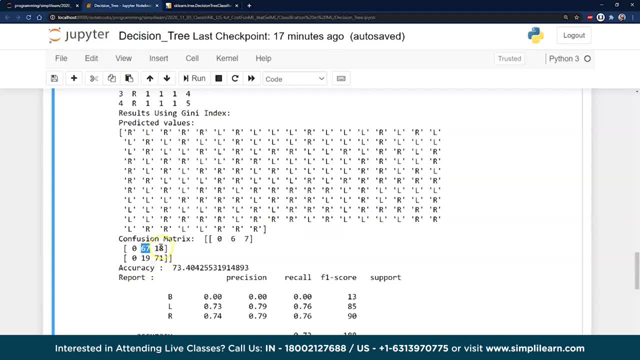 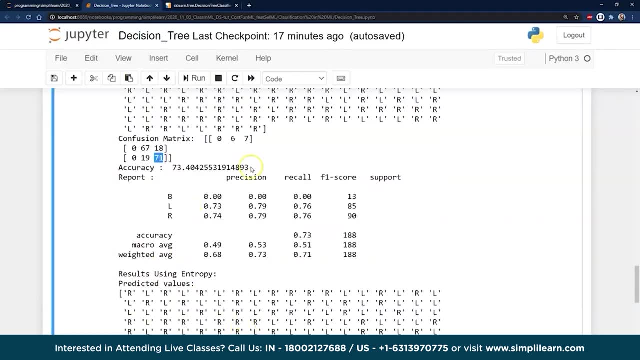 as it tells you 18 out of the 18 missed things and tells you to go the wrong direction. And here we are going the other way: 19 to 71. And of course we can back that up with an accuracy report on here and you can see the precision. 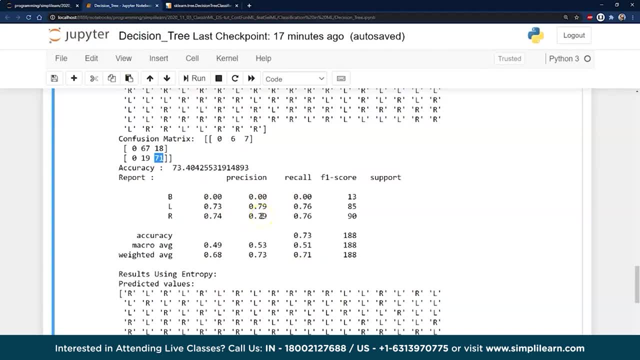 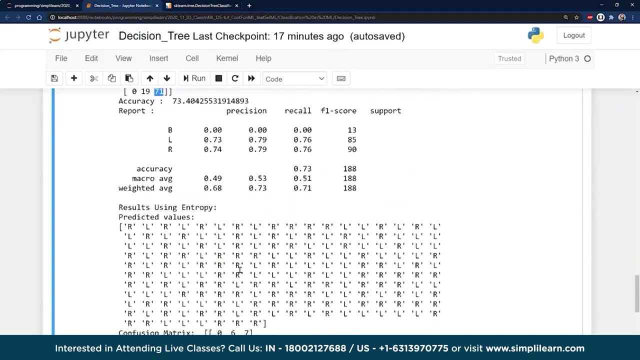 how well the left and right balance is 79%, 79% precision and so forth. And then we went and used the entropy and let me just see if we can get. so we can get them both next to each other. Here's our entropy of: 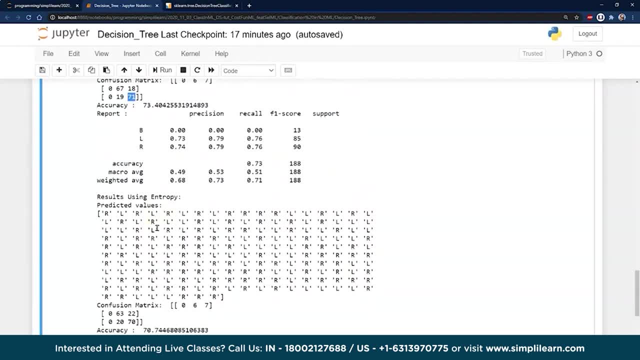 the first set up Our first model, which is the genie model 67, 18, 19, 71, 63, 22, 20, 70. Pretty close The two models. you know that's not a huge difference in numbers. This second, one of, 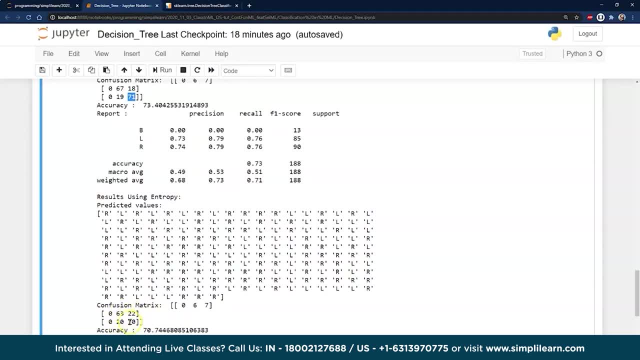 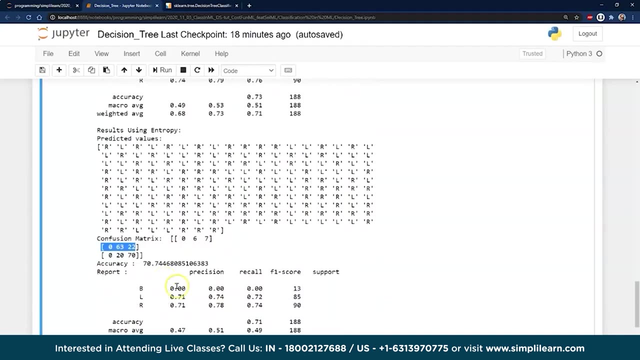 entropy did slightly. it looks like slightly worse because it did one better as far as the right balance and did what? is this? four worse on the left balance or whatever. So slightly worse. If I was guessing between these, I'd probably use the first one. They're so. 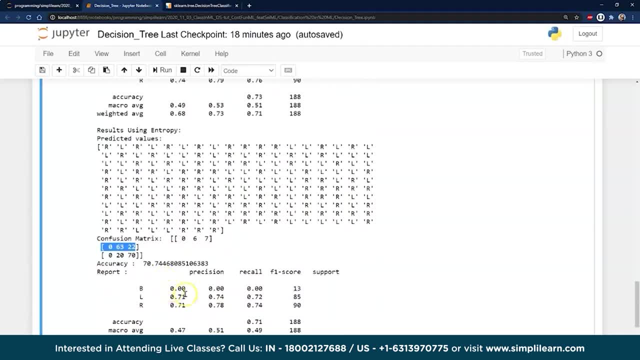 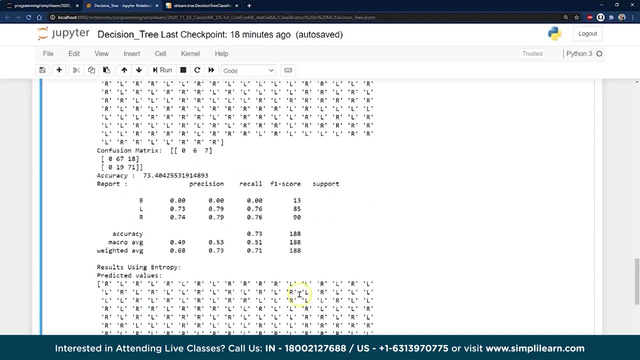 close, though that wouldn't be. it wouldn't be a clear choice as to which one worked better, And there's a lot of numbers you can play with here which might give better results, depending on what the data is going in. Now, one of the takeaways you should have from 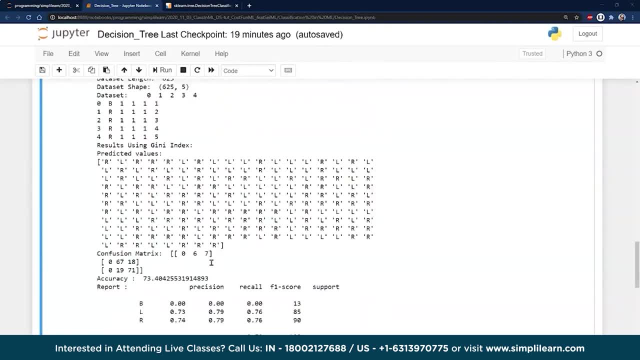 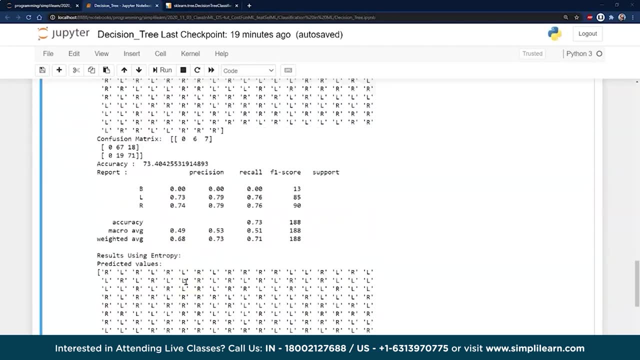 the different category routines we ran is that they run very similar. You certainly change the perimeters in them as to whether you're using, what model you're using and how you're using it and what data they get applied to, But when you're talking about the scikit, learn. 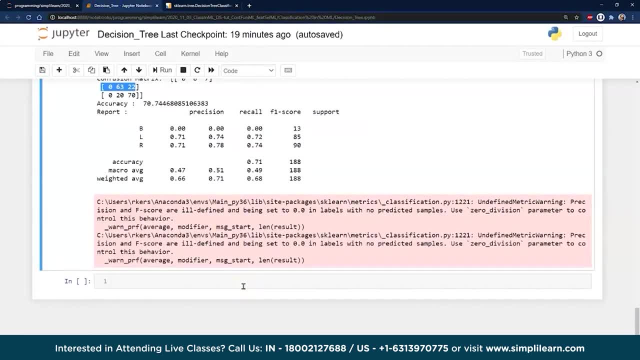 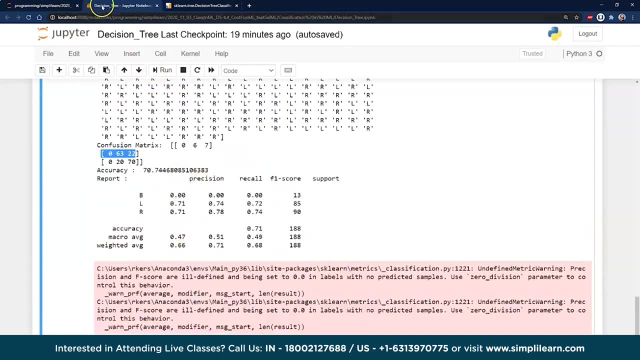 package. it does such an awesome job of making it easy. You split your data up, you train your data and you run the prediction and then you see what kind of accuracy, what kind of confusion matrix it generates. So we talk about algorithm selection. 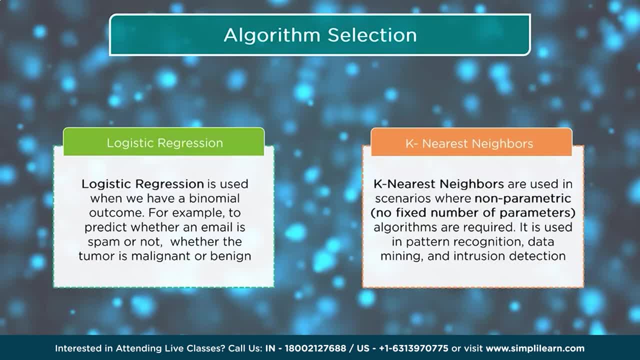 Logistic regression k- nearest neighbors. Logistic regression is used when we have a binomial outcome, For example, to predict whether an email is spam or not, Whether the tumor is malignant or not. The logistic regression works really good on that. You can do it in a k. 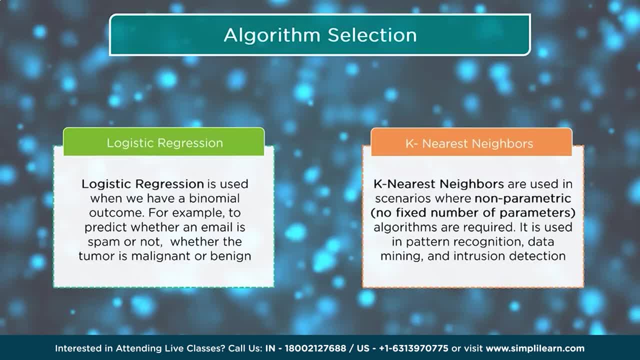 nearest neighbors. also, The question is, which one will it work better in? I find the logistic regression models work really good in a lot of raw numbers. So if you're working with, say, the stock market, Is this a good investment or a bad investment? 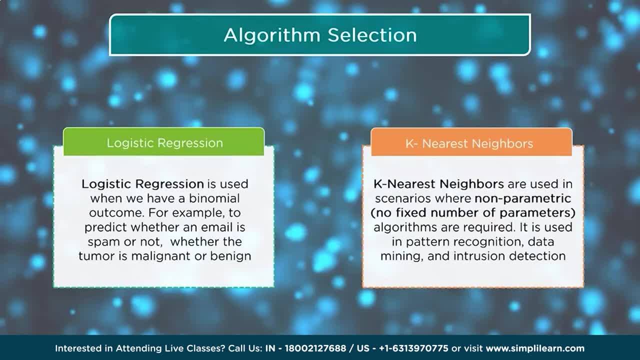 So that's one of the things. it handles the numbers better. K. nearest neighbors are used in scenarios where non-parametric- no fixed number of perimeters algorithms are required. It is used in pattern recognition, data mining and intrusion detection. So k means really good. 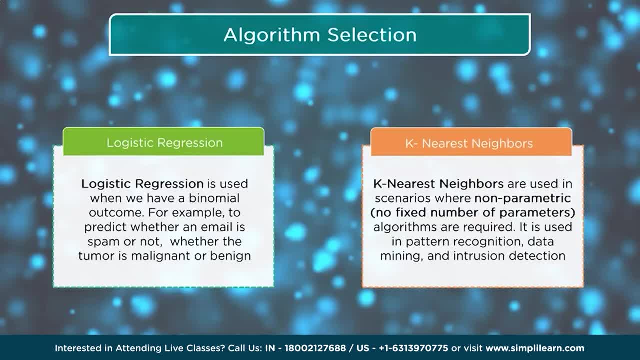 in finding the patterns. I've seen that as a preprocessor to a lot of other processors where you use the k nearest neighbors to figure out what data groups together. Very powerful package Support vector machines. Support vector machines are used whenever the data has. 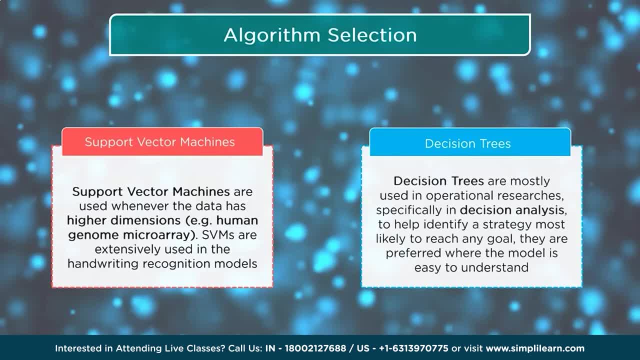 higher dimensions. The human genome microarray SVMs are extensively used in the hard handwriting recognition models And you can see that we were able to switch between the parabolic and the circular setup on there, where you can now have that donut kind of. 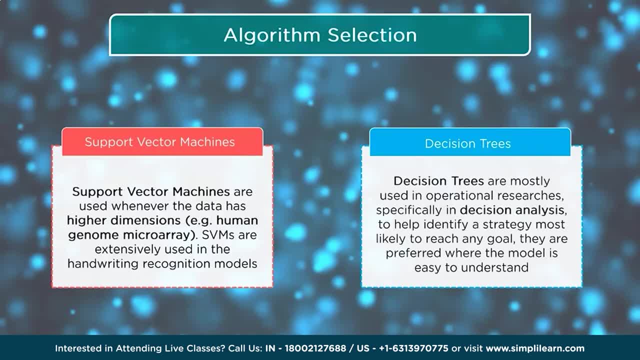 data and be able to filter that out with the support vector machine. And then decision trees are mostly used in operational researches, Specifically decision analysis, to help identify a strategy most likely to reach any goal. They are preferred where the model is easy to understand. I like 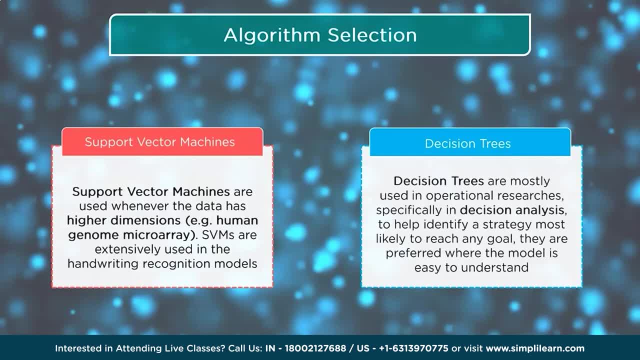 that last one. It's a good description, Is it easy to understand? So you have data coming in. When am I going to go to bed? You know, was it raining outside? You can go back and actually look at the pieces and see those different decision modes. 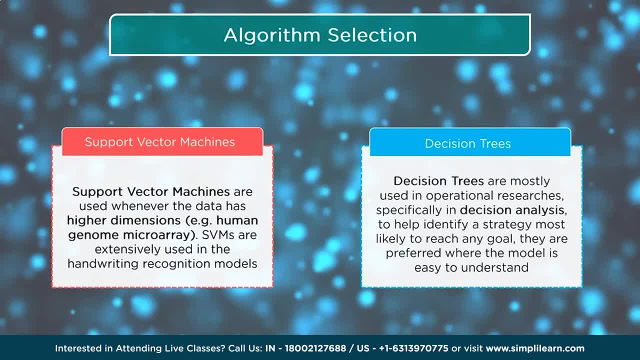 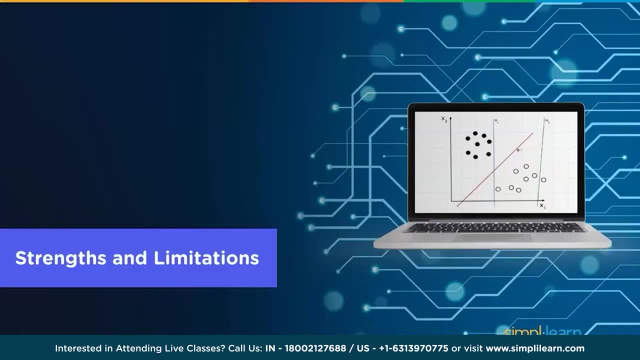 It takes a little bit more to dig in there and figure out what they're doing, but you can do that and you can actually help. you figure out why People love it for the why factor So strengths and limitations? Big one on all of these. 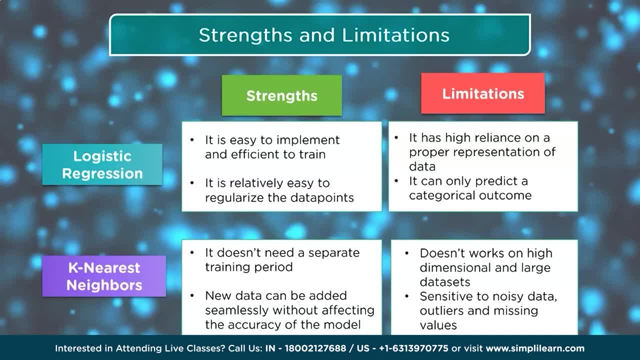 The strengths and limitations We talk about logistic regressions. The strengths are: it is easy to implement and efficient to train. It is relatively easy to regularize the data points. Remember how we put everything between 0 and 1? When you look at logistic regression models, 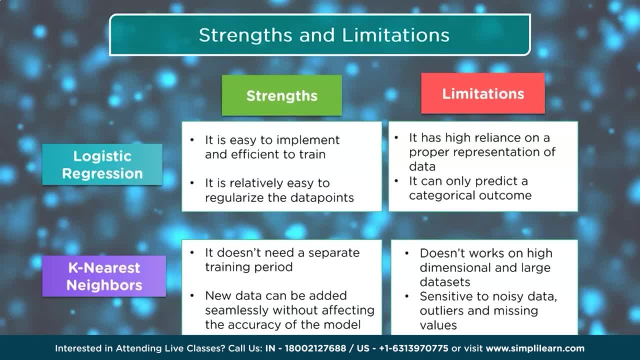 you don't have to worry about that. as much Limitations as a high reliance on proper representation of data. It can only predict a categorical outcome With the k nearest neighbors. it doesn't need a separate train period. New data can be added seamlessly without affecting the. 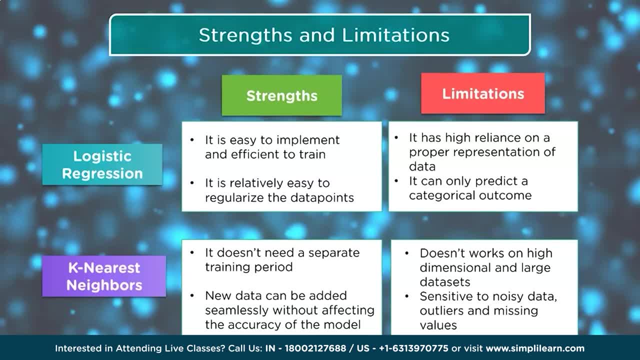 accuracy of the model. Kind of an interesting thing because you can do partial training. That can become huge if you're running across really large data sets or the data is coming in. You can continually do a partial fit on the data with the k nearest neighbors. 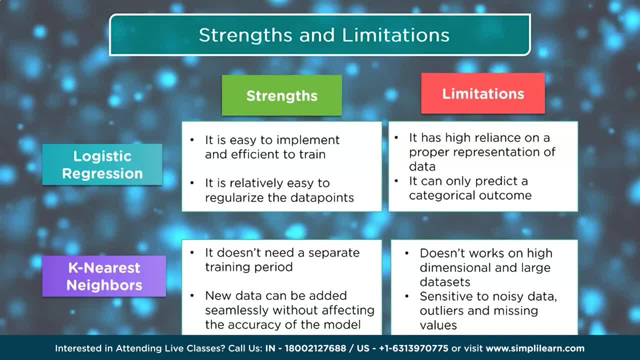 and continue to adjust that data. It doesn't work on high dimensional and large data sets. We were looking at the breast cancer, 36 different features. what happens when you have 127 features or a million features? What do you have a million features in? 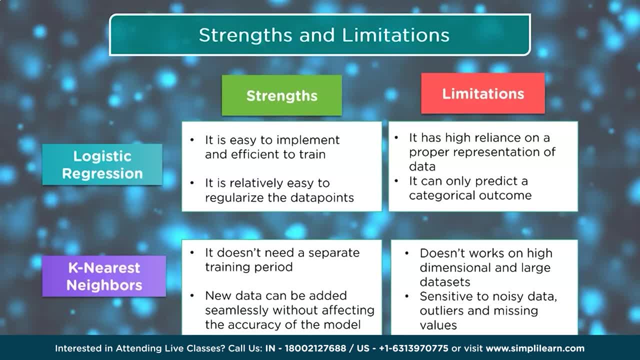 If I was analyzing the legal documents, I might have a tokenizer that splits the words up to be analyzed. That tokenizer might create one million different words available that might be in the document for doing weights Sensitive to noisy data outliers and missing values. 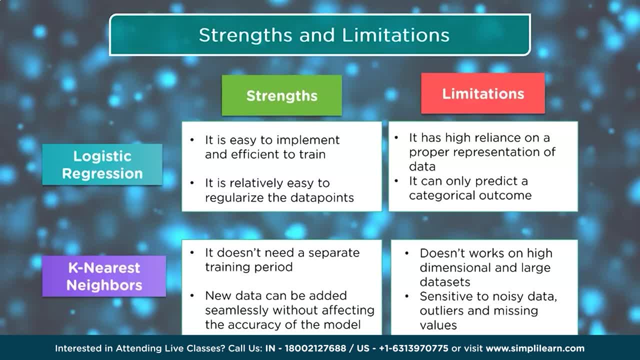 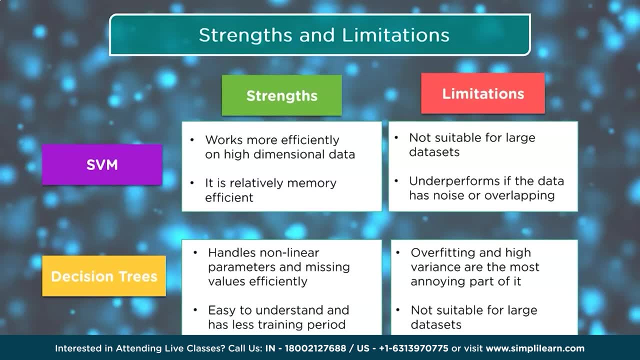 That's a huge one with k nearest neighbors. They really don't know what to do with the missing value. How do you compute the distance if you don't know what the value is? The SVM works more efficiently on high dimensional data. It is relatively 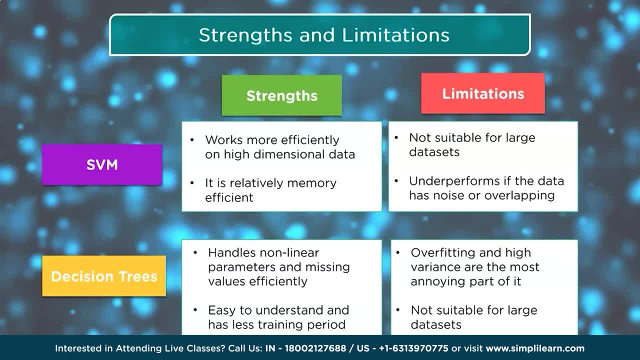 memory efficient. It's able to create those planes with only a few different variables in there, as opposed to having to store a lot of data for different features and things like that. It's not suitable for large data sets. The SVM- you start running this over gigabytes of data causes. 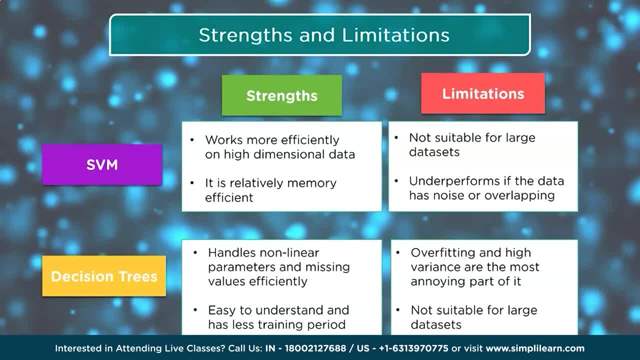 some huge issues. Underperforms if the data has noise or overlapping. That's a big one. We were looking at that where the SVM splits it and it creates a soft buffer. but what happens when you have a lot of stuff in the middle? that's hard. 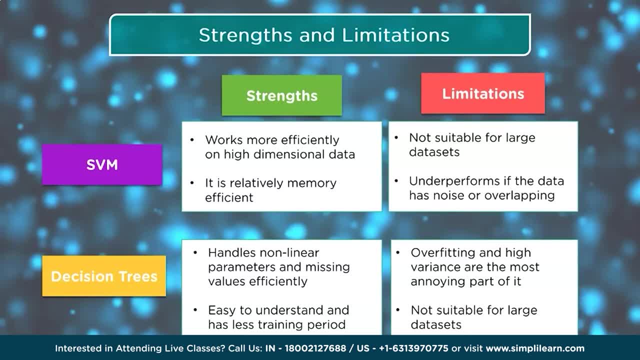 to sort out and doesn't know what to do with. That causes SVM to start crashing or not perform as well. Decision trees Handles non-linear perimeters and missing values efficiently. The missing values is huge. I've seen this in the wine tasting data sets, where they have three. 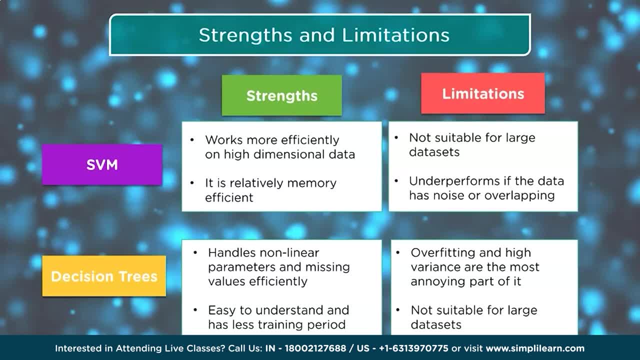 different data sets and they share certain features, but then each one has some features that aren't in the other ones and has to figure out how to handle those. Well, the decision tree does that automatically, instead of having to figure a way to fill that data in before processing. 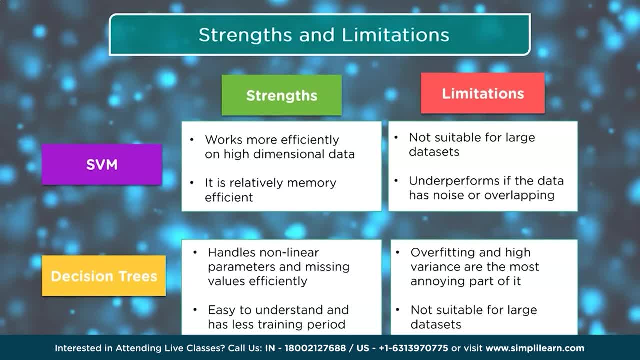 like you would with the other models. It's easy to understand and has less training period, So it trains pretty quickly. It comes up there and just keeps forking the tree down and moving the parts around, and so it doesn't have to go through. 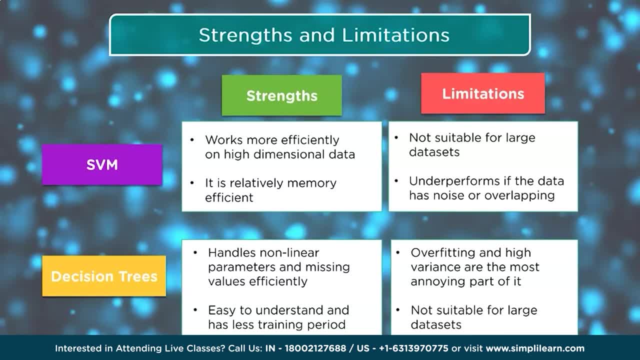 the data multiple times. guessing and adjusting It just creates the tree as it goes. Overfitting and high variance are the most annoying part of it. That's an understatement. That has to do with how many leaves and how many decisions you have to do. 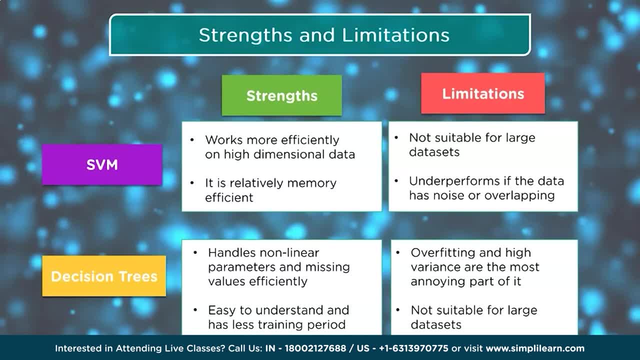 The more you have, the more overfit it is to the data. It also just in making the choices and how the choices come in, it might overfit to a specific feature because that's where it started at and that's what it knows. 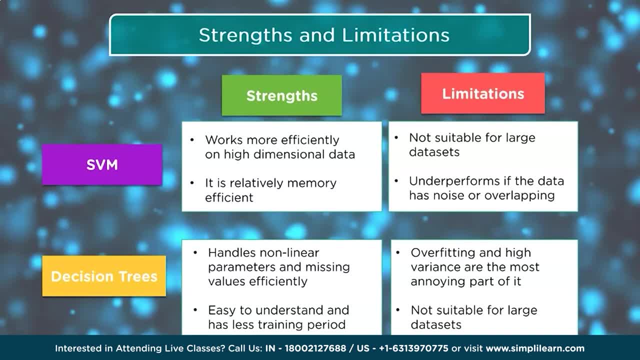 It really is challenged with large data sets. They've been working on that with the data forest, but it's not suitable for large data sets. It's really something you'd probably run on a single machine and not across a data pool or anything. Decision Tree, one of the many 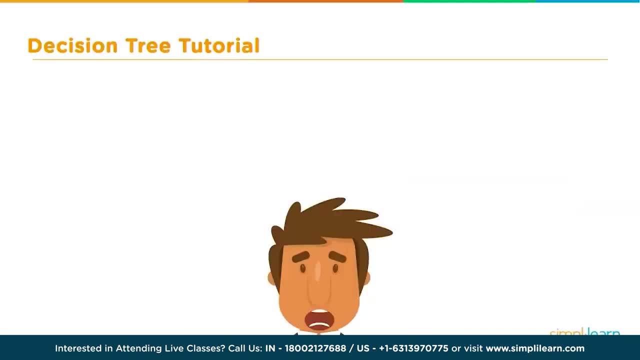 powerful tools in the machine learning library begins with a problem. I think I have to buy a car. So in making this question, you want to go. how do I decide which one to buy? And you're going to start asking questions. Is the mileage greater than 20?? 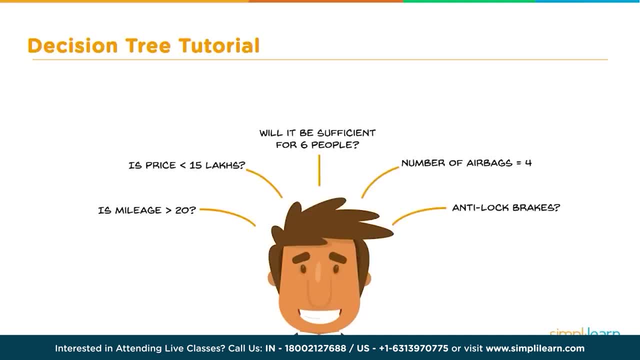 Is the price less than 15?? Will it be sufficient for six people? Does it have enough airbags, Anti-lock brakes? All these questions come up Then as we feed all this data in, we make a decision, And that decision comes up. 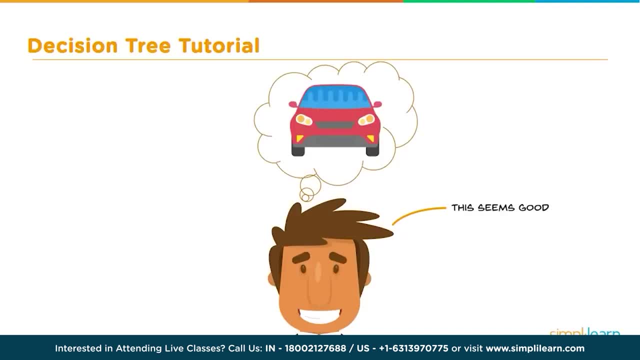 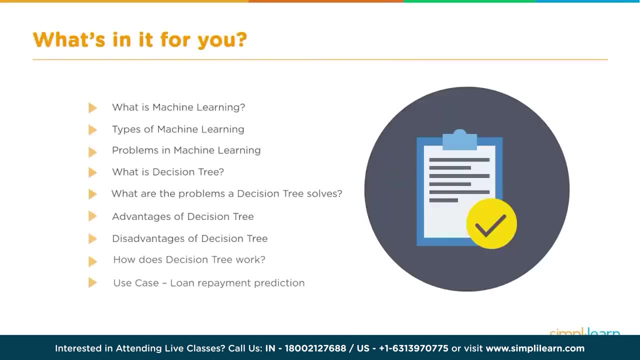 oh hey, this seems like a good idea. Here's a car. So, as we're going through this decision process using a decision tree, we're going to explore this, maybe not in buying a car, but in how to process data. What's in it for you? 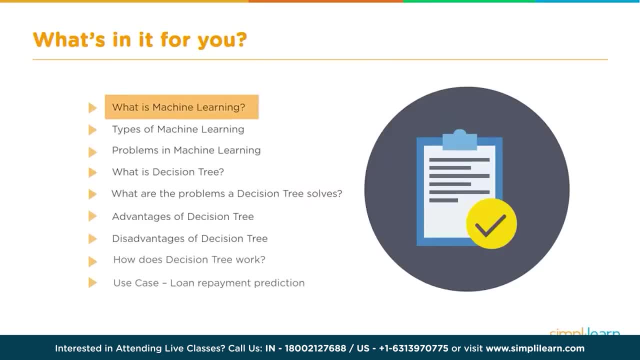 Let's start by finding out what is machine learning and why we even want to know about it for processing our data, And we'll go into the three basic types of machine learning and the problems that are used by machine learning to solve. Finally, we'll get into what is. 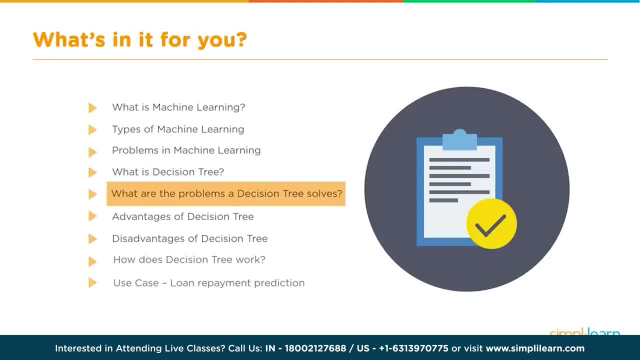 a decision tree? What are the problems a decision tree solves? What are the advantages and disadvantages of using a decision tree? And then we want to dig in a little deep into the mechanics: How does the decision tree work? And then we'll go in. 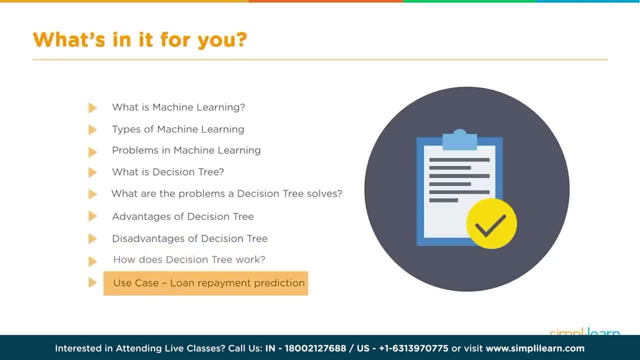 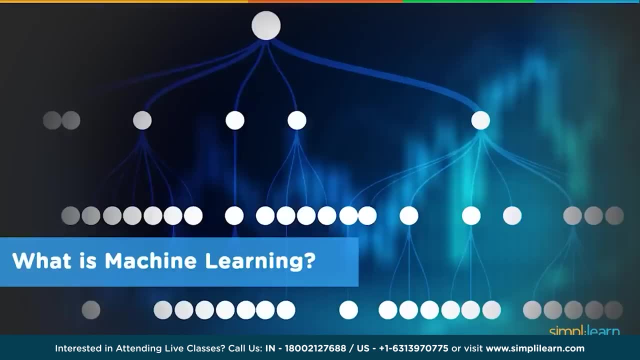 and do a case- loan repayment prediction- where we actually are going to put together some Python code and show you the basic Python code for generating a decision tree. What is machine learning? There are so many different ways to describe what is machine learning in today's world and illustrate it. 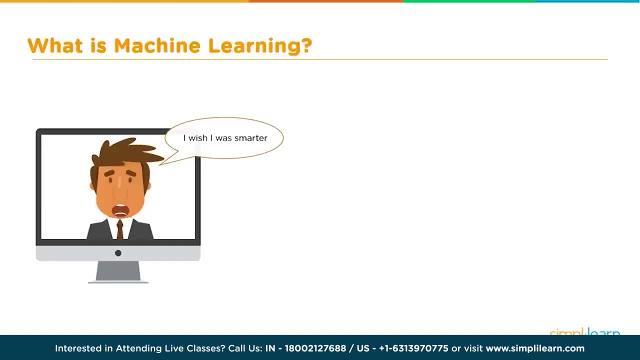 We're going to take a graphic here and making decisions or trying to understand what's going on. and really underlying machine learning is people wish they were smarter, wish we could understand the world better. So you can see a guy here who's saying, hey, how can I understand? 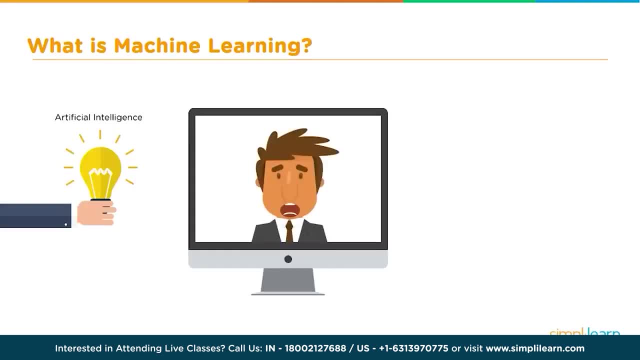 the world better. And someone comes up and says: let's use artificial intelligence. Machine learning is a part of artificial intelligence- And now he gets a big smile on his face because now he has artificial intelligence to help him make his decisions And they can think in new ways. So this: 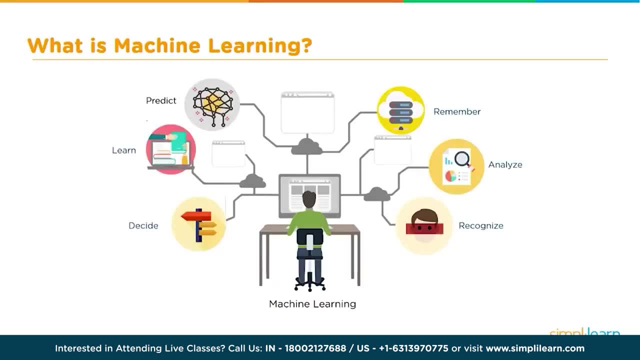 brings in new ideas. So what is machine learning? This is a wonderful graph. here You can see where we have learn, predict, decide. These are the most basic three premises of machine learning. In learning, we can describe the data in new ways and be able. 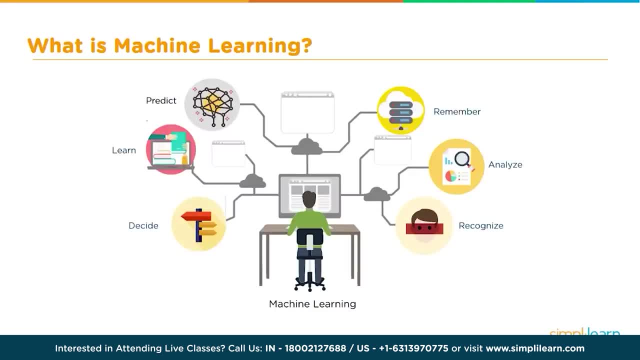 to learn new aspects about what we're looking at, And then we can use that to predict things and we can use that to make decisions. So maybe it's something that's never happened before, but we can make a good guess whether it's going to be a good investment or not. 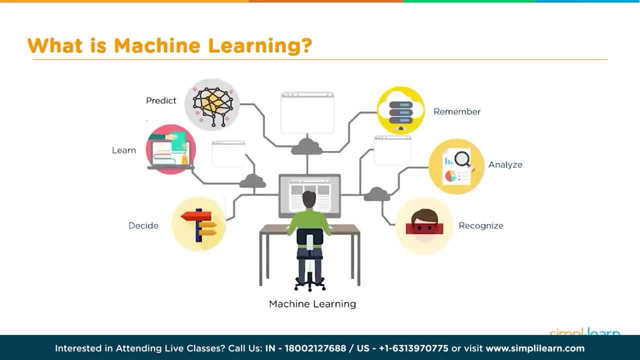 It also helps us categorize stuff so we can remember it better, So it's easier to pull it out of the catalog. We can analyze data in new ways we never thought possible. And then, of course, there's the very large, growing industry. 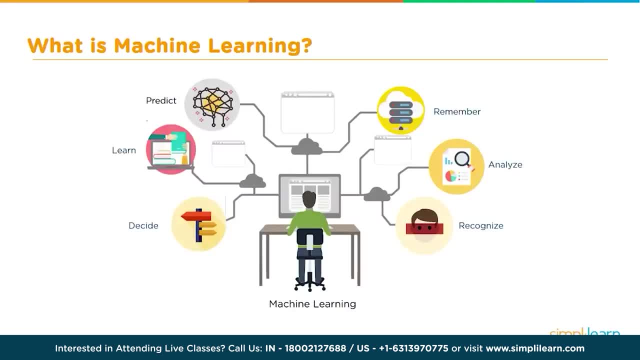 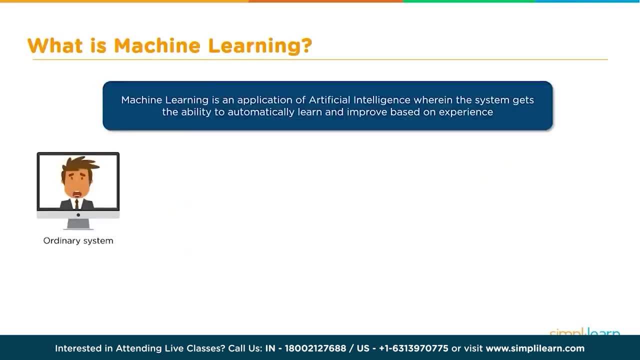 of recognize. We can do facial recognition, driver recognition, automated car recognition. All these are part of machine learning. Going back to our guy here who's in his ordinary system and would like to be smarter, make better choices: What happens with machine learning is an application. 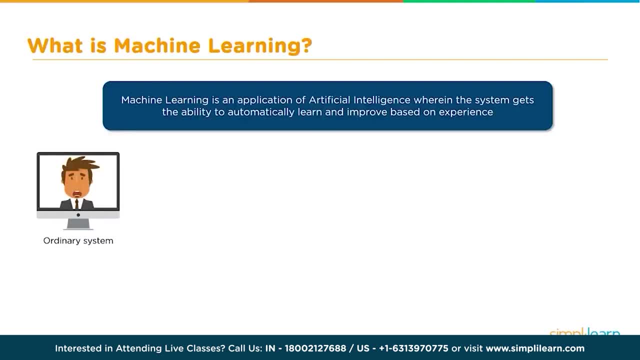 of artificial intelligence, wherein the system gets the ability to automatically learn and improve based on experience. So this is exciting because you have your ordinary guy who now has another form of information coming in, And this is with the artificial intelligence: helps him see things he never saw or track things he. 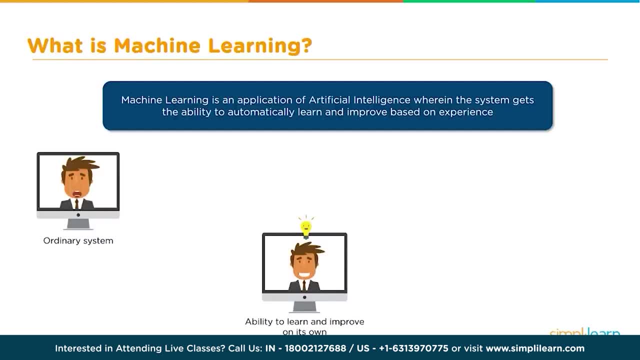 can't track. So instead of having to read all the news feeds, he can now have an artificial intelligence sorted out, so he's only looking at the information he needs to make a choice with. And of course, we use all those machine learning tools back. 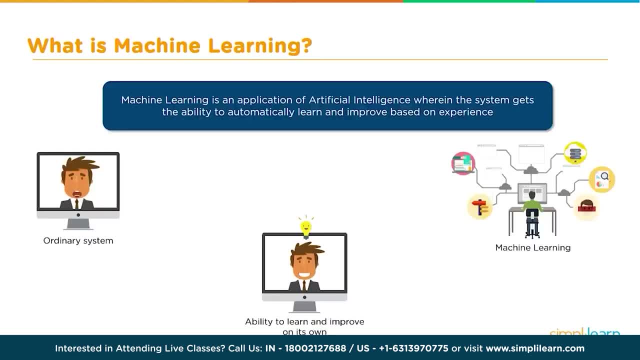 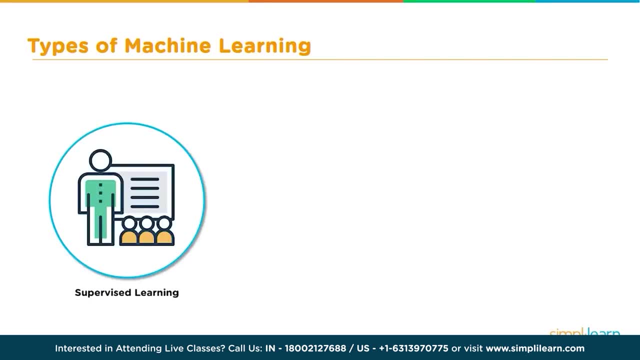 in there and he's now making smarter choices with less work. Types of machine learning. Let's break it into three primary types of learning. First is supervised learning, where you already have the data and the answers. So if you worked out a bank, you'd already have a list. 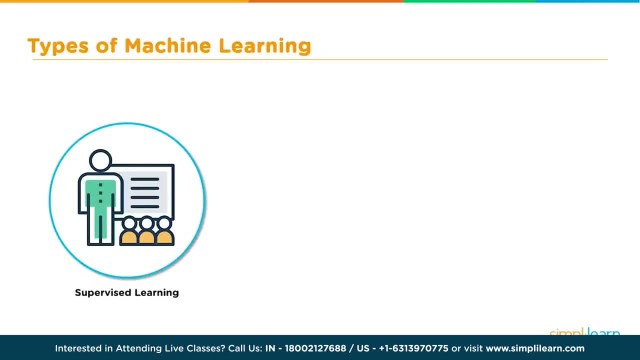 of all the previous loans and who defaulted on them and who made good payments on them. You then program your machine learning tool and that lets you predict on the next person whether they're going to be able to make their payments or not on their loan, If you have one. 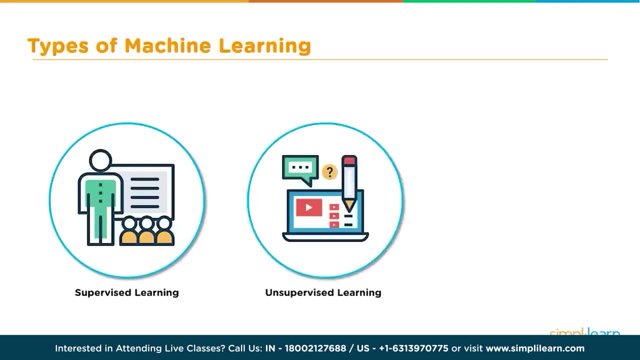 category where you already know the answers. the next one would be: you don't know the answers, You just have a lot of information coming in. Unsupervised learning allows you to group liked information together, So if you're analyzing photos, it might group all the images. 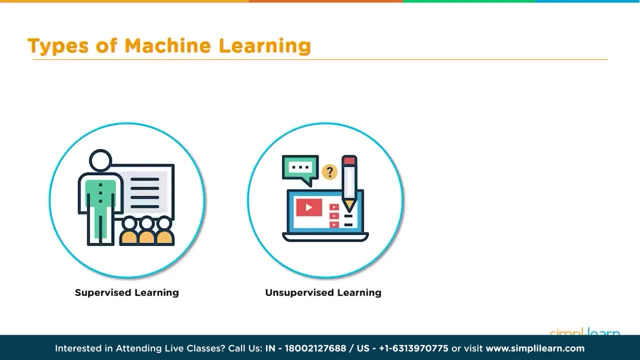 of trees together and all the images of houses together, without ever knowing what a house or a tree is, Which leads us to the third type of machine learning. The third type of machine learning is reinforcement learning, Unlike supervised or unsupervised learning you don't have. 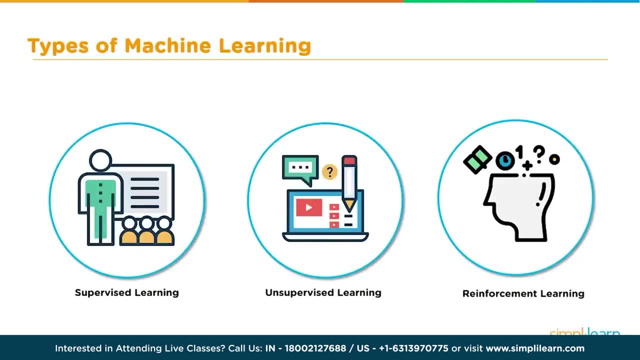 the data prior to starting. So you get the data one line at a time and then, whether you make a good choice or a bad choice, the machine learning tool has to then adjust accordingly, so you get a plus or minus feedback. You can liken this to the way a human 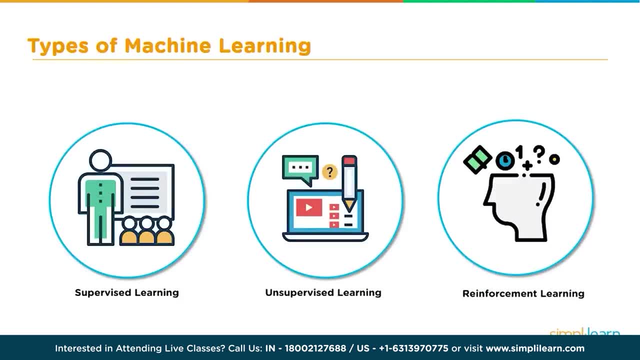 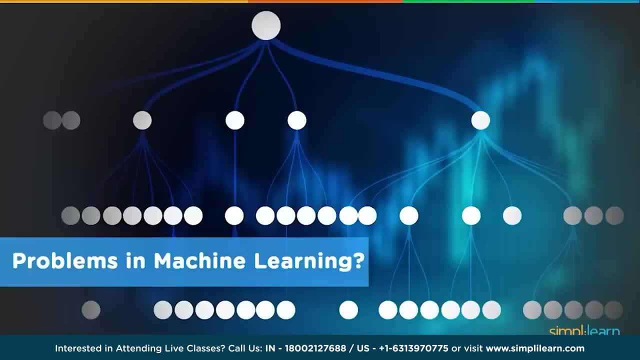 learns. We experience life one minute at a time and we learn from that, And either our memory is good or we learn to avoid something. Problems in machine learning. To understand where the decision tree fits into our machine learning tools, we have to understand the basics of some of the machine. 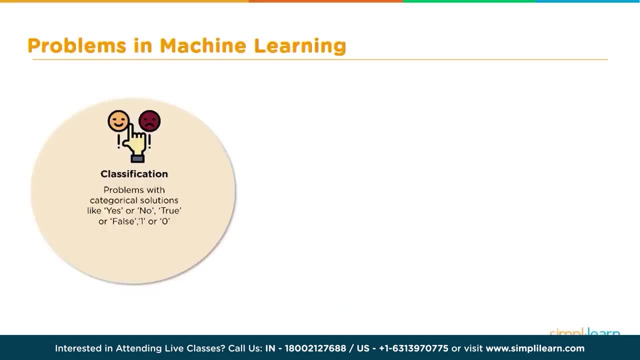 learning problems, And three of the primary ones fall underneath classification Problems with categorical solutions like yes or no, true or false, one or zero. This might be: does it belong to a particular group, yes or no? Then we have regression problems. 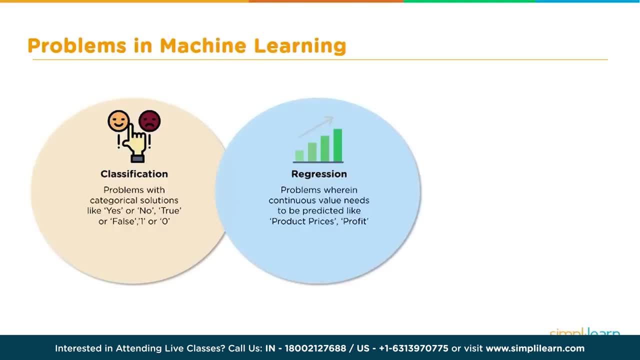 where there's a continuous value needs to be predicted, like product prices, profit, And you can see here- this is a very simple linear graph. You can guess what the next value is based on the first four. It kind of follows a straight line, going up And clustering. This is: 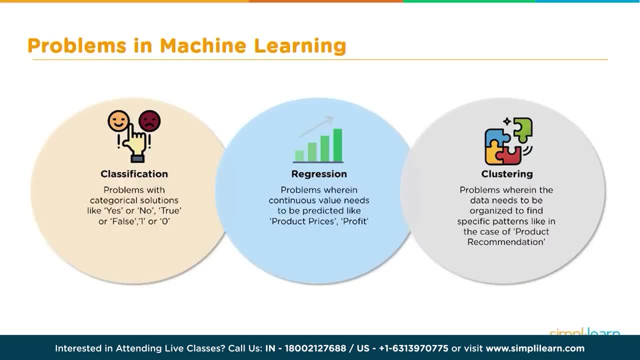 problems where the data needs to be organized to find specific patterns, like in the case of product recommendation. They group all the different products that people just like you viewed on a shopping site and say people who bought this also bought this. The most commonly used for the decision tree is for: 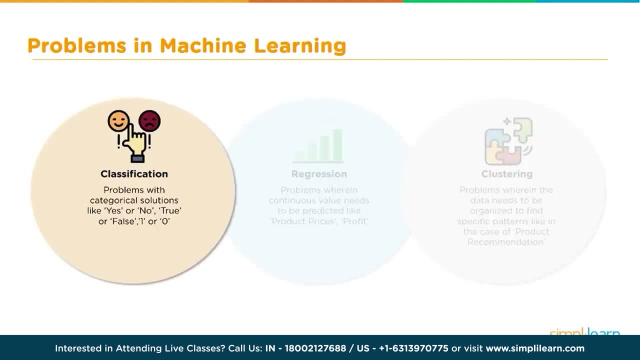 classification For figuring out: is it red or is it not, Is it a fruit or is it a vegetable, Yes or no, True or false, Left or right, Zero or one. And so we talk about classification. we're going to look. 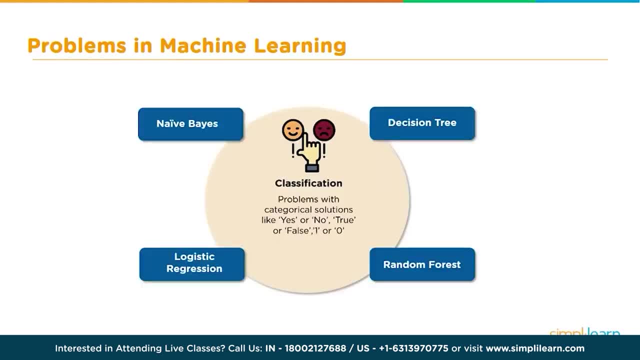 at the basic machine learning. These are the four main tools used in classification. There's the knave, Bayes, logistic regression, decision tree and random forest. The first two are for simpler data. So if your data is not very complex, you can usually 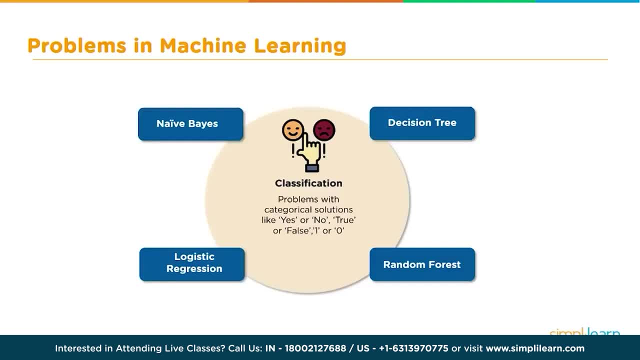 use these to do a fairly good representation by drawing a line through the data or a curve through the data. They work wonderful in a lot of problems. But as things get more complicated the decision tree comes in And then, if you have a very large amount of 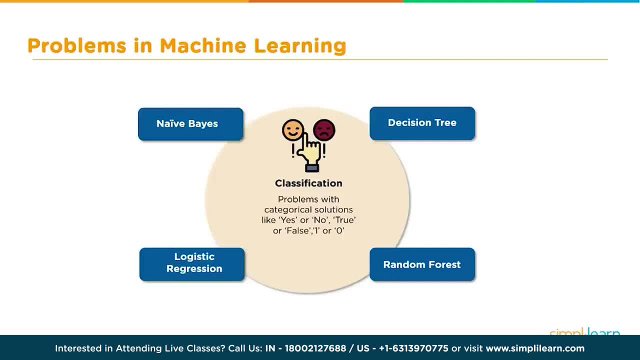 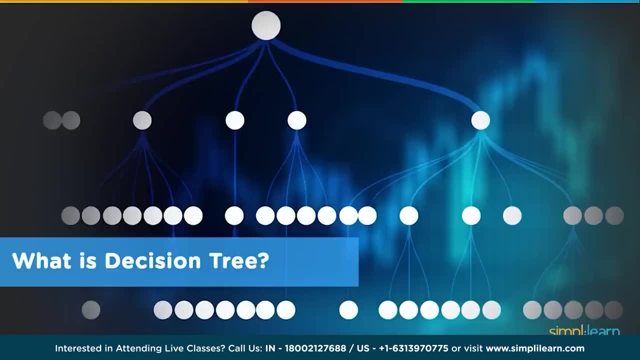 data you start getting into the random forest. So the decision tree is actually a part of the random forest. But today we're just going to focus on the decision tree. What is a decision tree? Let's go through a very simple example before we dig in deep. Decision tree: 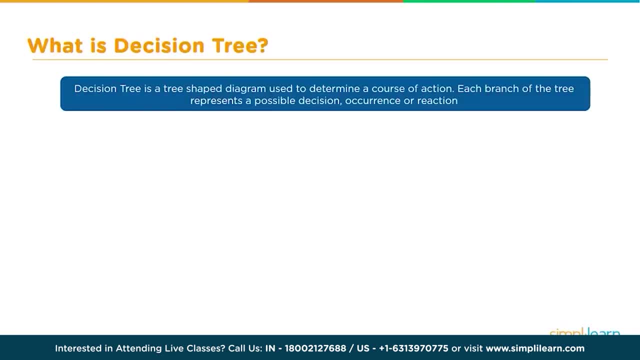 is a tree-shaped diagram used to determine a course of action. Each branch of the tree represents a possible decision, occurrence or reaction. Let's start with a simple question: How to identify a random vegetable from a shopping bag. So we have this group of vegetables in here. 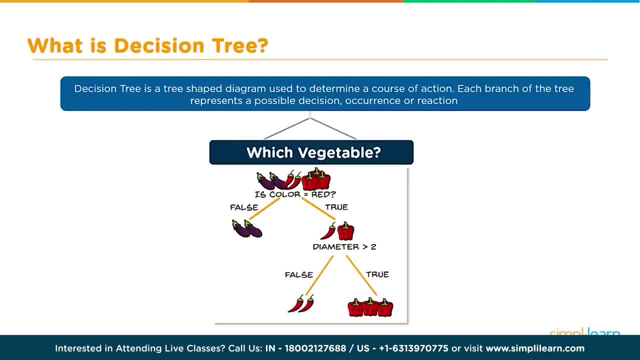 And we can start off by asking a simple question: Is it red? And if it's not, then it's going to be the purple fruit to the left, probably an eggplant. If it's true, it's going to be one of the red fruits. 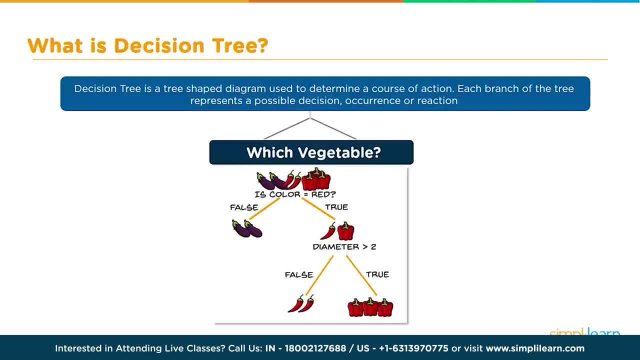 Is the diameter greater than two? If false, it's going to be what looks to be a red chili, And if it's true, it's going to be a bell pepper From the capsicum family. So it's a capsicum. 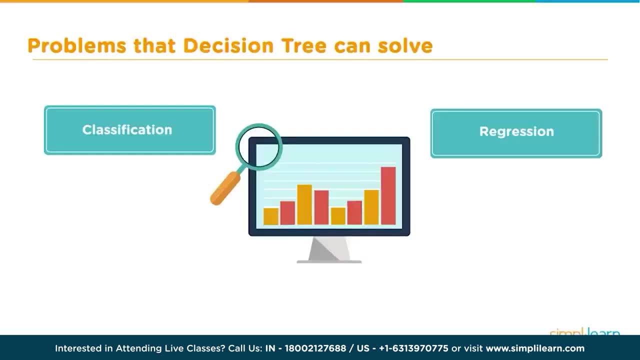 Problems that decision tree can solve. So let's look at the two different categories the decision tree can be used on. It can be used on the classification- the true, false, yes, no. And it can be used on regression, where we figure out what the next. 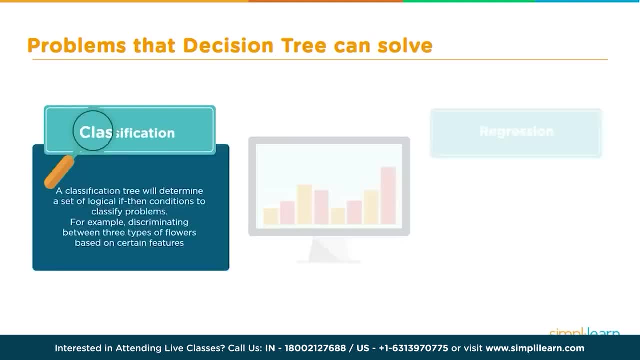 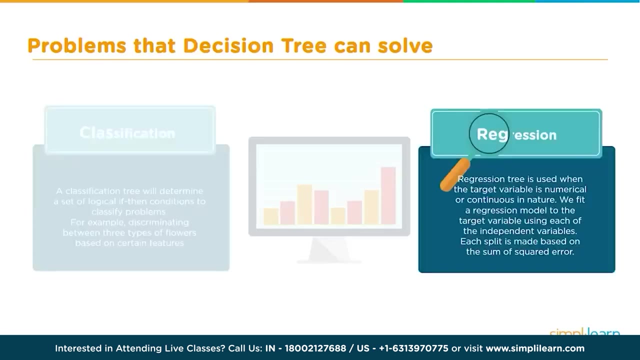 value is in a series of numbers or a group of data. In classification, the classification tree will determine a set of logical if-then conditions to classify problems, For example, discriminating between three types of flowers based on certain features. In regression, a regression tree. 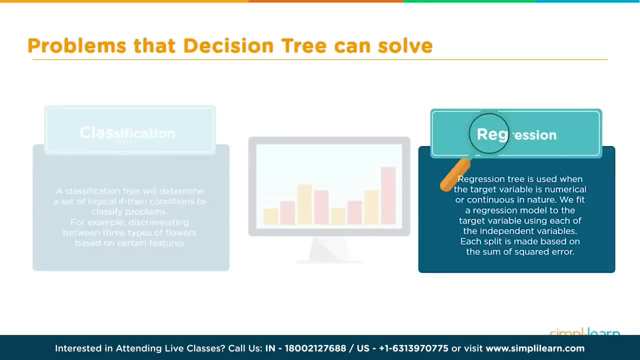 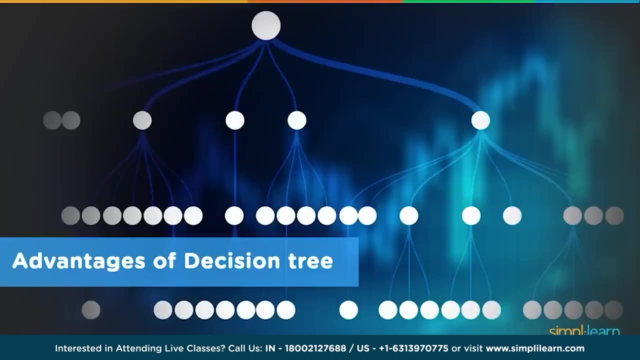 is used when the target variable is numerical or continuous in nature. We fit the regression model to the target variable using each of the independent variables. Each split is made based on the sum of squared error. Before we dig deeper into the mechanics of the decision tree, let's take a look at 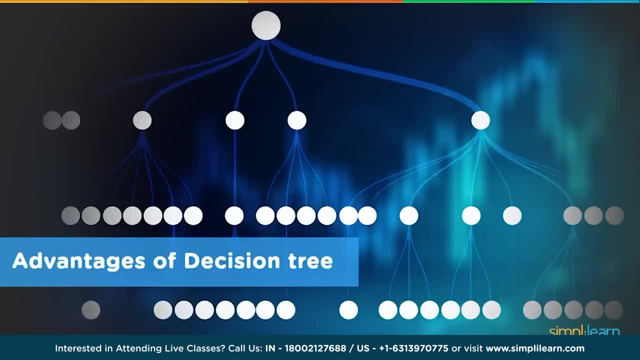 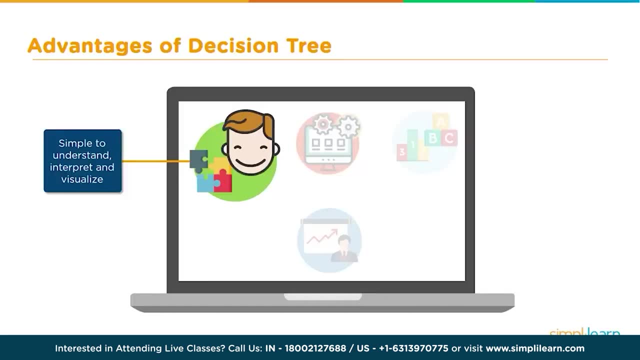 the advantages of using a decision tree And we'll also take a glimpse at the disadvantages. The first thing you'll notice is that it's simple to understand, interpret and visualize. It really shines here, because you can see exactly what's going on in a decision tree. 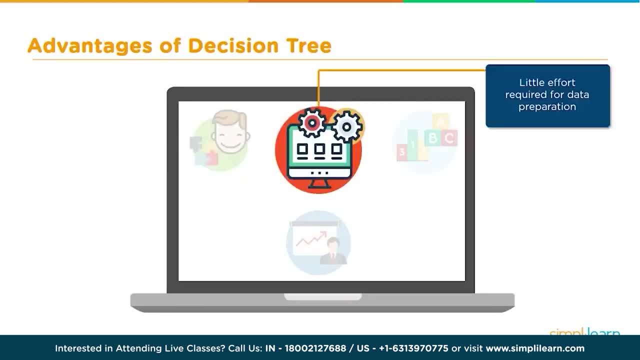 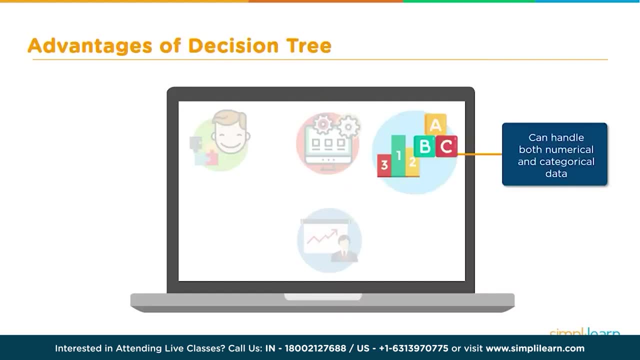 Little effort is required for data preparation, so you don't have to do special scaling. There's a lot of things you don't have to worry about when using a decision tree. It can handle both numerical and categorical data, as we discovered earlier, And non-linear parameters. 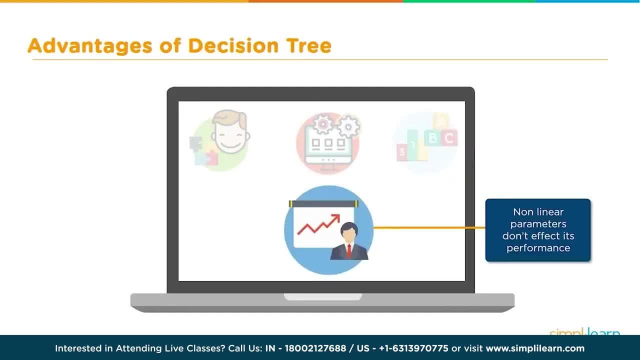 don't affect its performance. So even if the data doesn't fit an easy curved graph, you can still use it to create an effective decision or prediction. If we're going to look at the advantages of a decision tree, we also need to understand the 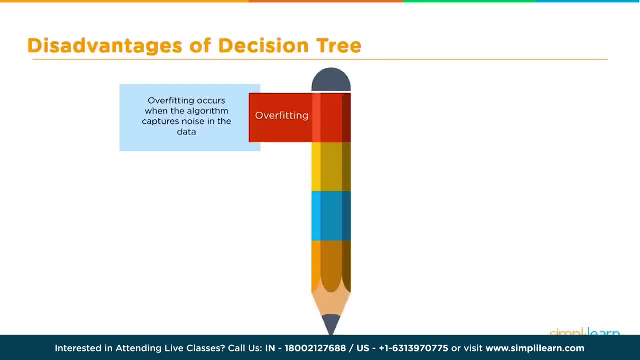 disadvantages of a decision tree. The first disadvantage is overfitting. Overfitting occurs when the algorithm captures noise in the data. That means you're solving for one specific instance instead of a general solution for all the data- High variance- The model can get unstable. 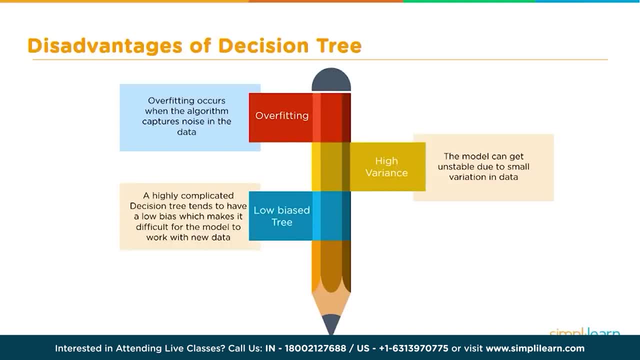 due to small variation in data. Low bias tree: A highly complicated decision tree tends to have a low bias, which makes it difficult for the model to work with new data Decision tree important terms. Before we dive in further, we need to look at some. 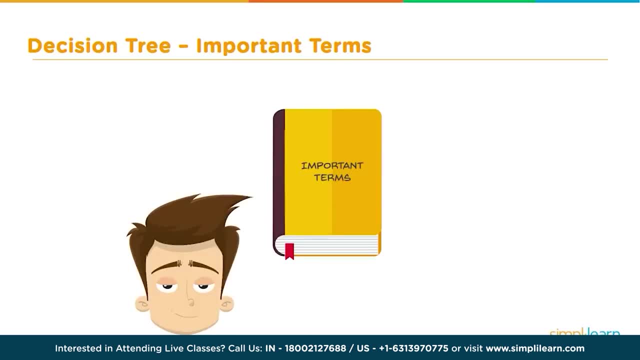 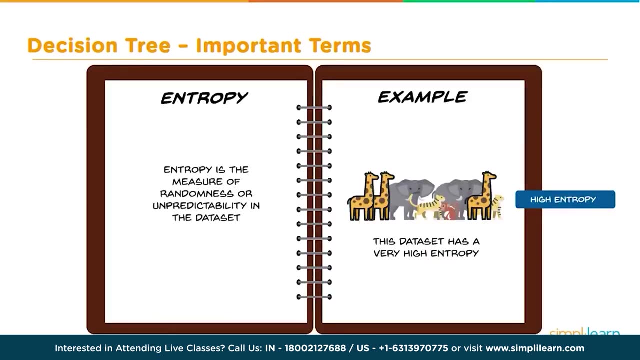 basic terms. We need to have some definitions to go with our decision tree and the different parts we're going to be using. We'll start with entropy. Entropy is a measure of randomness or unpredictability in the data set. For example, we have a. 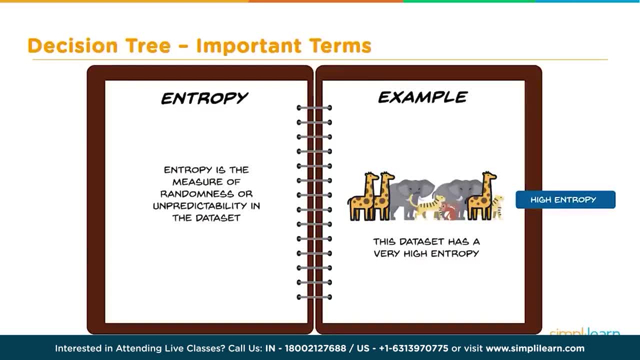 group of animals. In this picture there's four different kinds of animals And this data set is considered to have a high entropy. You really can't pick out what kind of animals it is based on looking at just the four animals, as a big clump of. 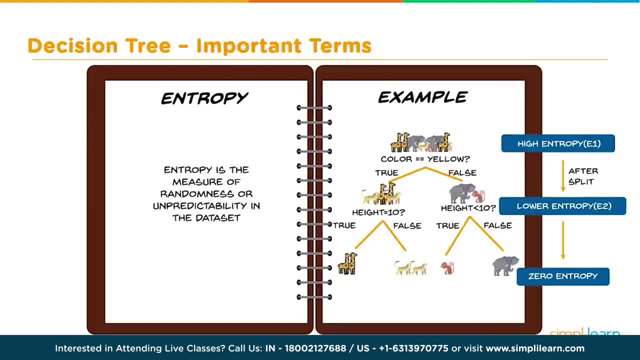 entities. So as we start splitting it into subgroups, we come up with our second definition, which is information gain. Information gain, It is a measure of decrease in entropy after the data set is split. So in this case, based on the color yellow, we've split. 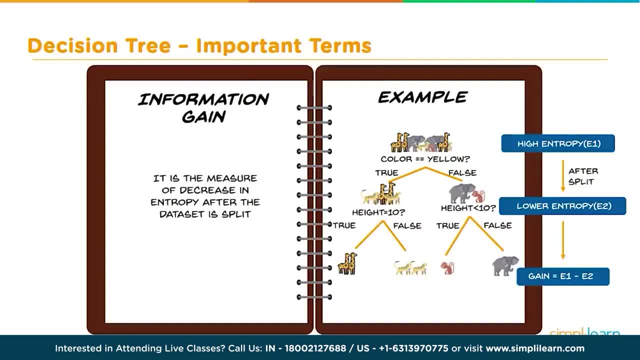 one group of animals on one side as true and those who aren't yellow as false. As we continue down the yellow side, we split based on the height. true or false equals 10.. And on the other side, height is less than 10,. true or? 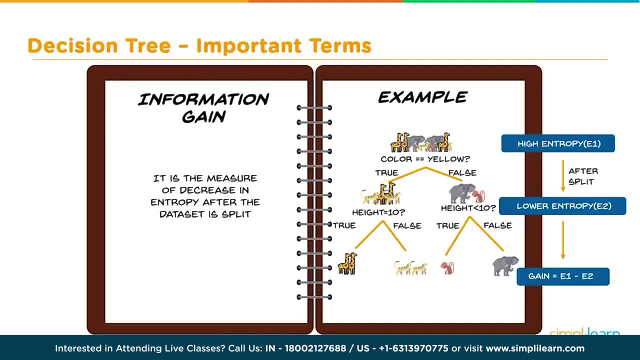 false And, as you see, as we split it, the entropy continues to be less and less and less, And so our information gain is simply the entropy E1 from the top and how it's changed to E2 in the bottom, And we'll look. 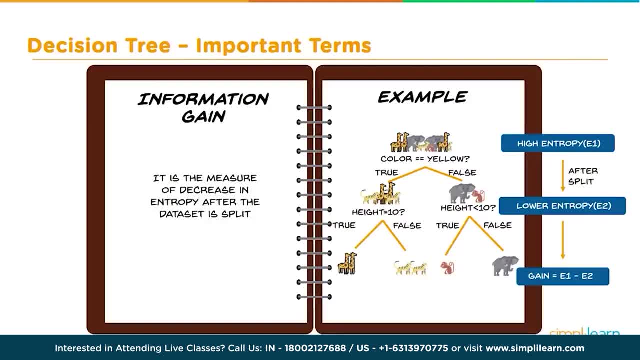 at the deeper math, although you really don't need to know a huge amount of math when you actually do the programming in Python, because they'll do it for you. But we'll look on the actual math at how they compute entropy. Finally, we want to know the different parts. 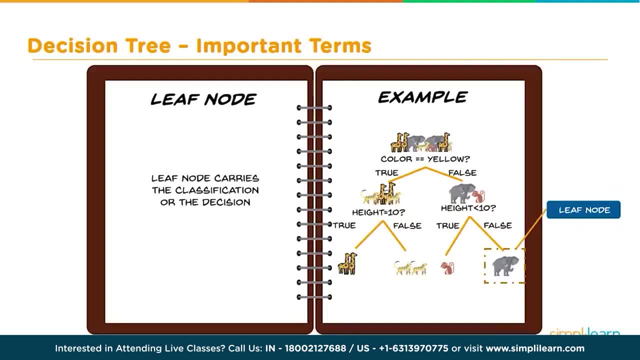 of our tree and they call the leaf node. Leaf node carries the classification or the decision, so it's the final end. at the bottom, The decision node has two or more branches. This is where we're breaking the group up into different parts. And finally you have 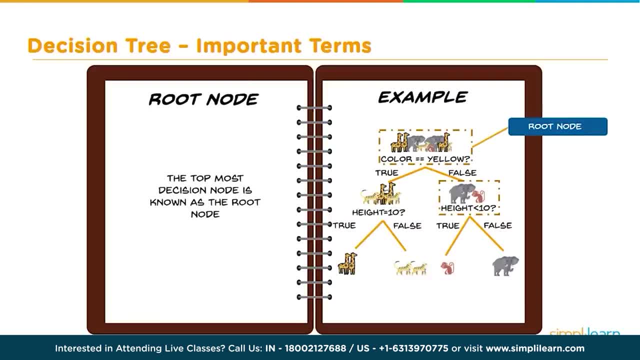 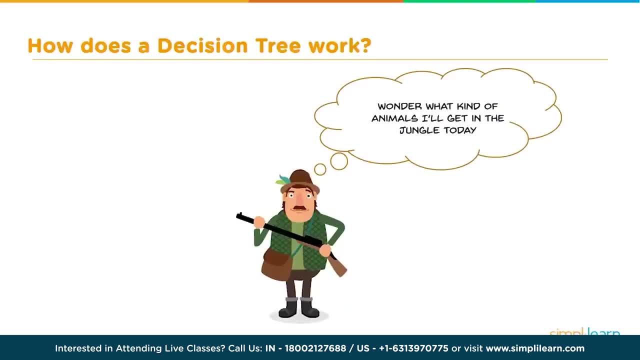 the root node. The top most decision node is known as the root node. How does a decision tree work? Wonder what kind of animals I'll get in the jungle today. Maybe you're the hunter with the gun or if you're more into photography, you're a photographer. 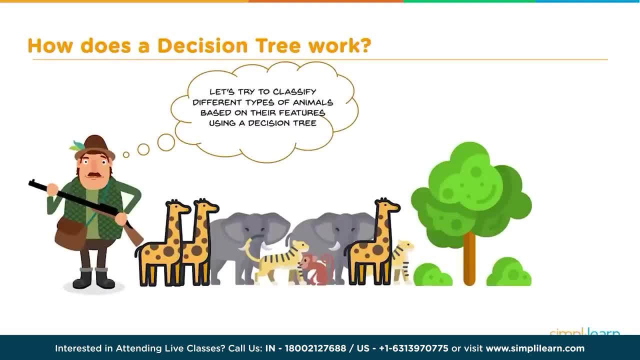 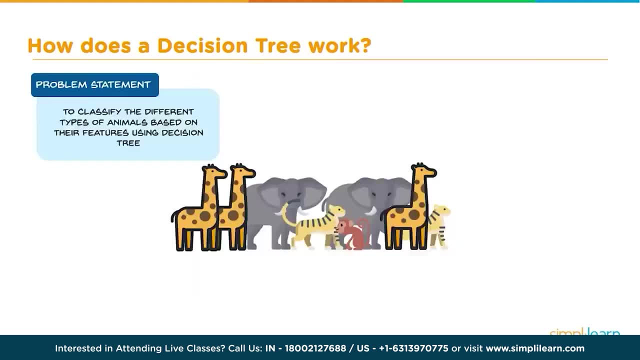 with a camera. So let's look at this group of animals and let's try to classify different types of animals based on their features using a decision tree. So the problem statement is to classify the different types of animals based on their features using a decision tree. 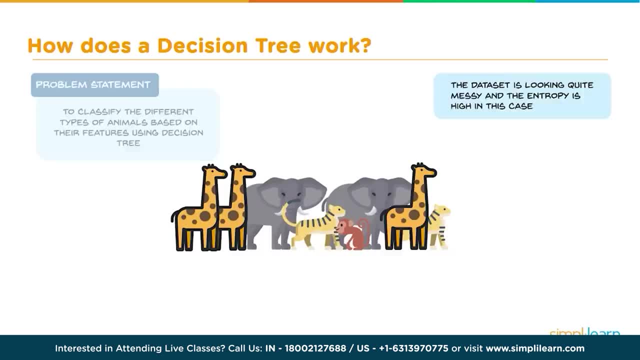 The data set is looking quite messy and the entropy is high in this case. So let's look at a training set or a training data set, And we're looking at color, we're looking at height, and then we have our different animals. 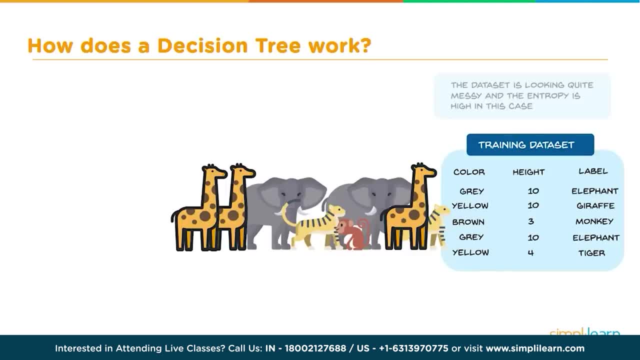 We have our elephants, our giraffes, our monkeys and our tigers, And they're of different colors and shapes. Let's see what that looks like and how do we split the data. We have to frame the conditions that split the data in such 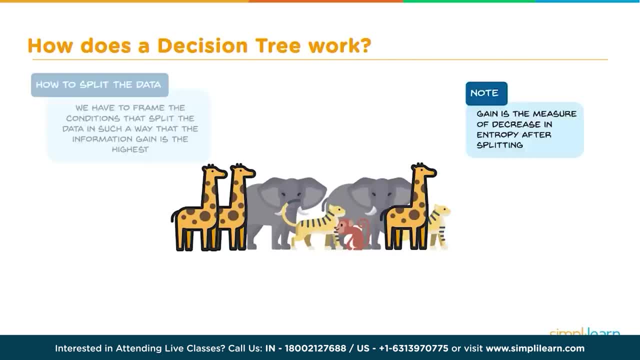 a way that the information gain is the highest. Note: gain is a measure of decrease in entropy after splitting, So the formula for entropy is the sum. that's what this symbol looks like. it looks like kind of like a funky E of K where I equals 1. 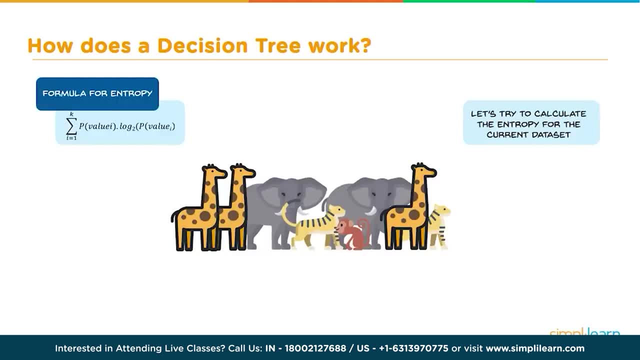 to K. K would represent the number of animals, the different animals in there, where value or P value of I would be the percentage of that animal. Time times the log base 2 of the same, the percentage of that animal. 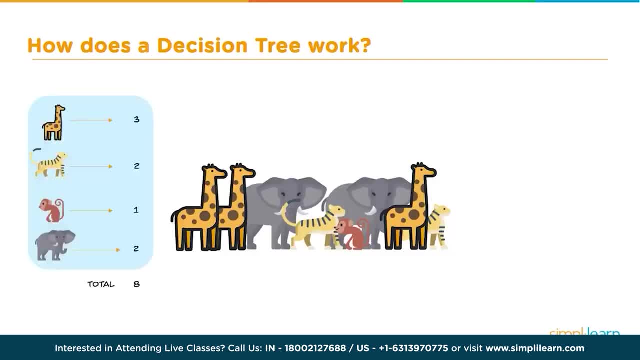 Let's try to calculate the entropy for the current data set and take a look at what that looks like. and don't be afraid of the math. You don't really have to memorize this math, just be aware that it's there and this is. 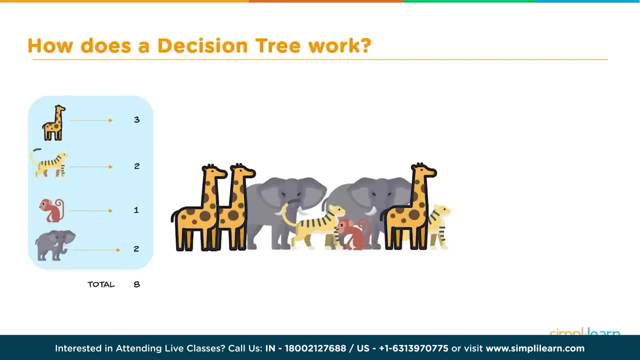 what's going on in the background. And so we have 3 giraffes, 2 tigers, 1 monkey, 2 elephants- a total of 8 animals gathered, And if we plug that into the formula, we get an entropy that equals 3. 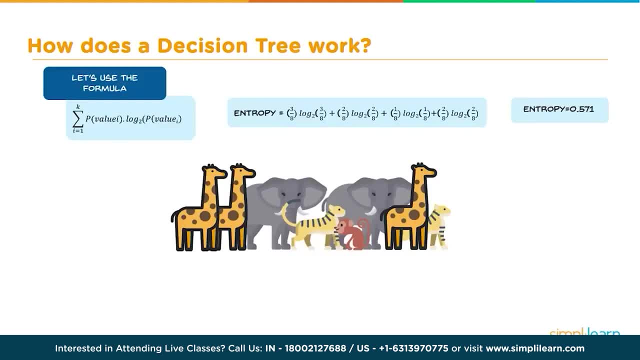 over 8, so we have 3 giraffes, a total of 8, times the log. and usually they use base 2 on the log, so log base 2 of 3 over 8, plus in this case. 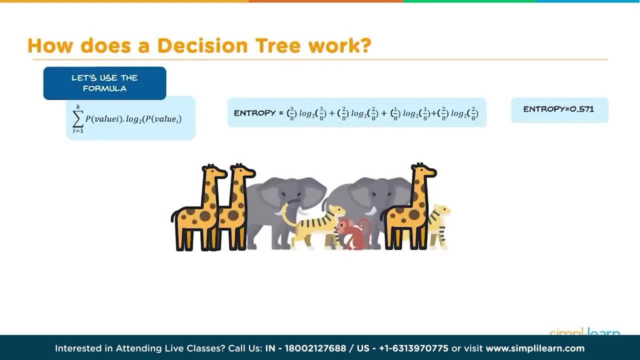 let's say it's the elephants: 2 over 8, 2 elephants over a total of 8, times log base: 2, 2 over 8, plus 1 monkey over a total of 8, log base: 2, 1 over 8,. 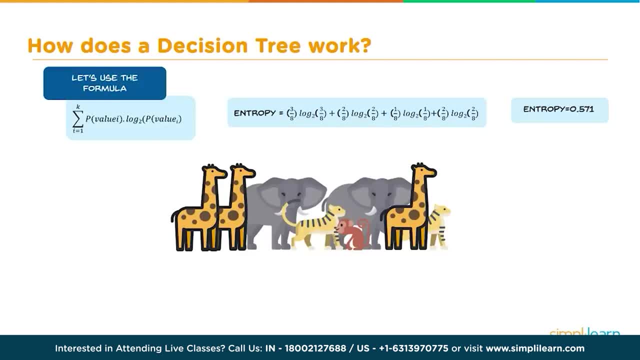 and plus 2 over 8 of the tigers log base, 2 over 8. And if we plug that into our computer, our calculator- I obviously can't do logs in my head- we get an entropy equal to 0.571.. 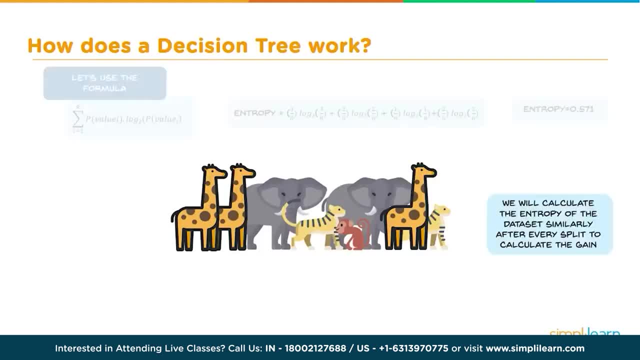 The program will actually calculate the entropy of the data set. similarly, after every split, to calculate the gain. Now we're not going to go through each set, one at a time, to see what those numbers are. We just want you to be aware that this is a 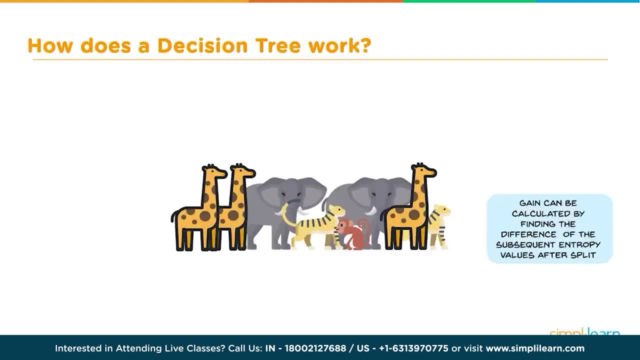 formula or the mathematics behind it. Gain can be calculated by finding the difference of the subsequent entropy values after a split. Now we will try to choose a condition that gives us the highest gain. We will do that by splitting the data using each condition and checking that the 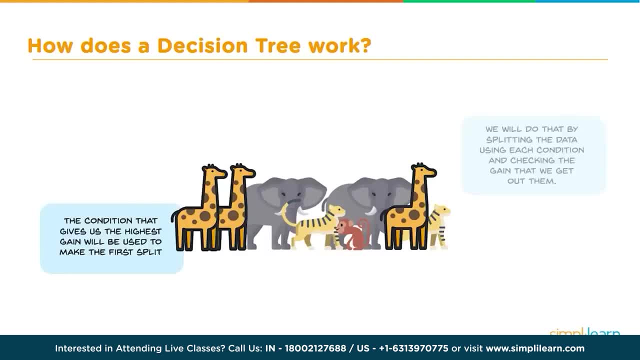 gain we get out of them. The condition that gives us the highest gain will be used to make the first split. Can you guess what that first split will be? just by looking at this image, As a human, it's probably pretty easy to split it. Let's see if. 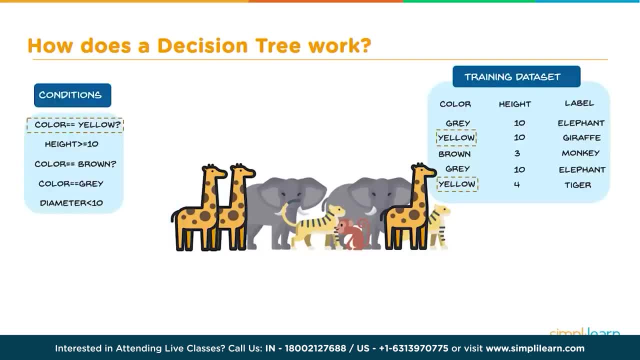 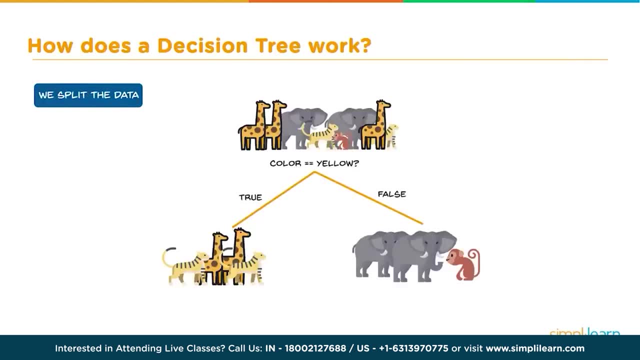 you're right. If you guessed the color yellow, you're correct. Let's say the condition that gives us the maximum gain is yellow. So we will split the data based on the color yellow. If it's true, that group of animals goes to the left. 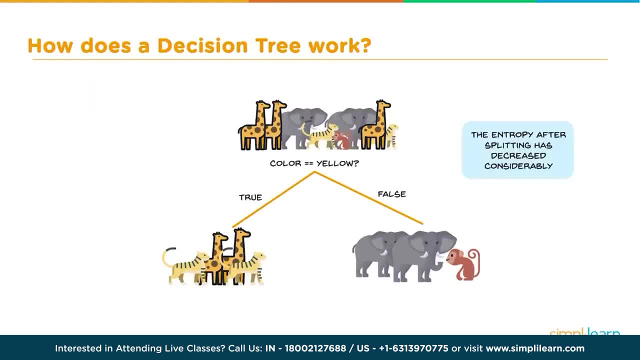 If it's false, it goes to the right. The entropy after the splitting has decreased considerably. However, we still need some splitting at both the branches to attain an entropy value equal to zero. So we decide to split both the nodes using height as the condition, Since every 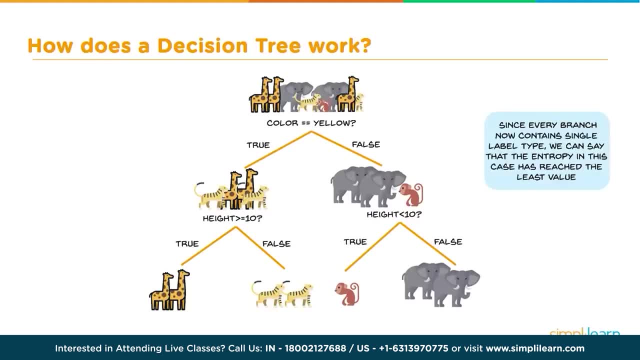 branch now contains single label type. we can say that entropy, in this case, has reached the least value. And here you see, we have the giraffes, the tigers, the monkey and the elephants, all separated into their own groups. This tree, 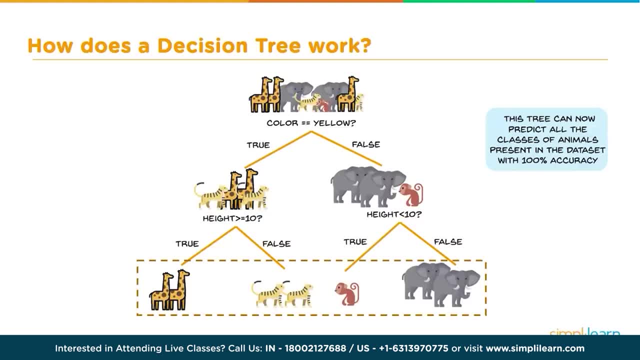 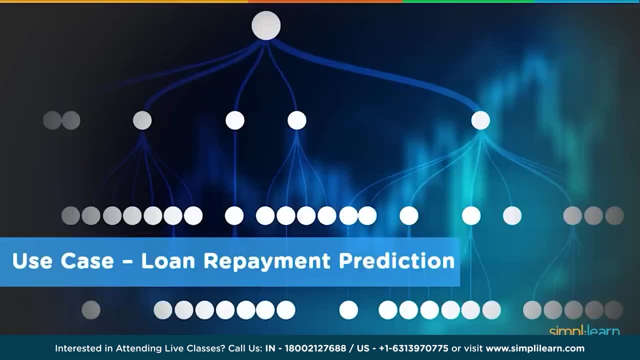 can now predict all the classes of animals present in the data set with 100% accuracy. That was easy Use case: Loan repayment prediction. Let's get into my favorite part and open up some Python and see what the programming code and the scripting looks like In here. 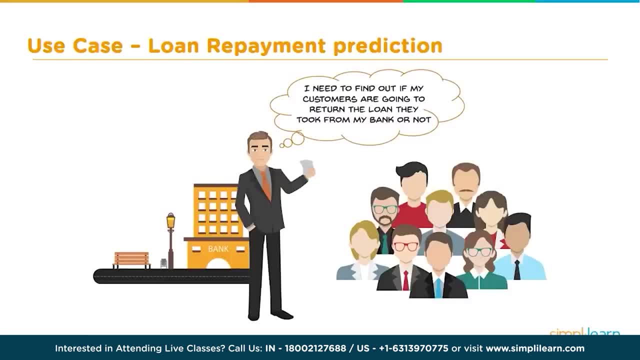 we're going to want to do a prediction And we start with this individual here who's requesting to find out how good his customers are going to be, whether they're going to repay their loan or not for his bank, And from that we want. 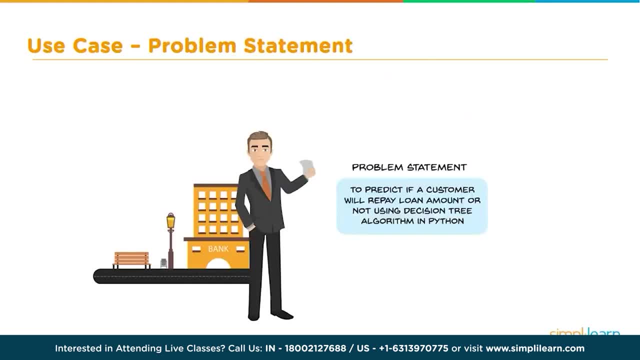 to generate a problem statement to predict if a customer will repay loan amount or not. And then we're going to be using the decision tree algorithm in Python. Let's see what that looks like and let's dive into the code In our first few steps of implementation. 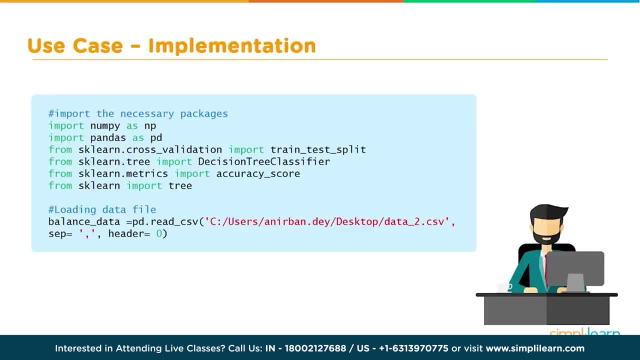 we're going to start by importing the necessary packages that we need from Python, And we're going to load up our data and take a look at what the data looks like. So the first thing I need is: I need something to edit my Python and run it in. So let's flip on. 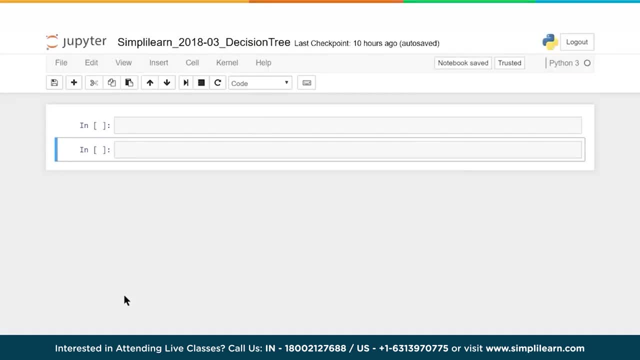 over, And here I'm using the Anaconda Jupyter notebook. Now you can use any Python IDE you like to run it in, But I find the Jupyter notebook's really nice for doing things on the fly, And let's go ahead and just paste that code in the beginning. 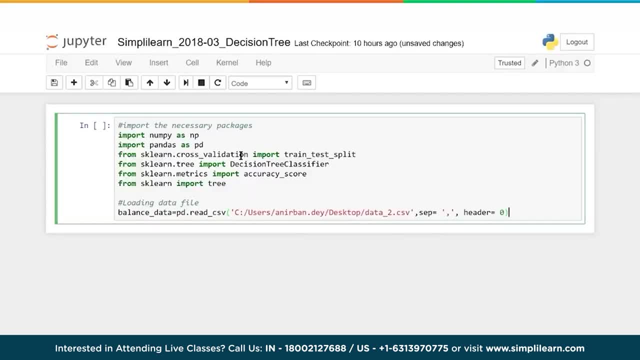 And before we start let's talk a little bit about what we're bringing in, And then we're going to do a couple things in here. We have to make a couple changes as we go through this first part of the import. The first thing we bring in is: 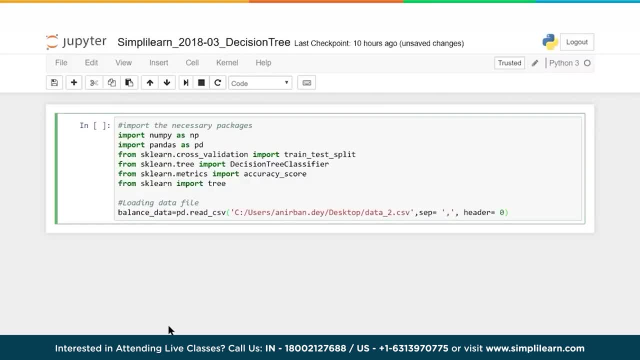 numpy as np. That's very standard When we're dealing with mathematics, especially with very complicated machine learning tools. you almost always see the numpy come in for your numbers. It's called number Python. It has your mathematics in there. In this case, we actually could take. 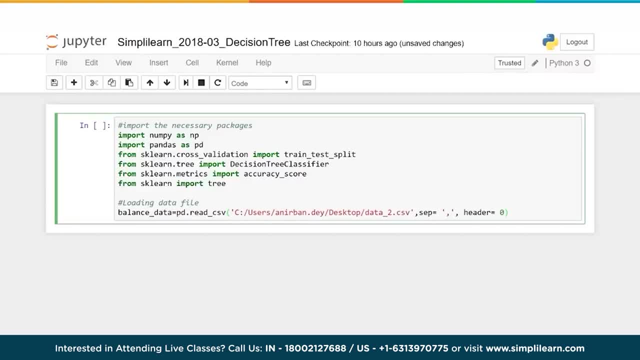 it out, But generally you'll need it for most of your different things you work with. And then we're going to use pandas as pd. That's also a standard. The pandas is a data frame setup And you can liken this to taking. 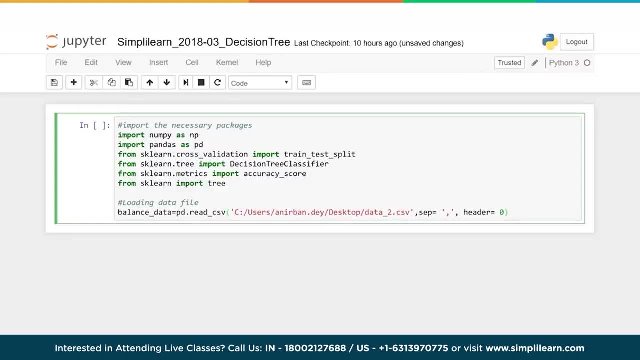 your basic data and storing it in a way that looks like an Excel spreadsheet. So as we come back to this, when you see np or pd, those are very standard uses- you'll know that that's the pandas And I'll show you a little bit more. 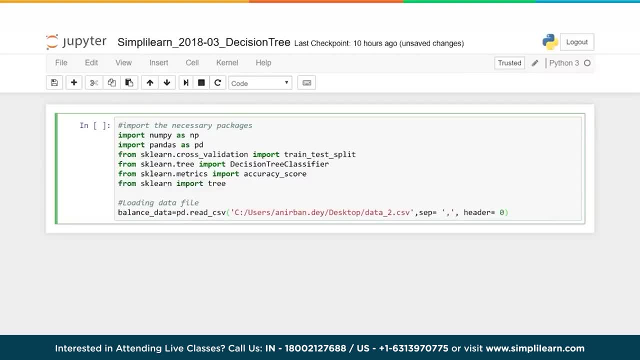 when we explore the data in just a minute, Then we're going to need to split the data. So I'm going to bring in our train, test and split. And this is coming from the sklearn package: cross validation. In just a minute we're going to change. 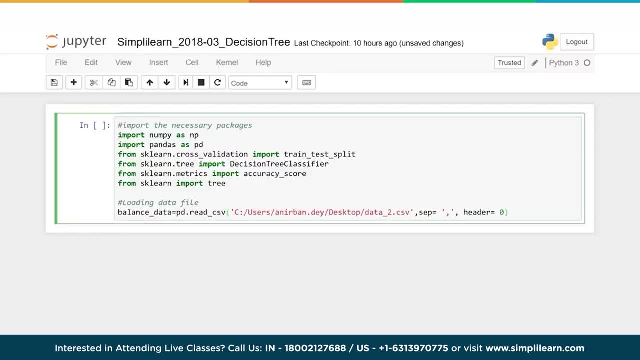 that, And we'll go over that too. And then there's also the sktree import decision tree classifier. That's the actual tool we're using. Remember I told you, don't be afraid of the mathematics, It's going to be done for you. Well, the decision tree classifier. 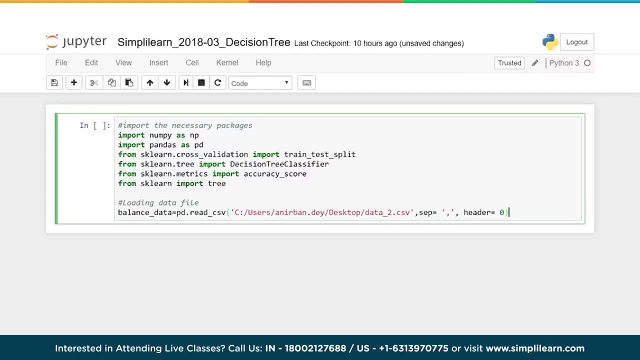 has all that mathematics in there for you, So you don't have to figure it back out again. And then we have sklearnmetrics for accuracy score. We need to score our setup. That's the whole reason. we're splitting it between the training and testing. 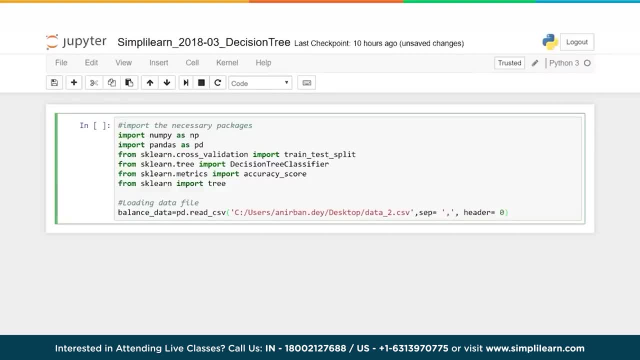 data. And finally, we still need the sklearn import tree And that's just the basic tree function that's needed for the decision tree classifier. And finally, we're going to load our data down here And I'm going to run this And we're going to get. 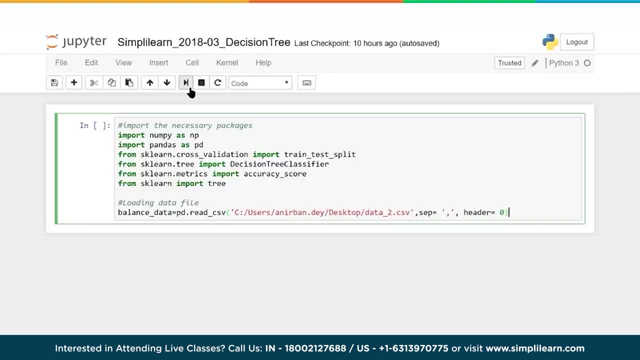 two things on here. One, we're going to get an error And two, we're going to get a warning. Let's see what that looks like. So the first thing we had is: we have an error. Why is this error here? Well, it's looking. 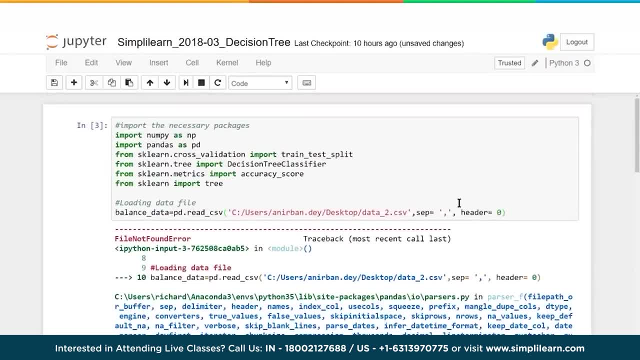 at this and says: I need to read a file And when this was written, the person who wrote it, this is their path, where they stored the file. So let's go ahead and fix that And I'm going to put in here my file path. I'm just going to call it. 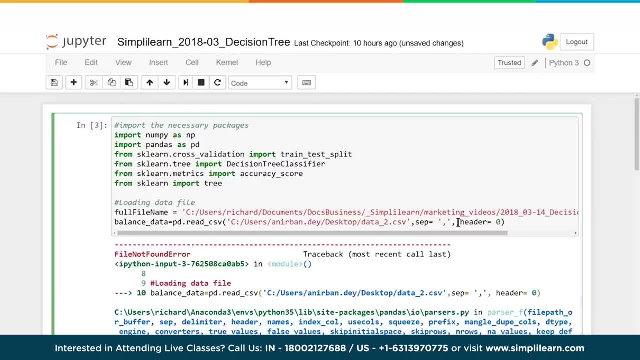 full file name And you'll see. it's on my C drive And there's this very lengthy setup on here where I stored the data2.csv file. Don't worry too much about the full path because on your computer it will be different: The data.2.csv. 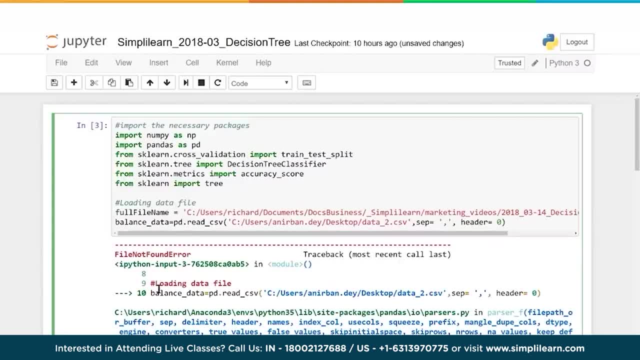 file was generated by sklearn. If you want a copy of that, you can comment down below and request it here in the YouTube, And then, if I'm going to give it a name- full file name- I'm going to go ahead and change it here. 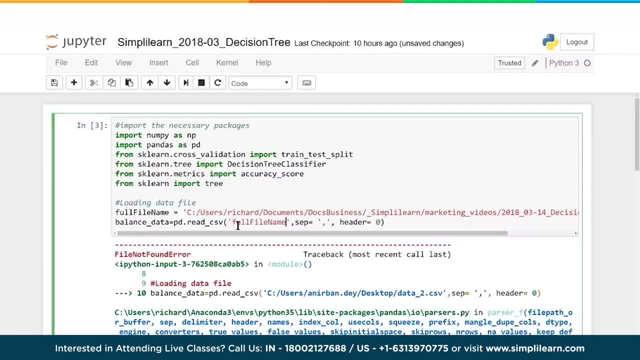 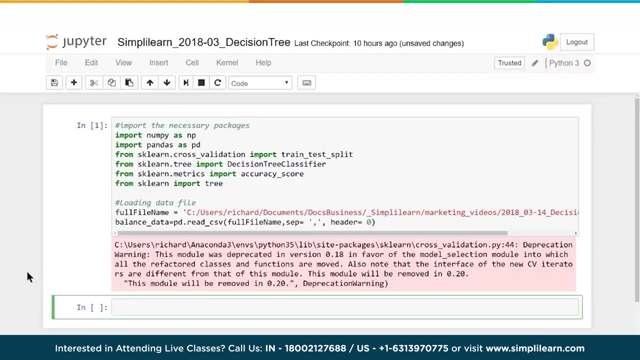 to full file name. So let's go ahead and run it now and see what happens. And we get a warning. When you're coding, understanding these different warnings and these different errors that come up is probably the hardest lesson to learn. So let's just go ahead and take. 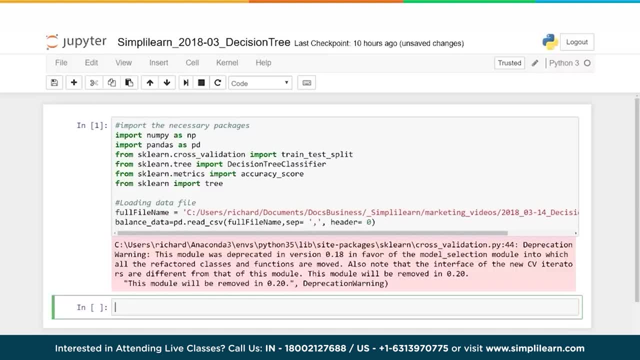 a look at this and use this as a opportunity to understand what's going on here. If you read the warning, it says the cross validation is depreciated. So it's a warning on it's being removed And it's going to be moved in favor. 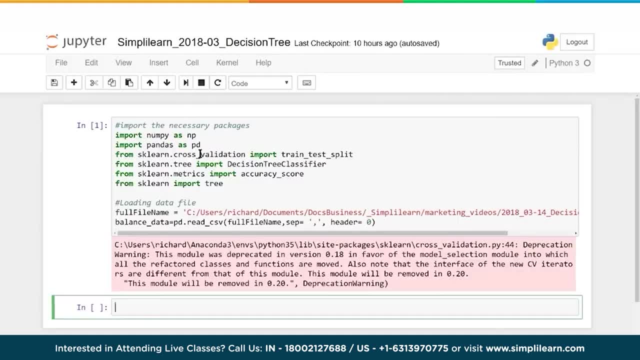 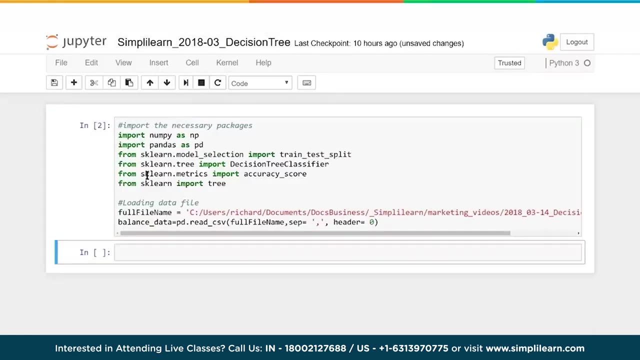 of the model selection. So if we go up here, we have sklearncrossvalidation, and if you research this and go to the sklearn site, you'll find out that you can actually just swap it right in there with model selection. And so when I come in here and I run it again, 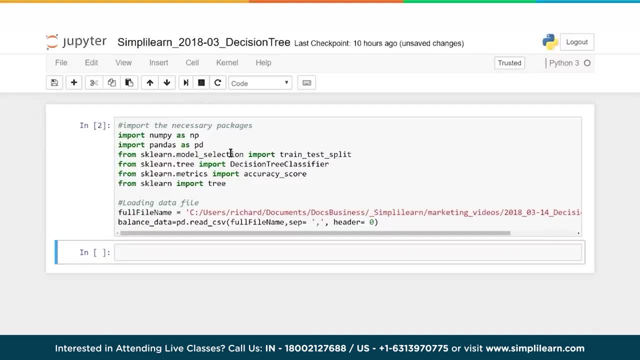 that removes a warning. What they've done is they've had two different developers develop it in two different branches, And then they decided to keep one of those and eventually get rid of the other one. That's all that is, And very easy and quick to fix. 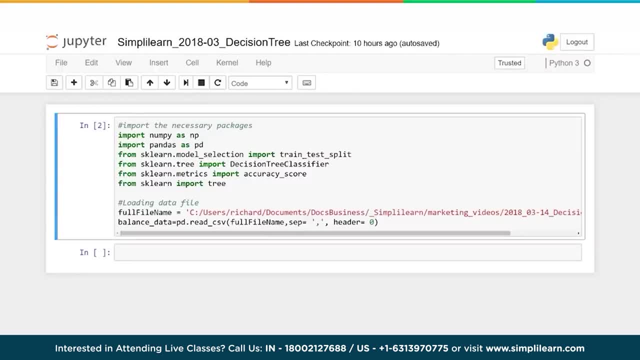 Before we go any further, I went ahead and opened up the data from this file. Remember the data file we just loaded on here, The data underscore two dot csv. Let's talk a little bit more about that and see what that looks like, both as a. 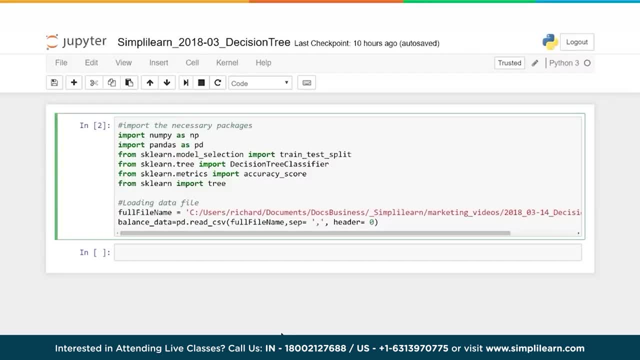 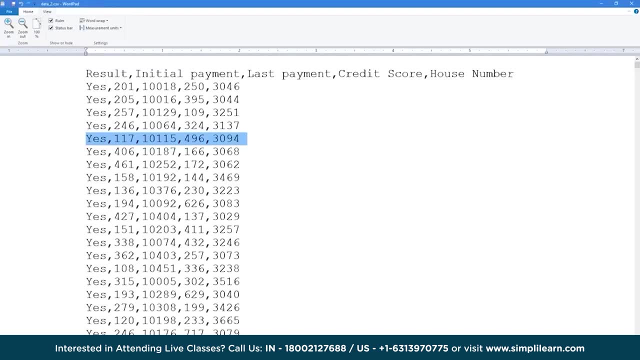 text file because it's a comma separated variable file and in a spreadsheet. This is what it looks like as a basic text file. You can see at the top they've created a header. It's got one, two, three, four, five columns. 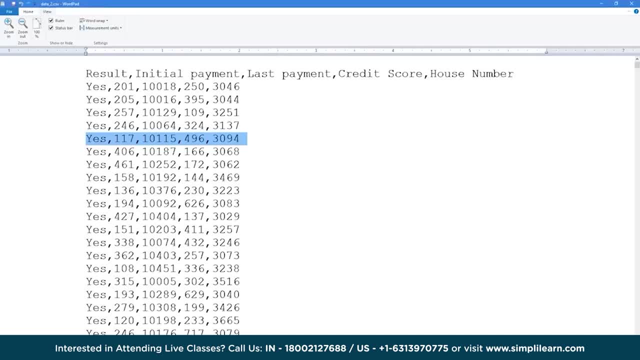 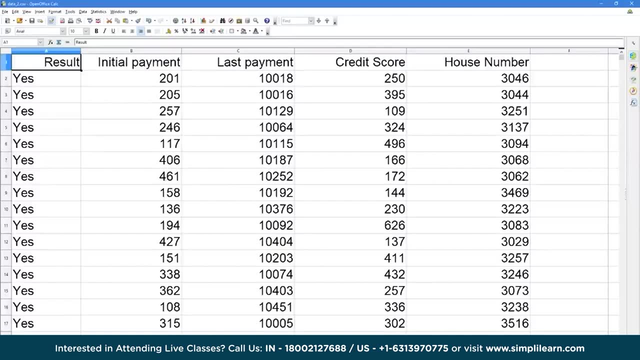 And each column has data in it. And let me flip this over because we're also going to look at this in an actual spreadsheet, so you can see what that looks like. And here I've opened it up in the open office, calc, which is pretty much the same as Excel. 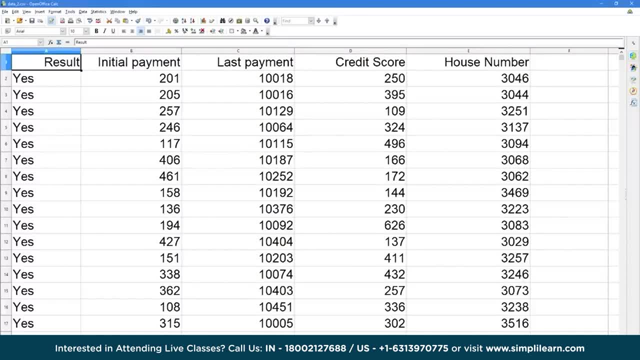 And zoomed in and you can see we've got our columns and our rows of data A little easier to read. in here We have a result. yes, yes, no, we have initial payment. last payment. credit score: house number. 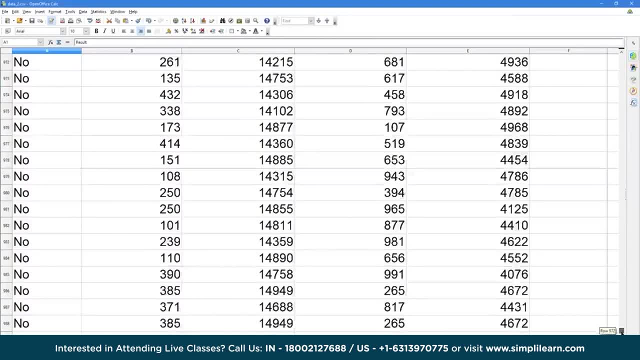 if we scroll way down, we'll see that this occupies a thousand and one lines of code or lines of data, with the first one being a column and then one thousand lines of data. Now, as a programmer, if you're looking at a small 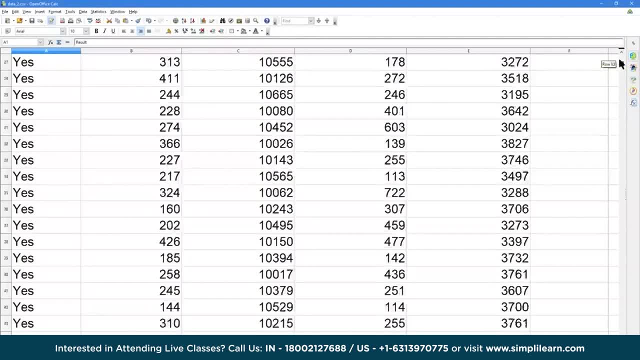 amount of data. I usually start by pulling it up in different sources so I can see what I'm working with. But in larger data you won't have that option. It'll just be two large. so you need to either bring in a small 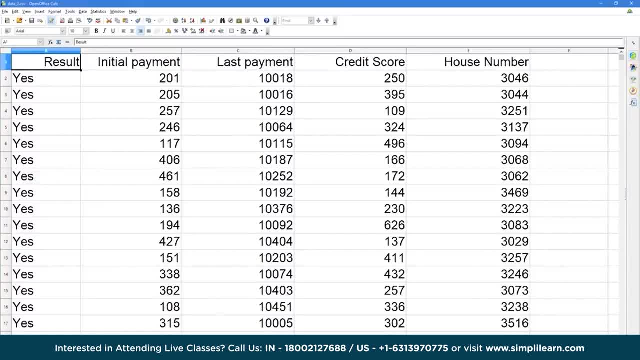 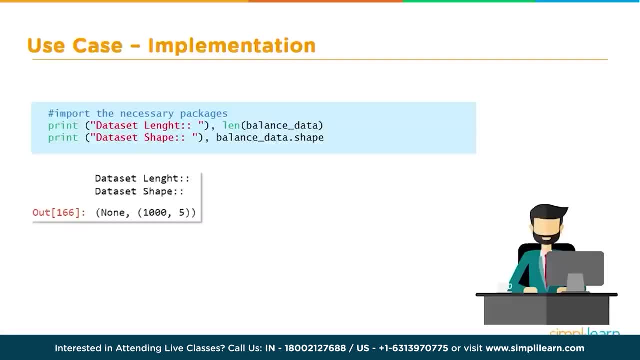 amount that you can look at it like we're doing right now, or we can start looking at it through the Python code. So let's go ahead and move on and take the next couple steps to explore the data using Python. Let's go ahead and. 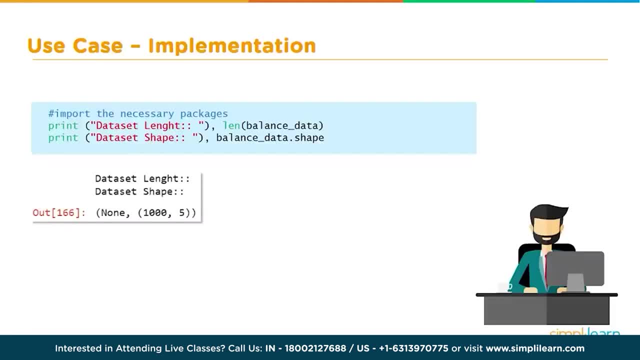 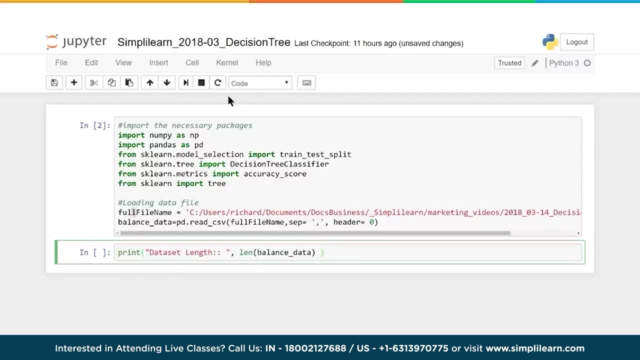 see what it looks like in Python to print the length and the shape of the data. So let's start by printing the length of the database. We can use a simple lin function from Python And when I run this you'll see that it's a thousand. 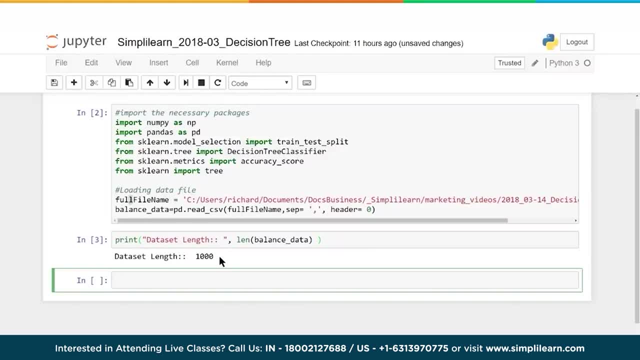 long, And that's what we expected. There's a thousand lines of data in there. if you subtract the column head. This is one of the nice things when we did the balance data from the Panda Read CSV, You'll see that the header is: 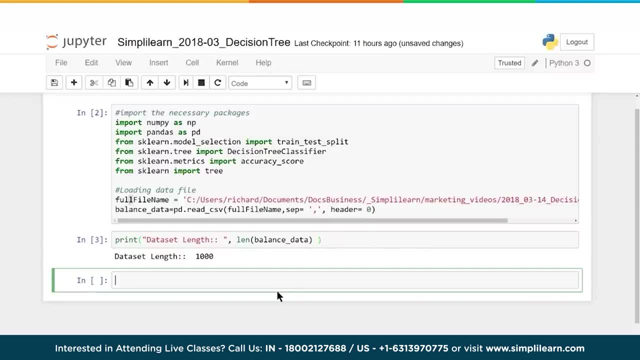 row zero, so it automatically removes a row and then shows the data separate. It does a good job sorting that data out for us, And then we can use a different function. Let's take a look at that And again, we're going to. 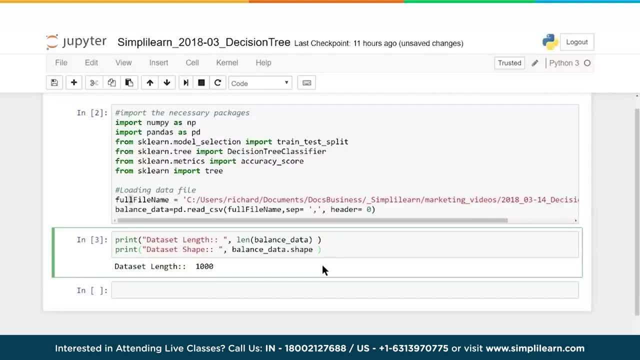 utilize the tools in Panda And since the balance underscore data was loaded as a Panda data frame, we can do a shape on it, And let's go ahead and run the shape and see what that looks like. What's nice about this shape is not only does 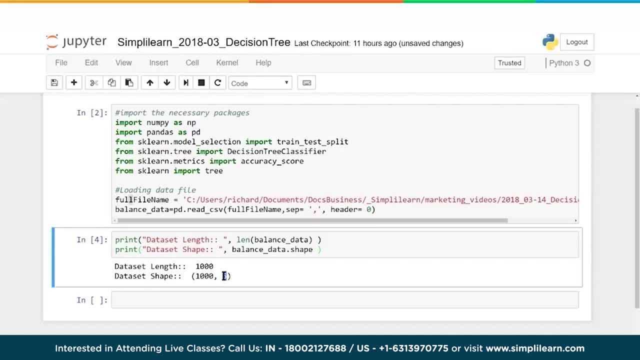 it give me the length of the data. we have a thousand lines. it also tells me there's five columns. So when we were looking at the data, we had five columns of data. And then let's take one more step to explore the data using Python. 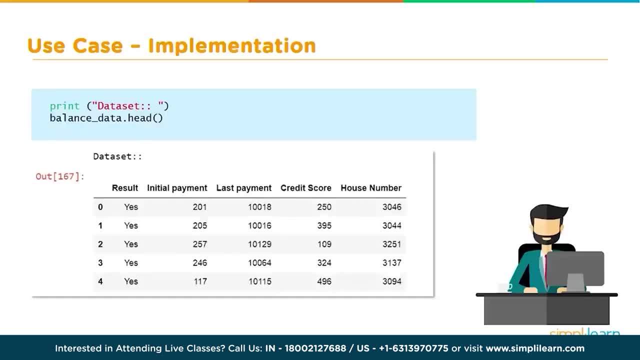 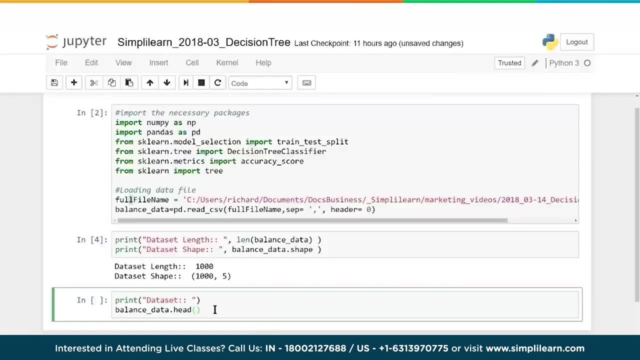 And now that we've taken a look at the length and the shape, let's go ahead and use the Pandas module for head- Another beautiful thing in the data set that we can utilize. So let's put that on our sheet here and we have print data set. 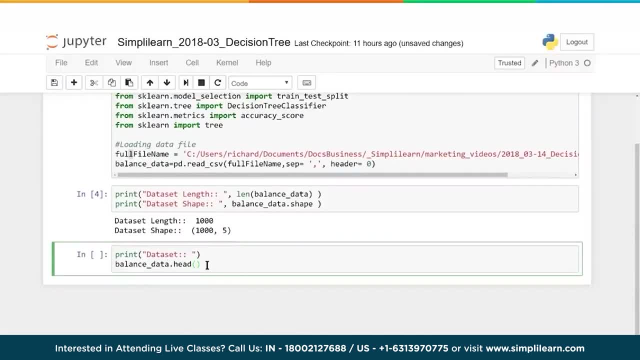 and balance data dot head And this is a Pandas print statement of its own, So it has its own print feature in there. And then we went ahead and gave a label for our print job here of data set, just a simple print statement. And when we run, 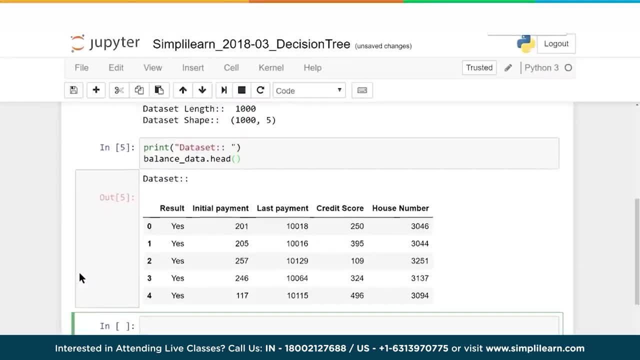 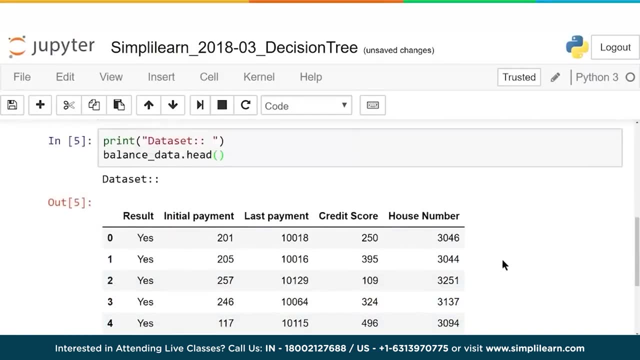 that, and let's just take a closer look at that. Let me zoom in here. There we go. Pandas does such a wonderful job of making this a very clean, readable data set So you can look at the data, you can look at the column headers. 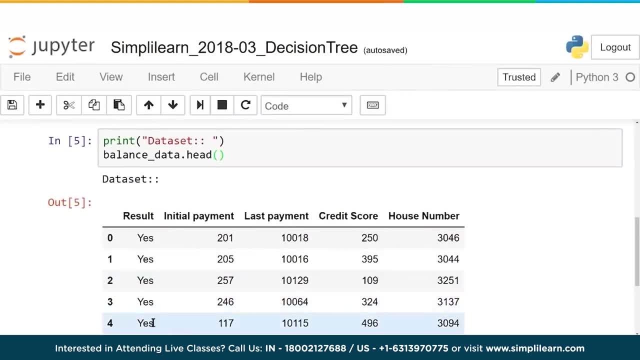 you can have it. when you put it as the head, it prints the first five lines of the data And we always start with zero. So we have five lines. we have zero. one, two, three, four instead of one, two, three, four, five. 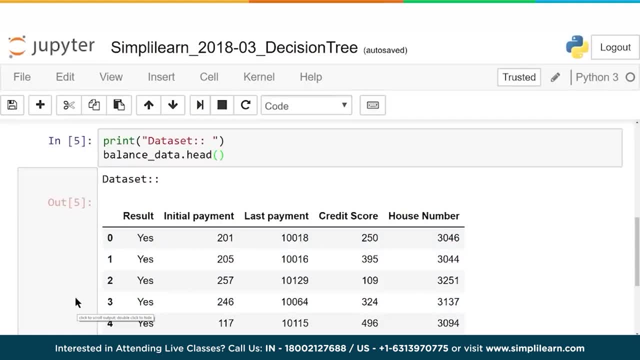 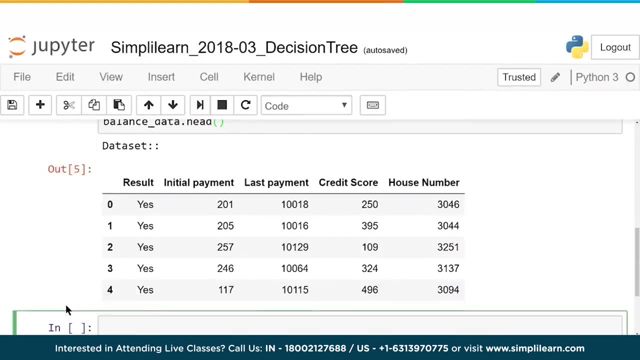 That's a standard scripting and programming set. is you want to start with the zero position? And that is what the data head does. It pulls the first five rows of data, puts it in a nice format that you can look at and view- Very powerful. 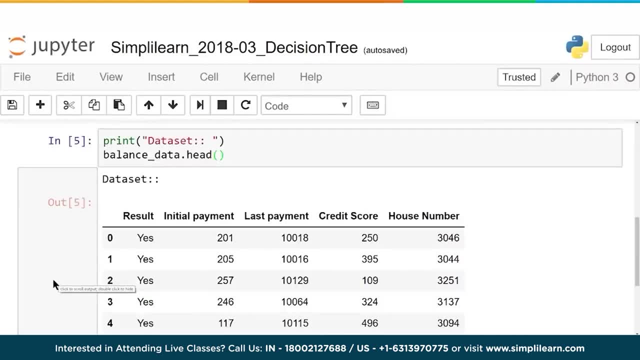 tool to view the data. So instead of having to flip and open up an Excel spreadsheet or open OfficeCal, or trying to look at a Word doc where it's all scrunched together and hard to read, you can now get a nice open view of what you're working with. 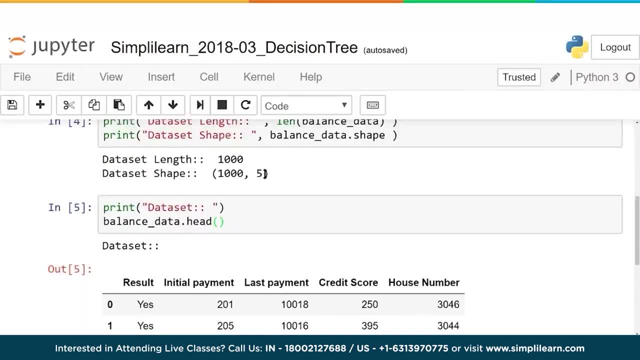 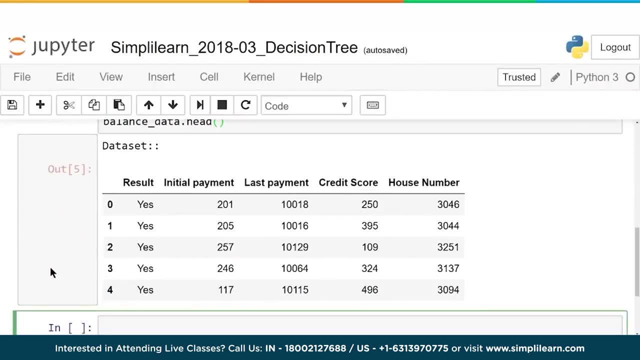 We're working with a shape of a thousand long, five wide, so we have five columns And we do the full data head. you can actually see what this data looks like: The initial payment, last payment, credit scores, house number. 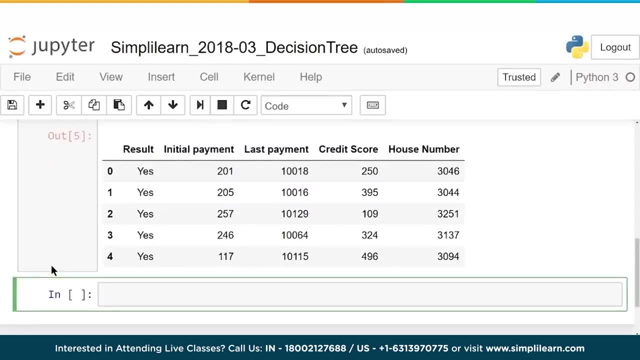 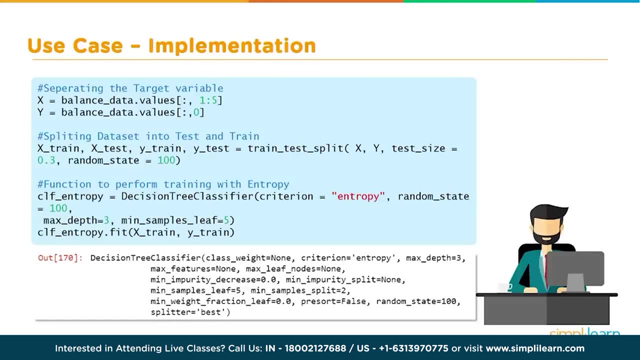 So let's take this, now that we've explored the data, and let's start digging into the decision tree. So in our next step, we're going to train and build our data tree, And to do that, we need to first separate the data. 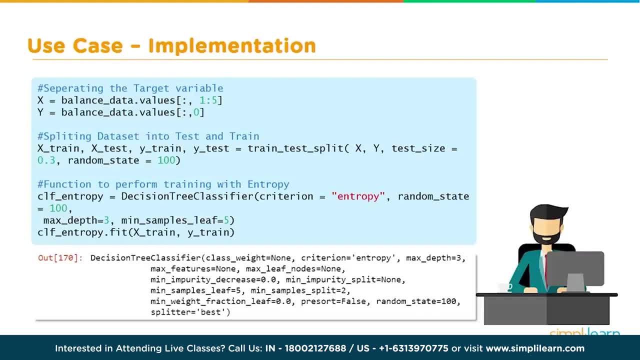 out. We're going to separate it into two groups so that we have something to actually train the data with, and then we have some data on the side to test it, to see how good our model is. Remember, with any of the machine learning, you always want to have some kind of test. 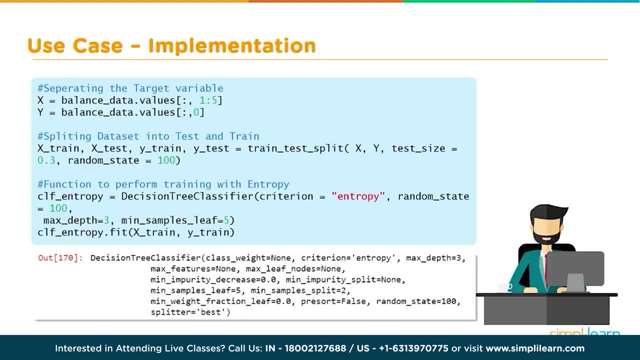 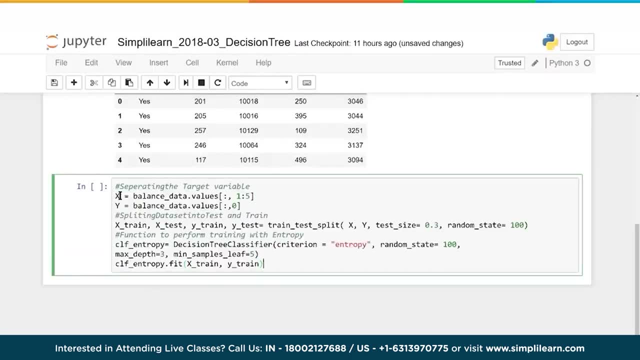 set to weigh it against. so you know how good your model is when you distribute it. Let's go ahead and break this code down And look at it in pieces. So first we have our x and y. Where do x and y come from? Well, 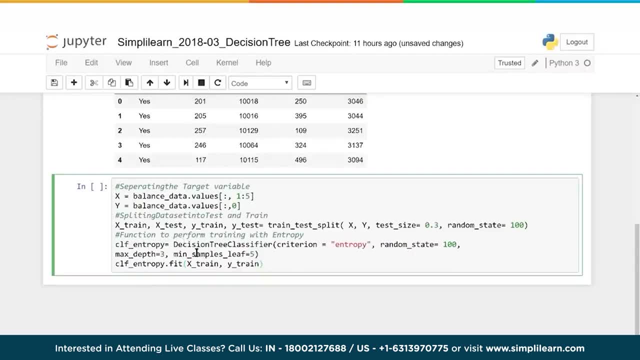 x is going to be our data and y is going to be the answer or the target. You can look at it as source and target. In this case, we're using x and y to denote the data in and the data that we're actually trying to. 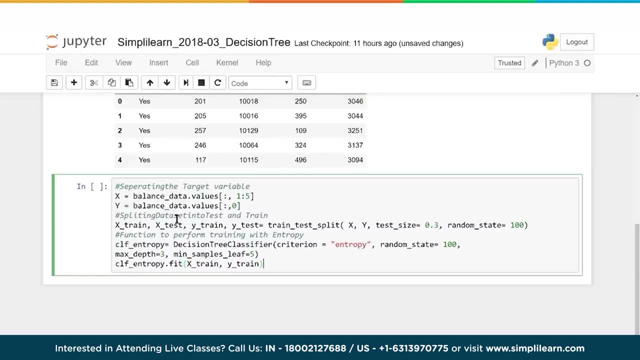 guess what the answer's going to be, And so to separate it we can simply put in: x equals the balance of the data. dot values. The first brackets means that we're going to select all the lines in the database. so it's all the data. 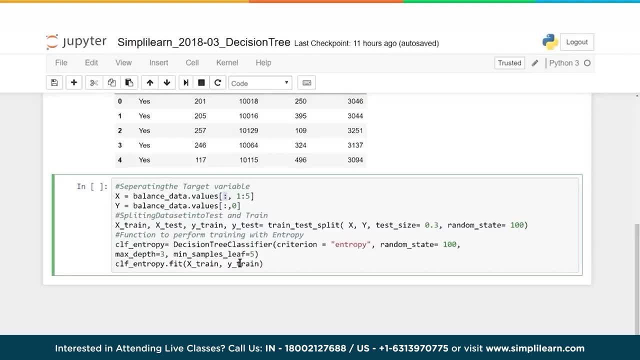 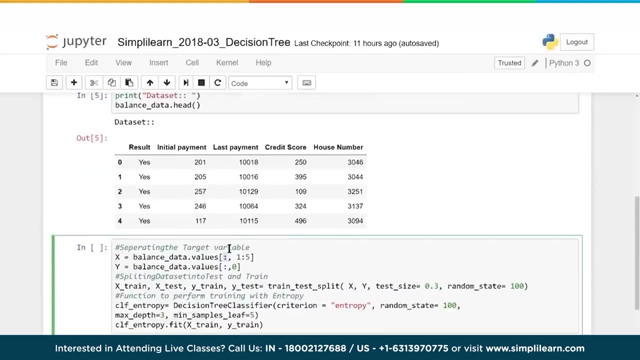 And the second one says we're only going to look at columns one through five. Remember we always start with zero. Zero is a yes or no and that's whether the loan went default or not. So we want to start with one. If we go back up here, 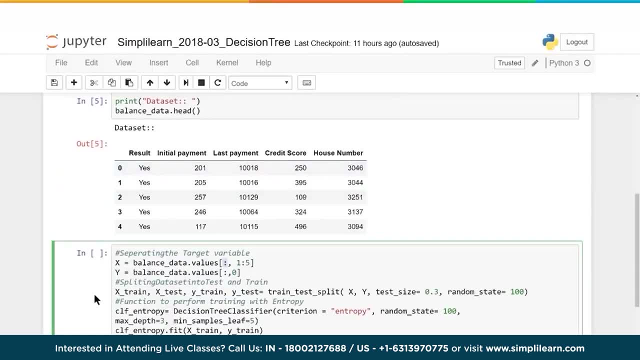 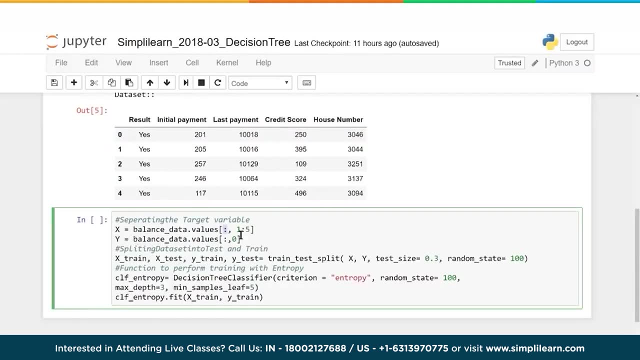 that's the initial payment and it goes all the way through the house number. Well, if we want to look at one through five, we can do the same thing for y, which is the answers, and we're going to set that just equal to the. 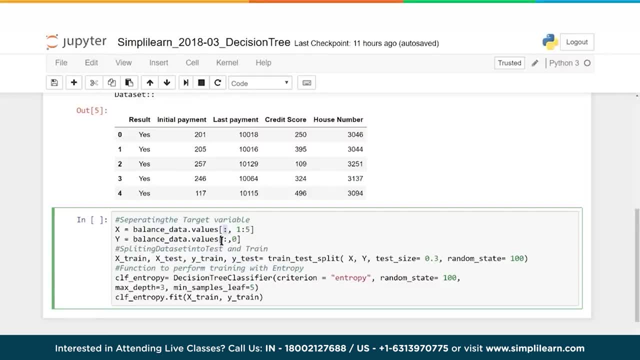 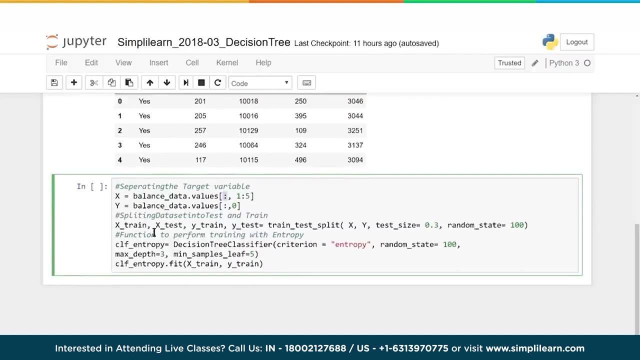 zero row. So it's just the zero row and then it's all rows going in there. So now we've divided this into two different data sets, One of them with the data going in and one with the answers. Next we need to split the data. 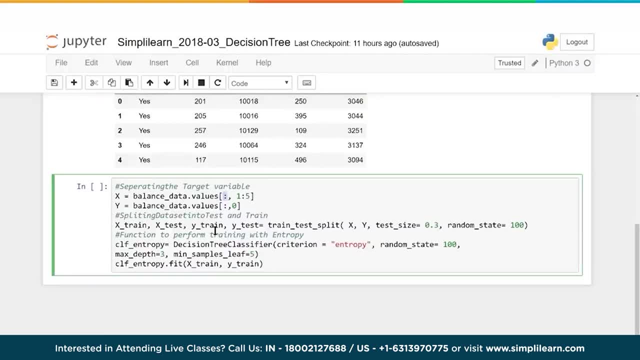 And here you'll see that we have it split into four different parts. The first one is your x training, your x test, your y train, your y test. Simply put, we have x going in where we're going to train it and we have to. 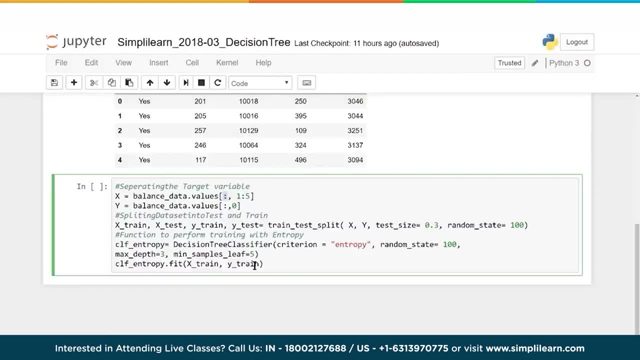 know the answer to train it with. And then we have x test, where we're going to test that data And we have to know in the end what the y was supposed to be. And that's where this train test split comes in that we loaded earlier in the modules. 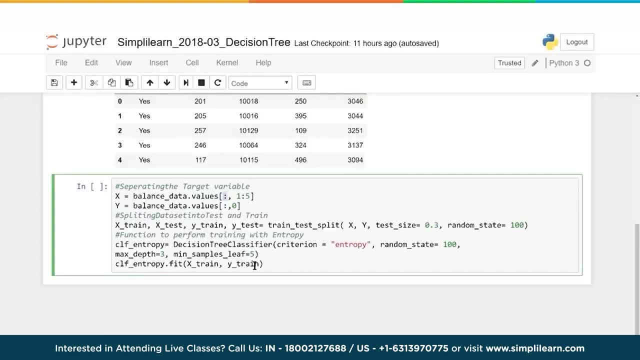 This does it all for us And you can see. they set the test size equal to .3, so that's roughly 30% will be used in the test. And then we use a random state, so it's completely random which rows it takes out of there. 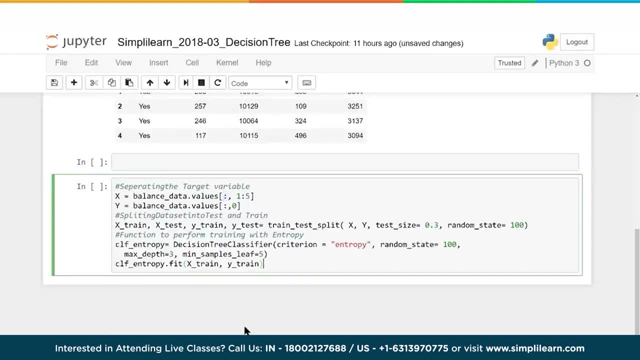 And then finally we get to actually build our decision tree And they've called it here clf, underscore, entropy, That's the actual decision tree or decision tree classifier, And in here they've added a couple variables which we'll explore in just a minute. 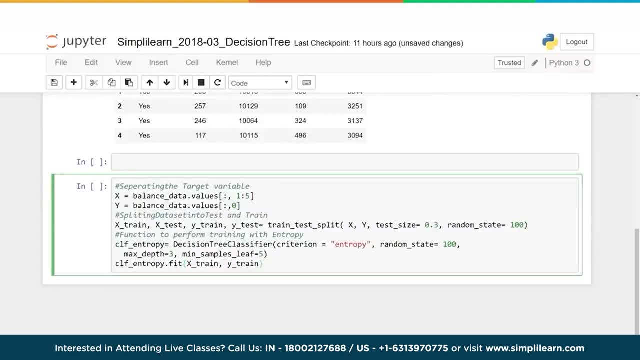 And then, finally, we need to fit the data to that. So we take our clf entropy that we created and we fit the x train, and since we know the answers for x train are the y train, we go ahead and put those in. 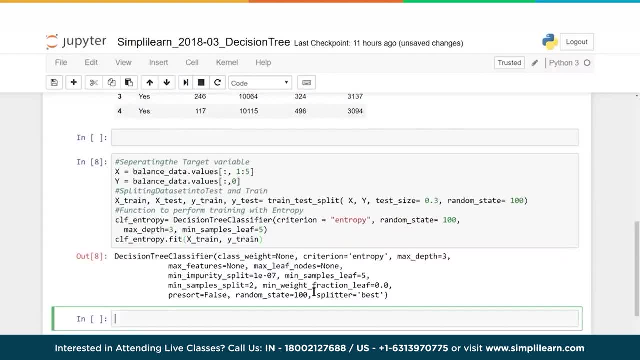 And let's go ahead and run this. And what most of these sklearn modules do is when you set up the variable- in this case we set the clf entropy equal to decision tree classifier- it automatically prints out what's in that decision tree. There's a lot of variables you can play. 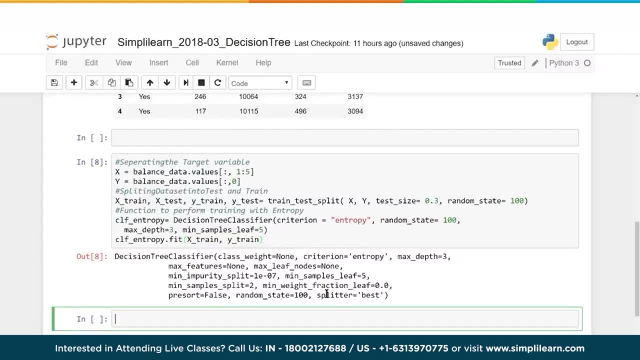 with in here And it's quite beyond the scope of this tutorial to go through all of these and how they work. But we're working on entropy. that's one of the options We've added that it's completely a random state of 100, so 100%. 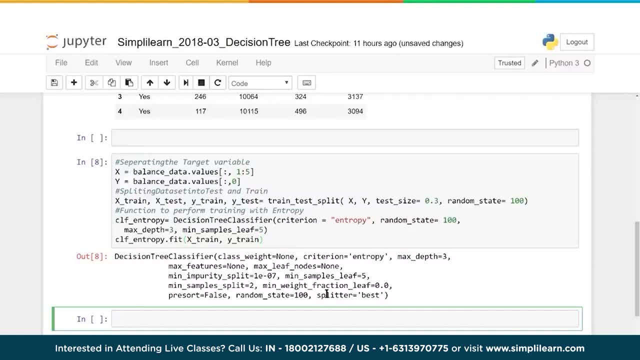 And we have a max depth of 3.. Now, the max depth, if you remember above when we were doing the different graphs of animals, means it's only going to go down 3 layers before it stops, And then we have minimal samples of leaves as 5.. 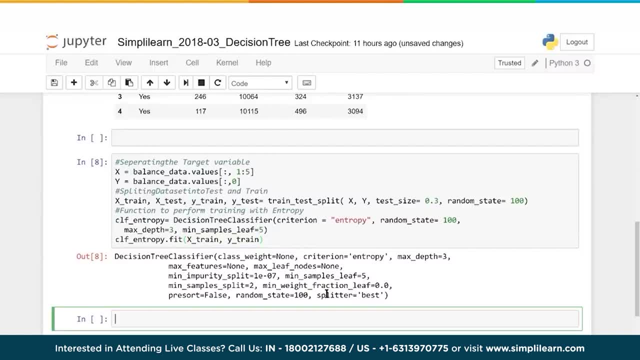 So it's going to have at least 5 leaves at the end. So we'll have at least 3 splits, we'll have no more than 3 layers and at least 5 end leaves, with the final result at the bottom, Now that we've created. 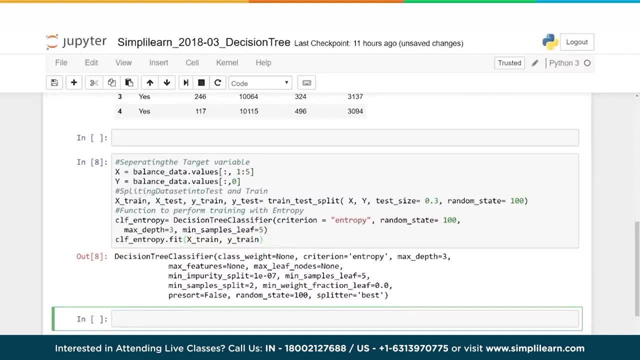 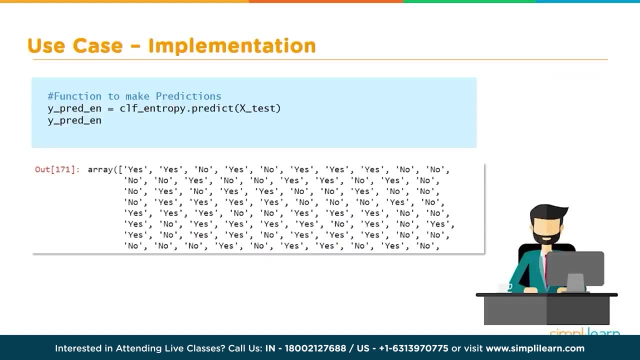 our decision tree classifier not only created it, but trained it. let's go ahead and apply it and see what that looks like. So let's go ahead and make a prediction and see what that looks like. We're going to paste our predict code in here. 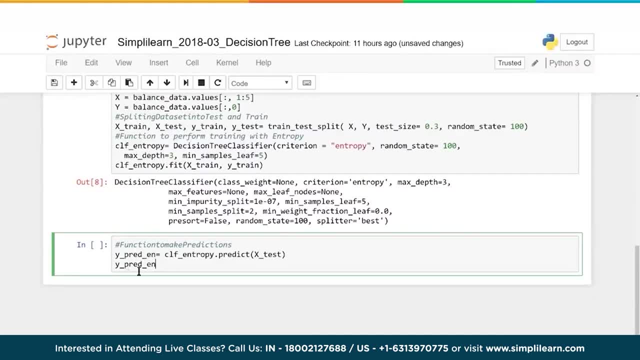 And before we run it, let's just take a quick look at what it's doing. here We have a variable, yPredict- that we're going to do And we're going to use our variable clfEntropy that we created, And then you'll see predict. 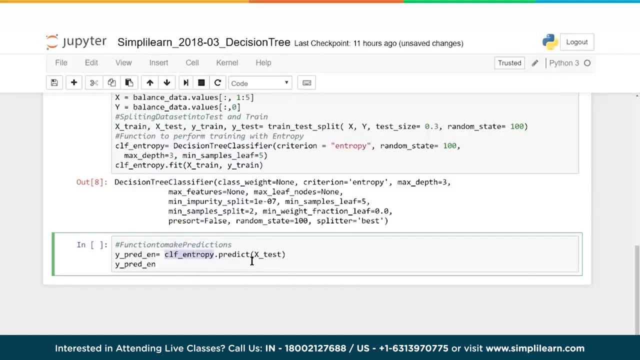 And it's very common in the sklearn modules that their different tools have the predict when you're actually running a prediction. In this case, we're going to put our xTestData in here Now, if you delivered this for use- an actual commercial use- and 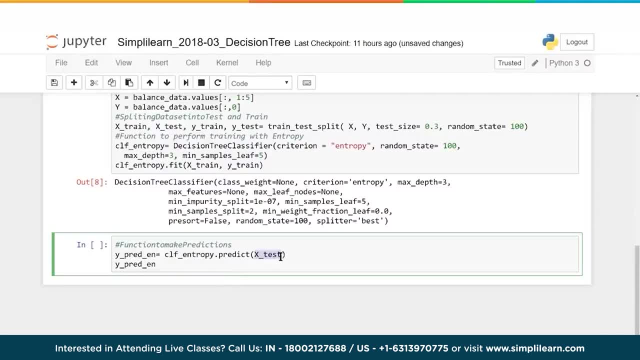 distributed it. this would be the new loans you're putting in here to guess whether the person's going to be pay them back or not. In this case, though, we need to test out the data and just see how good our sample is, how good our tree. 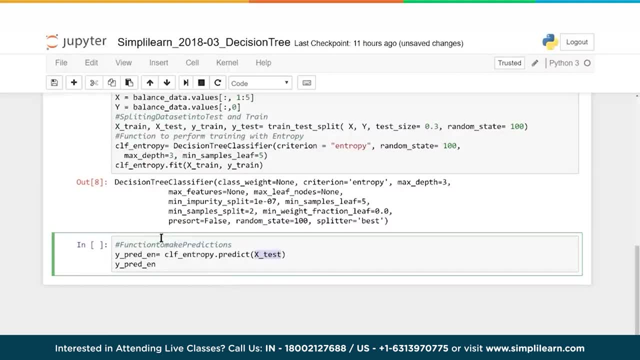 does at predicting the loan payments. And finally, since Anaconda Jupyter Notebook works as a command line for Python, we can simply put the yPredict e in to print it. I could just as easily have put the print and put brackets around yPredict e in to print it out. 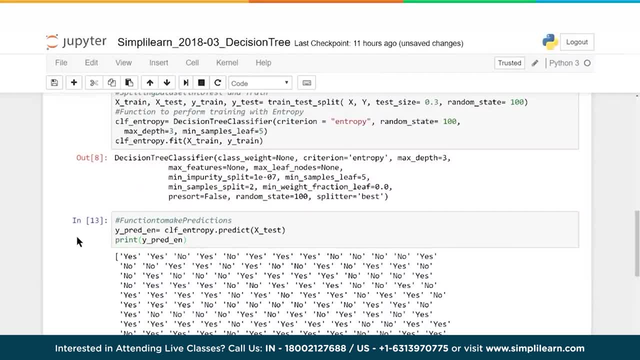 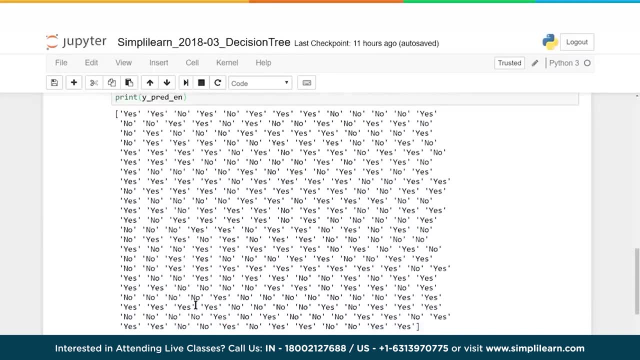 We'll go ahead and do that. it doesn't matter which way you do it, And you'll see right here that it runs a prediction. This is roughly 300 in here. Remember it's 30% of 1000, so you should have about 300 answers in here. 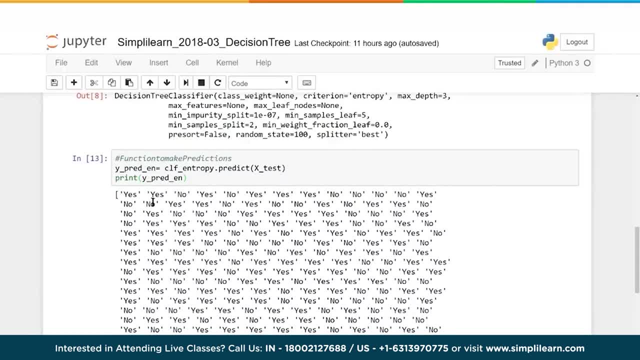 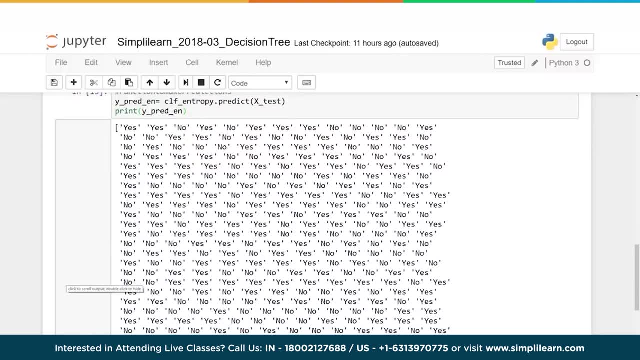 And this tells you which each one of those lines of our test went in there, and this is what our yPredict came out. So let's move on to the next step, where we're going to take this data and try to figure out just how good a model we have. 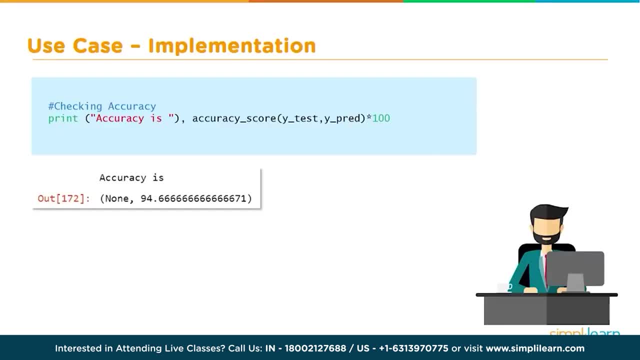 So here we go. since sklearn does all the heavy lifting for you and all the math, we have a simple line of code to let us know what the accuracy is, And let's go ahead and go through that and see what that means and what that looks like. 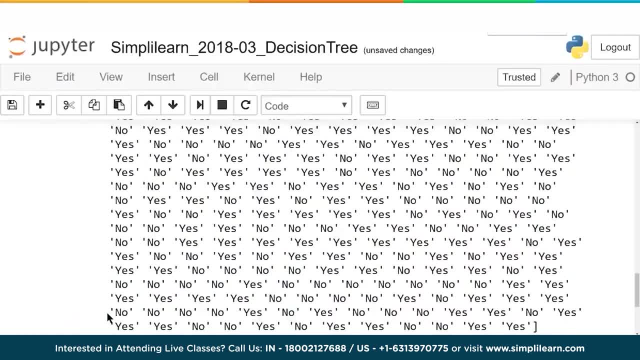 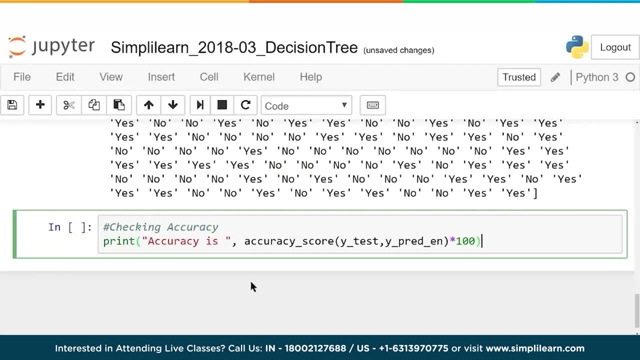 Let's go ahead and paste this in and let me zoom in a little bit. There we go, See, we have a nice full picture And we'll see. here we're just going to do a print. accuracy is, and then we do the accuracy score. 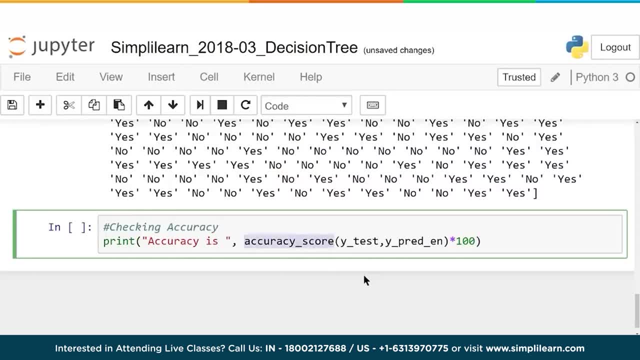 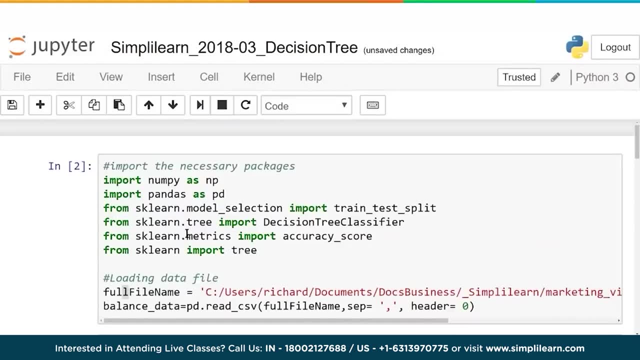 And this was something we imported earlier, if you remember, at the very beginning. Let me just scroll up there real quick so you can see where that's coming from. That's coming from here, down here, from sklearnmetrics import accuracy score And you could probably run a script. 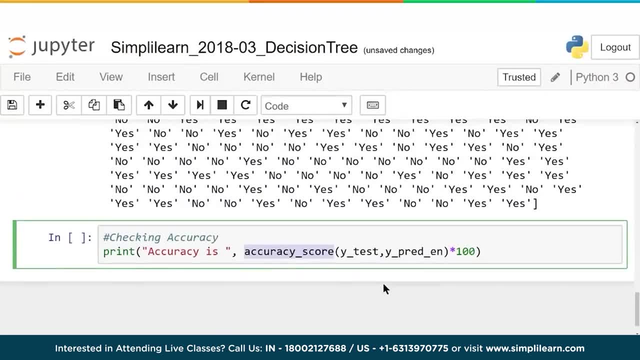 make your own script to do this very easily. How accurate is it? How many out of 300 do we get right? And so we put in our yTest- that's the one we ran the predict on- And then we put in our yPredictEn. 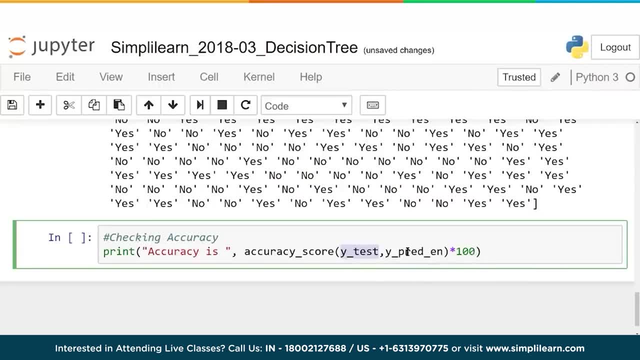 that's the answers we got And we're just going to multiply that by 100, because this is just going to give us an answer as a decimal And we want to see it as a percentage And let's run that and see what it looks like. 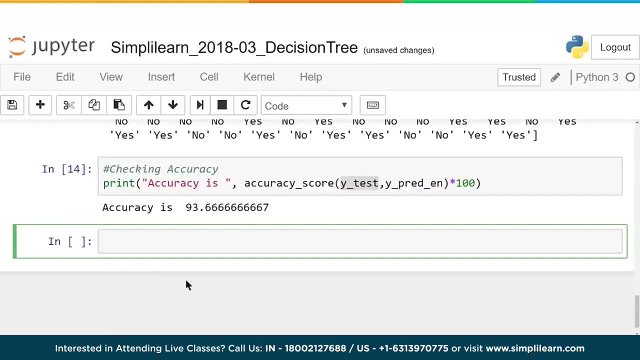 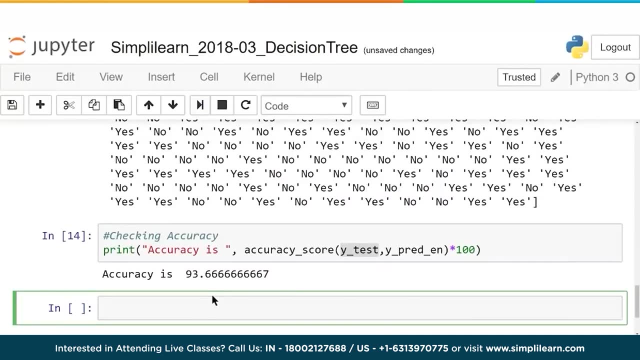 And if you see, here we got an accuracy of 93.66667.. So when we look at the number of loans and we look at how good our model fit, we can tell people it has about a 93.6 fitting to it. So just a quick recap on that. 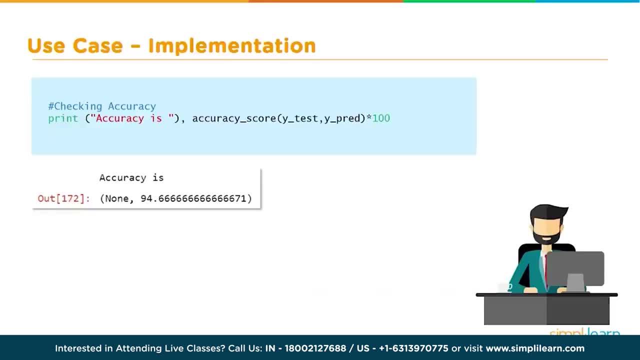 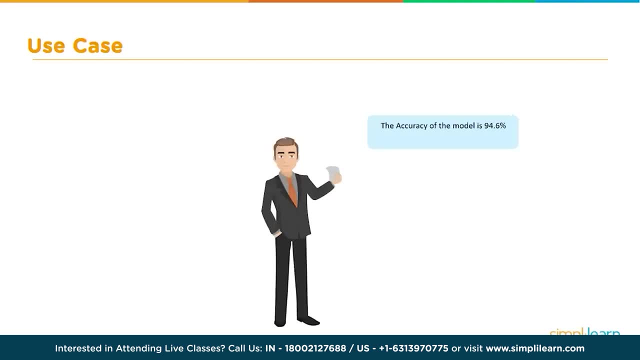 We now have accuracy set up on here, And so we have created a model that you can use that uses the decision tree algorithm to predict whether a customer will repay the loan or not. The accuracy of the model is about 94.6%. The bank can now use this model. 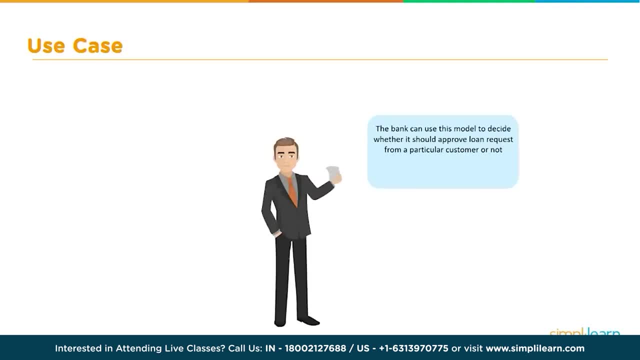 to decide whether it should approve the loan request from a particular customer or not, And so this information is really powerful. We may not be able to, as individuals, understand all these numbers, because they have thousands of numbers that come in, But you can see that this is a smart decision. 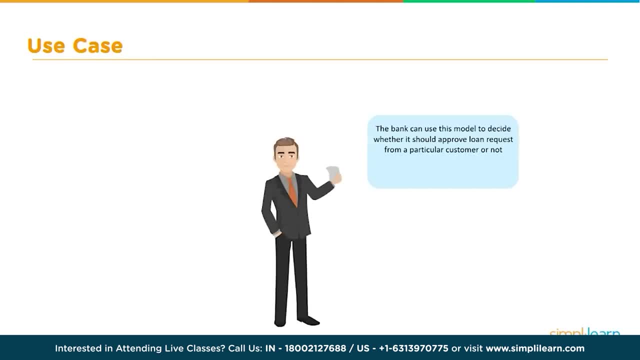 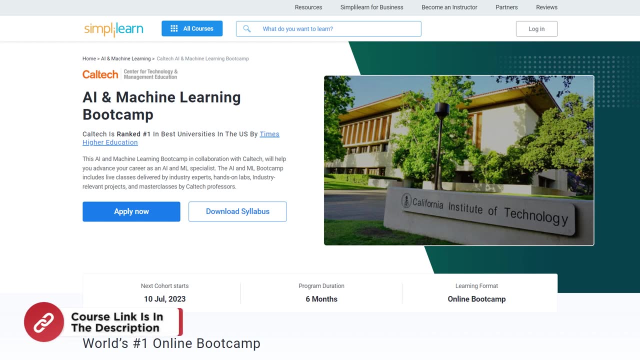 for the bank to use a tool like this to help them to predict how good their profit is going to be and how many are going to default or not. And now we are thrilled to present our AI Bootcamp that is designed to equip you with the knowledge and skills 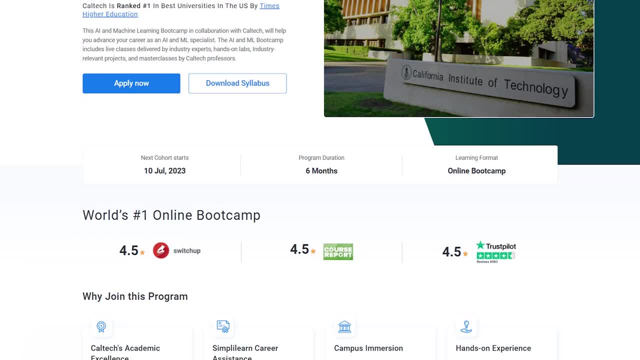 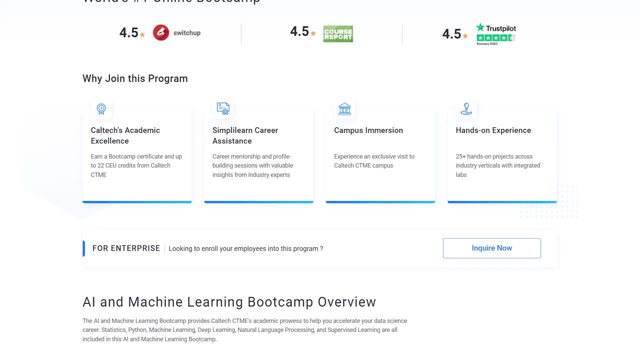 you need to thrive in this fast paced and ever evolving field. In this 6 months intensive and immersive learning experience, you will have the opportunity to dive head first into the subject matter, gaining hands on experience and building a strong foundation in AI. We believe in a practical approach. 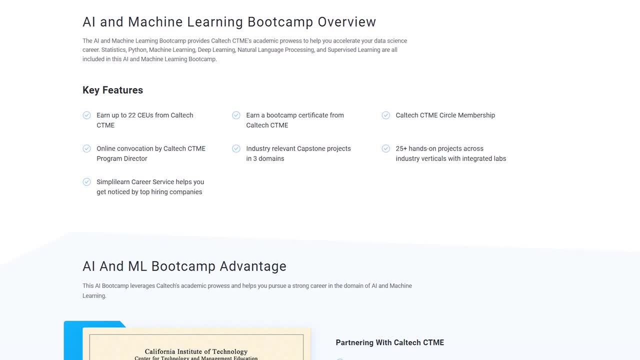 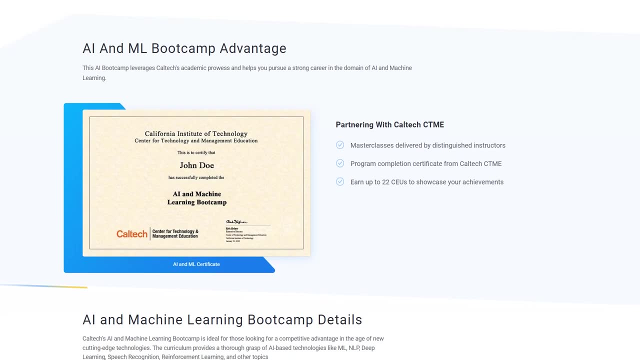 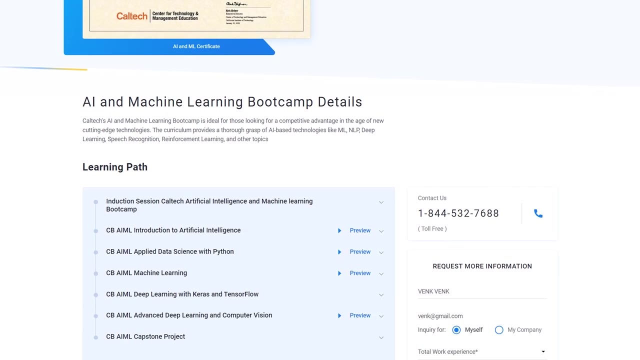 where you will work on 25 plus hands on projects across various industry verticals, providing you with real world experience. What sets our bootcamp apart is our partnership with Caltech CTMA, ensuring academic excellence and industry recognition. By successfully completing the bootcamp, you will earn a prestigious certificate. 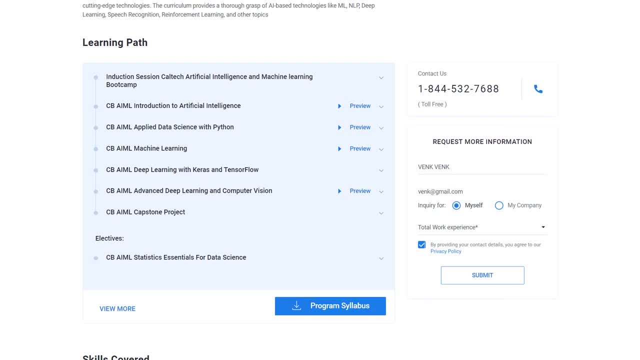 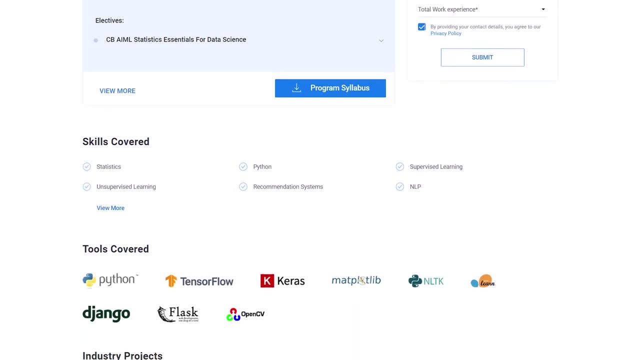 and up to 22 CEU credits from Caltech CTMA validating your expertise in the field. So are you ready to embark on this transformative journey? Are you ready to unlock the power of AI and take your career to new heights? If so, enroll in our AI Bootcamp today. 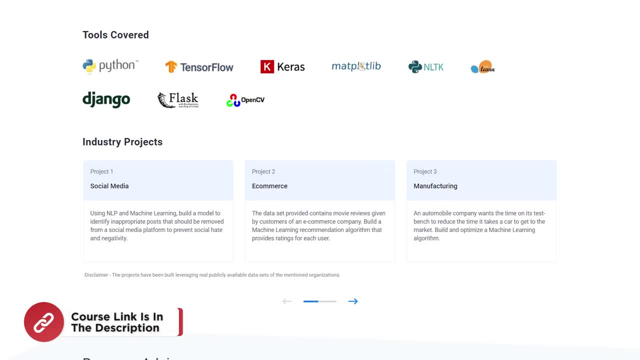 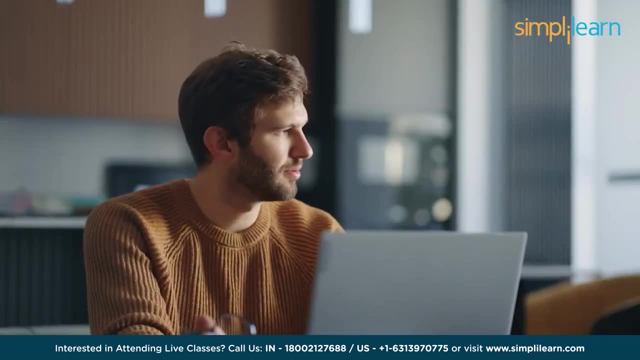 and become part of the AI revolution. The course link is mentioned below And in the description box below. Ever get stuck while writing an email, finding the right words, Or stuck on that article you can't find the final words for. Well, to get rid of this writer's block. 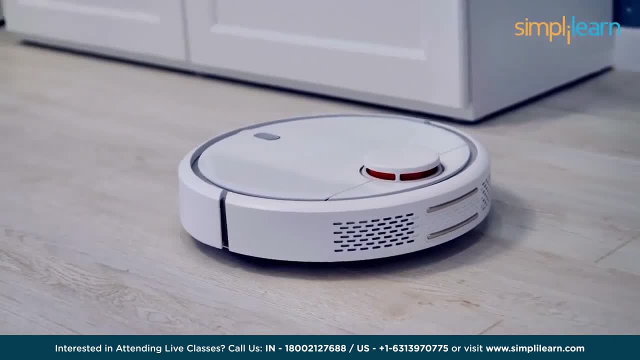 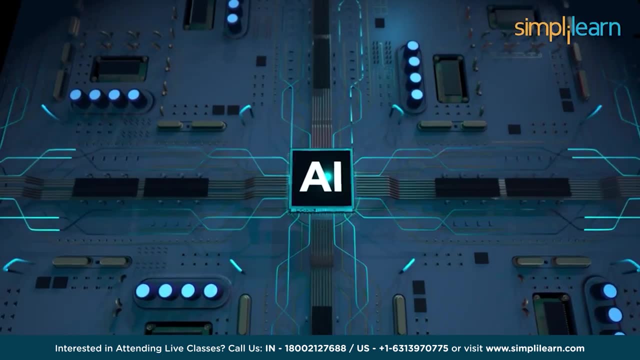 a myriad of AI tools help you achieve your targets. We are now at a time when artificial intelligence tends to do many jobs better and more efficiently, due to the lack of human error. It's not just content creation: AI can find use in a ton of scenarios. 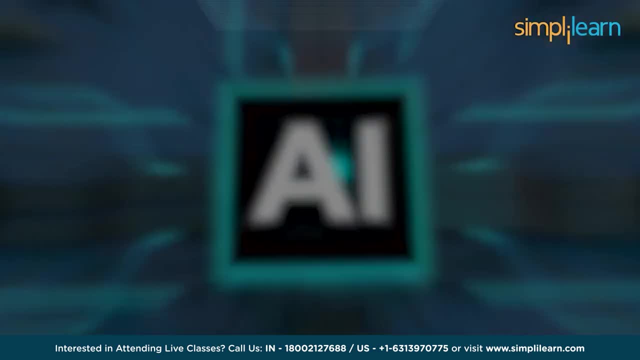 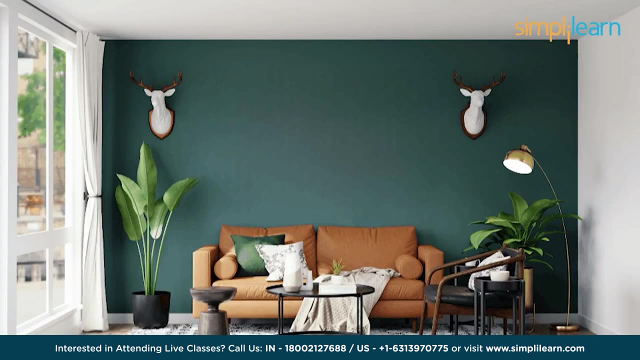 Let us go through some of the best AI tools available today that can boost your productivity. At number 10, you have Magic Eraser by Magic Studio. This tool allows you to remove unwanted images from your pictures. Using artificial intelligence, it can decipher. 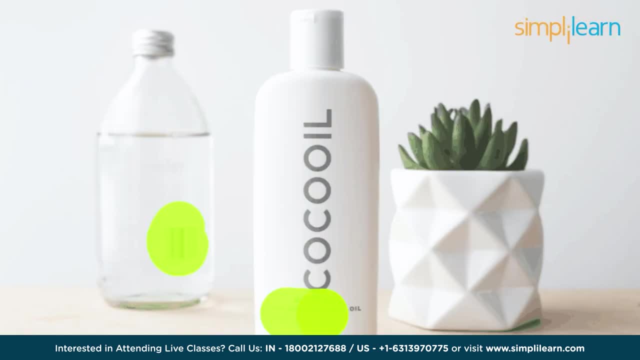 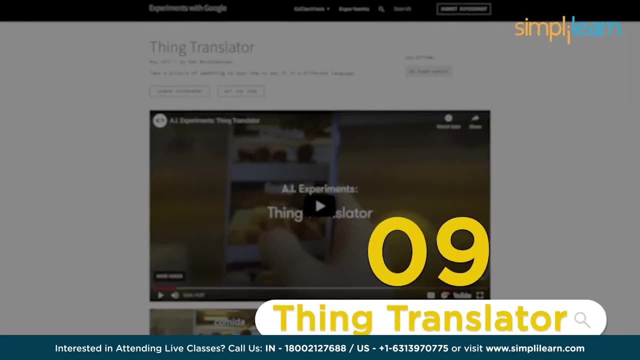 the backgrounds and remove unnecessary elements out of a picture, Be it unwanted birds on a landscape shots or branding on social media posts. Select the element to be removed using the eraser and let the tool work its magic. Next, at number 9,, we have the Thing Translator. 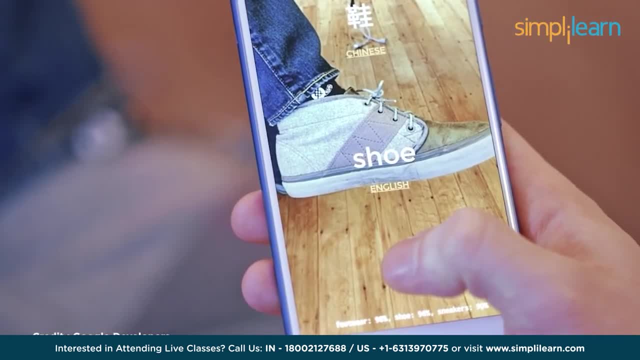 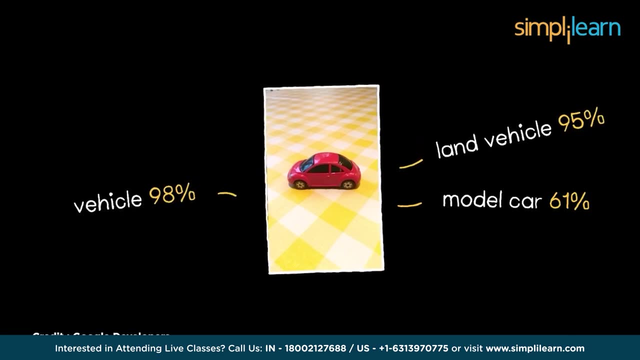 This tool allows users to point their camera at an object and hear the translation in a different language, Using the Cloud Vision API and the Translate API of Google. the translator serves as a godsend for foreign travelers or just people trying to learn new languages. 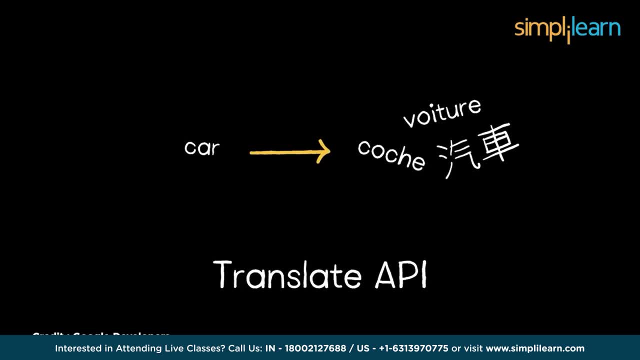 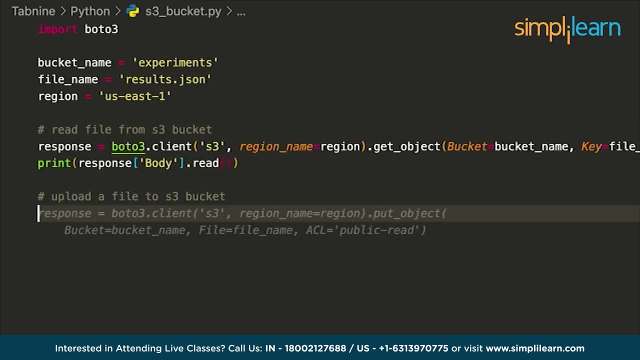 With both the Google APIs set to develop even more over time, expect the Thing Translator to become more helpful than ever. At number 8, we have Tab9.. Tab9 analyzes and recommends your next blocks of code based on the context and syntax. 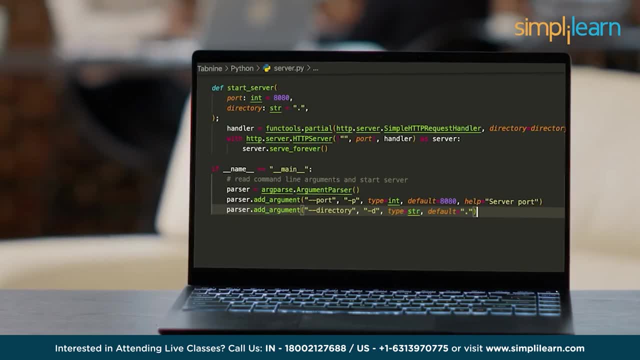 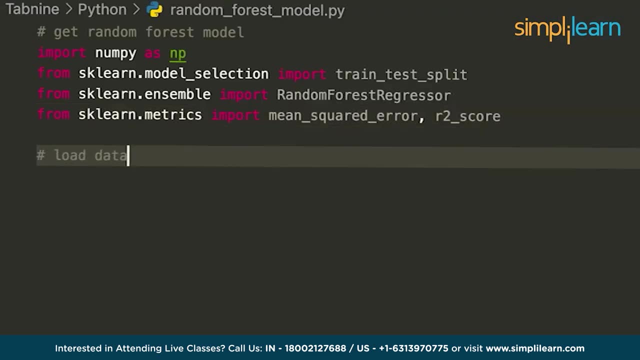 Get lengthy, accurate and creative code completions to become a more efficient developer. Tab9's AI completions may be executed on a developer's laptop, behind a firework or even on the cloud. It recommends code completions based on your 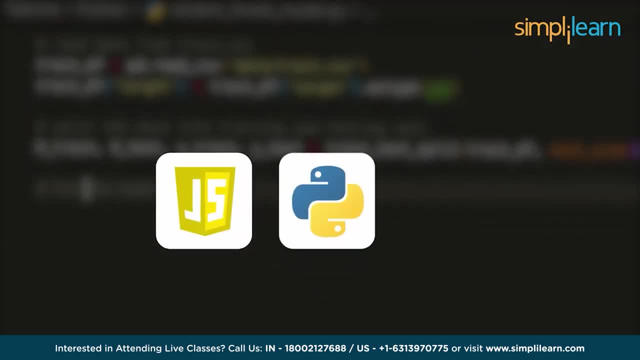 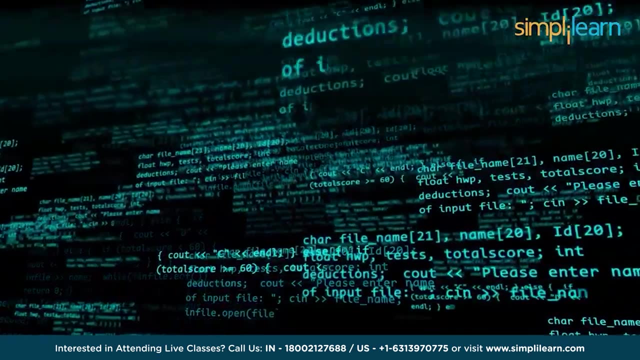 coding tendencies. It also supports integration with other languages such as JavaScript, Python and TypeScript, and even more niche languages such as Rust, Go and Bash. Irrespective of what your tech stack looks like, Tab9 will boost your speed. 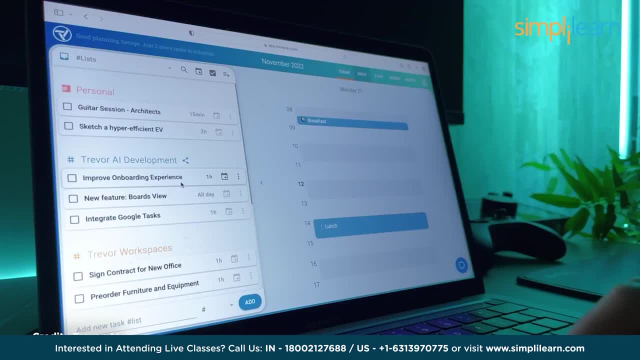 At number 7, we have Trevor AI. Trevor AI is a daily planning program that leverages intelligent time blocking to connect your list of activities and calendar. It supports integration and two-way sync with services like Google Calendar and Todoist, taking control of how you spend your time. 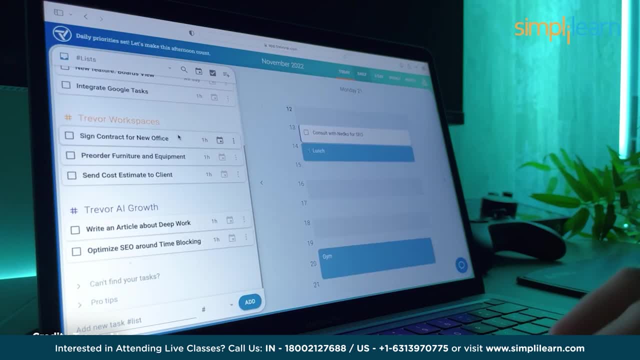 based on schedules and time frames. It helps plan your habits and work life in a streamlined approach to your day, using artificial intelligence. This helps you focus on the individual tasks rather than worrying about cramming your busy schedule into the entire day. At number 6,, we have Deep Nostalgia. 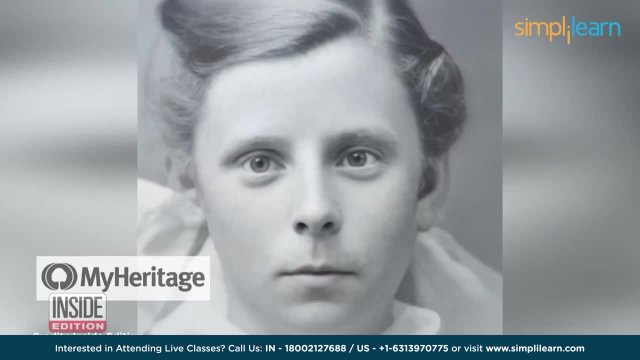 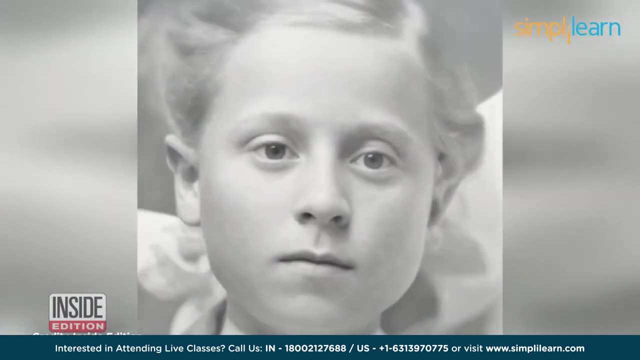 Deep Nostalgia is an online tool developed by a company called MyHeritage and can animate faces from old pictures. MyHeritage licensed this unique technology for animating photographs from DID, which is a firm specializing in video reconstruction using deep learning. 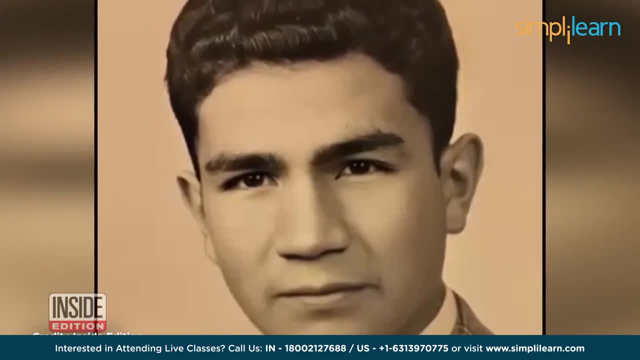 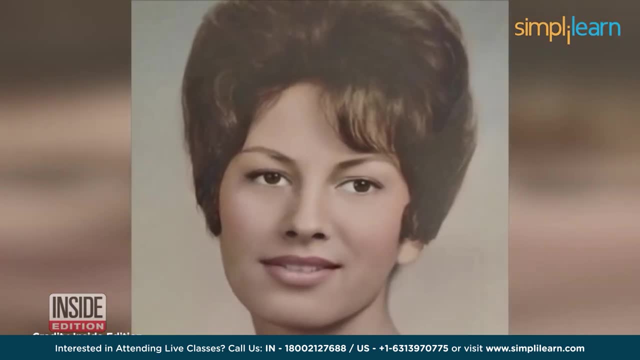 MyHeritage uses this technology to animate the faces in old images and generate quality, life-like video footage. The tool works equally well for black and white pictures and photographs taken in color, So, needless to say, the results are pretty astonishing and can be quite moving in many cases. 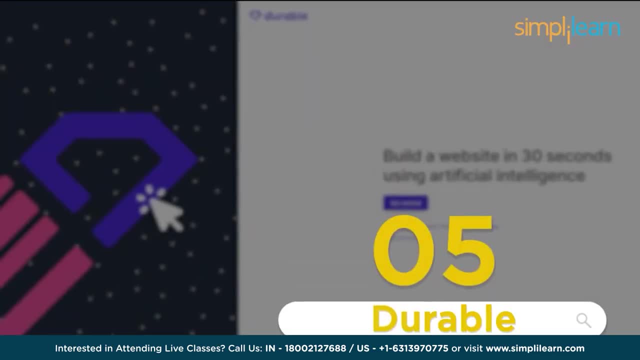 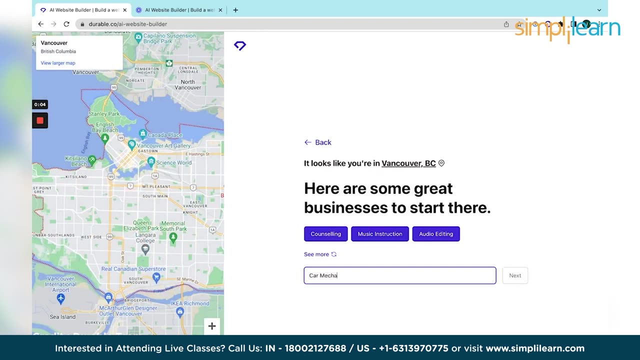 Number 5 on our list goes to Durable. Durable helps create sample websites in under 30 seconds for people starting a new business or who are generally not well versed in web development. Just choose the type of business you are running and the name of your company to get. 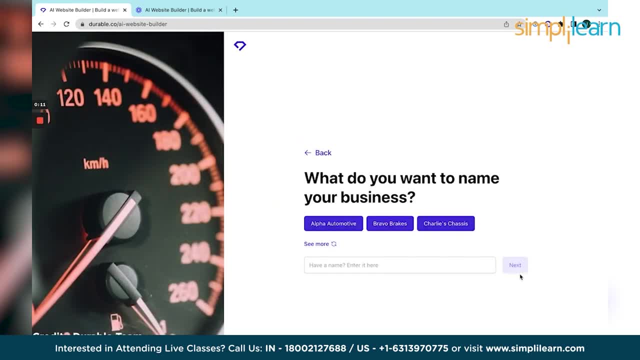 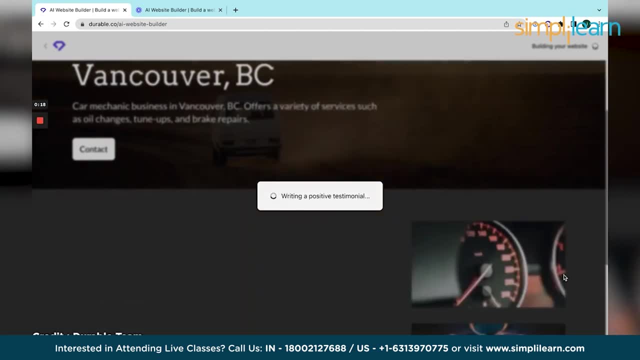 sample designs made immediately, From spaces assigned to customer reviews to buttons allotted for social media profiles. Durable ensures the websites match the latest trends in web development. You can restyle the colors and headings, or sign up to further customize the website based on your requirements. 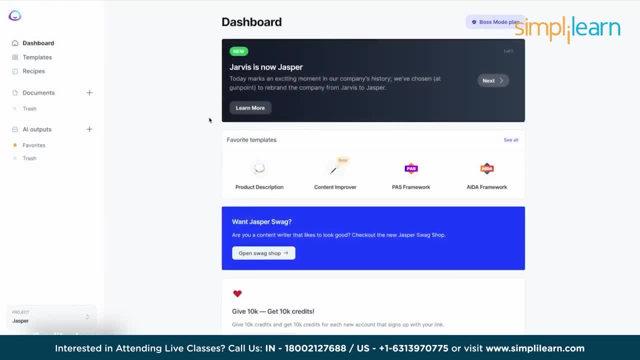 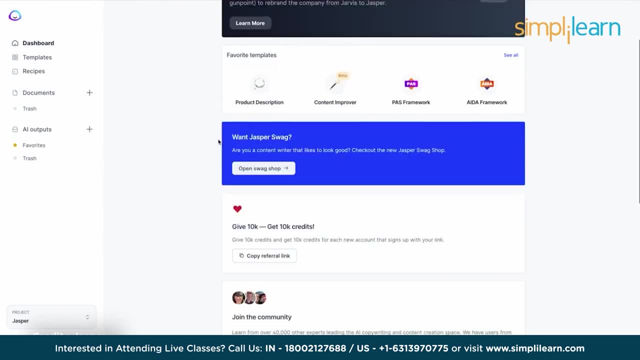 At number 4 we have Jasper. With the growth of AI, everything it's only a matter of time until AI is utilized to produce content for your blog, social networks, websites and other platforms. Jasper AI, formerly known as Jarvis, is a low-cost service that generates 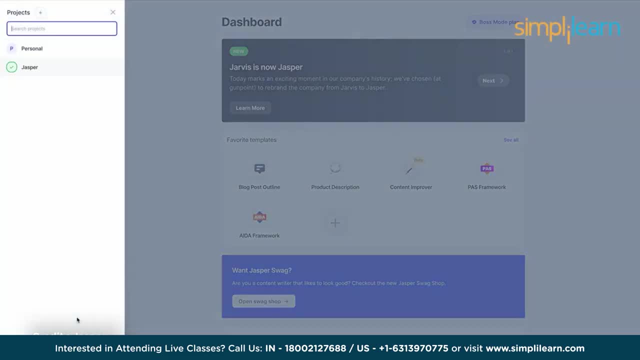 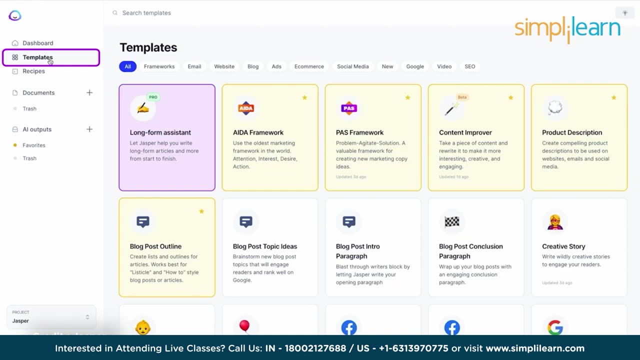 original material, such as blog entries, for you. It's simple enough for almost anyone to use. All you have to do is enter the URL information about what you want to address, and the AI will do the rest. providing over 50 templates, Jasper can handle a significant amount of. 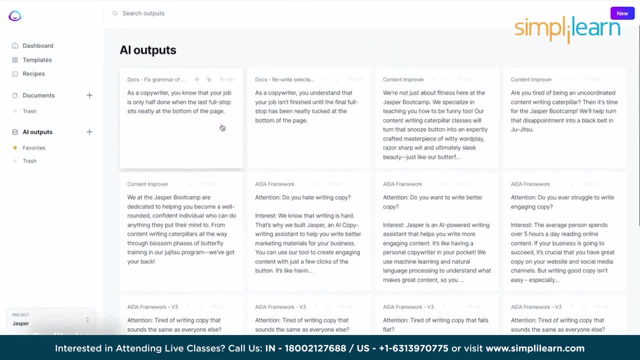 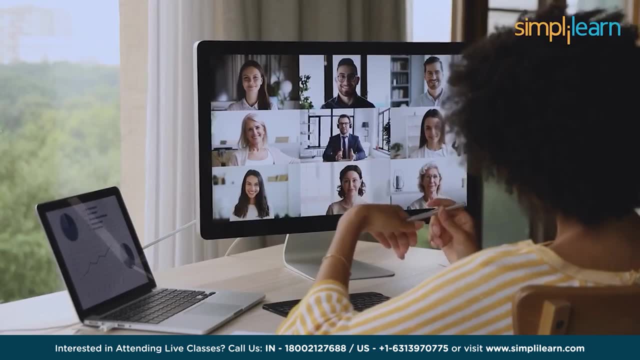 the heavy lifting. for topics that are often written about, The AI can provide a solid foundation of information to which you can subsequently add your own unique insight. Number 3 on our list goes to Tetra. With Tetra, you don't have to note down. 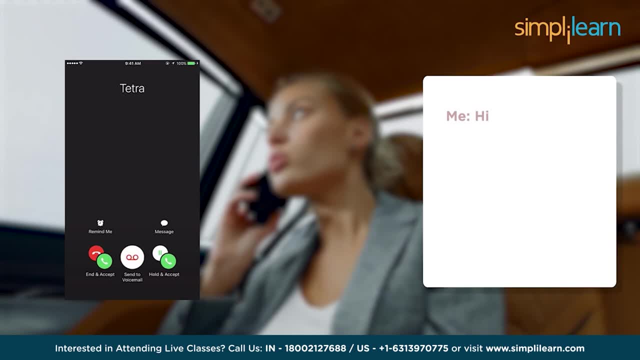 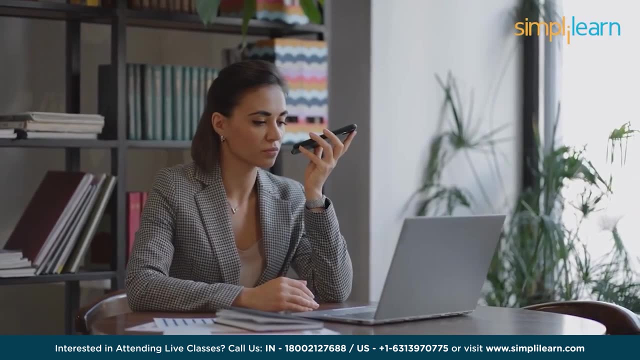 your minutes of meeting. every day, Tetra dials into your calls and essentially takes notes for you, allowing you to focus on the discussion now and remember all of it later. Touch recognition has yet to reach the level where it can function as a viable alternative. 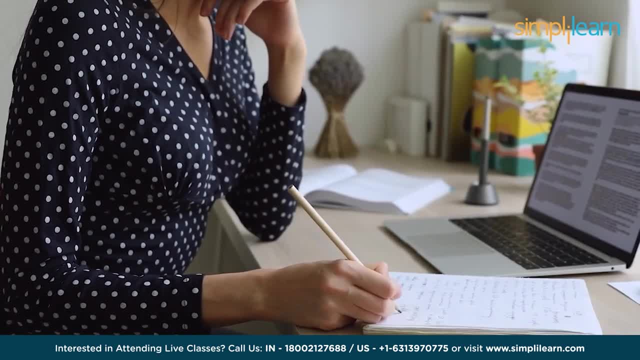 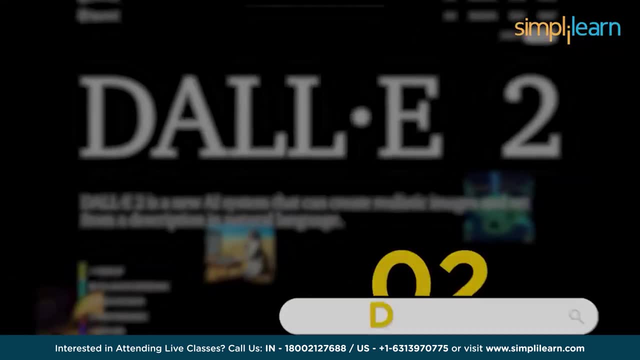 Tetra also has a notes viewer, with each audio byte synced with the notes. This level of detail allows you to focus on the meeting's discussion without making individual notes throughout the call. At number 2, we have the Dolly 2.. 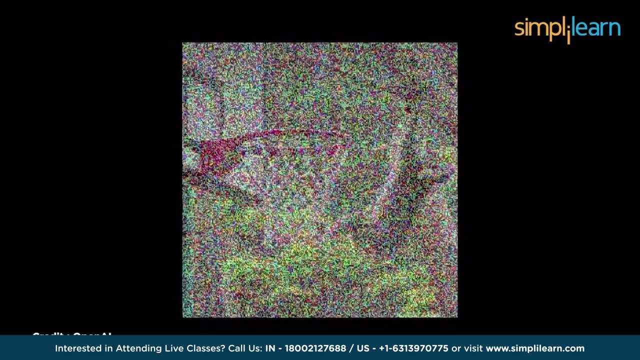 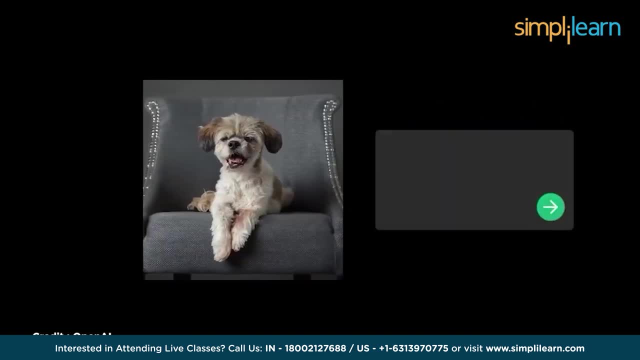 The latest groundbreaking text-to-picture generator from OpenAI is called Dolly 2.. It enables users to produce visuals in response to text cues. Users can use this generator to transform their imaginative thoughts into life-like graphics. If you scroll through Twitter and look for the hashtag. 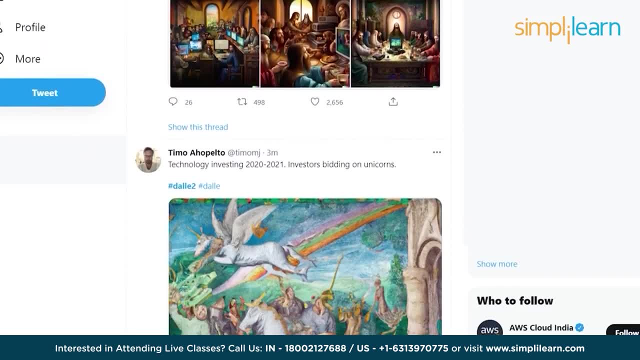 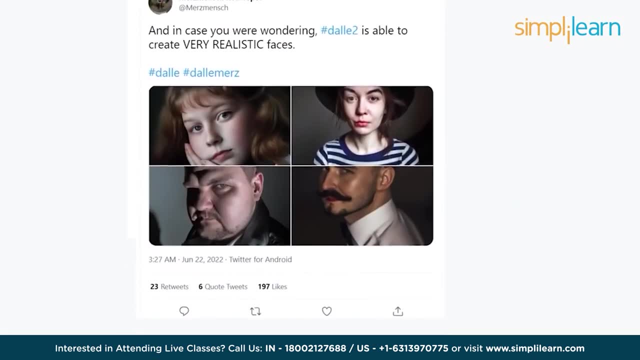 Dolly 2, you will be greeted with many images and artworks shared by many people, based on different topics. From Victorian era-style pictures of aliens to just plain portrait-style images, Dolly 2 has all its bases covered. regarding variety, The AI is taught. 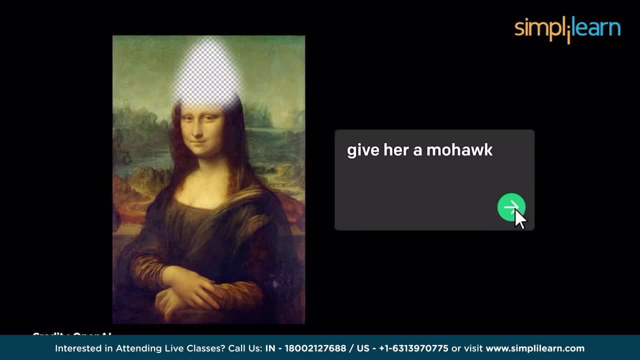 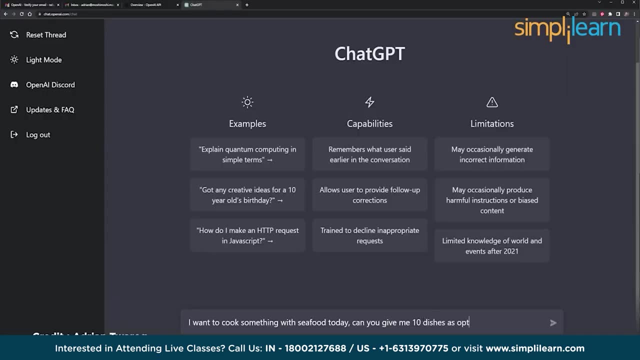 via deep learning, how to make text-to-image associations, which the model later uses to recreate the relevant images. Finally, we have ChatGPT at number 1.. OpenAI has unveiled ChatGPT, a powerful new chatbot that uses an improved version. 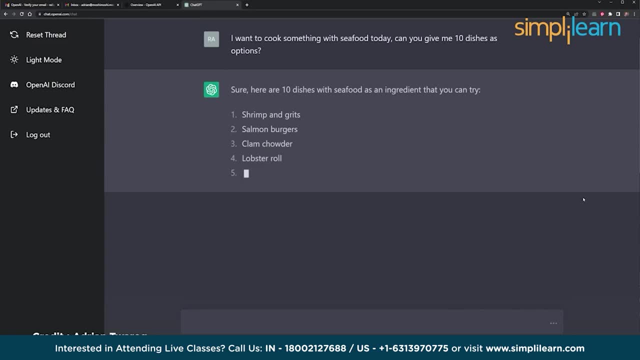 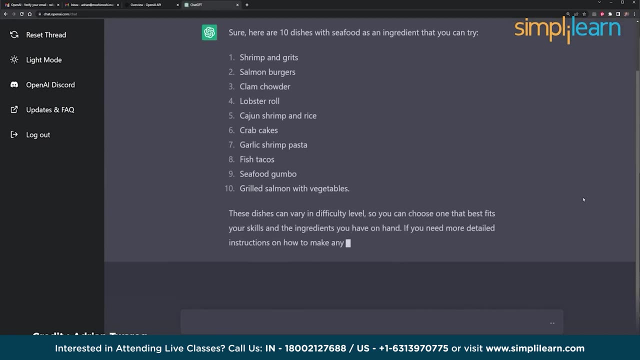 of its AI technology. to converse in plain English: While GPT has existed for a while, this model has reached a critical point. It is beneficial for a broad range of activities, from developing software to generating company ideas, to composing a wedding toast While prior. 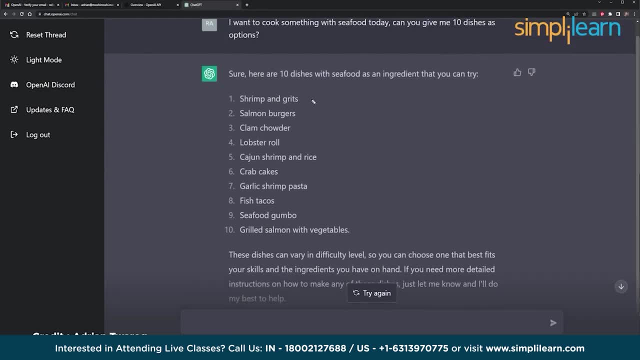 iterations of the program could potentially execute these tasks. the output quality was far worse than that of a typical person. Since its debut, Twitter has been bombarded with people using it for unusual and bizarre purposes, such as creating weight-loss strategies and children's novels, and 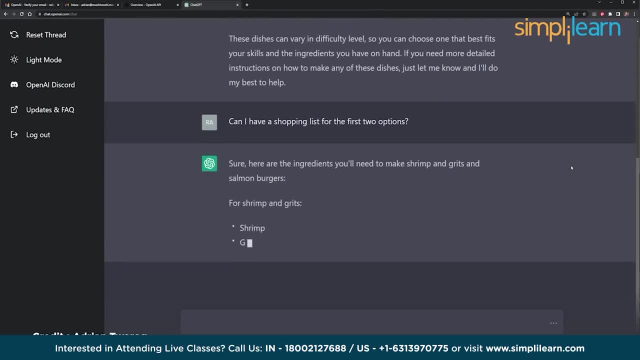 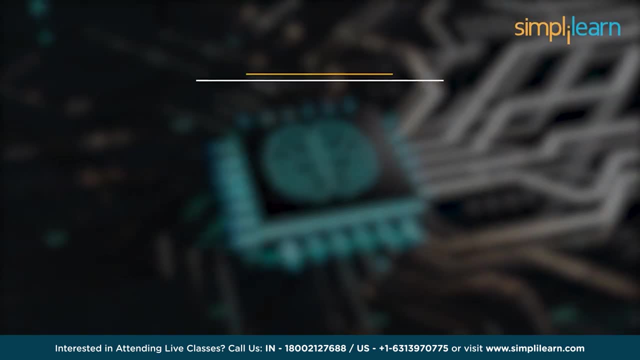 providing instructions on retrieving a peanut butter sandwich from a VCR. It seems ChatGPT will serve as an important monument for artificial intelligence to be welcomed in the consumer sphere. So that wraps up our video on the top 10 AI tools for 2023.. 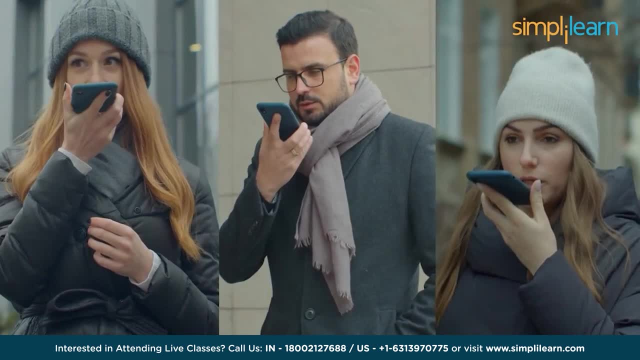 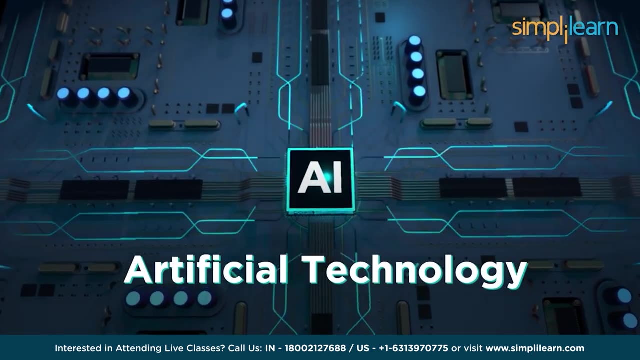 Ever wondered how Google Maps can provide the fastest route almost instantly? Have you ever considered the speed and accuracy of virtual bots like Google Assistant or Siri? All of them are powered by artificial technology- AI for short. Riding on the data science hype train, the global AI. 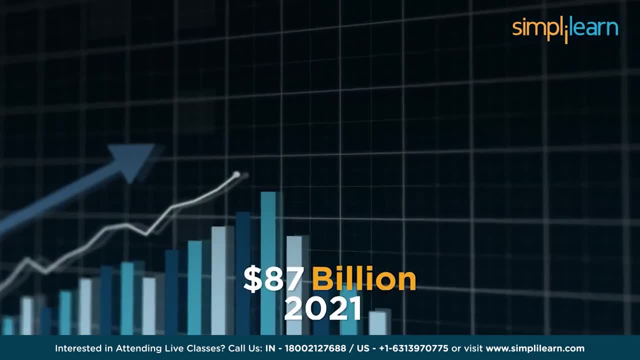 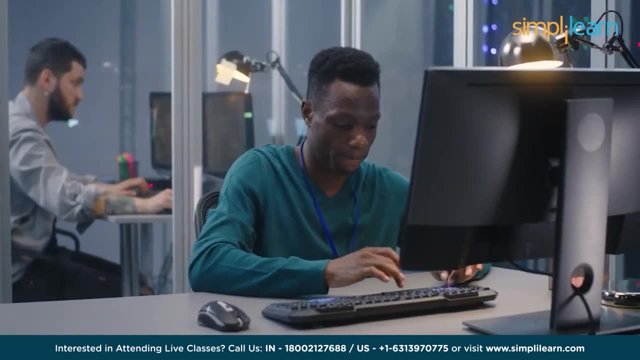 market is projected to go from around $87 billion in 2021 to nearly $1,600 billion by 2030.. Artificial intelligence has impacted almost all sectors of the IT domain, but its significance in the robotics industry is unmatched. Even Tesla has. 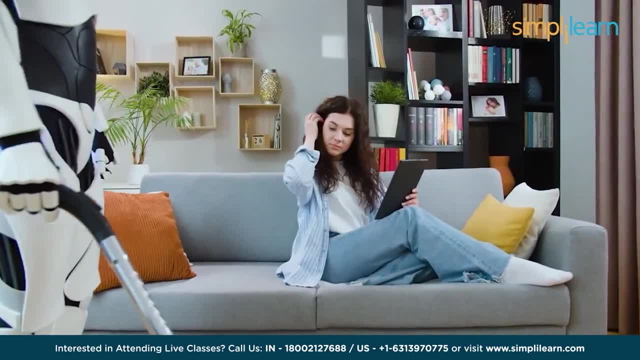 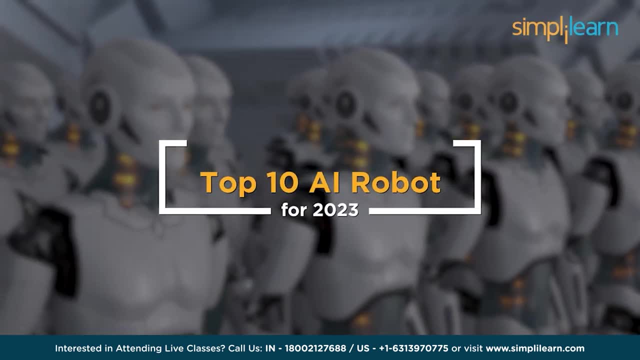 announced a new humanoid robot named Optimus, recently built to perform daily activities and help in Tesla factories. In today's video, let's go through some of the most advanced AI-based robots, paving the way for a faster and smarter future in 2023.. 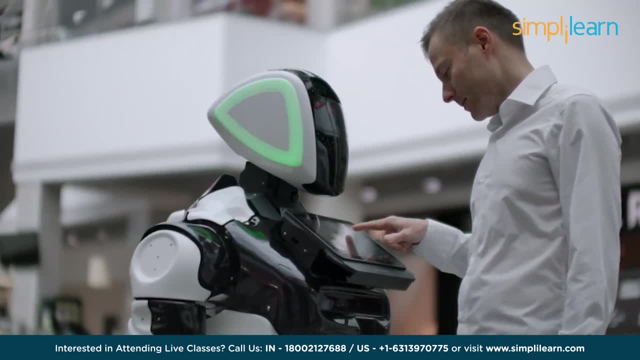 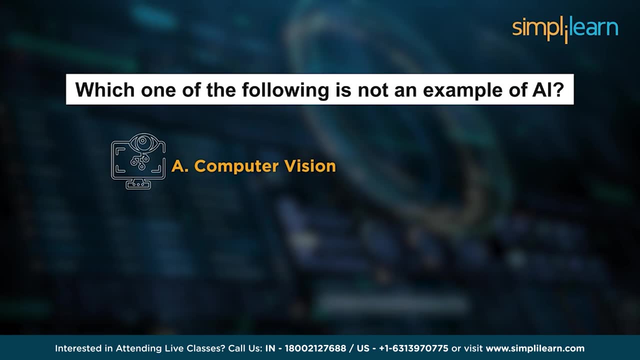 Before we start, here's a question for the AI enthusiasts watching this video. Which one of the following is not an example of AI? Is it A- Computer vision, Is it B- Web design, Is it C- Voice recognition Or D- Robotics? 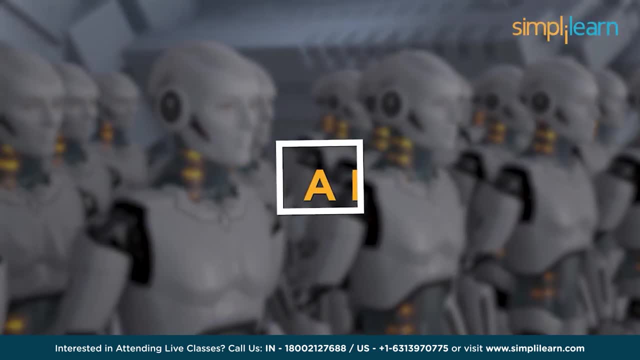 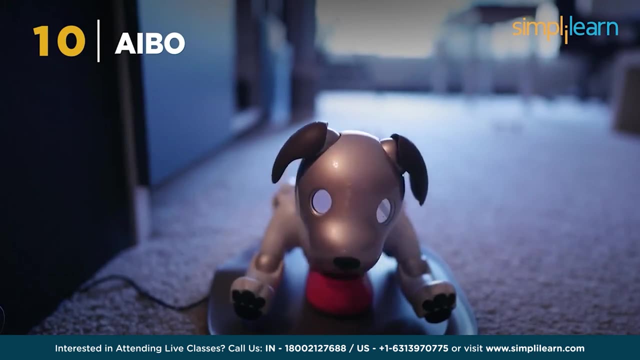 Please leave your answers in the comments below, And that's our cue to get started with the top 10 AI robots for 2023.. Number 10 on our list is AIBO. AIBO is a charming little robot dog created by Sony. This robot was 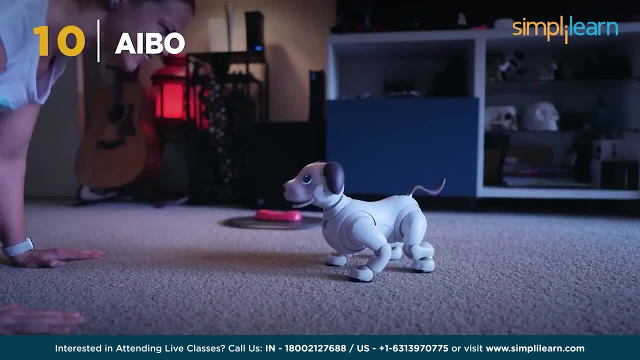 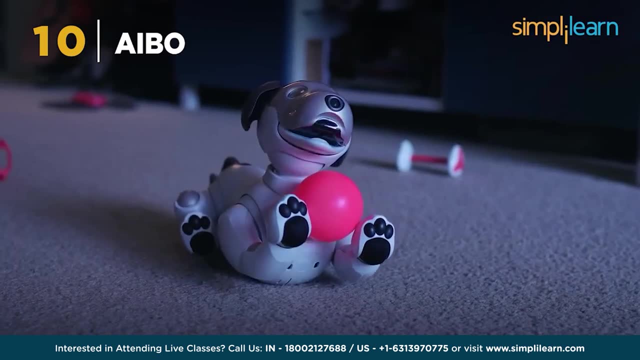 retired nearly a decade ago but has been brought back with even greater human operation capabilities. This artificial puppy responds to words of praise or head scratches, can learn tricks and seeks out owners. A very important feature of AIBO is that it has an app that owners. 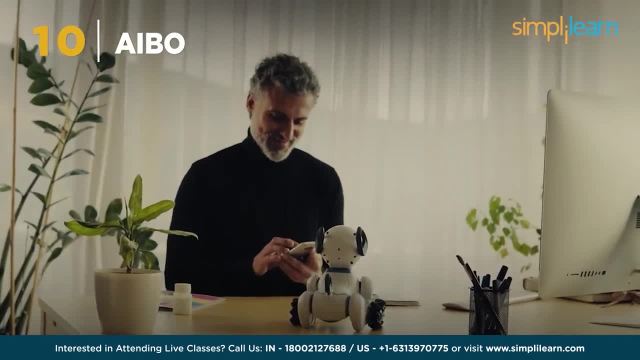 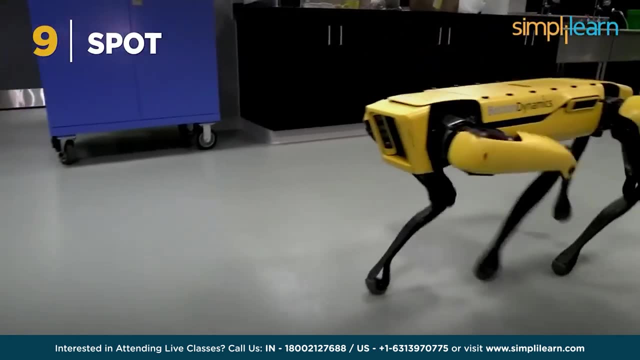 can use to alter system settings or add new tricks and store memories by connecting to the cloud AI system. Next, on number 9,, we have Spot Former. Spot robot, also known as Spot Mini, is really a four-legged robot produced by Boston Dynamics. 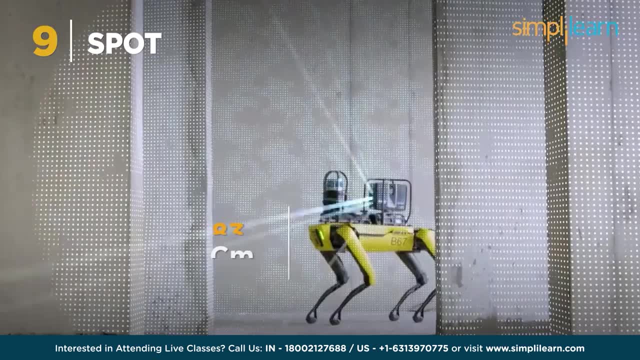 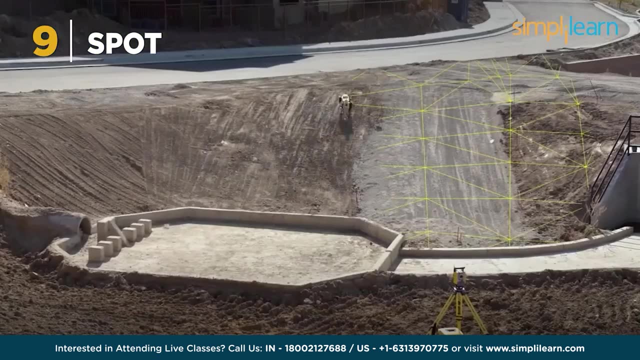 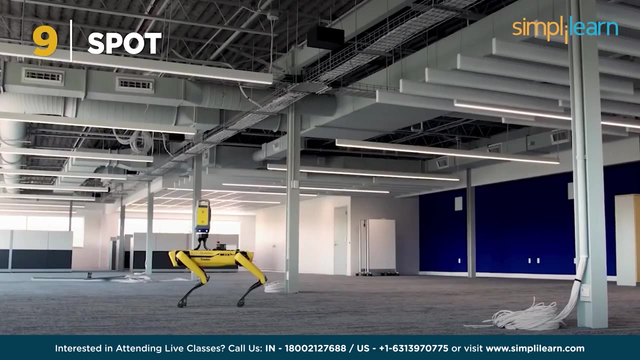 an American robotics company. Spot is 83 cm tall and weighs only 25 kg. Spot can perform various tasks, including walking stairs and navigating rugged terrain. It's small enough to be used indoors as well. Spot's unique selling point is that it can go places other. 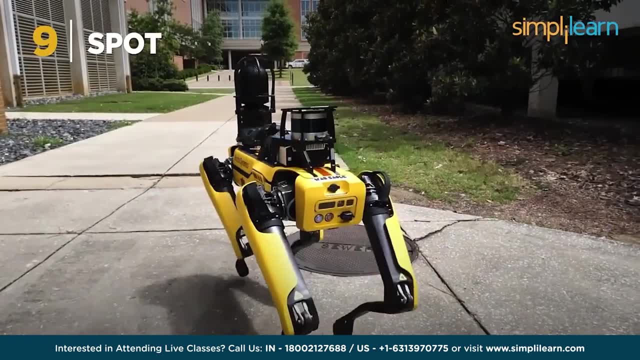 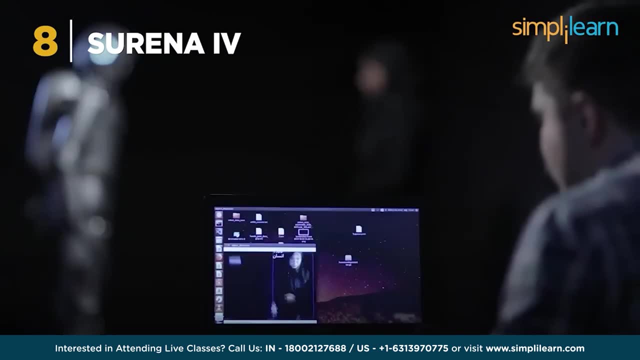 wheeled robots cannot all while carrying cargos of up to 14 kg of examination gear. On number 8, we have Surina 4.. Surina 4 is a humanoid robot created by scientists at the University of Tehran, The fourth generation of Iran's 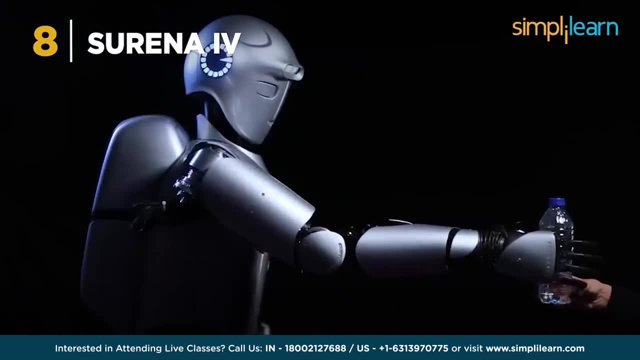 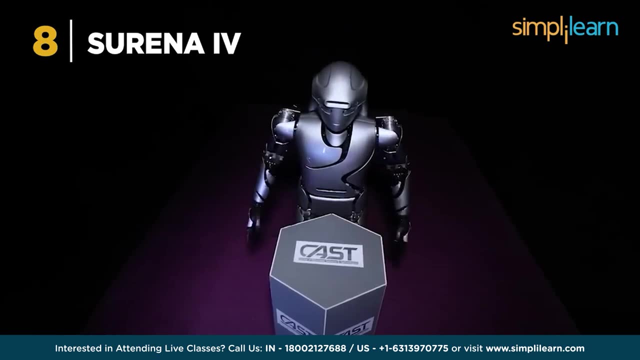 Surina robot can imitate a human position, grip a water bottle and write its name on a whiteboard. The robot, which took four years to develop, can track objects properly and its new hands permit it to manipulate various objects from delicate 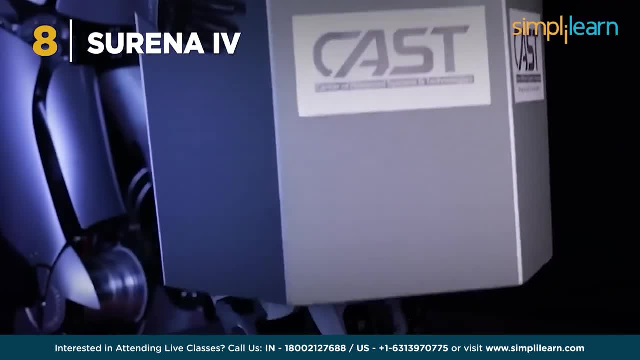 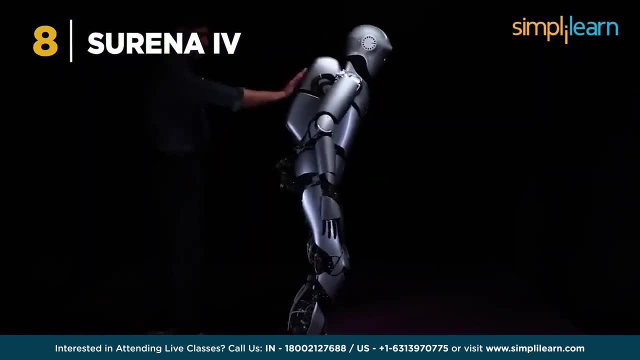 gestures to using power equipment. However, the improvements are not only internal. Surina 4's exterior has been updated with new plastic panels, making the robot appear sleek and just slightly threatening. Next we have Aquanaut at number 7.. 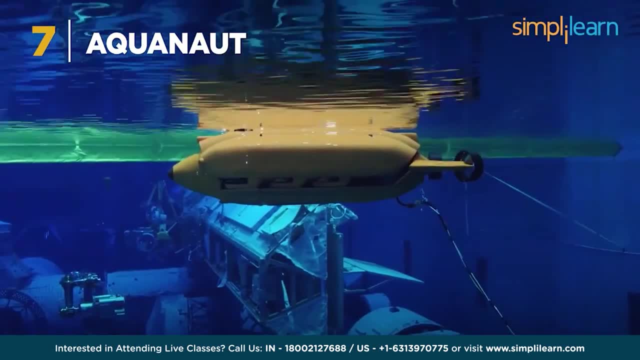 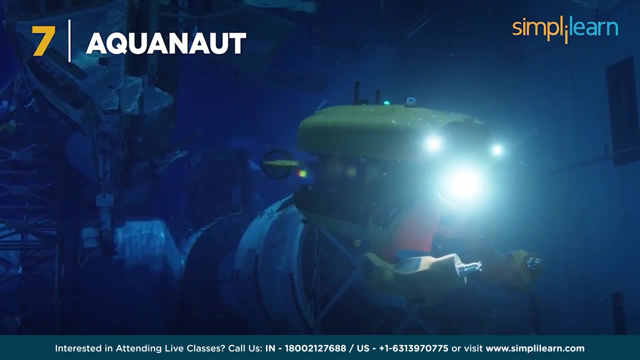 Aquanaut is a shape-shifting underwater robot developed by Houston Mechatronics Inc in Texas. The Aquanaut's design allows it to morph from a sleek and small submarine to a slightly humanoid form with two extended arms, allowing it to perform various jobs underwater. 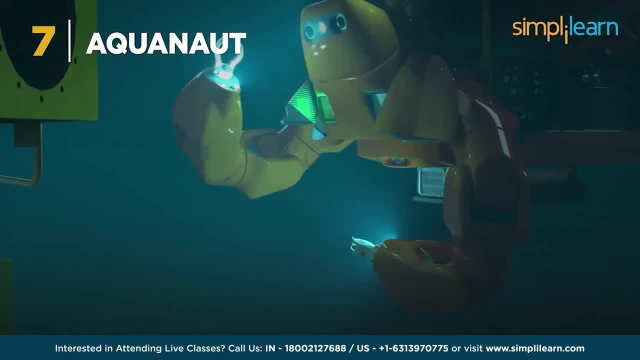 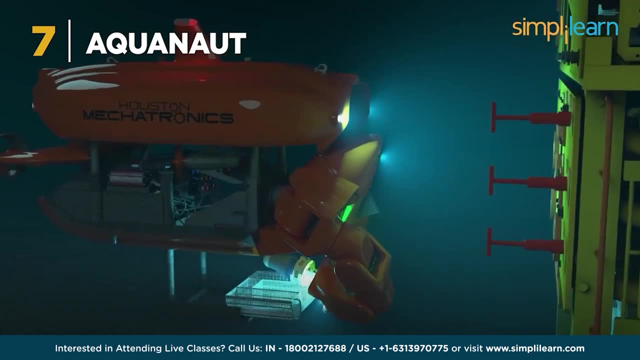 Aquanaut was created to address a long-standing problem in offshore oil and gas, which was the cause of maintaining offshore sites. With no similar device on the market, the Aquanaut might have a significant advantage because it can accomplish this task without the inconvenience of 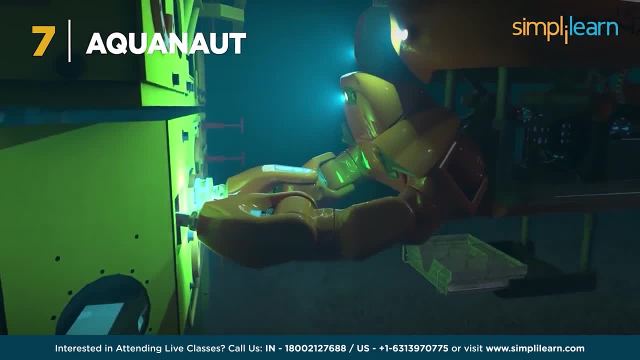 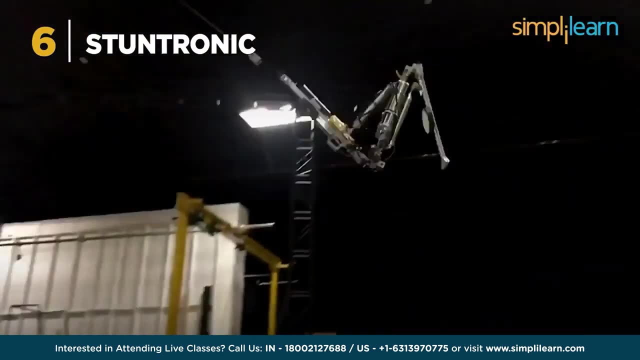 being tied to a support vehicle and with only minimal oversight from a human operator. At number 6, we have Stuntronic. Stuntronics are simple animatronic stunt doubles. Each Stuntronic employs onboard sensing to perform numerous flips. 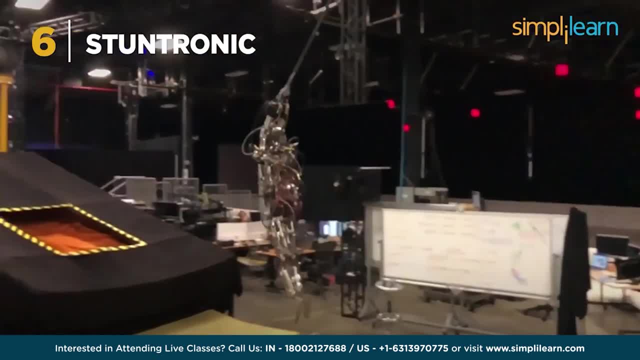 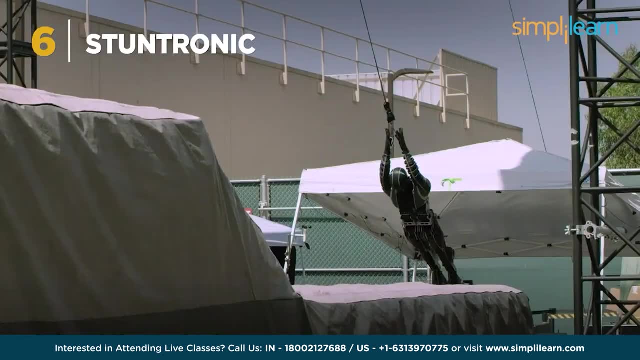 twists and postures with repeatability and precision, combining modern robotic technology with the investigation of untethered dynamic movement. The initiative to investigate stunt double animatronics began with an attempt to manage the landing of a figure hurled from a window. 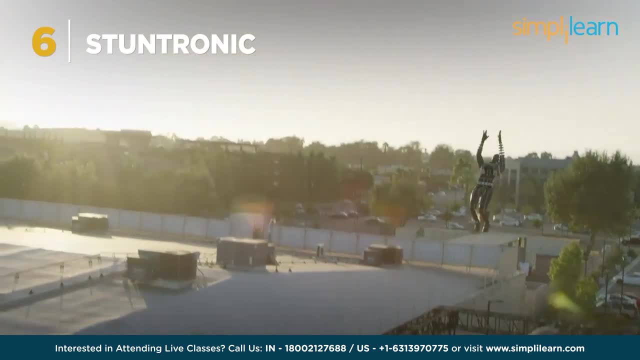 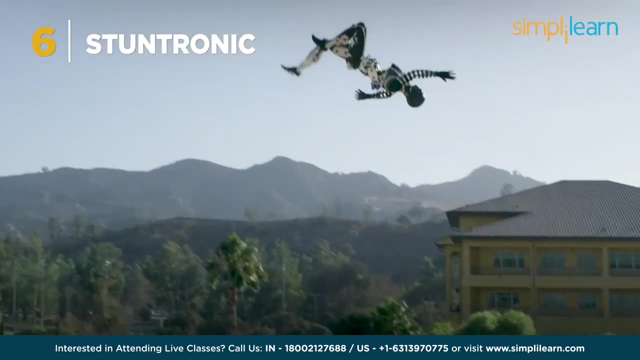 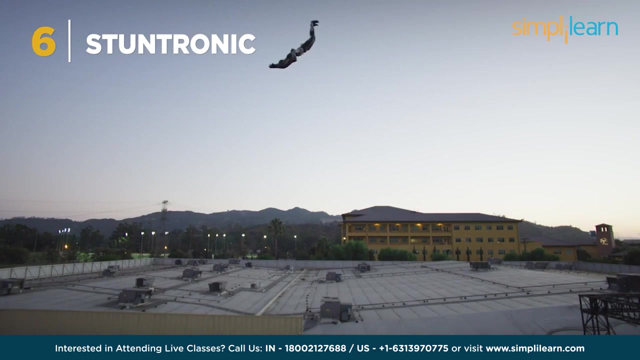 by Walt Disney Studios. Meanwhile, Disney research experts worked hard to utilize angular momentum conservation to enable fine airborne motion control. A union of the two projects allowed the team to construct the Stuntronics platform, which is ready to bring a wide range of dynamic characters to life. 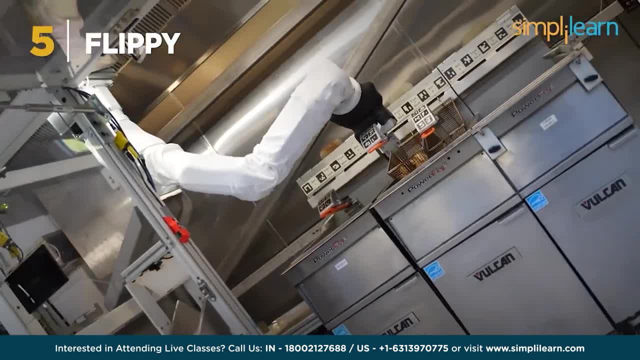 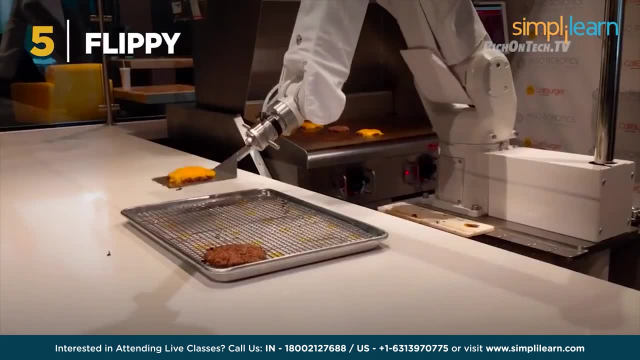 At number 5, we have Flippy. Flippy is an autonomous robotic kitchen assistant that can assist chefs in preparing freshly cooked burgers and fried foods such as crispy chicken tenders and tater tots, For example, while cooking at the grill. 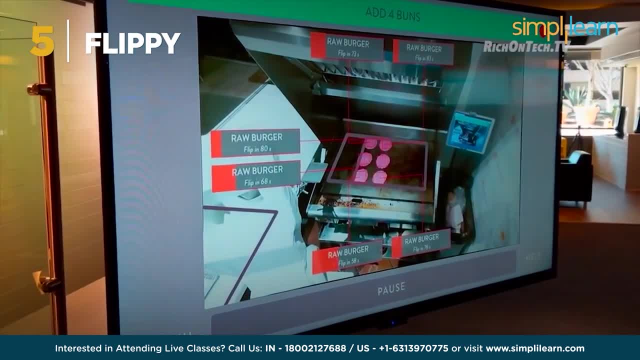 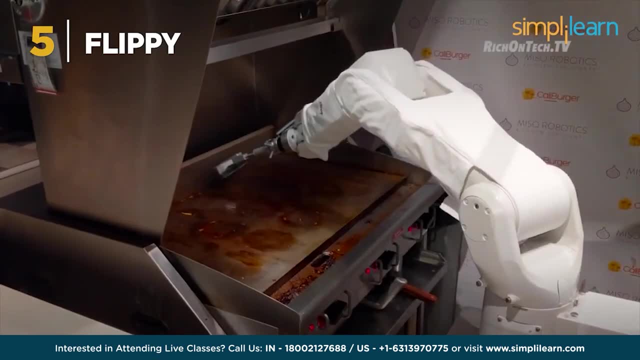 it can automatically detect when the raw burger patties are placed, monitor each patty in real time and switch between spatulas for raw and cooked meat. Flippy's brain is powered by cloud connected artificial intelligence, allowing it to learn from its environment. 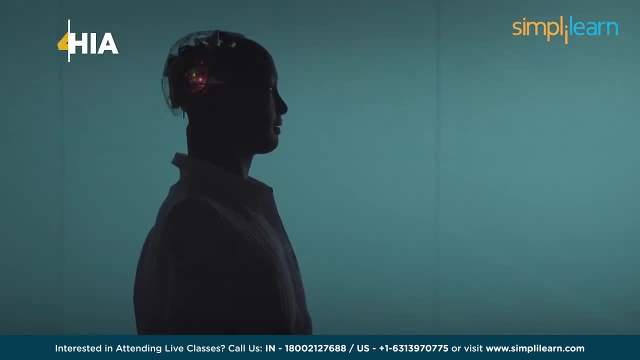 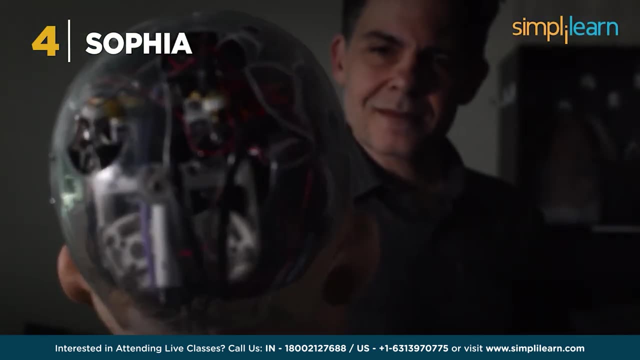 and acquire new abilities over time. Next, we have Sophia at number 4.. Sophia is regarded to be the most intelligent humanoid robot. She made her debut in 2016,, and her interaction with humans was the most extraordinary thing you'd ever witness in a machine. 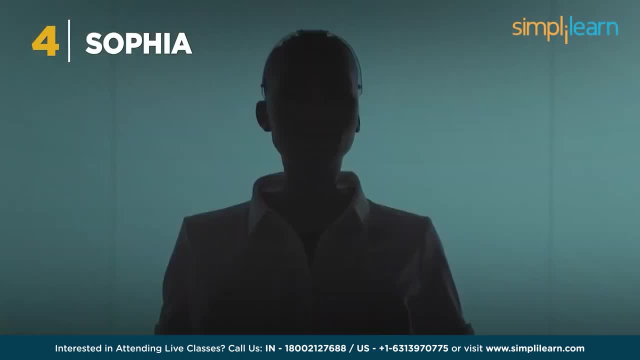 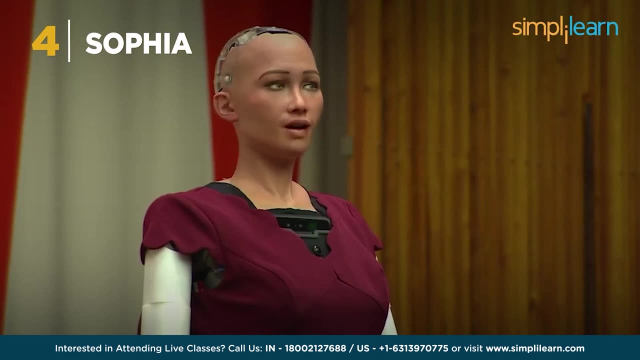 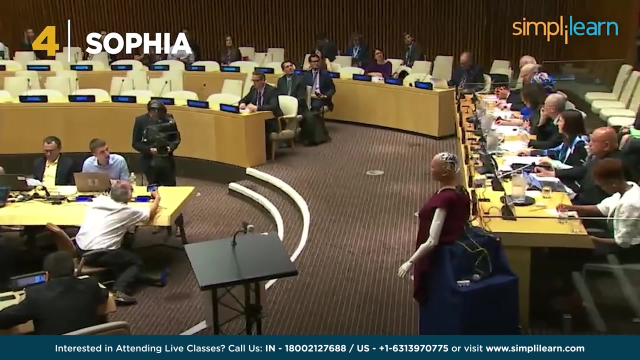 Hanson Robotics, based in Hong Kong, developed her to integrate as an elderly companion in healthcare facilities or crowd management at events. Sophia is the world's first robot citizen and the UN Development Program's first robot innovation ambassador. Sophia has integrated neural network models and artificial intelligence. 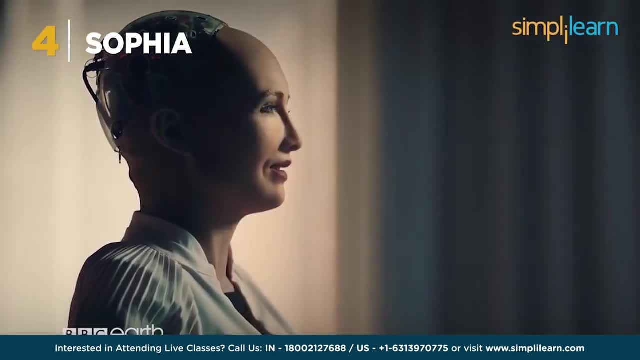 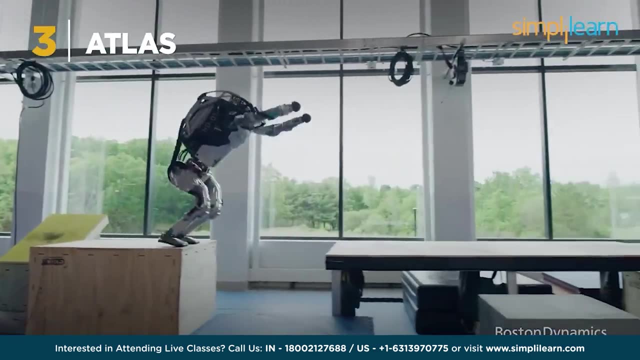 to recognize human faces and make up with their gestures and emotions. At number 3, we have Atlas. Atlas is a humanoid robot created by Boston Dynamics and renounced for its unmatched ability to jump over obstacles, do backflips and dance. 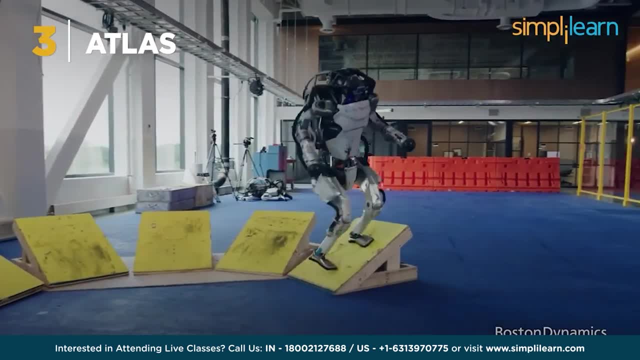 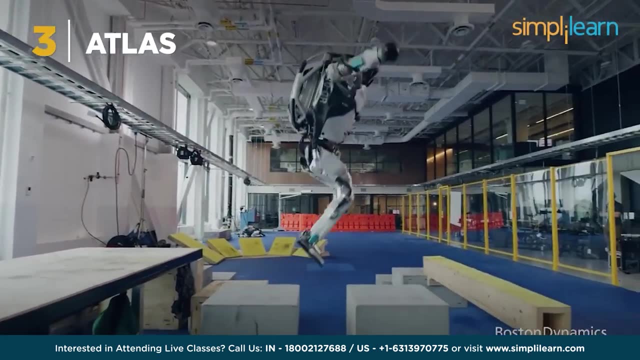 Atlas completes a parkour track in one of the company's most recent videos. Its evolution has been nothing short of remarkable. Aside from the spectacular acrobatics, it demonstrates some interesting foundational abilities, such as awkwardly shifting its equilibrium after landing. Atlas' behavior has also been 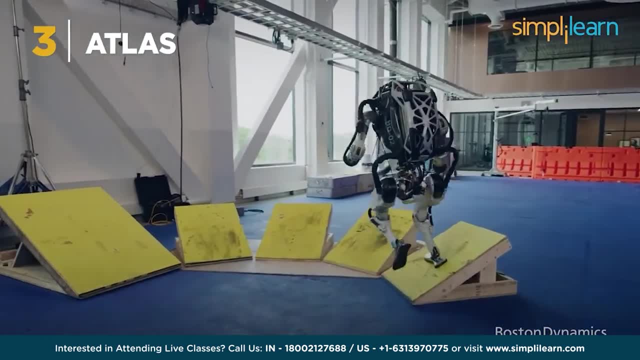 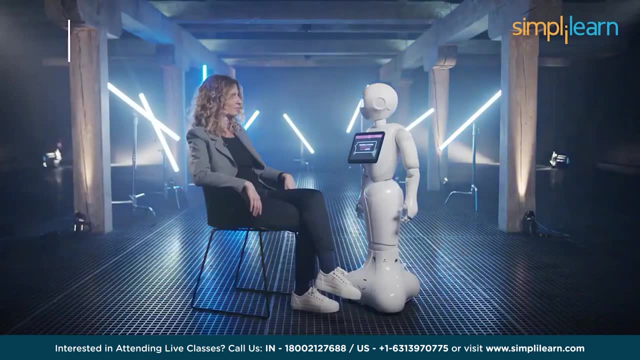 extended by providing it with a selection of template behaviors, such as leaping and vaulting, and allowing it to adapt those behaviors to the new scenarios it finds. Next we have Pepper. in the second position. The Pepper robot is among business's most sophisticatedly commercially available. 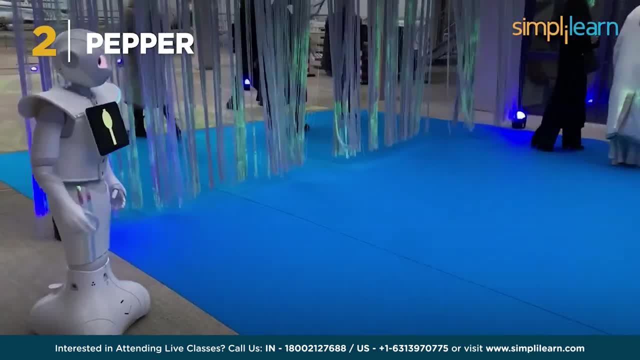 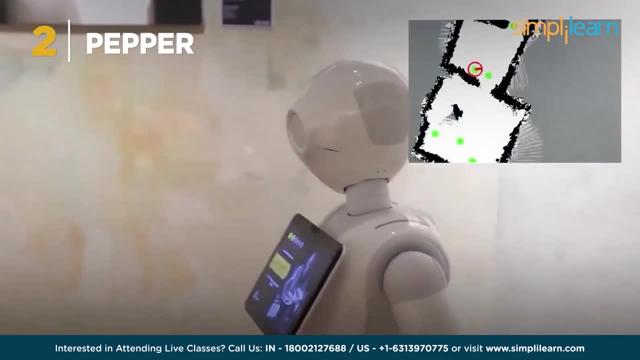 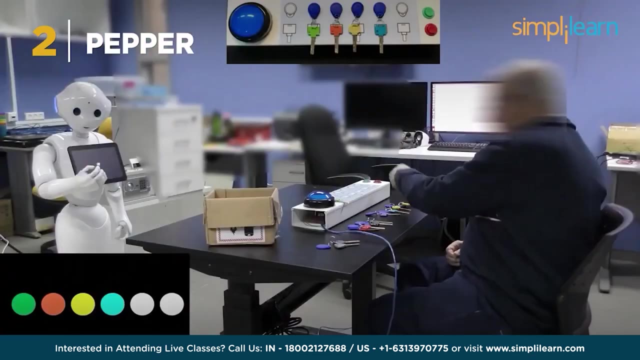 social robots today. Softbank Robotics designed it to be friendly and engaging, as well as to put people at ease, and is equally at home with infants as it is with adults. Pepper can hold conversations and incorporate knowledge from those talks into his words. It may be trained to recognize items. 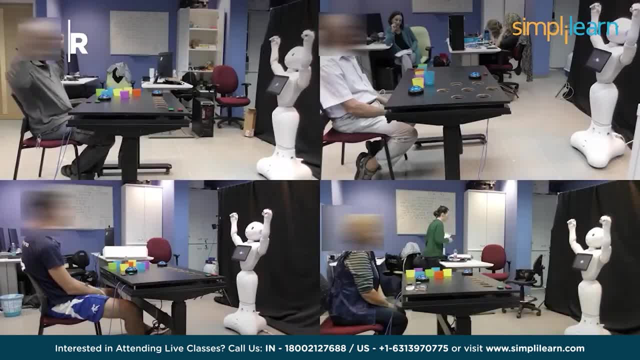 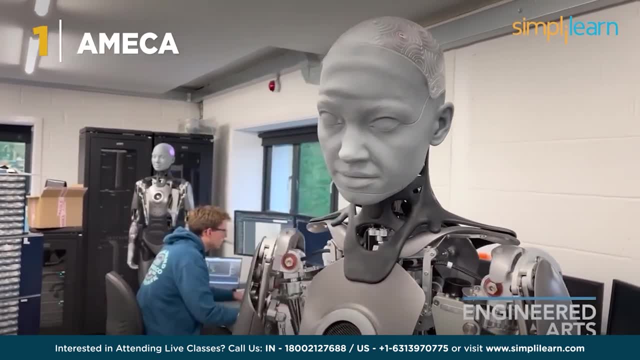 pick them out in a room and make decisions to enlighten or amuse them. Finally, at number one, we have Amica. Engineered Arts describes Amica as the world's most advanced human-shaped robot, reflecting the cutting edge of human robotics technology. 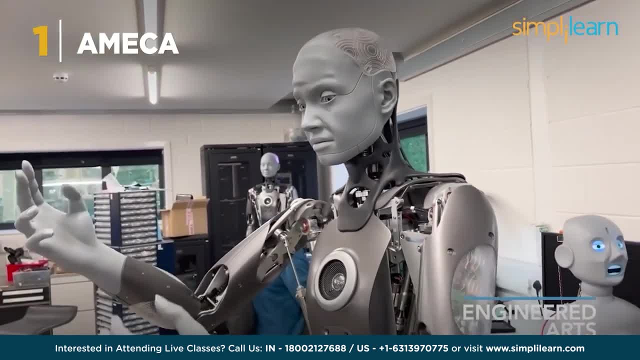 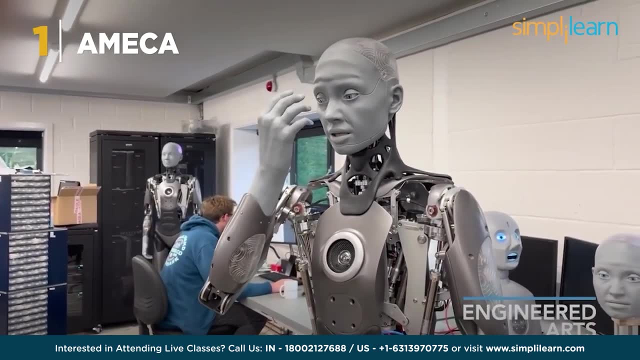 The robot can mimic expressions fairly well and responds to all questions articulately. Engineered Arts' Amica hardware is based on the research into human and robotics and is built on their proprietary Mesmer technology. Amica's articulation of artificial limbs, ligaments, motors. 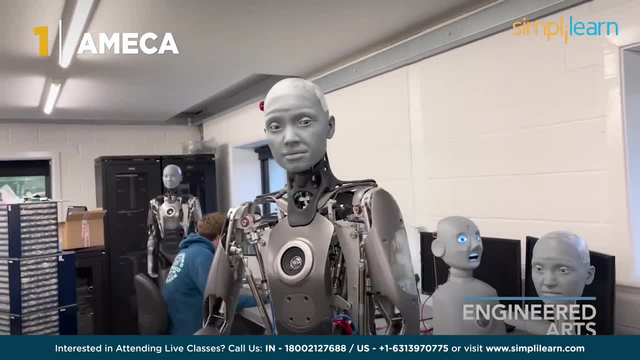 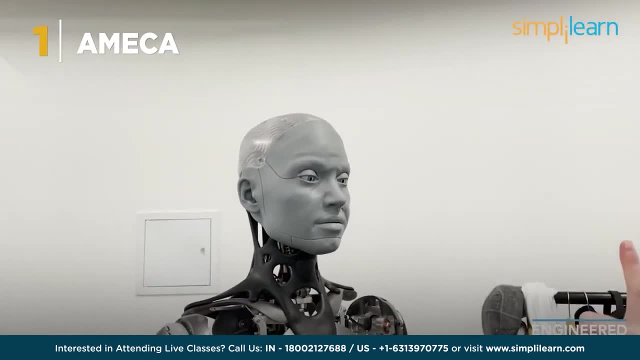 and sensor arrays are made with cutting edge technology. As shown in movies, the rise of AI usually results in chaos. Amica's developers, on the other hand, argue that the scientific breakthrough will be used for a different purpose, claiming that Amica will serve as a future face. 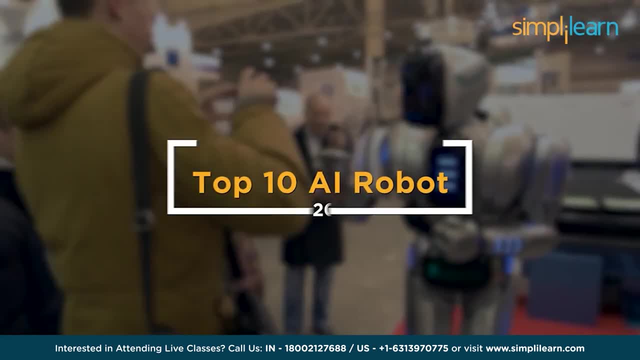 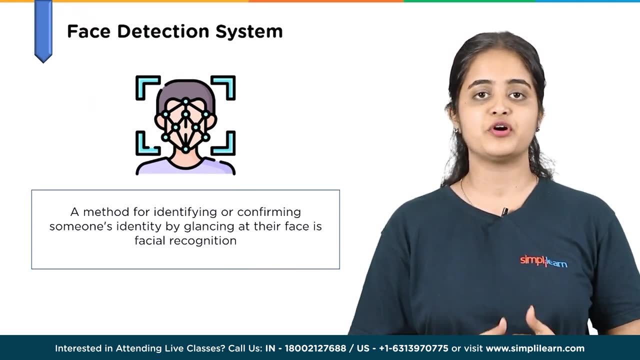 of robots. So that wraps up the top 10 AI-powered robots for 2023.. Face Detection System: It is a form of biometric recognition. a method for identifying or confirming someone's identity by glancing at their face is called facial recognition. 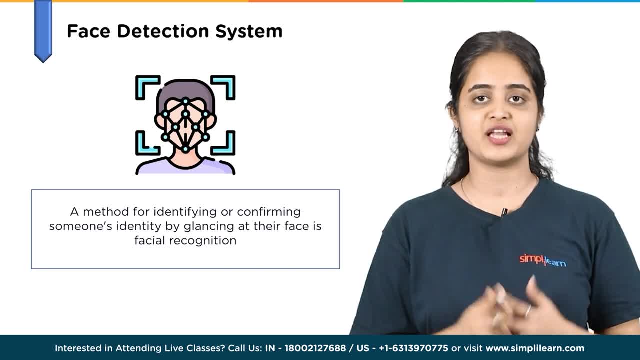 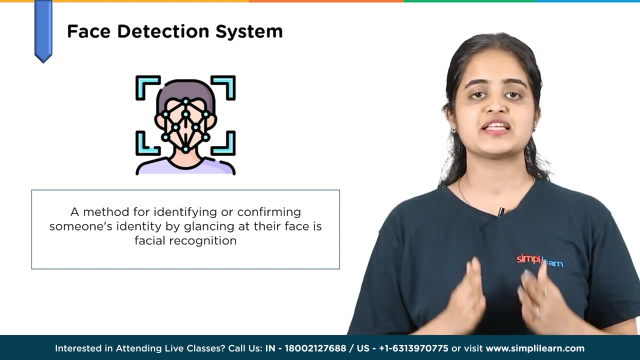 People can be identified by securing a match on facial ID. using this technique, Real-time visuals, videos and photos can be the sources to run face detection. This technology is mostly employed in security and law enforcement. OpenCV is the best technology to create it. 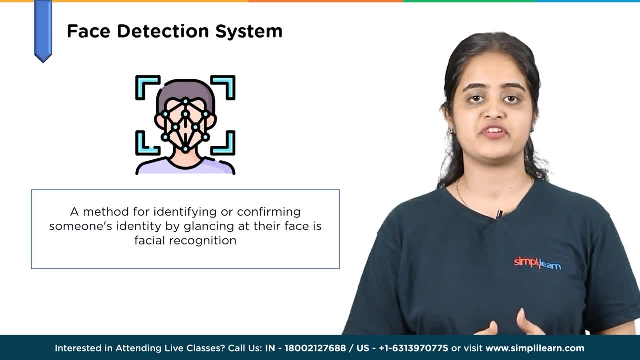 A Python package called OpenCV is made specifically to address computer vision jobs. Computer vision is a process used in the processing of images by computers. It is concerned with the in-depth comprehension of digital photos or films. It is necessary to automate operations that can be performed. 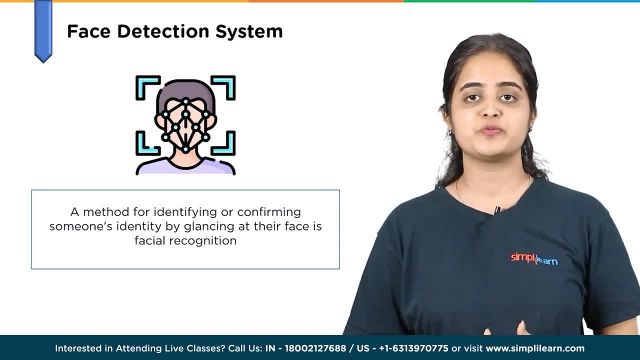 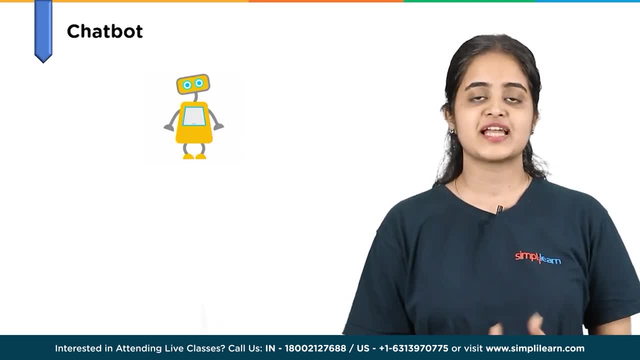 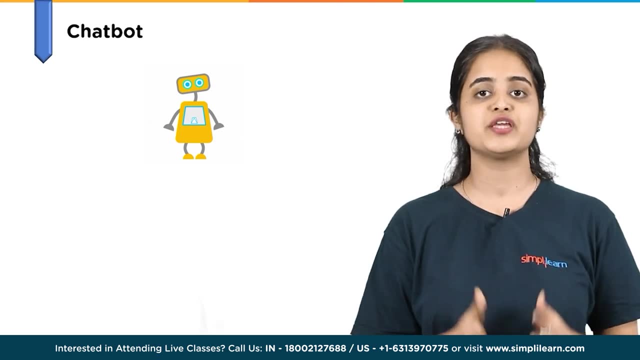 by human visual systems. Therefore, a computer should be able to identify items like a statue or a lamp post, or even the face of a human being. Second one is chatbot. It is the best idea if you have chosen chatbot as your project topic. 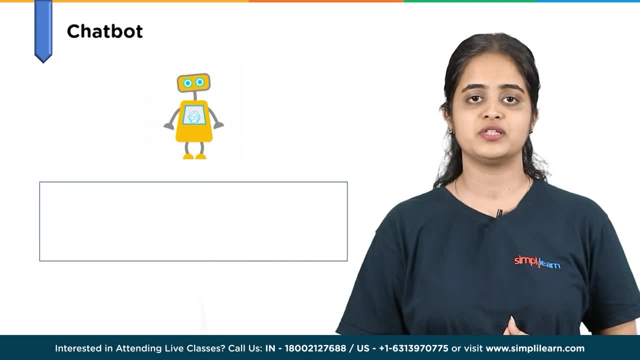 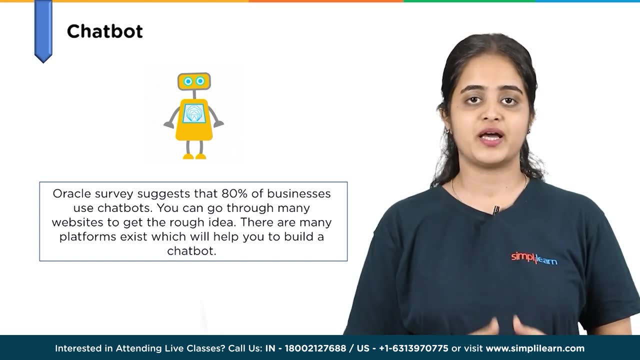 This will make your resume more attractive. in case you are looking for a job, An Oracle survey suggests that 80% of the businesses uses chatbot. You can use Python, Java, Ruby, C++ or PHP as a programming language to develop a chatbot. 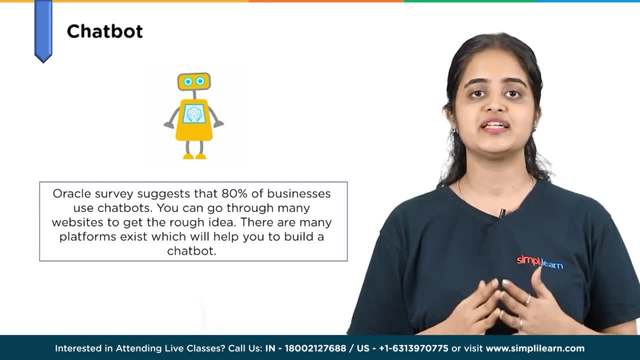 Designing and building NLP chatbots that accept speech and text data is made easier by using the dialogue flow. You can go through many projects to get the rough idea. There are many platforms which will help you to build a chatbot, Regardless of how excellent. 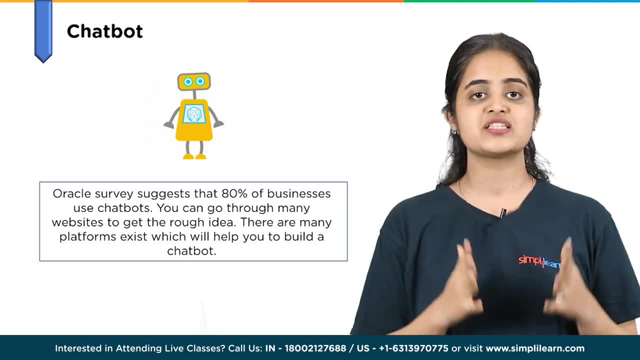 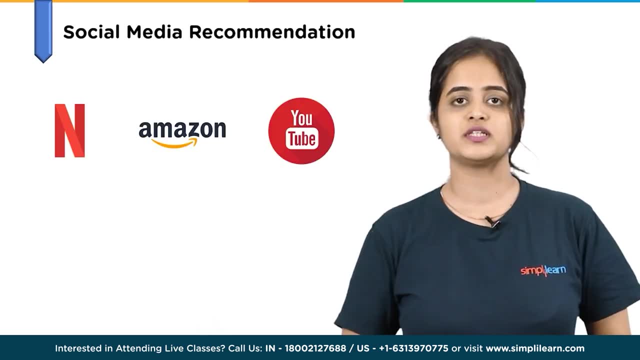 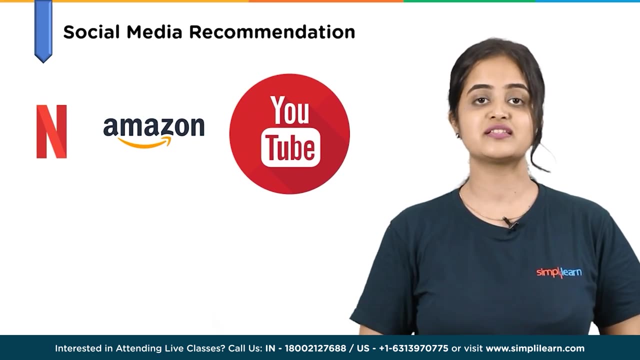 your chatbot is. there is always room for development. The finest chatbot developers constantly enhance their bots over the time using AI and machine learning. Social Media Recommendation System. The rise of web services like Netflix, Amazon and YouTube is the basis of recommender systems. 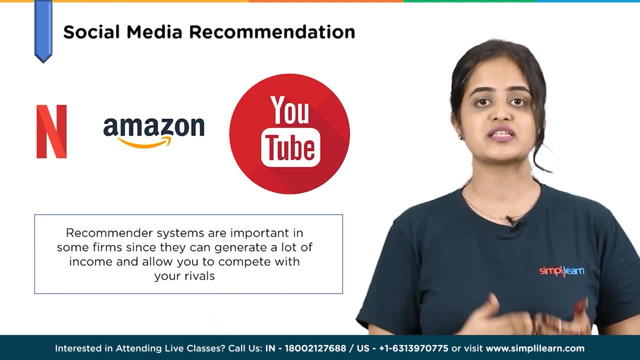 in our daily lives. They are algorithms that insist users in finding information that is pertinent to them. Recommender systems are important in some firms, since they can generate a lot of income or allow you to set yourself apart from rivals In order to provide recommendations. 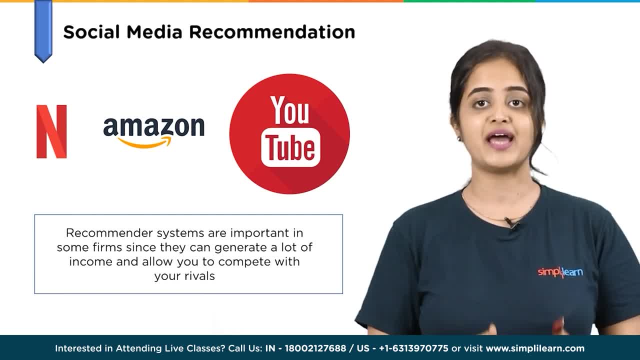 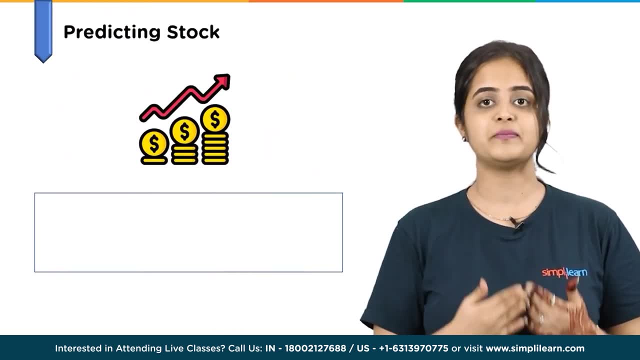 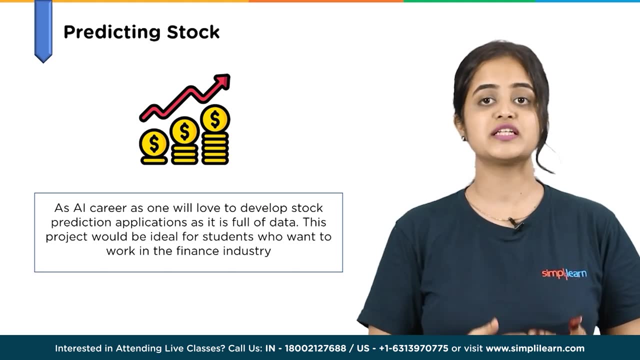 it evaluates the relationship between the user and the object, as well as the parallels between users and positions. This application is widely applicable everywhere. As AI career aspirants, one will love to develop stock prediction applications. as it is full of data, This project would be ideal. 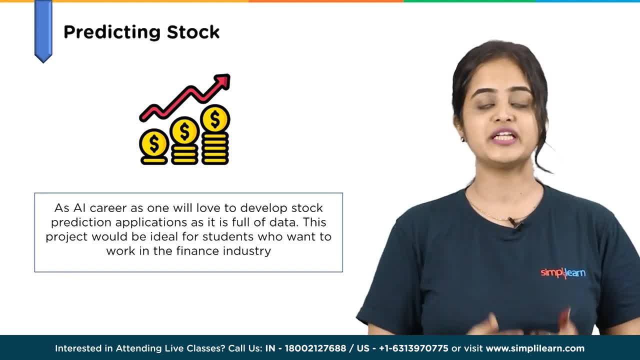 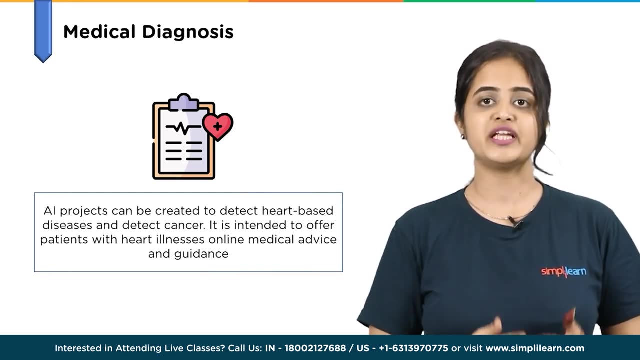 for students who want to work in the finance industry, because it can provide a better understanding of various aspects of the field. Coming to Medical Diagnosis, This project is advantageous from a medical standpoint. AI projects can be created to detect heart-based diseases and also detect cancer. 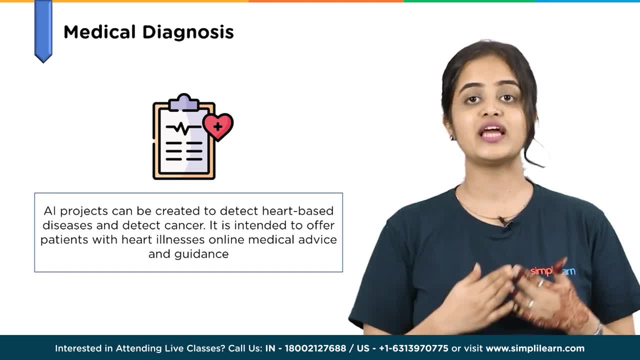 It is intended to offer patients with heart illness online medical advice and guidance. After processing the data, this system will search the database for any illnesses that might be connected to the given details. Using data mining techniques, this intelligent system determines the disease that the patient's 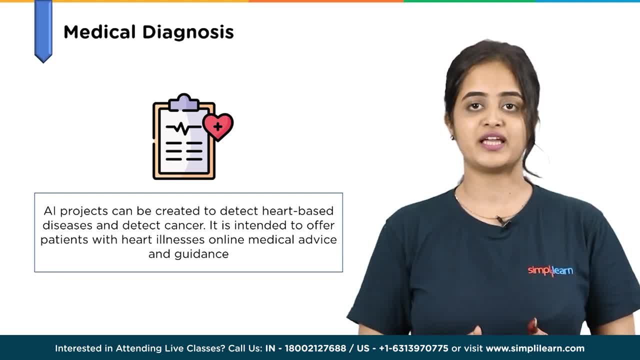 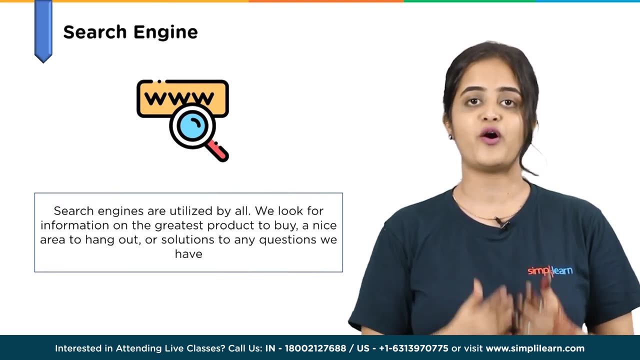 information most closely resembles, Based on the system diagnosis. users can then speak with qualified medical professionals. Users of the system can also view information about various doctors Coming to an important project, that is, Search Engine. Search Engines are utilized by all We look for information on. 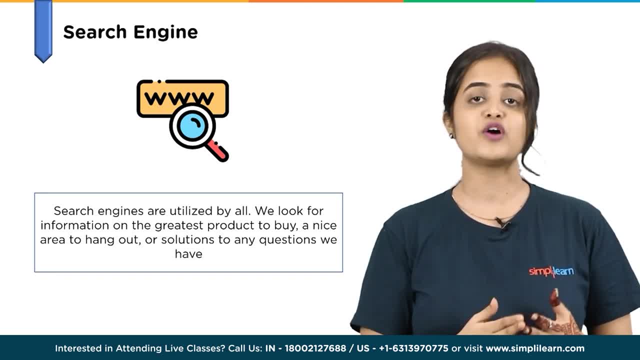 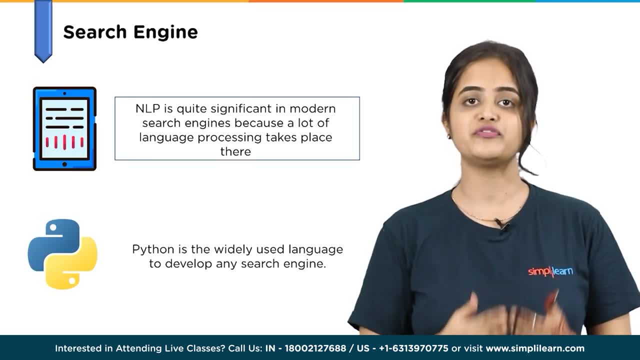 the greatest product to buy, a nice area to hang out or solutions to any questions we have. NLP is quite significant in modern search engines because a lot of language processing takes place there. NLP is a widely used language to develop any search engine. 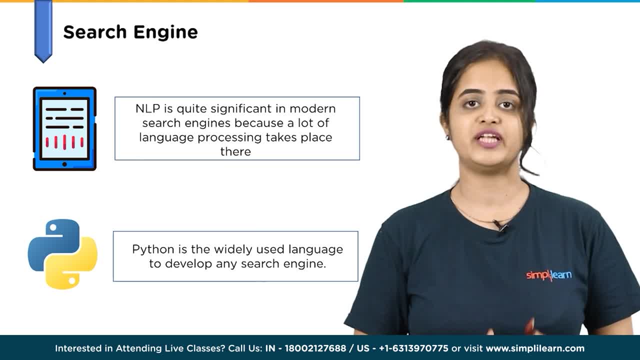 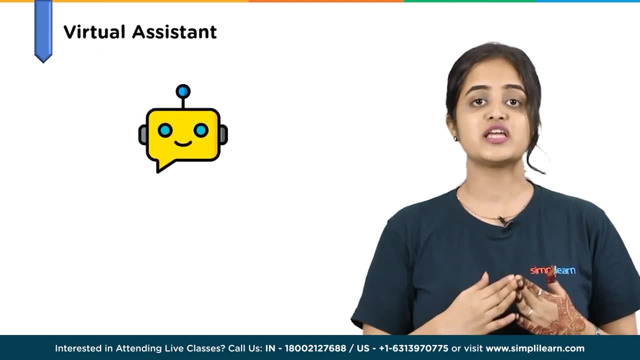 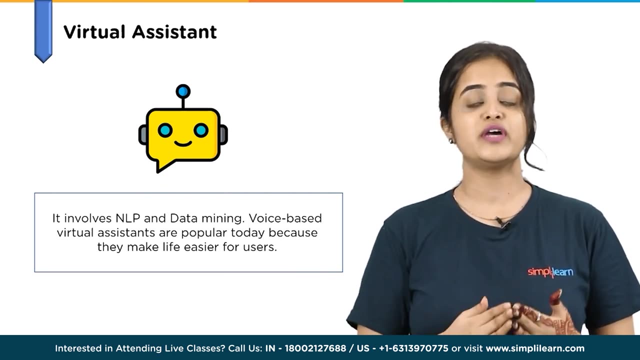 Search engine is mainly confined with lots and lots of data. It is helpful for any AI career aspirants. Next is Virtual Assistants. Here the challenge is to build a virtual assistant to assist user. Why do you need virtual assistant in your devices when you are? 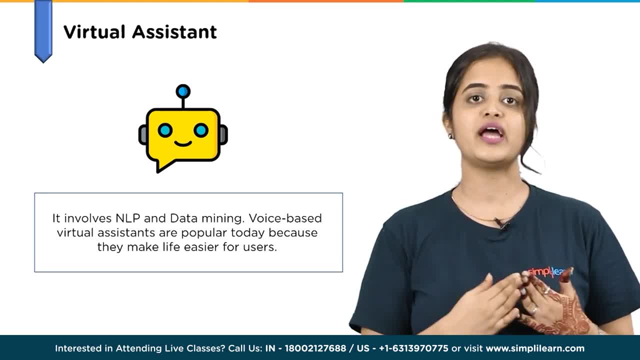 building your own. It is also interesting for a ML developer to build a virtual assistant. It involves NLP and data mining. Voice based virtual assistants are popular today because they make life easier for users. NLP is utilized to comprehend human language in order to 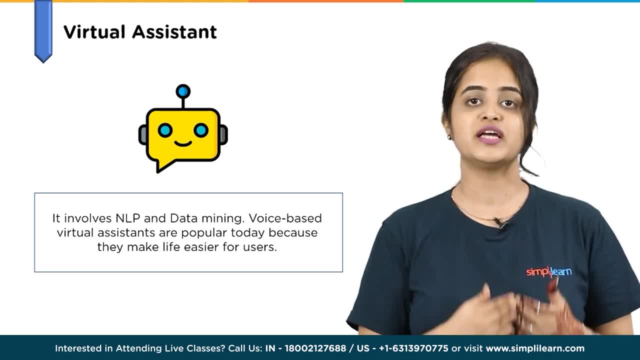 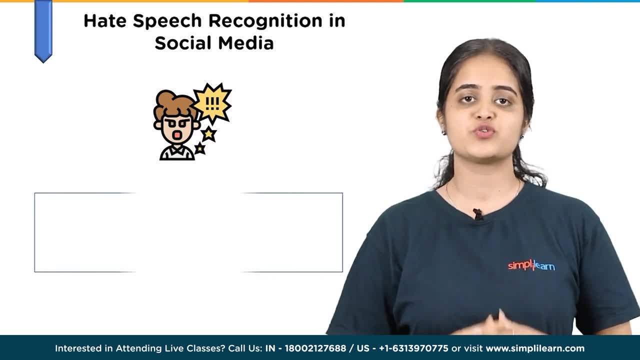 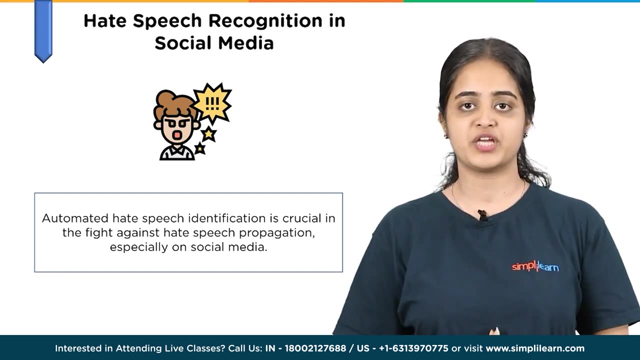 construct the system. When a voice command is received, the system will translate it into machine language and store the commands in its database. Hate Speech Detection in Social Media. Automated hate speech detection is a crucial weapon in the fight against hate speech propagation, especially on social media. 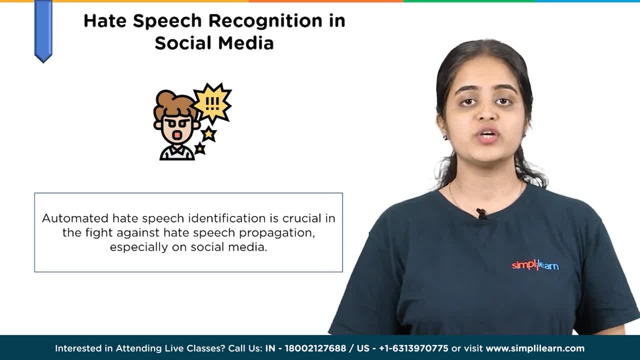 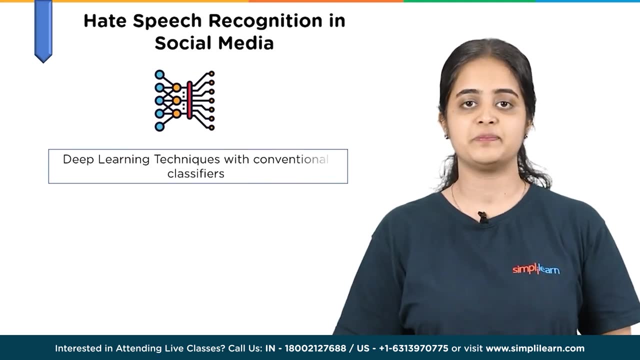 For the job. many techniques have been developed, including a recent explosion of deep learning based system For the objective of detecting hate speech. a number of techniques have been investigated, including conventional classifiers, classifiers based on deep learning and combination of both of them. On the other hand, 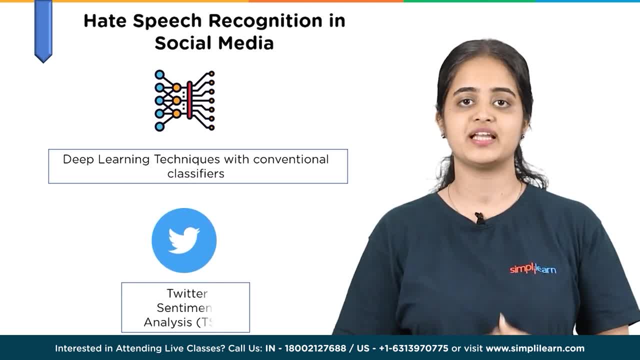 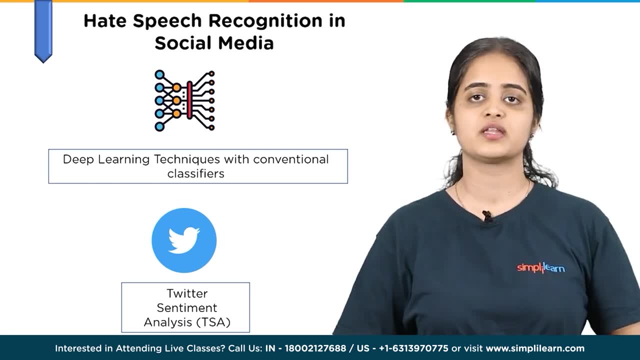 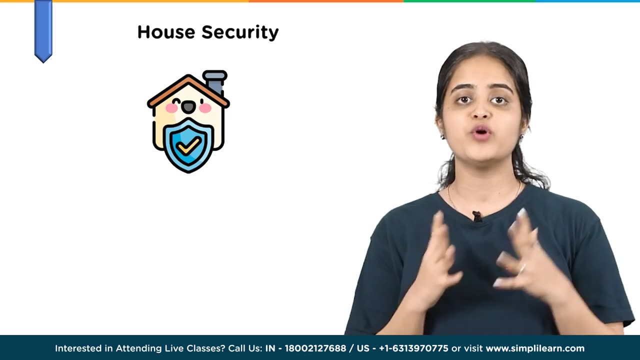 a number of dataset benchmarks, including Twitter sentiment analysis, have been introduced and made available for the evolution of the performance of these algorithms, And the last one is Predicting House Price. You will need to estimate the sale price of a brand new home in any place for this assignment. 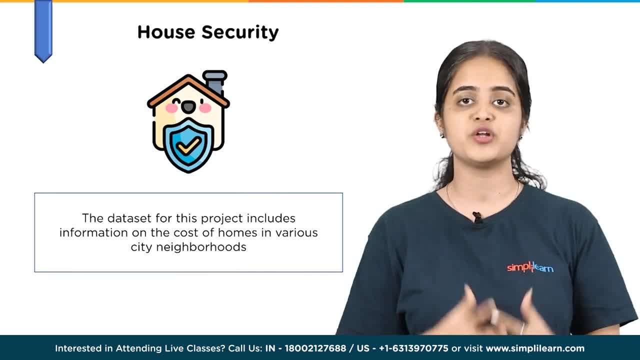 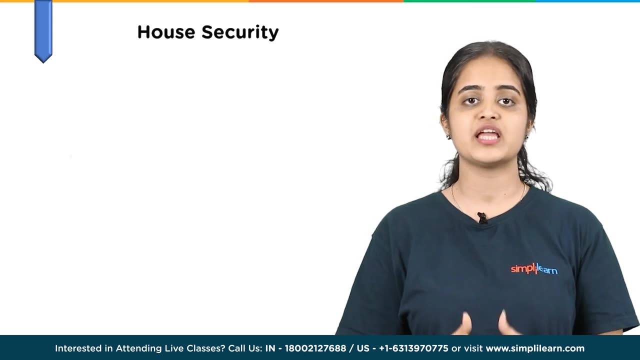 The dataset for this project includes information on the cost of homes in various city neighborhoods. The UCI Machine Learning Repository is the place where you may find the dataset needed for this research. You will also receive other dataset with information on the age of the population, the city's crime rate. 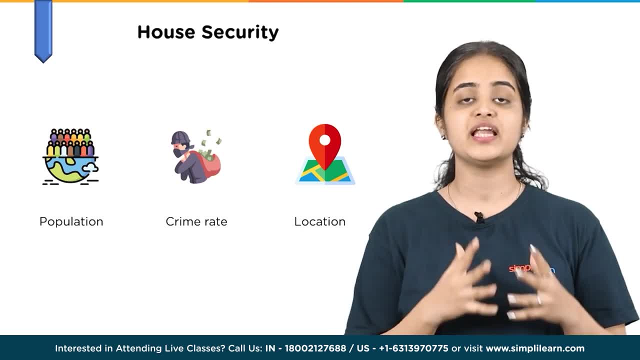 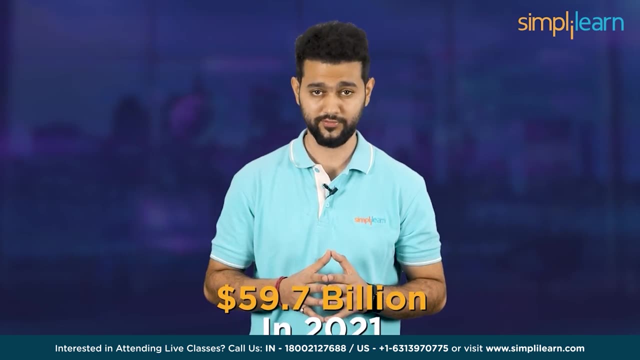 and the location of non-retail enterprises, in addition to the pricing of various residences. It's an excellent project to test your knowledge if you are a newbie. Popular market research projects that the market for artificial intelligence will grow from $59.7 billion in 2021. 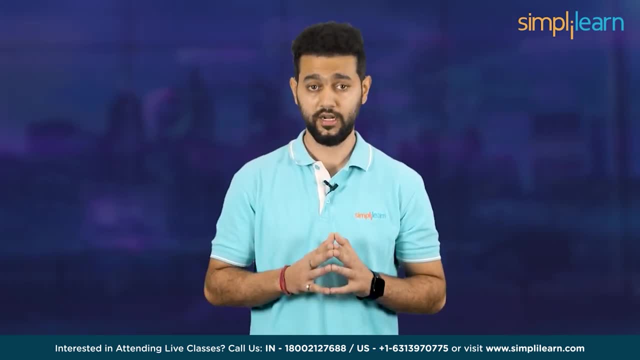 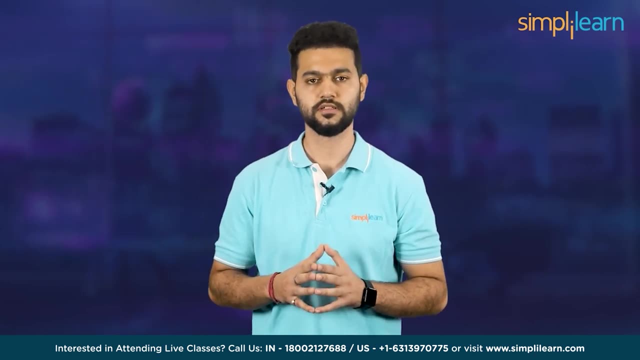 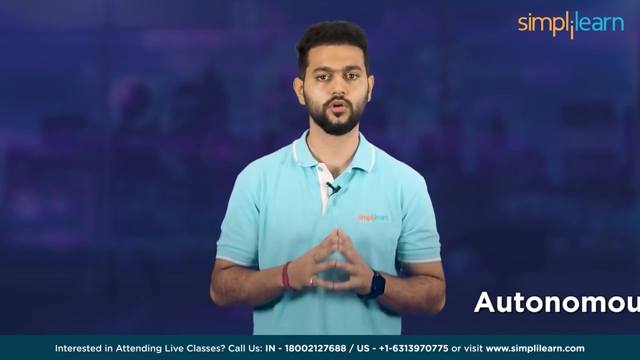 to $422.4 billion in 2028.. Artificial intelligence, automation and robotics are disrupting almost every business. Companies that don't invest in AI services risk becoming obsolete, Whether in machine learning, smart applications, appliance digital assistants or autonomous vehicles. Numerous companies 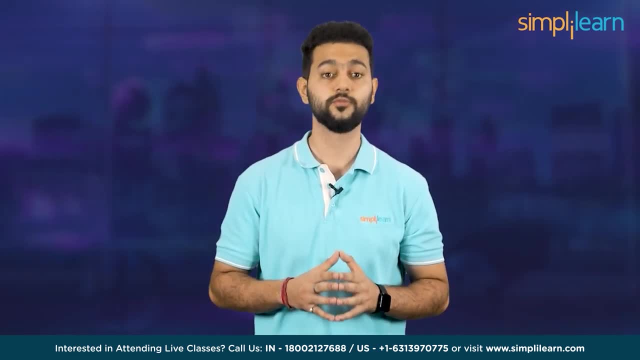 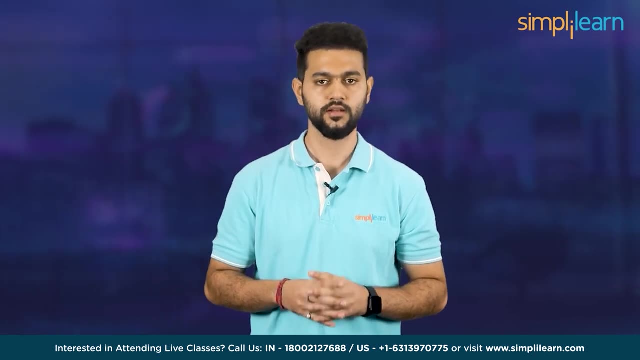 stand to benefit from AI, but a handful of them have proven to be the game changers for 2023 and beyond. So, hey, everyone, you are already watching. Simply Learn. and here we are with the list of top 10 AI companies in 2023. 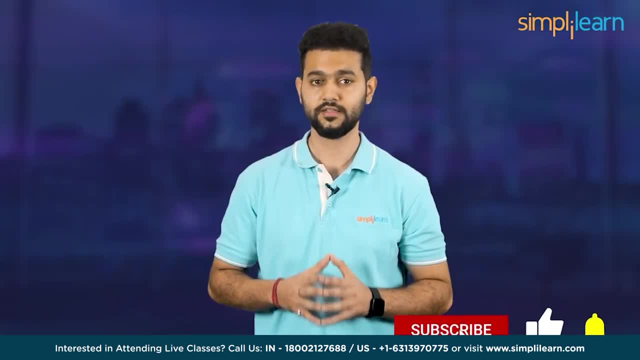 If you love watching videos like these, do hit the subscribe button to never miss an update from Simply Learn. So let's explore and learn about them one by one, starting with the 10th position, which is UiPath. Robotic Process Automation, or RPA, is a technology developed 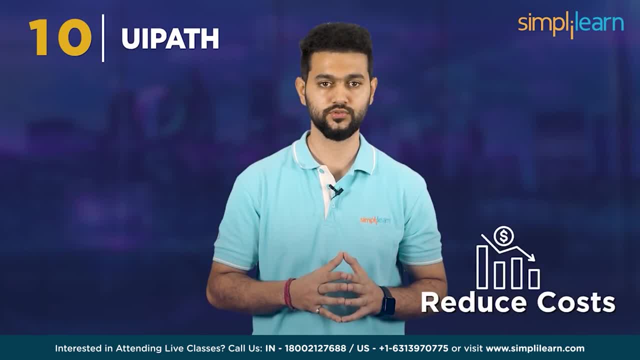 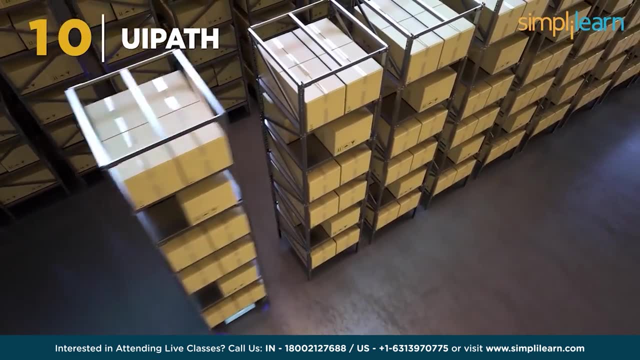 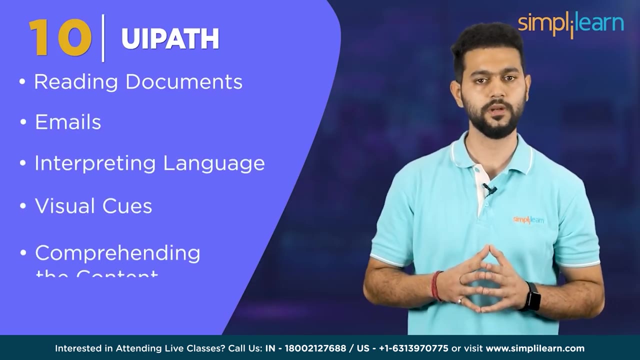 by UiPath that helps businesses to boost productivity and reduce cost by automating time consuming and repetitive operations. Software robots can be equipped with UiPath AI technologies to carry out duties including reading documents and emails, interpreting language and visual cues and comprehending the content and the intent of the communications. 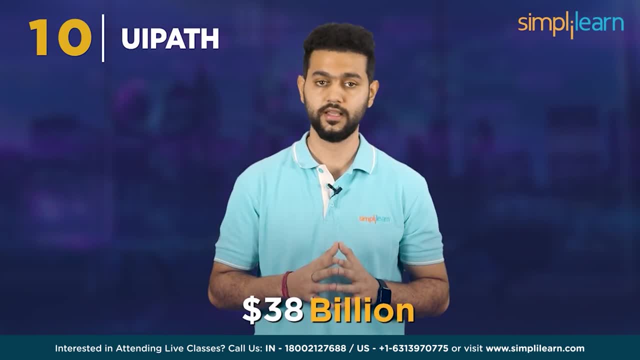 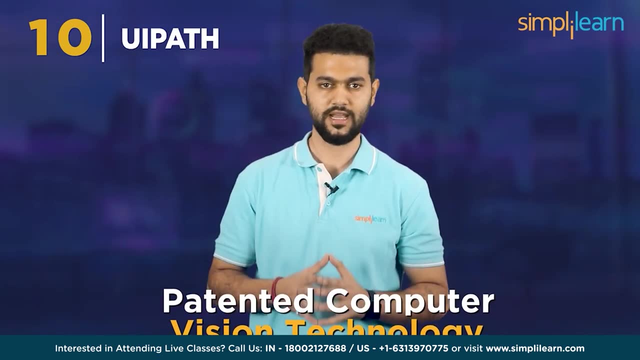 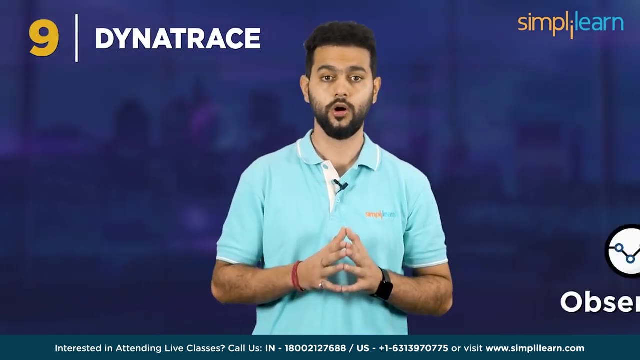 The RPA market is estimated to be worth 38 billion, and UiPath offers distinct advantages over the competitors thanks to its patent computer vision technology and wide range of bot technologies. In the 9th position, we have Dynatrace. The services offered by Dynatrace include observability. 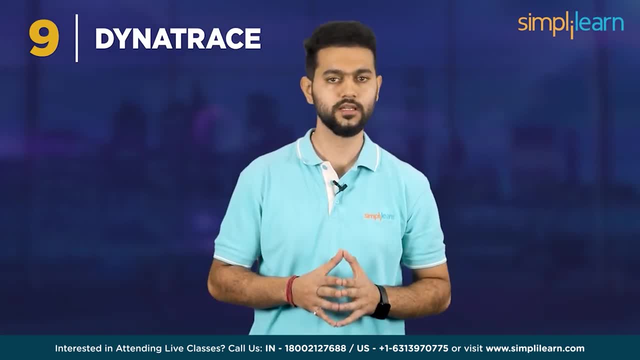 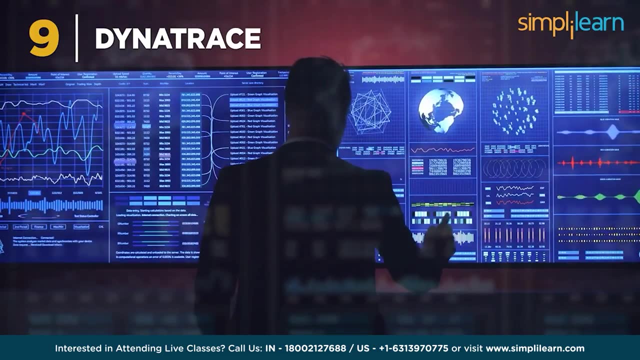 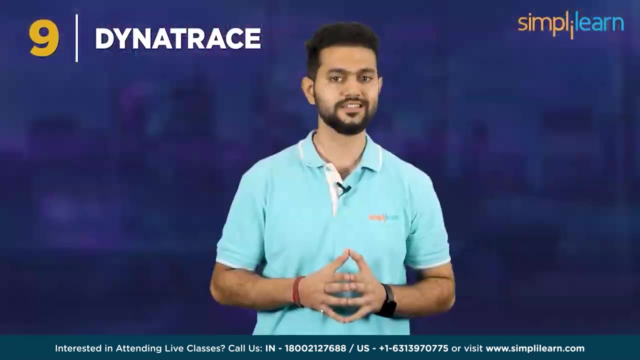 and infrastructure monitoring. The Davis AI engine developed by the business can analyze 368 trillion dependencies each second. Davis can quickly locate problems in a company's digital ecosystem, explain what went wrong and evaluate and rate likely commercial ramifications. The company estimated a market worth 285.42. 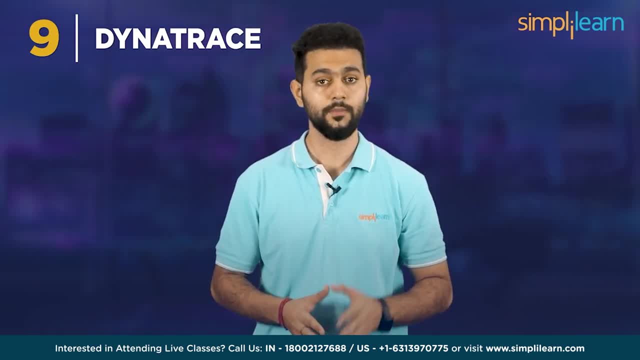 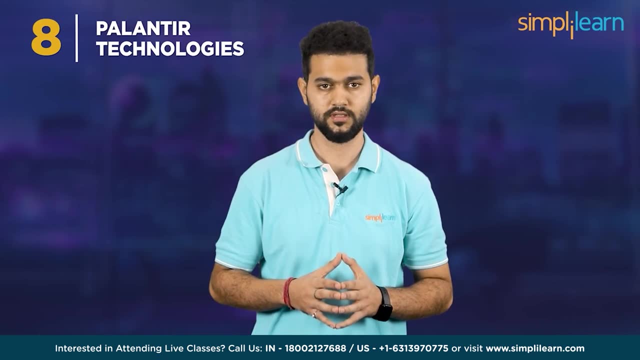 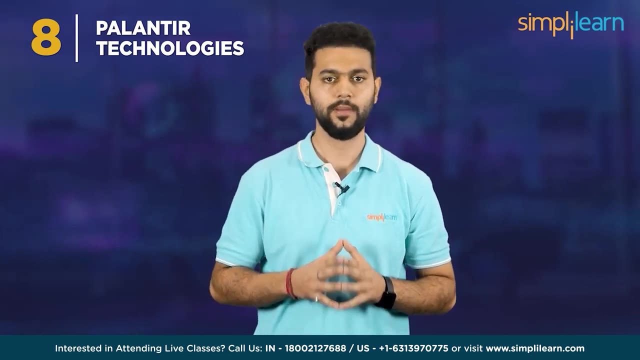 million and is poised to grow revenue by roughly 20% annually throughout at least 2025.. Then, at the 8th position, we have Palantir Technologies. Data analytics software startup Palantir Technologies uses AI to analyze data. According to revenue and market share. Palantir. 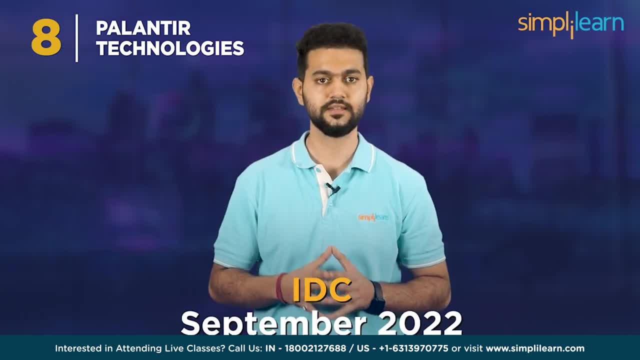 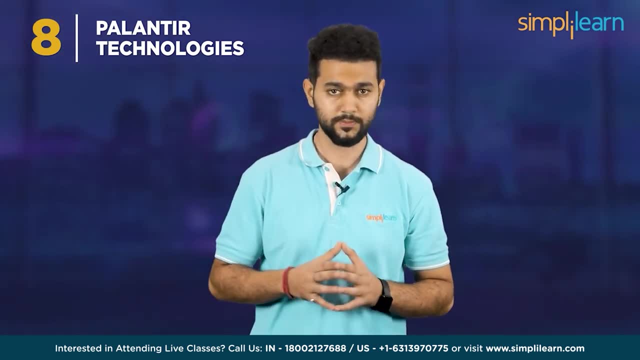 was ranked as the top AI software platform globally by IDC in September 2022.. The United States intelligence and defense industries account for a sizeable portion of Palantir's revenue. The business just won a new 85.1 million contract from the. 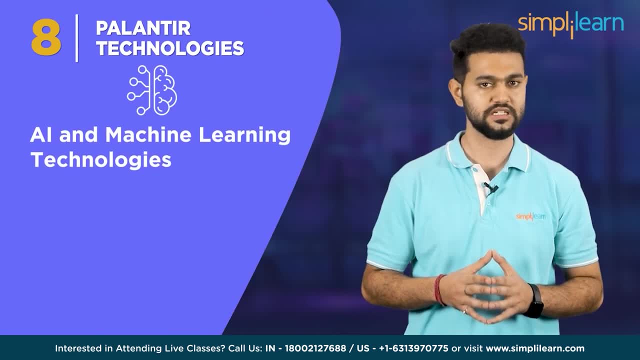 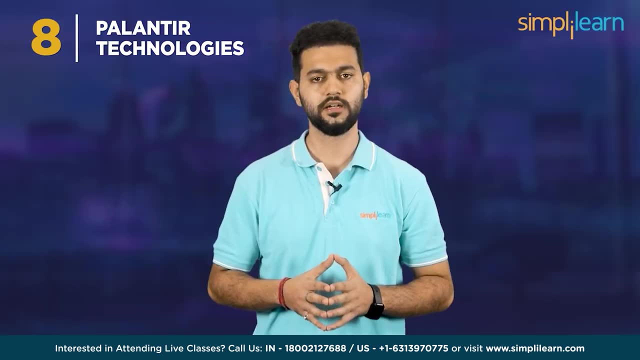 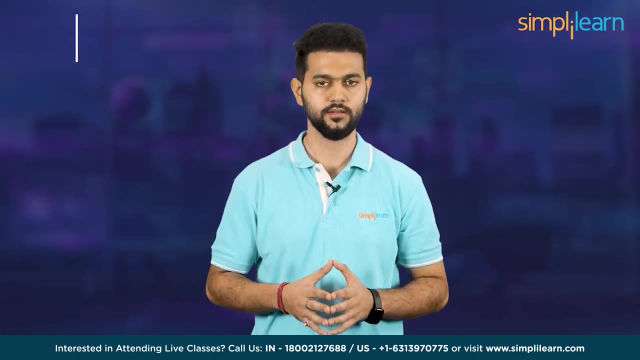 US Army Marshal Command to assist with developing AI and machine learning technologies to enhance equipment reliability, improve predictive maintenance and improve supply chains. Palantir may deliver revenues closer to the higher end of analysis estimates: roughly 2.5 billion in 2023.. Then, at the 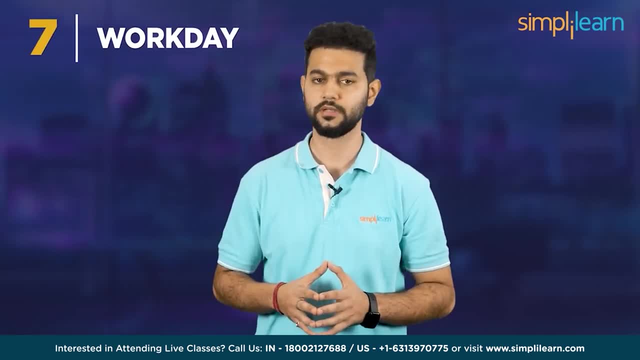 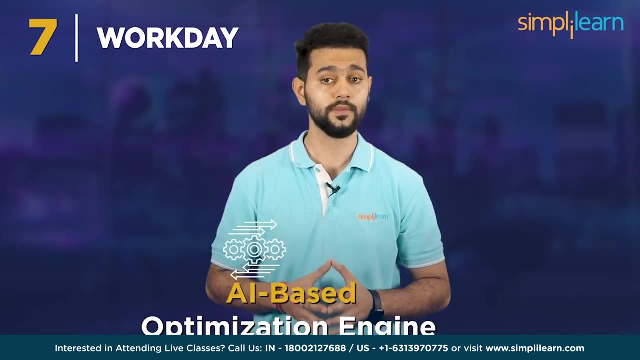 7th position is Workday. Workday is a provider of cloud-based applications with an emphasis on human resources management. With the assistance of Workday's distinctive AI-based optimization engine, businesses can manage challenges with hiring and staffing fluctuation: labor demand shift. 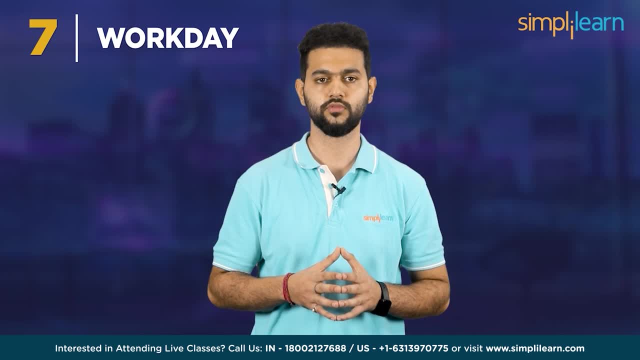 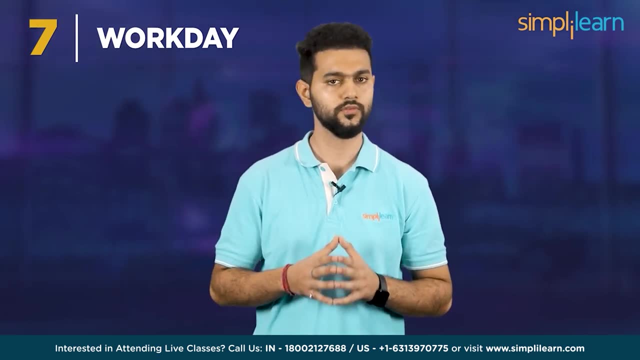 scheduling and prioritizing, and more. In April 2022, Workday incorporated Barista, an AI-powered virtual assistant from Espressif, into their platform. Workday is raising 2023 market worth to almost 1.53 billion representing. 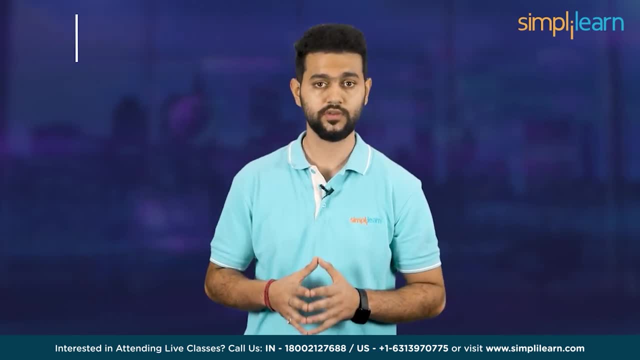 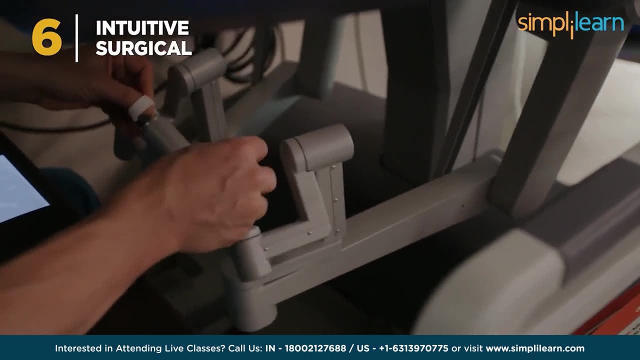 year-over-year growth of 22%. Now, in the 6th position, we have Intuitive Surgical. The Da Vinci surgical system offered by Intuitive Surgical performs minimally invasive procedures using cutting-edge robots and computerized visualization technology With the help of big data. 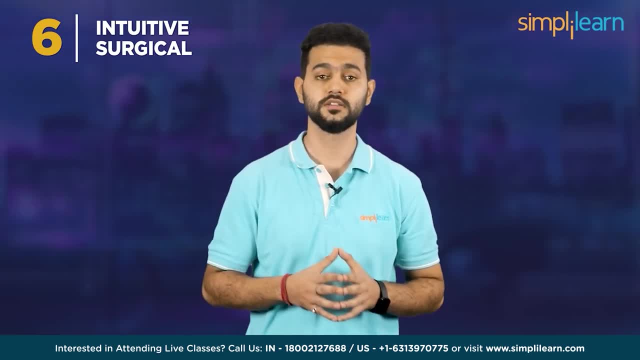 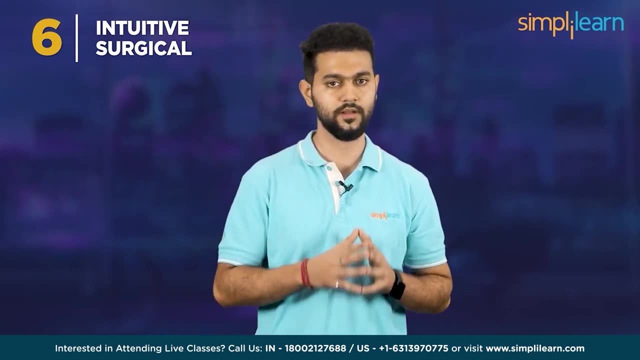 an AI-intuitive is developing tools that will help surgeons by improving their training and offering them real-time direction. Despite the fact that the Da Vinci surgical system has been approved by the US FDA for 22 years, Intuitive reported a 13% year-over-year. increase installed in the system. most recent quarter: The global intuitive surgical market is projected to reach $6.5 billion by 2023. Moving towards the 5th position we have IBM. For years, IBM has been developing strategies to use its AI supercomputer. 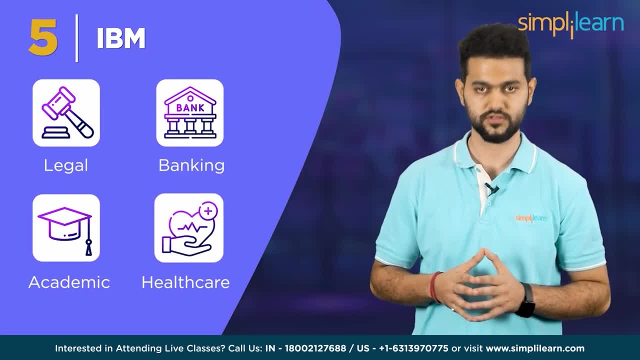 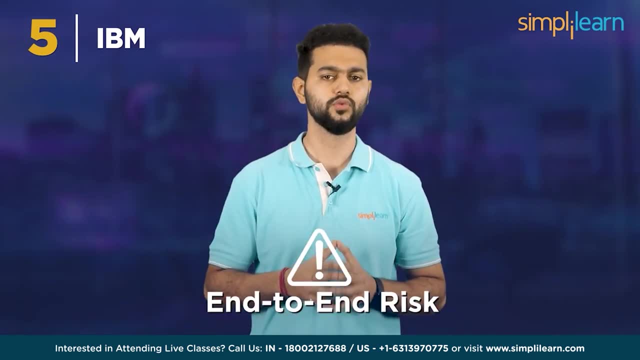 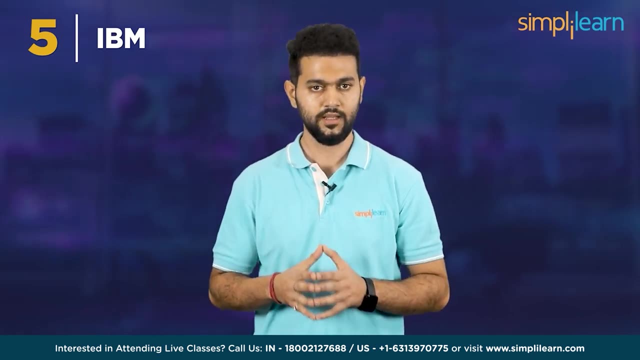 to alter the legal, banking, academic and healthcare industries. IBM's clients harness the power of AI to stay current on ever-changing regulations by providing an end-to-end risk and compliance management. IBM continues to dominate the market for the other breakthroughs in AI and its 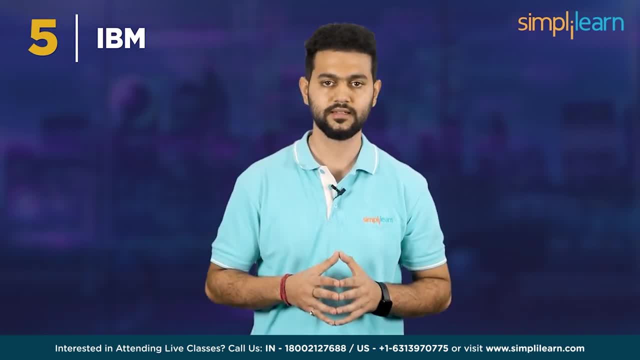 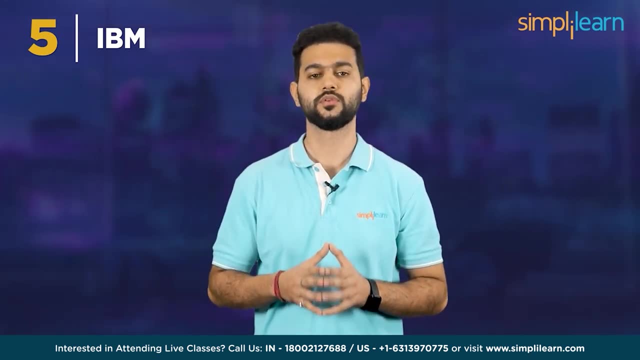 AutoAI and AutoML products can help data scientists build and improve AI and machine learning models. The market worth of IBM in 2023 will range from $14.4 billion to $16 billion. Following that in the 4th position is NVIDIA. 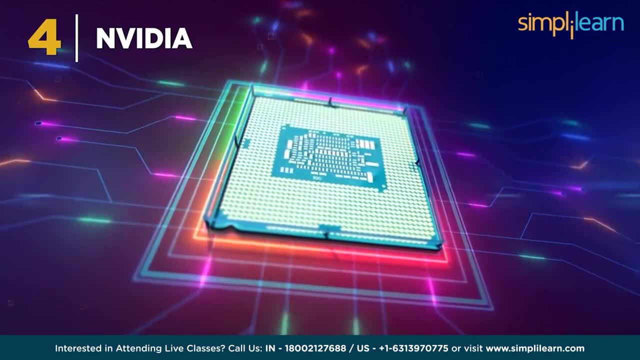 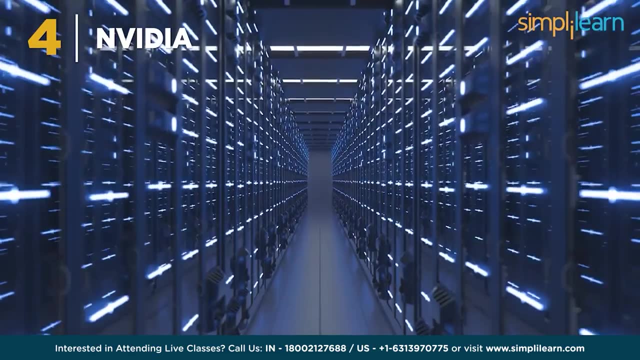 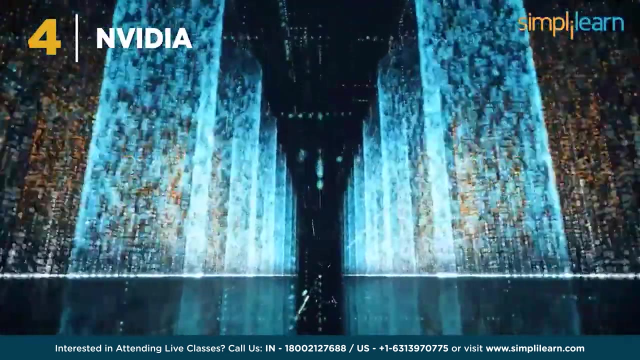 High-end chipmaker NVIDIA provides the significant computing power needed for advanced AI applications. In reality, one of the world's fastest supercomputers, Leonardo, is powered by NVIDIA graphics processing units. The parent company of Facebook Meta Platforms is building the biggest AI supercomputer. 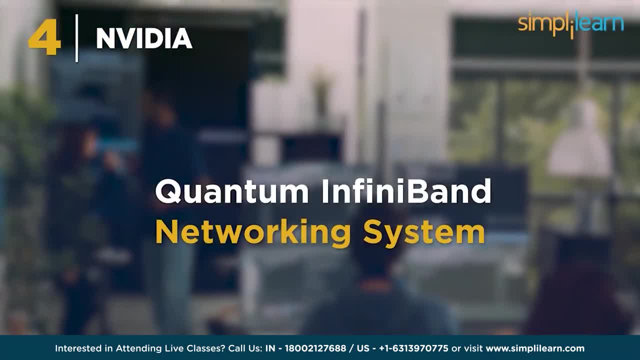 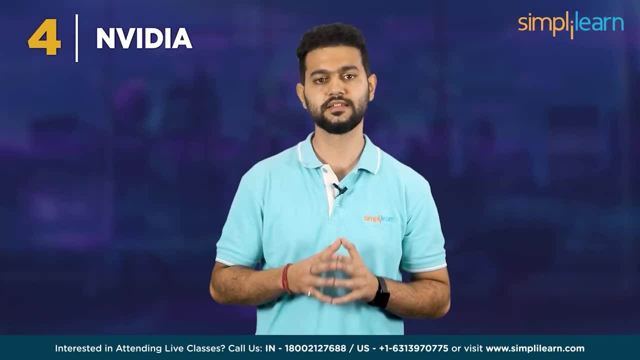 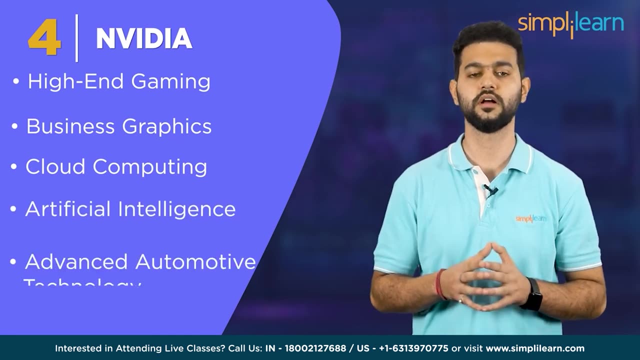 in the world. Meta also owns NVIDIA's Quantum Infiband networking system and 6080A 100 NVDA graphics processing processors. NVIDIA is a significant supplier for fast growing industries like high-end gaming, business graphics, cloud computing, artificial intelligence and advanced 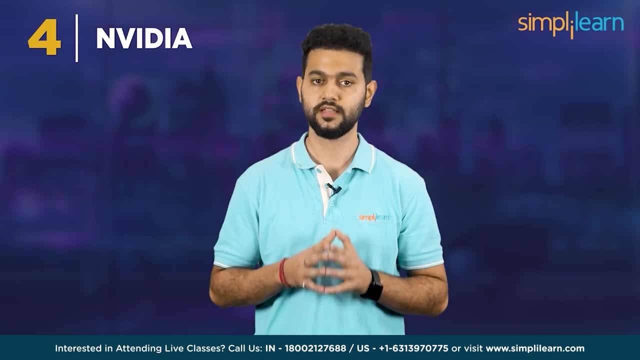 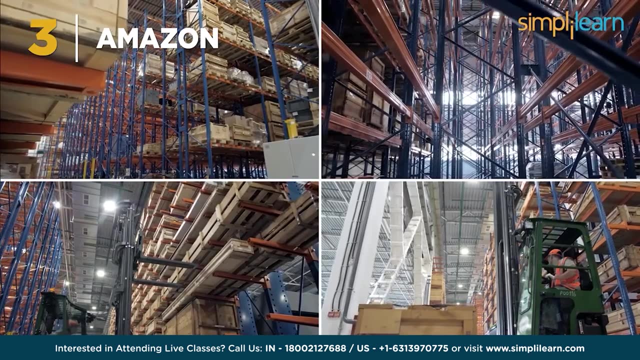 automotive technology. NVIDIA's outlook for 2023 revenue is expected to be around $6 billion. Here comes the top three in the list, And in the third position we have Amazon. AI is integrated into every aspect of Amazon's business, including. 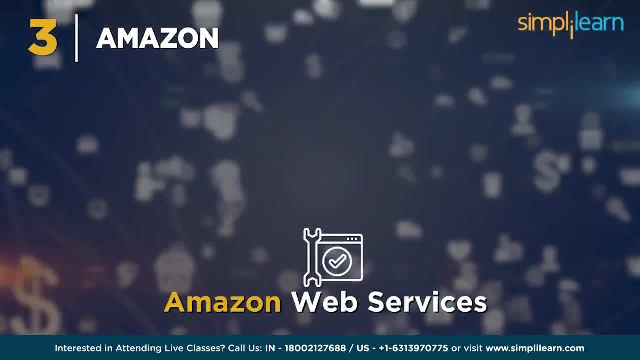 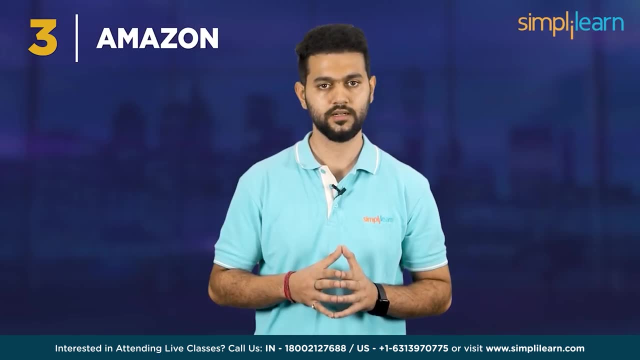 e-commerce, search engines, targeted advertising and Amazon Web Services. Amazon Alexa, one of the most popular virtual assistant, is already present in many American homes. Amazon said in August that it would pay $1.7 billion to acquire a robot called RBT, a maker of home. 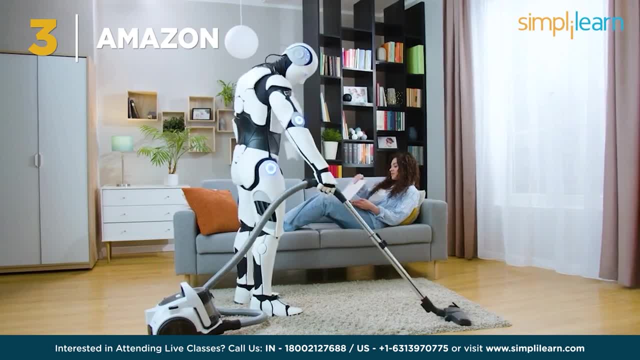 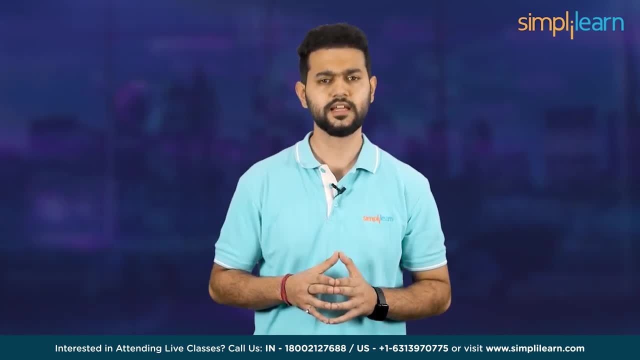 robots. This action can allow Amazon to boost the use of AI in households worldwide. Amazon expects a $491 billion market worth between 2023 and 2027.. In the second position is Alphabet. Alphabet, the company that owns Google and YouTube, uses 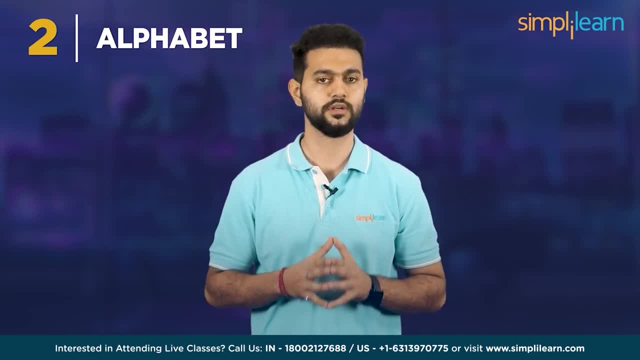 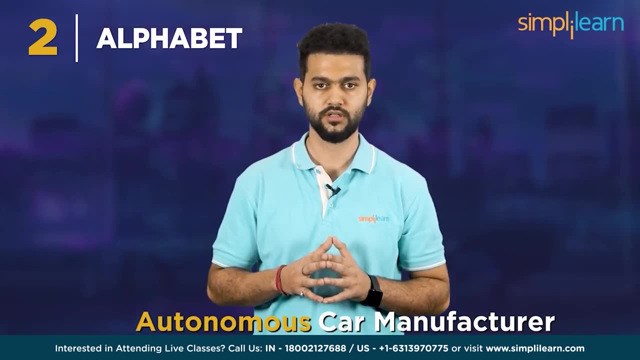 AI and automation in practically every part of its business, including ad pricing, Gmail spam filters and content promotion. In addition, it is the parent company of the autonomous car manufacturer Waymo and the AI software business DeepMind, which created history in 2022 when it became 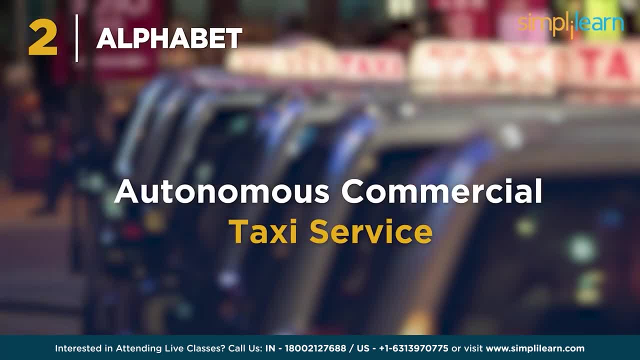 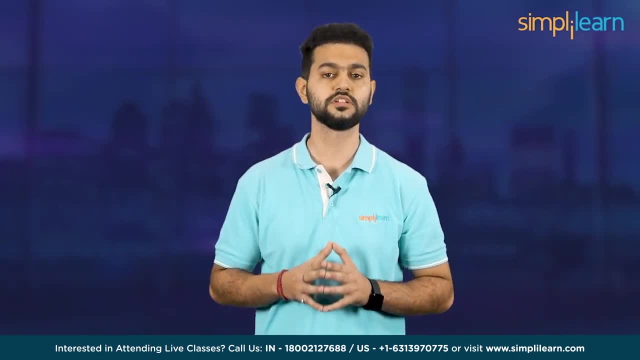 the first completely autonomous commercial taxi service to operate on public routes. The market worth of Alphabet in 2023 will be around $70 billion, and the first position on the list is Microsoft. In 2020, Microsoft announced the construction of a new 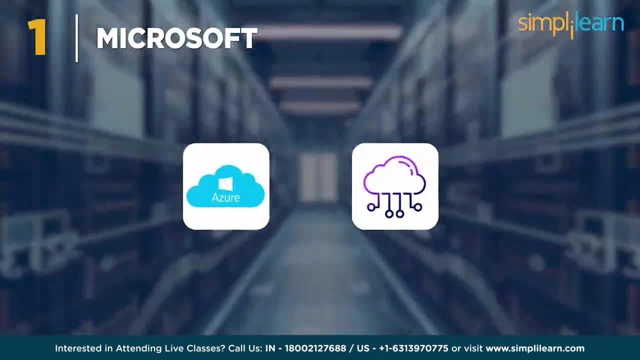 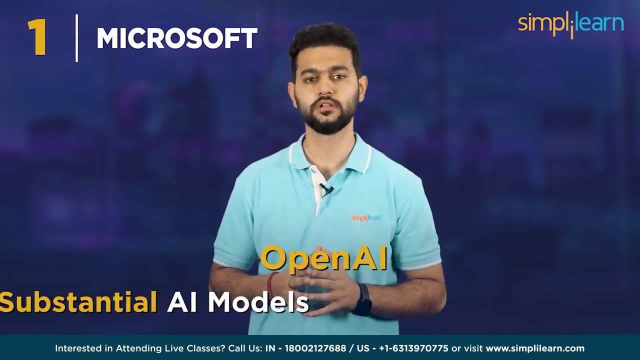 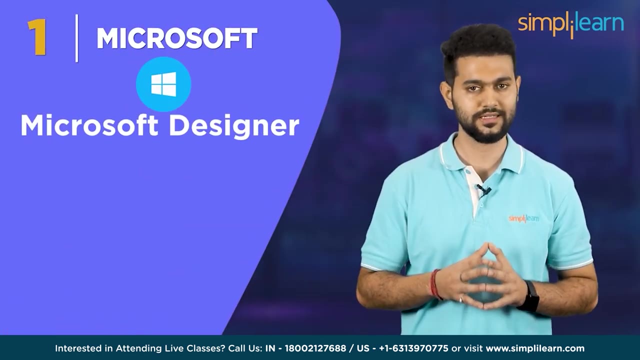 supercomputer hosted on Azure, Microsoft's cloud computing network. The supercomputer was created in collaboration with OpenAI to train AI models, producing substantial AI models and related infrastructure for programmers and other businesses. In October, Microsoft released Microsoft Designer, a graphic design. 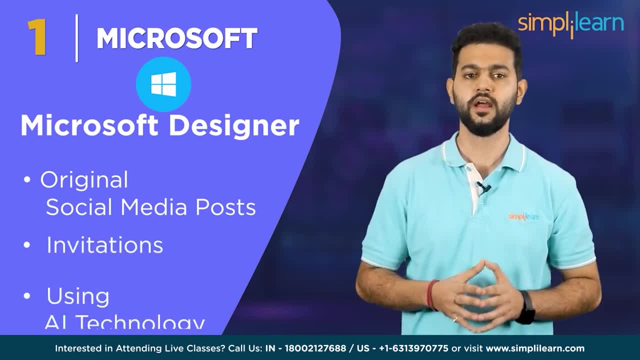 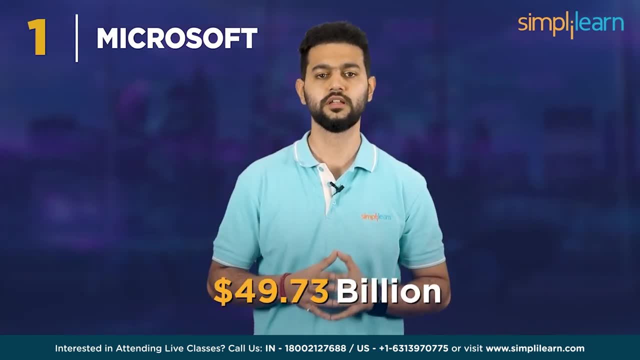 tool that makes original social media posts, invitations and other graphics using AI technology. Microsoft, the tech giant, is expected to earn a market worth of $49.73 billion, And with that we have come to the end of this list of the top 10 artificial. 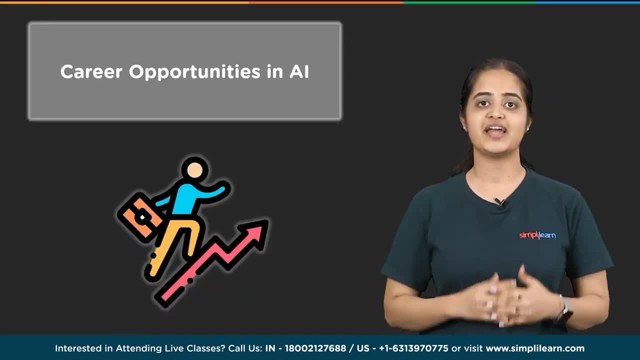 intelligence companies of 2023.. Opportunities in AI have increased significantly in recent years. The surge in jobs related to AI is legitimate due to its widespread involvement in crucial fields. According to Indeed, the pay range for jobs involving artificial intelligence is between $160,000. 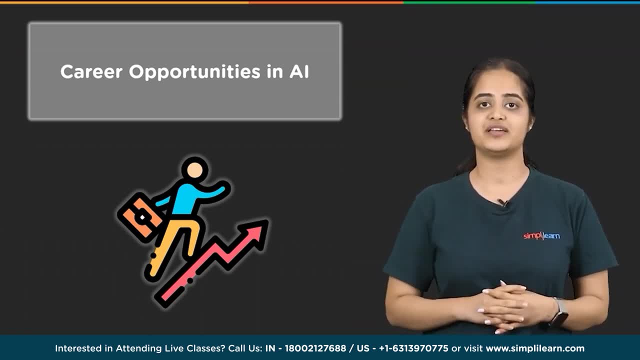 to $3,050,000 and can go even higher. So we have come up with a list of leading career opportunities in artificial intelligence, along with companies hiring for those roles. But before we begin, here is a question for you. Who do you? 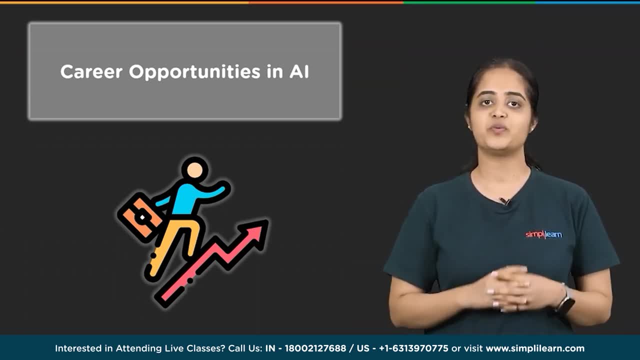 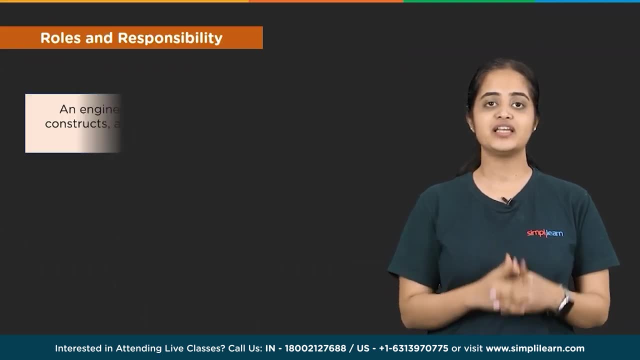 think is currently leading the AI market? Let us know in the comment section below. So, without any further delay, let's get started. Starting with our list, we have robotics engineers. An engineer in robotics creates prototypes, constructs and tests machines and updates the. 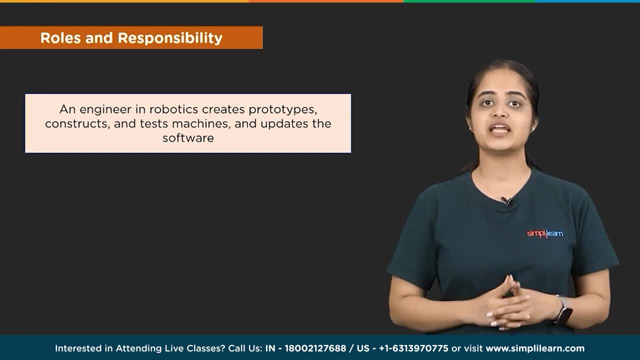 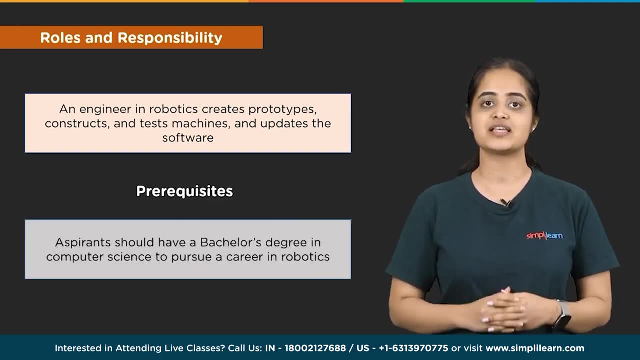 software that manages them. Additionally, they investigate the most affordable and secure way to make their robotic system. Aspirants should have a bachelor degree in computer science and pursue a career in robotics, with additional training or certification in automation is advantageous. Robotics engineers are in high demand. with 9000 plus job openings in India and 8000 plus openings in the US. Top companies like Amazon, Bosch and Flybase are hiring robotics engineers with salaries as high as $160,000 in the US and Rs 27 lakhs in India. 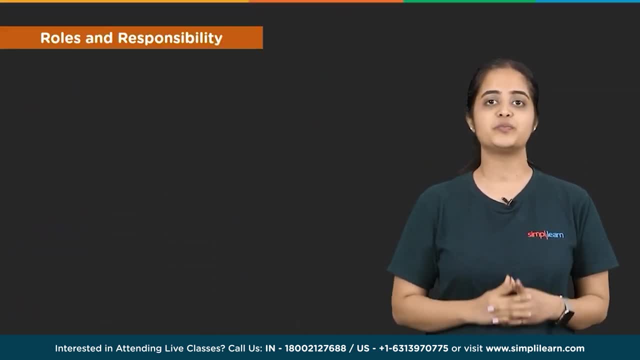 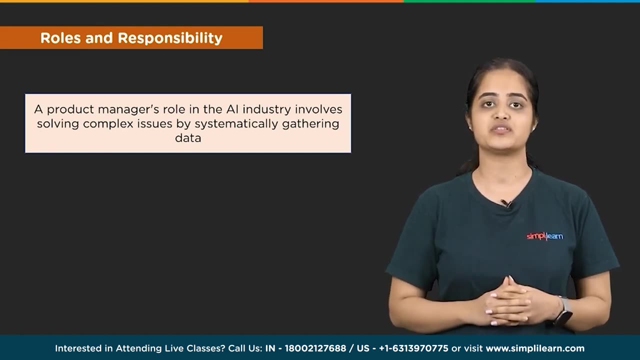 Next up on our list, we have product manager. The role of a product manager is to recognize and express user requirements, market research and creating competitive evaluations, and also creating a product's vision and putting emphasis on a product's strengths and qualities. Freshers. cannot join as a product manager. It requires basic experience of 2-3 years in the field of product and software development. According to Indeedcom, an average of 2000 plus jobs are currently available in India and 20000 plus job vacancies. 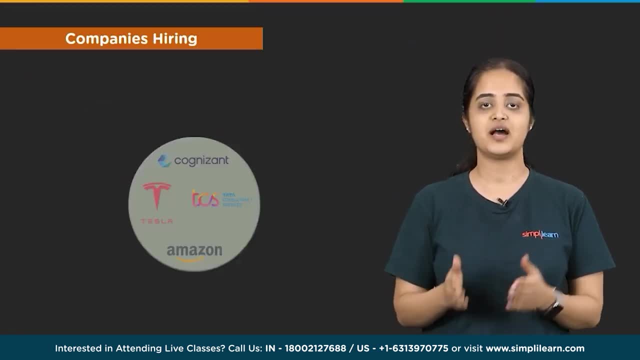 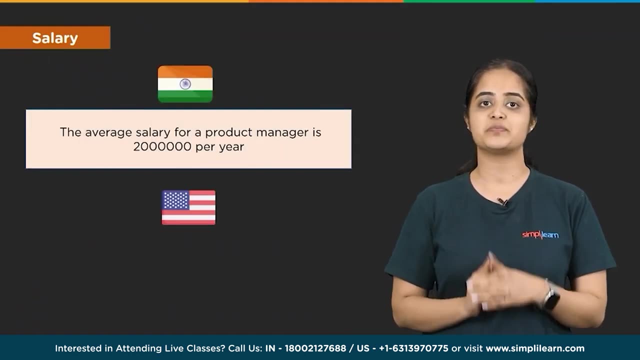 are there in the US with top companies. hiring are Tesla, Amazon, PCS, Sprinkler, Cognizant, etc. with a salary as high as $160,000 per year in the US and Rs 20 lakhs per annum in India. Up next we have 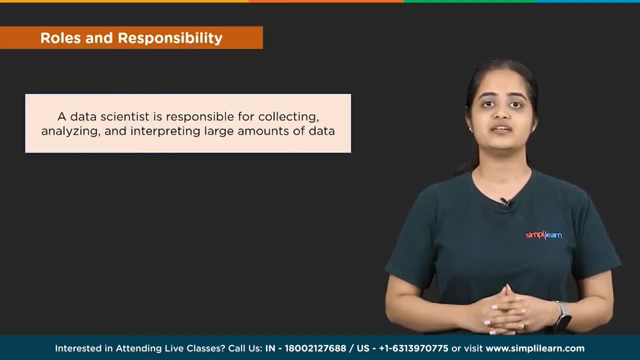 data scientist. They mainly deal with lots of data. Extraction of knowledge from all collected data is the subject matter of data science. It was also voted the sexiest job of the 21st century. Good news is there is no need for any special degree, As 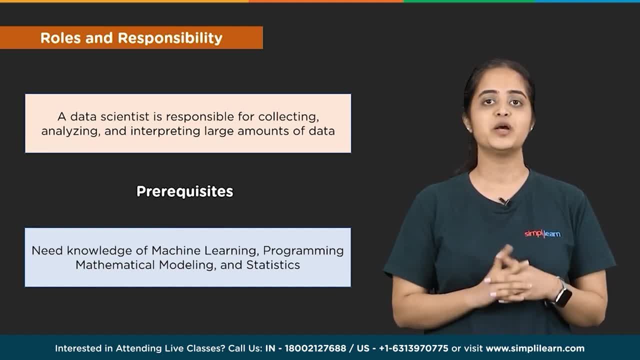 a data scientist, you need to have knowledge of machine learning, programming in Python, R, Java and mathematical modeling. Being a fresher, you can join as a data scientist too. Data scientists are in demand, with 17000 plus vacancies in the US and 3000 plus vacancies in India, and big businesses like Accenture, TCS, IBM, Google, JP Morgan, Deloitte, Bank of America recruiting data employees with salary going as high as $200,000 per year in the US And Rs 15 lakhs per annum. 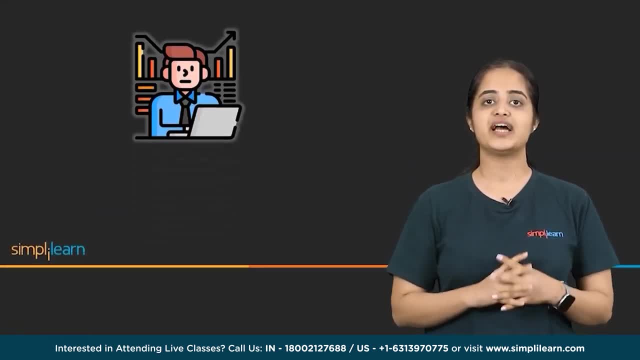 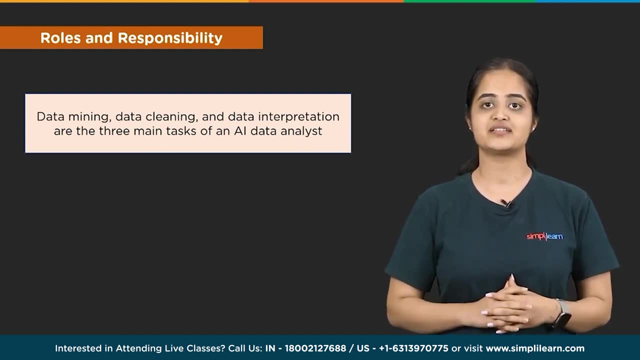 in India. Moving forward in our list, we have AI data analyst. Data mining, data cleaning, data interpretation are the three main tasks of an AI data analyst. Data cleaning allows for the gathering of the necessary information for data analysis. An AI data analyst makes inferences. 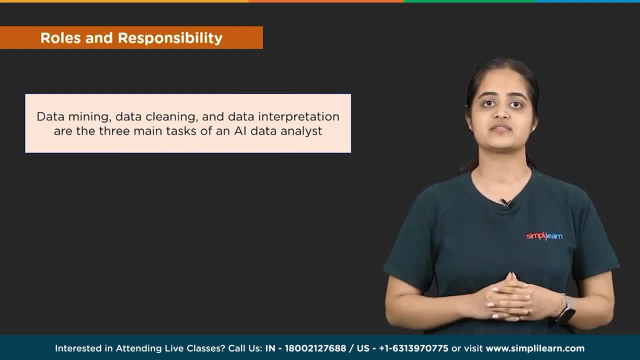 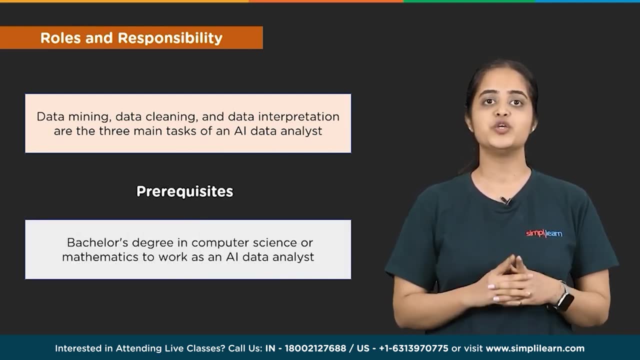 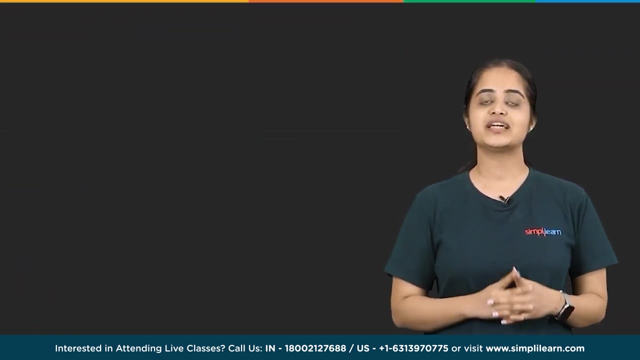 from the data using statistical tools and techniques. You need a bachelor degree in computer science or mathematics to work as an AI data analyst. To get this job, you must have a thorough understanding of regression and be able to use MS Excel. According to indeedcom, there are currently: 700 plus AI data analyst jobs available in the United States and 16000 plus job vacancies in India, with top companies like Accenture, IBM, Wipro, TCS and Capgemini recruiting them, and salaries going as high as $100,000. 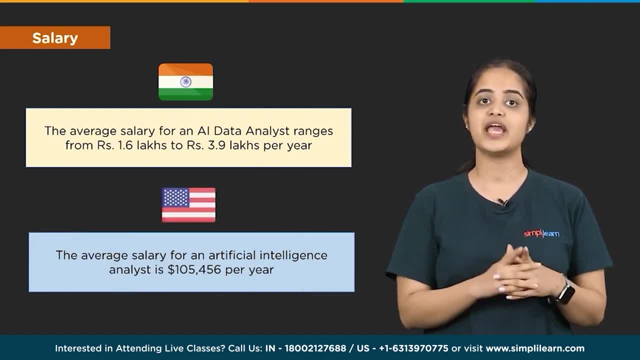 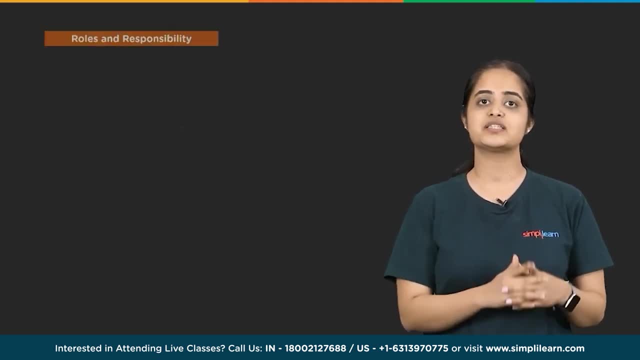 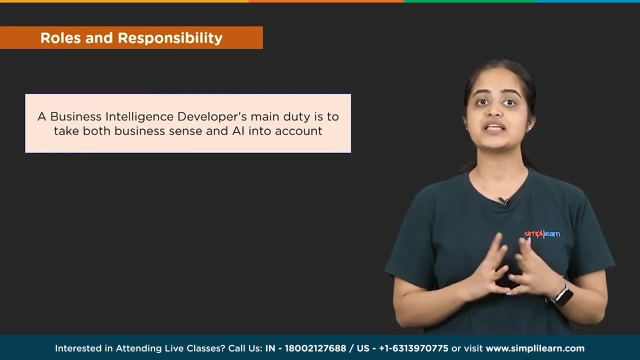 per year in the US and Rs 8.5 lakhs per annum in India. The next job opportunity in AI is business intelligence engineer. A business intelligence developer's main duty is to take both business sense and AI into account. They evaluate complex data. 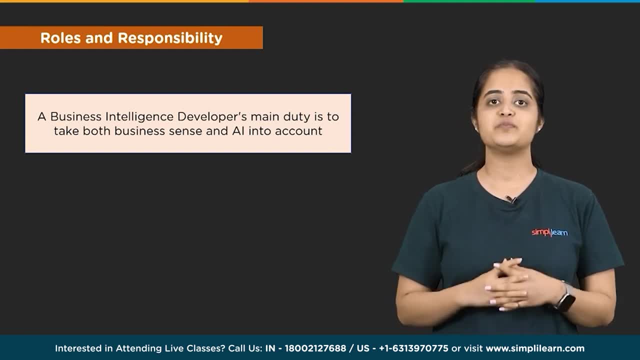 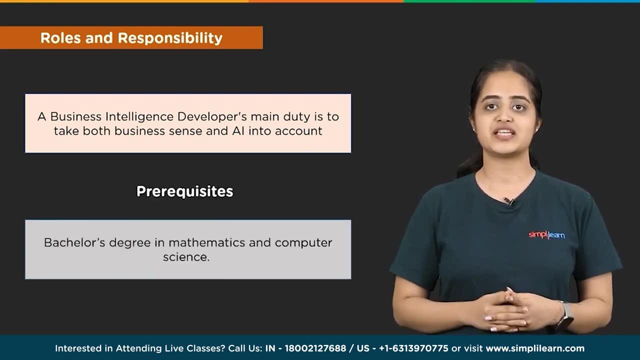 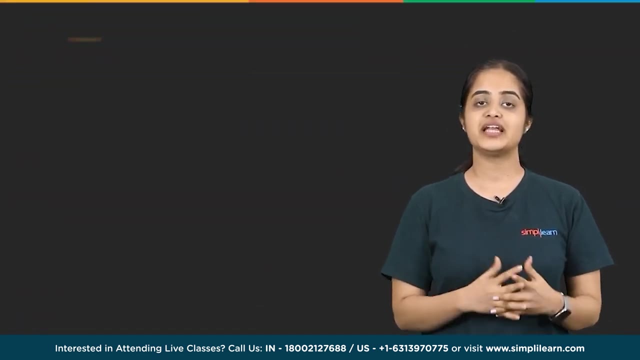 sets to identify various business strengths. They assist in boosting a company's earnings by planning, creating and sustaining business intelligence solutions. To become a business intelligence engineer, you are required to have a bachelor degree in mathematics and computer science. According to indeedcom, there are 8000. 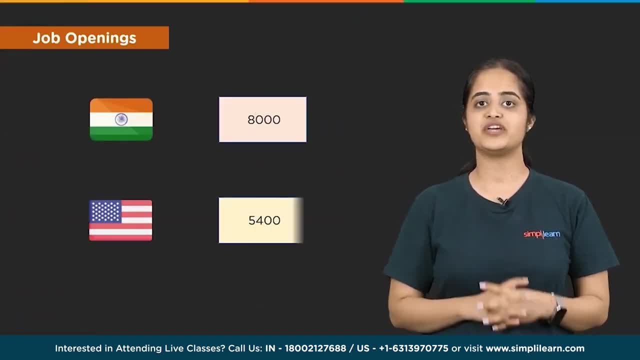 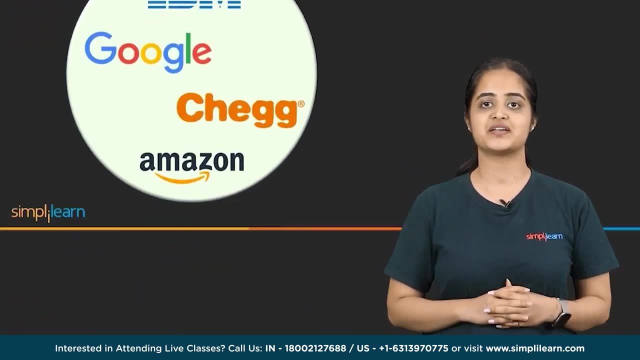 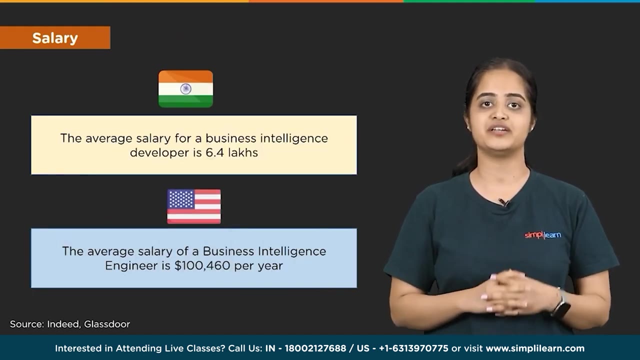 plus jobs available in India and 5000 plus job vacancies in United States. Companies hiring are Amazon development centre, IBM, AWS, etc. With this salary going as high as $100,000 per year in the USA and Rs 15 lakhs per year in India. 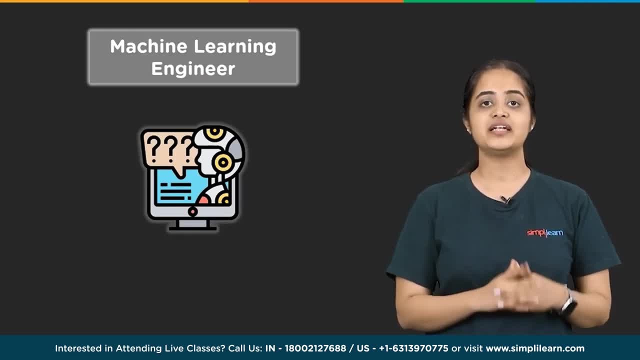 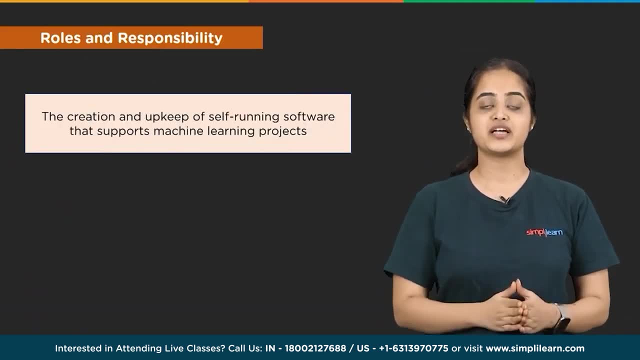 Coming to the top 3 jobs available in AI, at number 3 we have machine learning engineer. Artificial intelligence is known to include machine learning. It runs simulations using the varied data provided and produces precise results. They are constantly in demand from the businesses and their position. 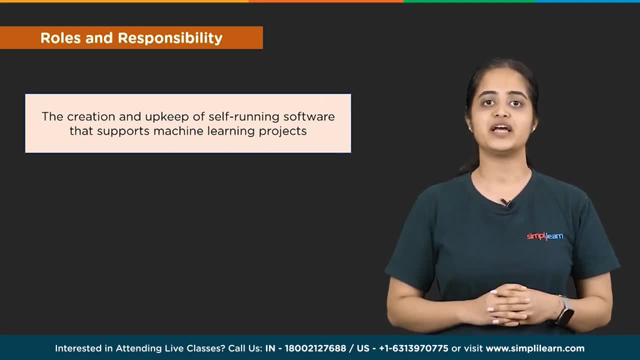 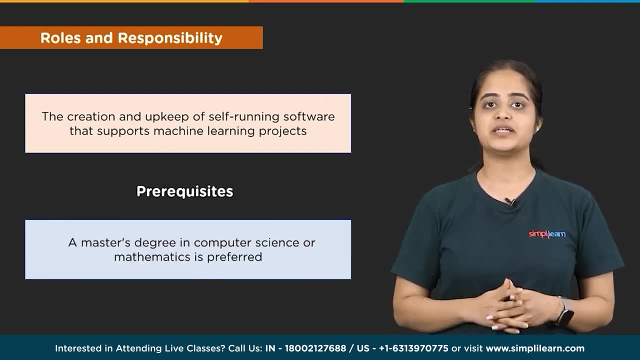 seldom goes unfilled. They handle enormous amount of data and have exceptional data management skills. The ability to code, use computers and understand mathematics are requirement for success as a machine learning engineer. A master's degree in computer science or mathematics is highly preferred. The necessary technological stats include python, R, Scala and Java. A deep understanding of neural networks, deep learning and machine learning algorithm is very helpful. Coming to job opportunities, Glassdoorcom predicts 13000 plus job vacancies in the US and 27000 plus jobs. 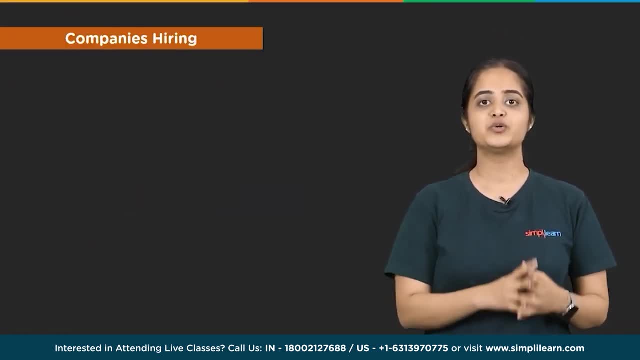 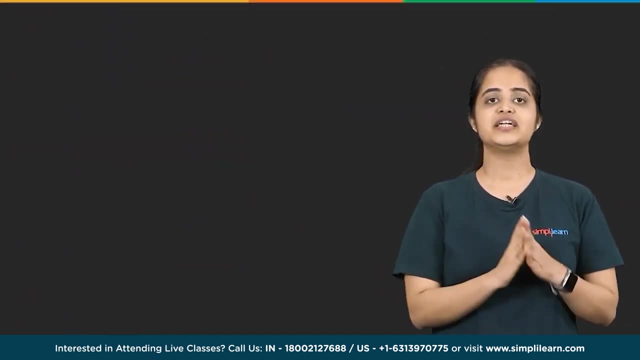 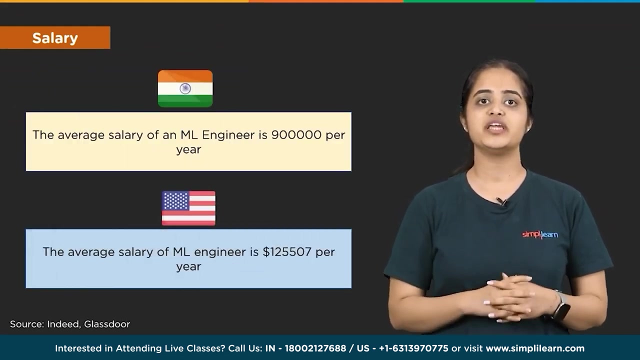 available in India, with companies like Mathwork, Google, Amazon, Microsoft Azure, IBM, etc. Hiring them, with salary going as high as 150000 per annum in the US and Rs 10 lakhs per year in India, Coming at runner up position. we have 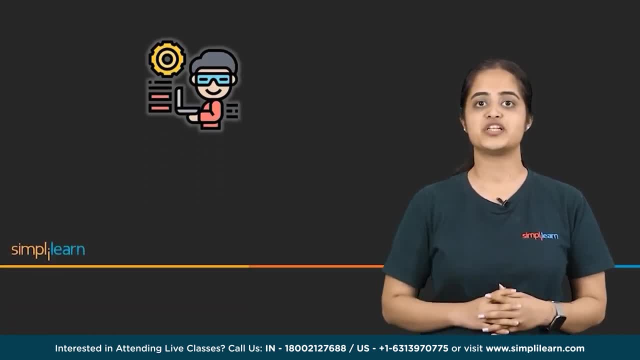 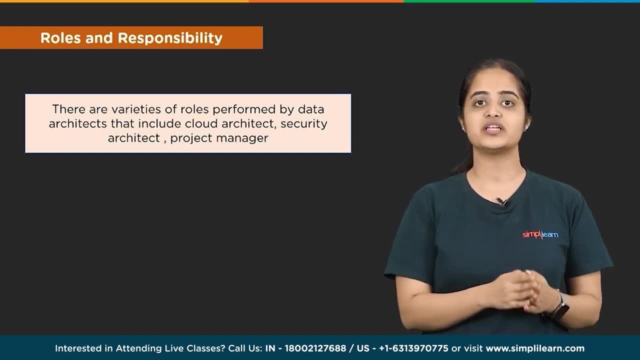 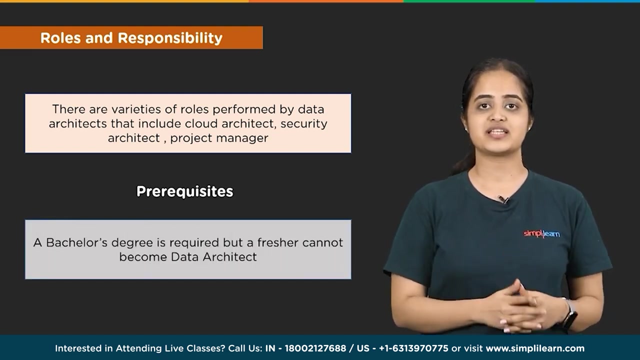 data architect. Data architects are IT specialists who utilize their knowledge of computer science and database architecture to assess and analyze an organization's data infrastructure. Fresher graduates cannot become data architects. A bachelor degree in computer science and computer engineering or related subject is the absolute minimum. 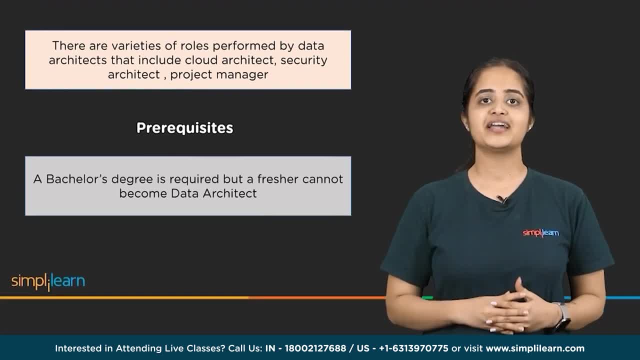 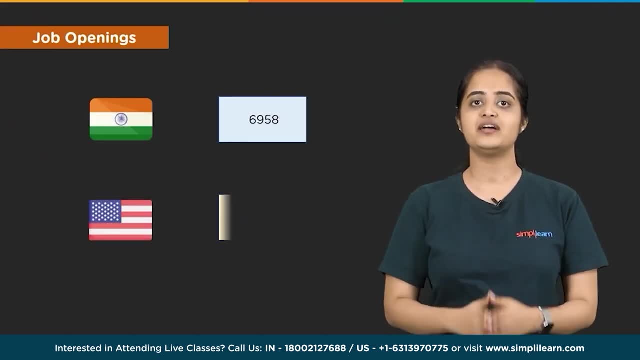 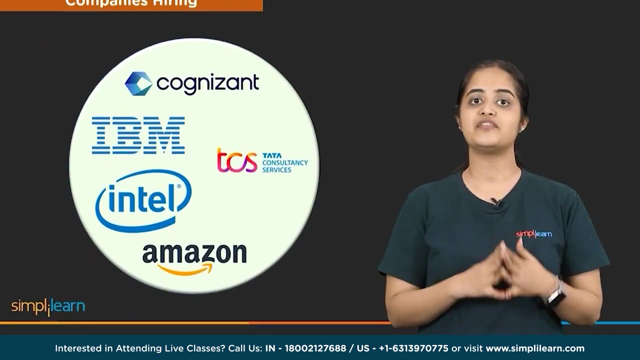 requirement to become a data architect. Data architects are in high demand, with 52000 job vacancies in the US and 7000 plus jobs in India, and top companies hiring data architects are Amazon, IBM, Tesla, Intel, Wipro, with the average salary quite high as 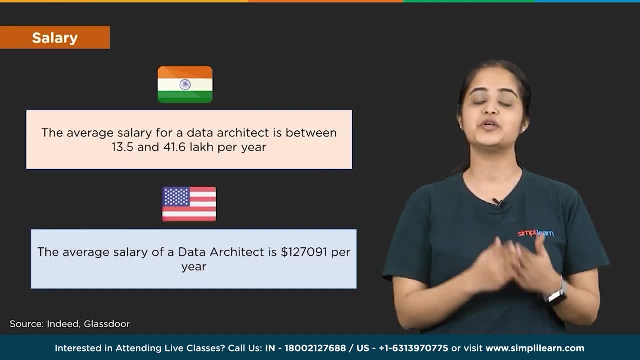 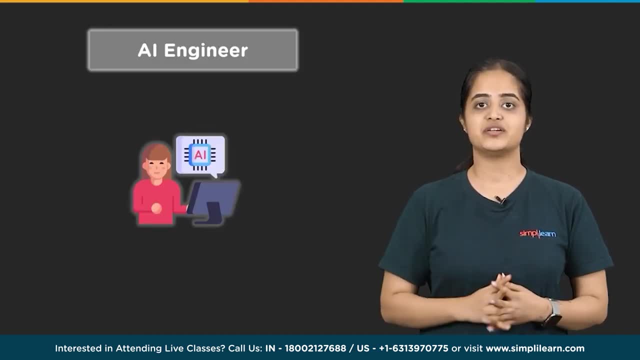 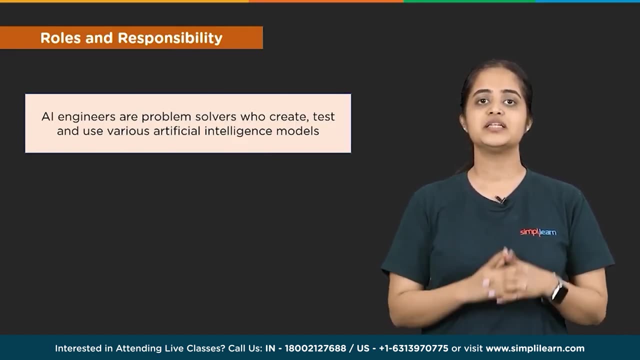 $200000 per year in the US and Rs 21 lakhs per annum in India, And topping our list of job opportunities in AI is AI engineers. AI engineers are problem solvers who create, test and use various artificial intelligence models They manage. 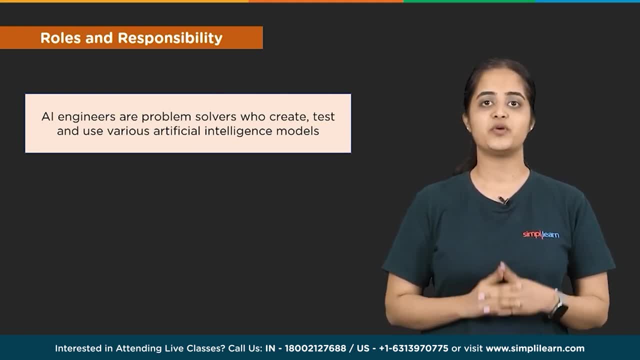 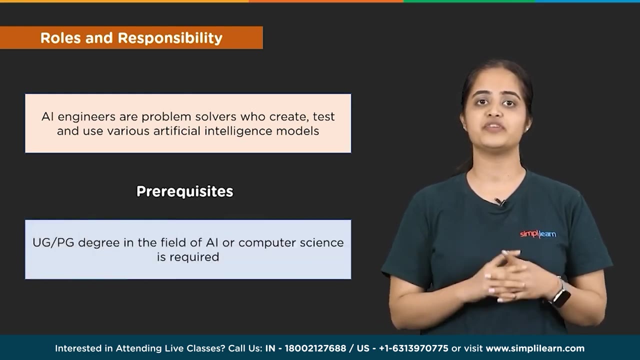 the AI infrastructure well. To create practical AI models, they use neural network knowledge and machine learning methods. These models enable one to gain business insights, which aids the organization in making wise business decisions. UG or PG degree in the field of AI or computer science is required. 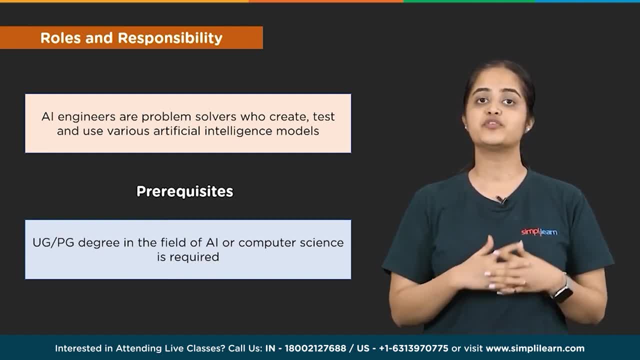 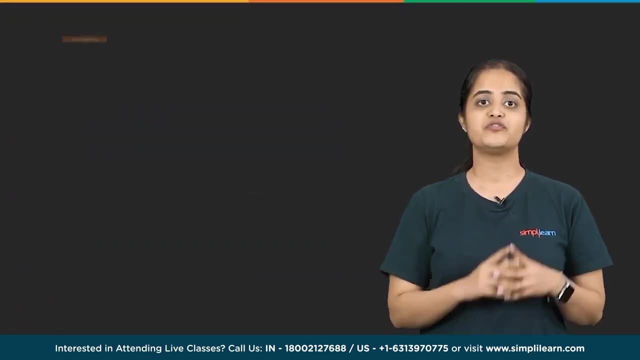 in addition to that, you can hold certifications from any reputed organization with which will add up to your resume. Please check out and enroll to the AI program by Simply Learn in collaboration with Purdue University. The link is provided in the description below. Job openings for an. 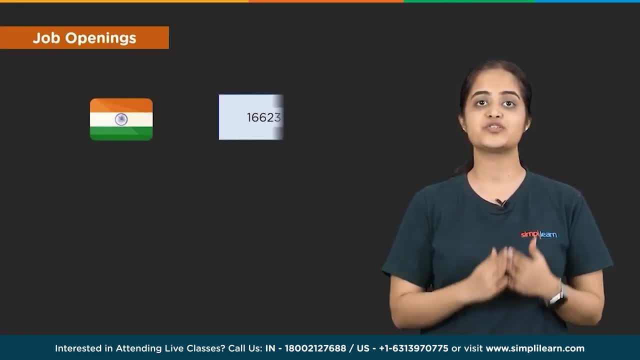 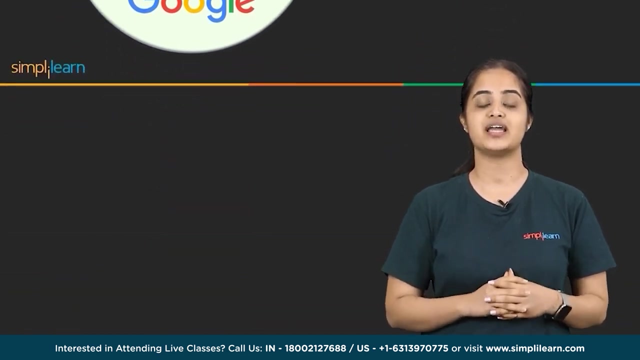 AI engineer are quite high, with 35000 plus job vacancies in the US and 4000 plus jobs in India, and tech giants like Accenture, TCS, IBM, Google, JP Morgan, Deloitte, Bank of America recruiting them with salary going as high as. 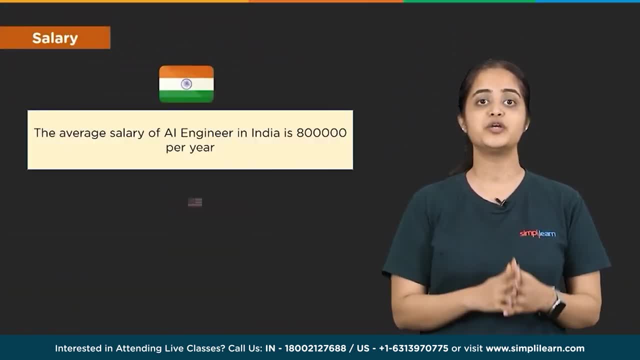 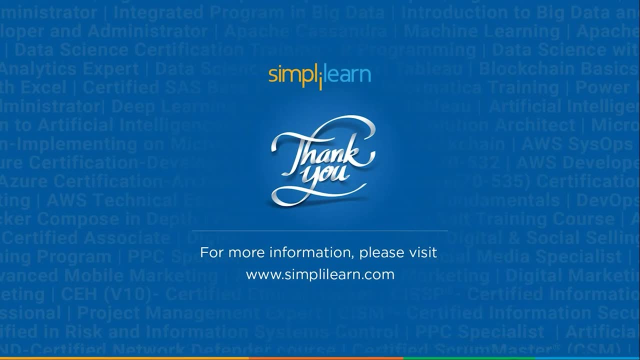 $200,000 per year in the US and rupees 10 lakhs per annum in India. And this was all for this AI basics video. Hope you guys found it informative and helpful. If you like this session, then like, share and subscribe. 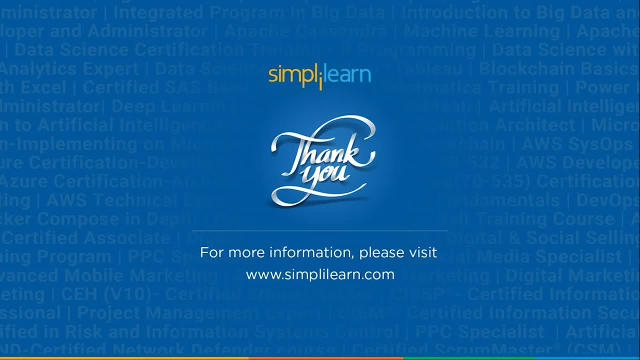 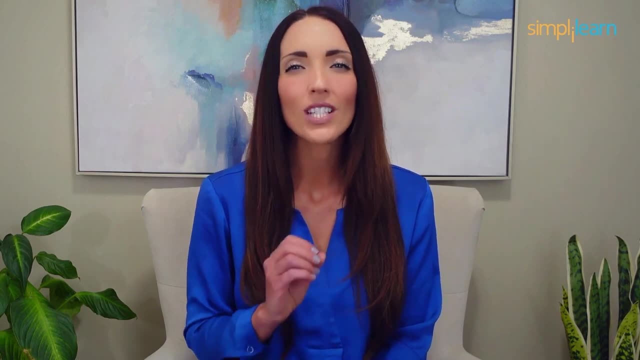 If you have any questions, then you can drop them in the comment section below. Thank you for watching and stay tuned for more from Simply Learn. Staying ahead in your career requires continuous learning and upskilling, Whether you are a student aiming to learn today's top skills. 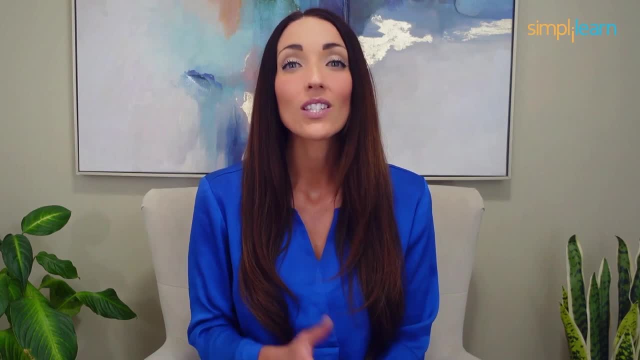 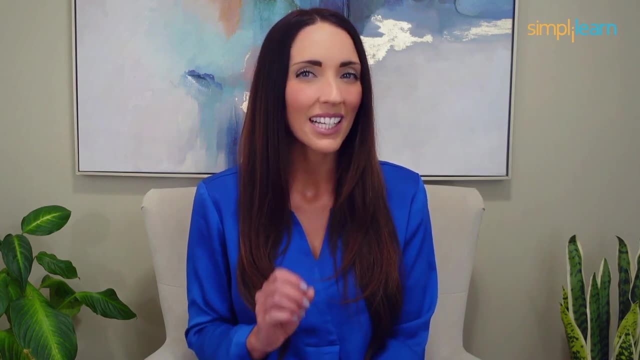 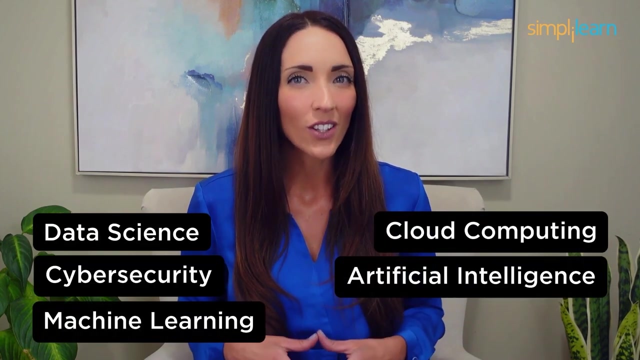 or a working professional looking to advance your career? we've got you covered. Explore our impressive catalog of certification programs in cutting edge domains, including data science, cloud computing, cyber security, AI, machine learning or digital marketing, Designed in collaboration with leading universities and top corporations.